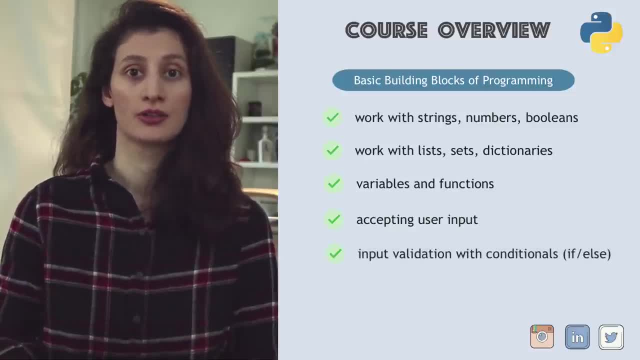 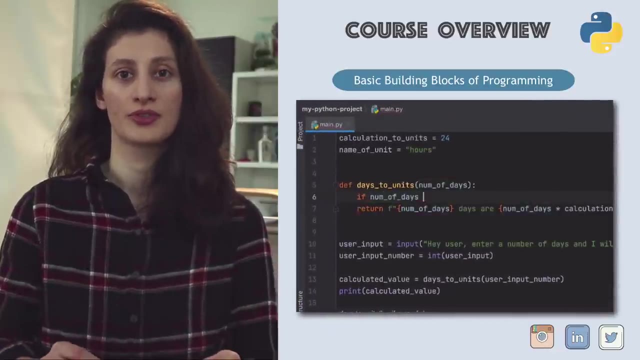 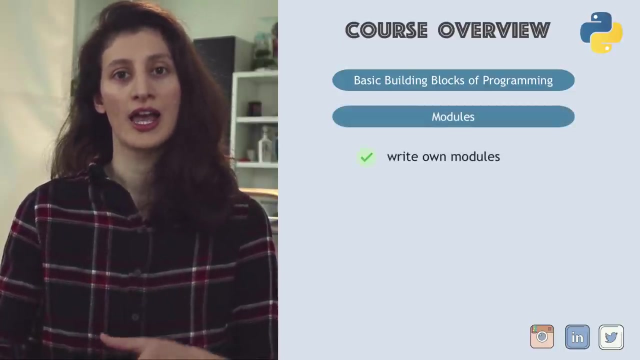 validate the user input using conditionals, Error handling with try, accept and also learn loops with while and for loops, and again why we actually need them. You will learn all these concepts with hands on examples. As a next step, you will learn how to modularize your program by writing your own modules and then see how to use some built in Python modules. With all this knowledge, we can. 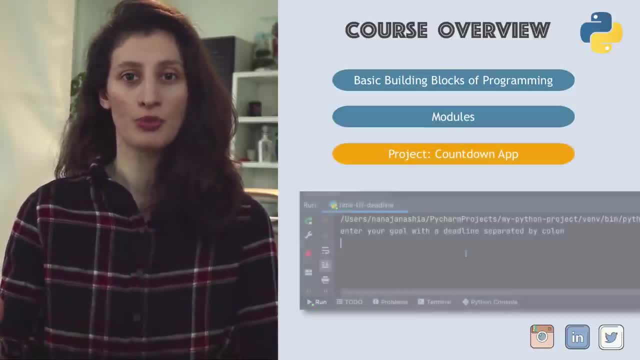 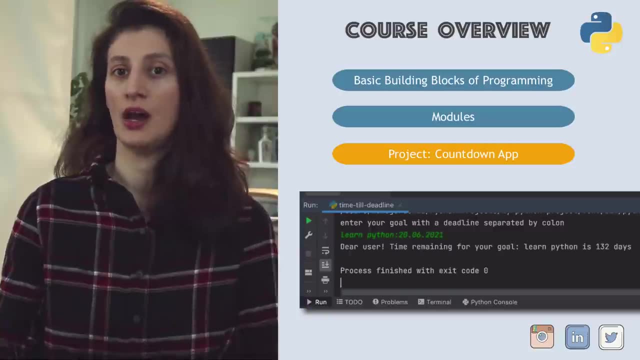 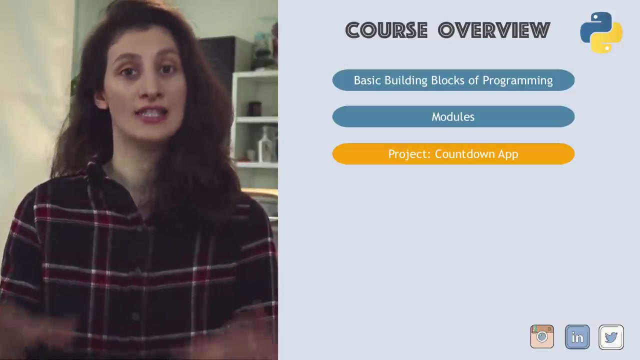 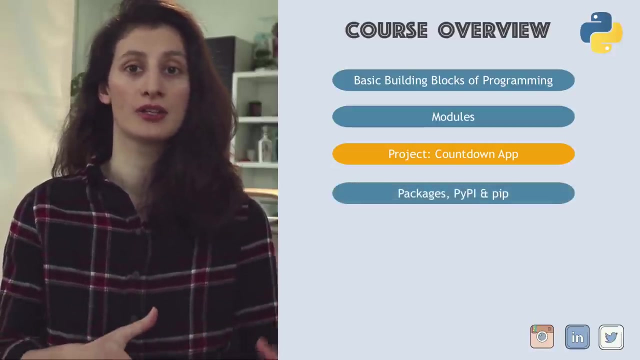 then build our next demo project to write a small program that accepts a goal and a deadline as user input and then outputs the number of days remaining till the goal deadline. Within this exercise you will learn how to use the date time module to work with dates. After that you will learn about packages and comparison of package versus module, and we will use an external Python module. 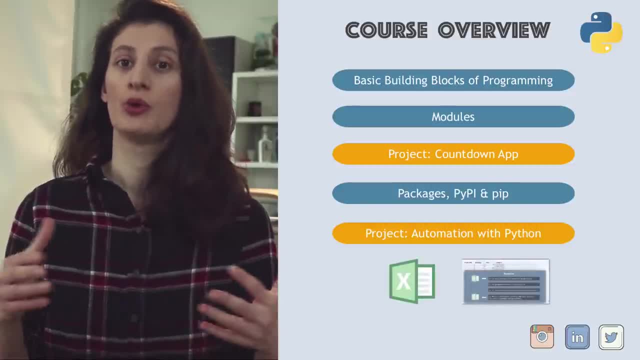 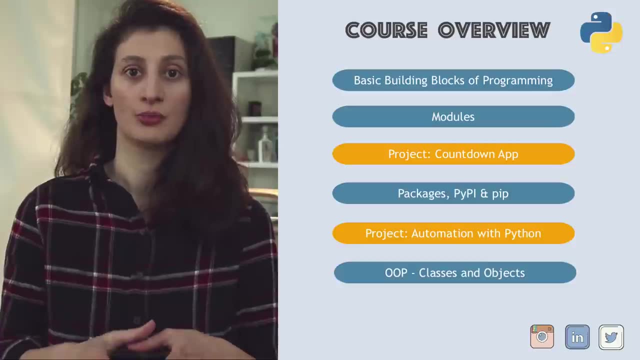 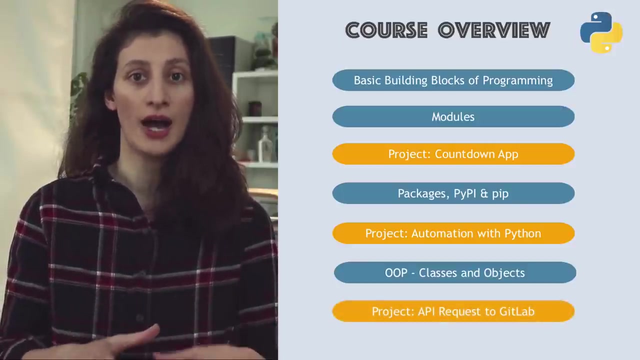 package in our next demo project, in which we will automate some tasks for working with a spreadsheet file. Finally, we dive into object oriented programming. You will learn what classes and objects are in programming, and Python specifically, and why this concept is so useful. in the final demo project, You will learn another common use case with Python, which is communicating with other applications over the internet By 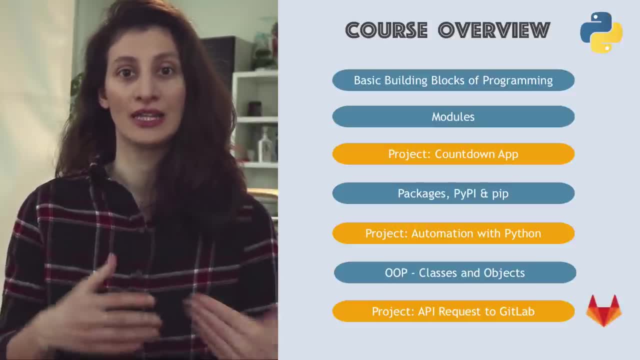 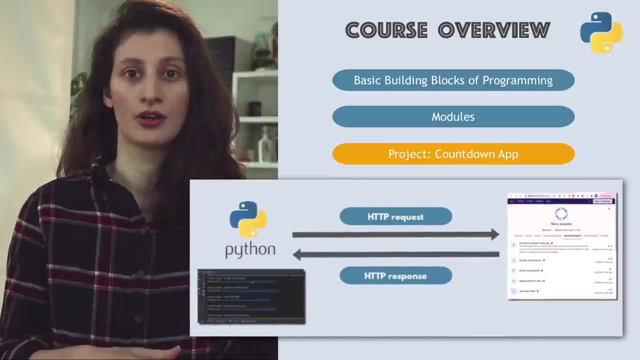 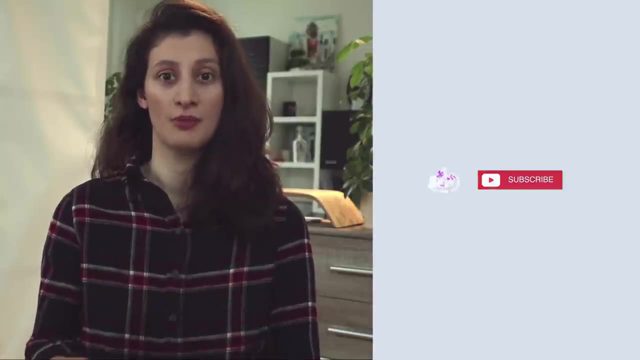 making a request to fetch some data from GitLab API. In this specific case, we will list the GitLab projects of a specific user. So that's what we're going to learn. If you like this course, don't forget to give this video a thumbs up. I'm really excited to teach you. 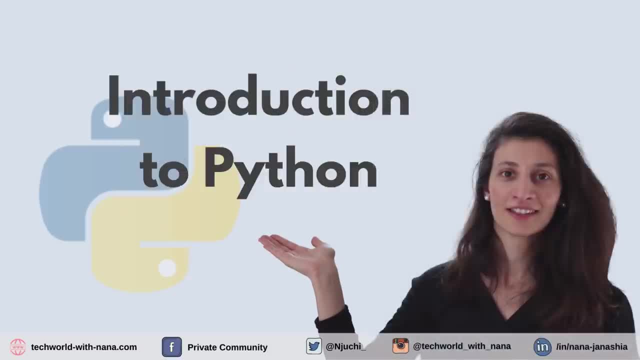 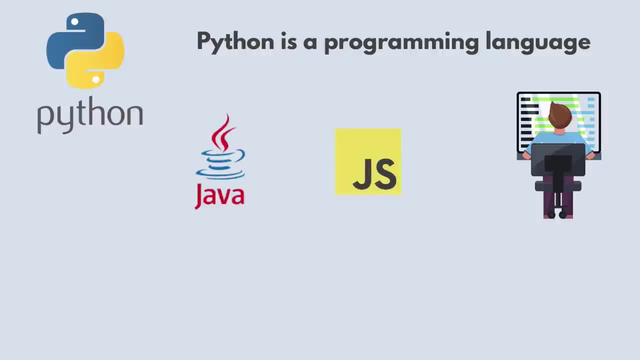 all of this. So let's get started. First of all, Python is a programming language just like Java or JavaScript. Python, compared to other languages, has two very big advantages. First of all, it's easy to learn. It has a simple syntax and it's very easy to set up. 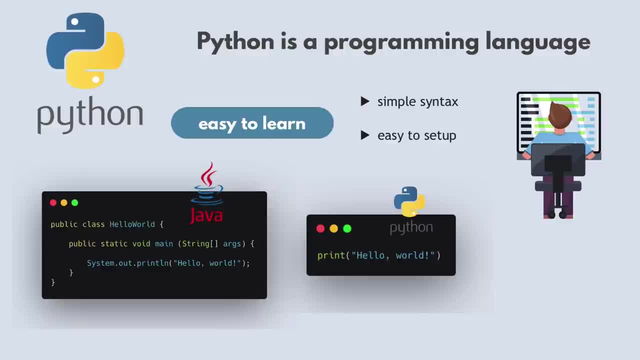 and get started with, for example, compared to Java, where you need some initial configuration before you can even start your application, But it's equally or even more powerful than Java. Now, what makes a language powerful? or how can I say that Python is more powerful? 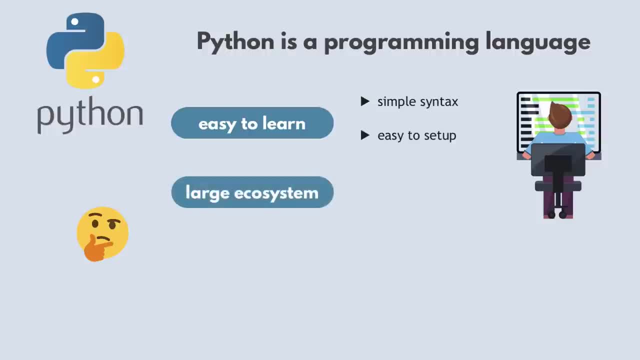 Well, that comes from the ecosystem, which means libraries and modules that Python developers themselves develop, but also external developers create and maintain. So the more people adopt the language, the more powerful it gets, because new libraries and so new functionalities get added to it. And the second advantage is that it's flexible. Now, what does a flexible mean? 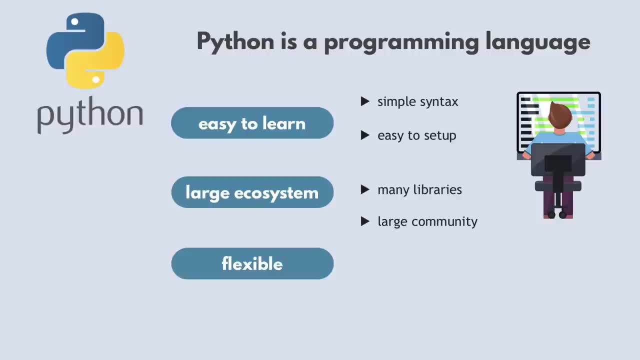 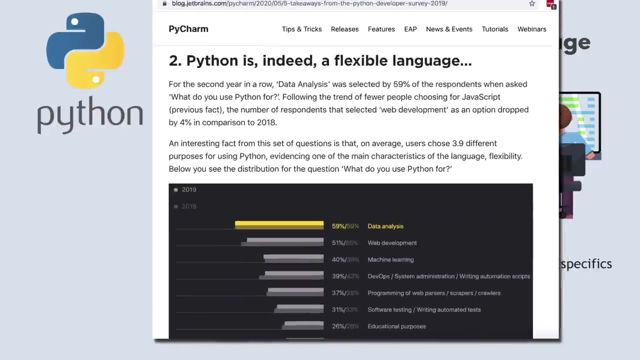 in this case. What makes a language flexible? It is easy to mold to your wishes, so you are not limited or restricted by the language specifics like syntax or data types or some other constraints or even library functionalities. You can extend Python widely And, as one of the results of this flexibility, Python also 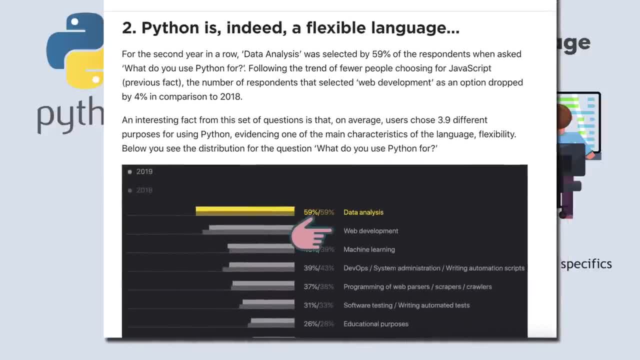 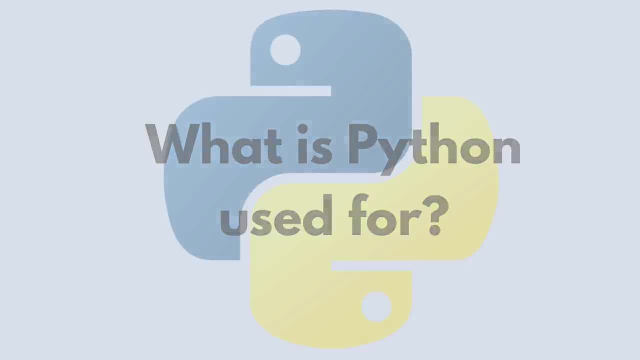 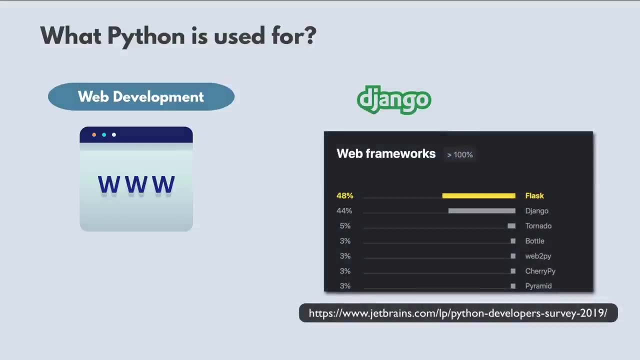 became a multipurpose language, meaning it is used for many different categories. So let's see what these categories are. First, you can use it to write web applications. the popular libraries for that are Django or, more lightweight Flask. Python became extremely popular because of the rise of data science. 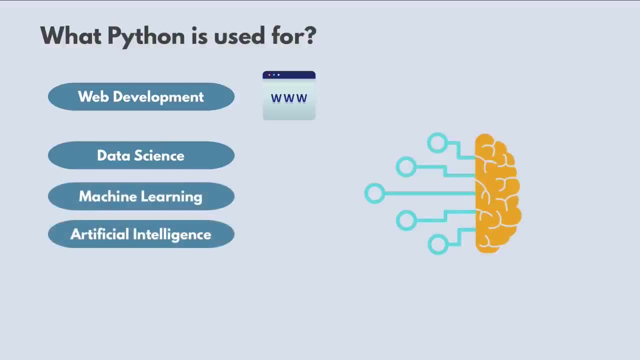 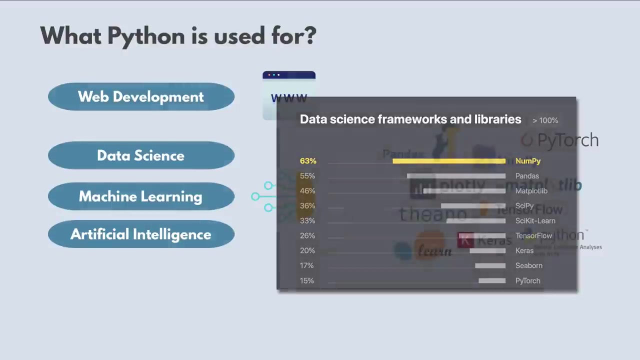 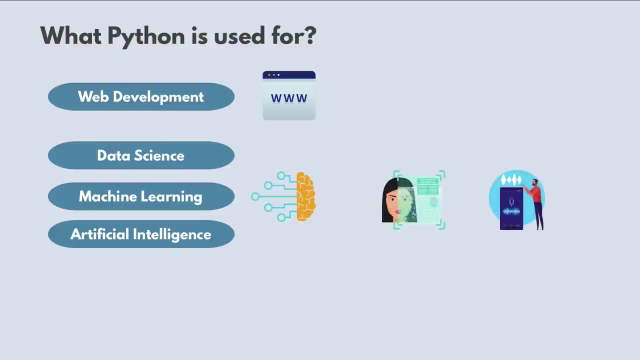 machine learning and artificial intelligence industries, And more and more libraries were created and are still being added for Python. for all these categories they are very popular and highly used libraries for data analysis and data visualization, libraries for artificial intelligence projects, for things like face recognition, voice recognition and a bunch of very powerful. 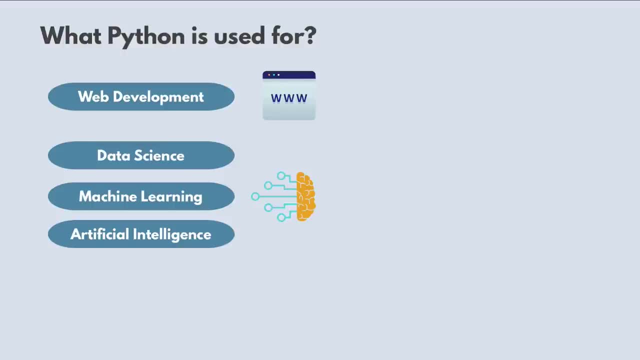 and widely used machine learning libraries. Python is also often used for data collection, like scraping the web, creating web crawlers. There are basically programs that collect data from internet which you can save and then process later. Again many different powerful libraries to do all of that And finally, automation with Python. Python has many great 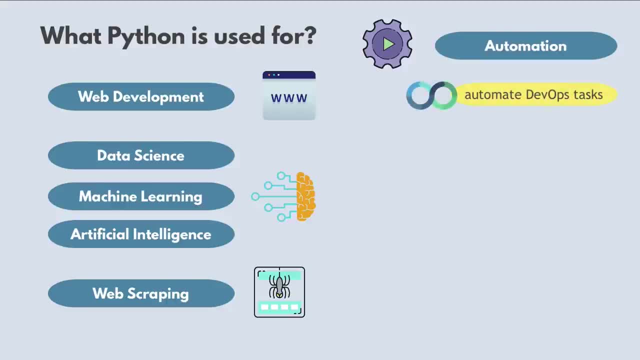 libraries to automate DevOps tasks, for example, starting from CICD pipelines to cloud platforms and monitoring your infrastructure, etc. You can also write Python scripts to do automated backups, cleanups on the servers, etc. In addition to DevOps tasks, you can also automate just general tasks with Python. 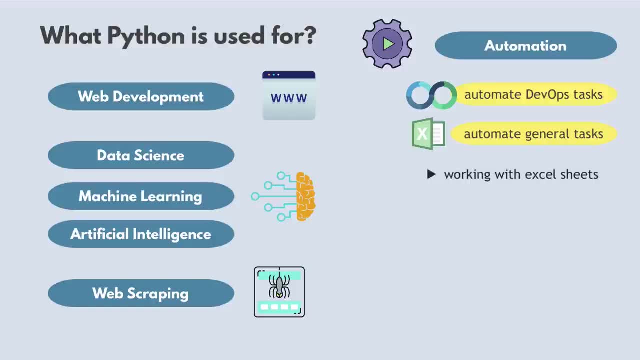 like when working with Excel sheets, which is a common use case in many big companies, or automating some task on your own laptop. And there are also libraries for mobile development, gaming, desktop applications, But these are less likely use cases for Python because 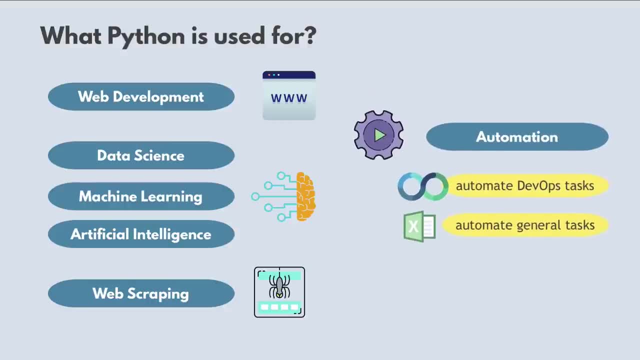 there are better alternatives for that. So you see that the use cases for Python are pretty valuable, but they are not really the best ones. You can actually throw them on the table. The and it actually spans several industries and it's mostly concentrated around data analytics. 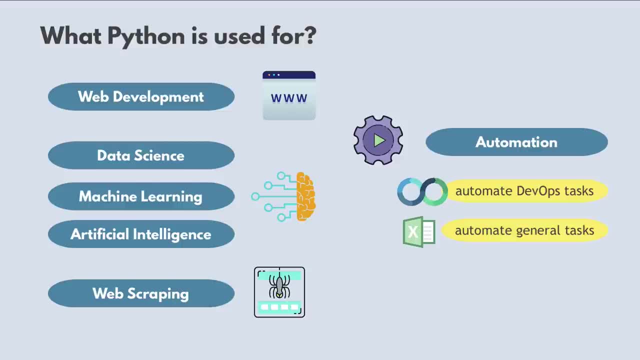 machine learning and automation areas, and note that this isn't the case for many other programming languages. usually one programming language is good for just few things and you should use something else for other use cases. so now you see how useful python knowledge could be and how it. 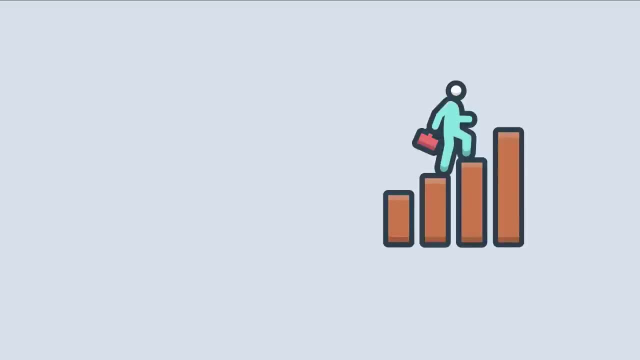 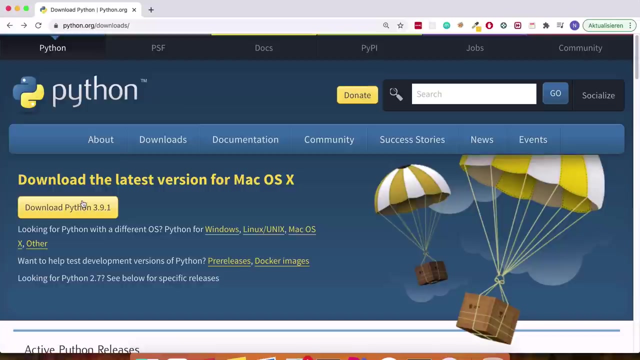 can help you in your job, but also make you more valuable at your work and for your entire team. i hope you are already excited to learn python, so let's get started. as a first step, we're going to configure our local python development environment, so the first thing we need is install python locally on our laptop. so first we install or download. 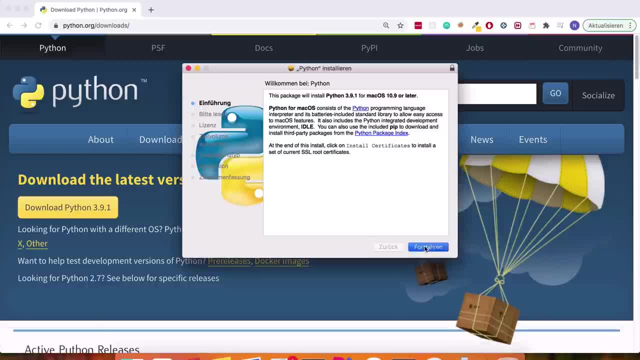 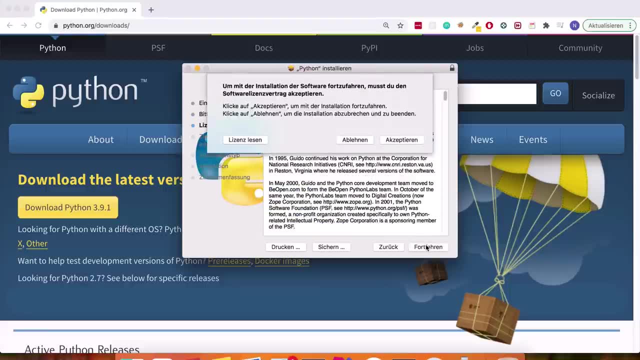 python on our laptop and then we're going to install python locally on our laptop. so first we install or download python locally on our laptop and then we're going to install python package for your specific operating system and then basically just click through the installer wizard to install python locally on your laptop. and note that if you're doing this on windows, 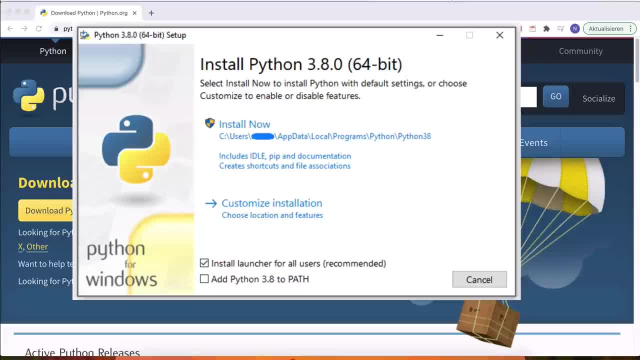 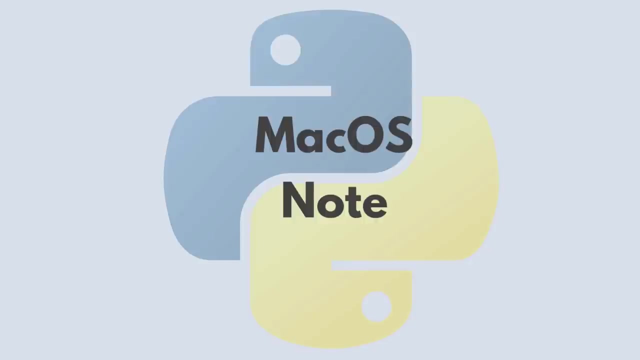 very important step in the installation process would be to check the add python to path option- basically that you see here, because by default it is unchecked and you have to check mark it so that after the installation you'll be able to execute python commands in your terminal. now an interesting note here: if you're using 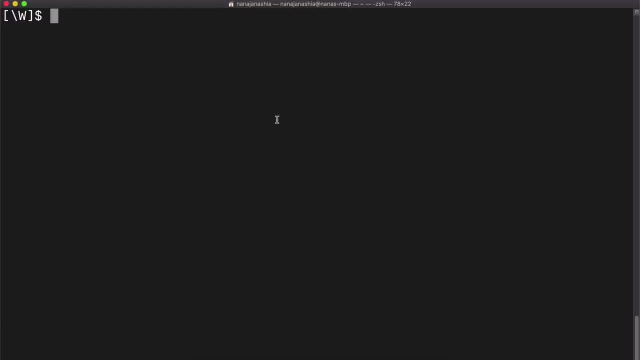 mac os, like i do, is that by default on mac os there is python already installed. so if i do python version and execute, i see that python version 2.7, 10 is installed and that is a python version that mac os, the operating system, itself, is using. however, for our tutorial and 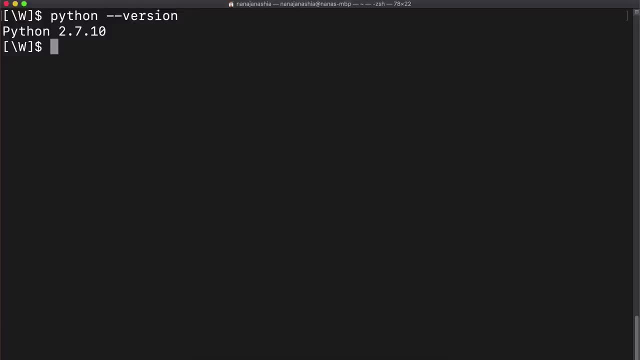 generally when working with python, we want to be using the newest version, which is python 3.. so we're going to leave that default python installation alone. we're not going to use that or touch that, and instead we're going to be using the python version 3 that we just installed locally. 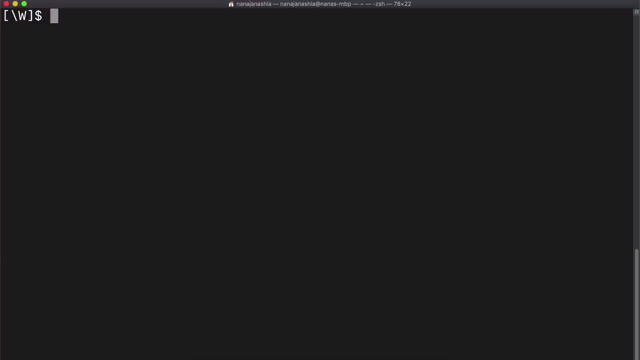 so now, if i clean this up and do that, we're going to see that python version 2.7, 10 is installed and we want to execute python version 3 commands. we're going to do python 3 instead and dash dash version, and that will give us the version. so that's how we can differentiate between. 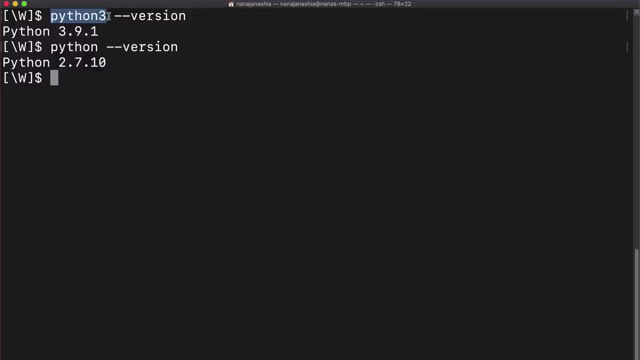 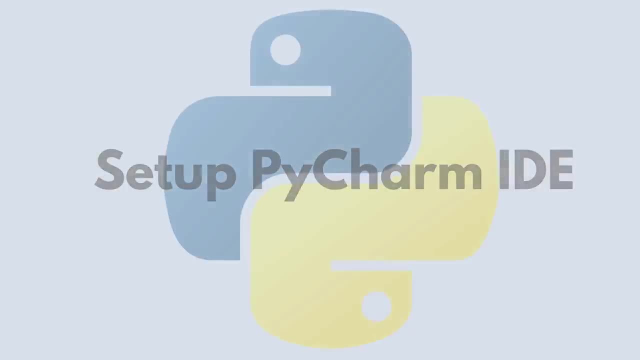 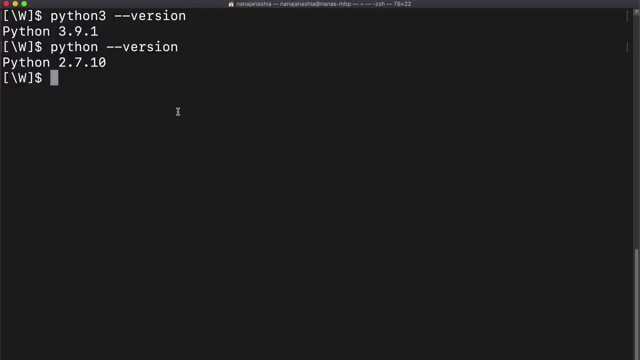 the already installed python and the newest version that we just installed, so just be aware of that difference. now that we have python available locally, it's time to download a code editor for python, because we're going to be writing files with python code, so we need a proper editor. 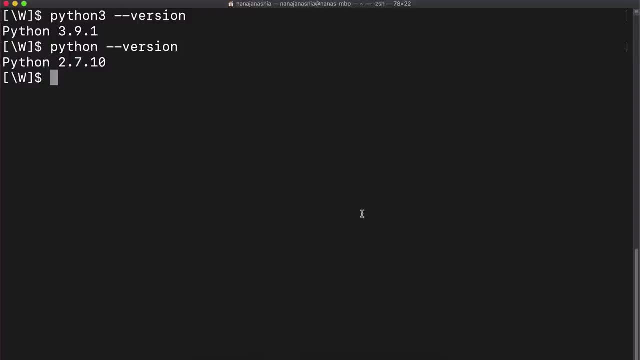 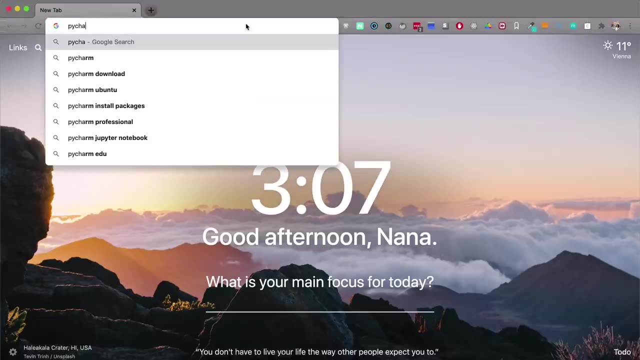 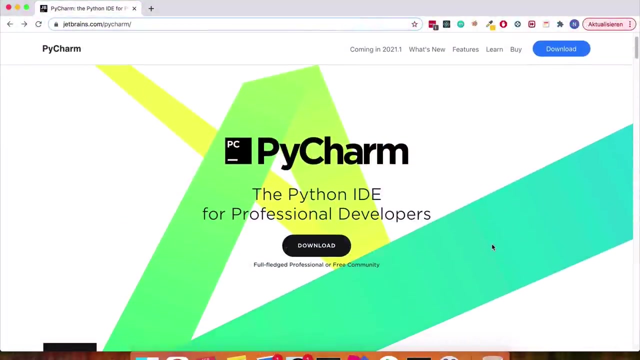 for writing python code, and actually the best python code editor available out there currently is pycharm, which is from jetbrains, so that's what we're going to be using throughout our tutorial. so let's go to pycharm. it is an intelligent code editor which makes it much easier to write code. 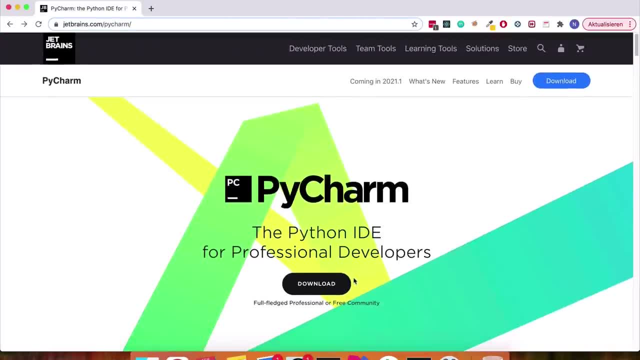 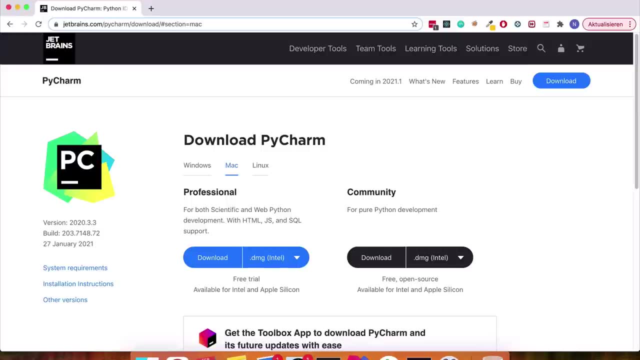 so it makes you actually very productive when writing code, and we will see why throughout the course. as you can see, there are two versions. we have the community version and professional. one community version is free and already has a lot of powerful features, but the professional edition gives you additional very useful features, especially if you're creating web applications. 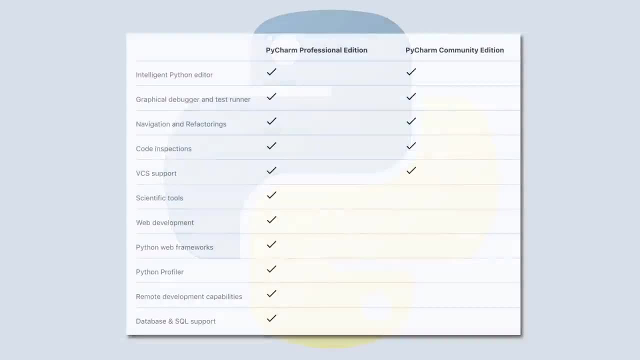 or scientific projects in python, so with professional version. additionally, you will get scientific tools that you can use and you'll be able to access the kfp version as well if you're use in scientific projects with python. but also you get support for python web frameworks and 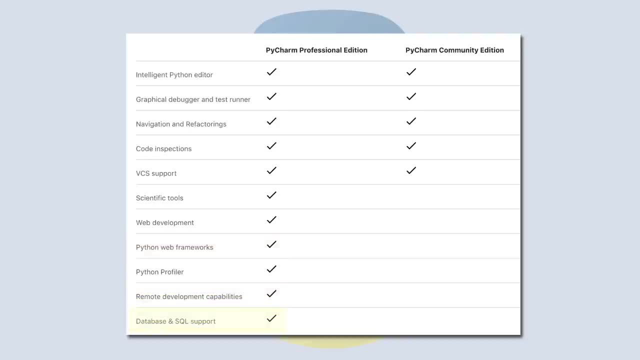 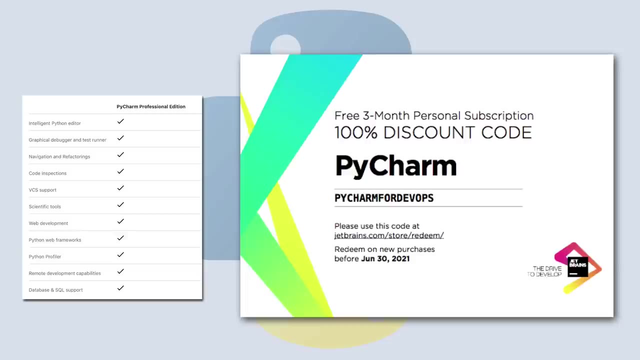 database integration, which can be, of course, very helpful if you're developing web applications. if you want to get the professional edition, jetbrains actually provided me with a code for my channel to try it out for three months for free. just use my code when you install it. 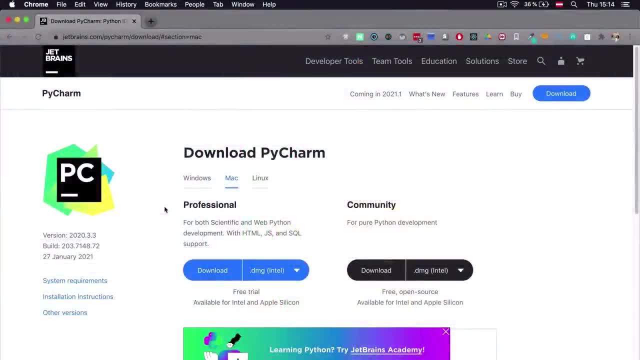 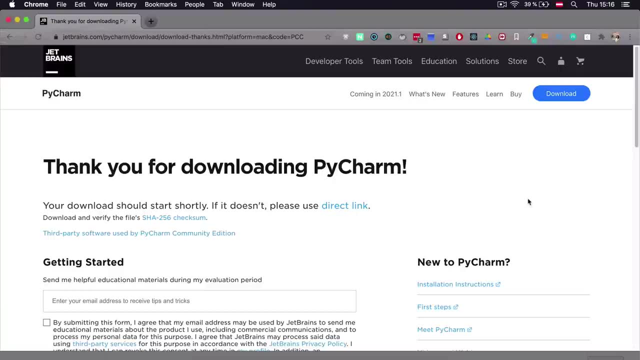 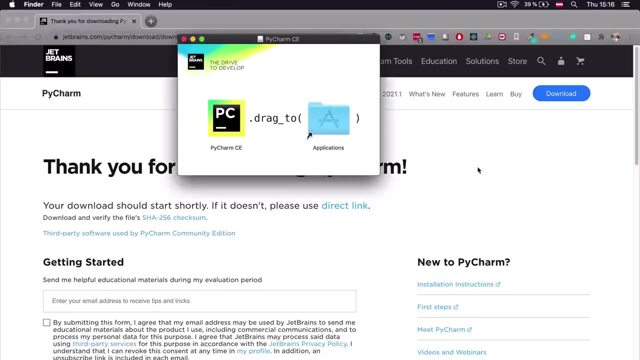 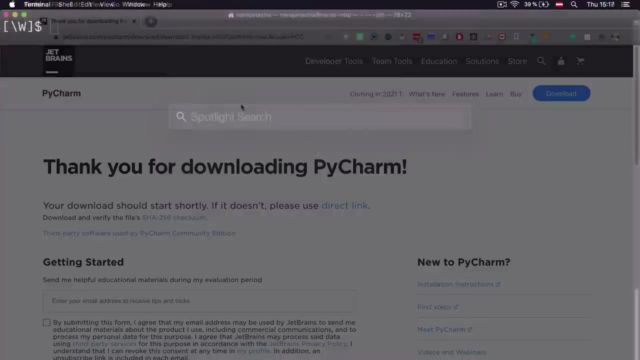 but for this demo community version is absolutely fine. so i will go with this one and install it and just click download, and once the pycharm installer is fully downloaded we can just click on it, move it to the application and now i can actually use it locally. so i'm just gonna. 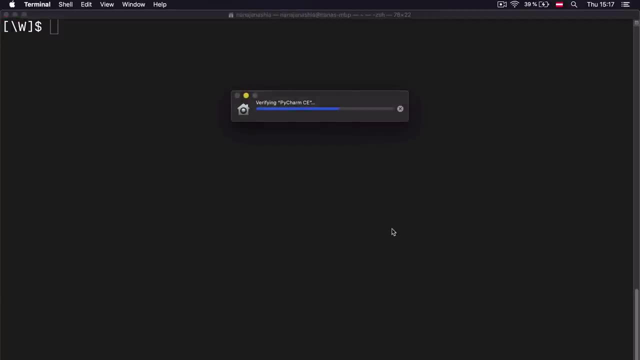 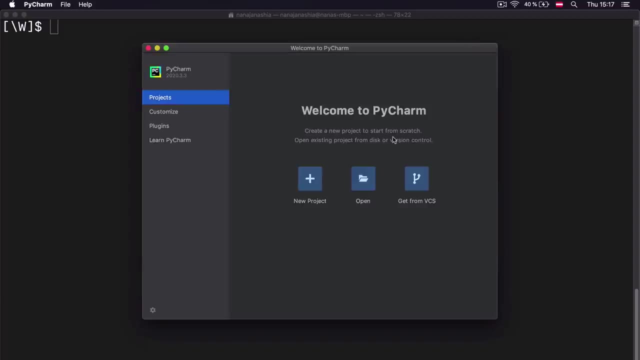 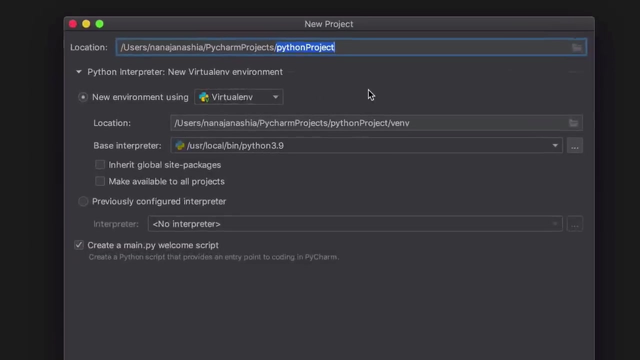 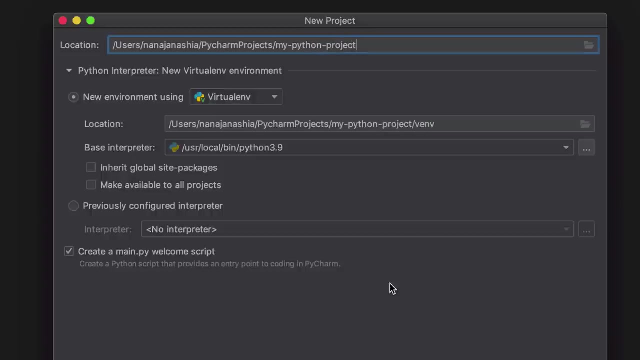 open the application and we're gonna take a quick tour around pycharm. it's actually pretty simple to set it up and there you go. we have our pycharm and we can now create a new project and let's call it my python project and that's it basically. we don't need to. 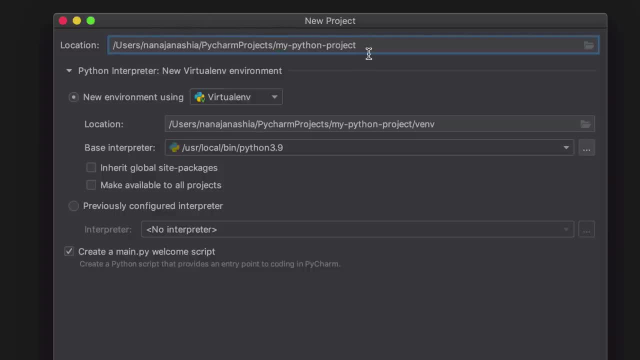 change anything else. and here you see the location basically of where this application folder will be created. you see, pycharm projects folder got created in my users directory. so this is basically very convenient because all my pycharm projects or my python projects that i create using pycharm will be created in one location. and here you also see that python. 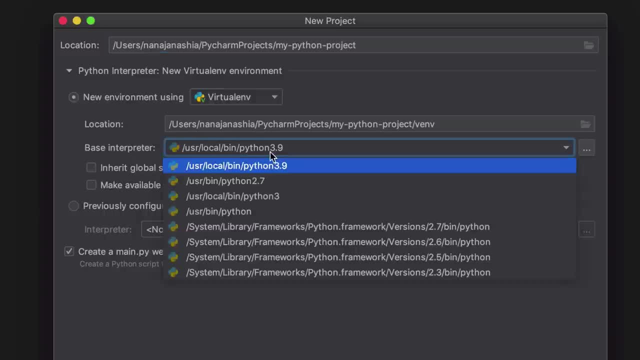 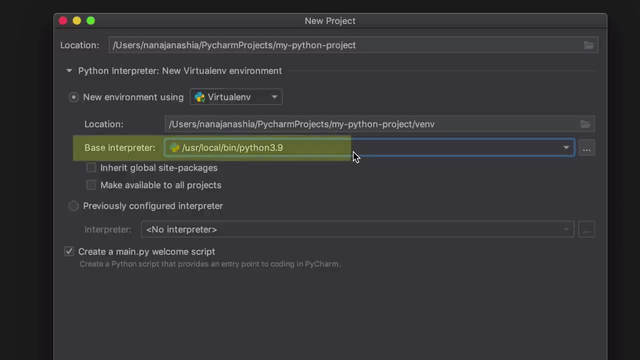 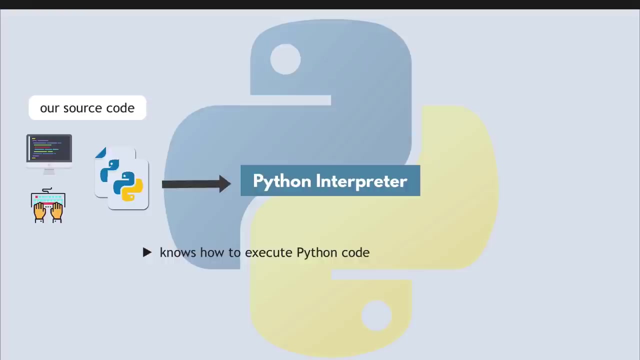 version 3 that we installed is automatically being used for this project, which is exactly what we want, and you see, it says base interpreter, and python interpreter is basically a program that knows how to execute python code. it will know how to interpret or translate our python code into instructions that computer can understand. 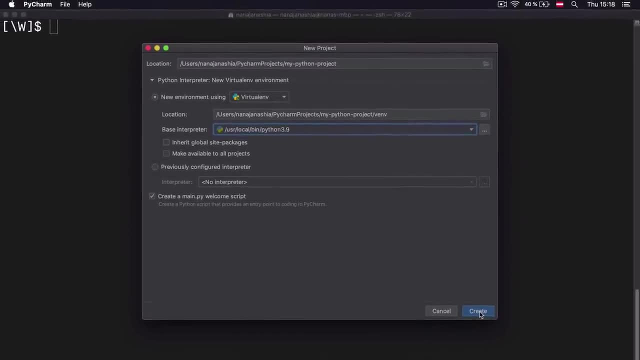 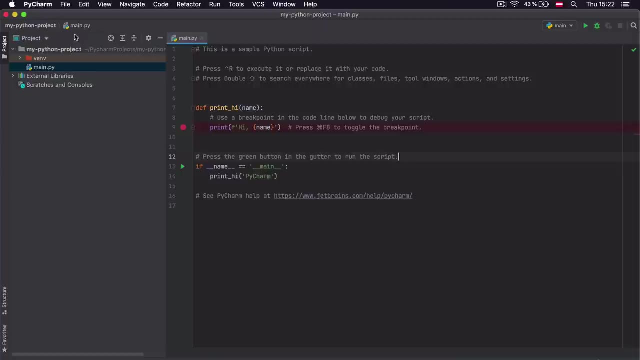 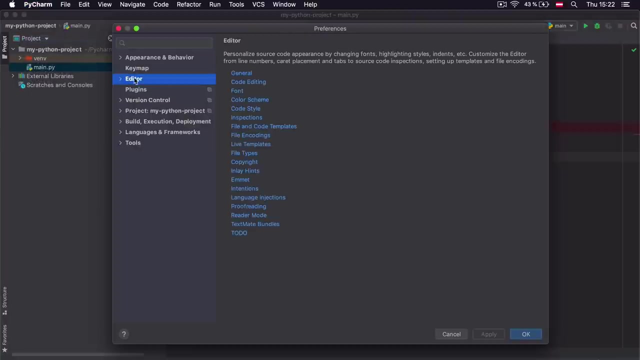 so with this configuration, we don't have to change anything. we're going to create our project. so first of all, i'm going to make all this a little bit bigger so that you can see the menu here on the side and the code a little bit better. so in preferences, editor font, we're going to set the size. 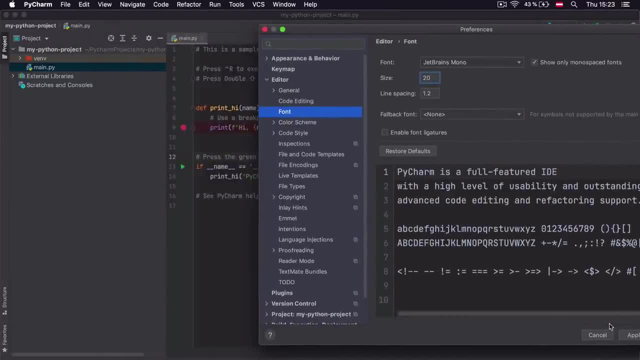 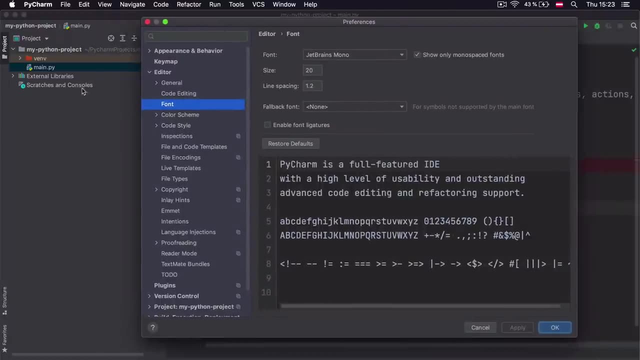 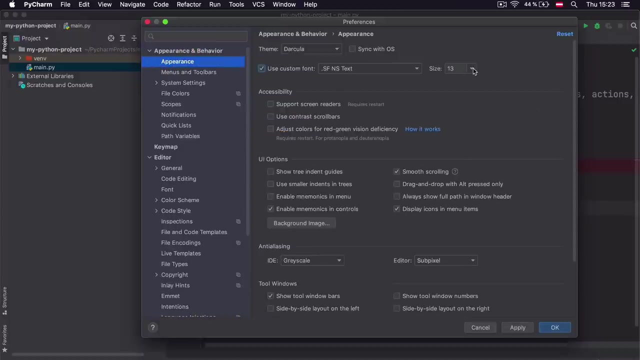 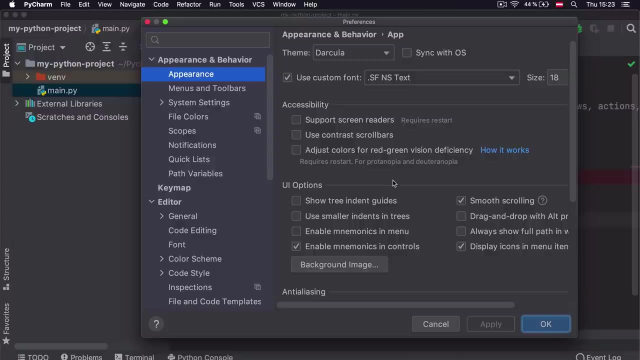 to 20. if i apply this right here, you see that this code editor font basically got bigger, and i also want to increase the size of this menu font here. so in appearance i'm going to set it to maybe 18, and there you go. so basically everything is bigger now, so you can follow along and see exactly what. 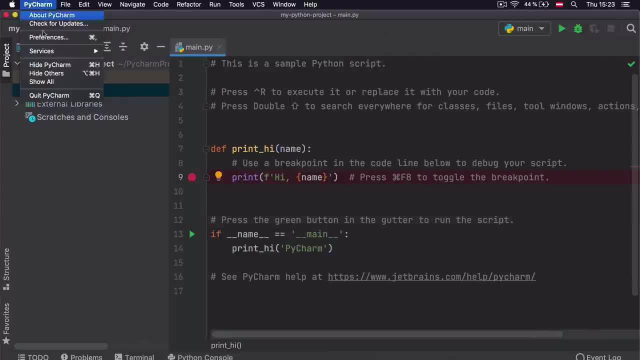 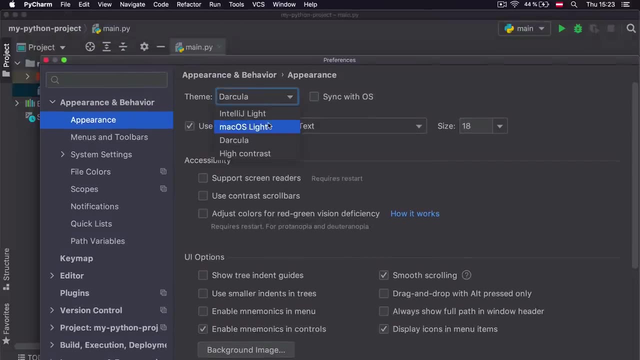 i'm typing, and also another note here is that this is basically where i'm going to use this font. if you want to configure your theme basically, So if you don't want it to be dark or maybe you want some other color scheme and you can select it here in appearance, you have four themes available. 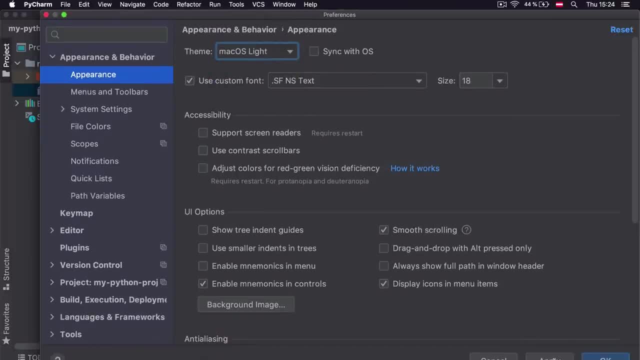 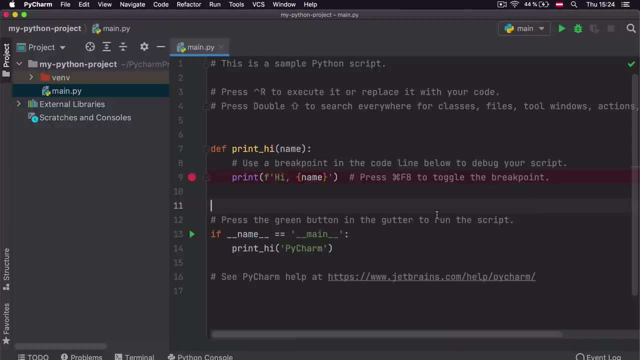 Let's actually try this one out and apply, And there you go, You have a different thing. I actually prefer this one. So let's look at that. So, as you see, we have a very simple project with one mainpy file. 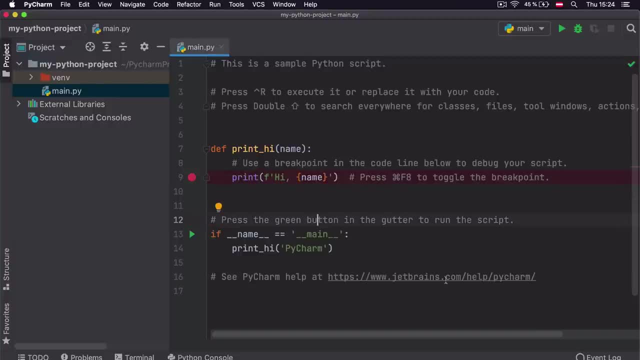 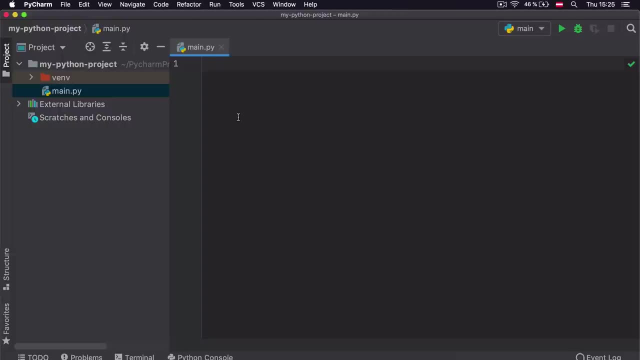 The extension is for Python files, which basically contains very simple code, And we're going to basically just remove all of these and start from a clean Python file state And in the next section we're going to dive right in and write our first simple Python application. 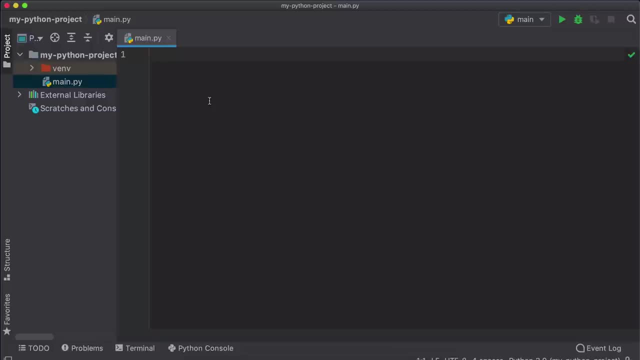 We're going to start with the simplest example In Python to basically learn Python syntax and get started as simply as possible. So first of all we're going to write a very simple application that just prints some output And in Python, when we want to print, basically display results of what we wrote. 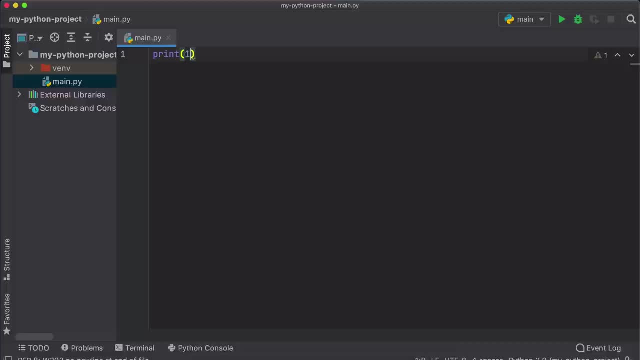 we use the syntax where we say print, and here we can pass in basically whatever we want to display. And now, if I want to see Whether this super simple application works, I can run it or execute it with this triangle here, and I have the output. 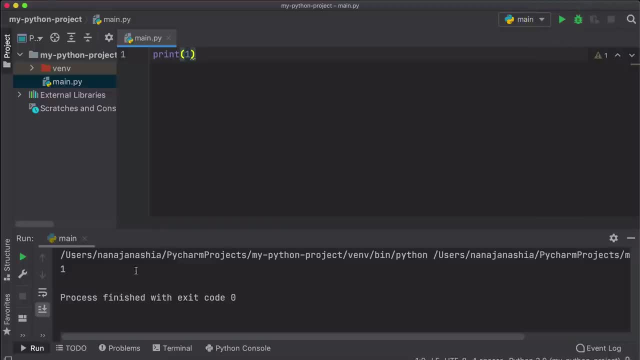 So basically the output is displayed or printed right here and I see the output is one. I can display some other values like 200 and run it, And there you go. Let's say, we want to display some text, Basically, whatever. 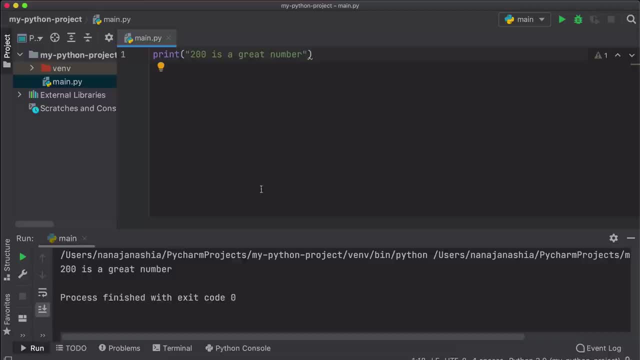 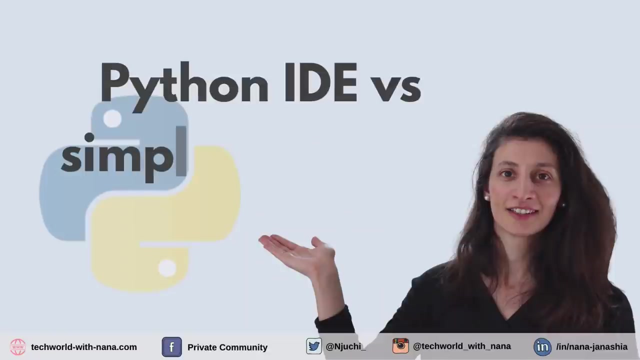 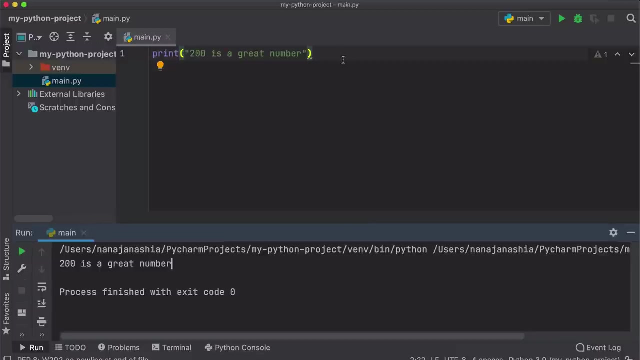 Some sentence and again triangle, And we have that output here, Right. So again very simple example of writing Python code that basically displays some information when we execute it. One thing that I want to note here is: you see that we write some code basically in this window, right here. 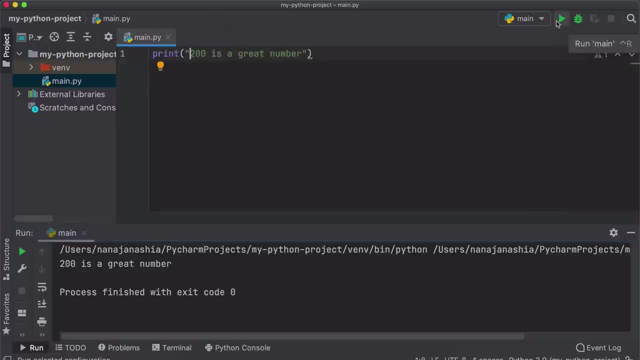 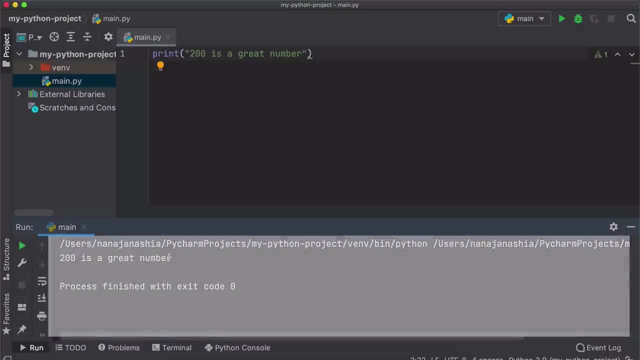 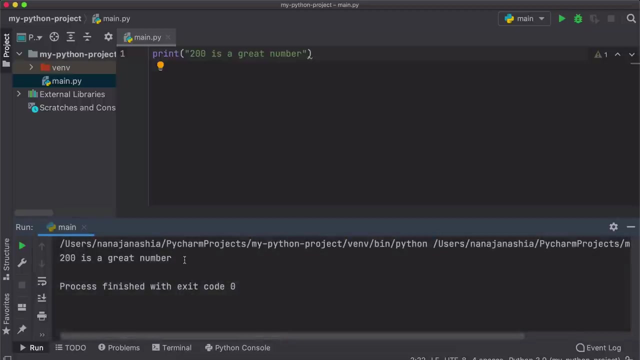 So in our main Dot pi file And when we run it or executed our code, we see some display in this window. So you may be wondering what is this window and why do we see some output right here? The answer to that is that whenever you were working with tools like pie charm, 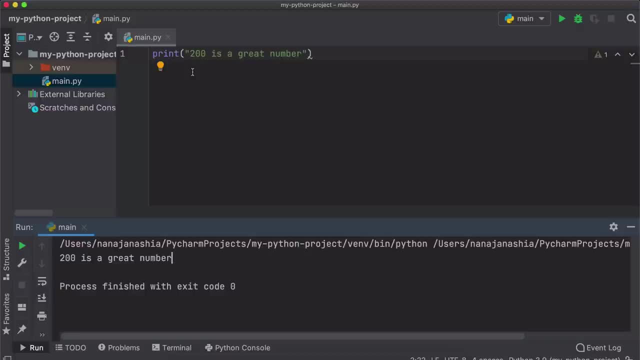 which basically have all the functionality that you need to write your code and then execute your code. you basically have everything in one place. So whatever we write, we can execute or run right away. now, without such tool, How would we write code and how would we execute that code? 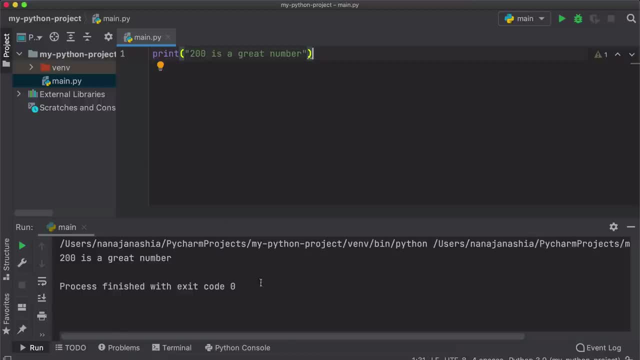 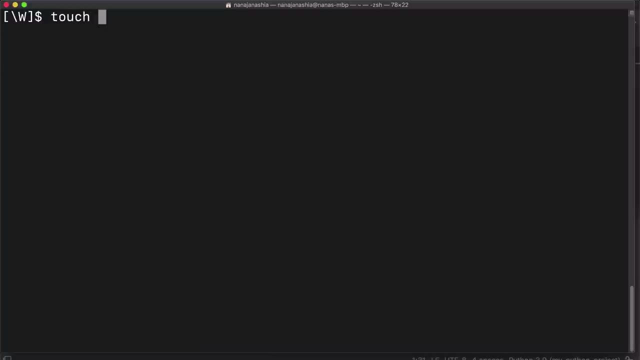 And this will help you understand what's going on here And to show that I'm going to go back to my terminal and I'm going to create a new file and I'm going to call it Test. I'm We're going to write the same. 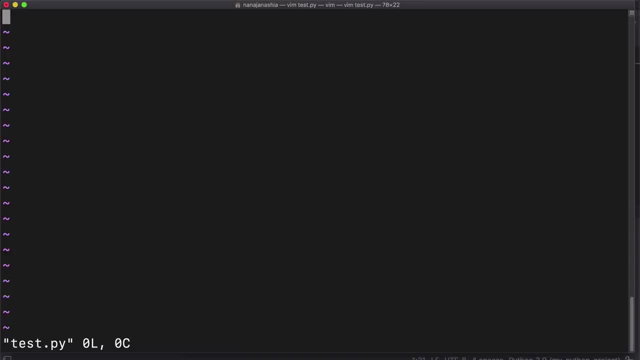 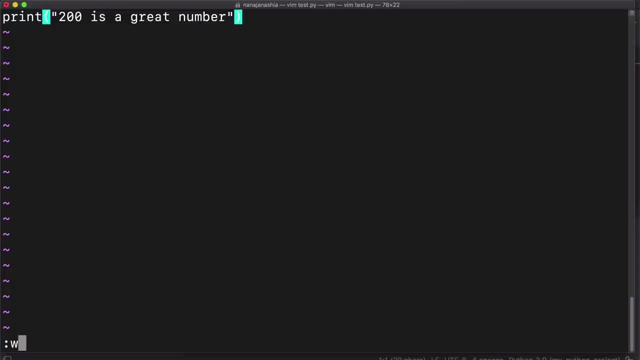 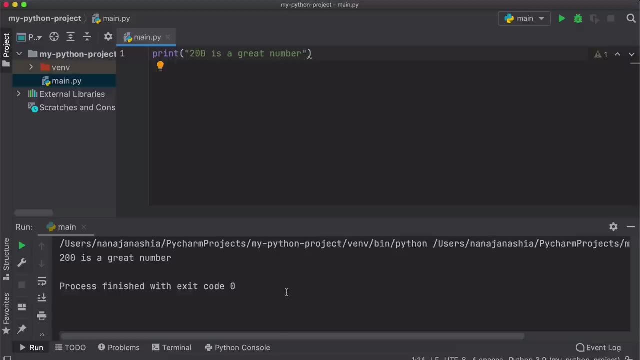 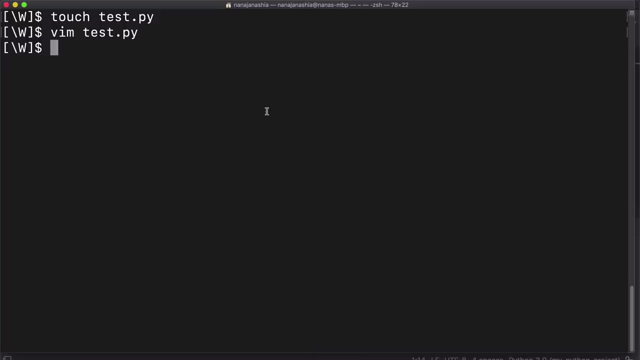 I'm just doing it directly in the command line and save it. So now we have the same identical file As here, but not inside our code editor, right? not inside these pie charm tool, and we have Python three available locally. So now, how do I actually 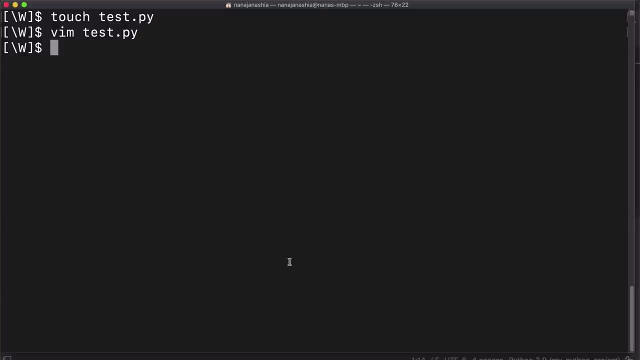 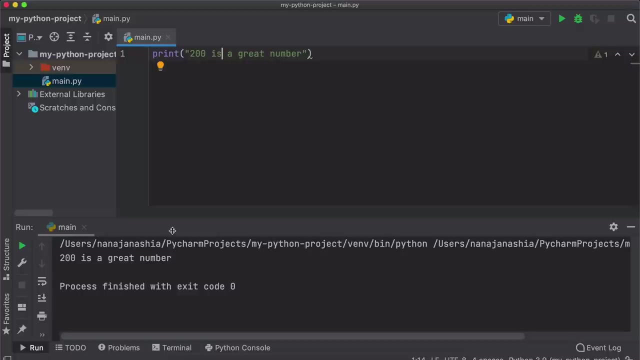 Execute a Python file outside these pie charm. I can do that using Python three: test dot, P, Y. If I do that, I get the same output in the command line. So basically what you see right here. this whole thing is integrated, So basically all in one place where you can write your code. 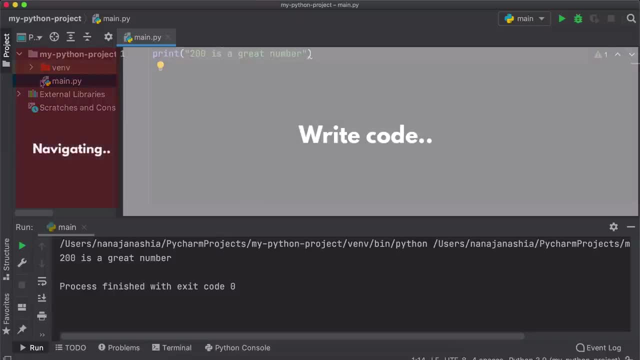 the editor. right here We can navigate your files in your project. So, basically, this is just a folder on your laptop and you can navigate the files here and you have the execution environment at the same time, So you don't have to go to terminal and execute Python three. 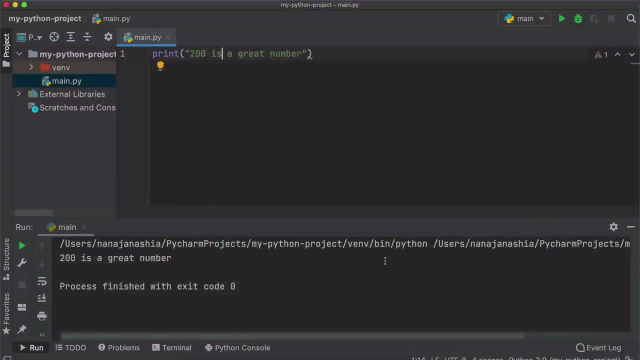 whatever you have everything in one place and tools that provide you with this type of environment for different programming languages. for Python, It happens to be pie charm. These are called ideas which stand for integrated development environment. integrated because you have everything in one place, So you don't need to use terminal. 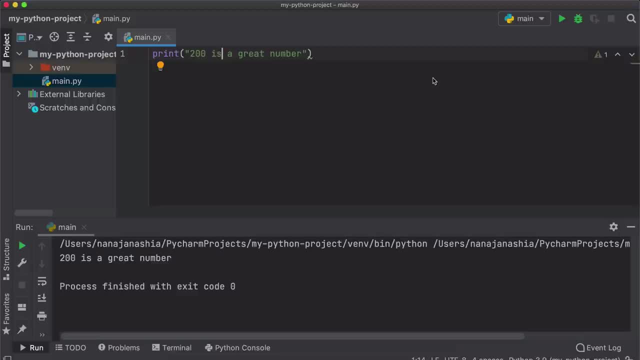 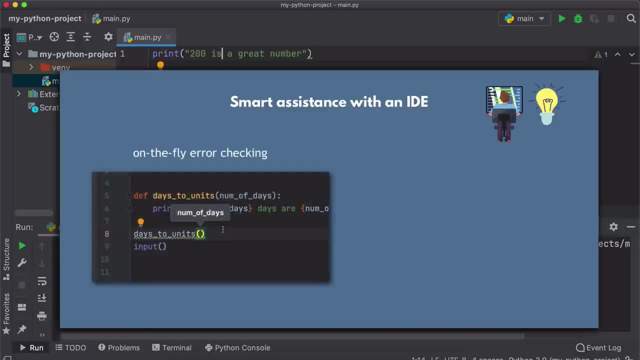 but in addition to this integration you get more cool features which helps you in writing Python code, for example, syntax highlighting, highlighting errors or code suggestions, autocomplete suggestions, and we will see those cool features actually Also throughout this course. So basically just makes your life as a developer easier. 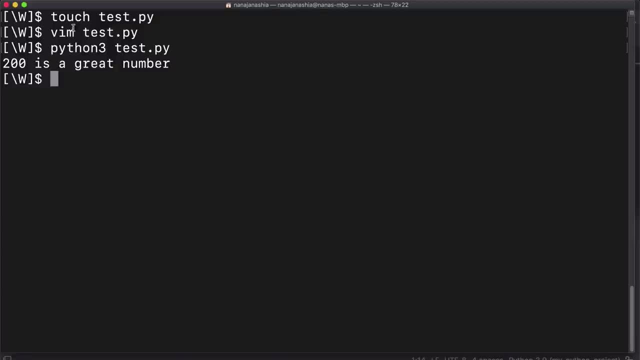 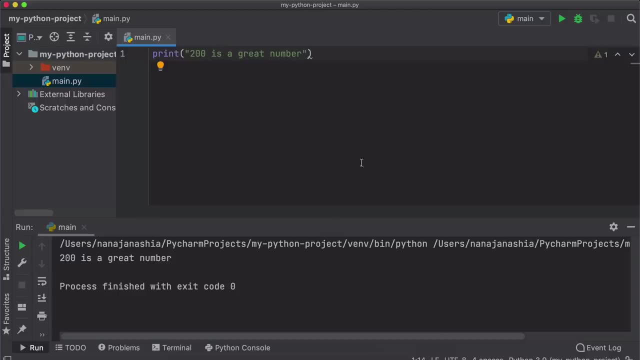 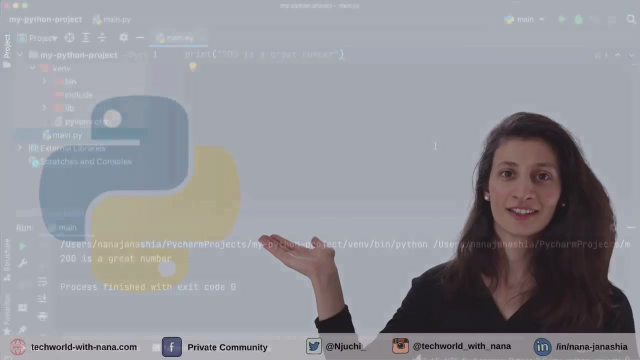 However, it's good to understand that connection between executing your files on the terminal when you don't have such a tool, versus executing and working on your application inside that tool- Awesome. So let's get back to our code editor file where we write our code. 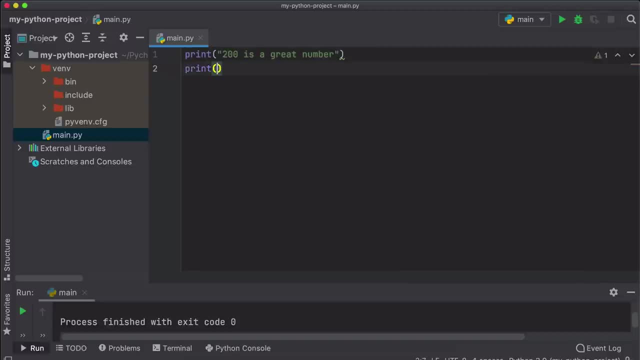 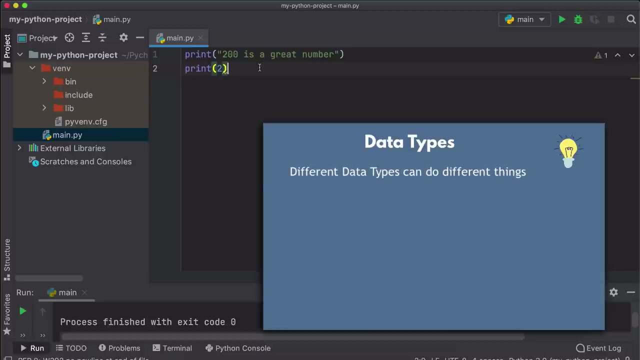 And till now we have done something really simple like print a text, basically, and print a number, right. And this leads to the first concept in programming languages, which are data types. So in Python, just like in any other programming language, 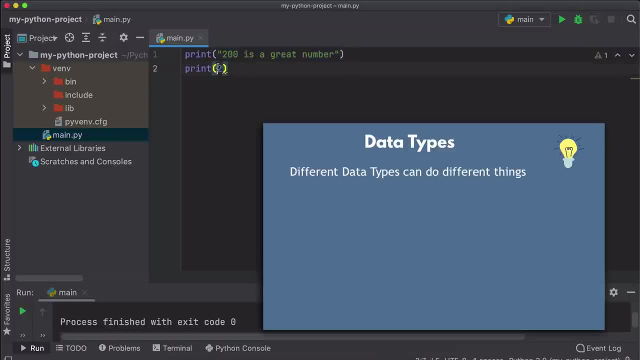 you have data types for text and numbers. The text data types are called strings, So everything within the double quotes is basically a string. But note that in Python you can also use single quotes for strings. So double quotes or single quotes, they both work the same. 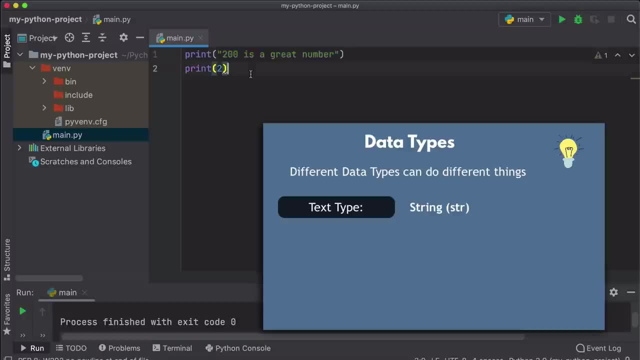 and there's actually no difference between them. And for numbers we actually have different data types. So for whole numbers like 220, but also zero and negative numbers as well, We have a data type called integer, and that's also how it's called in most programming languages. 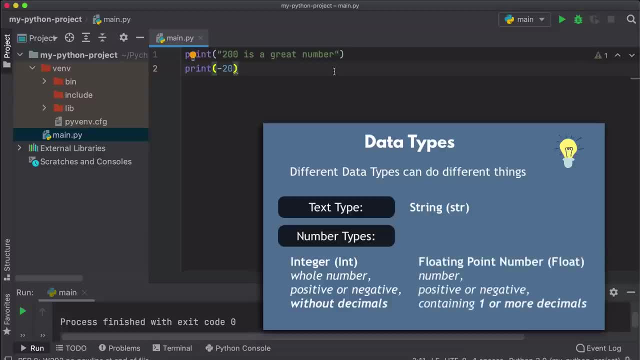 However, you also have numbers for currency, for example, how much a product costs, right? So if you have an online shop, you would have prices like this, for example. So these are basically numbers with precision. This could also be. 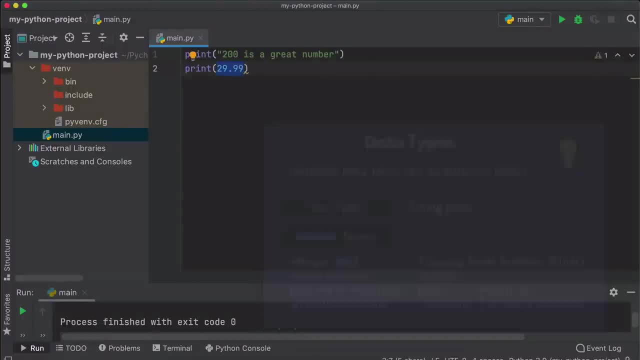 for example, when you're shipping something, you could have a weight of a package. that is also not a whole number but has a precision. So this type of numbers in Python and many other programming languages are represented as float data type. So again, 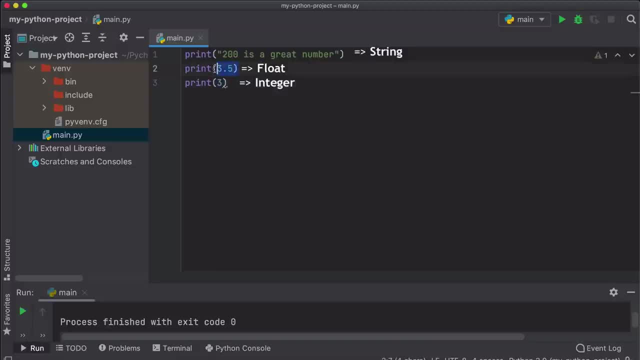 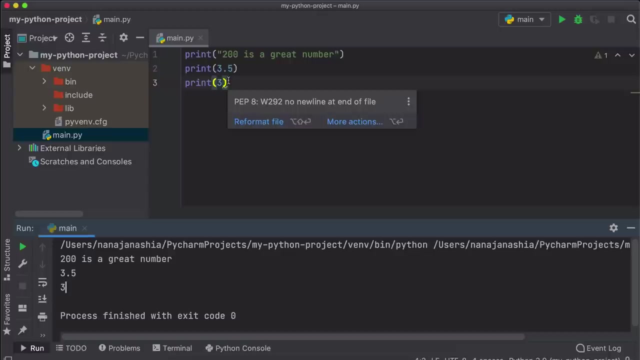 you have Integers and float data types and if we execute that, you basically see all of that printed as we wrote them. Now, obviously, printing values like numbers and text like this doesn't make much sense unless we're getting some useful information from our simple program right here. 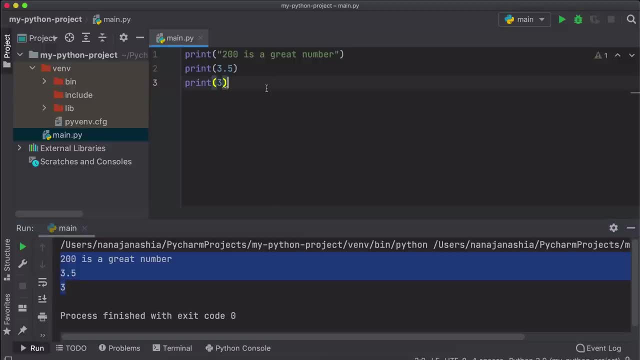 right. So let's do something more useful with Python. now Let's clean all this up and let's say we want to do some calculations. Very simple logic that basically calculates how many minutes there are in 20 days. So we have 20 days which have 24 hours per day. 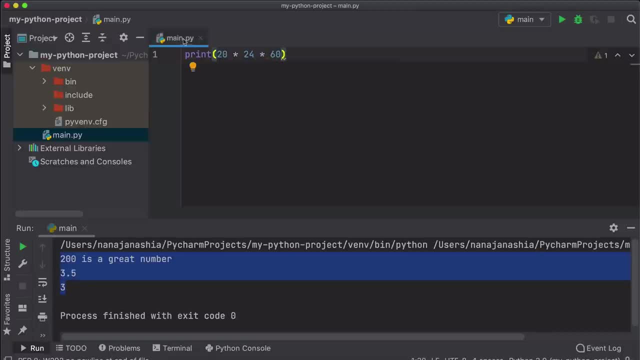 which have 60 minutes per hour. So this line will give us, Basically, calculation of minutes for 20 days. And there you go, That's our number. Now. this makes a little bit more sense, because now we have a program that actually does something for us. 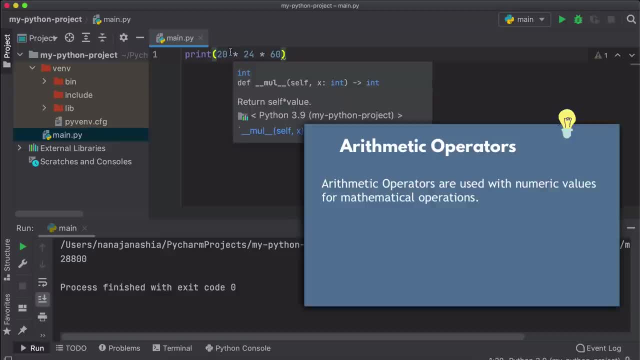 So basically, as you see, you can do any math operations on numbers in Python and again in many other programming languages. you can do plus, minus, division, whatever, just like you know it from basic math. However, I want to know right here something. 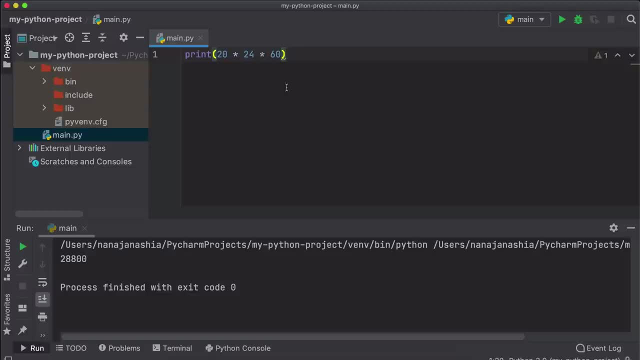 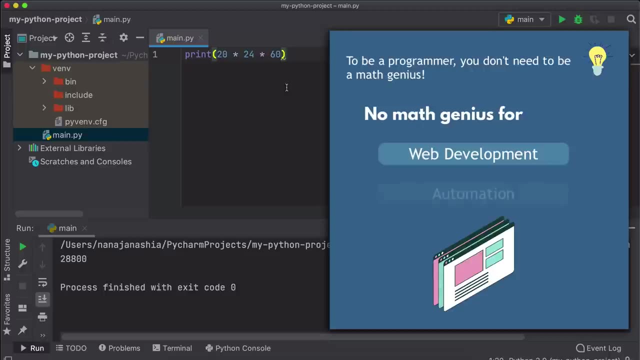 That many people think about programming and maybe are misinformed about, which is if you're doing web development or maybe DevOps automation with Python and not something like data science or data analytics. This is probably an example of the highest math knowledge that you need for programming in Python. 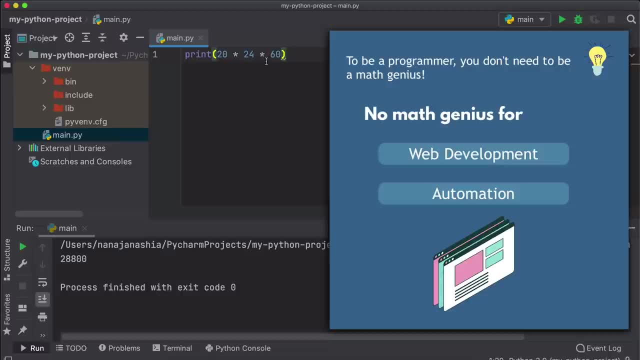 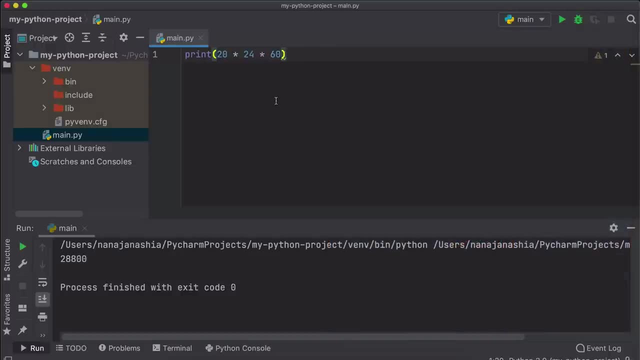 because, even though we're going to use some calculation examples- because they're just good As examples to show you the basic concepts of Python, you do not really need any advanced or even intermediate knowledge of mathematics when programming, because it's really not about meth. 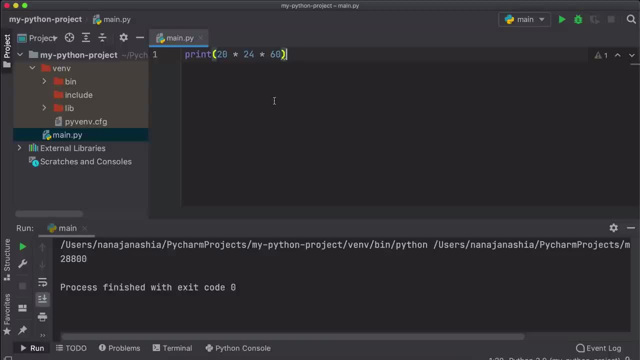 However, what you need is logical thinking, and we're going to be doing some of that and see that as examples, So just bear that in mind in case you are misinformed about that. So back to our example. we have this number that is displayed here as a result. 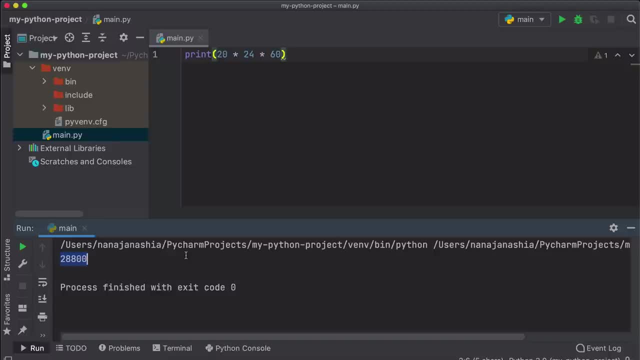 However, maybe if we use this program we don't remember or we don't know what this number stands for if somebody else is using. So we want to add some descriptive information about this number that says this is how many minutes there are in 20 days. 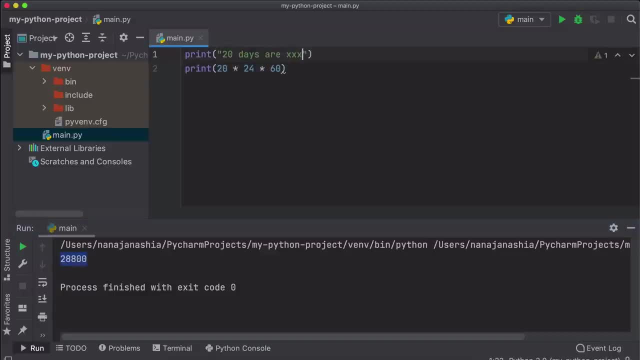 So basically we need a line that says 20 days, are this many minutes? And this should basically be exactly this calculation right here. So how do we put this calculation basically right here in the middle so that we end up with this whole phrase displayed right here? 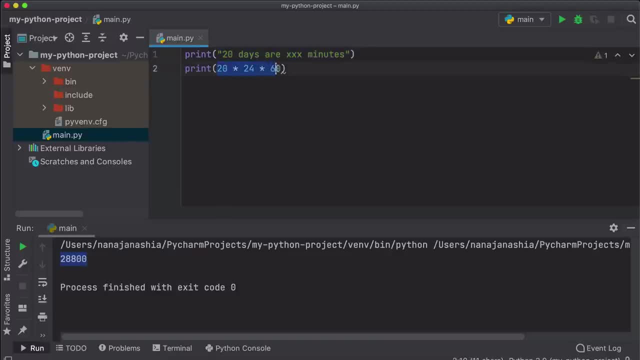 So how do we combine text and numbers, basically, or calculation of numbers, and in programming languages- Again, this is not specific to Python- We would do that using something called string Concatenation, and string concatenation is basically a fancy word for gluing together or combining multiple strings. 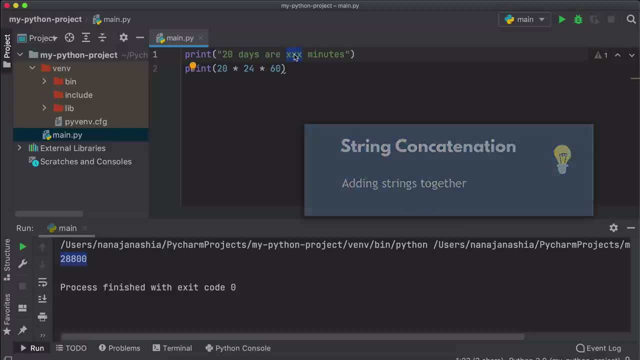 Now how does the syntax for that look like? We combine the strings using plus sign. So apart from adding numbers, obviously using plus, plus is also used in programming for combining multiple strings. So in our example we have three string values and we want to put them. 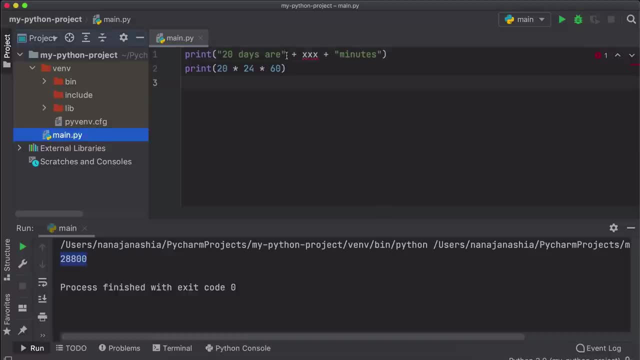 All together in one string or one sentence. We have the first string- 20 days are- and then we have the second string- minutes- and in the middle the third string, which will be the value of the calculation. However, if we just put a number here, 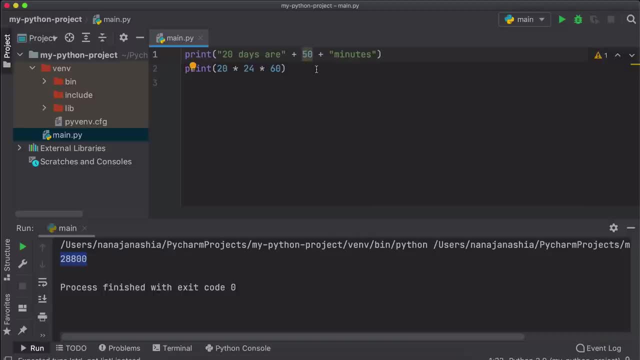 Python interpreter tells us it's not a string, it's a number, So we need to turn it into a string. Other programming languages do that automatically. in Python, We need to do that Explicitly, So we need to tell Python: take this number. 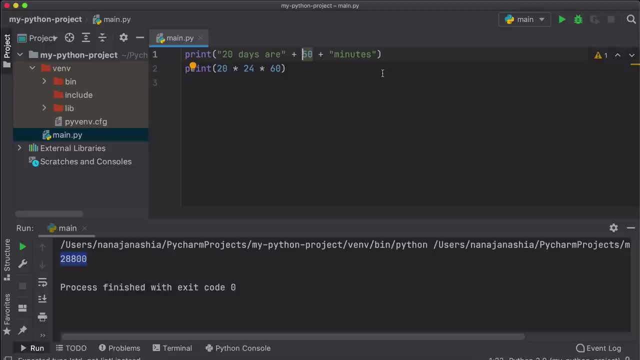 but not as a number but as a string, And we do that using a syntax That looks exactly like that. So, basically, we have a non string value, but we're telling Python we want it as a string because it needs to be printed out as a text. 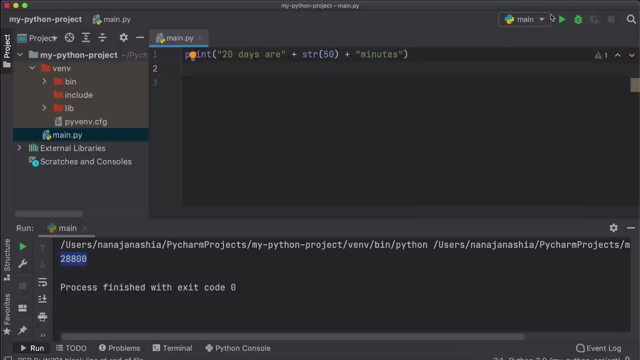 basically. So if I execute this line, let's see what happened. And there you go. We have our output just like we wrote it here, But you see that there are no spaces around. So basically, 50 is just really glued together without any space around. 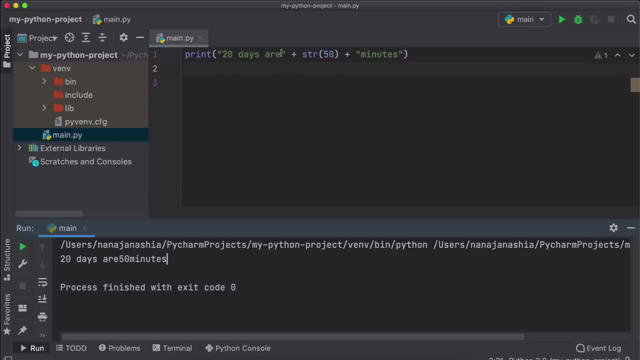 And how do we put spaces around these 50?? Basically, add a space here and a space here. Now, why does that work? Because this whole thing, for Python, is a string. again, because we are putting it within these quotes, So basically any character that you see on your keyboard right now. 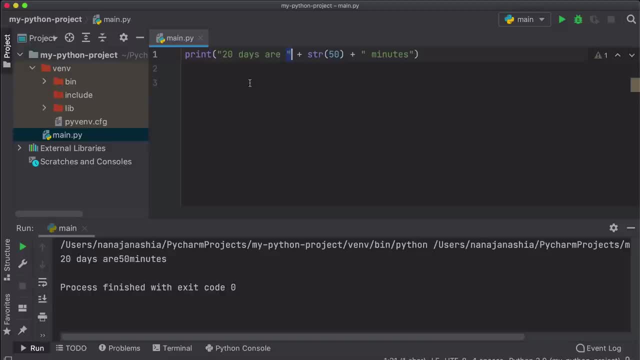 if you put it between those quotes, is interpreted by Python as a string including the space character, right? So if we execute it again, we have spaces around 50 in our sentence or phrase. looks fine, And if you're thinking right now, 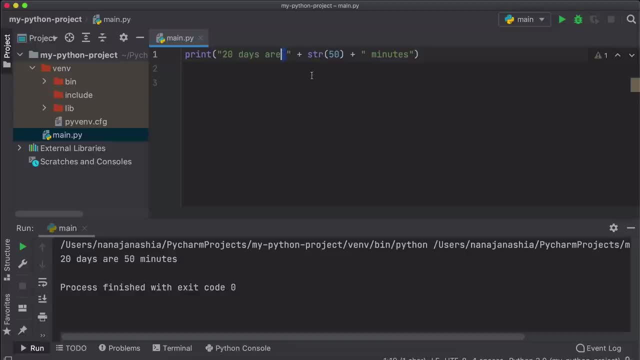 this is actually kind of annoying because first of all it looks ugly And also there's a high chance you're going to forget it. That is absolutely right. So in Python again specifically, there is a way to do it in a more elegant way. 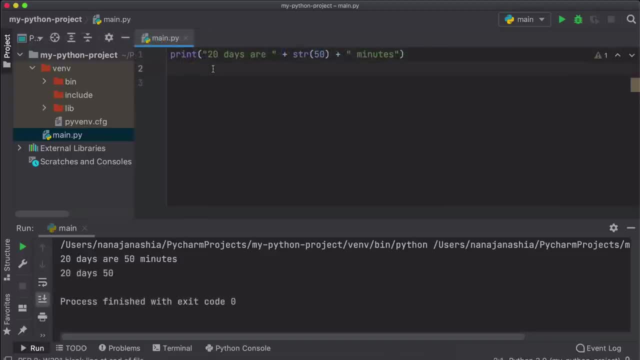 using a different syntax and a more elegant syntax, for that It's actually close. This is print And let's write that again. And instead of having these plus, we have curly braces and we write our number inside or whatever non textual value. 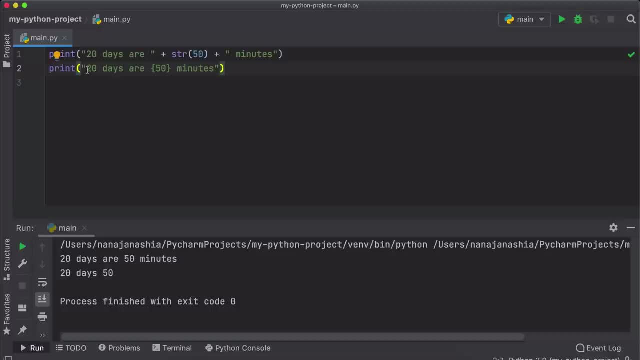 And at the beginning, right here, basically, before we start writing a string which starts with quotes, we just write the letter F and you see the syntax highlighting as well. Basically sees that this is not part of the text, It is non text value. 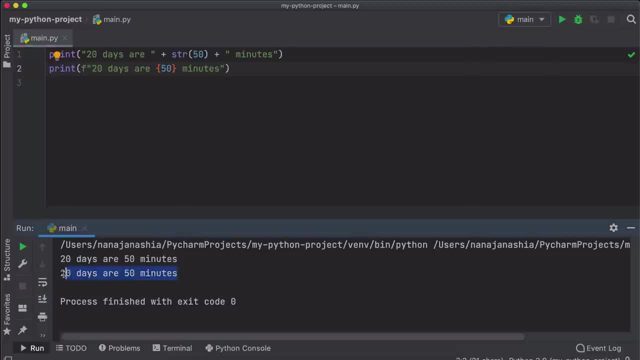 And if I execute it, I should see the same output from the second line, And this is really a way cooler way to write this instead of using plus. But this is something very common and also something that you would encounter in most programming languages. 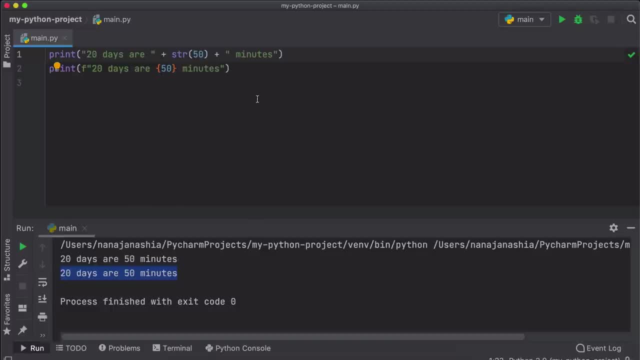 So just important to know that this is a syntax for string concatenation as well, So we can basically just remove it and use this syntax for our examples, and also know that this syntax is actually a new addition to Python, So it only works if you have a latest Python version in our project. 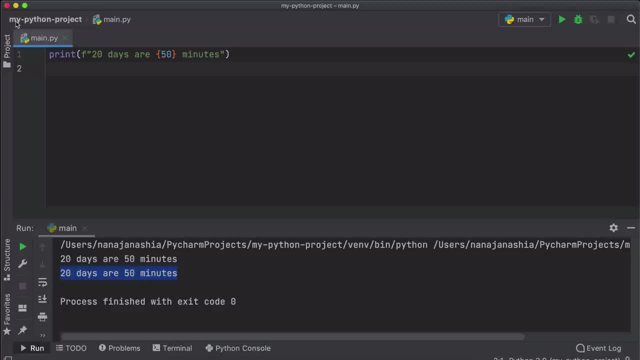 If you remember, we actually configured and chose version three, point nine, And that's why it works for us. If you use Python to, for example, Python version two, this syntax is not going to work for you. We can actually demonstrate it. 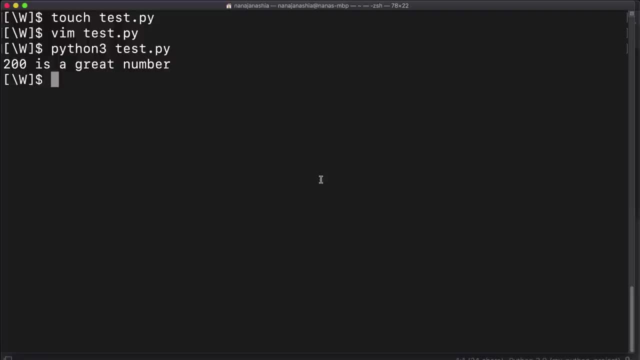 So I'm going to copy that line and I'm going to Change our test dot PI. And now, if I executed using my Python three, You see it works fine if I do it with Python, which is version two, point something: 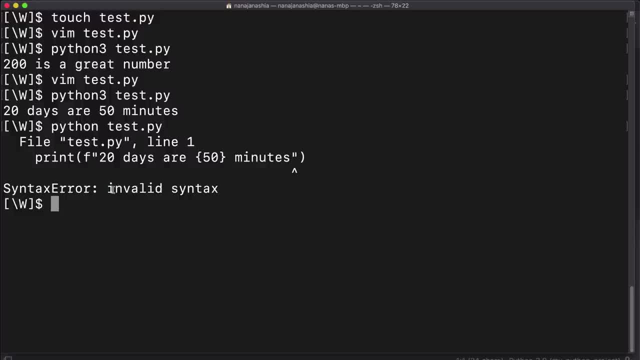 Let's see what happens. There you go. Syntax error: invalid syntax because Python version Two, point seven, point ten. So older version basically doesn't recognize this syntax. So just be aware of that. So this syntax actually only works for Python versions starting from three, point six. 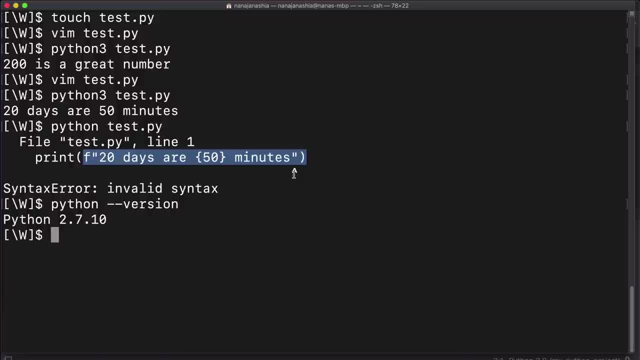 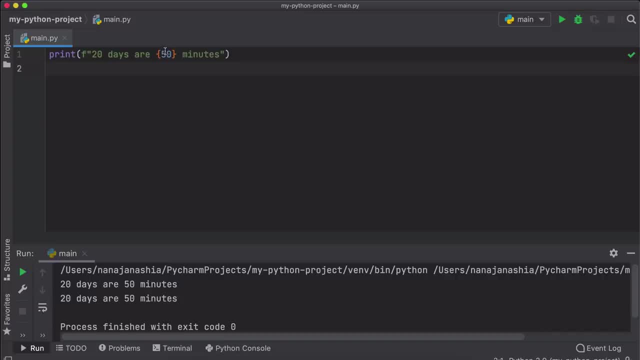 So everything below that, every Python version basically, will not recognize this syntax, as we see right here. So again back to our code. and now we just have a number here, But what we actually want is the calculation for getting the correct result right. 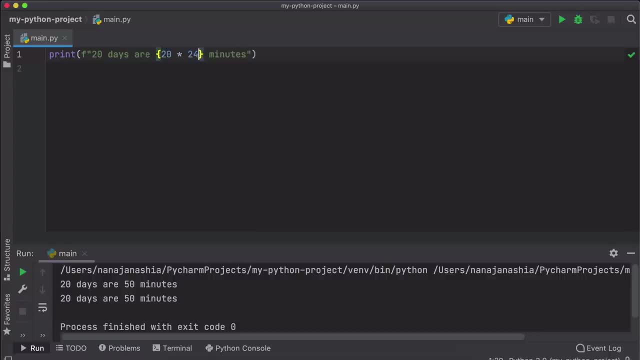 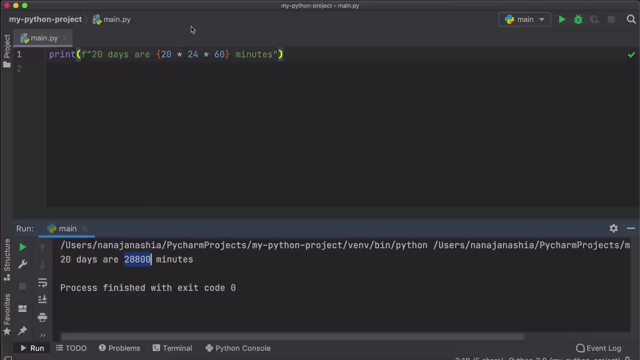 So we want again twenty days In hours and then in minutes. And if I execute it, you see that the calculation was done And here we have the full, complete sentence with the result in it. And if you're curious, this F actually stands for format. 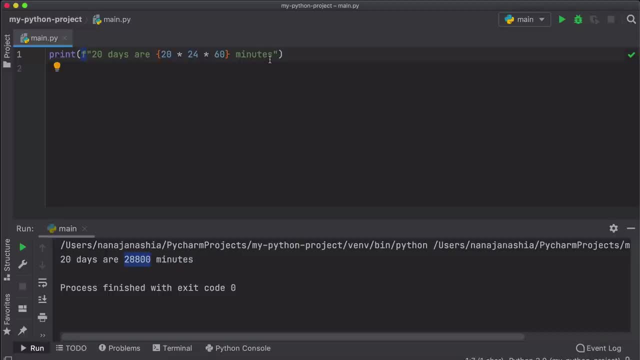 So this is basically formatting our text, Or our string, in a correct way. Awesome. So we have this line of code here that basically calculates for us how many minutes they are in 20 days. Let's say, we want to do the same for thirty five days. 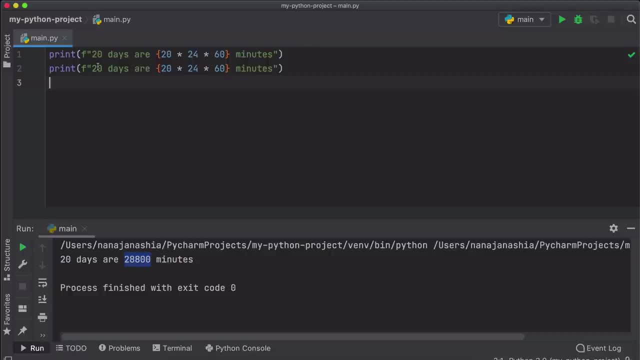 right. What we can do is basically copy that line and replace the values for twenty with thirty five And if I executed I get the same calculation but for thirty five days, and we can do that basically multiple times for different values. So let's say we want it for fifty days and we want the same calculation for. 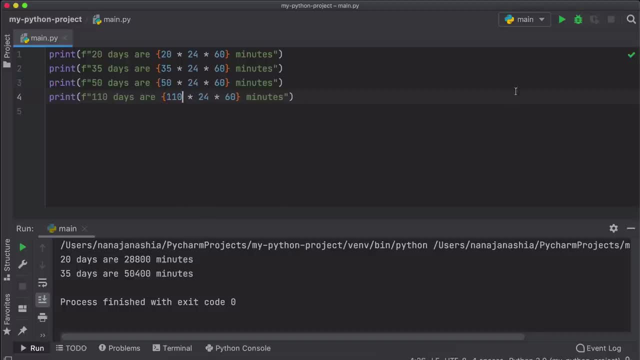 I don't know. let's say, hundred and ten days doesn't really matter, And we have obviously different number of minutes for each of these values. And now let's say we wrote this program, It's ready And we're using it. 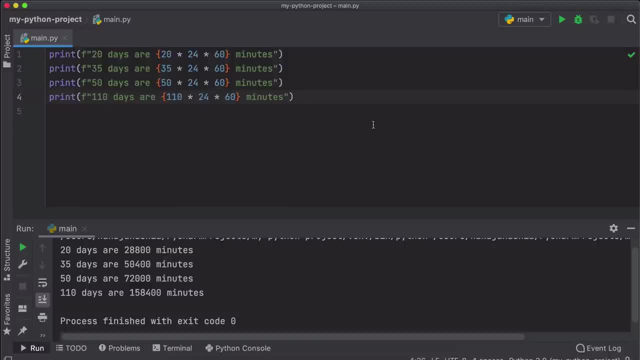 And at some point we decide. you know what? I want this program to actually calculate how many seconds there are. for this provided days instead of minutes. So what we would need to do in that case is basically change the calculation in all those four lines. 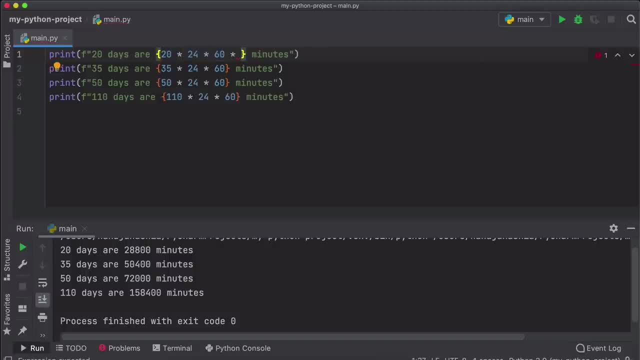 So instead of minutes, it should actually calculate number of seconds in a day, right? So we have the hours, minutes and seconds, And we would have to change the text as well here, And we would need to do that for each one of those lines. 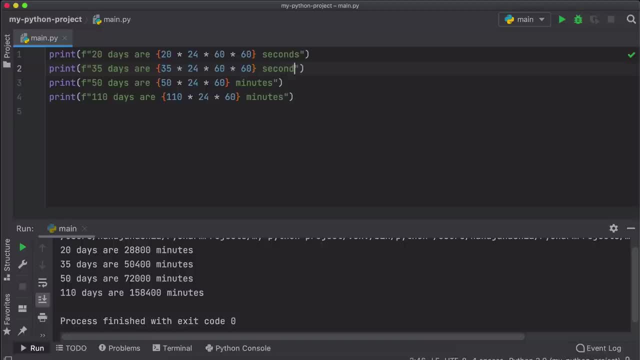 right. So we would have it here Like this: And again, if we need to modify this for hours or milliseconds or whatever, we basically have to do these changes multiple times, right? Even though, if you actually look at that, this is the same exact calculation for each. 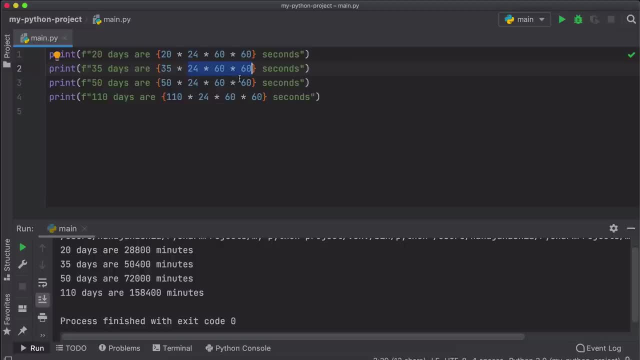 Line. that doesn't change right. If you want seconds, then this is the calculation that you need to do. So how can we actually avoid repeating the same calculation and the same text in our code? And the answer to that is variables. So in programming languages, 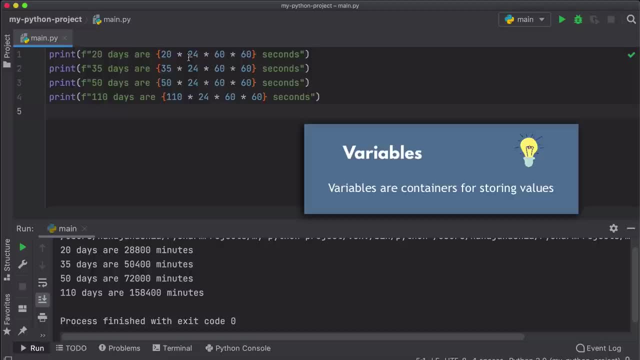 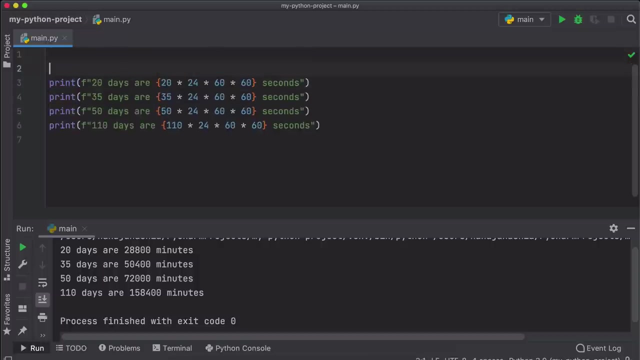 we have variables that basically hold values that will repeat throughout your code, that you can set once and use it in multiple different places. So, instead of basically repeating this calculation four times, we basically do this calculation once, like this, and we basically save this value in a variable so that we can use it whenever we need. 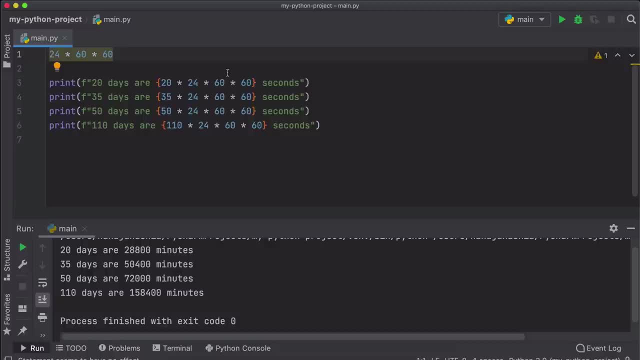 Right, And the way that variables are defined in Python is variable name. Let's call it two seconds Equals and whatever that value is, that repeats itself and they want to save into a variable. Now I want to make two notes here regarding the variables in Python. 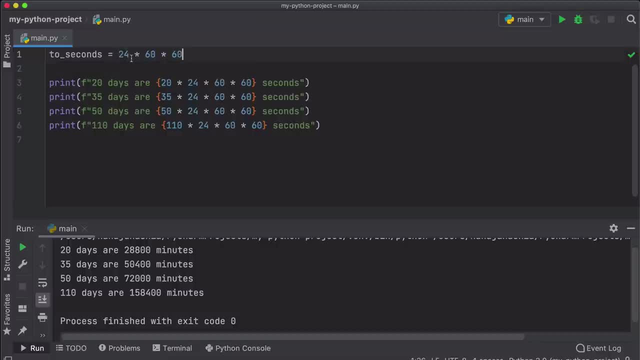 First of all in Python defining or creating a variable and giving it a value, like this syntax for that is actually very simple compared to other languages because you just have the variable name And the value. in many programming languages you actually have to define here some kind of data type for that variable. 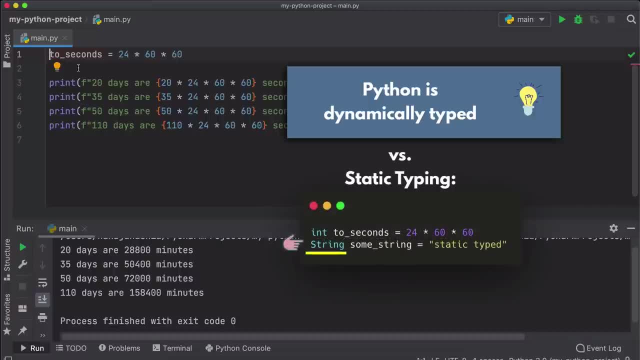 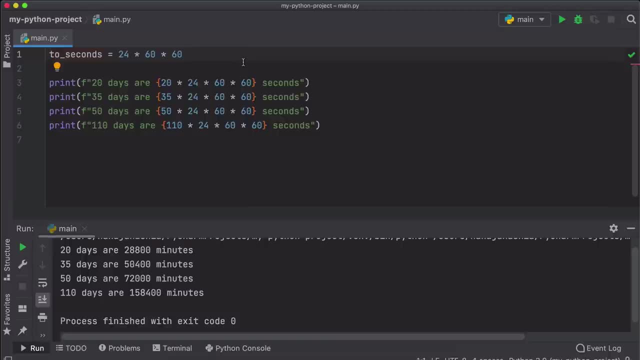 For example, if it's a number like float or integer or string, et cetera, in Python you don't have to define that, You just have name of the variable, Simple as that. The second one is the naming convention or standard for the variables. 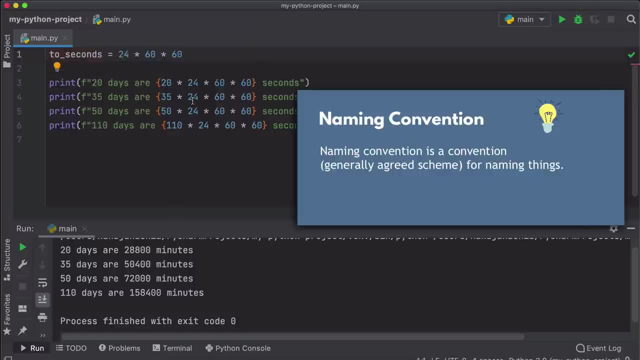 So we have two words. For example, if we name our variable calculation to seconds, right, we have actually three words here. So variables that are descriptive, So basically they tell you what this value actually is about. So they have multiple words in them. 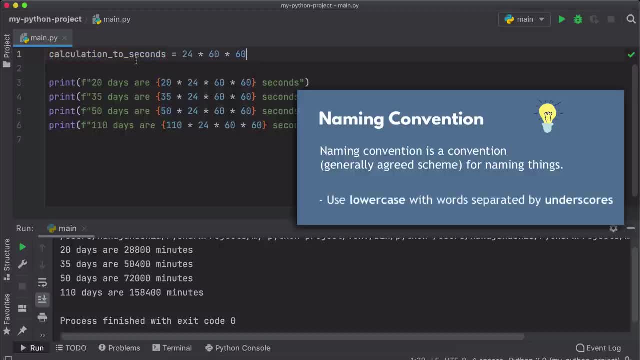 You can separate them using these underlines. again, in different languages The naming for variables can be different. in Python, This is actually one of the standard ways of defining variable with underscores, which I find a pretty nice and easy to read, So we're going to use this syntax basically throughout the course. 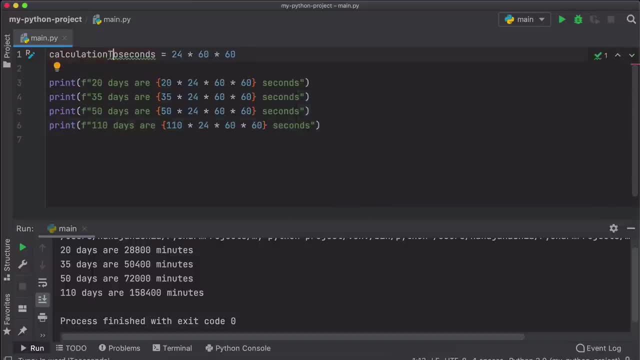 It will be totally and absolutely OK if we wrote it like this or if we used capital letters instead, But again, this is probably the most readable form and this is what we're going to use now here. Note that we can decide whatever name we want to give our variable. 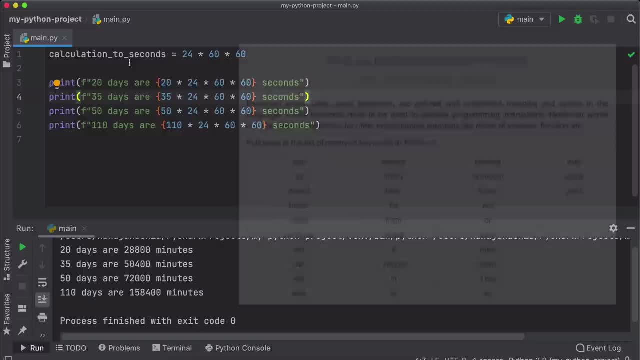 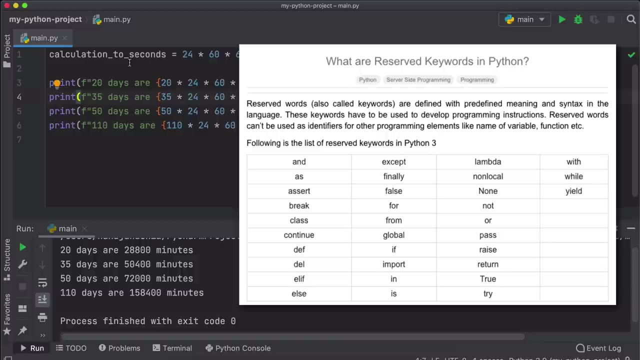 But in Python there are some specific words that have special meaning to Python. These are called Reserved words, So you can't use these words as variable names, and we will use some of these reserved words throughout the course. So you will see some examples. 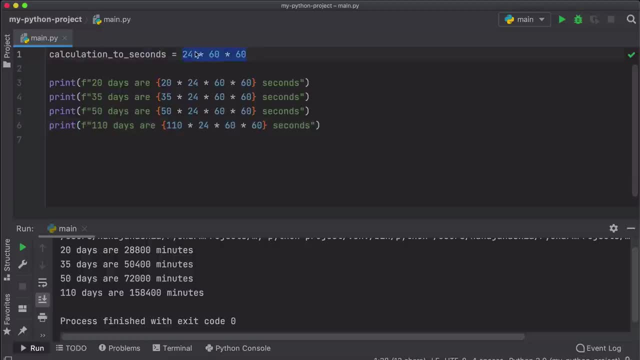 Great. So we have our variable defined here and this is the value that this variable gives us. So how do we replace now these repeating values with this variable? So we're going to delete that And again inside, we're simply going to. 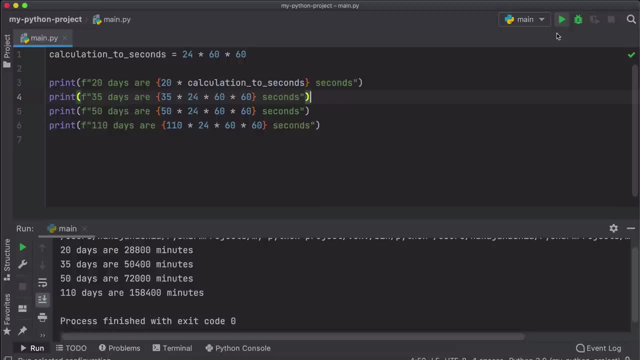 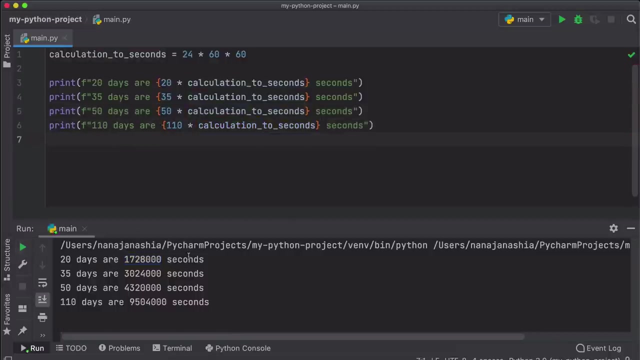 Copy the name of the variable. So let's execute And, as you see, we have our value printed just fine, and we're going to do the same for All those Values and again execute. Everything works just like before. Now you may be thinking: if we change this to minutes? 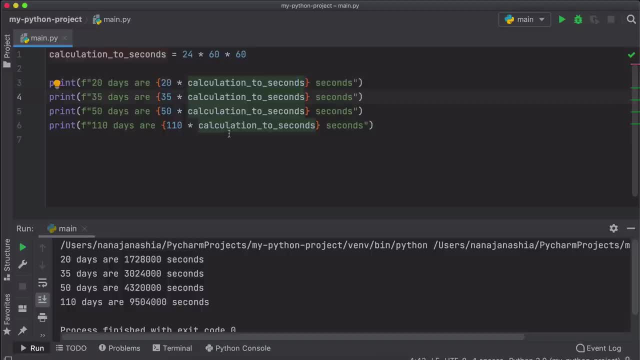 we would have to change the variable in all These places. So that's our case. We can basically just rename our variable something more generic. So let's say, calculation, two units, and this could be now any unit that we want. Second minute does matter. 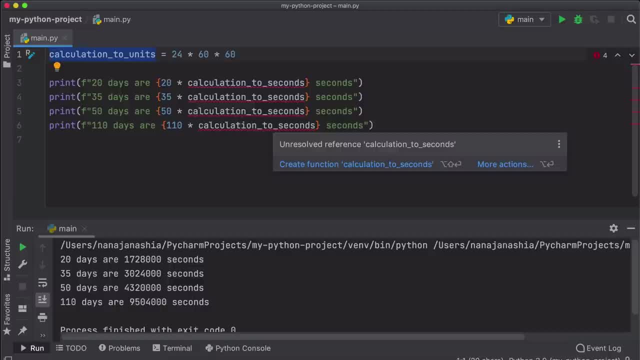 And this is exactly the advantage of variable, because you can name it whatever you want, Which basically just describes what this variable is about, And now You Won't have to change that again And we can also replace this one here accordingly, Since it's a text. 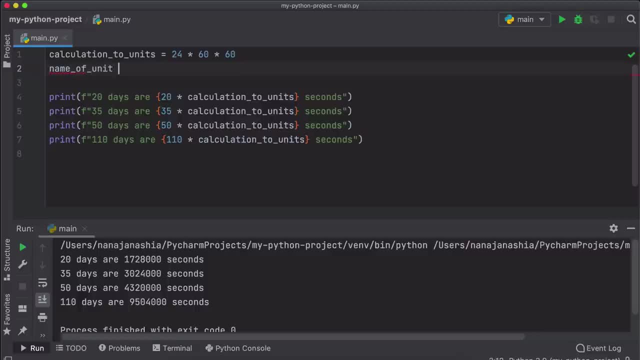 we can call it a name of unit, We can also call it unit, Doesn't really matter where the ones deciding what that variable name is. And once we have that variable, we can now replace it here. How do we do this? Because this is actually part of a text. 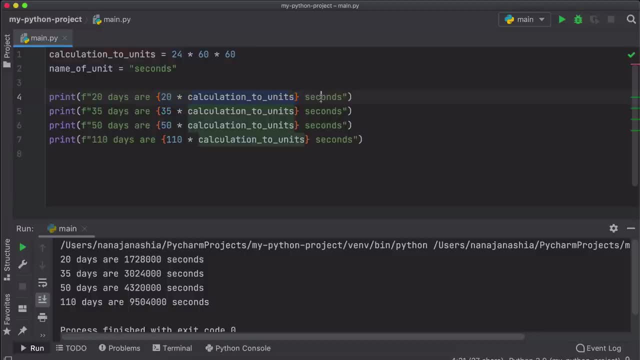 a string. the same way we did right here, We're going to Delete that and create an expression, create a syntax that basically tells Python: hey, this is not a string, This is a non string value, And you already know this could be either number or variable itself. 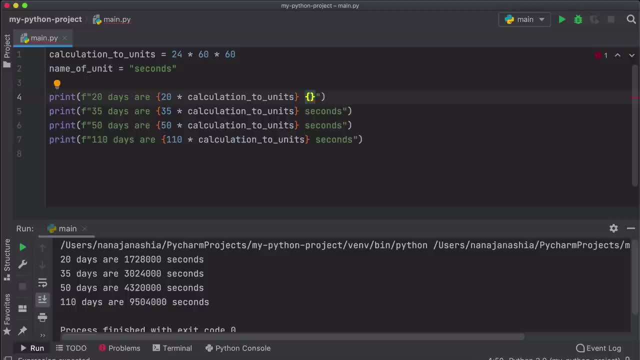 And so we're going to use the curly braces and the name of the variable And just like that we have substituted these values here And if I executed works perfectly fine, And we can do that In all four lines and our code is still working. 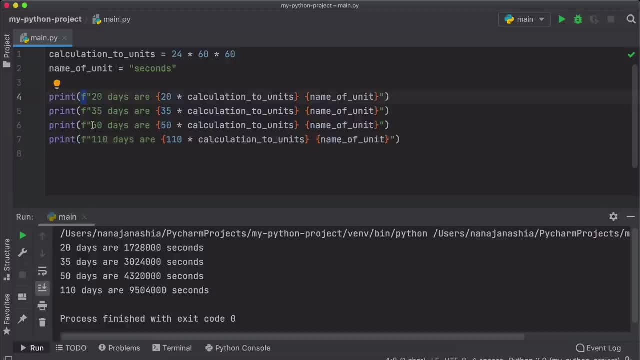 And this syntax right here, with this format at the beginning, basically prevents us or avoids, basically saves us from having a bunch of plus signs here and then space characters, et cetera. This all looks way elegant now. And now if at some point we actually 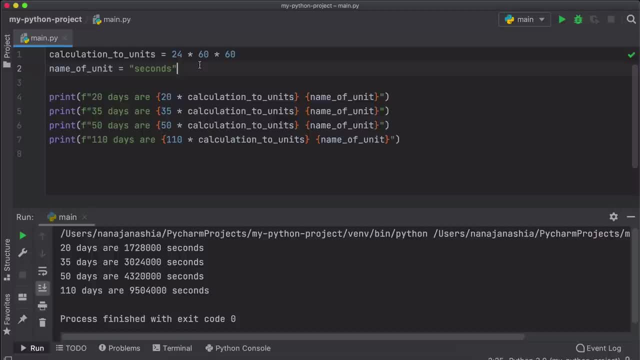 decide. you know what? I want this program to calculate how many hours there are in the given days instead of seconds, And we want to change the program to do that. We could basically just change the calculation here And instead of seconds we have hours. 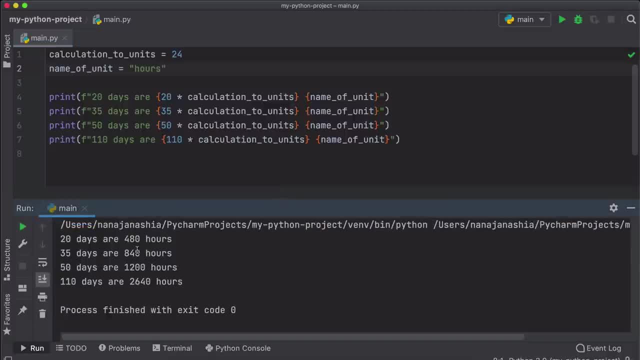 And if I execute, there you go. we see the changes right away. So this is why, when you're programming- doesn't matter which language, including Python- using variables will be probably some of the most frequent thing that you do, because you always have values that are repeating themselves and you want to write clean code. 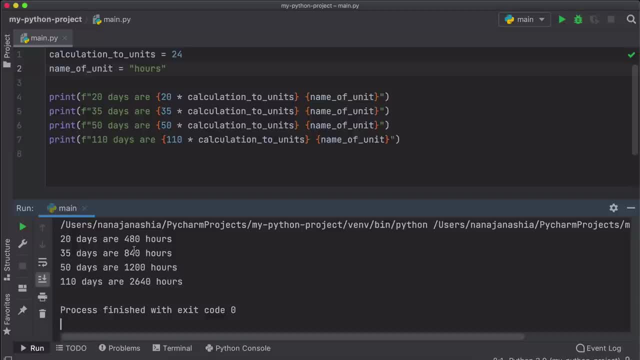 So you create variables, And one of the best practices when creating and using variables is, as we're using actually here- is to name your variables so that you later, and also other programmers who are working with you, understand what this variable actually does or what type of. 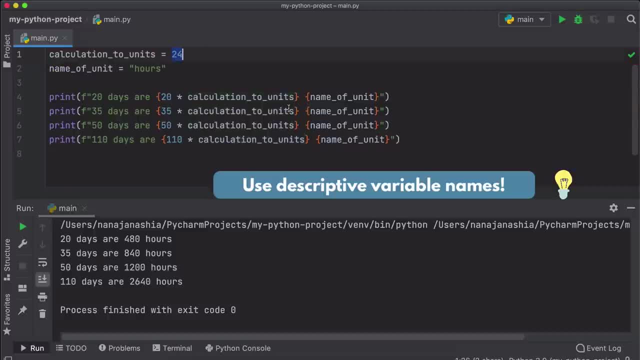 value it actually has, because if you just look at 24, you would probably not know what this 24 is about, right? But with variable, you actually know that this actually represents a number that is used for calculating units, right? It could also be more descriptive, like units for days. 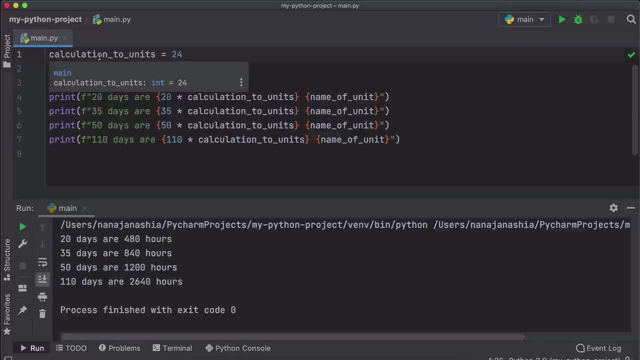 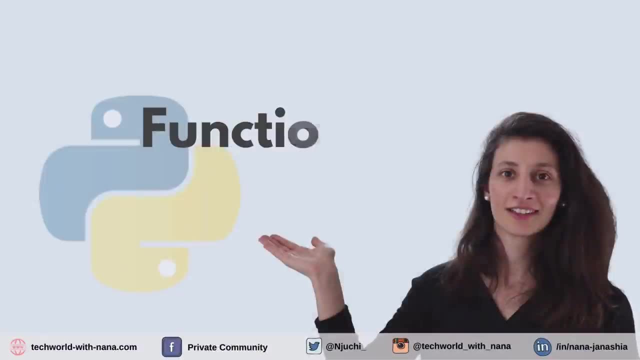 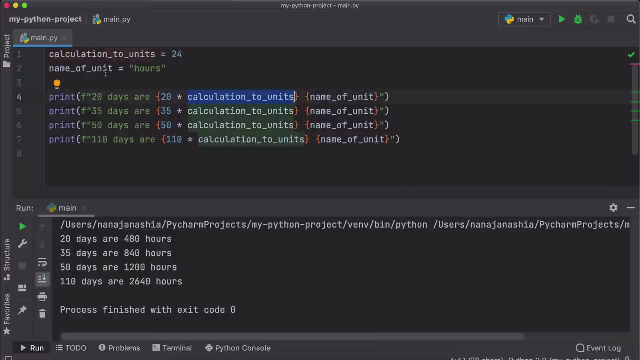 but generally, another advantage of variable is to basically describe that value as well that you're using in your code. Now, another thing you probably also noticed is that even though we're using variables here, so that we don't have to change those values in four different places, 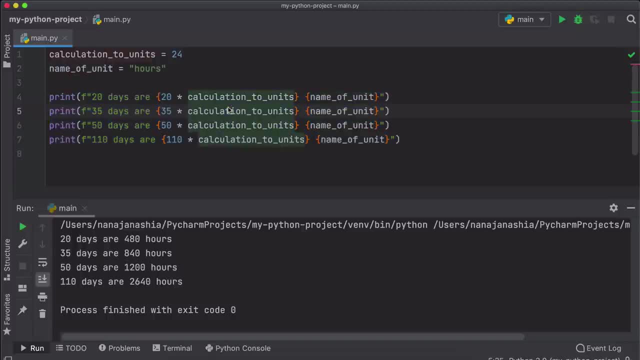 a lot of these four lines are actually pretty similar. The only difference in those four lines are actually these numbers right here. Everything else is exactly the same. So what if, instead, we wanted to make this code cleaner and basically I avoid this type of duplication in our code? 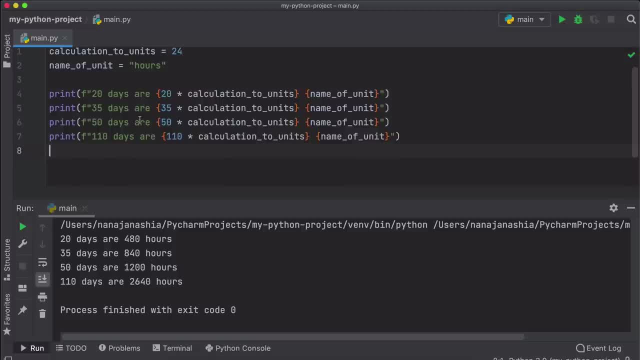 right. So, for example, if we did this for ten different values, we would have the same line, This long line, basically ten times right. So how do we avoid this type of duplication? So right here, we actually avoided duplication for specific values. 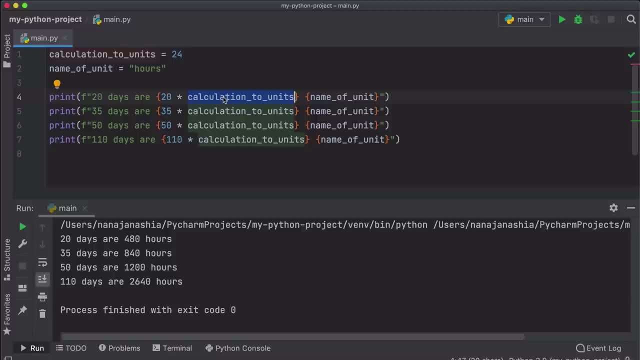 right Piece of string here, a whole calculation here. But how do we actually avoid duplicating a whole line, right, The, the whole piece of code basically, which has multiple different stuff in it, not just a value, And we do that using functions. So functions are basically blocks of code, like 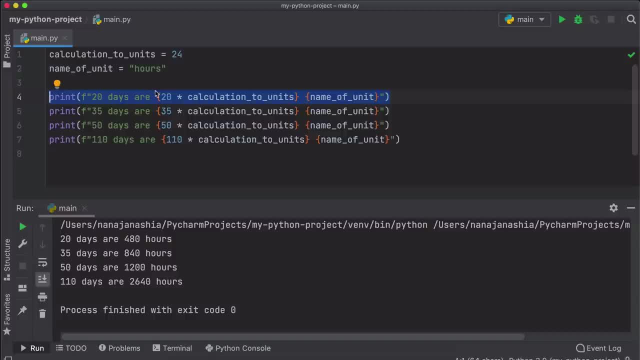 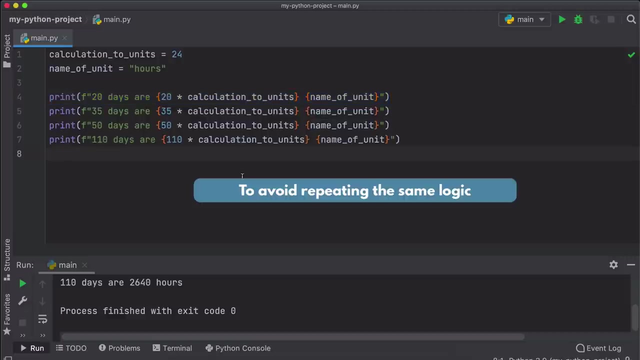 this Right, Or basically logic in code that does something. It's not just simply a value, but actually does something more complex that is again used in order to avoid repeating the same logic, or most of the same logic, in your code. So how do we create functions? 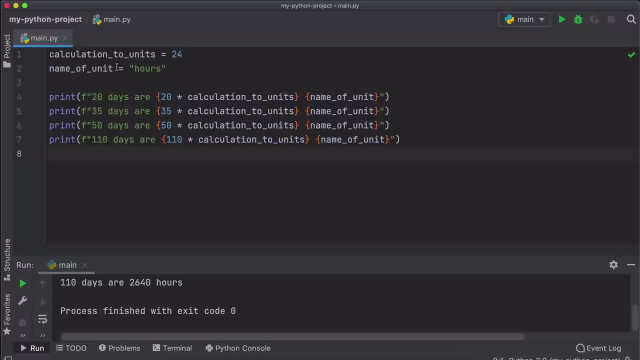 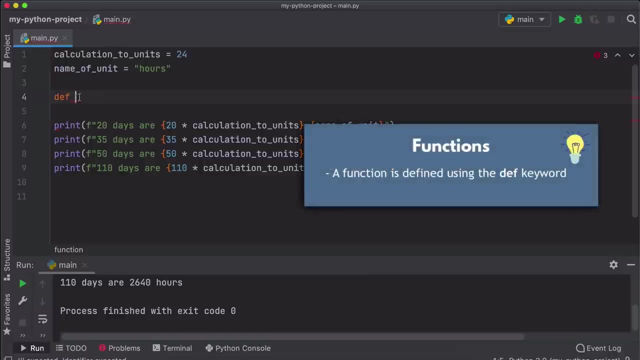 Just like we created variables, here we create functions, And the way we do that is using following syntax. right here Let's create our first function. We start with def. So we define a function just like we define a variable. But for function we need the function. 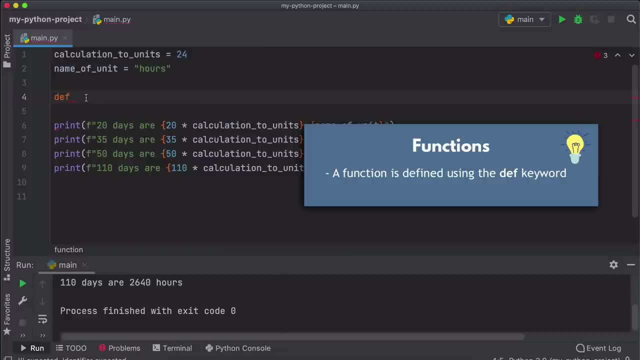 this keyword basically called death. And now we can give our function a name. just like we gave name to a variable, We can give our function a name, and here we can use the same standards like a variable. We can name the function something descriptive, something that actually 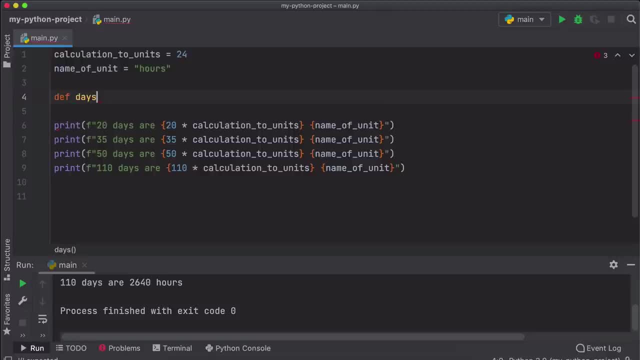 says what this function does. And let's call our function days to units, And then we have the brackets and a column. So this line basically defines a function. It tells Python: hey, whatever comes after, this is actually going to be a block of code that is going to be referred to, or is? 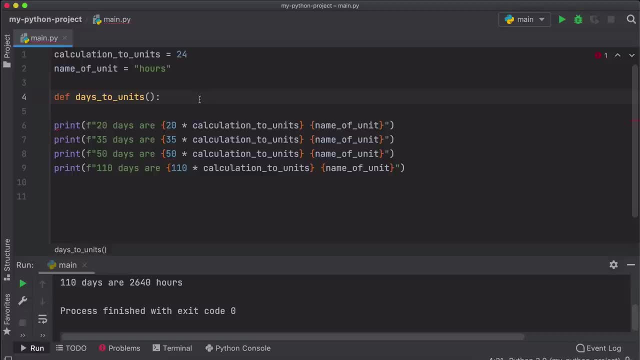 going to be named these two units? And how do you write a function? I'm just going to copy this one actually here And let's give us some space. And again, this is very specific to Python. We need to indent here with spaces And I'm going to paste in what I copied inside these two lines. 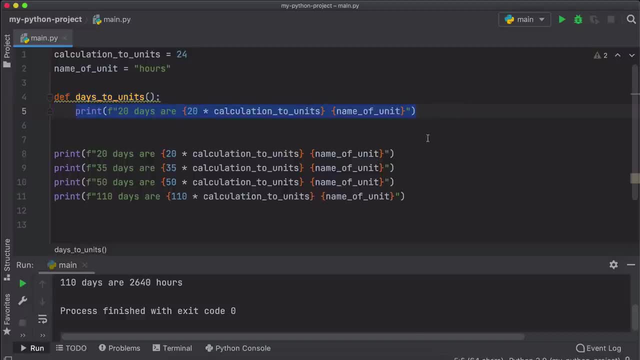 basically tell Python: this piece of code or this line of code- because we just have one line here- belongs to a function called these two units, And again we just have one line, but this could be function with hundreds of lines, Right, So I can write whatever I want. The next line: 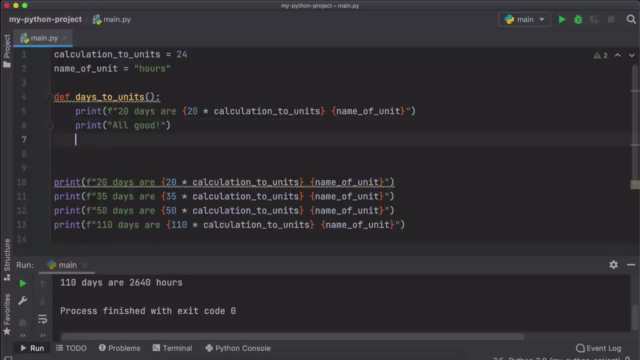 all good, And then I can do some calculations and I can basically write whatever logic I want here, and all of this will belong to this function. So now this logic is inside a function that is called these two units, And we can actually get rid of this. 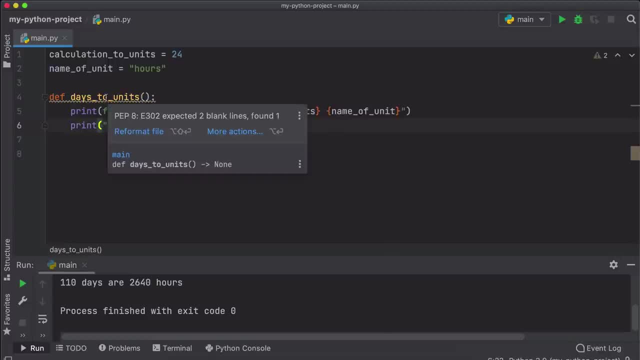 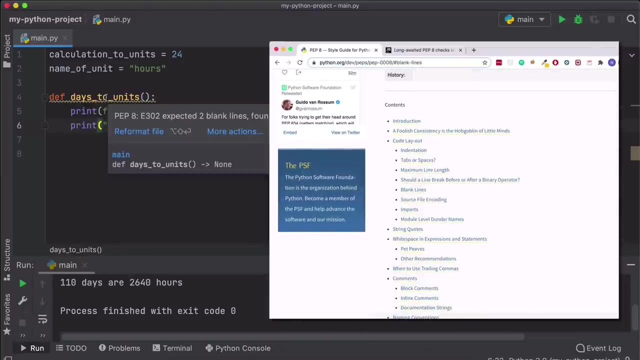 and test our function And here, if you noticed, we have this yellow line under the function name. That's actually a warning for our code style. It says we need two blank lines before. So PyCharm has a built in official style guide for Python that tells you how to style your. 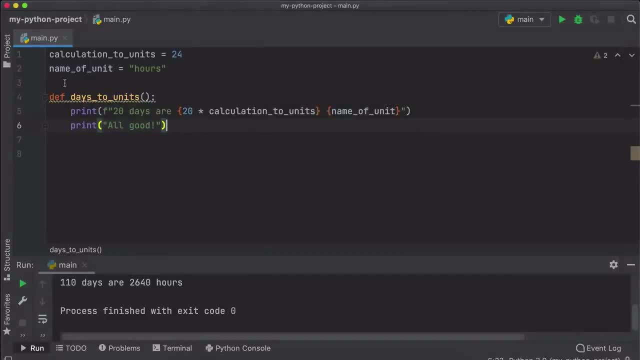 code or how to write your code correctly. Now, why is code style important? Well, just like you write code, you need to read code from other developers or your own code to understand what the code is actually doing. So it's important that code is. 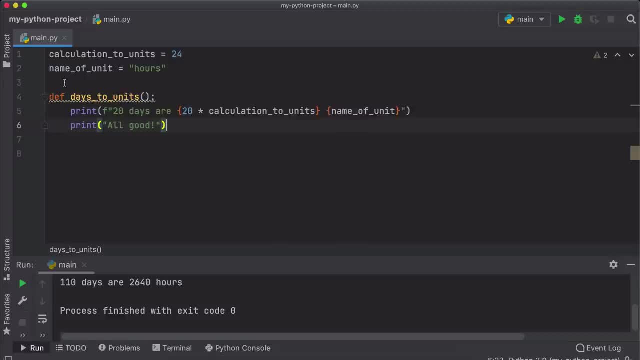 easily readable. So if you want to write code in Python, you need to write code in Python. So if you want to write code in Python, you need to write code in Python. And this is just another example of how an editor like PyCharm helps you to write code. So to fix the warning: 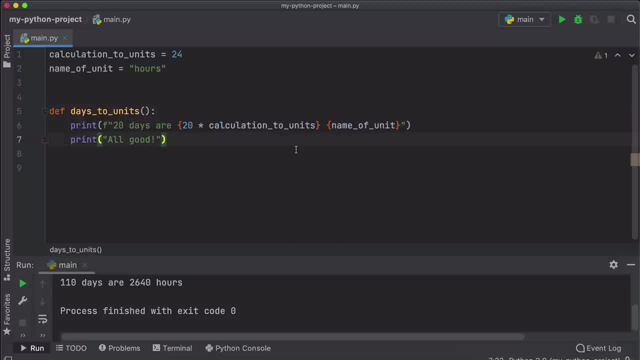 we're just going to add a new blank line before the function definition. So now what happens if I execute this block of code? I have the variables defined here that I'm using in the function, and then we have these two print statements. So what happens if I execute now? 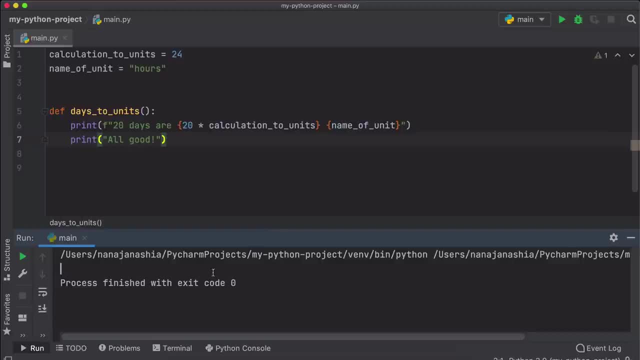 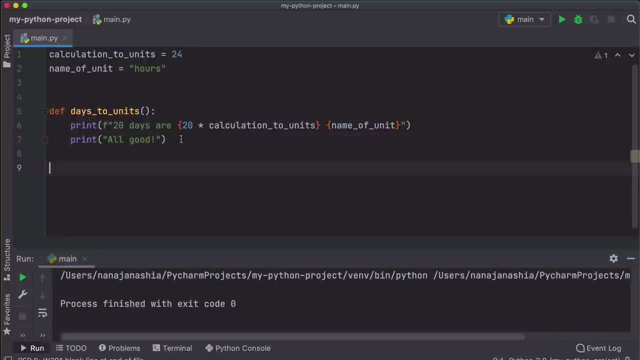 And, as you see, in the output here there is no output right. Nothing actually got printed. So what actually happened? Because we have those two print statements that we define in the function, but we don't see anything in the output. And the way it works is: whenever you create a 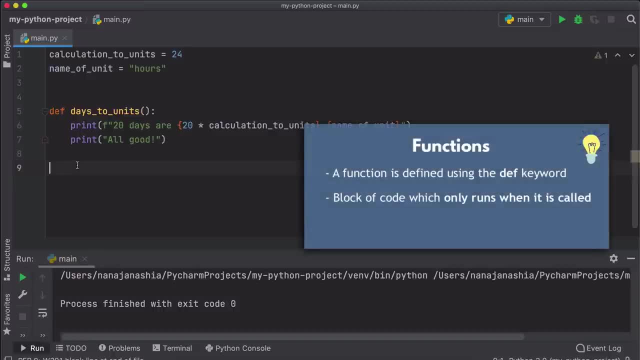 function or define a function like this, you actually have to use that function, right? Again, this is a similar concept to variables. We have created variables here and we're using that variable in our code. the same way, we create a function and we need to use that function. 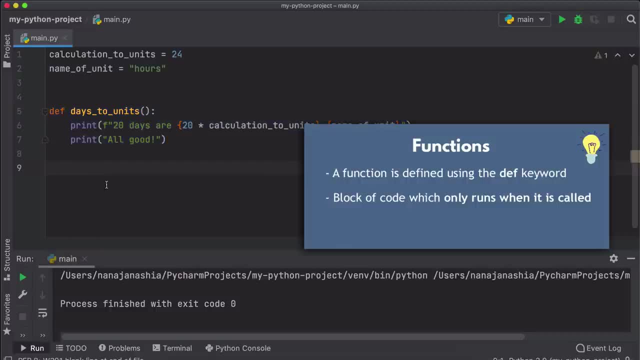 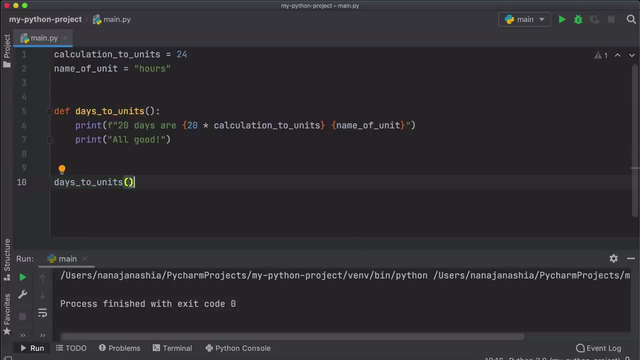 How do we use a function, Or in programming languages it's called calling a function or executing a function, And we do that using the name of the function, like this, And, as you see in the suggestion as well, using brackets like this. So this syntax here, basically. 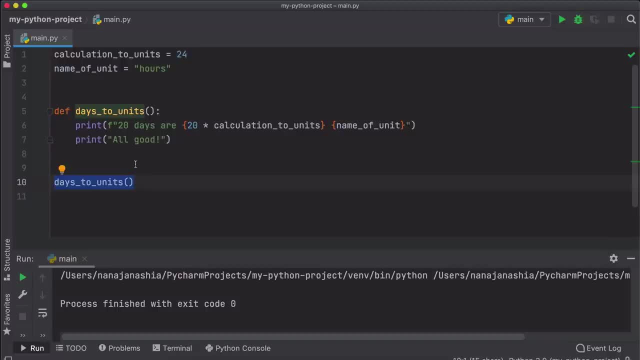 is what we call calling the function that we defined right here, or using that function. So now, if we execute it, there you go. You see that those two lines got executed and we have the results here. So we're creating variables and we're using that here. 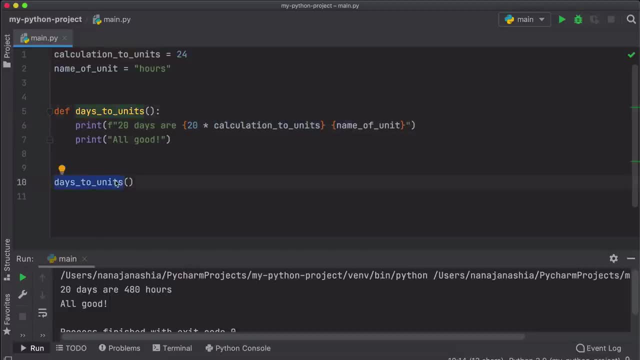 We're creating a function and we're using that function here. And note the difference between using a variable and using a function. Python knows this is a function because we are providing this and we have these brackets at the end, right. That tells us we're making a function call, basically. 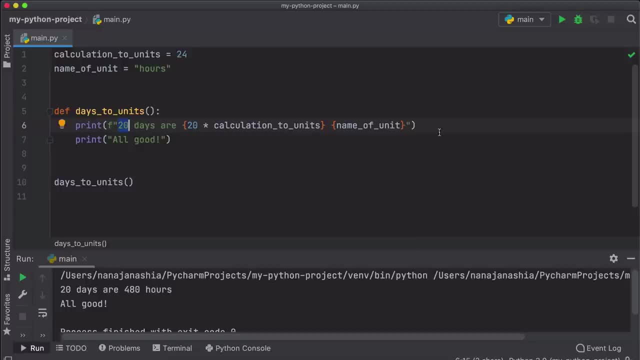 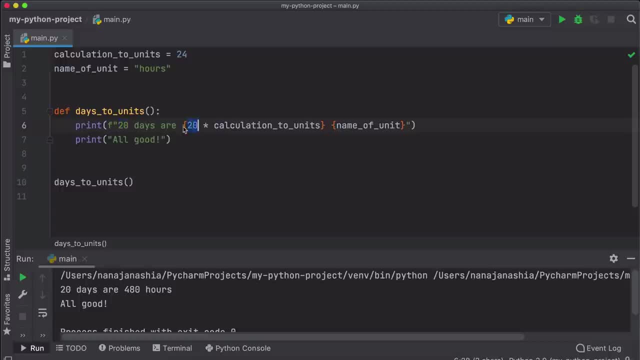 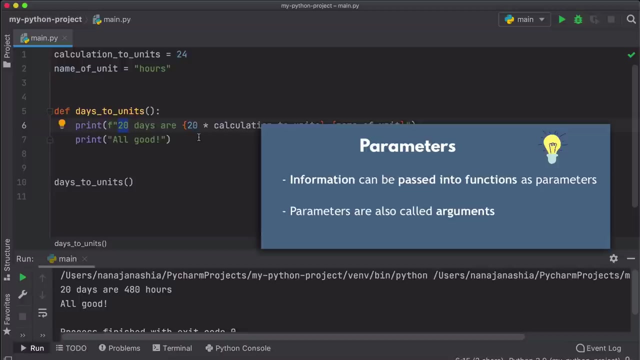 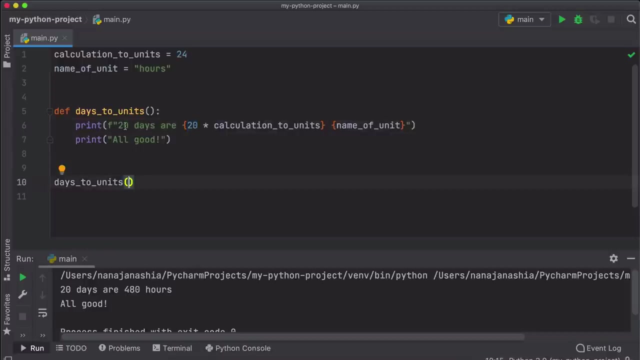 Everything else, except for these two values right here, actually stay the same, And we do that in programming by giving our functions some kind of input value, which are also called parameters. So instead of having this 20 basically here hard coded, as we say here and here we provide that value of 20 or 35 or whatever that value is. 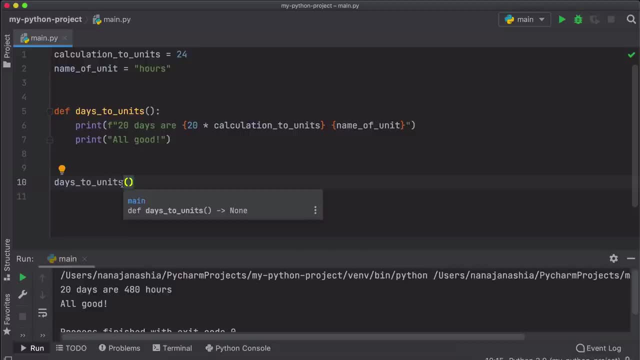 Basically whenever we use the function. So we are telling Python: use these days to units function with a value of 20, or use that function with a value of 35. And where we define this input parameter in functions is very simply by defining this parameter between those brackets. 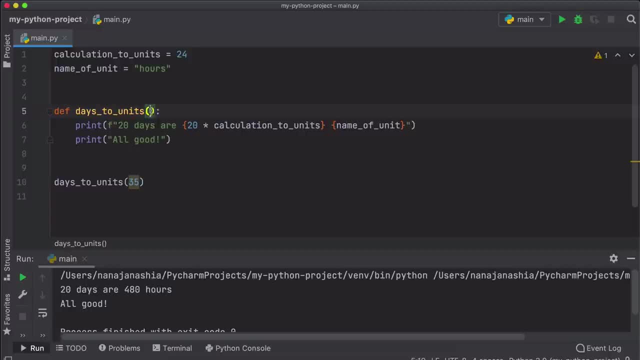 Right, So this is where the input. we as programmers define the input parameters. So, right here, How do we define that using our already familiar variables? So basically, right here, I'm going to define a variable and I'm going to call it whatever I want. 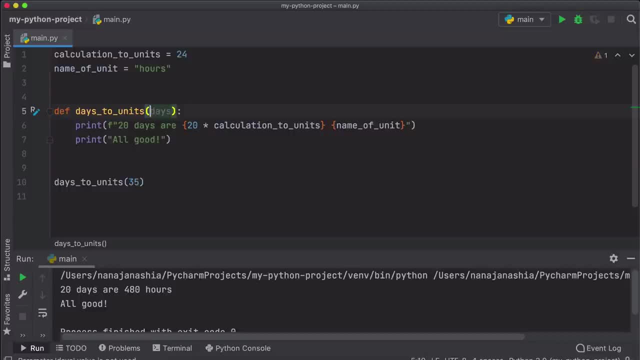 I'm going to call it days or number of days, But I'm not assigning a value to that variable Right, Like I did here, because I want it to be assigned whenever I use the function. So this basically tells Python That function days to units can be used using one input parameter, which is called number of days. 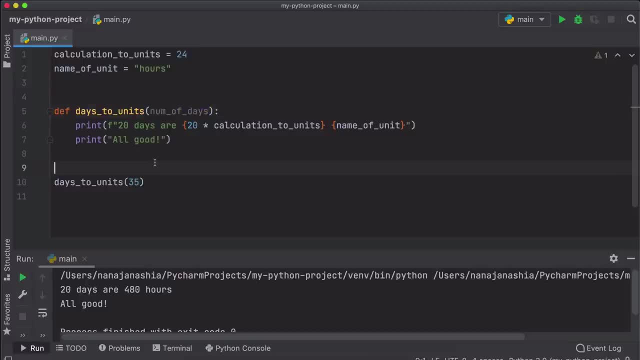 Right Number of days. So now, the last part which is remaining is replacing these values using this variable Right, And just like we do it in these two places where we're also using variables defined here, exactly the same way we're going to remove this. 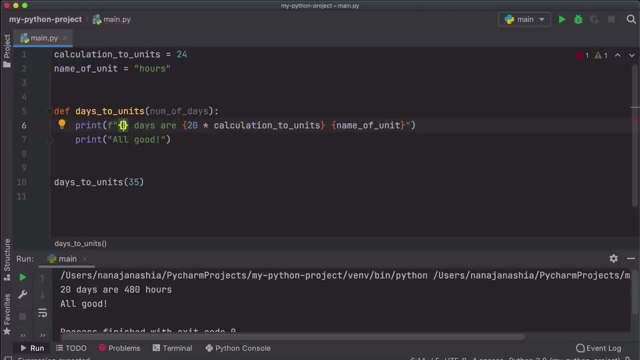 And Define a block for non textual value, and we're going to put our variable number of days here and also here. So you see now that our function actually doesn't have any fixed numbers in it. Instead we're using variables. We're using two variables that are defined outside that function and we're using one variable that is defined. 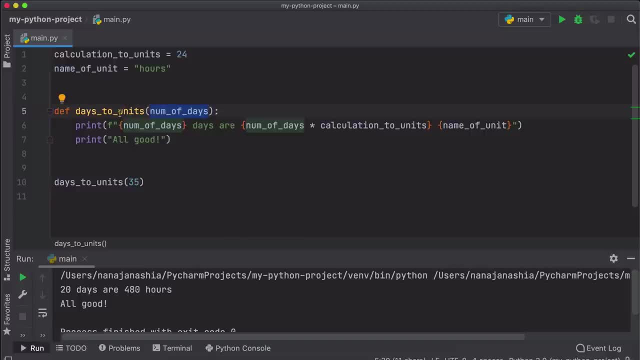 Right Within that function. Right, This variable actually belongs to that function. And now, as you see, whenever we want to use that function, we're telling Python: hey call this function called days to units, with a parameter, an input basically of thirty five. 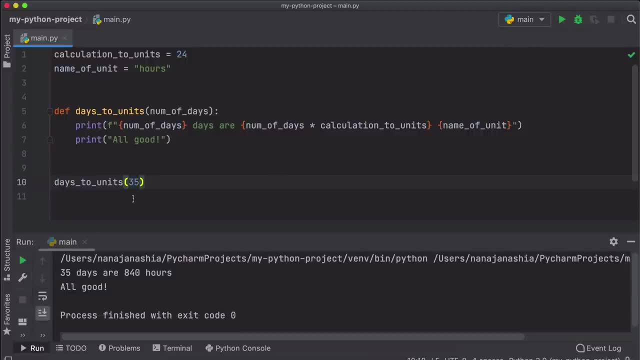 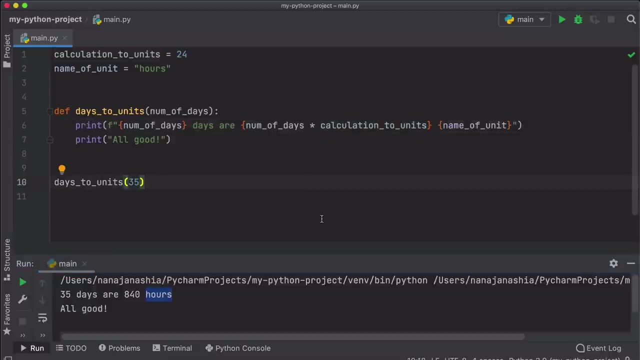 So now, if we execute it, by the way, we can also do it here. You see, thirty five days are and the calculation was done here and hours. And Now, if you go back to our previous example, where we wanted to calculate these for four different values, right, for different number of days, we can actually do the same. 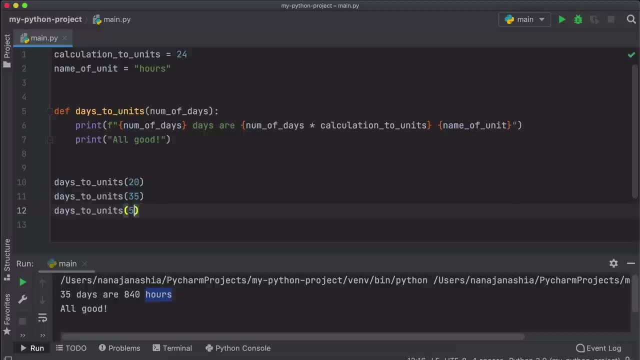 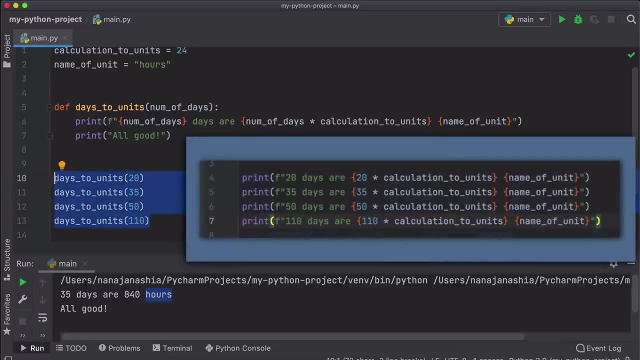 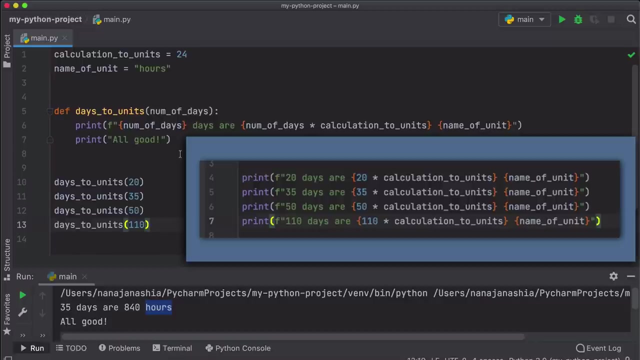 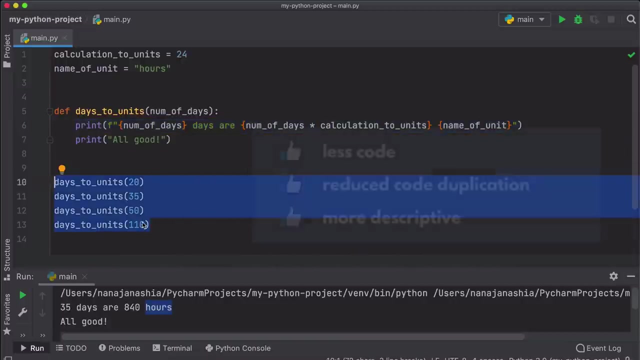 So we had twenty, then we had fifty and we had one hundred and ten, Right. So this basically gives us exactly the same logic that we had previously, but with different syntax, Right? So you see the difference That, instead of having this basically four times, we have much cleaner syntax where we actually see what this logic is doing, which is these two units. 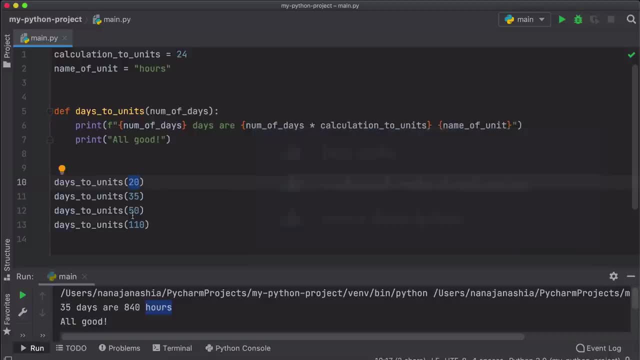 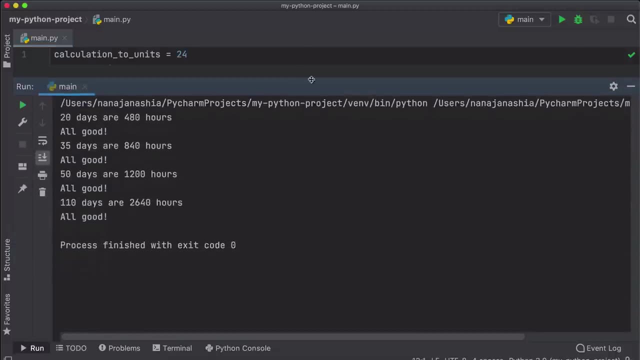 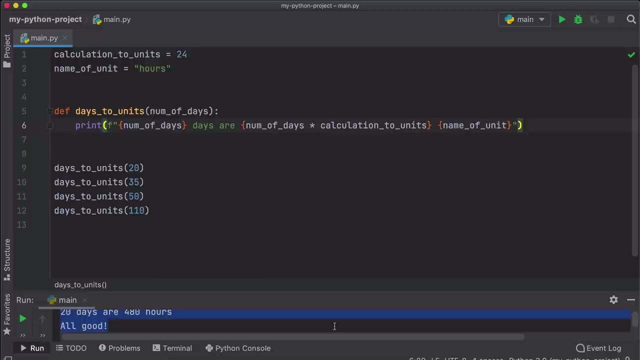 And then we have the number of days that we pass or give our function as parameter. And if I execute this, you see that it was printed four times for all different values. We can actually remove this line: Right, Right, Right. And now if we make some change in our function, for example, we change the name of this variable. 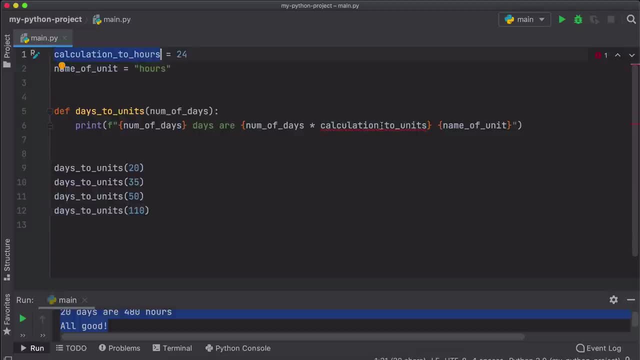 We want it to be hours instead of units. We just do it once in one place And that's basically it. So whatever changes we make inside that function- and that is actually the big advantage of using functions in code- whatever change we make inside, here it doesn't. 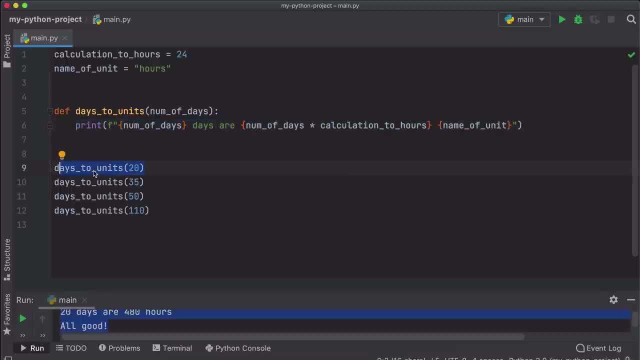 affect how we use the function, because for using the function we only need the name of that function and the input parameter. Now probably you're wondering what happens if I do not give my function a value. Let's delete those lines and let's say we do not provide any value here and we try to execute or call our function without the parameter and let's execute. 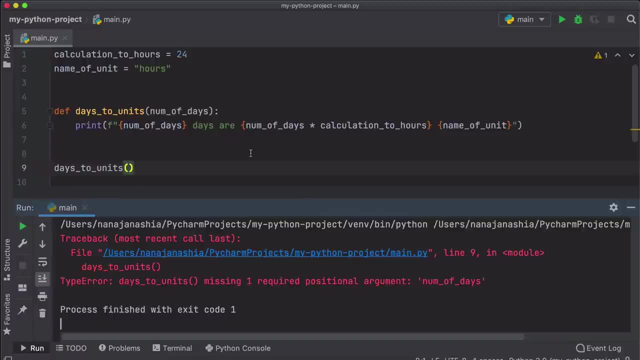 And you see that That's Python interpreter is complaining because we have told Python, here is a function called these two units And whenever I want to use that or my colleague another programmer wants to use that function, they have to provide an input value here. 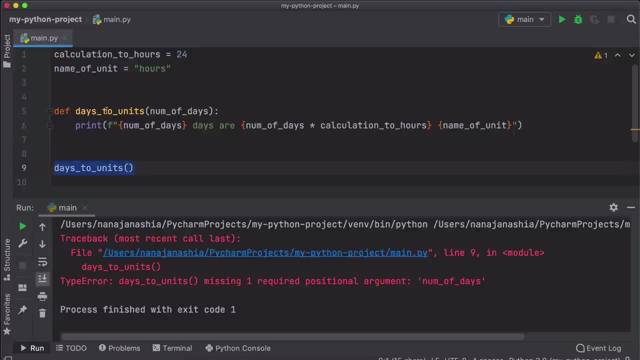 Right. So now, whenever Python sees the usage of that function and there is no input parameter that we are giving that function, it cannot execute that function. Right, Because basically this value is missing here, Right, And that's why we get an error which also says missing one required argument. 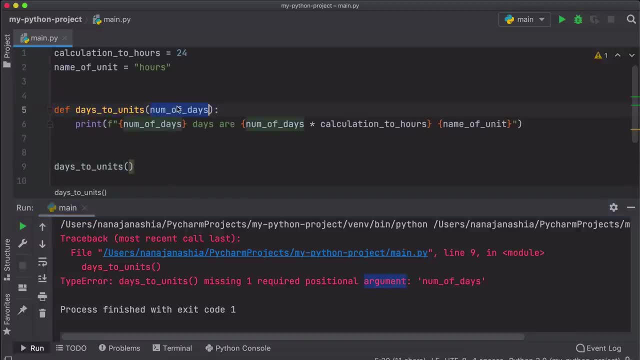 So, as you see, whenever we define a function with a parameter with input parameter, we have to also provide that input parameter. Another thing that you may be also wondering is what if I want to provide multiple input parameters to functions, How do I do that? 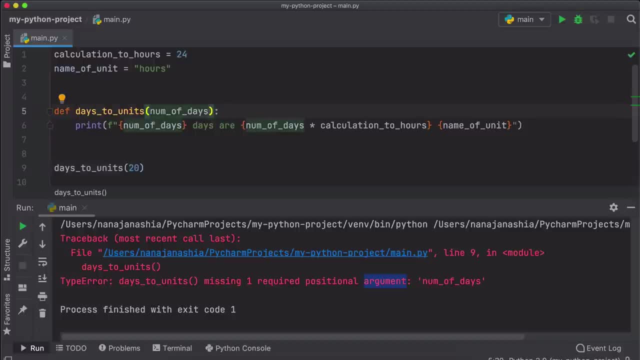 It's actually very simple. You can do that by simply defining here and other input parameter separated by comma, And let's say, we want to pass here something that we want to print out additionally like a custom message, as a real matter, And the same way, exactly the same way as the first one, we can actually use it in here. 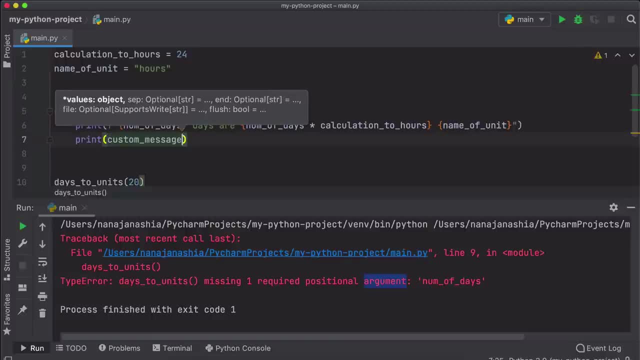 We can even create a new line and basically just print out that message, Right, And know that if you are Using a variable without stream- So basically it's just the variable itself- We're not using any text. in that case, You don't need this format. 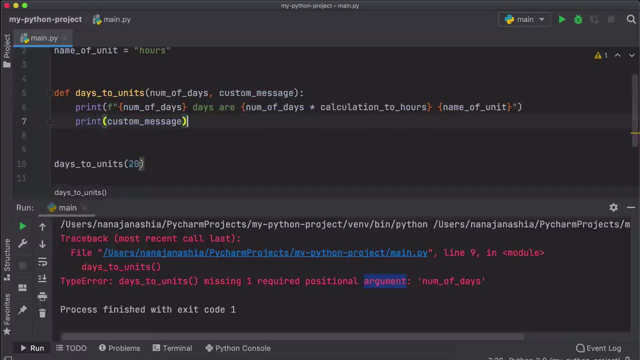 Right, So you can basically just print it out directly. And now again, we have told Python: I have this function and two input parameters are required, So I also need to pass to input values whenever I use that function. So now let me just 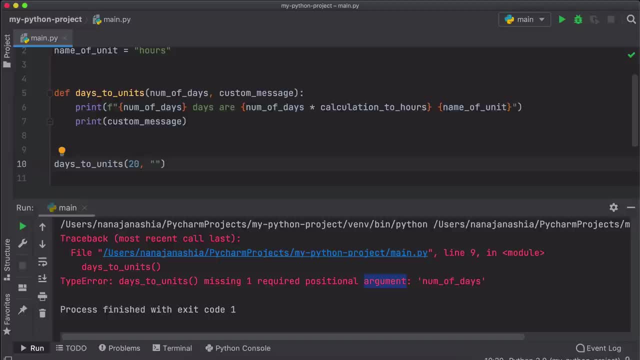 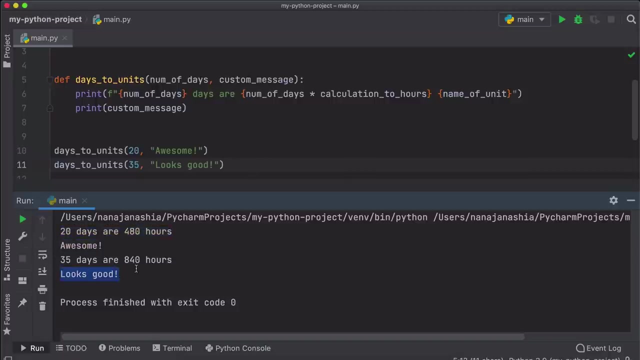 Pass in some custom message that say I'm happy about the calculation or I know I'm going to be happy, So let's say awesome. and let's do another calculation and this time I say looks good. And if I execute it you see that I get awesome the first time, and then 435, I get looks good. 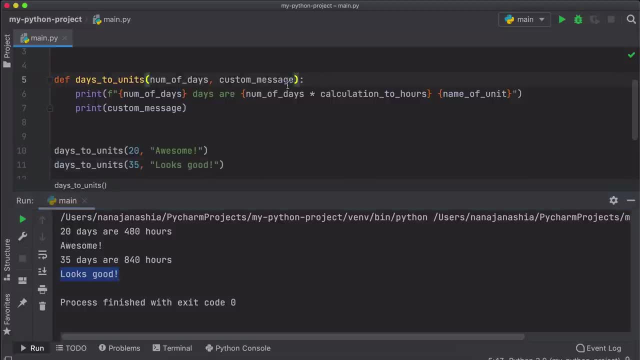 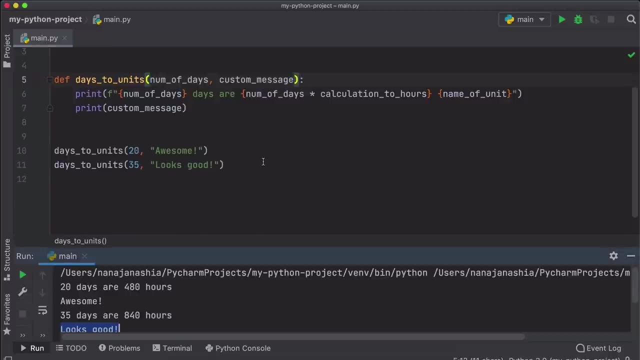 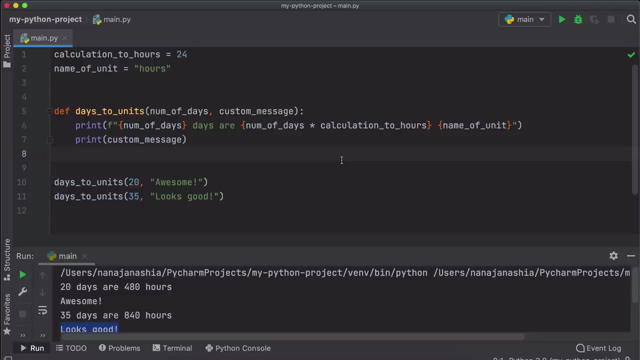 So you can basically define and provide as many input parameters as you want, Right, Right, Right, Common practice and also what you will see in just normal code basically is just a handful of input parameters, maybe one or two, So it's not actually overloaded with ten parameters. 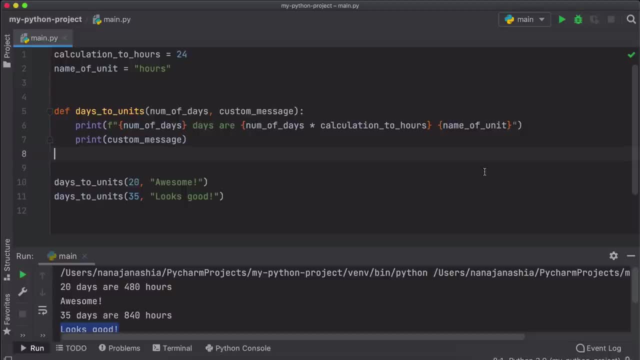 Cool, Now that we know functions and variables, why they're used, or why are they useful and how we use them. There is one point that I want to mention, Which is variable scopes in functions. What does it mean? As I mentioned previously, in this function we're using multiple variables, right? 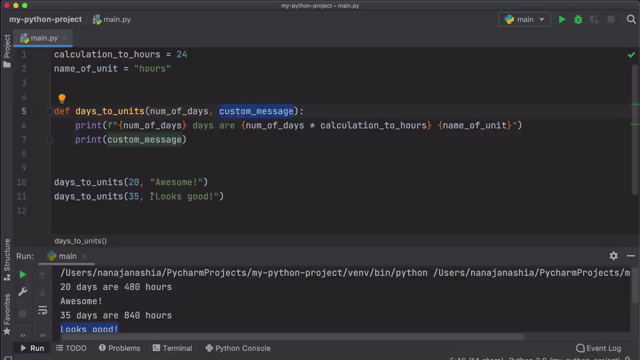 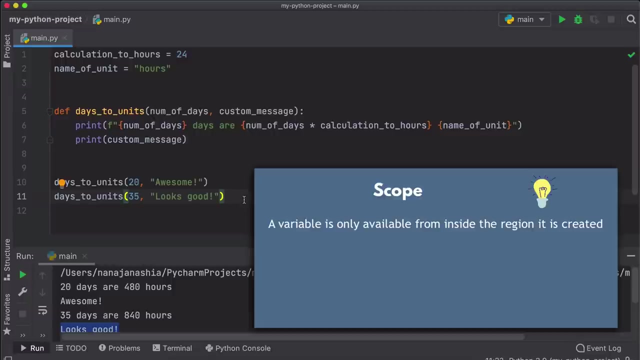 We're using two variables that are part of the input right That we provide when using the function and we're using two variables that are defined outside the function right Somewhere else in the code. So variable scope basically means where is the variable that function uses. 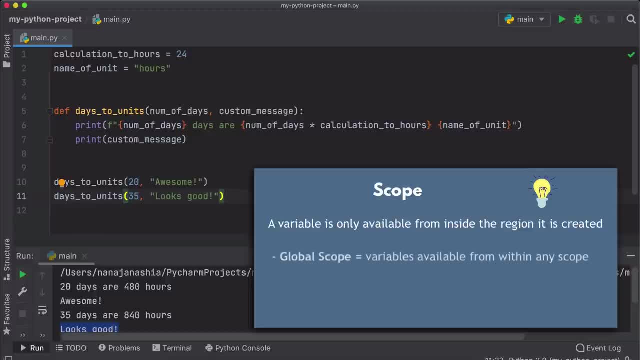 Defined and variable has a global scope for a function If it is defined outside the function, like these two variables right here, could be completely in a different file, not even the same file where the function is. So these are global variables, So all the functions that you have in your Python code can use those global variables. 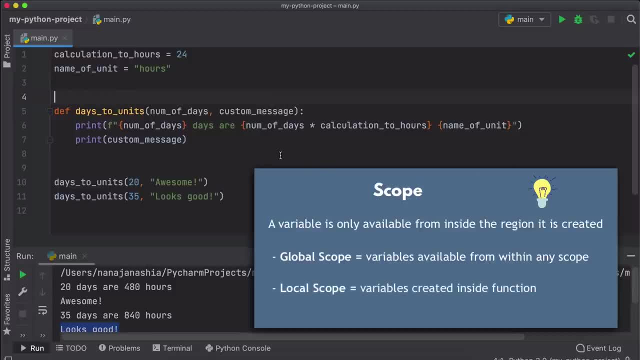 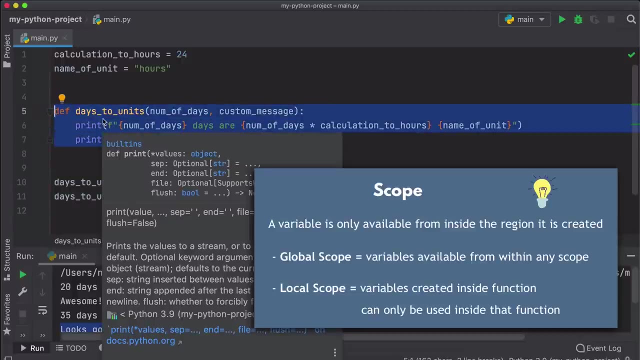 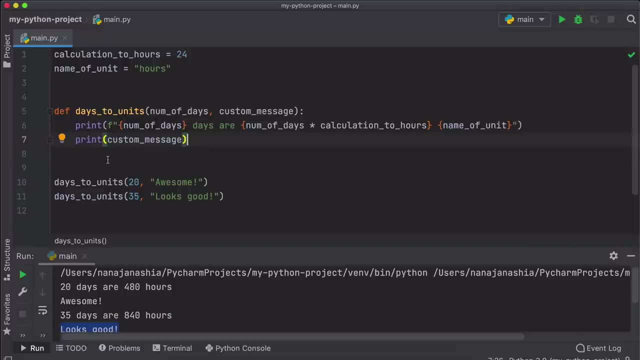 And then you have local variables. local variables are variables that are created within that Function, right? So these two variables are basically only available inside that function because it was created within the function. So internal scope and global scope. So that means that when we create another function, 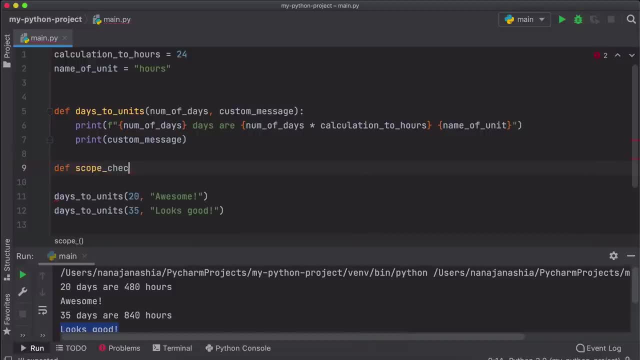 let's call it scope check, because that's what we're going to do. We want to test the scope In This function. I can access the global variables like name of units, but I cannot access the internal variables like number of days. 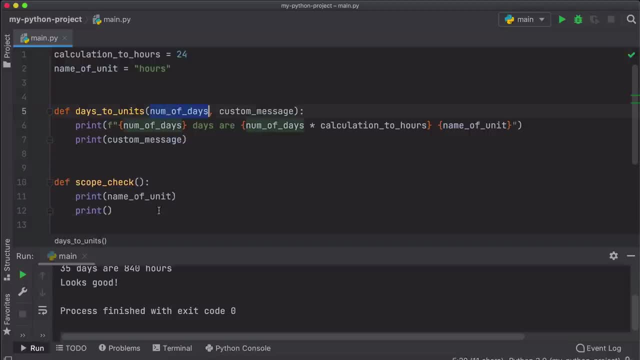 And let's actually test that. So I have none of units, which is a global variable defined here outside the function, And the second one I have a variable that is defined Inside another function, right? So, as I said, internal and, as you see, right here. 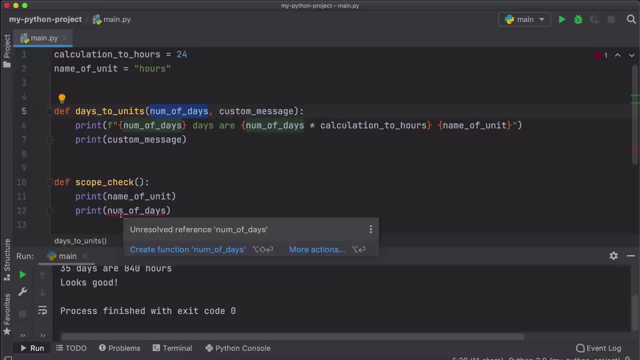 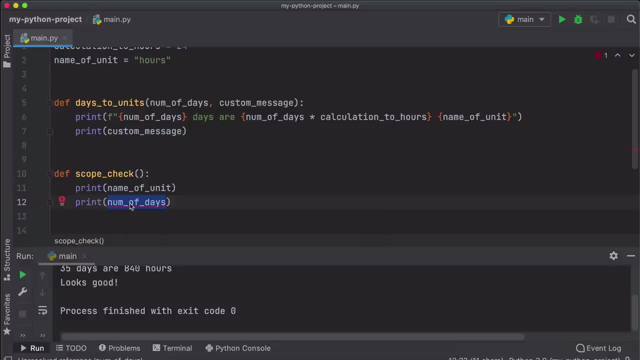 we're ready to get a red line underneath that says unresolved reference none of days. So for this function, basically, that variable is not visible, It's not accessible, It doesn't exist basically at all, And we can even test it out actually. 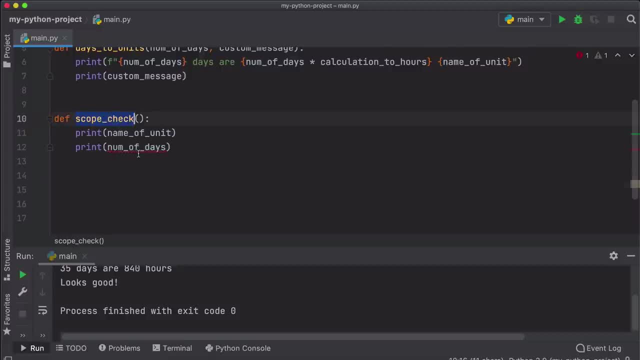 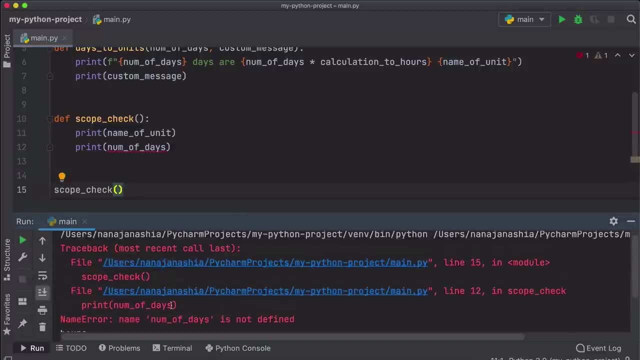 So, again, if we want to see the results, we have to actually use it. Use that function like this, run the function And if I execute it, you see that we get an error that says name: None of days is not defined. 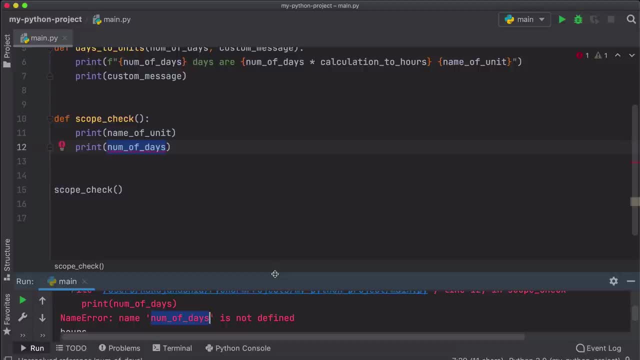 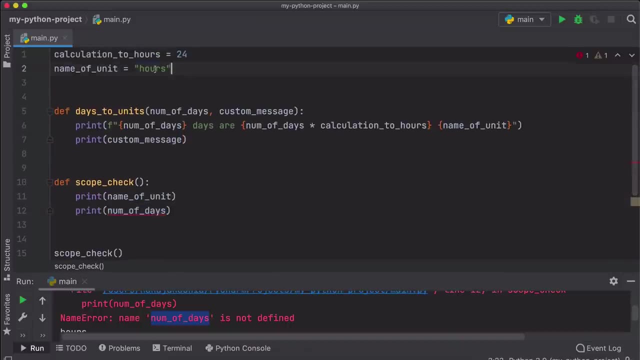 and it doesn't know that there is a function like that anywhere in code. However, it does recognize the global variable And that means that variables defined outside function itself- Global variables- are accessible to all the functions, And if you have variables defined, 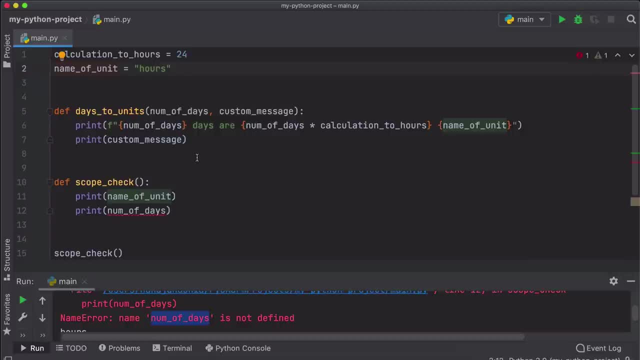 inside the function, then they're only accessible for that specific function and not for other ones. And that means actually that if none of days variable does not exist for scope check variable, we can actually create a variable inside scope check with the same name and we would have basically no problem at all. 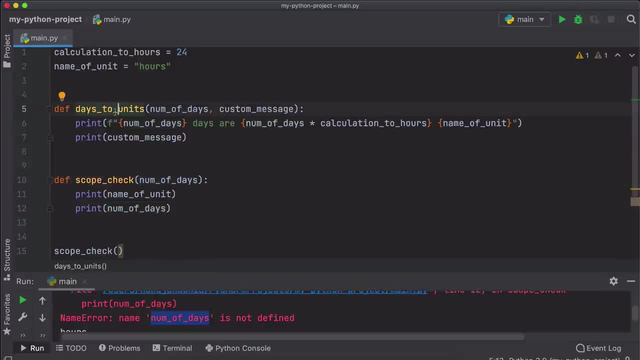 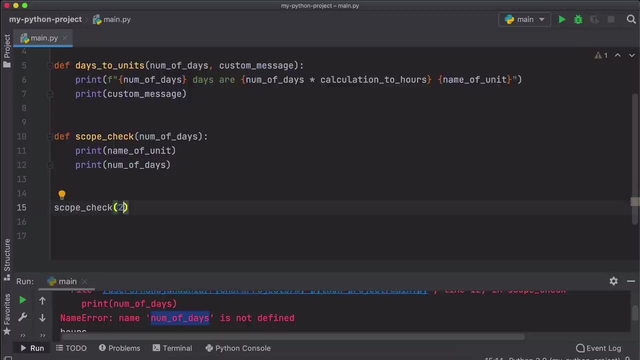 So this is not going to be a duplicate, because this function doesn't know about this variable The number of days here, And scope check doesn't know anything about variable number of days right here, And if we want to use that function now, we have to provide the value. 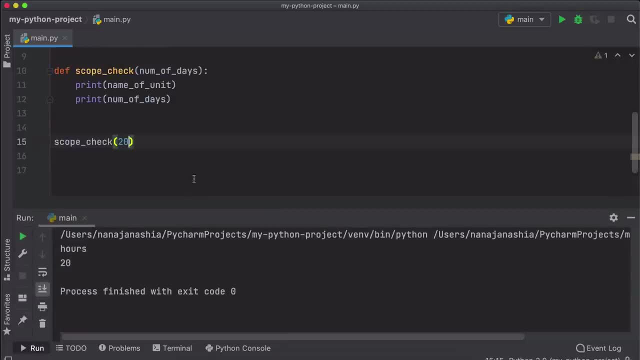 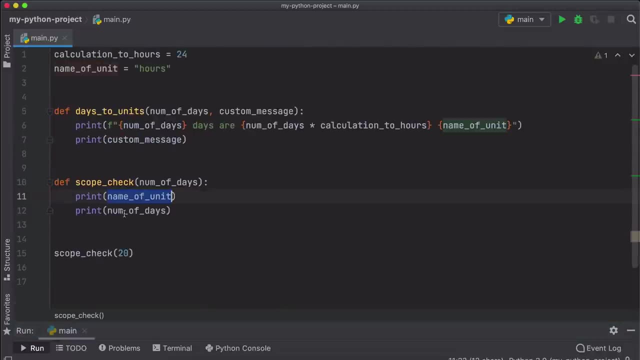 Let's do 20. And if I execute, there you go, you have name of units and the 20 that we provided. So global variable, local variable defined here. Another interesting thing is that, as I said, inside the function, 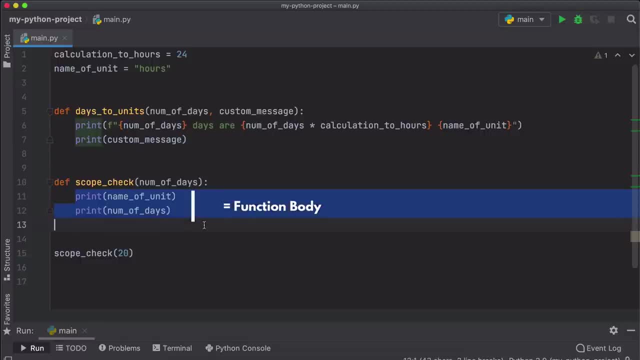 body sort of say. so this is basically whatever is part of the function right in this indentation is called function body. So we can create whatever logic we want inside that function body. So whatever I can do in Python generally, I can do inside the function body. 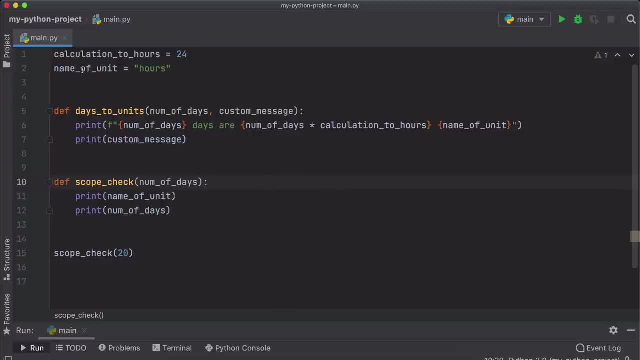 So one of those things is actually creating variables. right? Just like we created variables here, we can create variables here Like this: let's call it my variable and variable inside function, and we can print that out as well. So now we have three types of variables that we are using in this function. 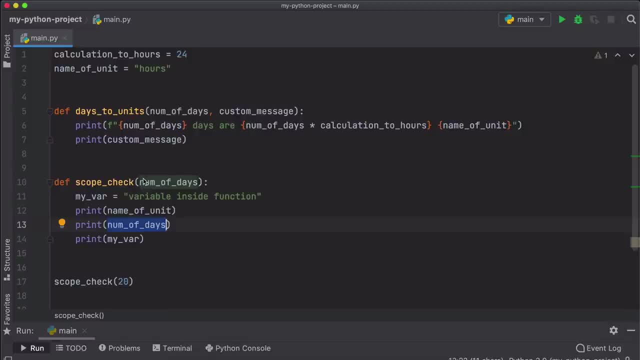 We have a global variable, We have internal variable that is passed in as a parameter and we have internal variable again. That is basically defined. So the variable isn't provided when we use the function, but it's basically just defined inside the variable. 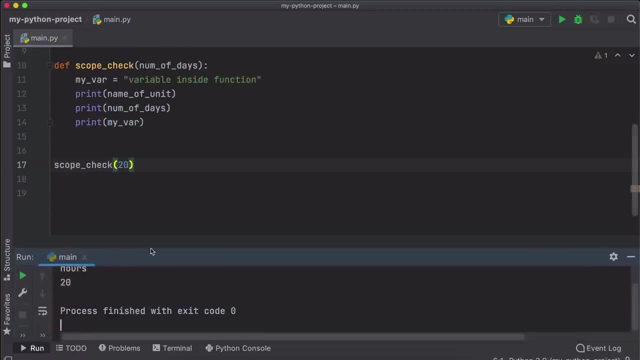 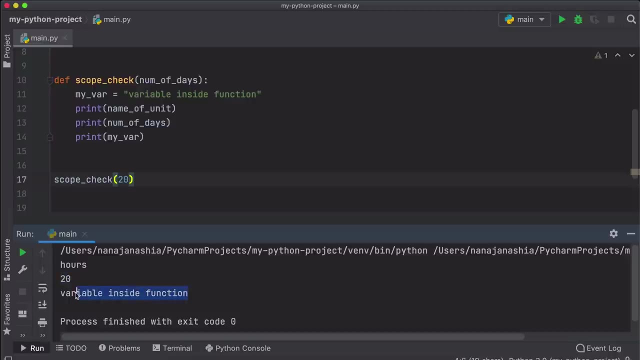 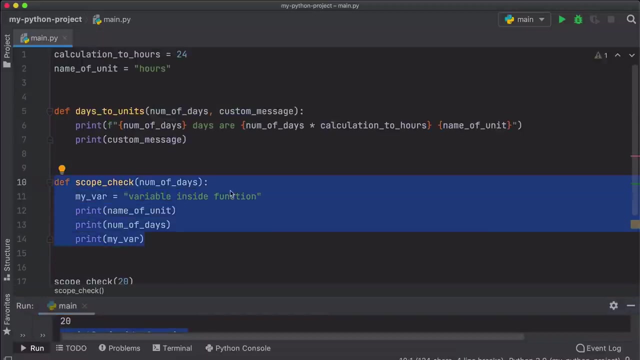 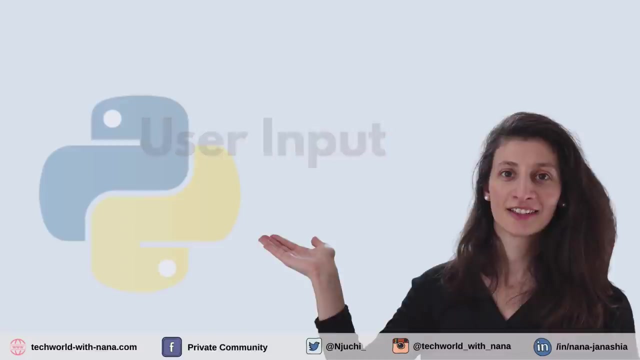 And again, if I execute this, see hours now updates and variable inside function text printed out like this: And obviously this is just for demonstration, but we're going to see more realistic examples of that In our projects. So I'm going to clean this up and we can move on to the next concept. 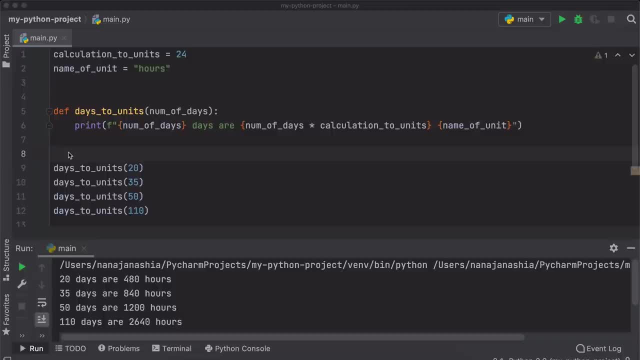 So now let's go back to the example where we calculate number of hours and we do that for four different values. Now, if you want this application to be really useful for us or somebody else, it doesn't help that we have to fixate here. 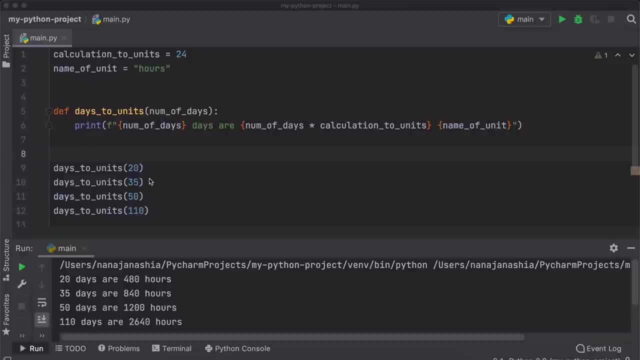 Just four different values, right? Right, The application should be able to take any value that we basically feed it, Right? So we should be able to provide any number of days and the program should calculate the number of hours in those days. So what we need here is user input. 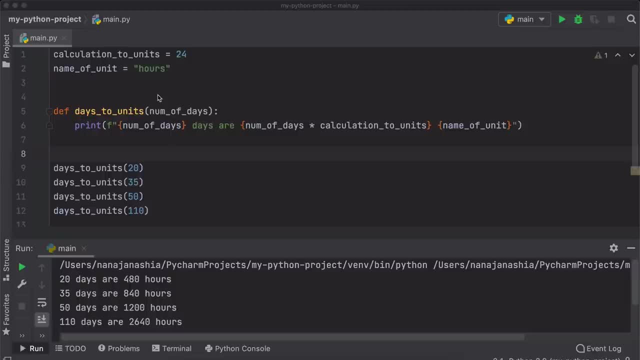 So when we give this application program to somebody else or use it ourself, it should allow some user input. So how do we write a program that asks for and accept User input and then does something- some kind of calculations, some kind of other logic- based on that user input? 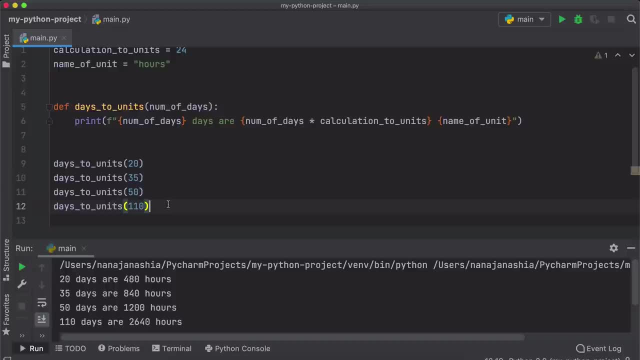 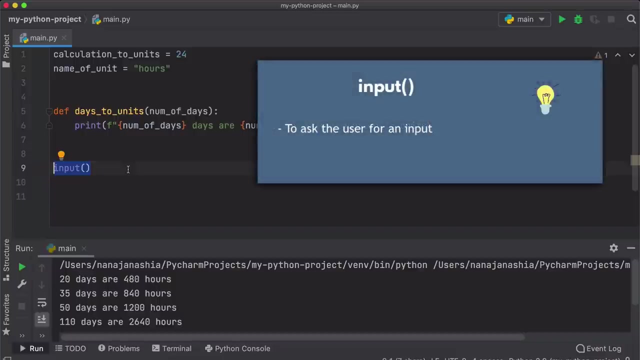 accepting a user input from a Python application is actually pretty easy. Let's get rid of all of these lines first, and we can do that by writing inputs, And this will basically give a user a prompt to enter some input value. Now you probably already see from the syntax that this looks very much like using our days to units function. 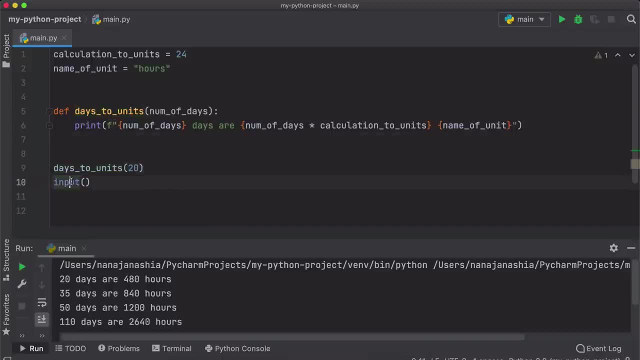 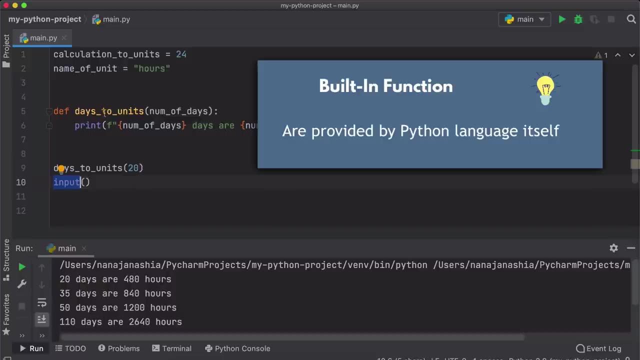 Right, In this case with the parameter. So input is actually a function that Python provides us with. So we didn't have to write this input function. Right, We wrote the days to units function, but input function is available in Python so that we can use it whenever we want. 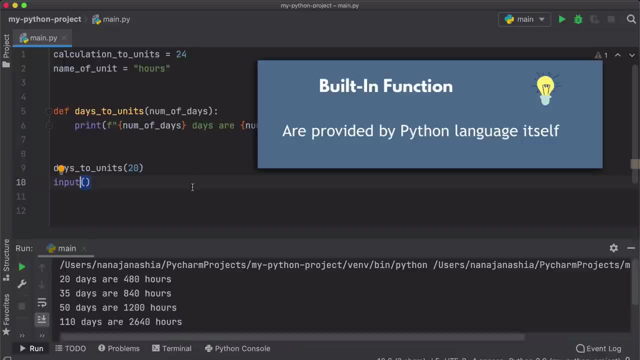 And this parenthesis here tells Python we want to call an input function and we're calling it or using a function without a parameter. So now we know that we can write functions ourselves for logic that we need, But Python has tons of functions that Python developers already wrote and it's part of Python and we can use it in our code. 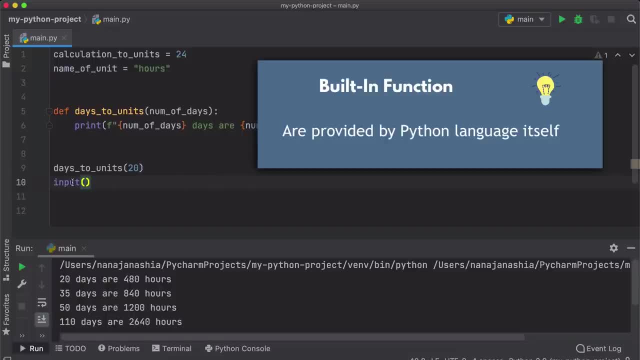 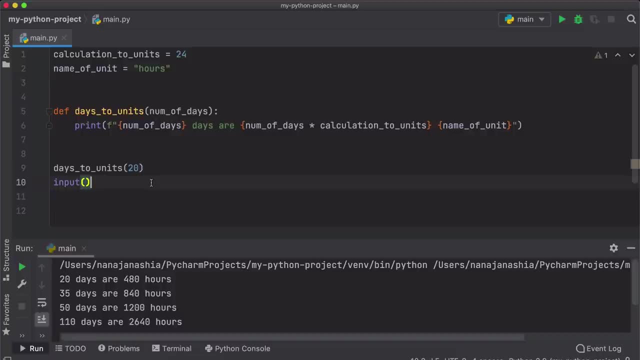 So they're not. everybody has to write their own inputs So we can write our own input. function logic and the code or the functions that Python provides are again part of this Python that we use in a project And, obviously, if you're using the latest version of Python, 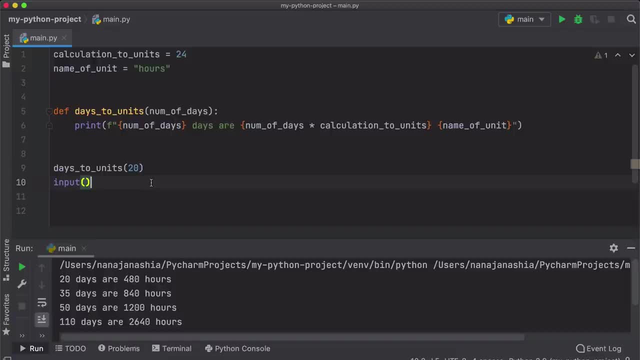 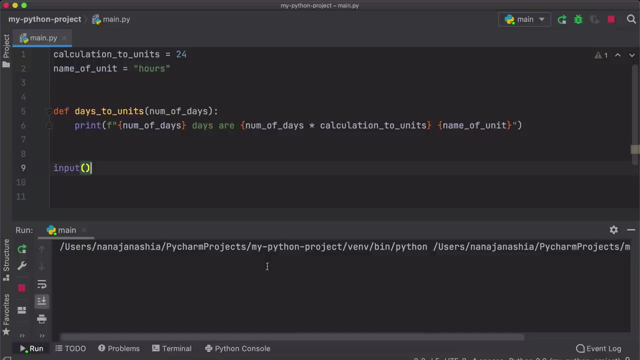 you will get the latest code and latest functions that Python basically provides. So back to our function execution and let's see what happens when we execute this Program. I'm going to run it and in the outputs you actually do not see anything other than my cursor is blinking here. 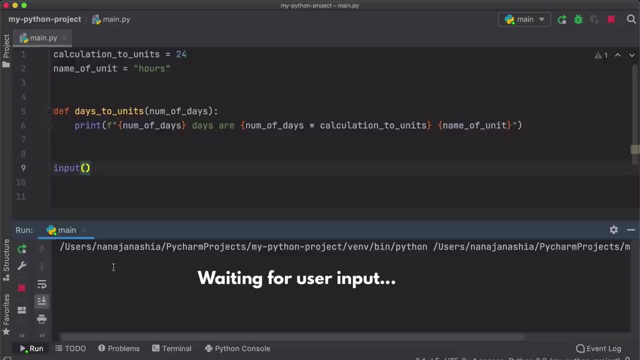 So it's actually waiting for user input. so I can actually type in something here. so I can do 20 and enter and process finished with exit code. So I was able to input something. doesn't really matter, It could also be a string. actually doesn't really matter. 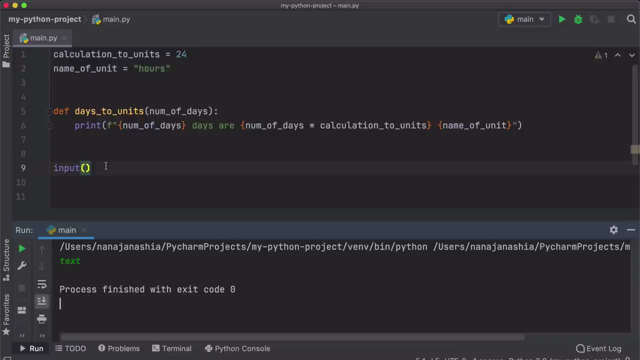 And program basically finishes. So that's the simplest usage of input. However, as you noticed here, running this program and basically having this blank output here is a little bit confusing. So if another user is using our program, they will probably be wondering what's happening here. 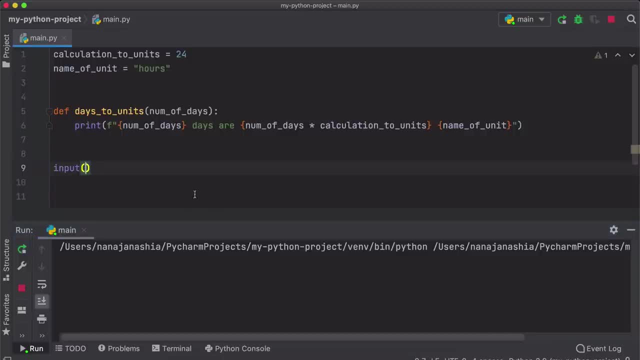 So what we can do is, in inputs function, we can provide a parameter that actually tells a user Something like enter a value for number of days, or something similar, so that it's not just a blank prompt. Right, So we can do that by passing in a parameter. 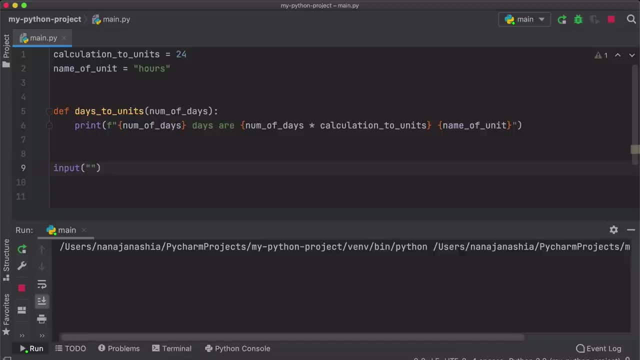 a string which is going to be our message. So we can do a user enter a number of days and I will convert it to hours. And here you see right now that the program wasn't finished because we didn't enter anything. So this program finished line wasn't output yet. 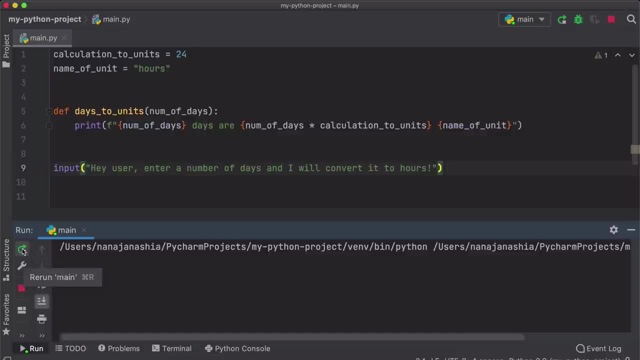 And that means the program is still running. It is still waiting for our input And in PyCharm, in this idea, if you want to terminate the program manually yourself, you can click this stop button And, as you see, process finished. 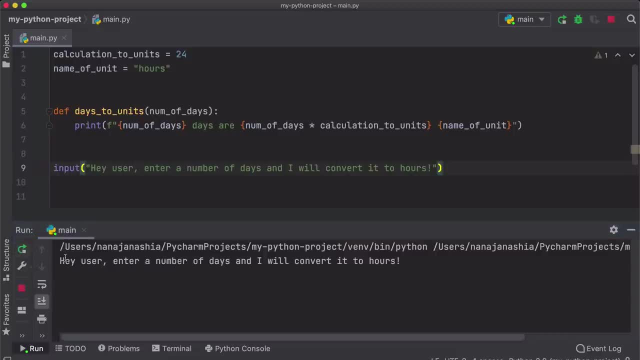 So now we can run the program again And, as you see, here we already have a message that we're displaying to the user so that they can enter the hours Right, And here we can provide our inputs 30. And there you go. 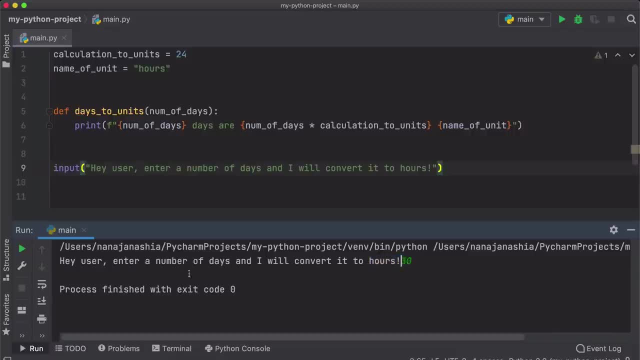 However, this doesn't look nice here. We actually want the user to get a prompt on the next line. How do we do that? As part of a string we can actually add a new line or new line character, basically, And that in programming is actually represented by backslash in and you see a special highlighting for that one. 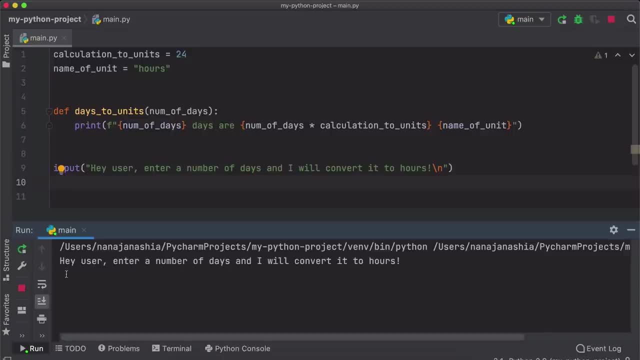 Let's execute- and you see that my cursor is on the next line. now And again, let's provide a value, enter and program ended. So we have now a more user friendly way of asking Program user for the input, instead of just showing an empty prompt, and we're getting user input. 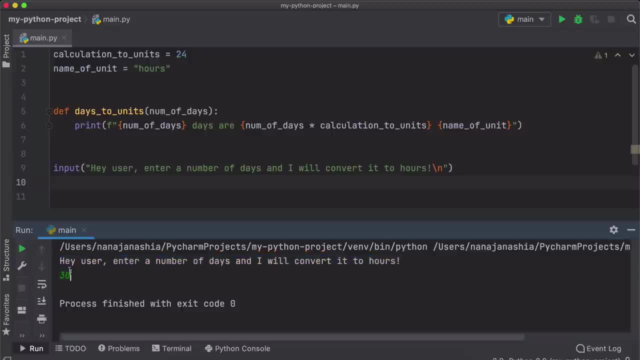 Now we're not doing anything with that user input, right? That input basically just finishes the program and that's it. We're not doing any calculation for that input. So how do we use the value that user enters here when input function gets executed? 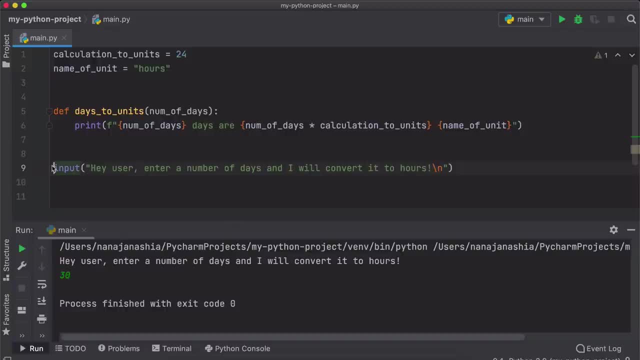 We do that- And this is a very important concept- by Assigning whatever result this function usage gives us, which is, in this case, user input, assigning that result to a variable. So right now it's basically executed and it's just wasted, right. 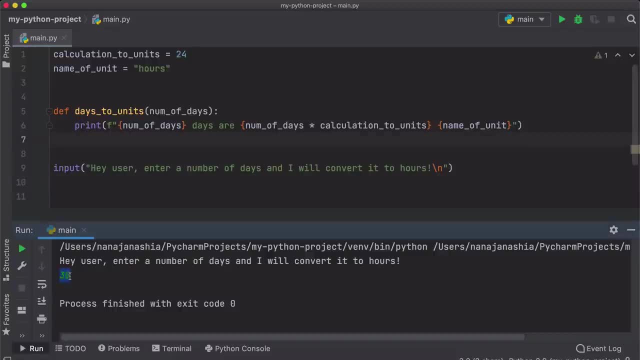 It just disappears. So instead we want to save that value, that entered input value, in a variable so that we can access it later. And we do that by, let's call it, user input variable Equals. So just like we created variables here with variable name and a value, 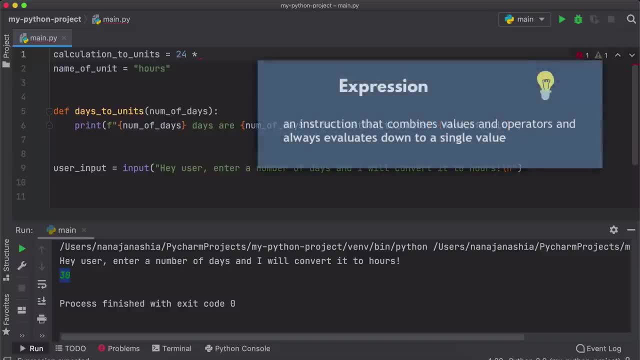 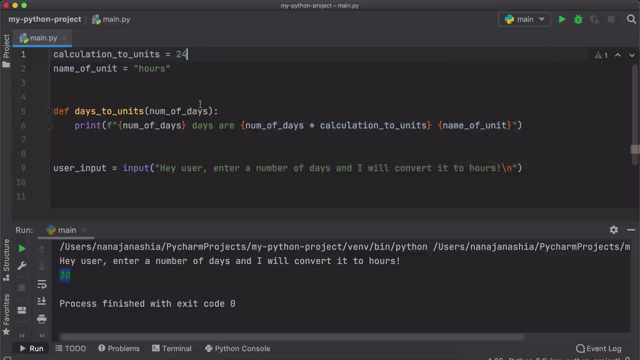 right, Or even an expression right. If we did a calculation here, that will be basically a whole expression, whole calculation. the same way, We can use values that function execution gives us to assign it to a variable. So now what I'm going to do is I'm just going to print the user input so that we can. 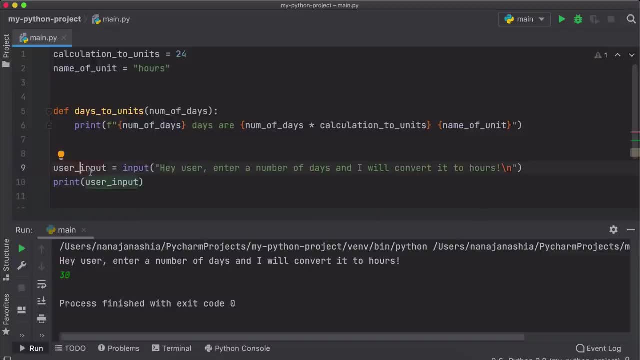 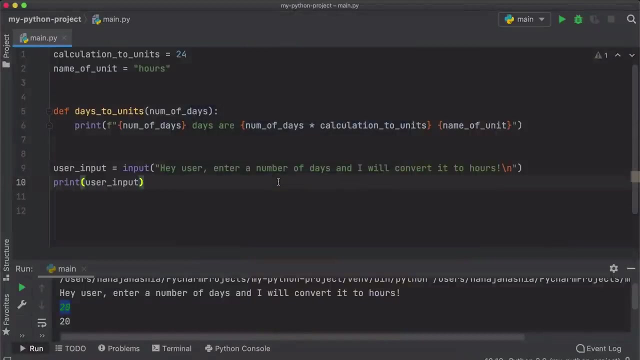 And see what value that user input variable has. So let's execute again. It asks for our input. Let's put 20 and print: user input gives us 20.. So user input variable value basically becomes whatever we provide as an input. Now that's a new concept and it could be a little bit confusing. 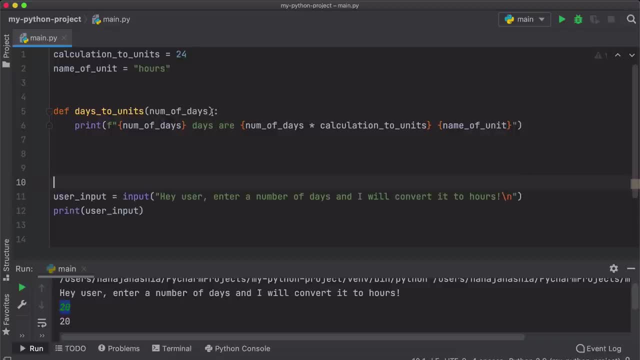 So let's see another example with our own function. What would happen if we assigned value of this to a variable? We get a warning, as you see here in the editor, which is one of the great things about it is that it basically gives you warnings when something is not correct. 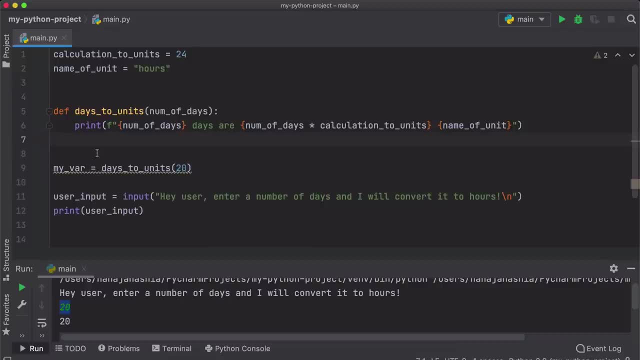 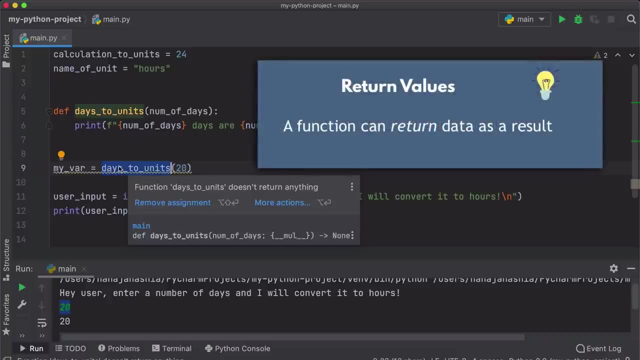 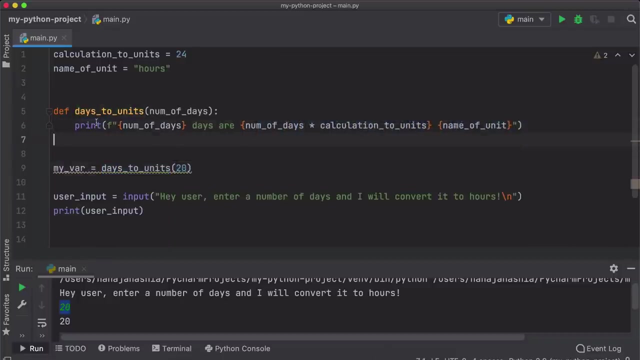 And the warning says: function doesn't return anything. So, basically, if we want to have some value as a result of function execution, we have to return some value in the function and how we do that, Instead of printing the value right away. 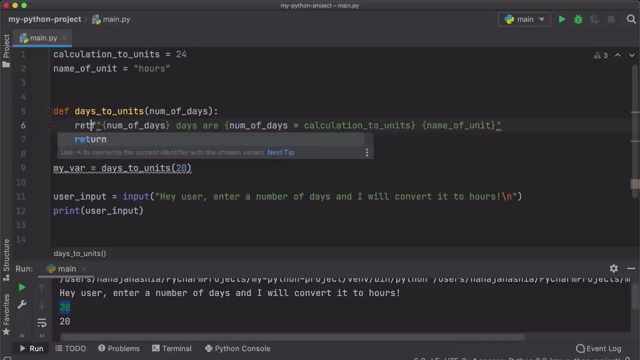 we can actually return that value using return keyword. Again, you see special highlighting here, just like here, because return is a special word that Python understands, that you want to basically give back a value, This value right here, as a result Of using the function. 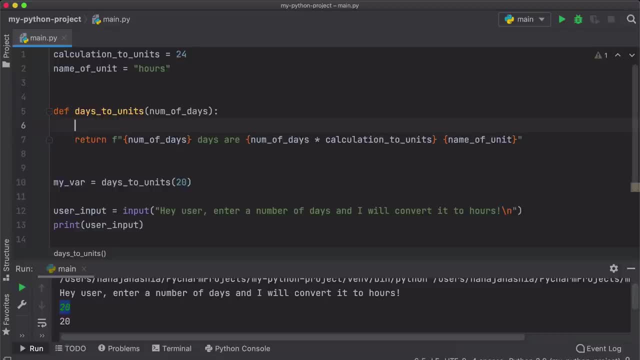 right, So you could have some logic here during the calculation, whatever, And then as the last line you can return that calculated value. And now the warning is gone, because we're actually returning something from the function. And when we return value from a function again, 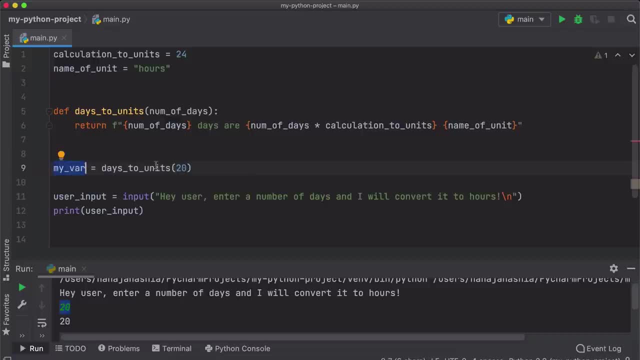 we can assign it to a variable so that we can use that value, whatever function return by referencing the variable, And one of that usages will be basically just to print it, just like we did before. like this: Let's delete it temporarily and test our program. 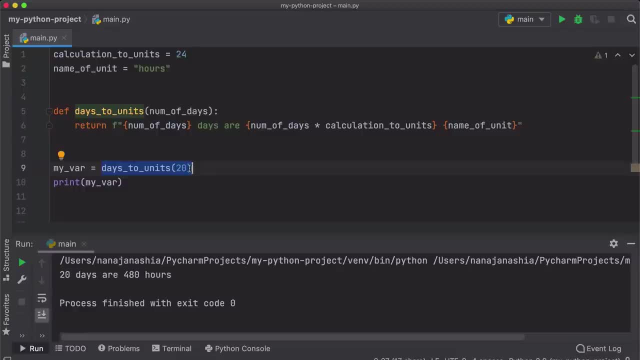 And there you go. You see that this function got executed with input 20.. This text, this display text basically, was put together in the function and was returned or was given back as a result, And we saved that, this whole string, basically, this whole sentence, in a variable called my bar. 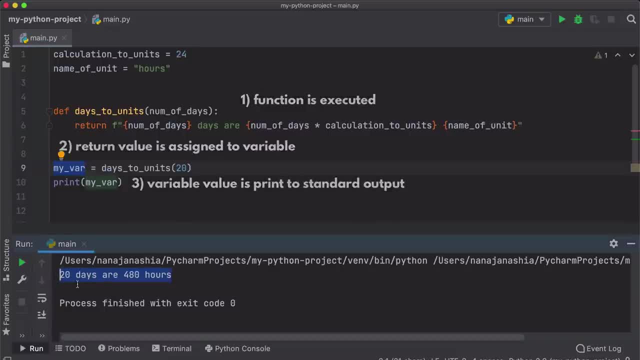 And when we print that my bar, we see that value printed out here And again, if we enter some other value, we would get different text And again, that is actually very important. concept of giving back some results from a function execution. 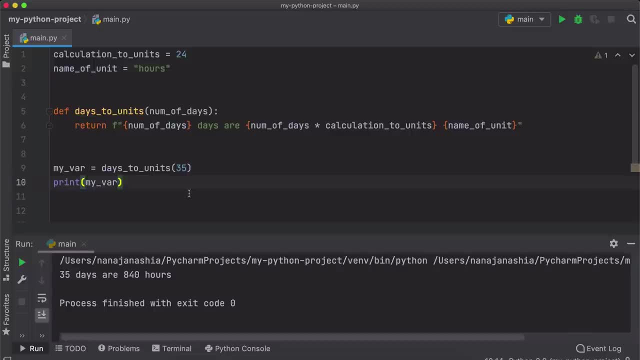 And you saw in our examples that you can have a function that doesn't return a value- just print something on, maybe does something else, or function that returns some value. You can have both types. So back to our example of user input. 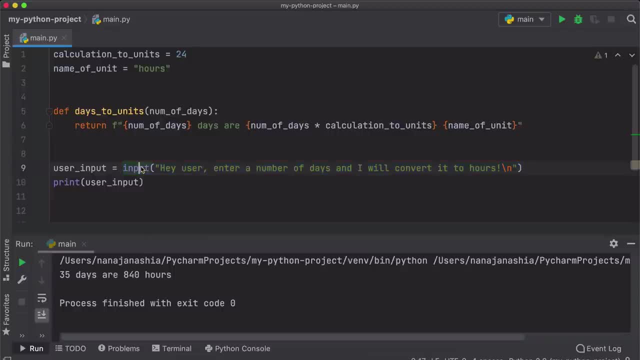 So now, hopefully, it makes sense that input function returns whatever value that user entered as a result and we can save it in a variable. and then X, X, is it later again. let's get rid of this line And now let's actually do the calculation on that user input number of days. 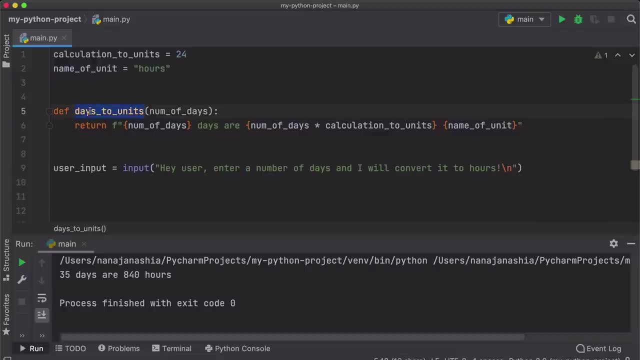 How do we calculate number of days? Very simple, by calling our function that actually does that. So we're going to call our function to calculate the number of hours for an input And the parameter that we pass in is going to be whatever the user provided. 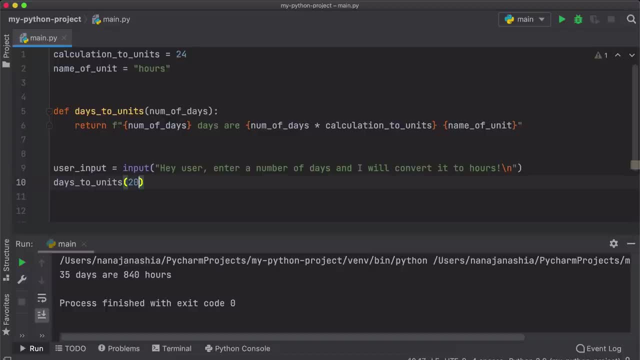 So instead of basically hard coding a value here ourselves, we give it a value that user provided instead. So the number of days will be the user input. And now again, because this function returns the whole string, it doesn't print it. 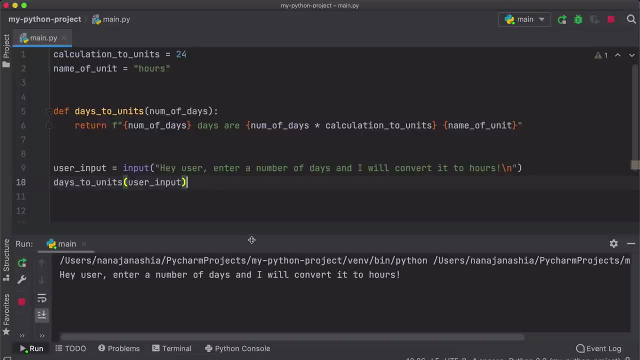 Remember, it just returns it. So when I execute this and I provide in some value, let's do 200.. You see that I don't have any output here because we didn't print anything. We. we basically just returned the value here. 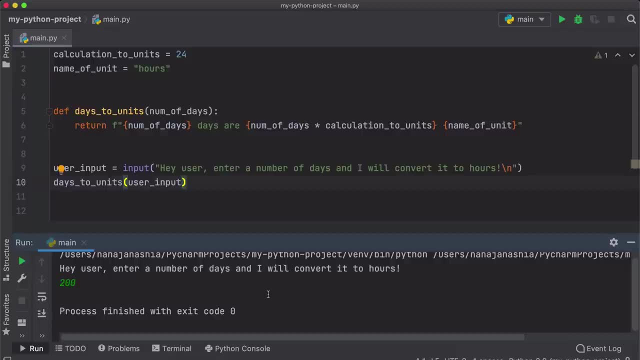 We didn't do anything with it. So the last piece missing here is to display the text, the string that function returns. So we save that return value first. Let's do calculated value. So we save this thing in calculated value variable And finally. 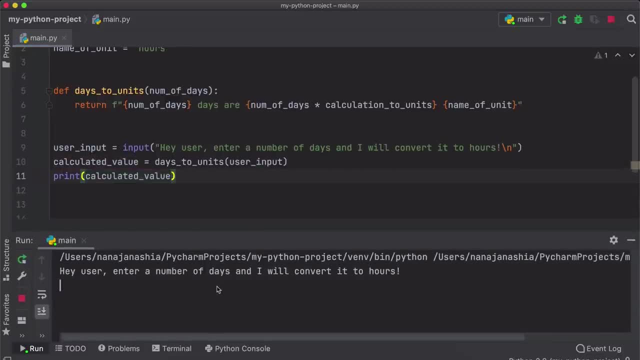 we can print it and I'll. let's execute it and let's see what happens. I'm going to type in 1010 days and let's see what we get now And you see, we have this weird value here as a result of the calculation. 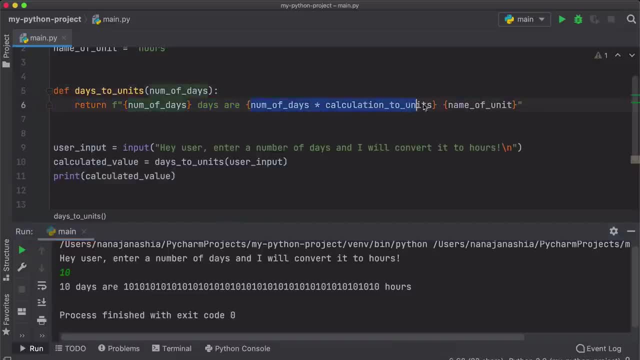 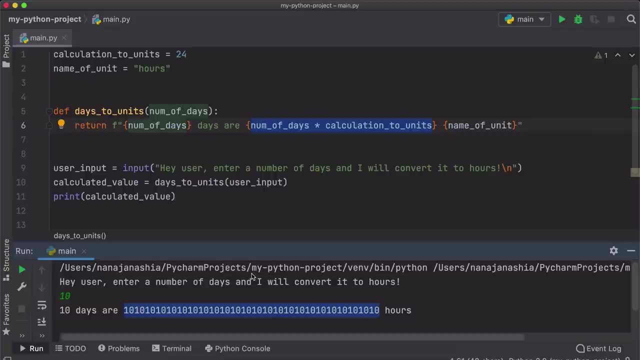 So what exactly happened? So this part of calculation, basically, which represents this number, didn't do a proper calculation, And the reason for that is because the input value that we get with inputs function is always treated As a string and not a number. 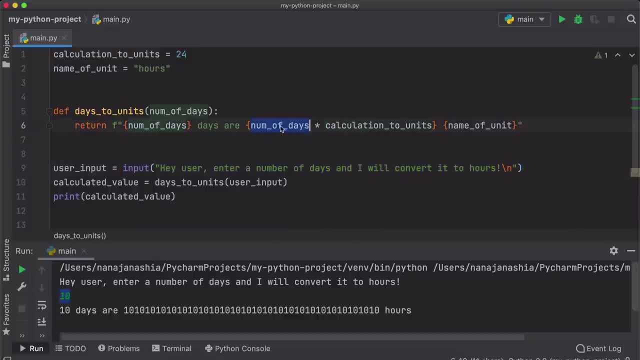 So basically at this place here, number of days inputs to 10 here is actually treated as a text and not a number, and where this weird result comes from is basically number 10 printed out 24 times. So instead of doing the actual calculation, 10 times 2410 is 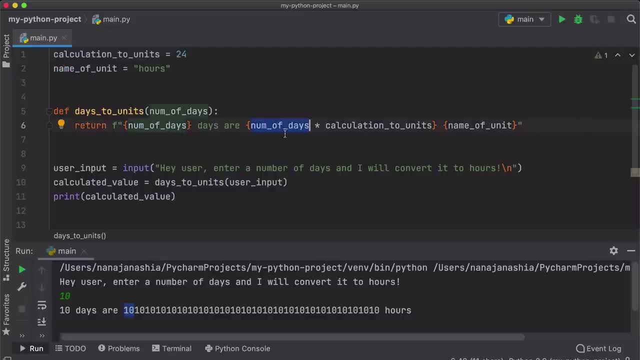 printed 24 times, and that's what happens when this is interpreted as As a string. So how do we make python see that number, see that input value as a number, as an integer and not a text or not as a string? and it's actually pretty easy to do. on the next line, the user. 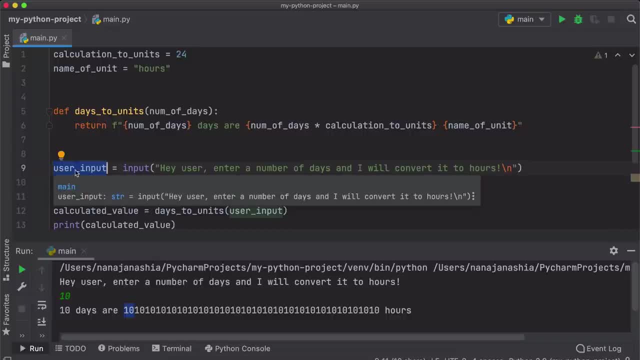 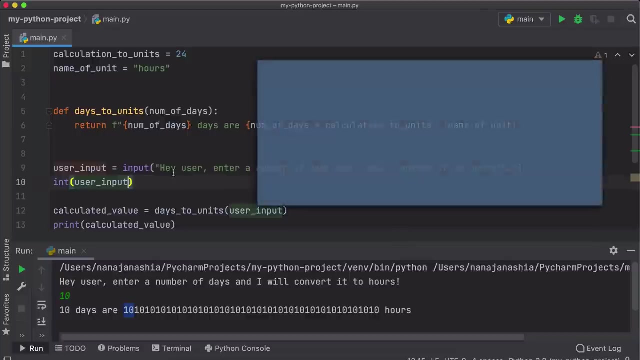 inputs again. We saw right here: It is a string, So we have to make it into a number and we're going to do that using int and user input And And that process of turning a value from one data type into another is called casting. 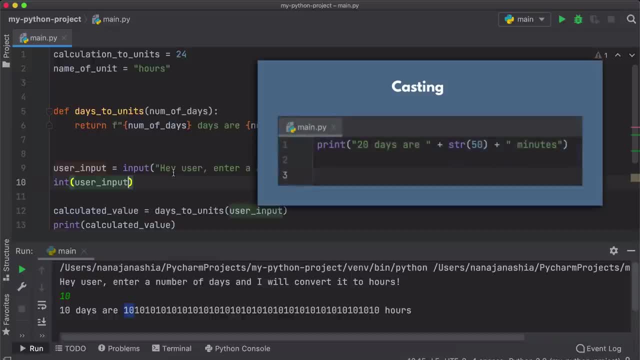 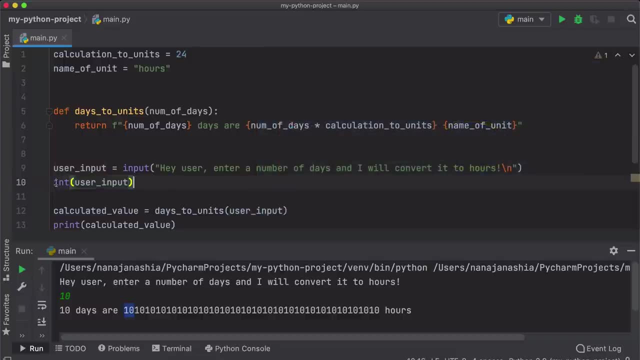 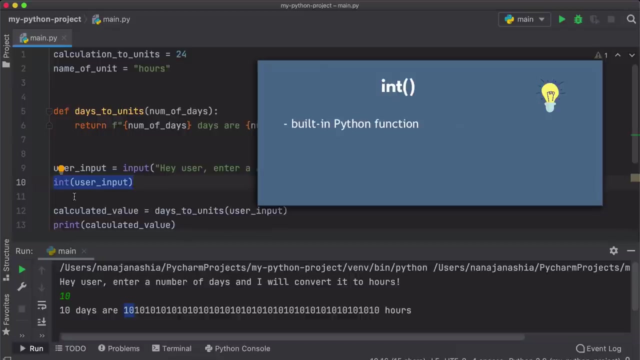 If you remember, we already saw an example of it when we turn a number into a string in the string concatenation. example again from the syntax, You should already know that this is a function call. So we're calling a function called int. again that python itself. 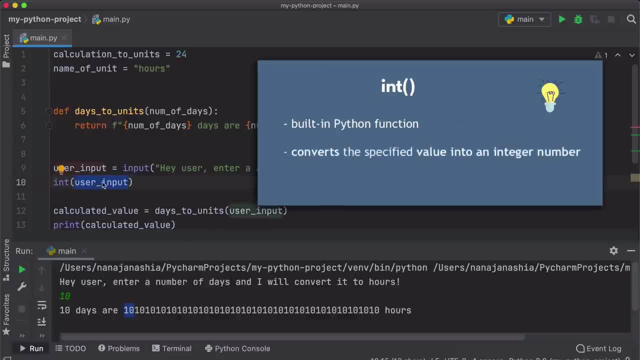 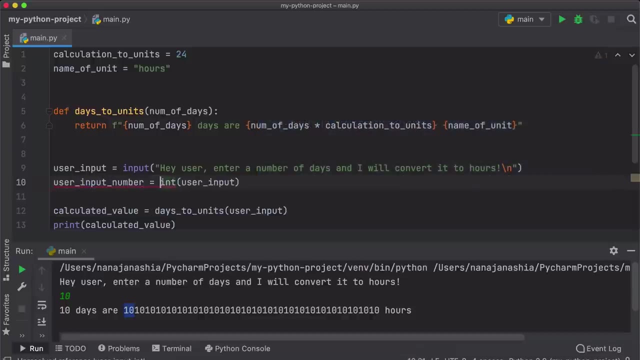 provides us with, because we didn't write that function and we're passing in one parameter which is a string, and we should get an integer from that string as a result, and we can save that number into a variable and let's call it user input number, and now we have 10 as a number instead. 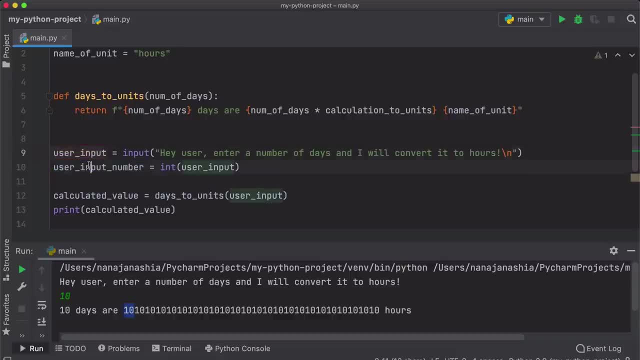 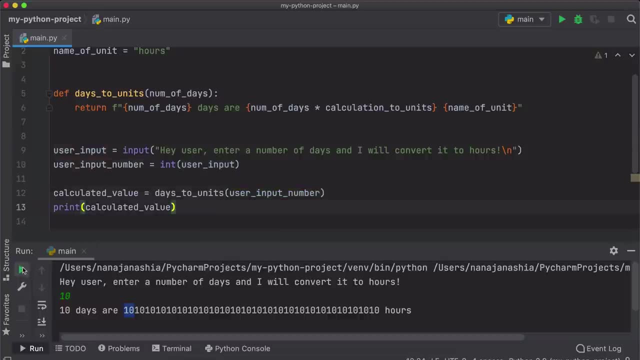 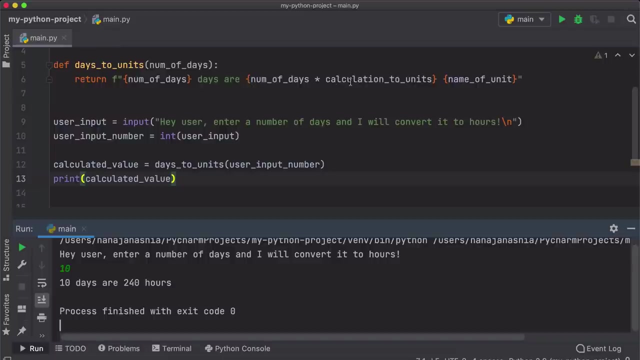 of as a string, and instead of passing in that string user input, we can now give our function number that it expects. Let's save it and execute. Let's put in 10.. And there you go Now. the calculation is correct. What I want to show you now is how this user input actually 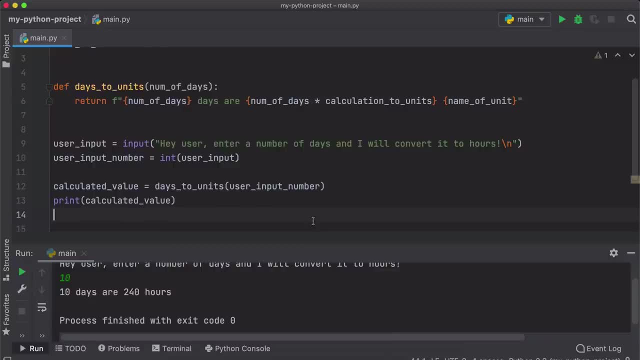 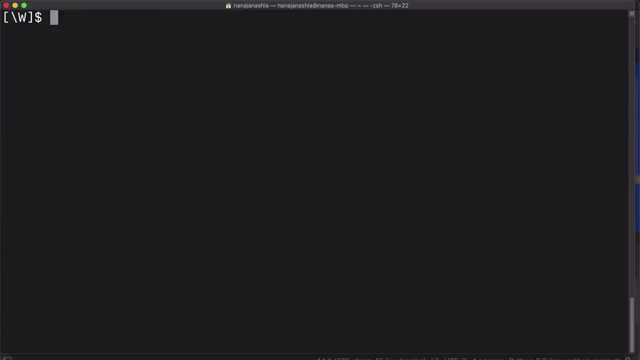 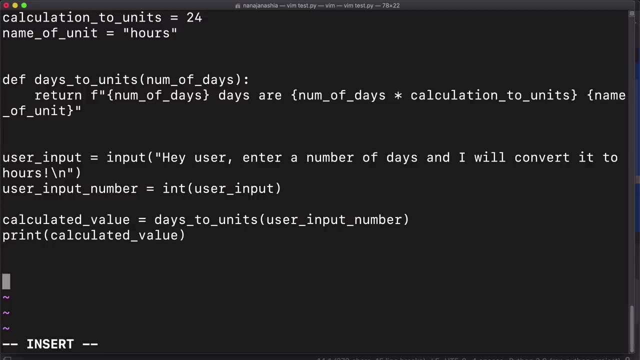 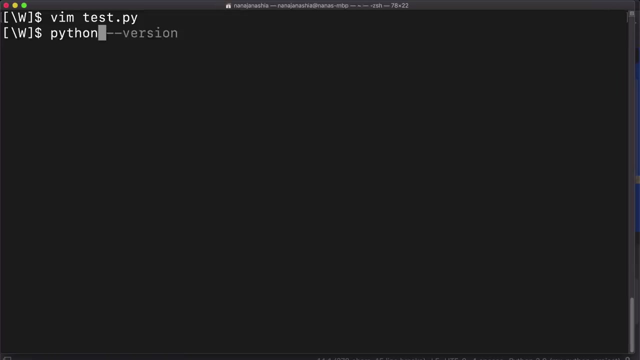 works without a code editor like pie charm. So I'm going to copy all this code and let's go back to our terminal And in our testpi I'm going to paste in our code And save and let's now actually see how the user input works. 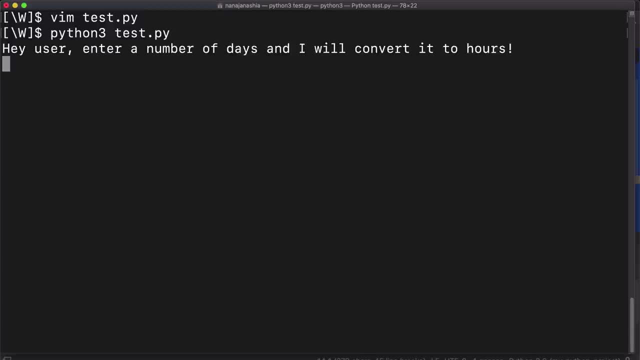 when we executed in a simple terminal window And as you see here we have the message first and the prompt is right here so we can enter a value. Let's do 25, enter and we have a result. 25 days are 600 hours. 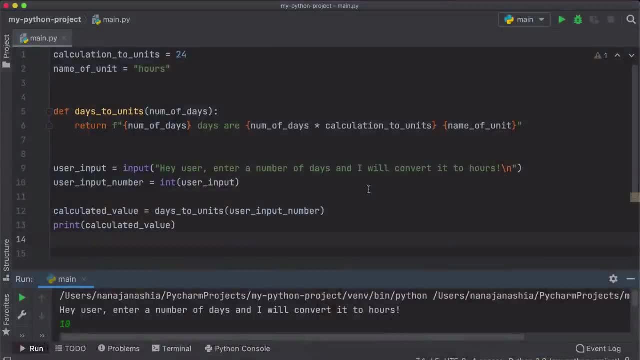 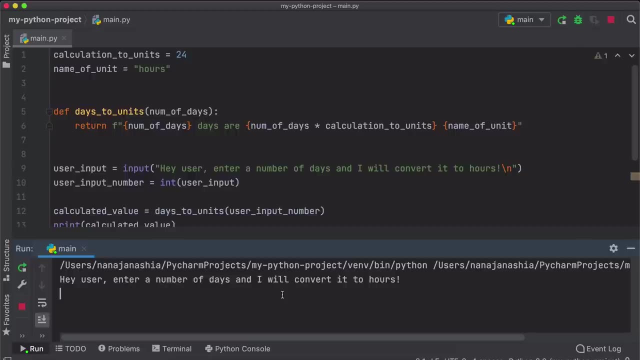 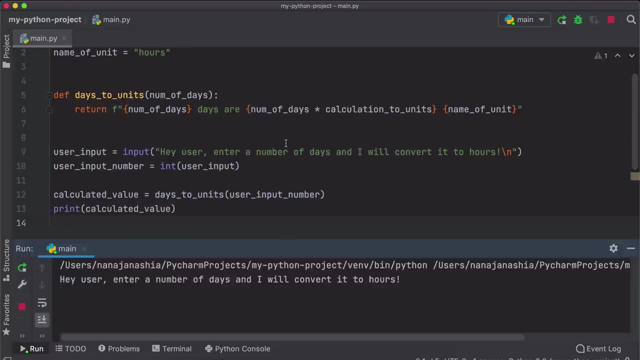 Great. So our program is working. It is converting the number of days to number of hours and accepts a user input. Now what happens if a user enters an invalid value here? So, for example, instead of a positive value for number of days, 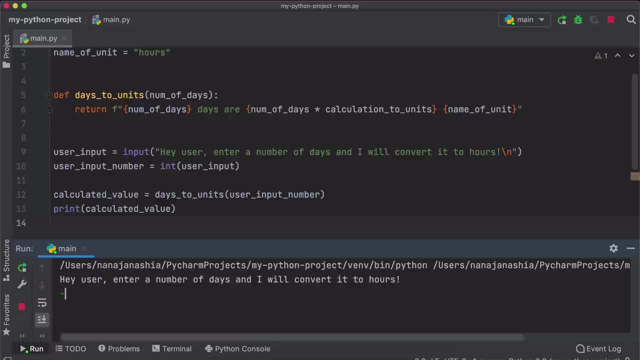 maybe they enter a negative value, like minus 10,, for example, and obviously that input value doesn't make any sense. but we are still calculating and Giving a value right. And this is another important concept in programming generally, that when we allow users to give our program some input value, we also 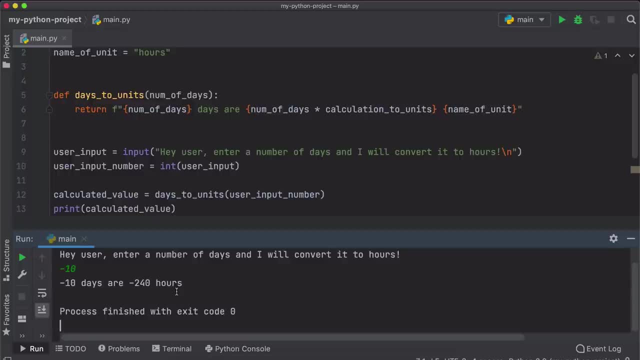 want to restrict them and basically validate that what they provided as input is a valid value for our program, specifically one that it makes sense, like in our case, minus 10 program still does the calculation but doesn't really Make sense. and second, it doesn't crash our program, right? 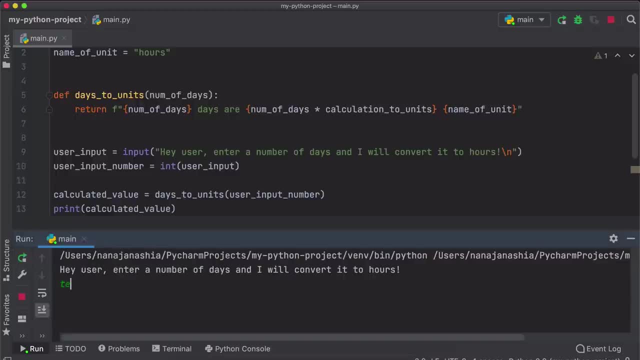 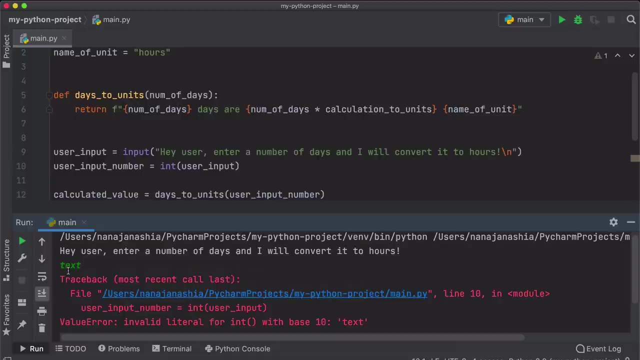 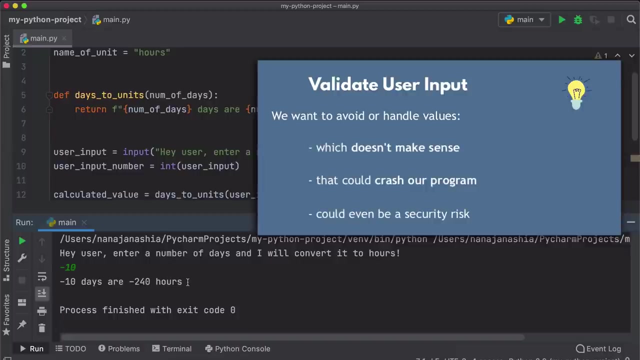 So now let's see what happens if we enter some text here. You see that the calculation didn't happen because we basically crashed the program application using that invalid user input doesn't make sense, or an input that crashes our application, because the calculation isn't even possible and we want to avoid. 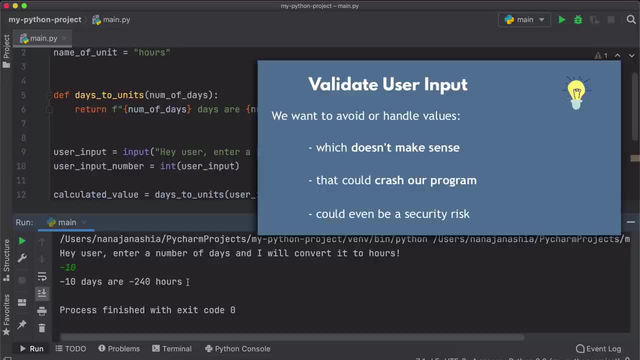 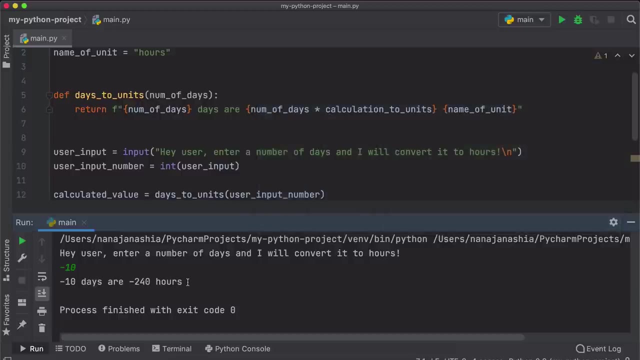 Users, basically either providing a nonsense value or a value that will crash our application. So we need to validate user input and this is again important concept in program because whenever you allow user input you always have to validate it. So in this part we're going to learn concept called conditionals and 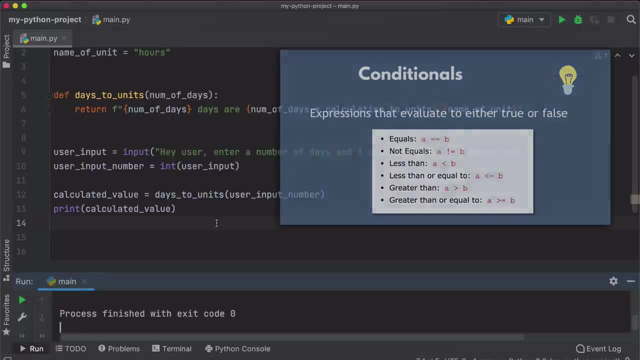 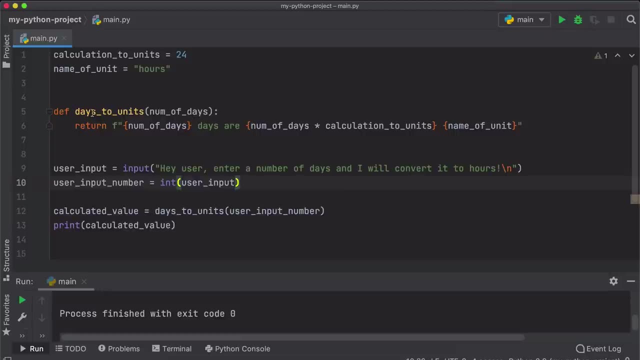 we're going to learn this concept with an example of validating a user input. So where are we? We're going to do the user input validation? We can do it in our function, right before we actually do the calculation. We can first validate: is it a positive number and not a negative one? 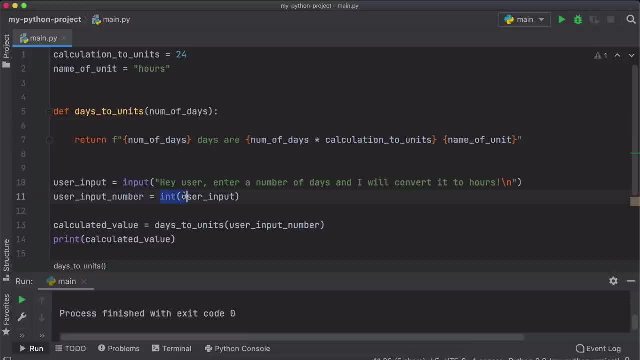 So user gives us their input, We convert it to a number and then we pass that number to our function. So negative 10, positive 10- that is a number basically- will be passed Onto our function. in right here we can check whether this variable. 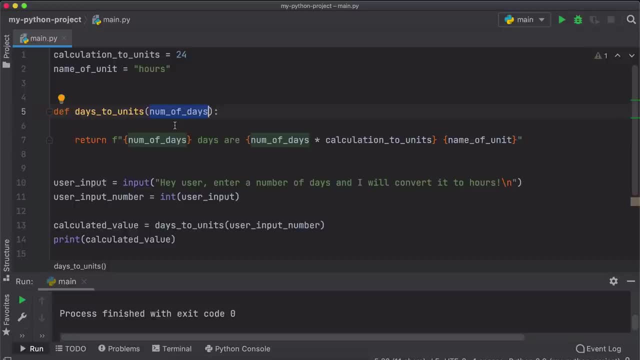 value here is a negative number or not. How do we do that? We do that using, if else, conditional statements. So very simple and intuitive to understand. We say: if number of days is greater than 0. Means it is a positive number. 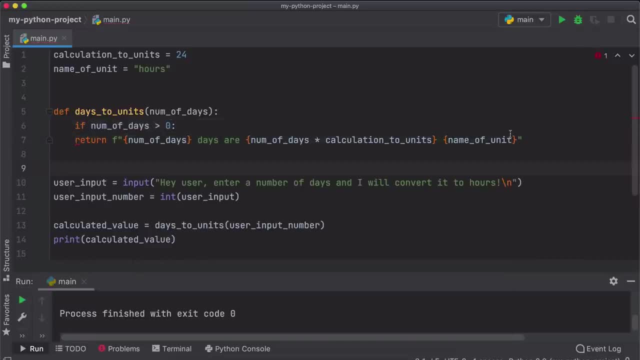 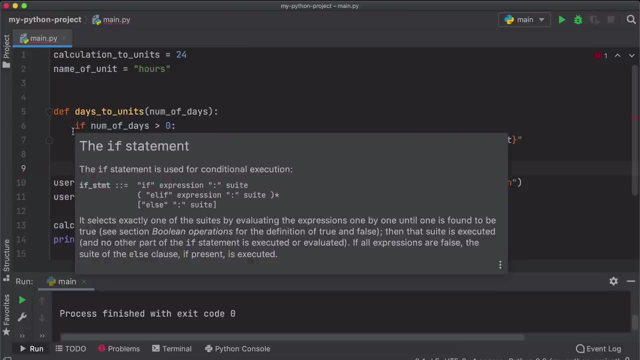 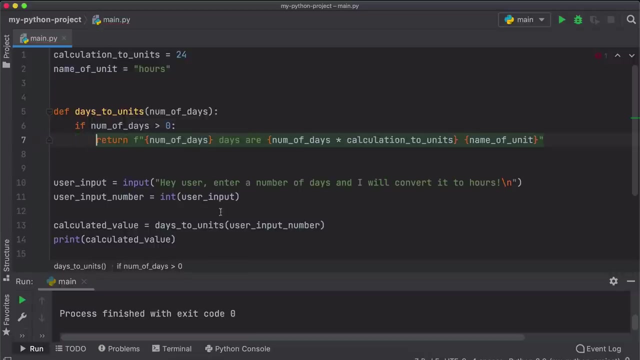 Then we want to do the calculation and return all of this. But you see that we have a red line here. So basically whenever we use if condition, we have to have a proper indentation. So all of this line basically goes indented for this line. 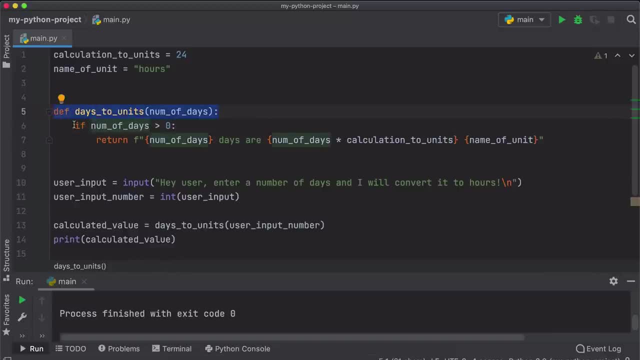 Kind of the same way as we indented the whole function body inside the function. whatever logic and whatever code is right here, Indented below the if condition will be executed if number of days is really greater than 0. So let's try that again. 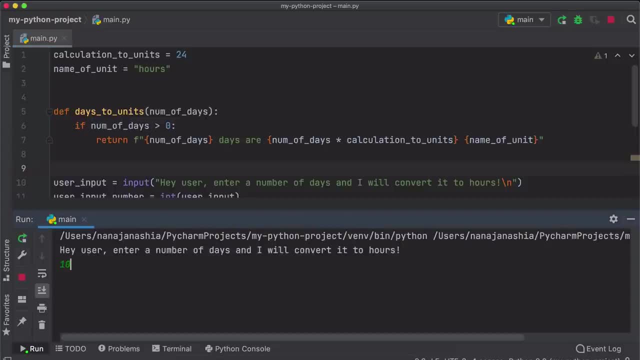 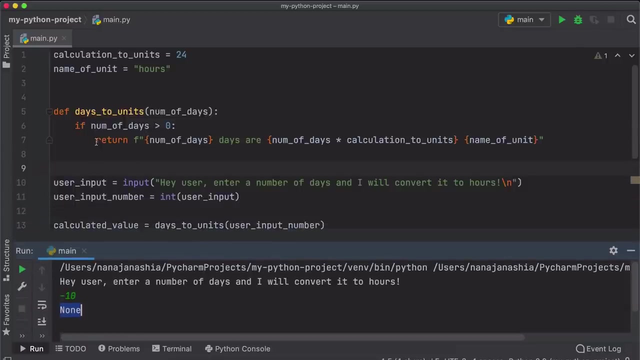 I'm going to execute it. Let's put a positive 10.. You see, 10 days are 240 hours got calculated. Now let's put minus 10 as an input and you see none, basically no output for us, because this line didn't. 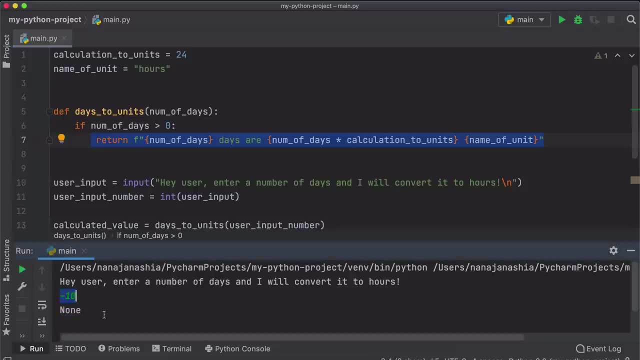 Actually get executed for minus 10 input value. Now what if we want to tell a user: Hey, this was an invalid value and that's why we didn't do the calculation instead of just showing none? We can do that by returning this feedback message or error message. 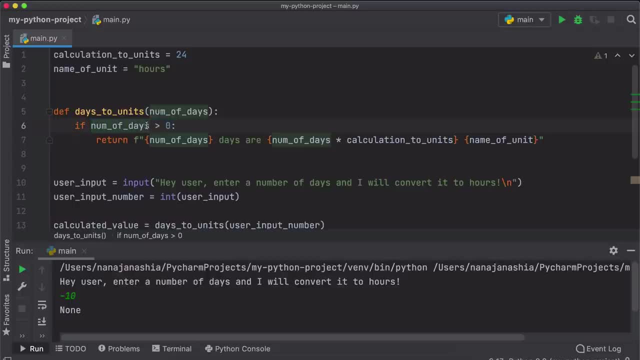 Whenever this is not true, So whenever number of days is not greater than 0,, we want to return something else, right Another message, and we can do that Using else, And the same way as for if we have the indentation, and whatever we write. 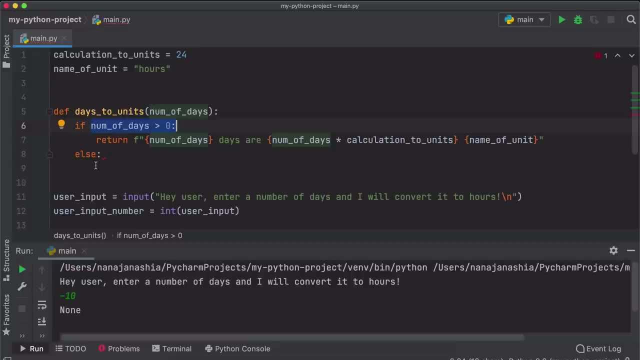 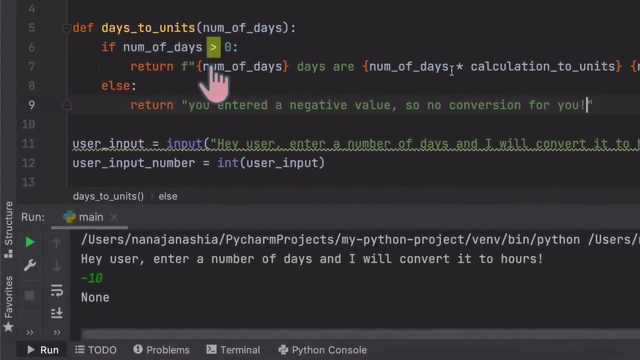 here will be executed if number of days is not greater than 0.. So here we are going to return you entered and negative value, So no conversion for you. And here it's time for another Special term in programming that greater than sign is called a comparison. 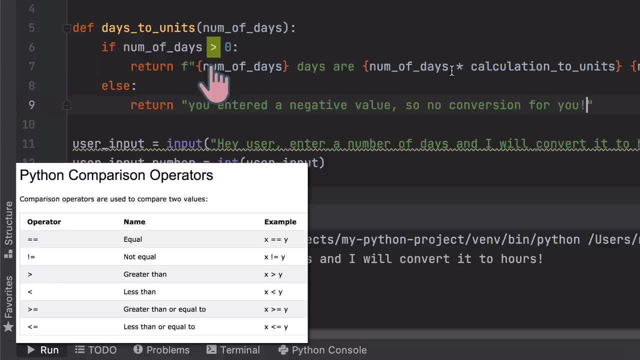 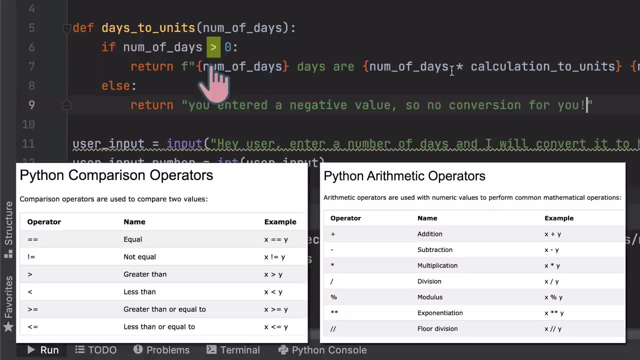 operator, and we have three of them. We have greater than, less than and equals, and these are called comparison operators because they are used in an operation to compare two values. and before in this course, we learned arithmetic operations like plus, minus, divide, multiply. So again, fancy words for simple concepts, but these are the official terms. 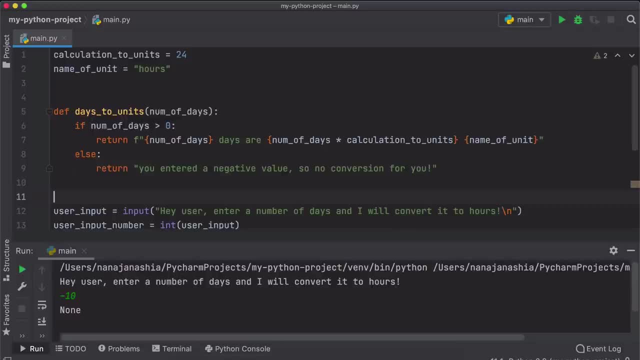 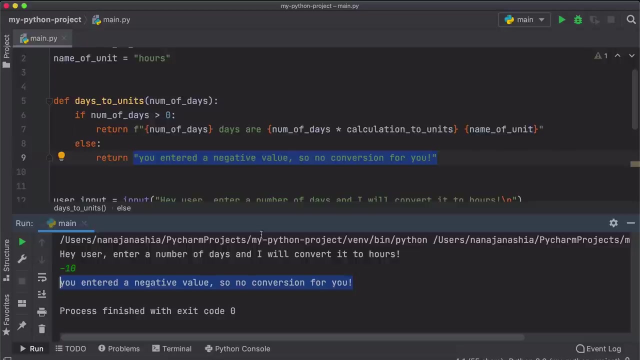 for this. So now, if someone mentions them, you will know what they're talking about. So now let's execute the application and let's provide minus 10, and you see that this line was printed as a feedback to the user. So, to go through the flow again, user gives us their input. in this case, 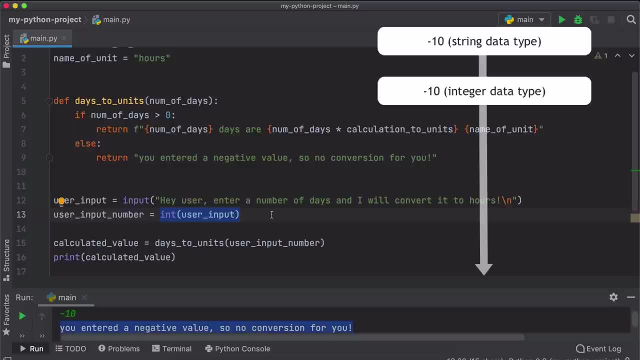 minus 10. we converted to integer, So now it's minus 10 integer and we pass it on To our days to units function and days to units function basically has this if else statement- that's how it's called in programming- and our if else. 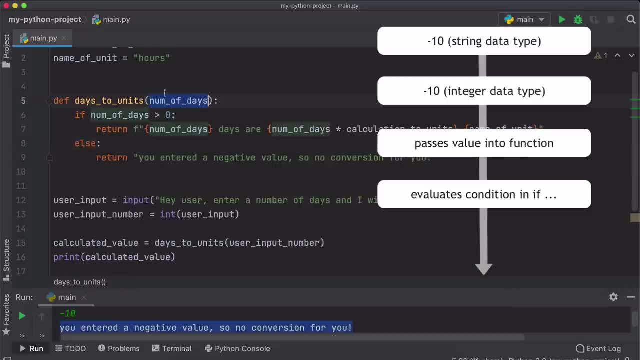 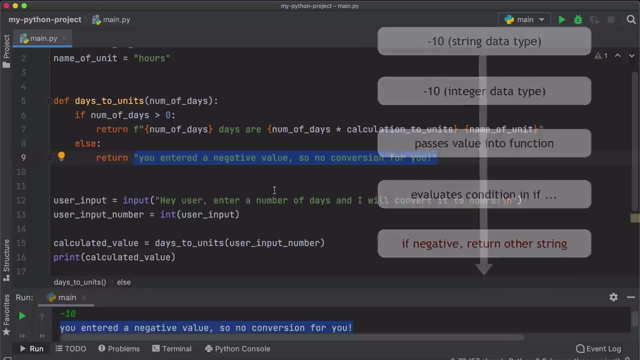 statement validates or checks whether these inputs is greater than zero. If it is, then the function will return this as a result. So basically the calculation with the proper message. else, So basically if this is not the case, then it will return basically just a feedback message for the user and know that else doesn't have such a 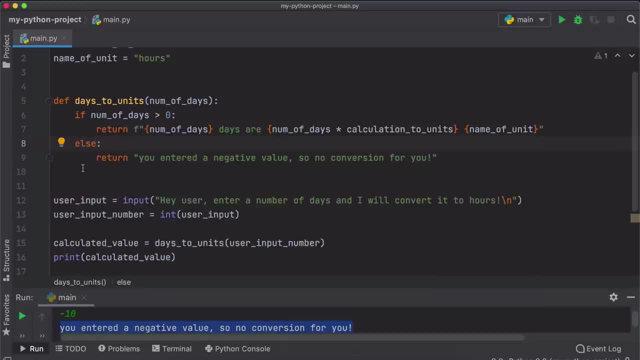 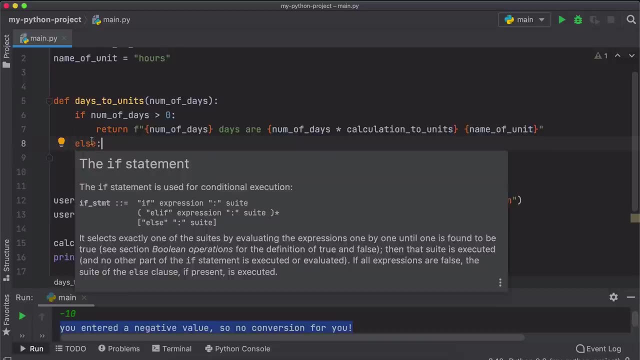 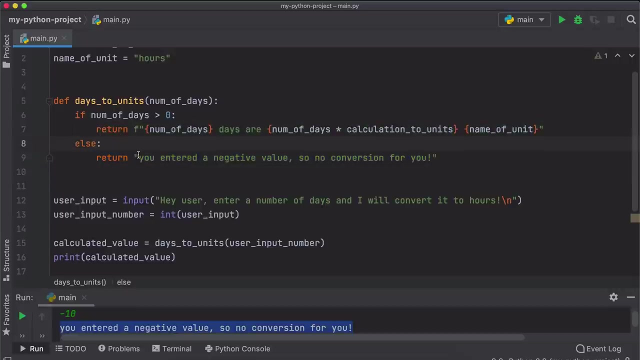 check here. We don't check number of days is less than zero, And the reason for that is because it doesn't check for less than zero, because it basically just decides if this is not true else, or in that case just do this. So we don't need additional check here. 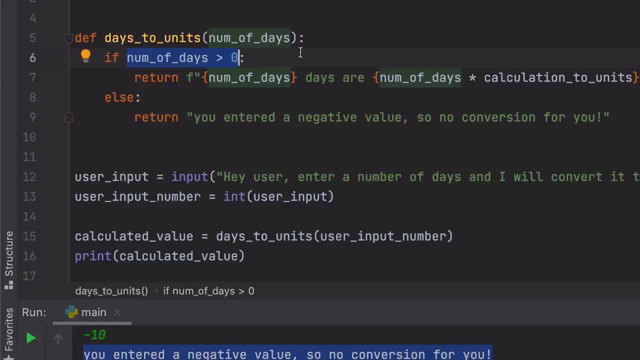 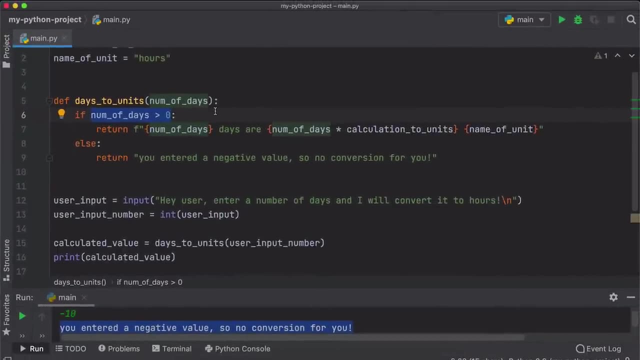 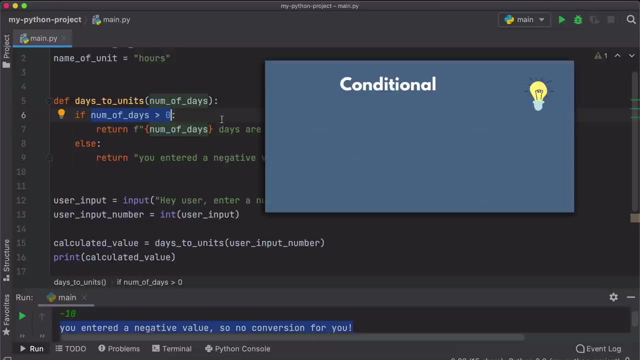 Now this segment right here, where we're doing the check, is called a conditional. So basically, we're providing our program a condition. If this condition is correct, then do something. Otherwise, do something else, and that conditional can be true or false. If winter 10, and this conditional will be true because it's greater than zero. 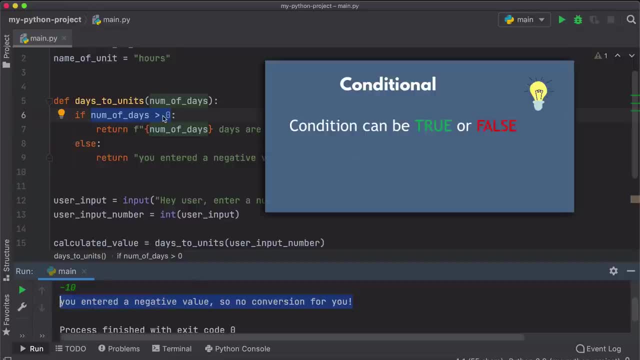 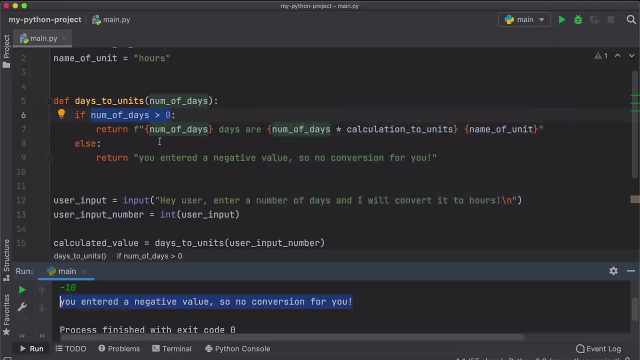 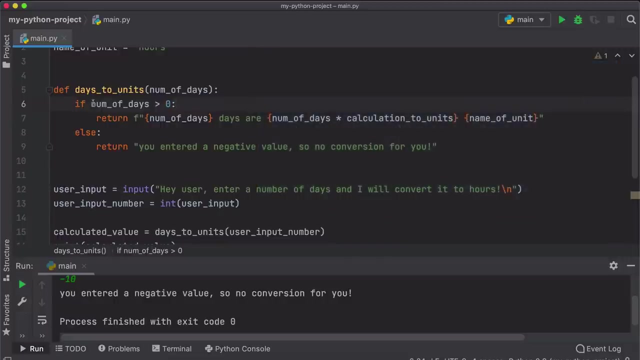 If we enter minus 10, then this conditional will be true, Negative. It's not greater than zero and those true and false values in programming actually are represented by its own data type, which is called Boolean. And in order to show it to you that this conditional either gives true or false, 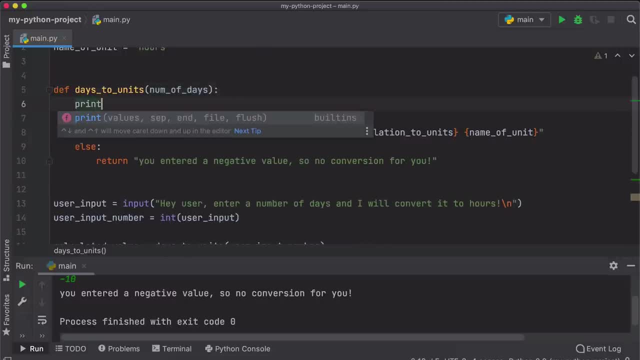 What I'm going to do is I'm going to print this conditional right before I do the check. So for a positive number input, this should print true, And if it's negative- so it's not greater than zero, This should print false. 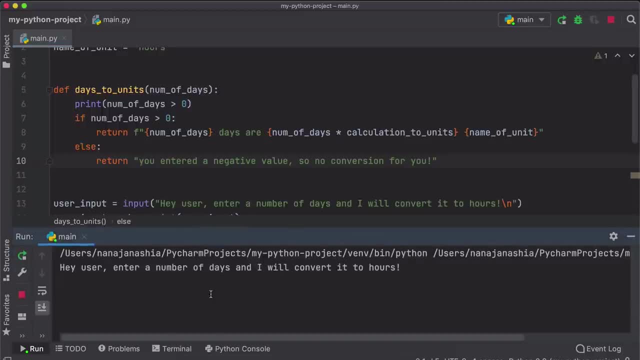 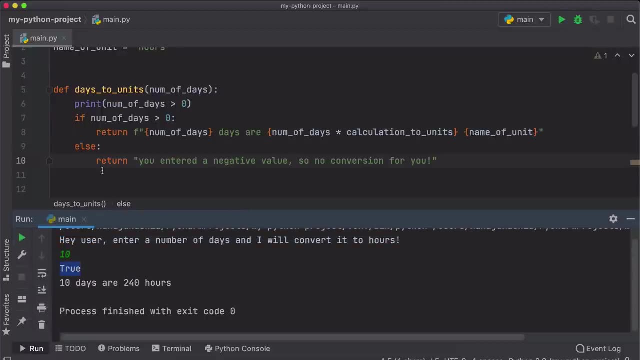 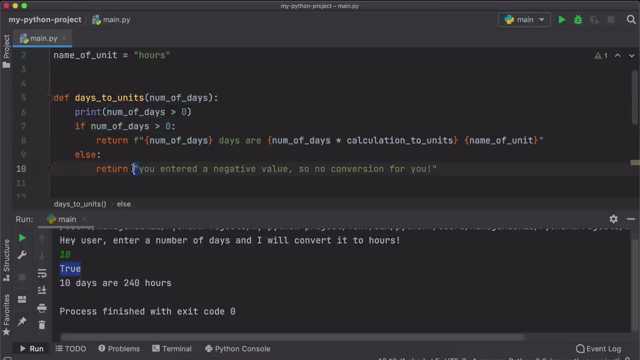 So let's test that out. First, I'm going to provide positive 10. And right here you see: true, because this condition is indeed true, And know that this is not a string. That's why we don't need quotes here, So we can basically just put in the whole expression in a print function. 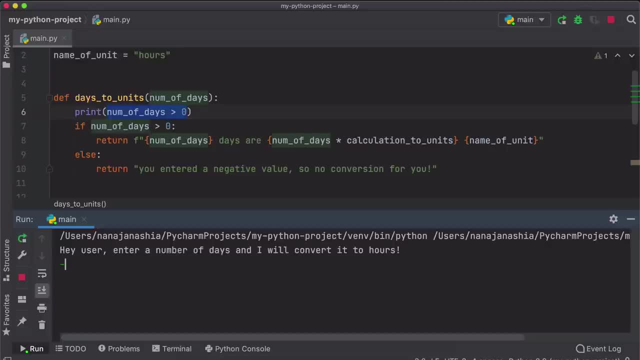 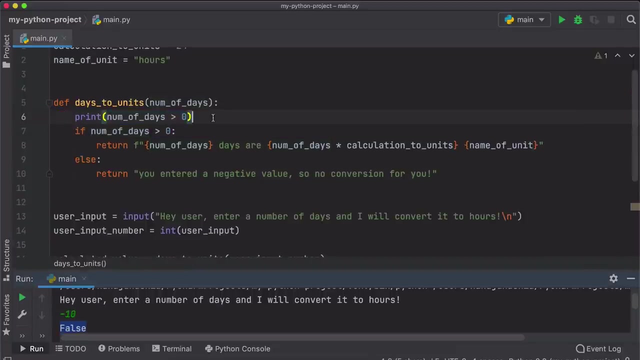 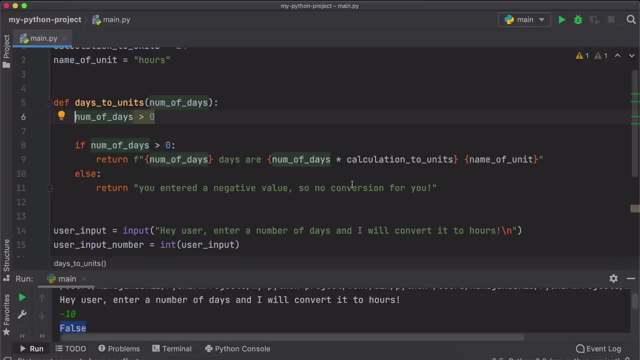 And now let's do the same with negative 10 and you see false And, as I said, true and false values belong to its own data type in programming, which is called a Boolean. And again we can demonstrate that instead of printing it out, we can save it into a variable. 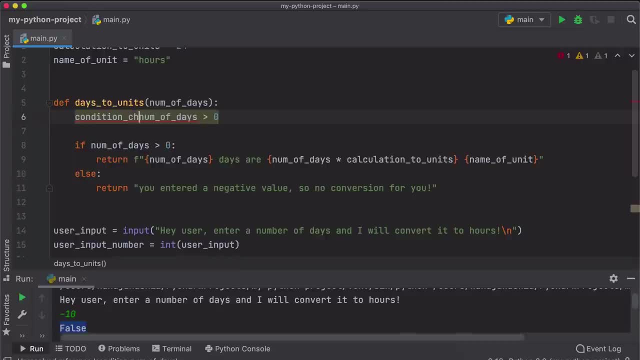 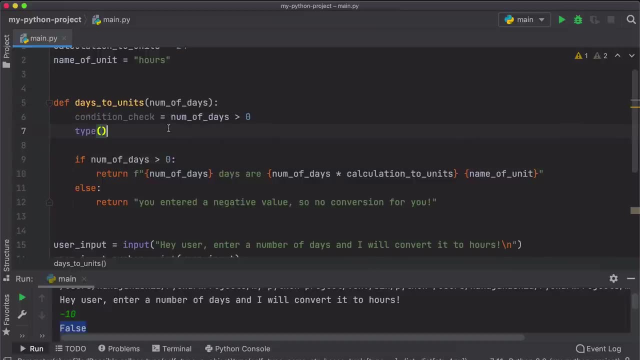 Let's call it conditional check, And in Python there is a function called type with checks or prints out, basically a type, data type of a variable or a single value. So if we pass it, so this will give us data type of conditional check. 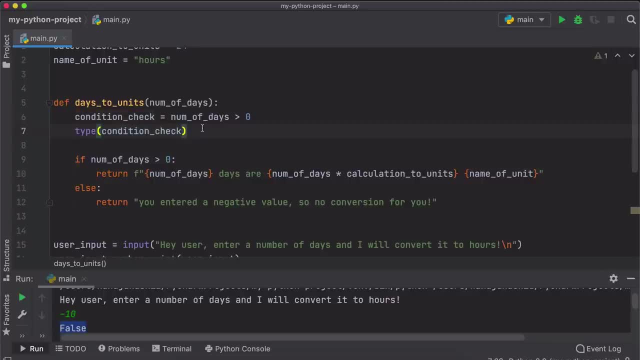 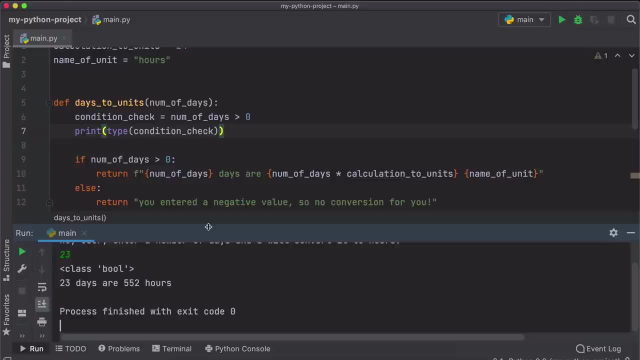 And obviously if you want to see that result, we need to print it. So print the whole thing. So it doesn't matter what we pass in this point And right here you see class Boolean. So this conditional check here, which has a value of true or false, is of type Boolean. 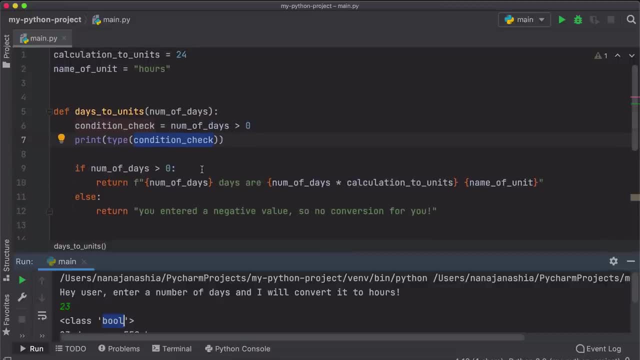 Now, there are two things that I want to note here. The first one is that you see that I am calling a function here which is type, And then whatever that function type returns, which is basically this output, here We are printing it. 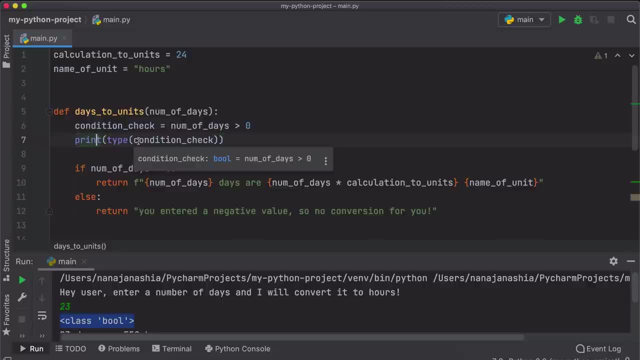 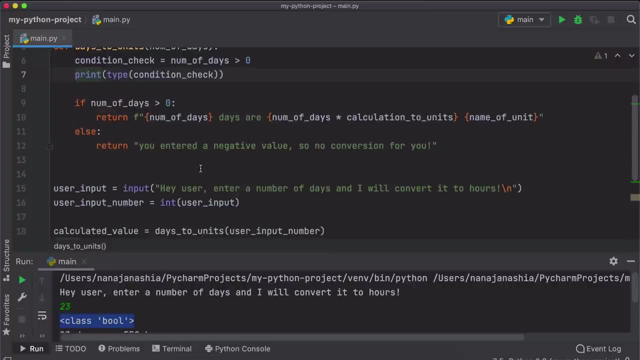 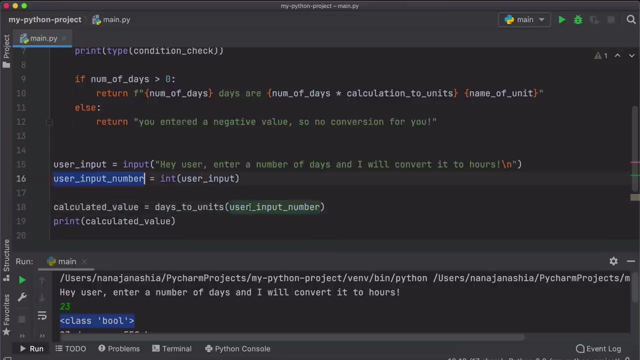 So we have two function calls that are basically nested, And that is absolutely fine. You can nest function calls. Another example of doing this nested function call would be, for example, right here: Instead of assigning these to a variable and then passing it, here we can actually save as that step. 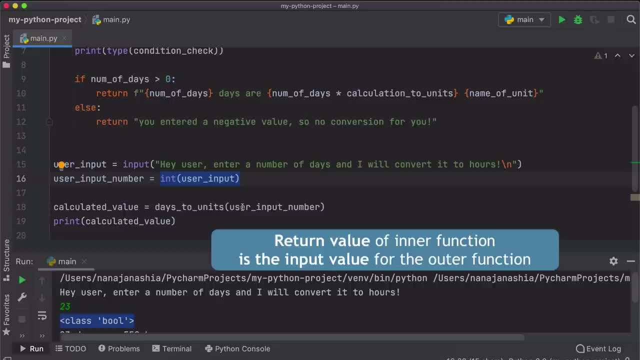 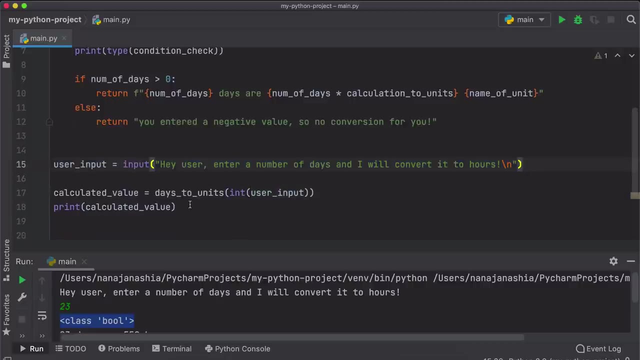 And in the days to units function call pass it as a value. So this is a perfectly valid syntax and you can do that, You can nest in the function calls and you would not need this additional step. And you can do that as many times as you want. 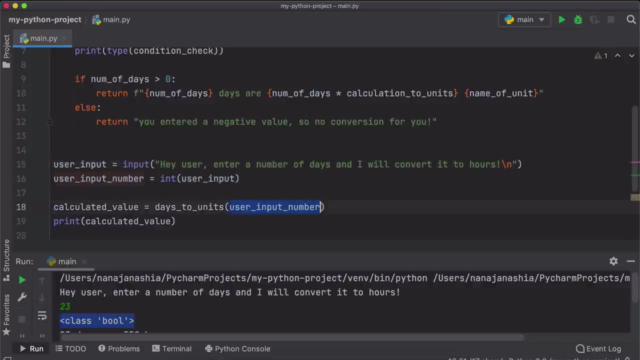 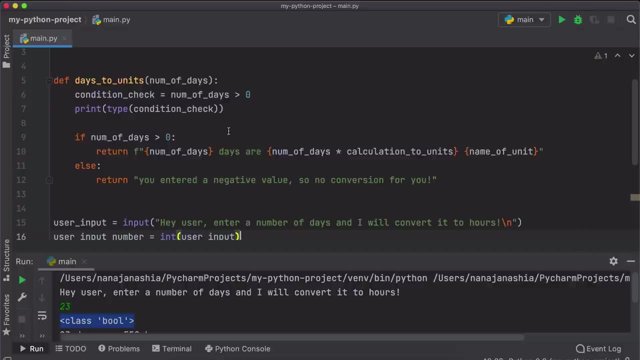 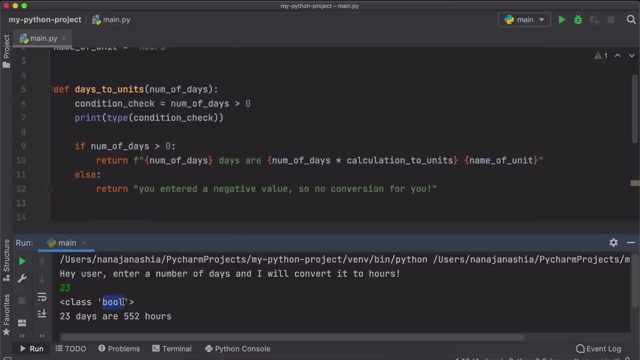 It just looks cleaner when you have that syntax a little bit separated and not have two, three, four function calls nested. So that's one thing, And another thing is, we just saw a class Boolean type here And let's actually see that same output for string. 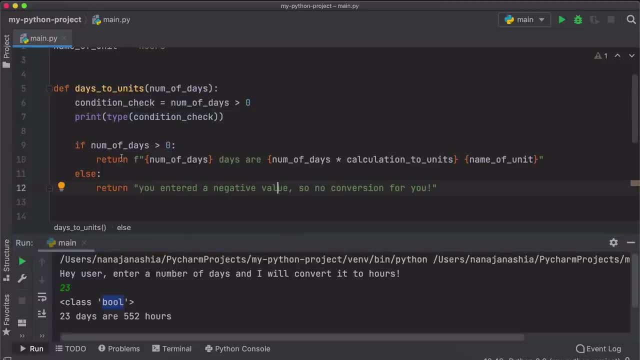 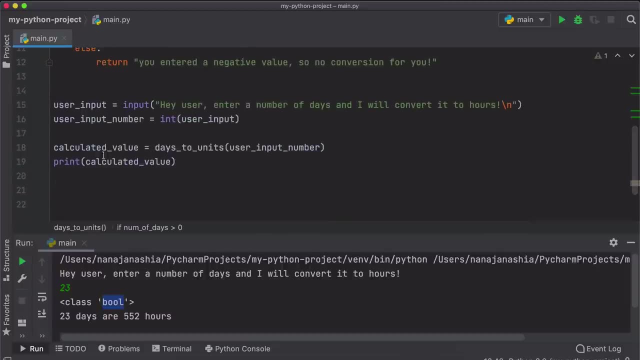 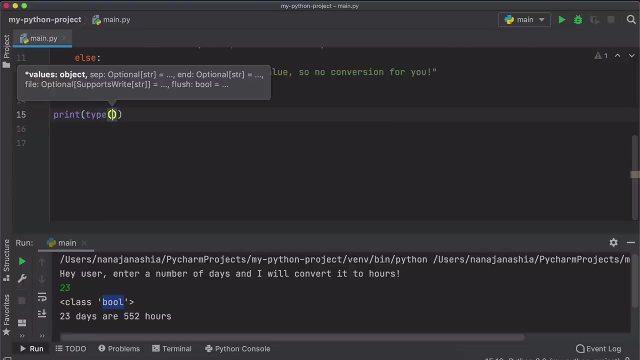 And number. So just for the demonstration, let's actually see the type of string and integer. Let's get rid of this for a second because we just want to test. So we're going to print the type of a string which says this should be a string type. 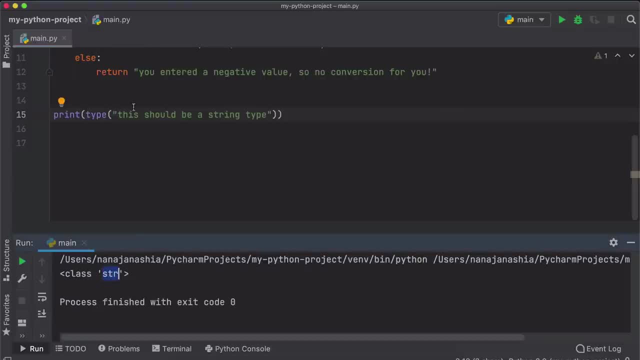 And execute, And you see class string. And now let's provide an integer, You see class int, And let's provide a float, And there you go, We have float. So this is a very handy way of checking the type, And we're going to need that, actually, in a later example. 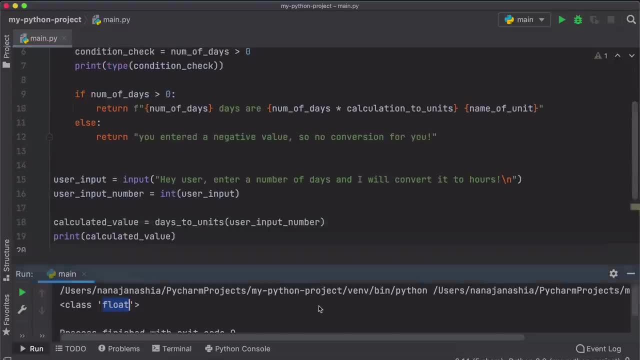 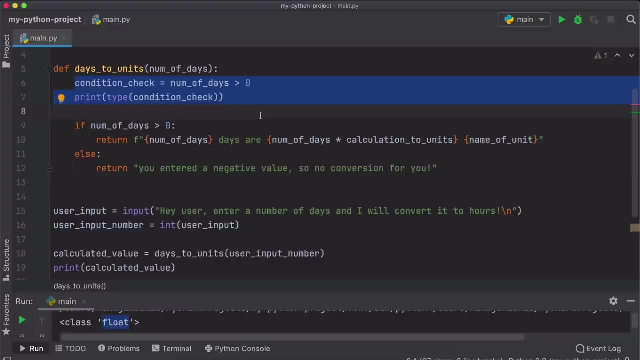 So back to our application. And one note about Booleans and conditionals Is that you're going to be using a lot of those in programming Because they're really the major or the core part of writing any kind of logic in programming. So you're going to need, if else, conditions and statements and Booleans in your application. 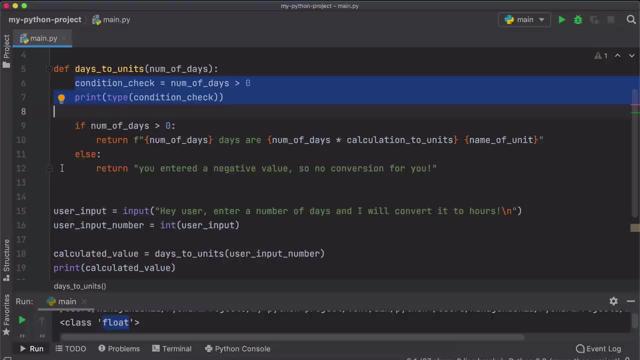 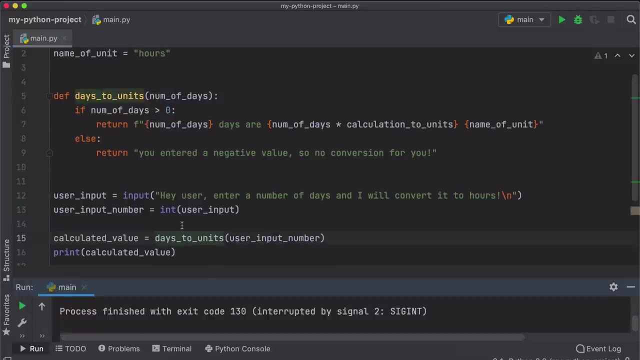 So it is a very core concept And we're going to be using a lot of them in our coming examples. So let's get rid of this code right here. And one note before we move on here is that the negative numbers are not being calculated because of this condition. 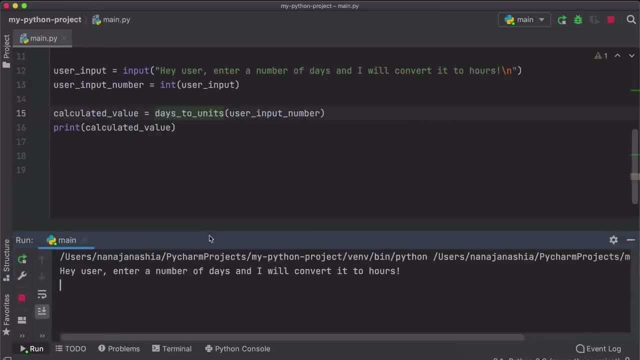 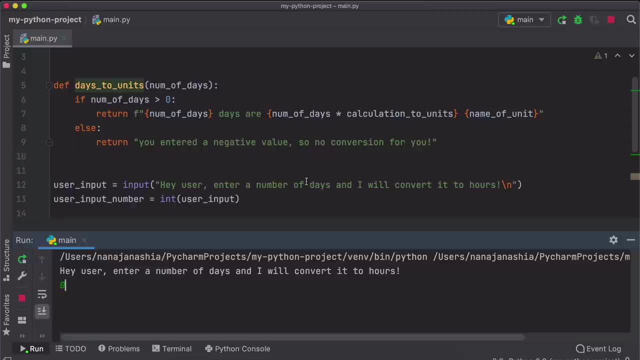 Now what about zero? Let's actually try that out. So I'm going to enter zero, Which is actually also valued. That doesn't make sense, because zero days input obviously will give zero of any units. So enter And right here you see. 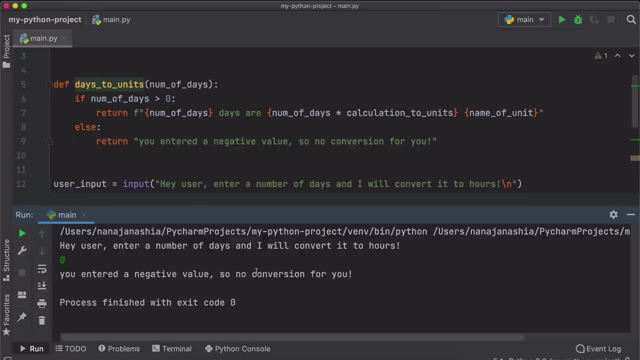 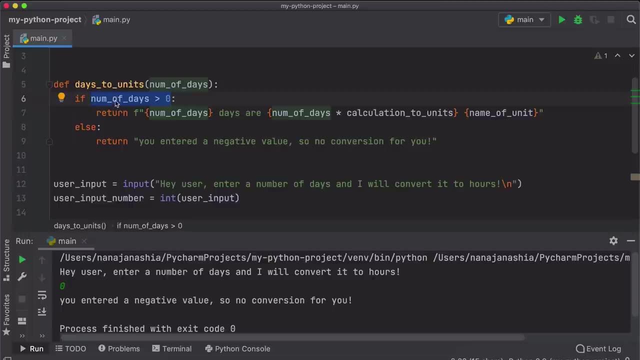 A feedback to user that says you entered a negative value, So no conversion for you. And the reason for that is because this condition here Number of days checks greater than zero, Which means that negative numbers and zero will not match this condition. So they will basically give you this feedback. 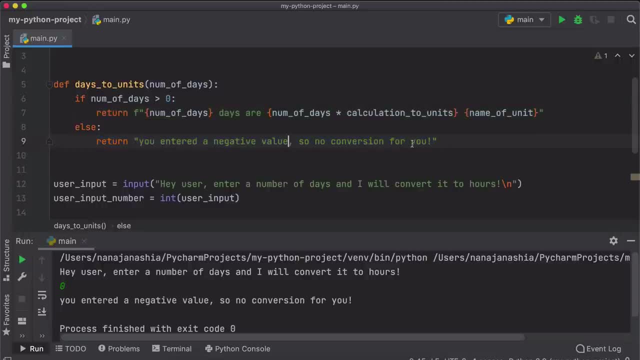 But our message says: you entered a negative value, Right, When we entered zero. What if we wanted to have a specific message? Have a specific message for a user if they enter zero And a specific one if they enter negative value Right. 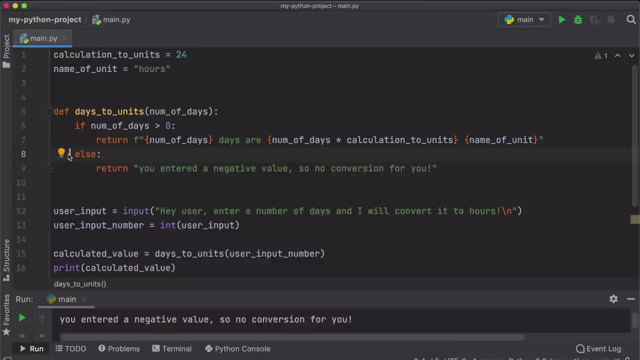 We want to differentiate between those two. How can we do that? In the if else statement? in programming We can have multiple conditionals, So basically we can have multiple ifs. So how do we do that? First, we check number of days is greater than zero. 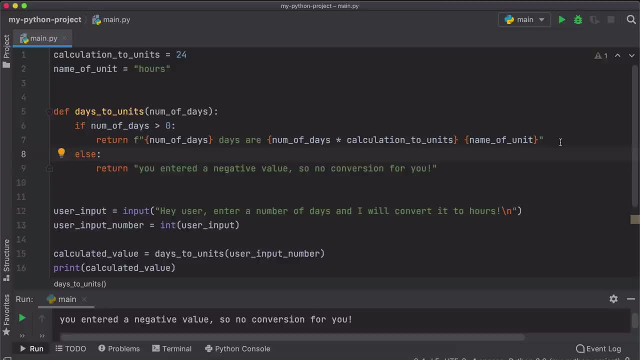 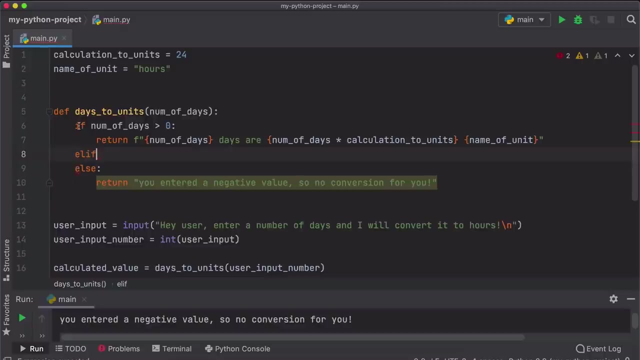 OK, Great. Now we want to check whether number of days is equal To zero, And we can do that using another if. here And in Python, The syntax for that is l if, Which basically is a combination of else and if. 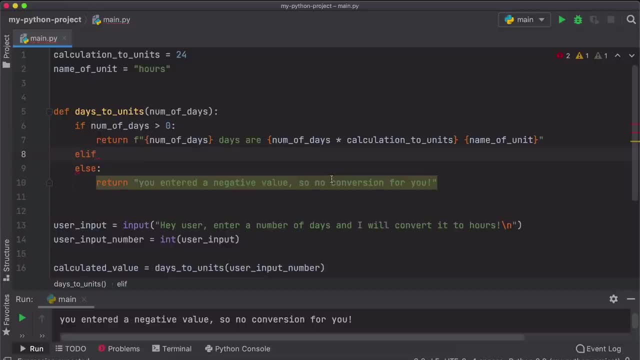 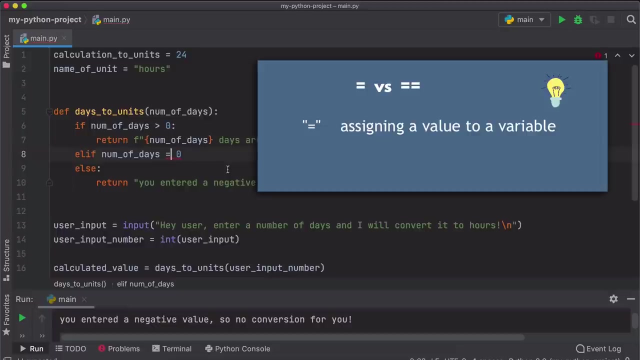 So if this is not true, Then we want to check another condition: Number of days equals zero. Now you know the equation sign. generally is this one right here? However, when we're checking whether something equals to something else, in programming, That equation check is represented with two equal signs. 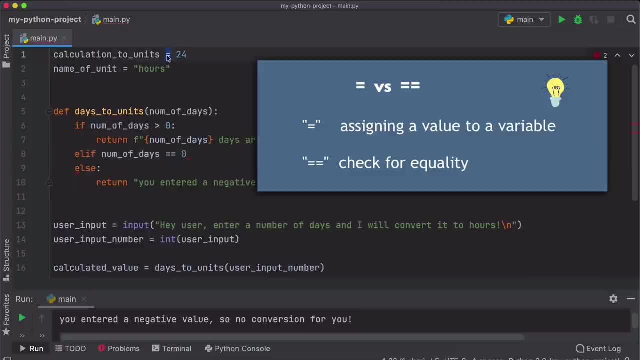 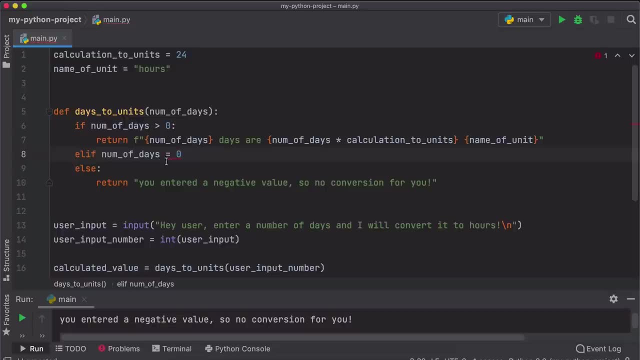 And the reason is because one equal sign is already used to represent assigning a value to a variable, So not to confuse those two actions in programming We have two equation signs when we want to check whether something equals a certain value And, just like here, we execute some logic whenever this condition is true. 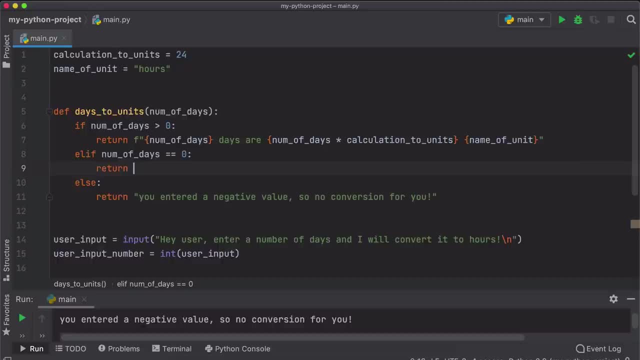 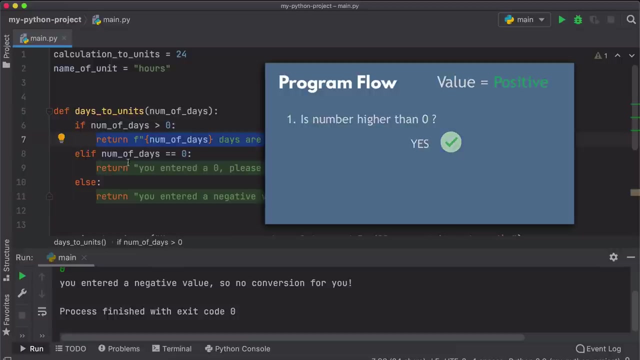 So in our case we want to tell the user: You entered at zero. Please enter a valid positive number. So now again to go through this logic flow: If the input value is A positive number, then function will return the calculation and the message. 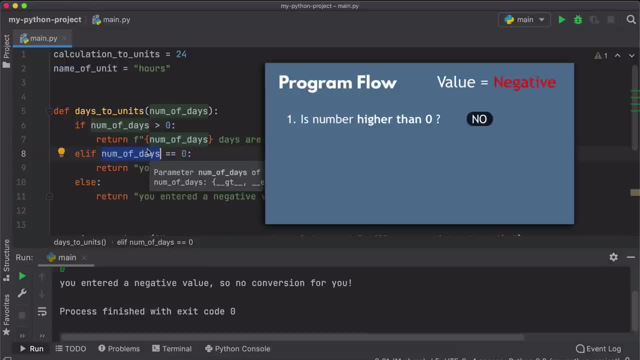 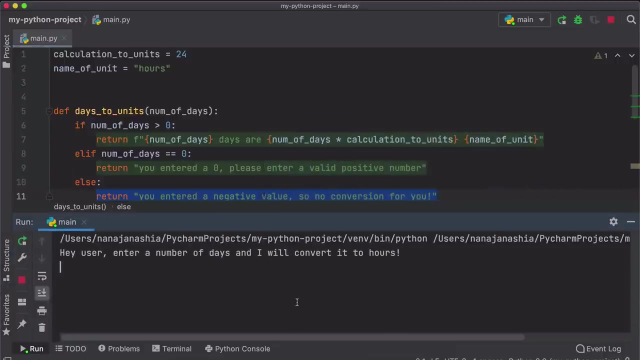 If it's not a positive number, then we will check additionally whether it's zero. If it's not zero, then this is a last condition. basically, Then we know that it has to be a negative number, right? So let's test this out. Let's enter a positive number. 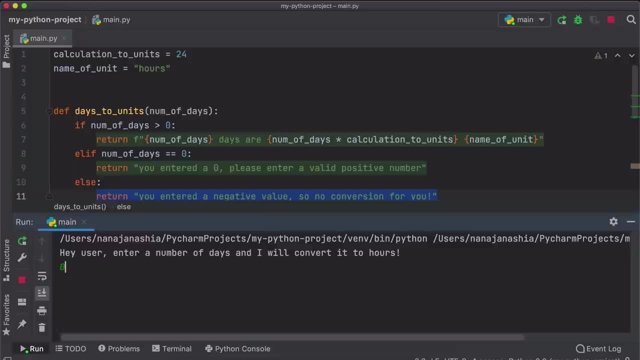 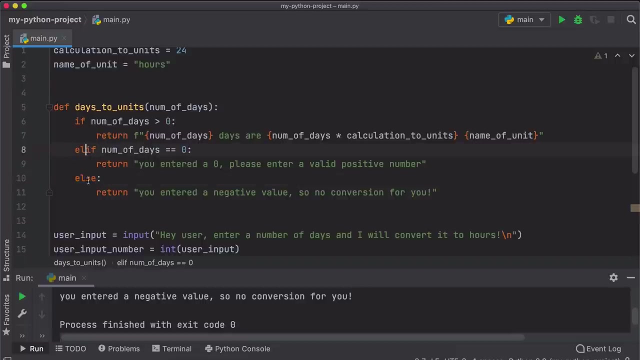 There you go. Let's enter zero. You entered zero. Please enter a valid positive number And let's enter negative one, And everything works perfectly. Note that you can have multiple L ifs between if and else statements And again note that L if has a condition, just like if statement else does not have any condition. 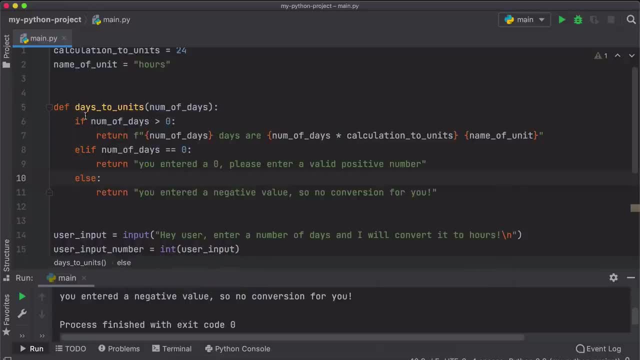 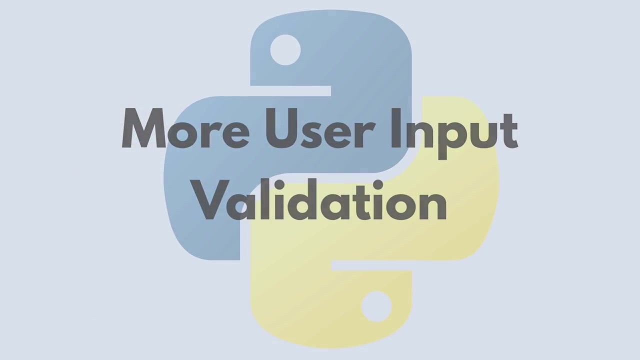 So this is like the fallback, So if everything previously stated, all the previous conditions, did not match, So they were all false basically, Then this is the logic that will get executed in that case. Great, So we have validated input value for users. 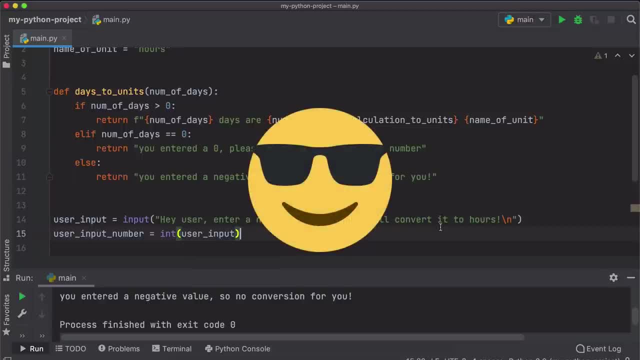 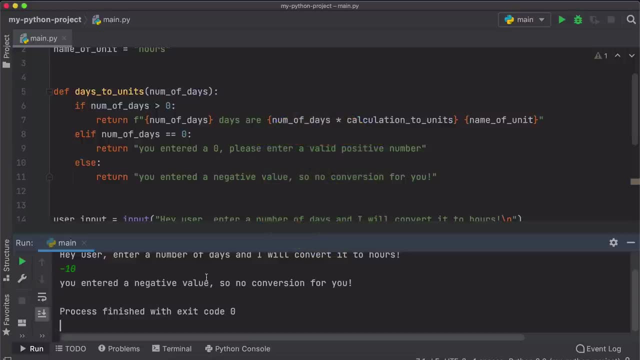 And we may feel pretty good about our program because it doesn't calculate anything for values that don't make any sense. However, we still have a problem. What happens if a user enters a text instead of a number, So basically anything that is null? 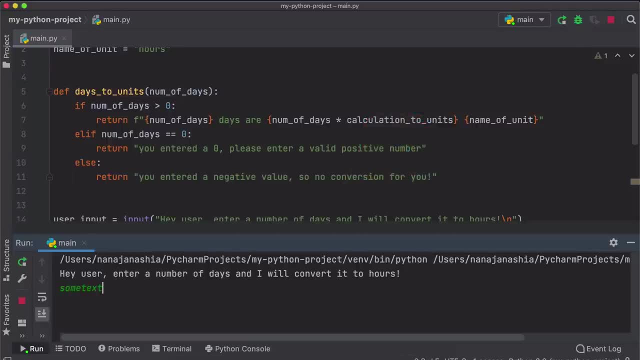 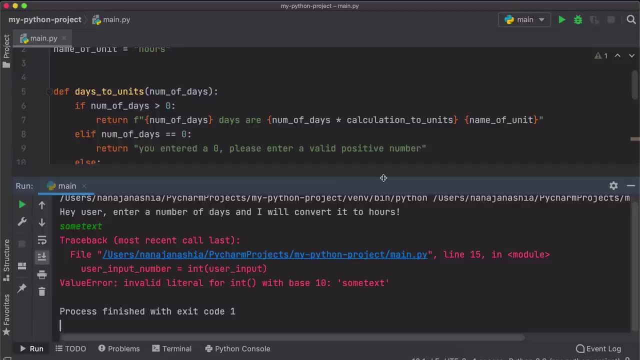 Not a number value, Doesn't really matter, Basically some text And if I enter, you see that our program actually crashed And this is actually a user input that we want to protect our programs from, Because we don't want to allow users to blow up our application. 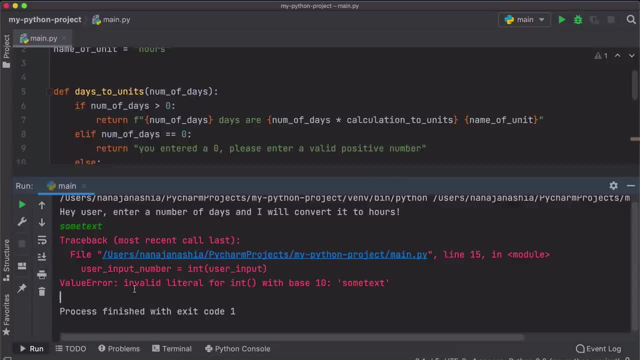 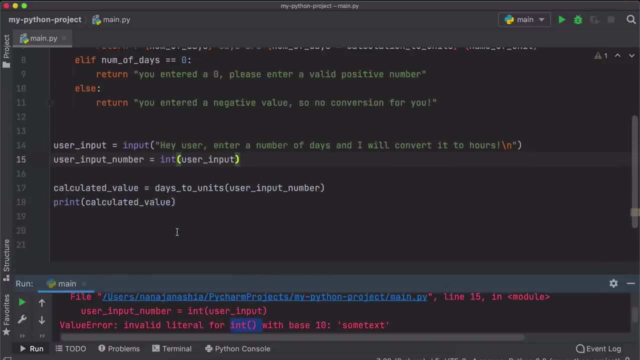 So let's see what happened. It actually says that we provided an invalid literal. Literal basically means the text itself Or a number, So basically a value that we entered For int function. That's the problem. So this function call basically just blew up. 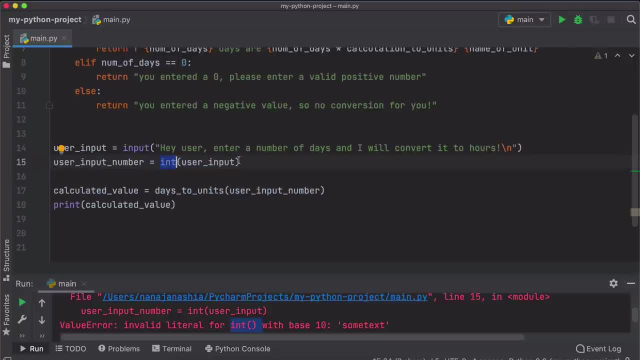 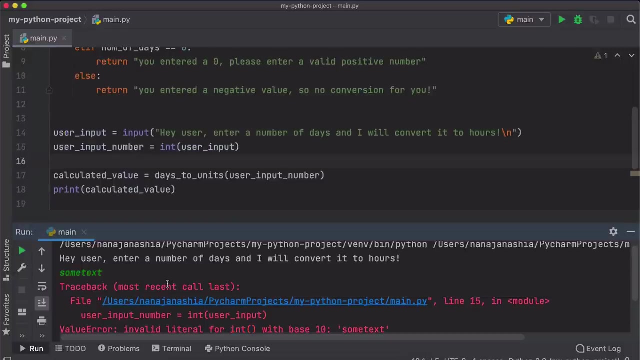 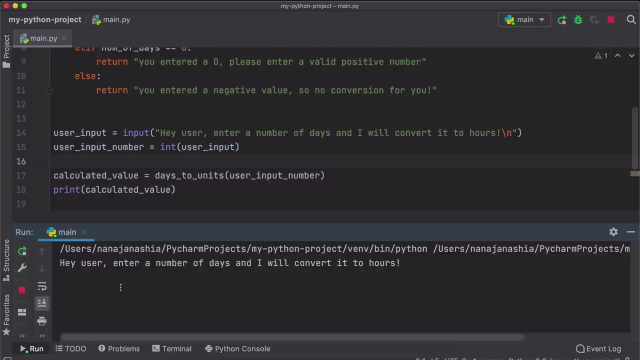 Because int function expects a value which is a string representation of a number. So basically, int expects something like this Or something like this. It doesn't expect my text Or some text, So our application crashed on some text input. Now let's see what happens if I provide a number. 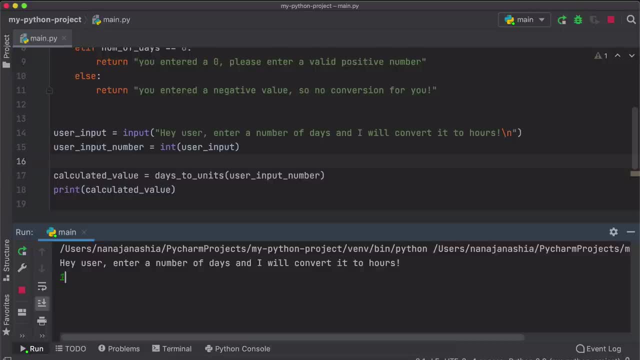 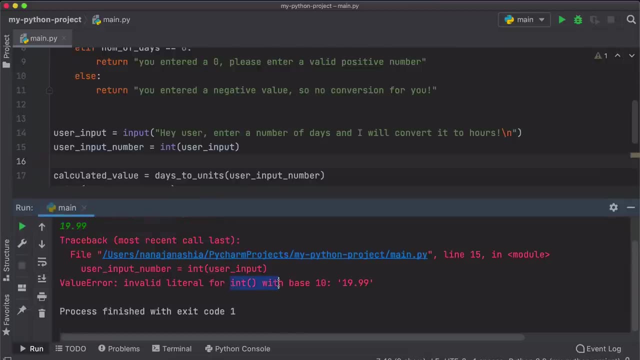 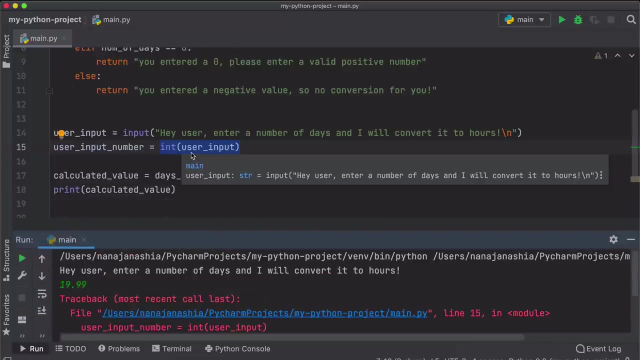 But a float number instead of integer. Let's enter 19.99. And enter And you see the same error. This function basically returns an error Because it cannot convert float into integer as well. So we have a problem here that whenever a user enters, 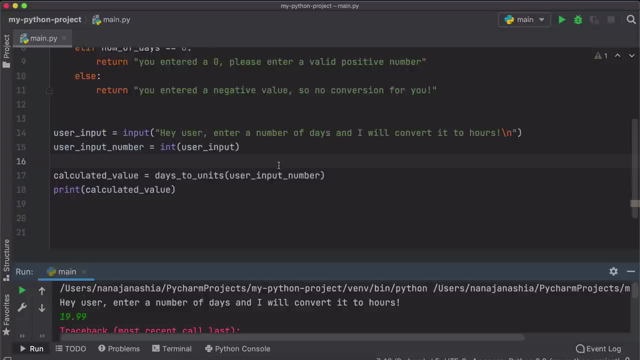 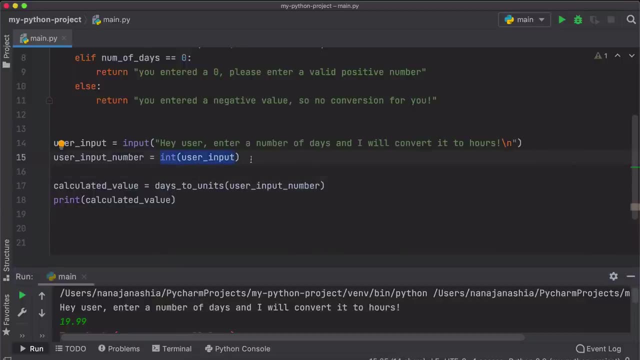 Anything which is not integer, Our program will blow up. So how do we avoid that? So basically, before the int function gets executed with an invalid value, We need to validate this whole thing and stop our program Before that happens. So we need the validation before int gets executed. 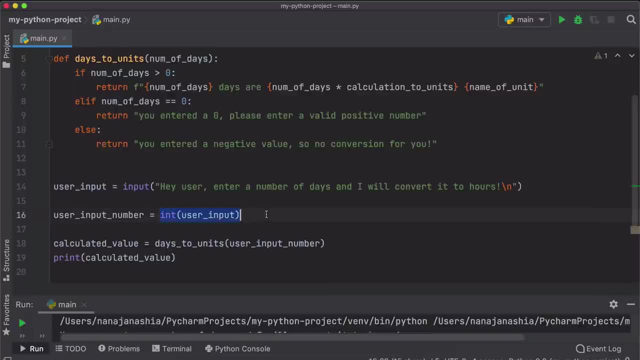 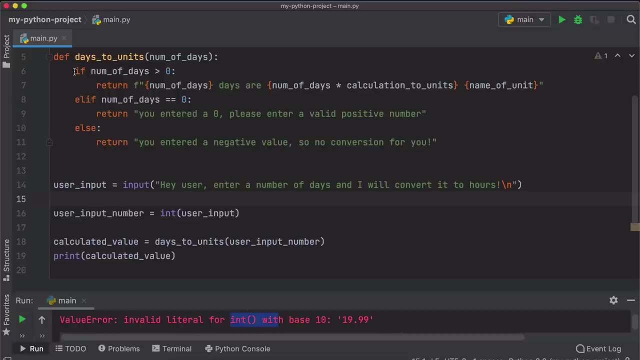 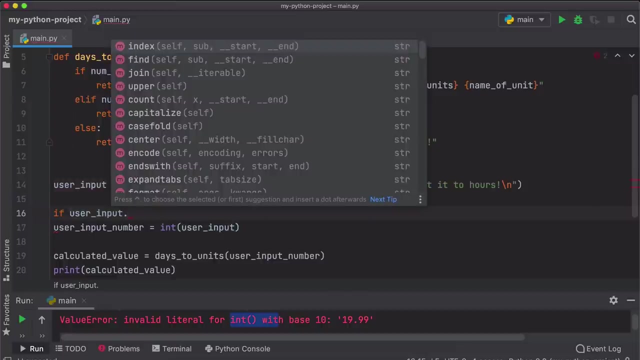 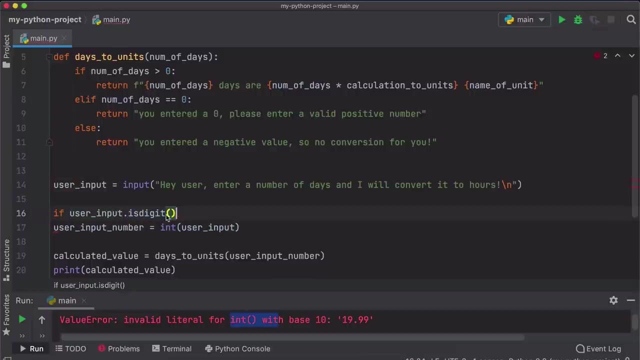 And we can do that right here. Right, So, before that line gets executed, We're going to do a validation And one way we can do that is using our familiar if else statement So we can say if user input is digit. So again from the syntax you know this is calling a function. 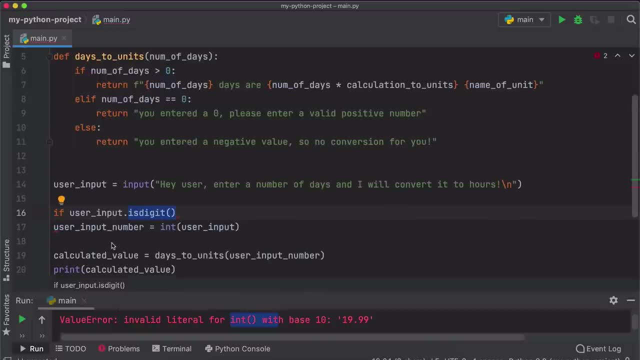 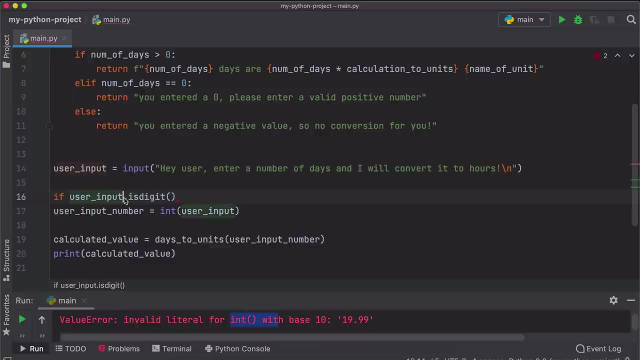 But note that instead of calling the function like this- So basically just stand alone- We have the syntax, where we have the variable Dot And then the function name. So instead of passing this as a parameter right here In the function brackets, 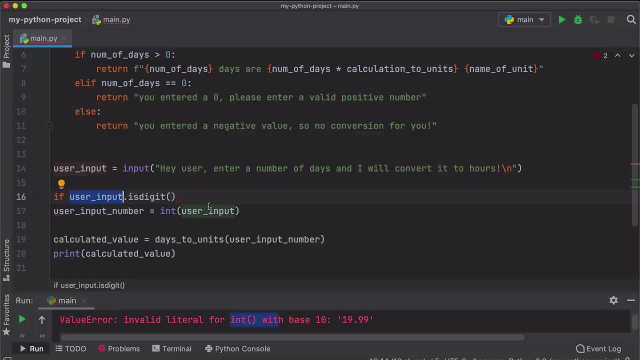 We are passing it as a parameter again, But using this syntax Right, So is digit function will execute for user input as a parameter And again in if we have conditions. So this will be either true or false. It's a Boolean. 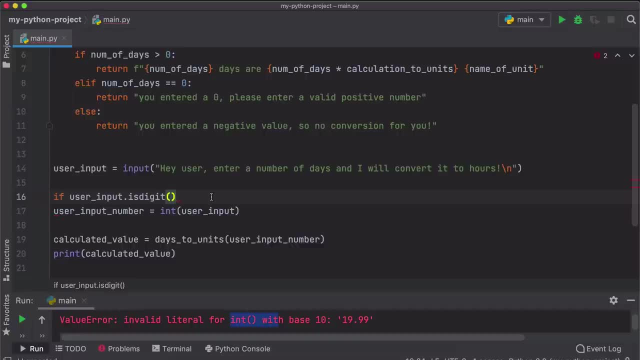 And if user input is digit, It's a number Basically. So basically this will filter out input values that are text, So basically they're not numbers, And if the input is digit, Then we want to execute this line And also the rest of our application. 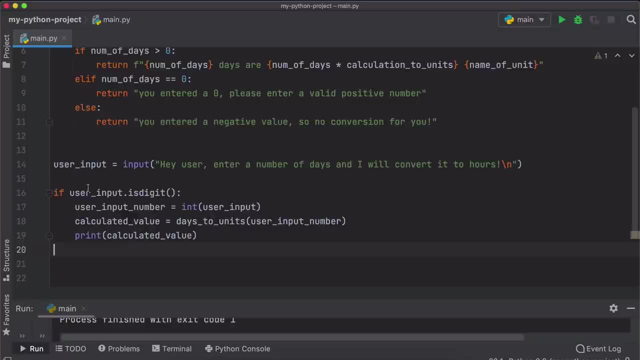 Like this. And if it's not true, So if the user input is not a digit, We don't want to execute anything in our application. We want to stop The execution and want to tell the user This was an invalid input value. 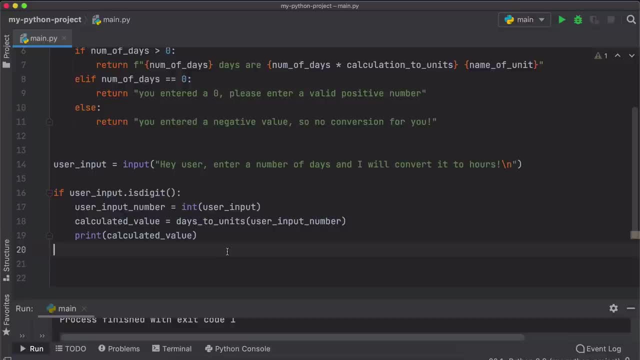 I'm not doing anything with my program so that it doesn't crash. So else, If not digit, We are telling the user Your input is not a number. Don't ruin my program. So now let's actually test it. So I'm going to execute. 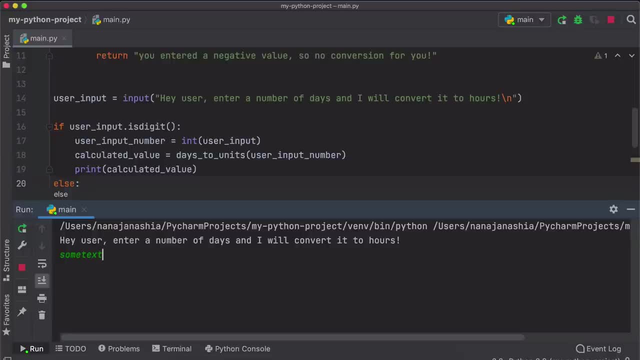 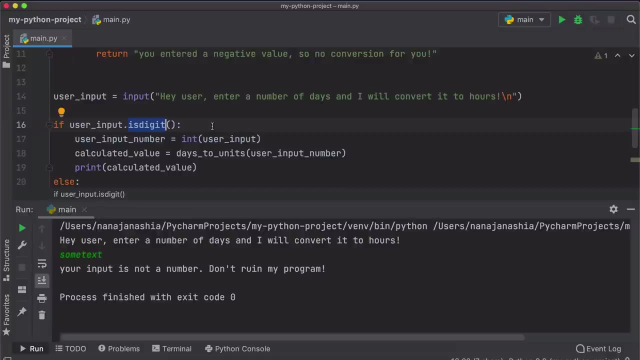 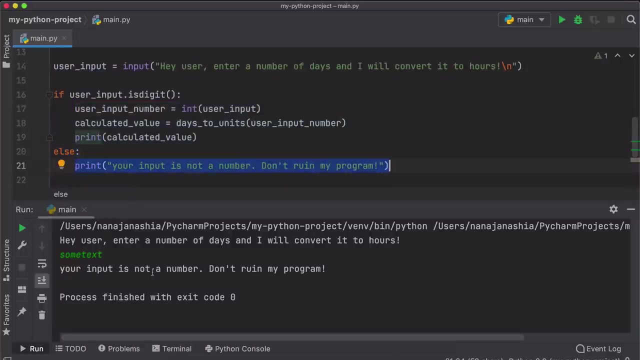 And write Some text. And there you go. So user input is digit was evaluated to false, So none of these got executed. instead, The else block was executed and printed a message for our user. So we basically avoided our application to crash with this check. 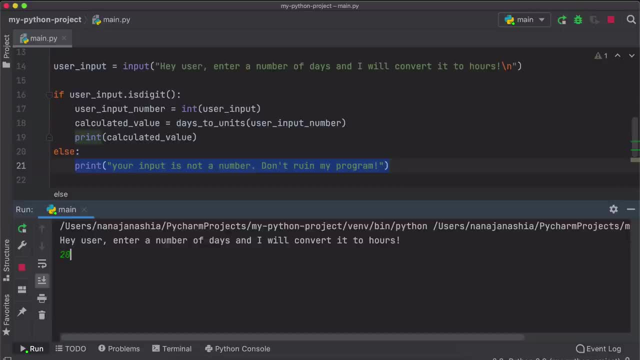 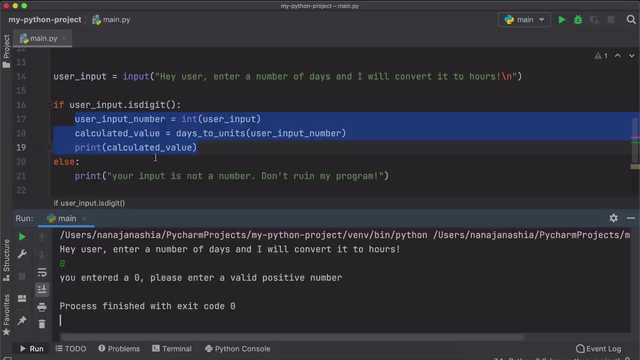 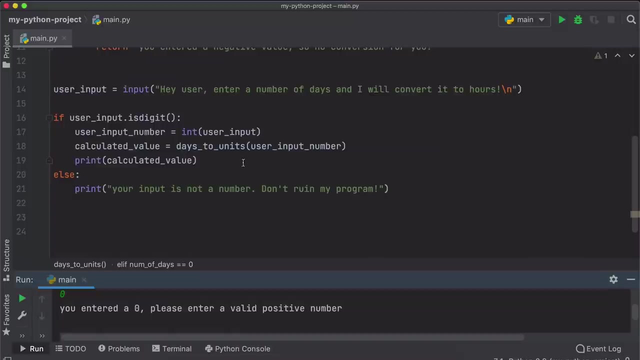 And if we try a proper number, It works. And if we enter zero, For example, The application will get executed and we will get our message from here. So our application is more or less protected And we're not allowing for a invalid input number. 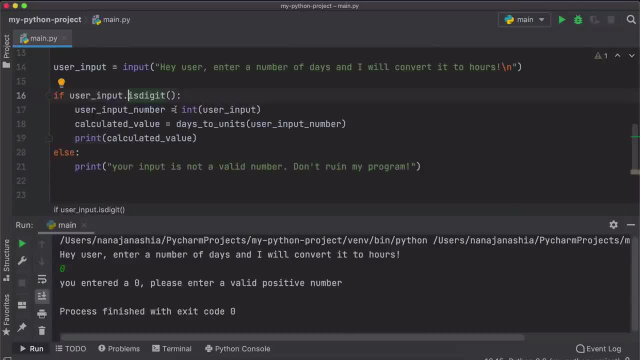 It's not a valid number. Now, we know that in programming there are different types of numbers. We have float numbers as well. So let's actually see what is digit function really checks. So let's actually try to provide a float number instead of integer. 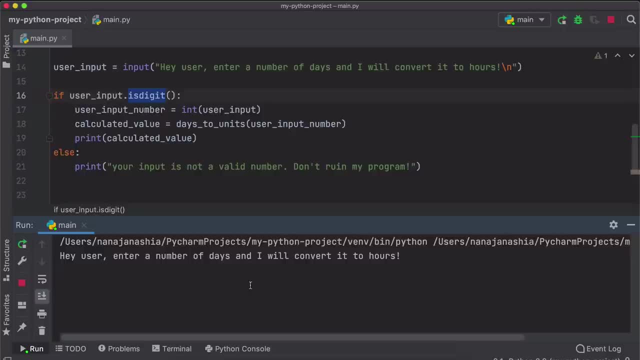 Which is not a proper valid input for our program. So I'm going to type in 19.99.. And you see that is digit is false for a float number. So we got the same. Your input is not a valid number, So I'm going to type in 19.99. 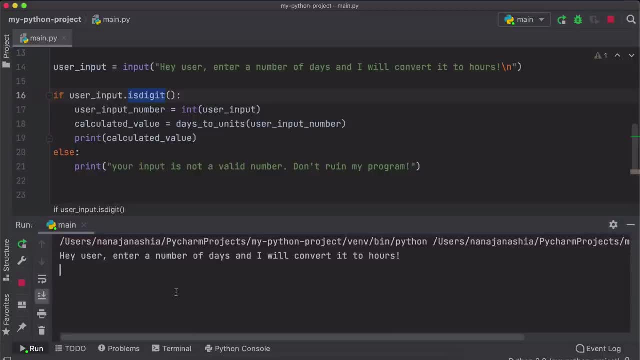 And you see that is digit is false for a negative number. And now let's actually try to enter a negative number And let's see if is digit function returns true or false. I'm going to enter And you see that else block got executed because is digit was false for a negative number. 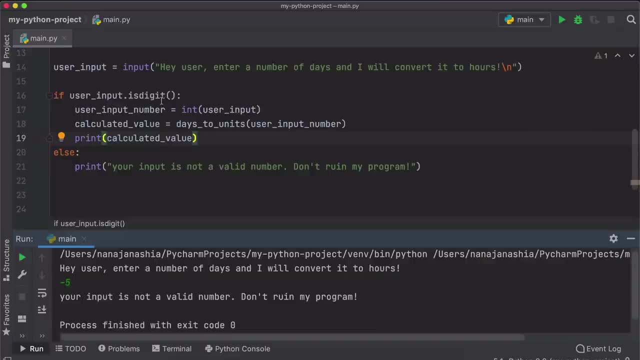 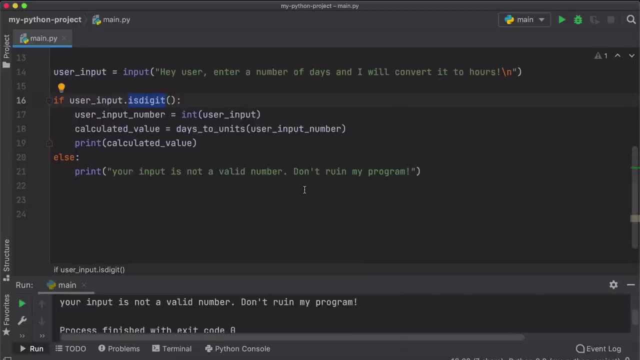 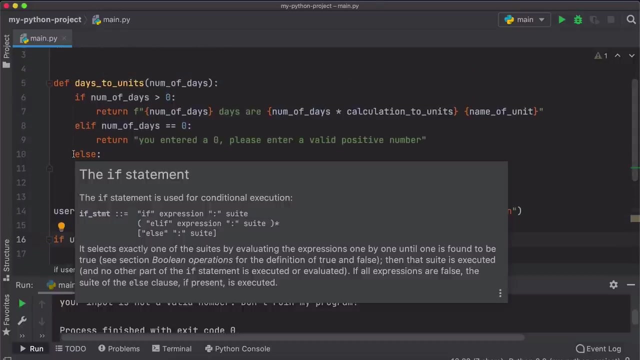 So basically, this function filters out a lot of the bad input for us To get a negative number. So I'm going to add input for us to protect our application from bad user input, And that also means that we don't need a check for negative values anymore. 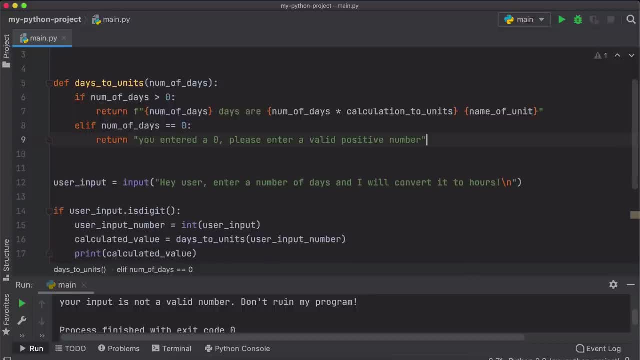 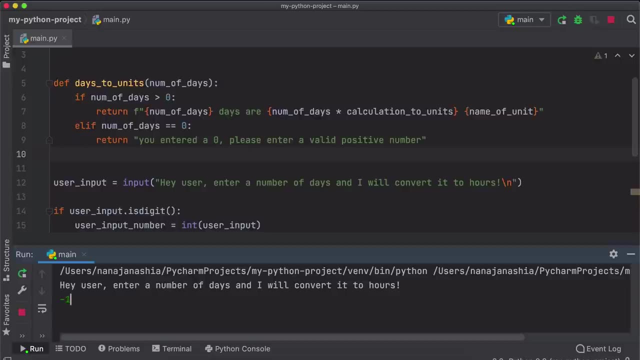 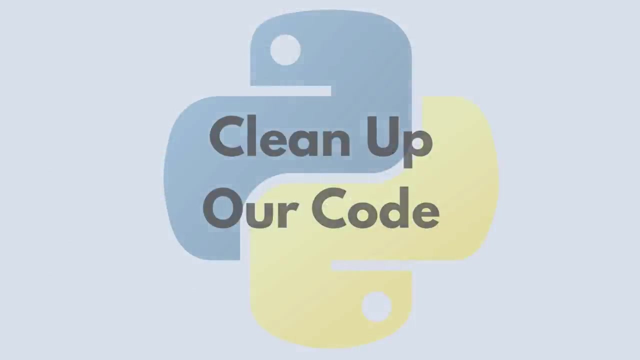 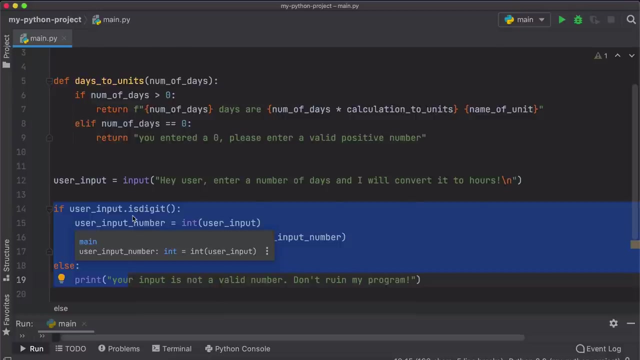 And, by the way, in Python you can actually have if statement without an else at the end. This will work perfectly fine And this could be our application. However, note that in programming we don't put this type of logic directly, like this: 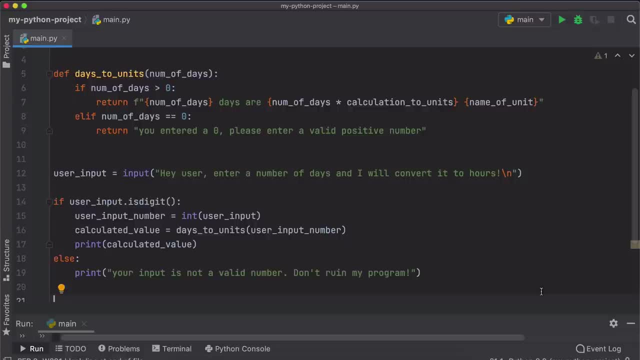 Basically outside of function. as a common and best practice, we encapsulate most of the logic, basically in functions. So as a cleanup for our code, We can take all this and put it into a function. So right here I'm going to create a function. 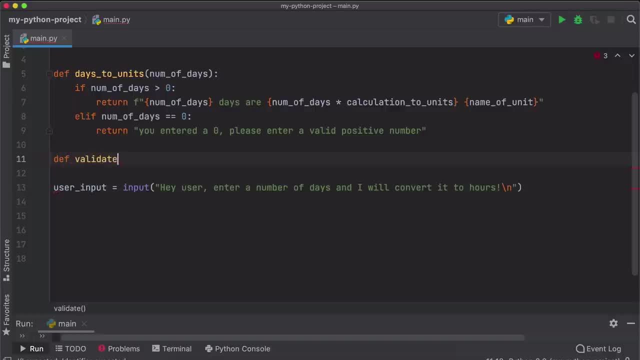 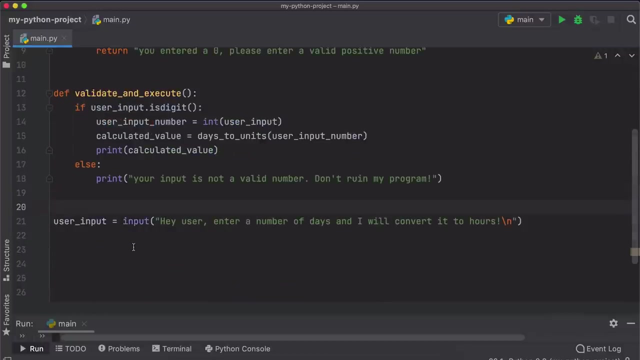 And let's call it validate and execute or something like this, And all the logic that I copied will be just simply pasted in that function like this. So now we have that logic nicely encapsulated in its own function. But, as you know, when we create a function, we have to call that function. 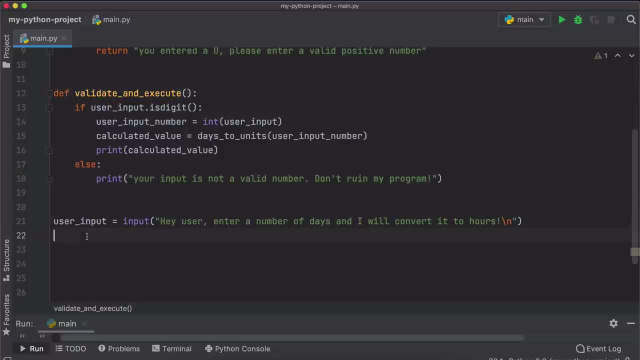 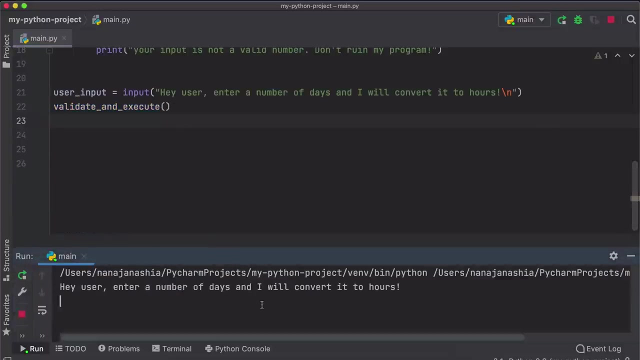 Otherwise nothing happens. So we're going to call it right here. We don't have parameters and we don't have to provide a user input, because user input is a global variable, So our function has access to it. Let's actually test it out. 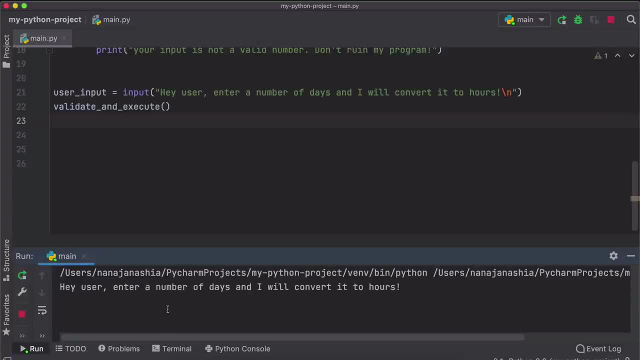 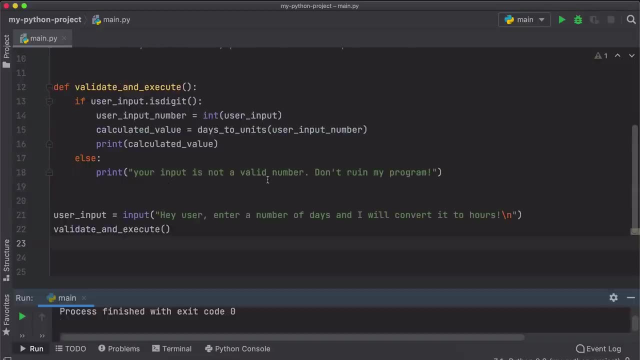 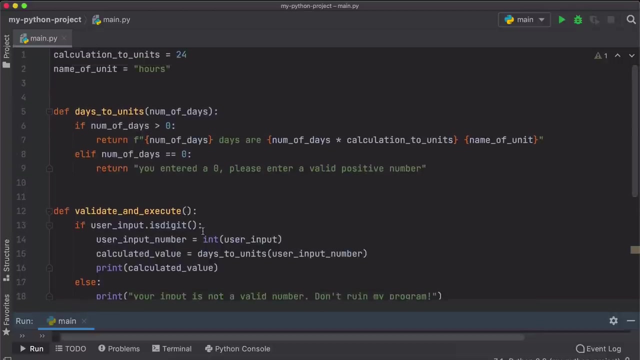 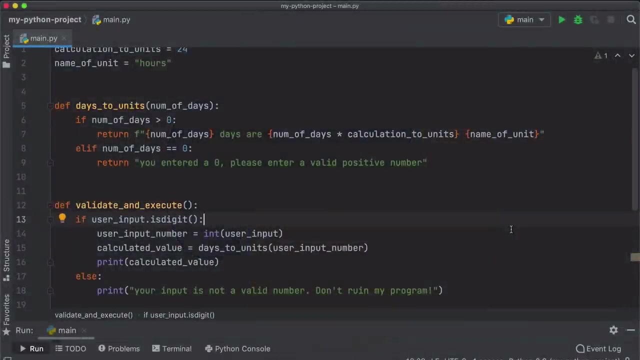 And it works. And let's provide some bad input- And it works too. So that's actually a proper way of writing code: Having every piece of logic in its own function with a proper description for the function. Now, as a next step, I want to show you also a concept or something that you will encounter very often in code which is nested, if else statements. 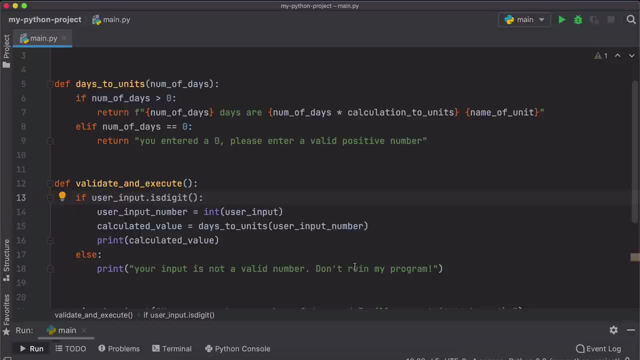 And I'm going to show that example by cleaning up our program a little bit. So, as you see, here we're doing validation intuitively. So we're doing validation in two different places. So we're validating user input here, but also inside these two units function itself. 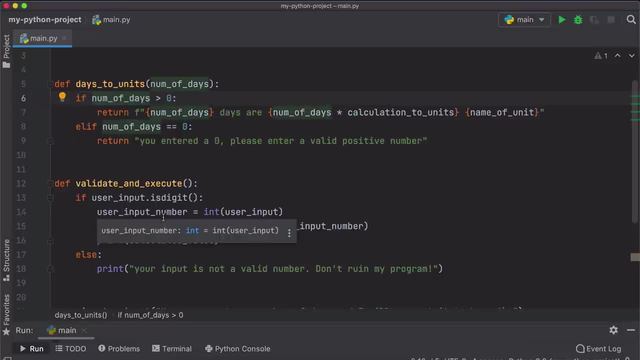 So what we can do is we can put all the validation in one place in this validate and execute function and basically have all the validate logic in here and let the days to units function just do the calculation and not the validation, And this way our functions and code will be a little bit more accurate. 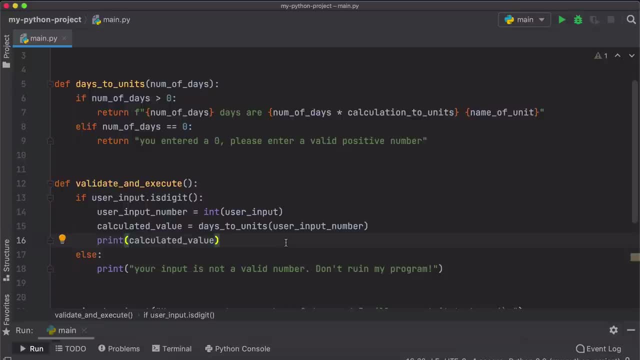 And that's what we're going to do. The code will be a little bit cleaner and more logically built. So, after we validate that user input is digit, we converted into an integer. So right here we have an integer value of the user input, so we can actually check whether that integer value is greater than zero or equal to zero. 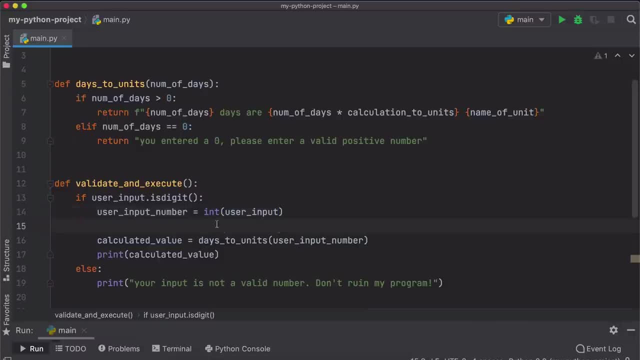 And we can do that right here, without passing it on to the days to units function And just like this. So we can do that. this if conditional, we're going to do user input number greater than zero. If that's the case, 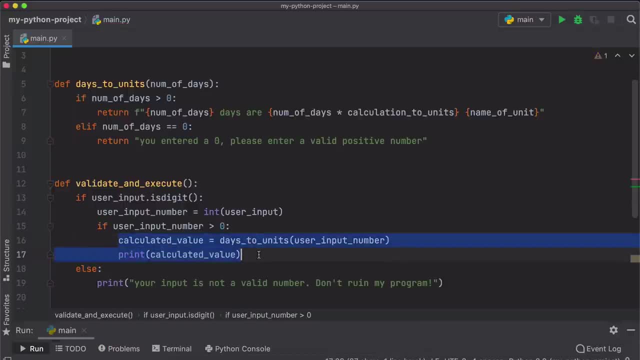 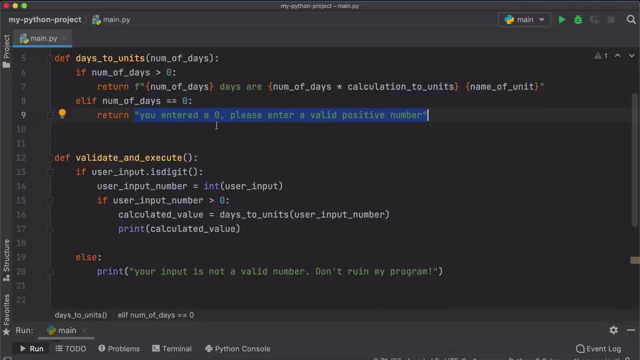 we want the calculation to happen, So both of these lines will get executed only if user input number is greater than zero And else, in our case, if it's exactly zero. we want to print a message to user: you entered zero And remember we've got the negative numbers already covered using 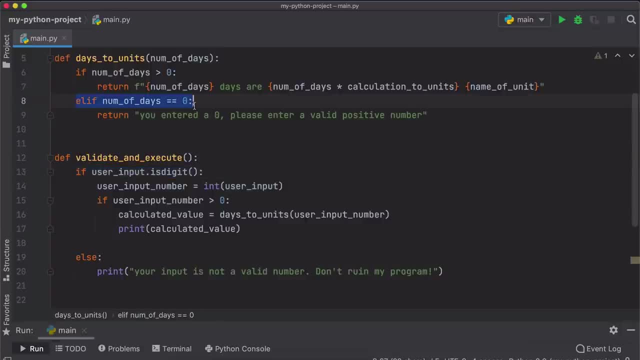 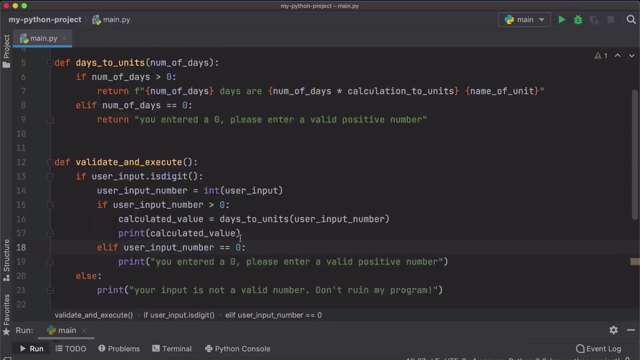 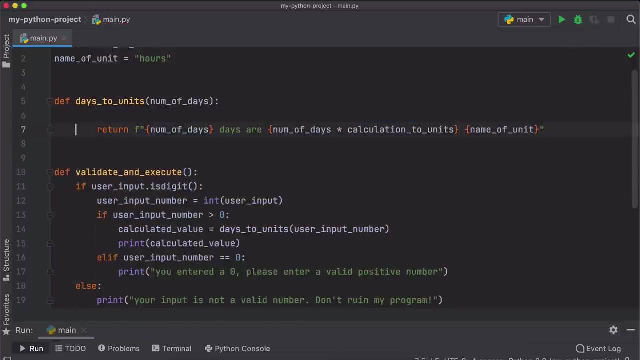 this condition here, So that's the one remaining. I'm just going to copy that and paste it right here. Variable is called user input number, So we'll fix that And we're going to print out that message. So that means we don't need any validation right here. We can simply do the calculation. 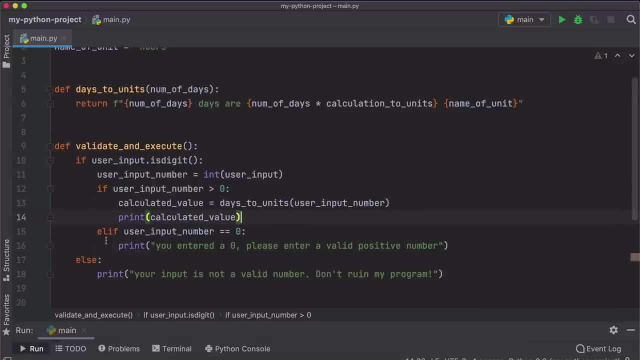 So, to go through this logical flow of if else or nested if else statements, we have the first if right here Also note that indentations for this if else. So basically they are on the same line here, same position, And the nested if else, or in our case, if they're also on the same. 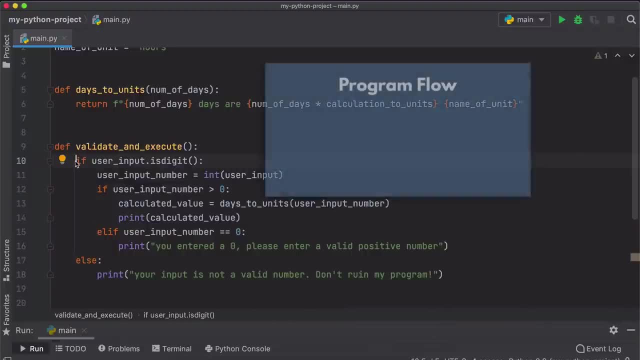 position. So again, first, that's the big validation. The first one is: is the user input digit in the first place? If not, we basically shut down the program. We print out a message to the user and that's it. If it is a digit, then we need additional. 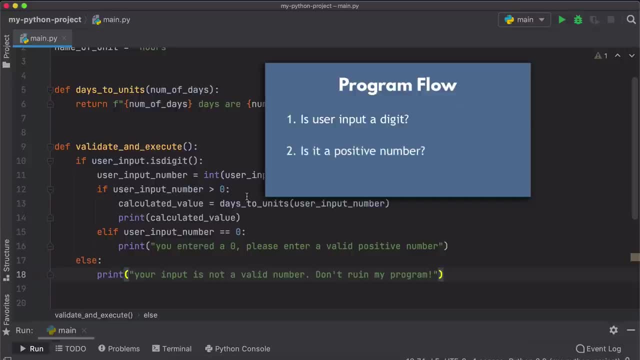 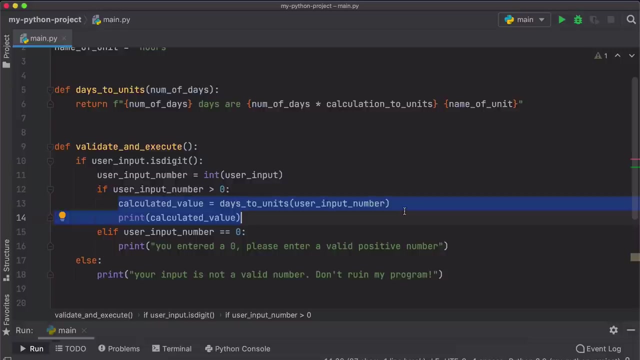 validation: Is that digit a positive number or is it a zero? So we do that additional validation using a nested if else statement And basically this line gets executed only if it is a valid number, If it's a positive number, And because of that we don't need any additional validation once. 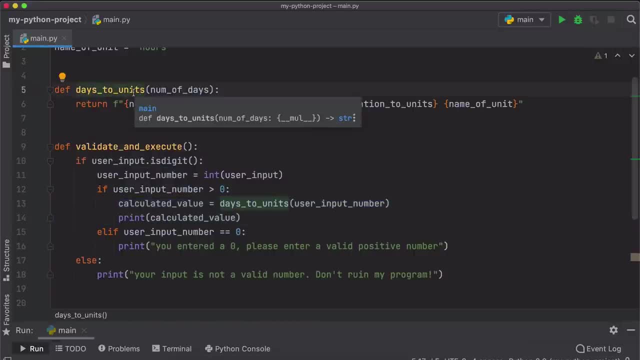 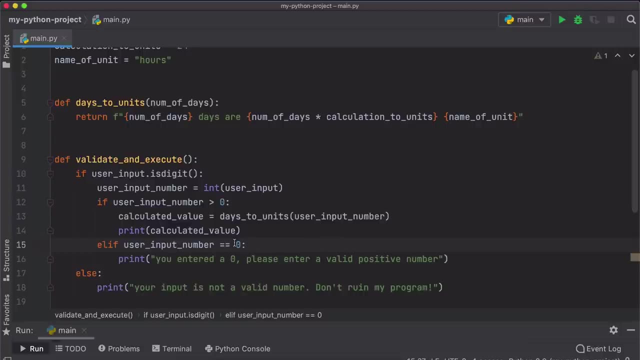 the days to units function gets called, And you probably already think and notice that nested if else statements are not the most beautiful thing in the world. They're pretty ugly actually, And especially if you have multiple of them or multiple else ifs in between. 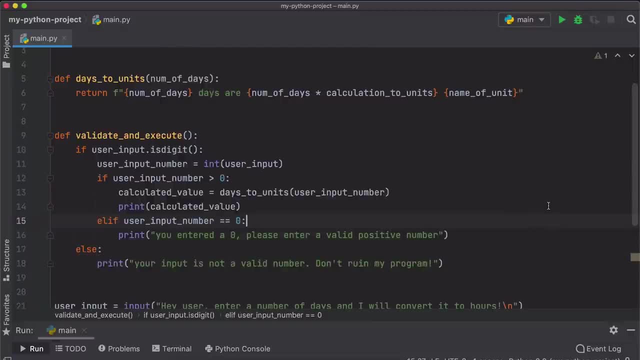 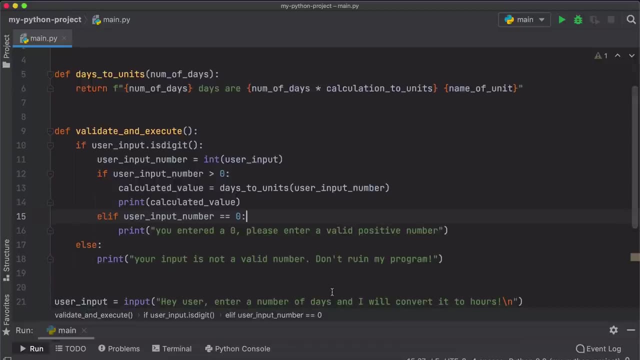 the function may actually end up looking pretty bad, So So it's not recommended to have multiple levels of this nested. if else statements in your code to basically just keep it clean. But, as I said, you will encounter it a lot in programs in application code, because sometimes you just have to write it like this: 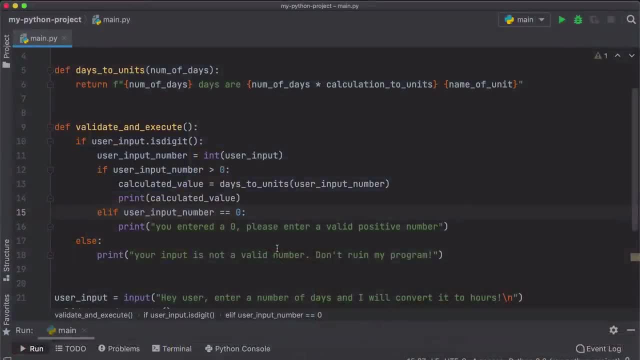 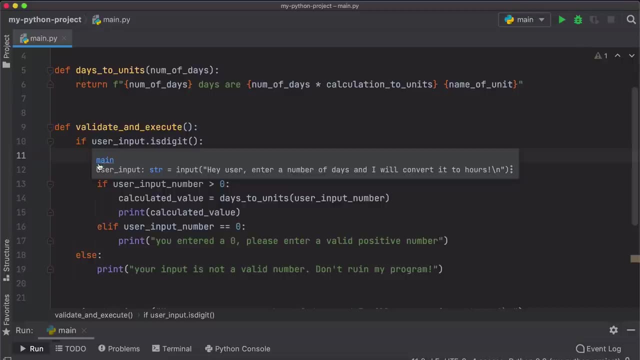 Another thing I want to show you here is something called a try, except in Python. So right here, as you see, we're validating User input, right, And then we're executing this part of code only if that condition is true. What if we had logic here where there were multiple places where something could go wrong? 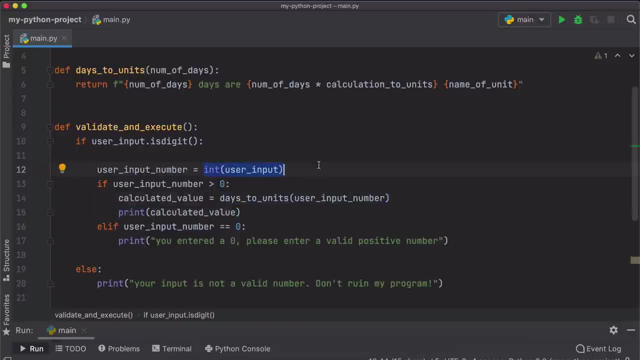 Let's say a function execution could basically just blow up because of a wrong input or even, as an example, maybe this is digit doesn't actually cover all the use, So maybe there is a value that user can input that will still blow up our progress. 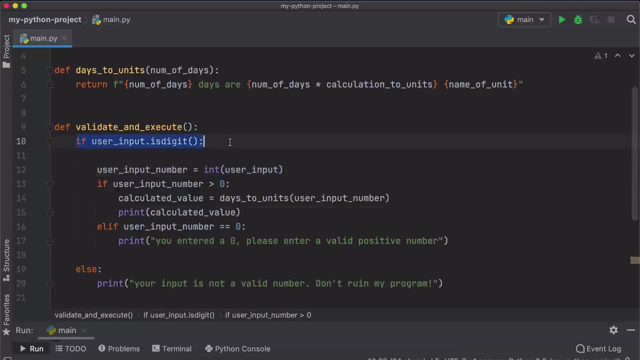 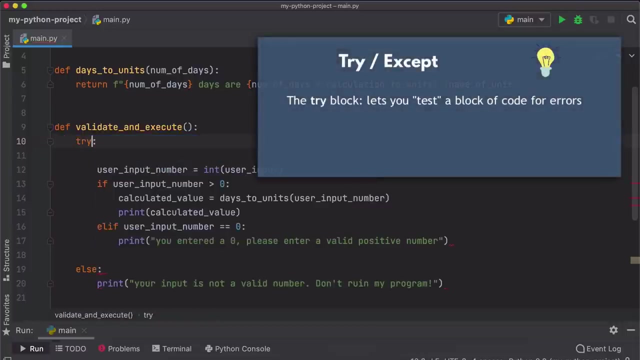 So, instead of checking each such possible scenario using ifs statements and then doing the actual calculation once all those things have been validated, what we can do instead is basically tell Python something like: Try executing this part of code here and if something goes wrong, 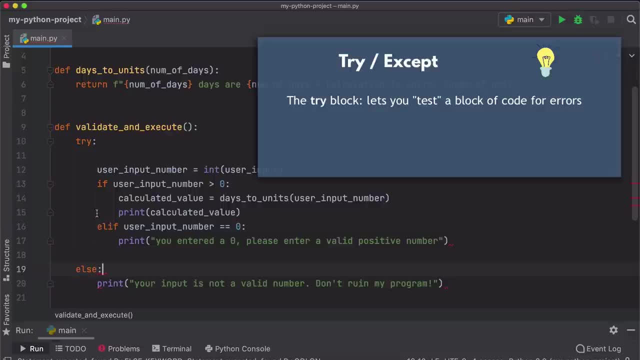 Let's highlight the function. something goes wrong. So if any line, any function call or any logic execution fails, we want to catch that error and we want to control what happens with that error ourselves programmatically, and then catch logic will be except and we're going to specify what. 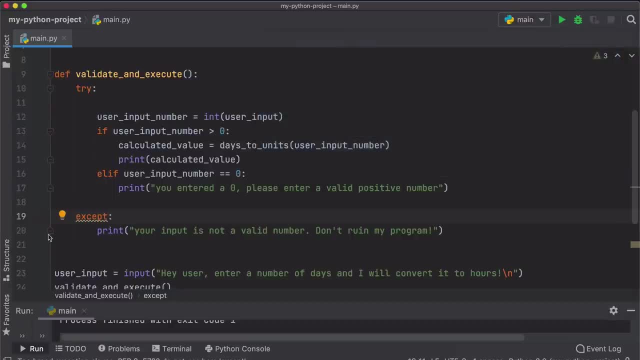 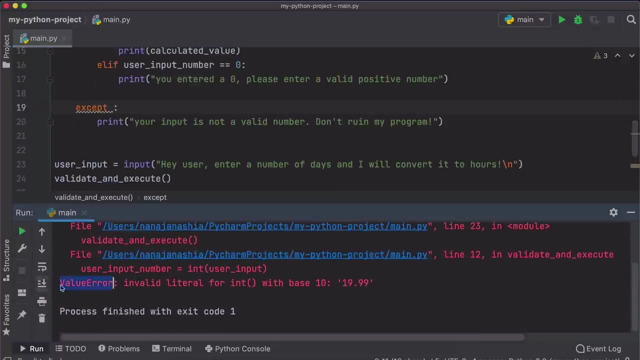 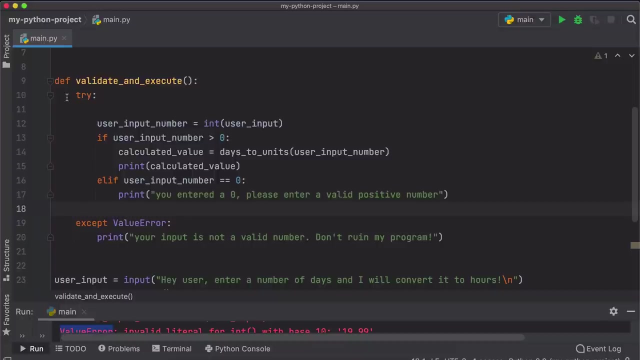 type of value we want to catch, basically using this block, and the name of that error type is actually what we saw in the output when we provided some text and a float, which is value error. So that's the error that we want to catch basically. So again, we tell Python: 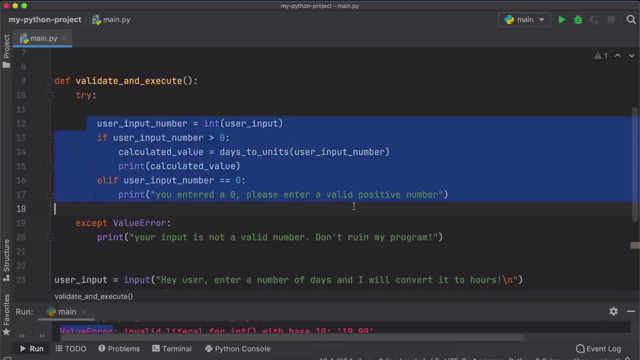 you know what, Try to execute this block of code here, And if one of those lines in that code results into a value error, then instead of just crashing the program, basically catch that error and print out a friendly message to a user. So 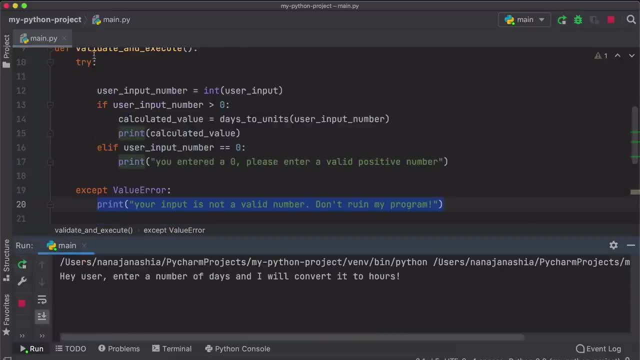 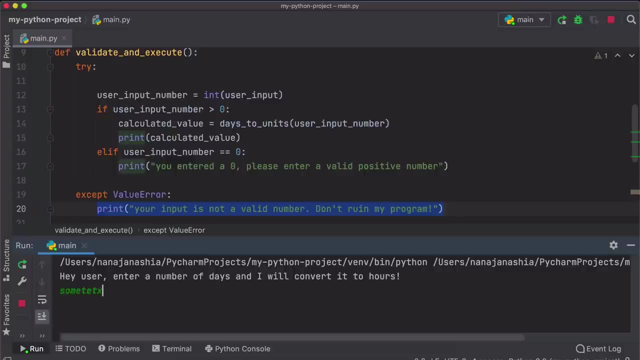 let's actually try this out and know that try doesn't have any validation, like if statement. So when I entered some text here, int function will actually be called With some text and it will result in a value error and this block will then handle that. 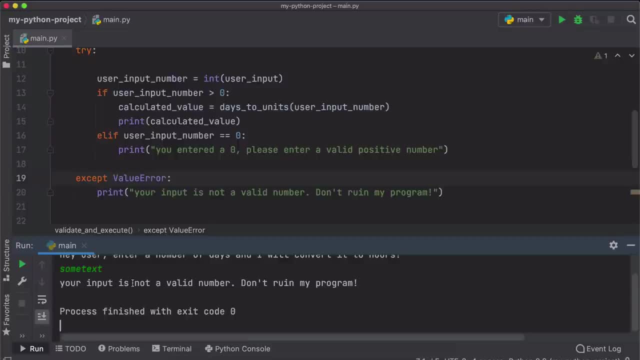 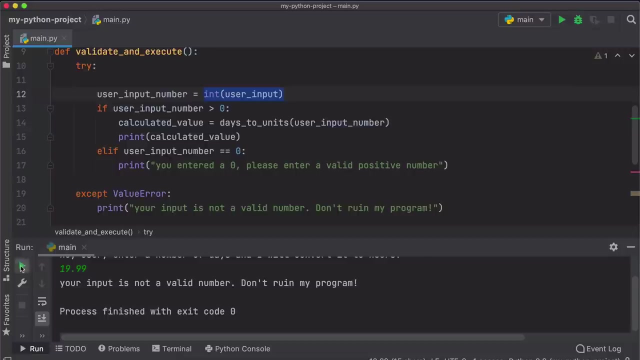 error. So I'm going to enter: and, and you see that your input is not a valid number. message got printed and the same will work for a float number. This is little noodle here. and you see that your input is not a valid number. message got. 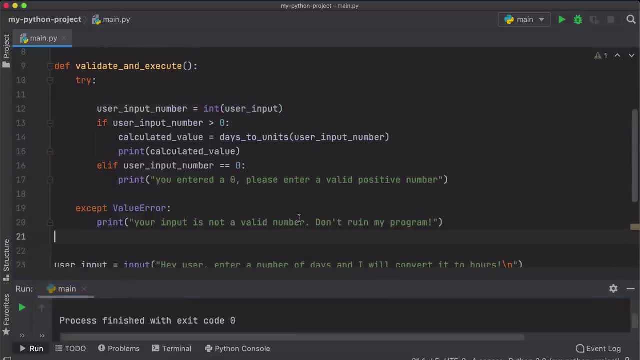 printed and the same will work for the number That also doesn't convert to integer and for proper integer value it will work. for just this small value will work fine. And again, difference between if L statement and using try except is that 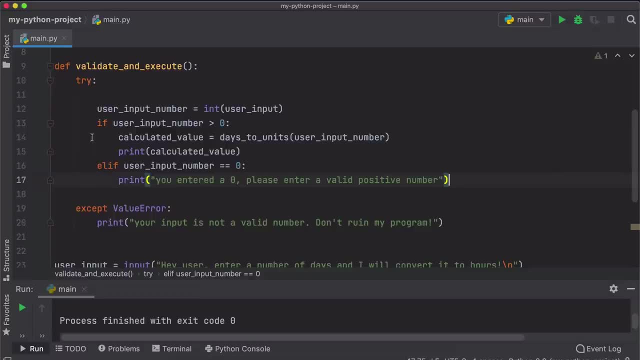 you can cover multiple such errors with this whole try except block Right. So you don't have to do the validation specifically, And that is especially useful for cases where you can't really validate something using if condition Right, If there is a chance. 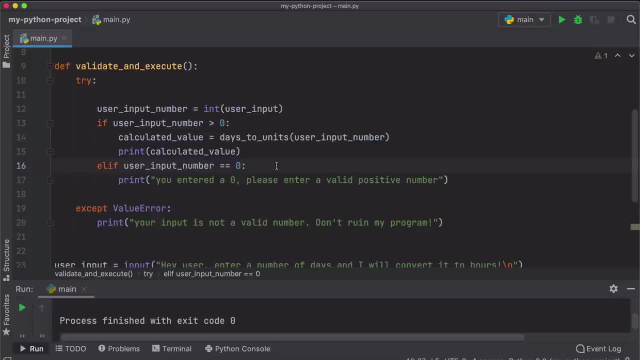 that you might miss something in that condition check. So basically you just say you know what, just try to execute with whatever value And if error happens, then I still got it covered. And an obvious difference between this, if else, is that here nothing actually. 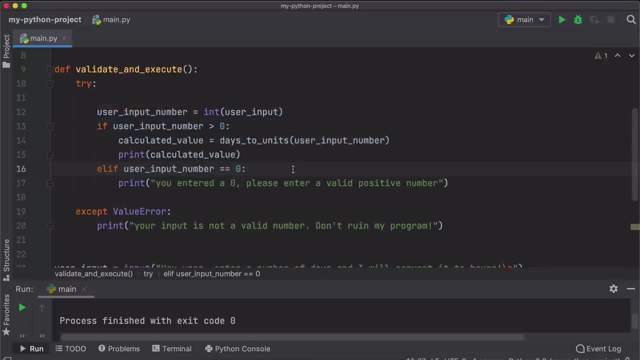 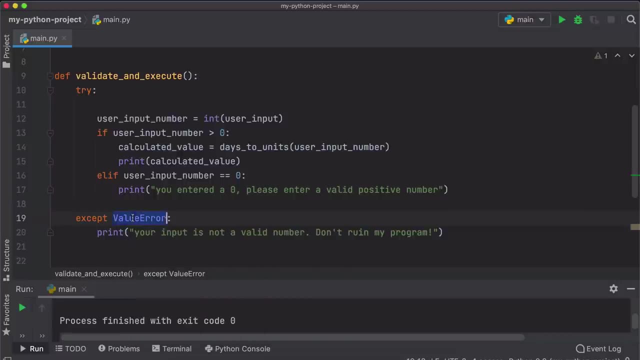 crashes the program, The program will still work. It's just a nonsense value with zero days, Right, And as you see here we have specified an error type, But with try except, what can also do is you can basically say: you know what I want to cover any type of 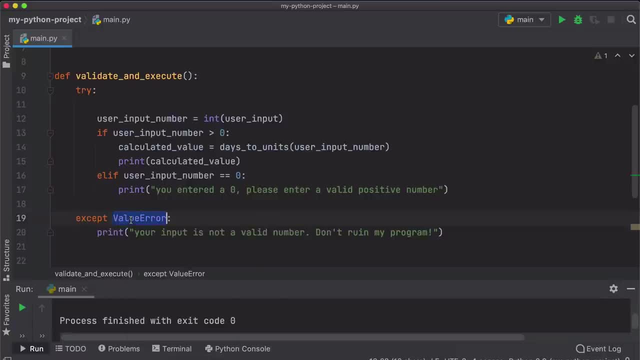 error. I don't care if it's a value error or some other type of error. Let me handle any type of error. In this case, you can basically just leave it without a specific type. You get a warning, though, that it's too general. However, this would work and you will be covering. 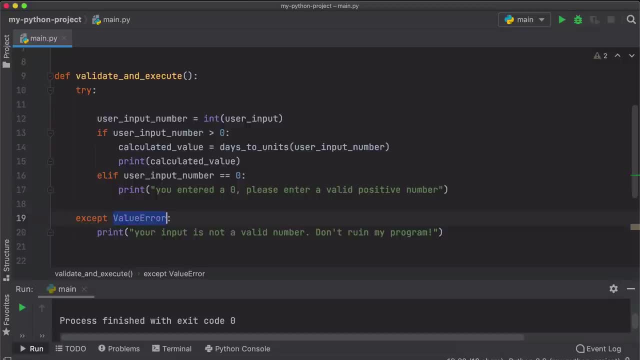 all the cases with it. But we can go back to our value error and know that in many programming languages this is actually called error Try catch. So except is actually pretty specific for Python. I personally think try catch makes more sense because you are catching any error that may happen right here and then basically, 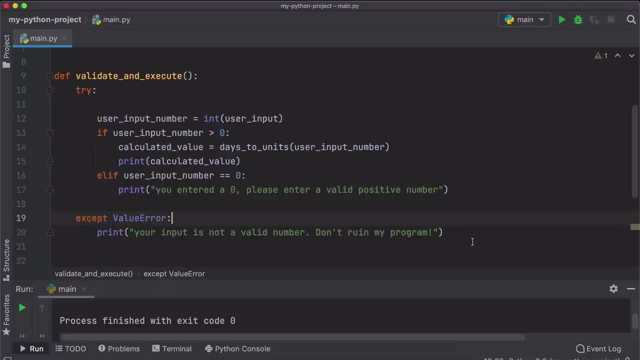 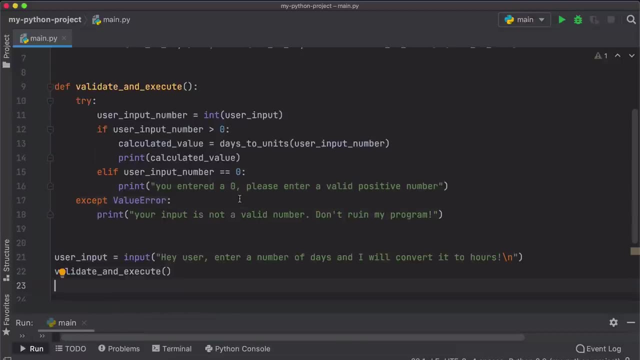 handling it in the catch block. So if you happen to hear or see try catch in other programming languages, note that this is the same thing as try except in Python. One thing that we're missing, because we converted that if statement into try except is now we're. 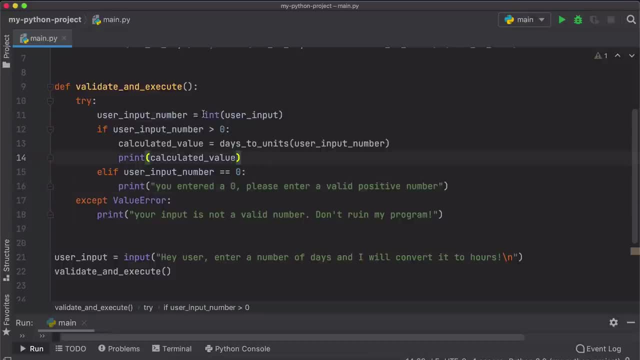 in. So we need to validate the negative numbers again, because negative numbers will not cause an error in our application, So they're not covered by this, except block here. So let's add back our previous, else block. And again, if neither of these are true, it means automatically. 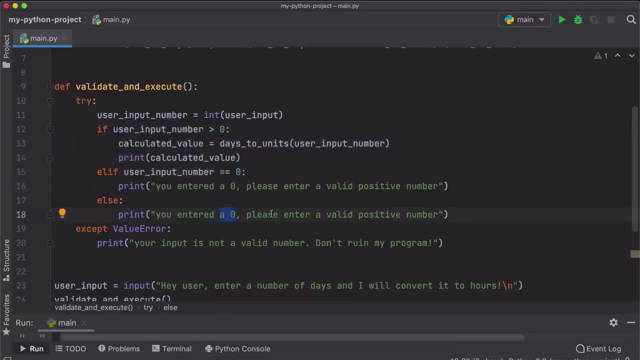 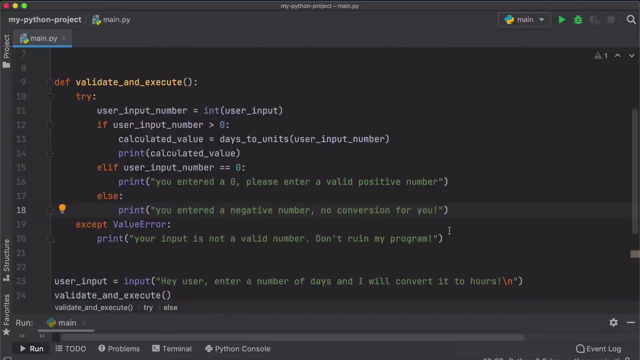 would mean that it is a negative number. So Let's print That message for a user: Enter negative number, No conversion for you. So now we got all the cases covered again, So let's try that out. That's 10.. 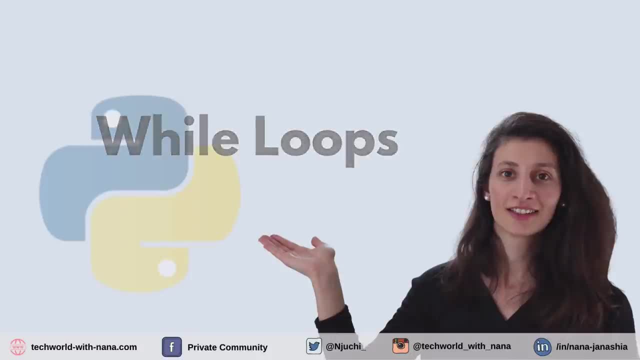 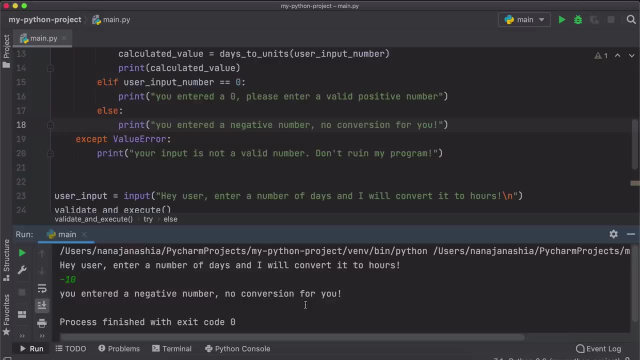 And there you go. Now there is one minor problem with our application, And that is we can only use it once. So basically, whenever we type in a value, it's Either calculated or gives us a message that we provided an invalid value. then the program basically exits. 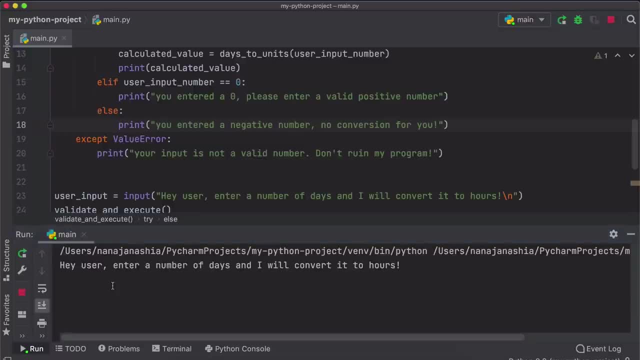 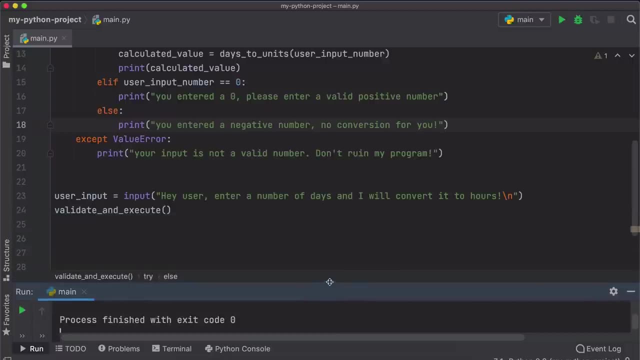 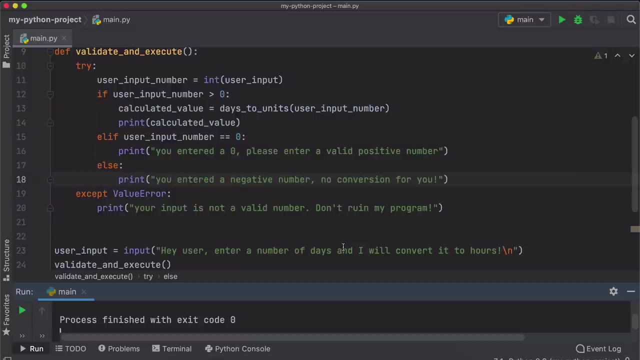 So if we want to do a calculation for another value then we have to restart the application provided a value and then do the same. So that's not very convenient if we want to use that program to basically Calculate a number of hours for many different values. 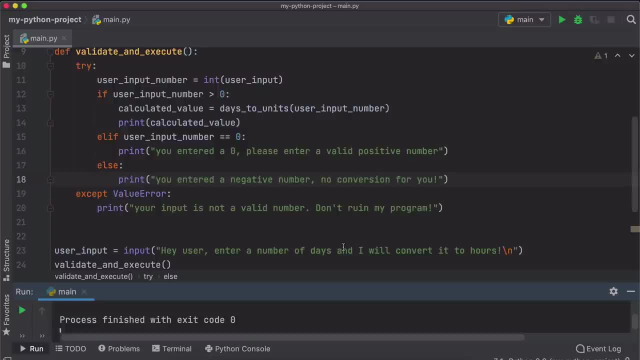 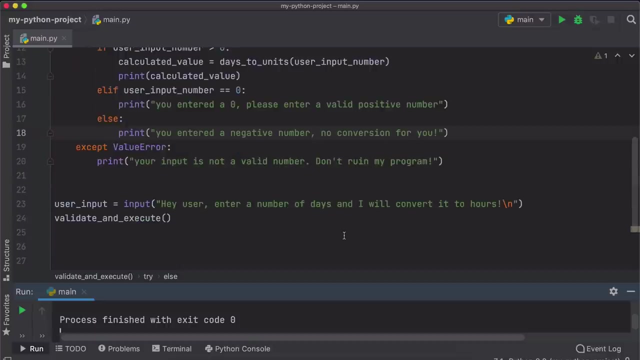 So basically we want to keep feeding it some different values for calculation because we don't want to restart the application over and over again. So how can we actually make the program continue after it's calculated the first value? So we want the program to basically just keep running and accepting our values. 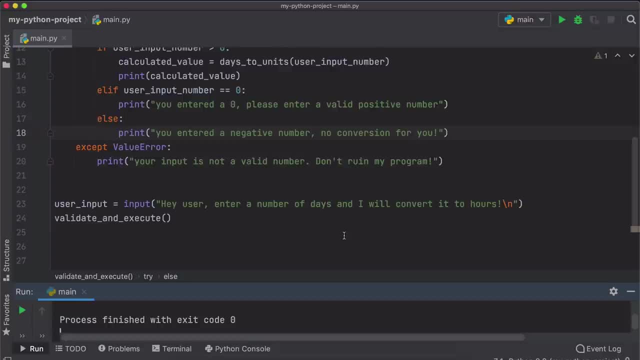 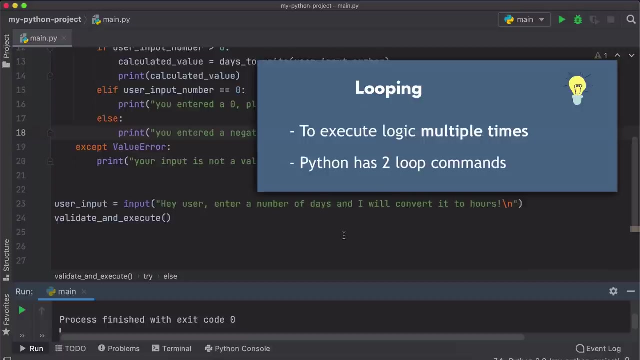 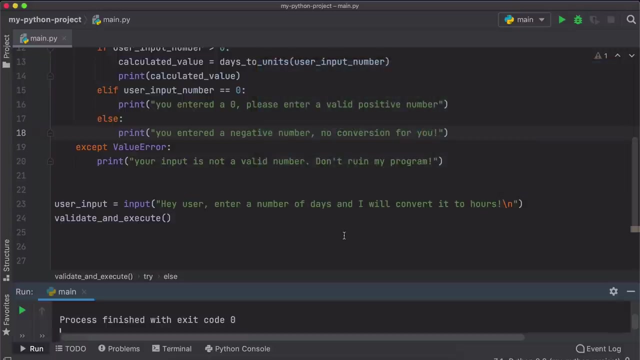 So how do we do that? And we can Implement the logic using something called while loop. concept of loops in programming is basically: you do the same thing, So the same logic gets executed multiple times in a loop, And how many times that logic gets executed is basically defined in the condition of that loop. 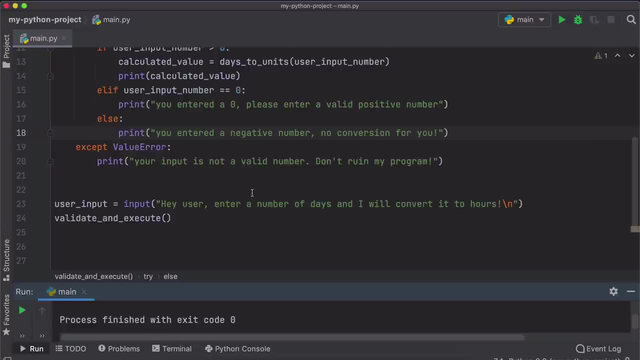 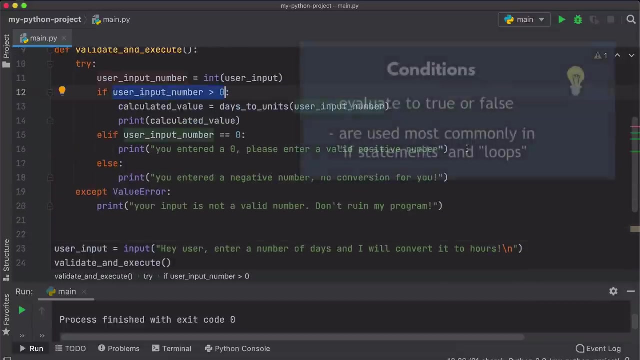 And the condition could be it should run ten times. or condition could also be It should run until some specific event happens in the application And conditions you already know from if L statement. conditions are basically logic that gives you either true or false. So condition is checking some logic and then giving you a result which is either true or false. 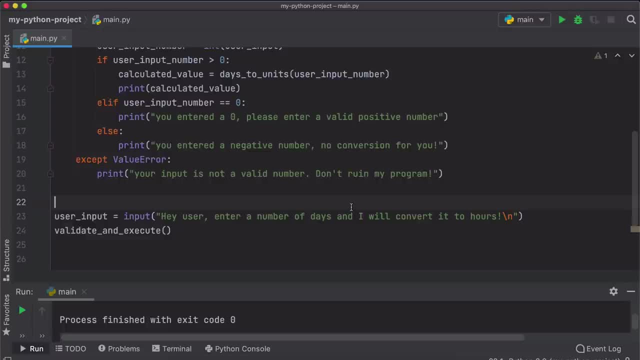 So now the question is: how many times do we want this application to run? in our case, Let's say we want to run indefinitely, Right, Until we actually stop it from here, until we kill the program. So it means the condition for that should always be true. 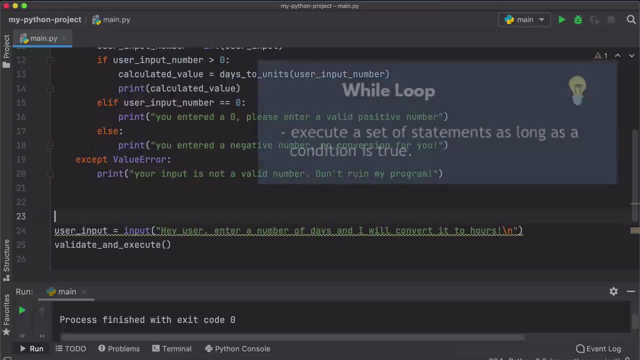 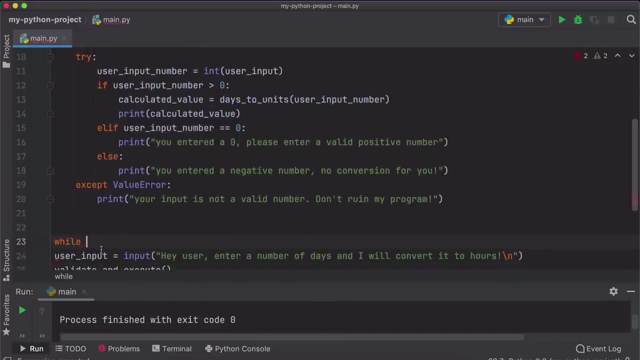 And for our application we're going to use a while loop, which is one type of a loop and very simple syntax: while, and while just like if actually takes a condition. this is going to be the condition for the loop. So, basically, we want to tell: 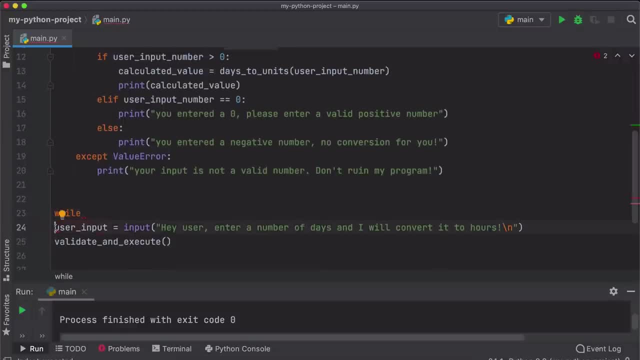 The while loop, How many times it should run the logic coming after it? And again, you know our familiar indentation: these two lines should execute in a loop over and over again, with some condition right here. So how many times do we want the program to execute in our specific case? 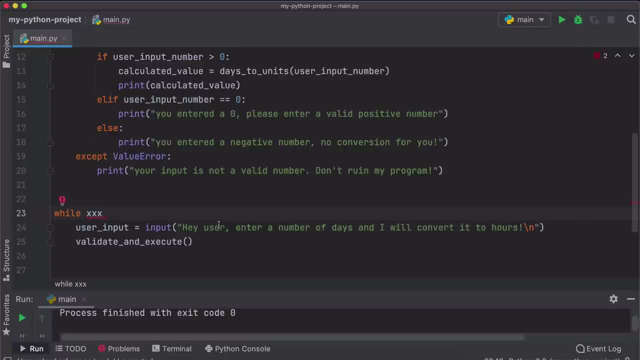 Well, when the program to run indefinitely until we actually stop it from here, Right Until we actually stop it from our editor. So that means that condition of the loop that decides whether the next lines should get executed or not, in our case should always be true, because if it's false, then the loop will stop. 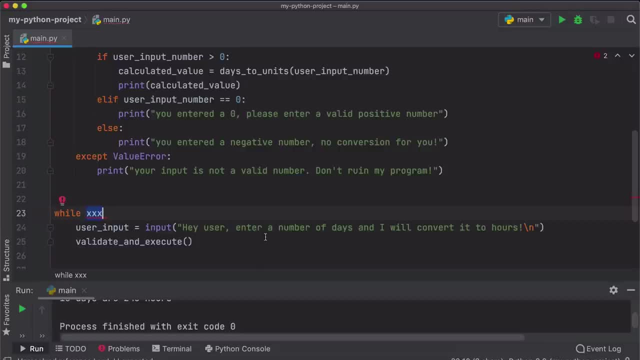 Right, No execution anymore. So how can we make sure it's always true? We just write true right here. And you remember I told you that In programming languages have their own data types. Well, they are also reserved words, even though this is just text representation. 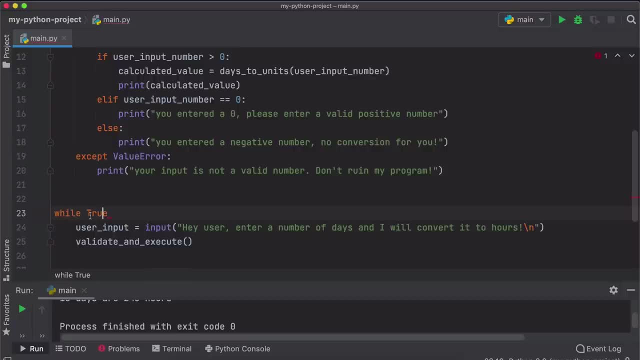 Basically, you see the highlighting here, just like for these other words, because Python knows this is a Boolean value of true. And note that again, specifically for Python, we actually write true with capital T, unlike in other programming languages. So this will basically be. 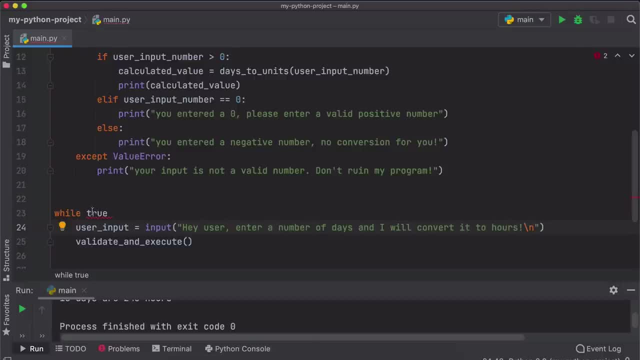 True, True, Just a string, So Python doesn't know what to do with it. but it recognizes true with capital T. So we're telling our loop Our while loop. the condition is always true. So basically run these two lines indefinitely, because the condition will never change. 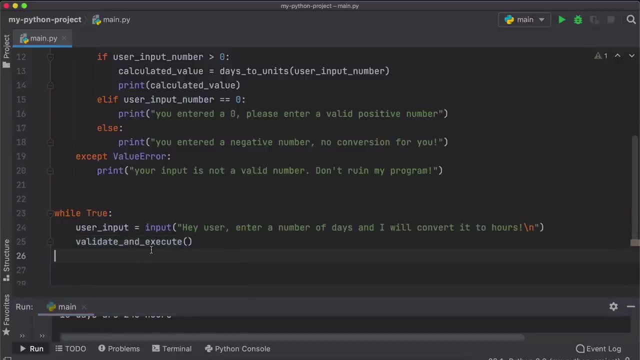 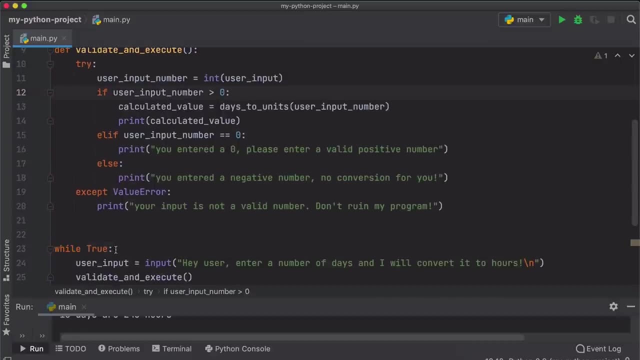 It's always going to be true, And the syntax is probably already familiar to you. We have the keyword, just like if or try. we can actually compare this Syntax to the if statement. So we have the while keyword here, then we have the condition. 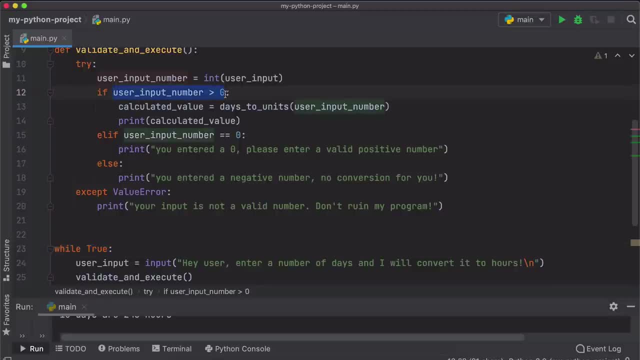 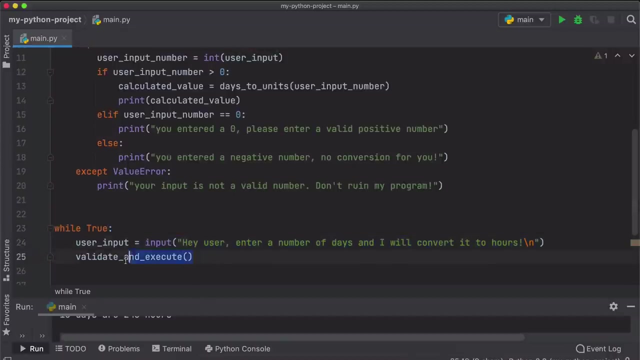 So this is the same type of condition as this one right here. It's just that with us is basically fixed true value. here It could be true or it could be false, based on the condition. And then we have the colon, and then we have the indentation for the next lines. 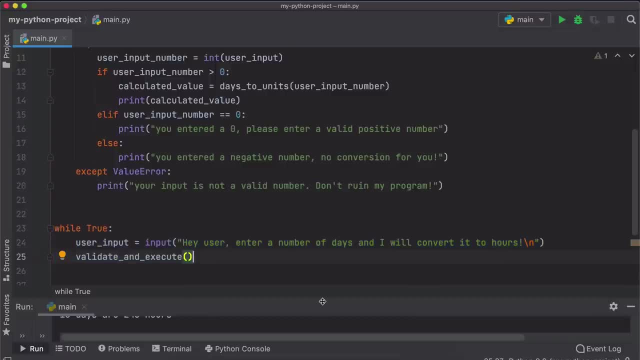 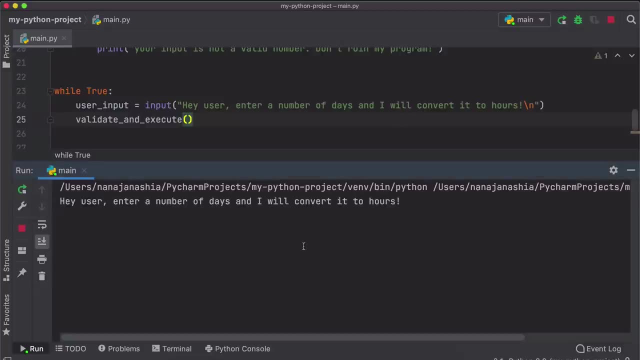 So all of these belong to the while loop. So that's basically it. We can now Execute the application and see that our program runs indefinitely. So this is the first one. Let's say we entered 10.. Awesome, We have a result. and then we have again the next execution where it's asking for our input again, and we can do minus 10.. 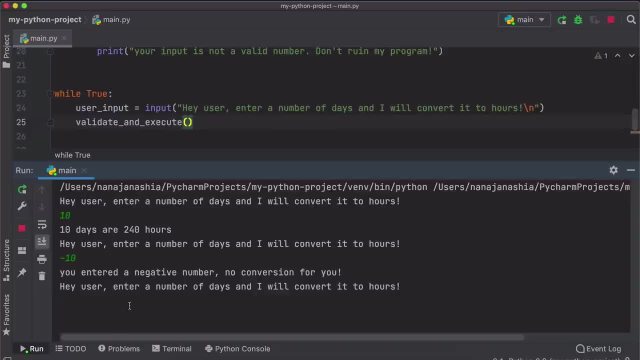 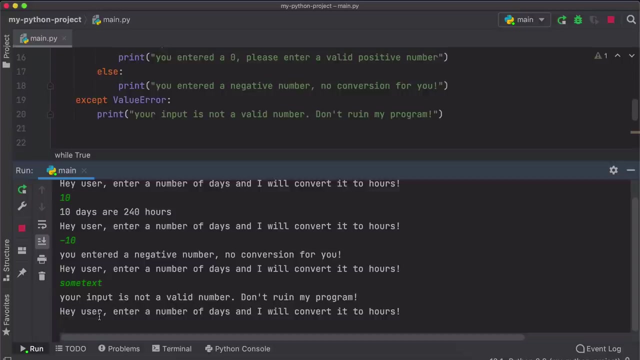 Now it's telling us we provided negative value, but we can enter the value again. Let's enter some invalid value. that should be handled By this value. error block: execute: it's not a valid number and application basically continues. So again, as you see, if you have an application that should continue running and basically get user input over and over again, 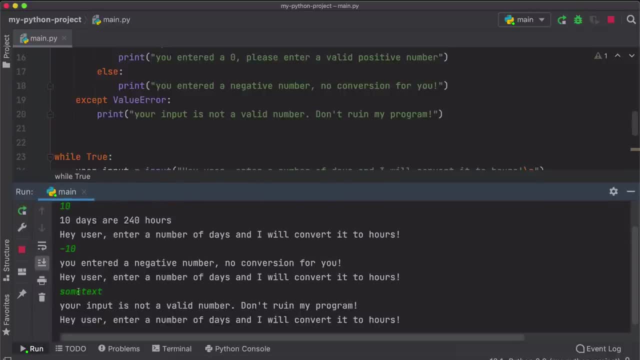 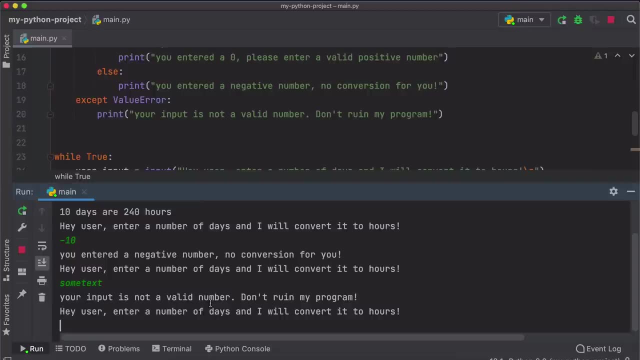 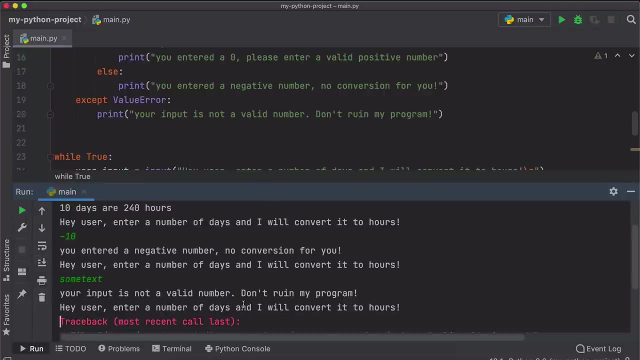 you don't want the application to be crashed at some point by some bad input. You want to catch and handle every type of input so that your application continues to run And if we want to Stop it, we can basically just shut it off here and process finished. 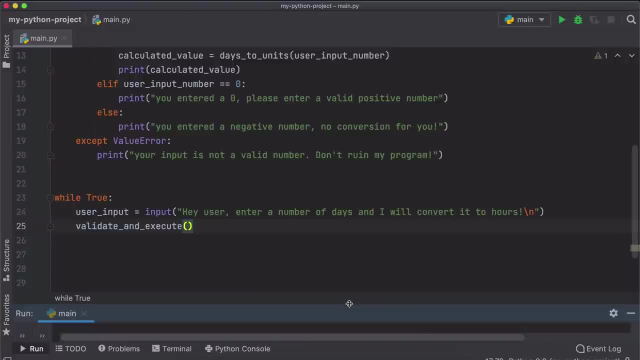 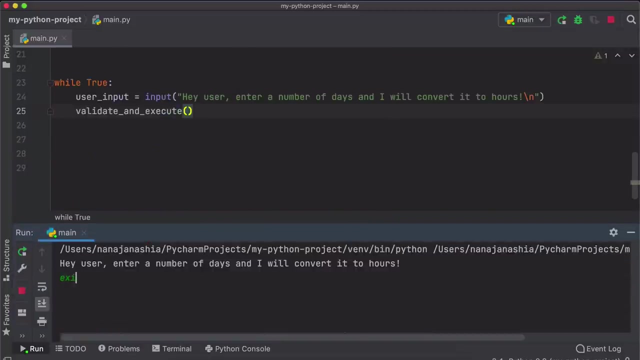 Now we can do one optimization in our program, and this would be to allow users themselves to stop the application using some specific input value. So, for example, When they type in exit, for example, the application should Stop only for that specific word, so it shouldn't run anymore. 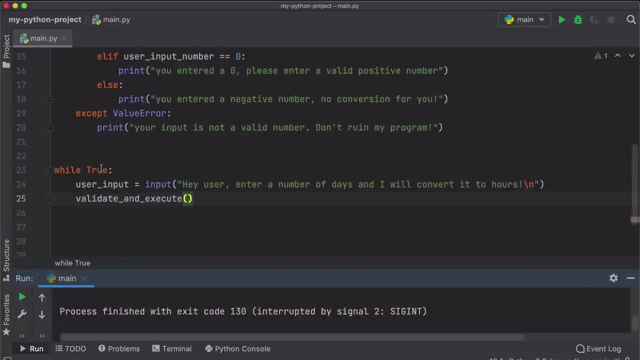 So how can we do that? So basically, instead of having a condition that is always true, we want a condition that says if the user did not input word exit, then continue running the program. If user entered exit, then basically just stop it. 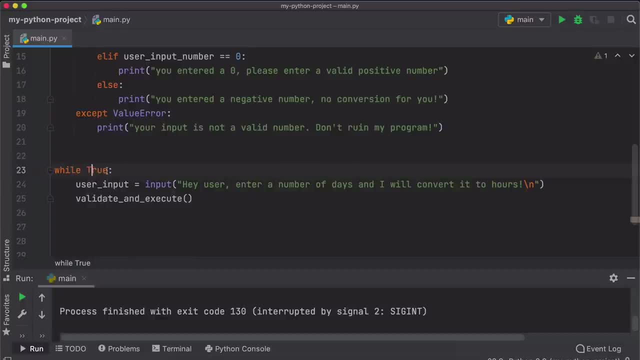 Right, So we need to change our condition right here. So here we want: User input is not exit, Right, So user input is not exit. Now, we didn't learn how to check for not equals- something Right, We have check for equality. 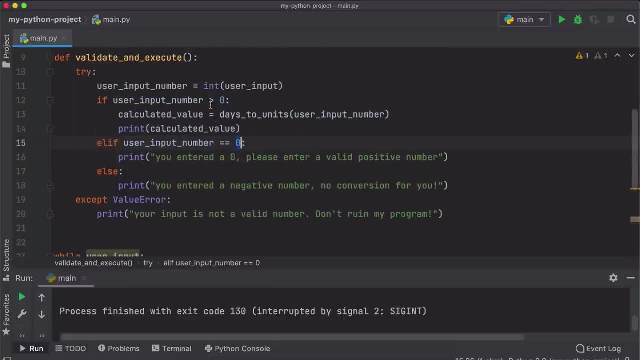 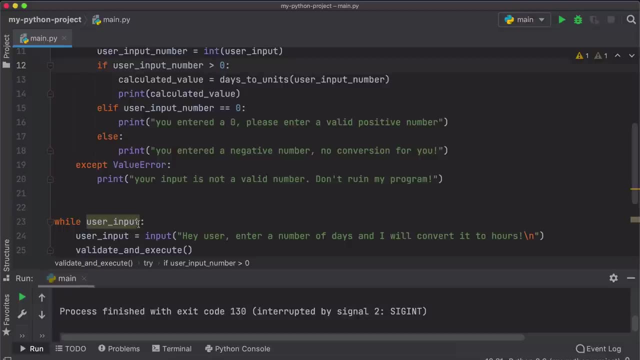 So we check whether input number equals zero, or if it's greater than or smaller than. However, we didn't learn how to check for not equals. not equals in programing- And this is Not specific, for Python- is expressed like this. So instead of two equation signs, we have an exclamation mark in equals. 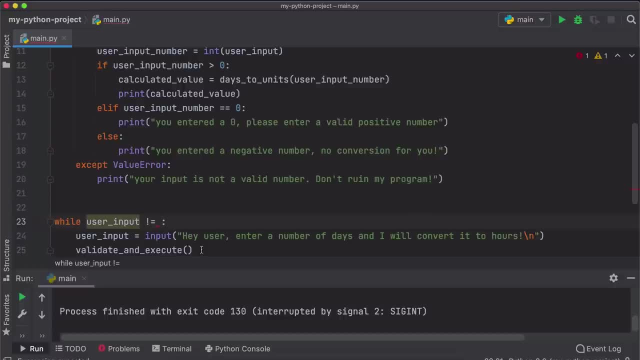 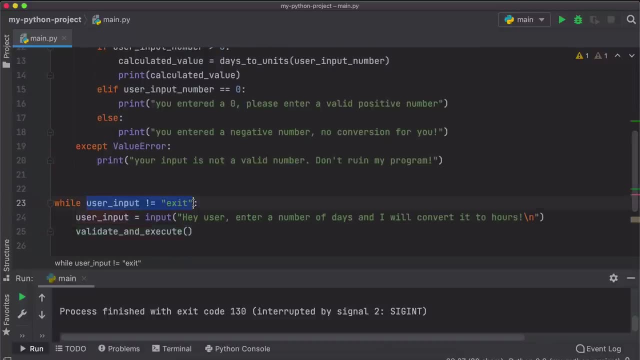 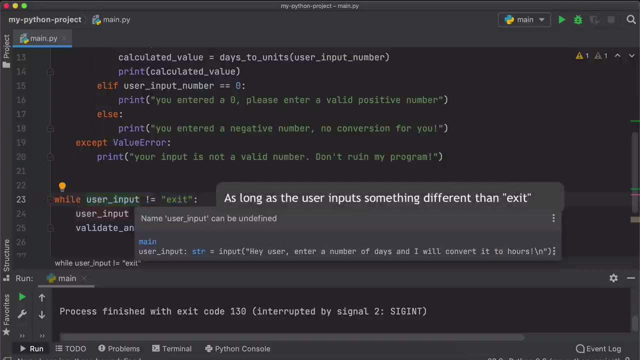 And if we want to compare it to a string, obviously we type that string. In our case it's exit. So, basically, this condition tells our while loop while user input is not exit, Right? So basically, this condition tells our while loop while user input is not exit. 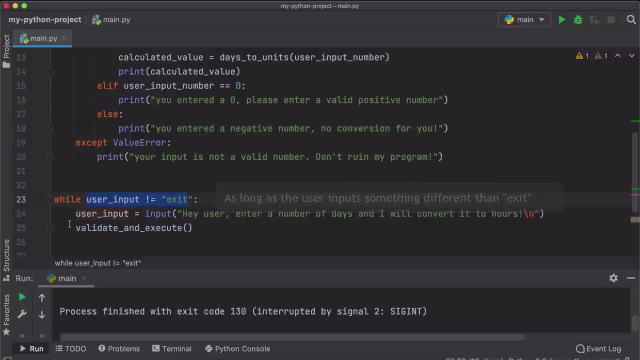 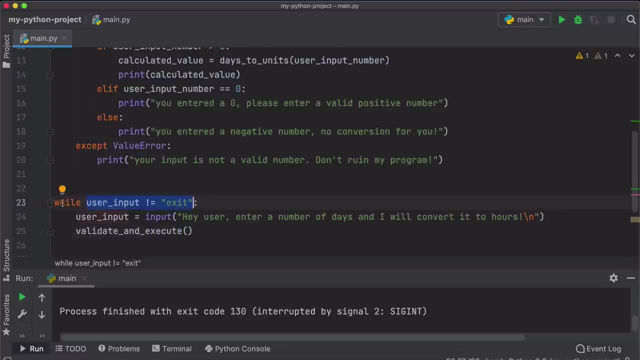 Right. So basically this condition tells our while loop, while user input is not exit, Continue running the program. So, while this is true, basically just keep moving on. But if user enters exit, this will not be true anymore. It will be false. 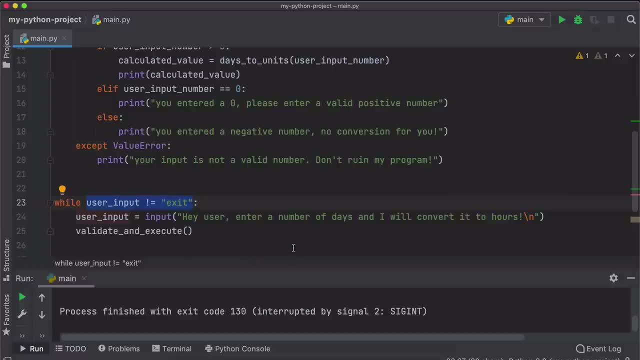 So loop will basically break and application will end. Now you see that we have a warning on this user input that we're using here, And if I hover over it, you see a message that says name user input can be undefined. So it's not always undefined, but it can be. 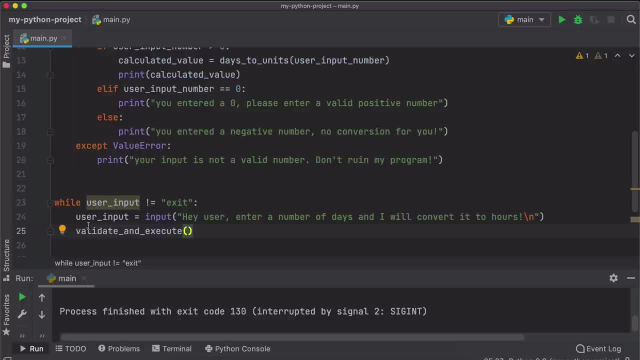 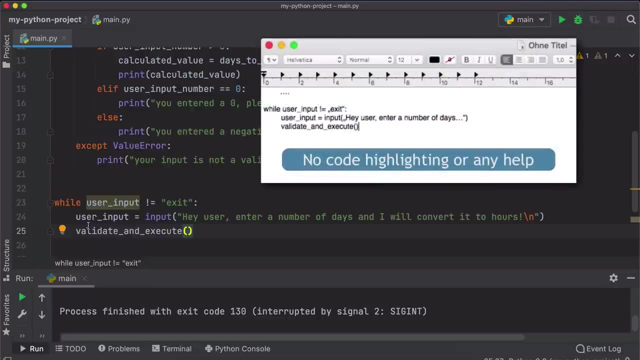 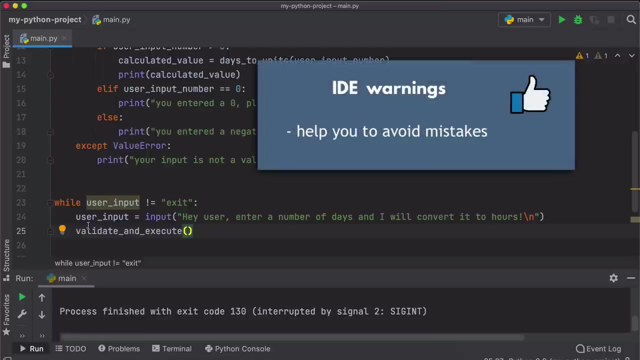 And here I want to mention again that PyCharm, because it's an intelligent editor, can give you actually this warning when otherwise, in a simple or normal code editor, you probably wouldn't get such a warning. So again, it helps you in avoiding some of the mistakes that you might accidentally make when writing code. 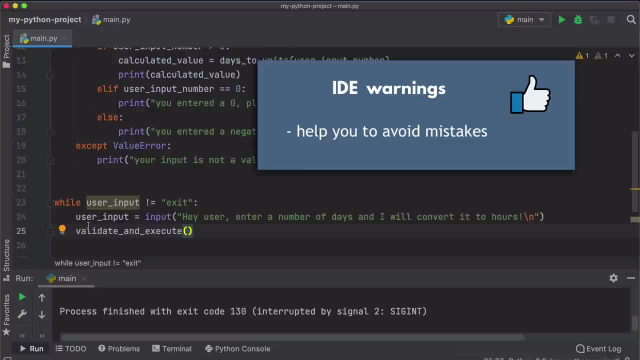 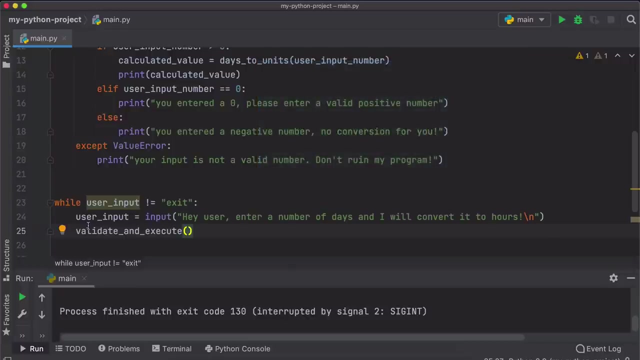 So, basically, it detects the errors or possible errors for you and tells you to fix it. So, again, this kind of intelligent warnings and error messages can be a lot of help when programming an application. And now let's fix that warning. So what's that all about? 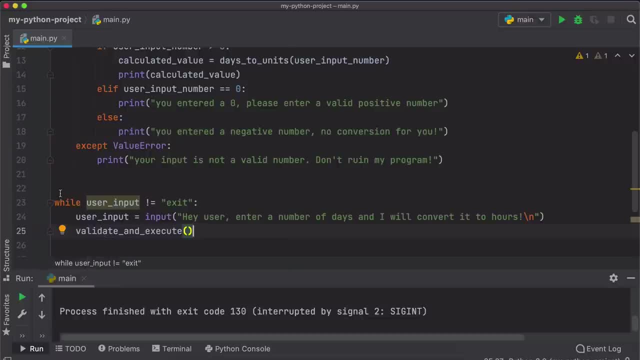 The problem is, on the very very first run of these while loop, user input variable itself will not exist. Why? Because we're creating that user input variable on this line first. our application will basically complain because when our while loop runs for the first time, 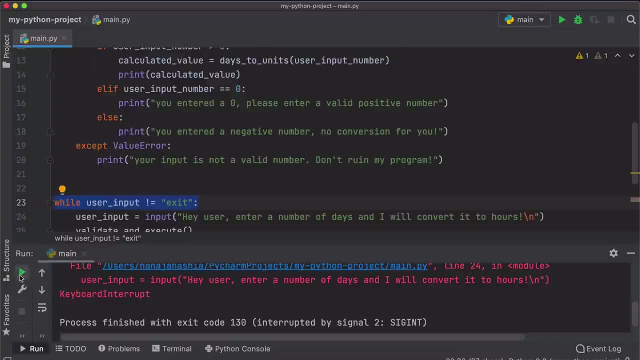 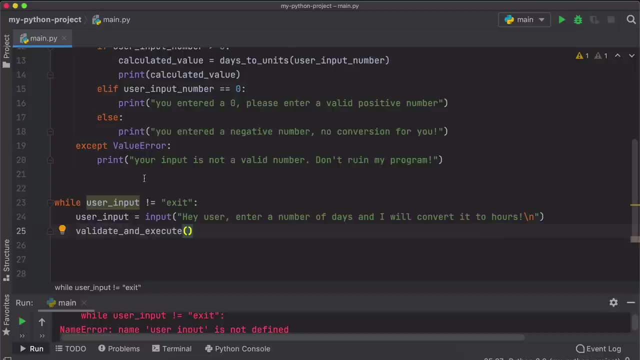 it will not be able to find user input variable. let's actually try that. and, as you see, user input is not defined, so we need to create that user input variable before the first execution of the loop. so, right here, we're going to create user input. so we're going to create this user input. 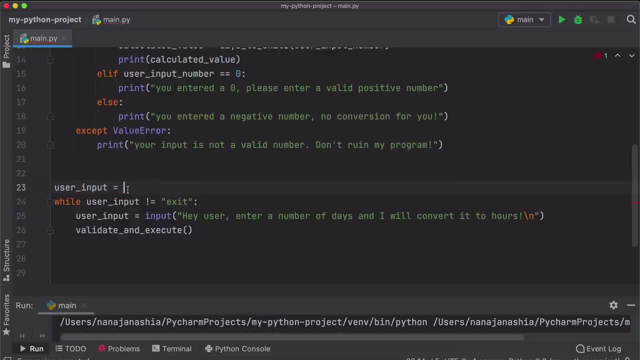 variable before the while loops first run, and it doesn't really matter what the value of that user input variable will be, because what matters is the variable exists. so the value is basically just empty and as long as it's not exit, the loop will start running and 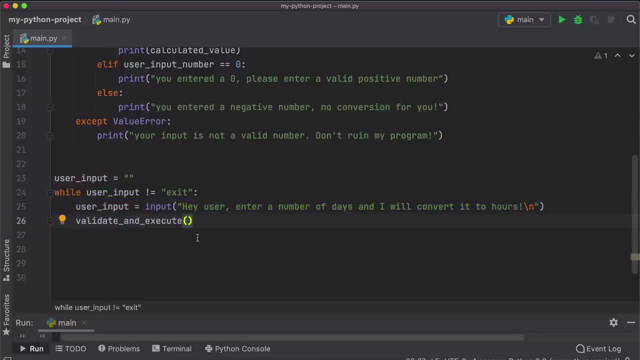 and and our application will get executed. so again, to go through the flow of this, we're creating a user input variable, then we're making sure it's not exit. if it's not, this line will get executed. so we get the input from the user. that's going to be our first input and then we call validate. 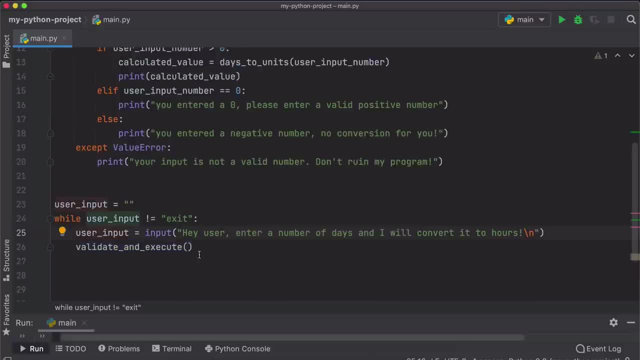 and execute function that basically does all the checks and execution. so that's going to be the first run of that loop. on the second run of the loop the condition will get reevaluated. so now the user input is what the user provided. so again python will check: is the user input exit? no cool, let's execute the program again. user will have to enter. 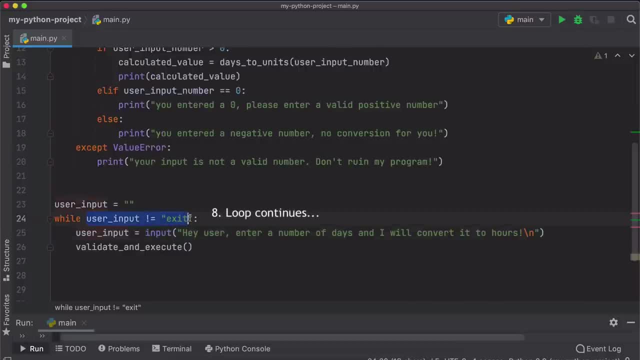 another value and then that value will get reevaluated. so note that after each time that this block of code has run and executed, every single value that user will get will get reevaluated, as an input will be evaluated over and over again. in that condition, and while user input is something, 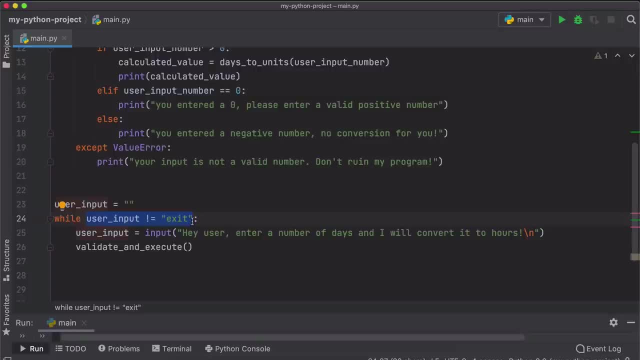 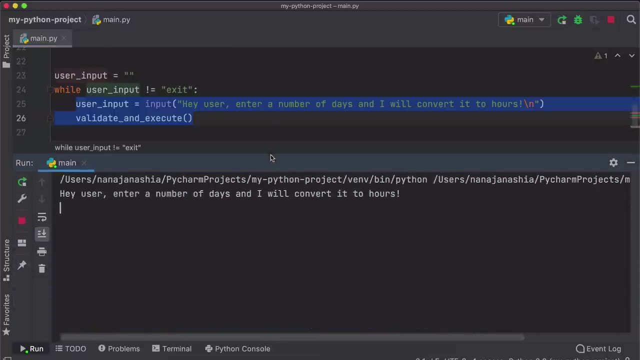 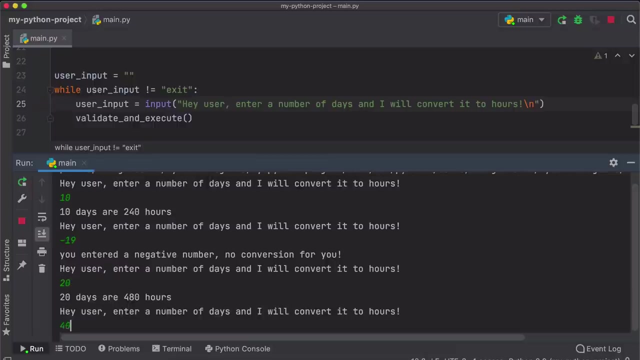 else than exit. it will run the program. if it is exit, then the loop will break. so let's actually test that. so this is our first message and our first input: let's do 10, it got calculated. let's do minus, minus, minus, minus, and we can do that over and over and over again. and now let's actually enter exit, and let's see. 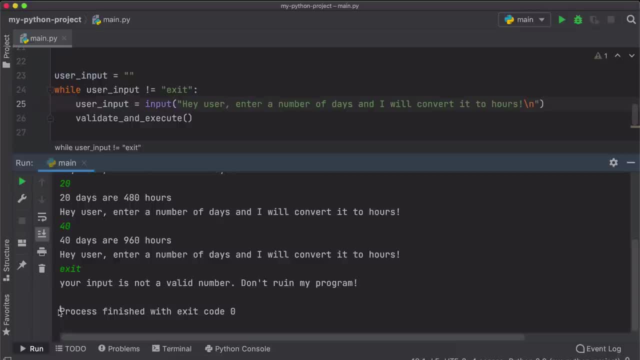 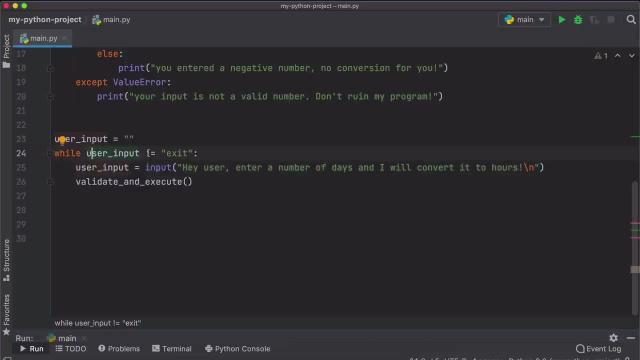 what happens and, as you see, the process finished with exit code. so our application actually stopped because this condition was not true anymore. it was false because we entered exit. so that's how we can allow users to finish the application. and two takeaways here. one is that we have to. 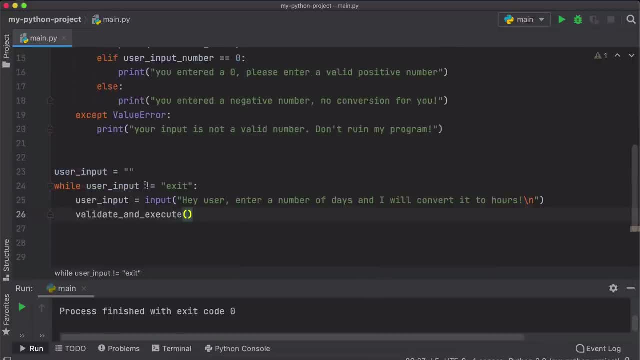 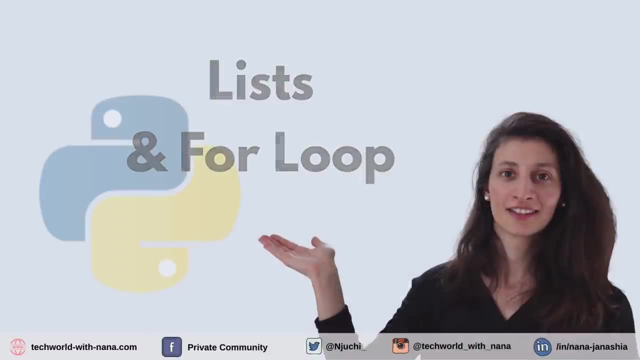 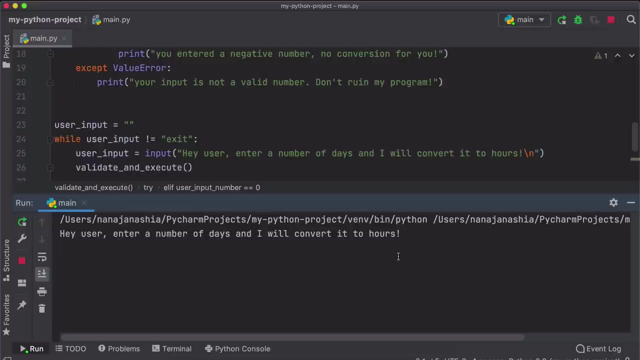 do a conditional in a loop and the second one is a negative equals check for values. great. so now we have our application that basically allows input multiple times and can be terminated with exit input. now what if i wanted to calculate number of hours for several days? but 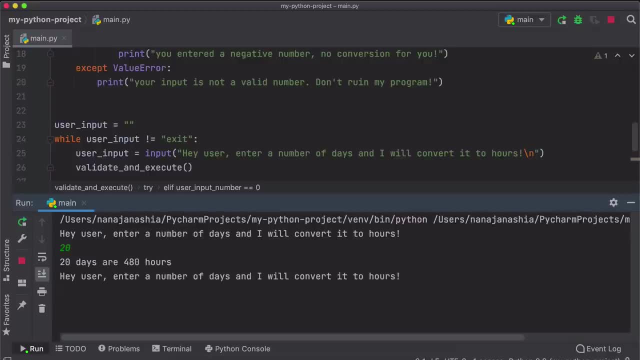 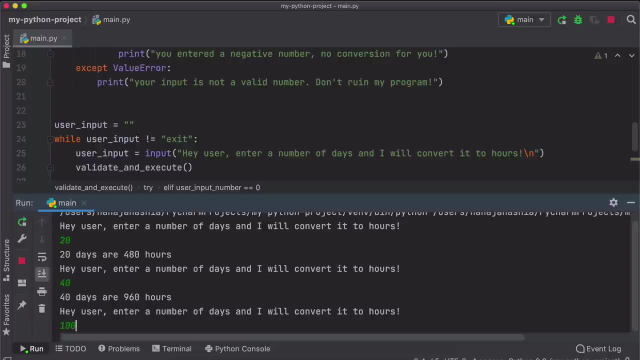 i didn't want to basically just pass it on one after another, because that's just too much effort for me. so let's say i wanted to give it 10 different values, but i don't want to type it in 10 times, right? i want that. 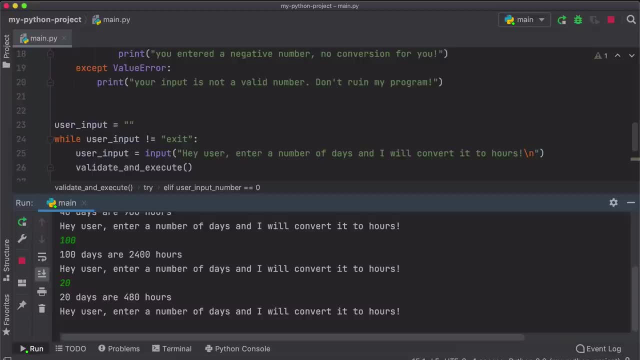 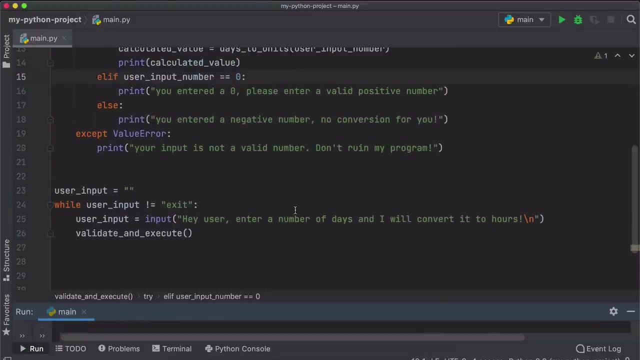 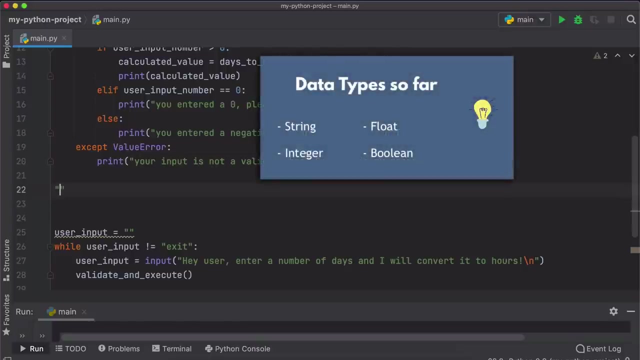 application to basically do the whole calculation for all those 10 values. but i just want to enter that list once instead of entering each value separately. so in this part we're going to learn another data type in python called list. so till now we have learned several data types, like strings, for example. 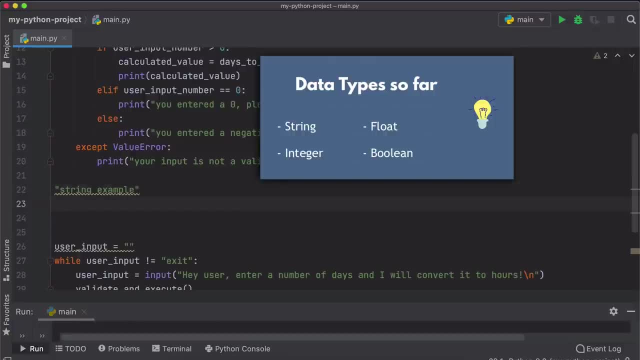 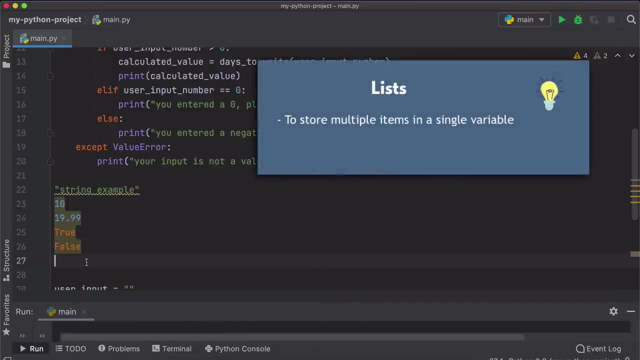 as well as integers and float numbers and boolean true or false. and list is just another data type and the syntax for list is using square brackets, and inside the square brackets we have a list of elements, and those elements can again be either strings, numbers or boolean values. in our case, we want to provide our 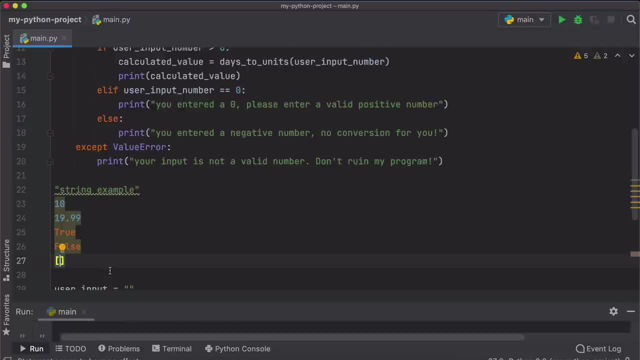 application with a list of number of days, right? so we're going to have a list of integers like this, and you can have as many values inside the list as you want, and these are going to be common, separated and the syntax will look like this. but again, as i said, you can have a list of 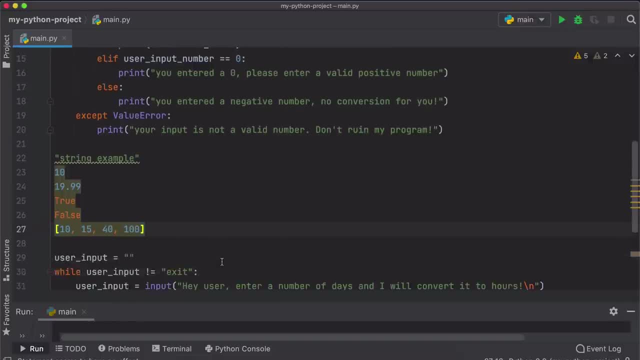 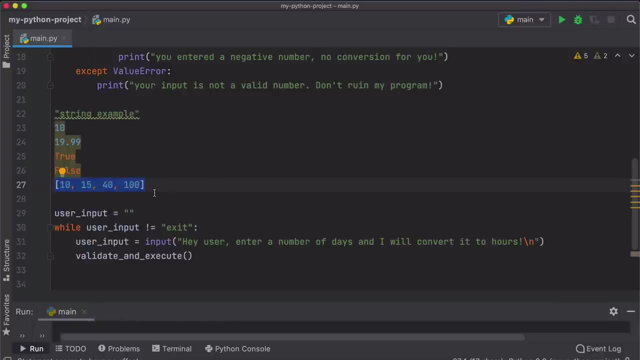 strings, list of booleans, etc. so, as i mentioned, we want to let user basically provide inputs as a list instead of those individual values, one at a time. so i'm going to copy this, let's clean this up and let's actually see what happens. if i just 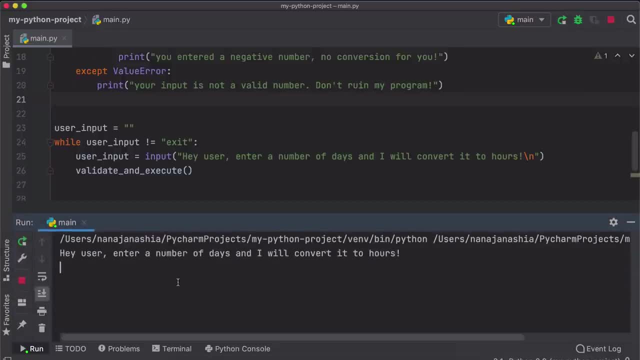 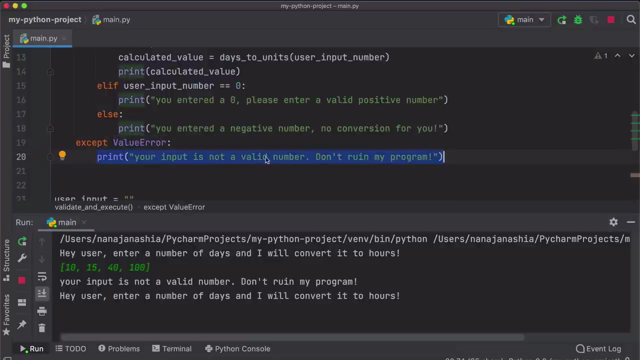 input that list as a value right here and enter. you see, program doesn't recognize that as a valid number, obviously because we have the check and causes a value error. that's why we get: your input is not a valid number. don't ruin my program message right here. so we want to. 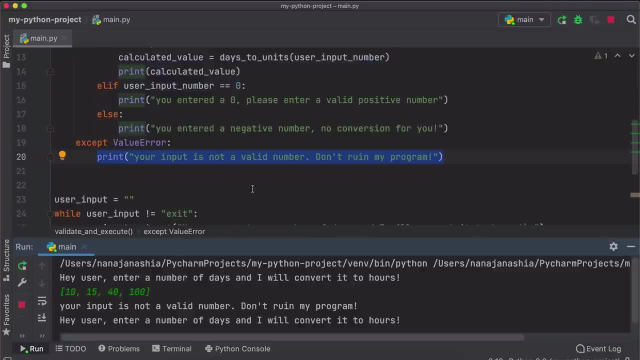 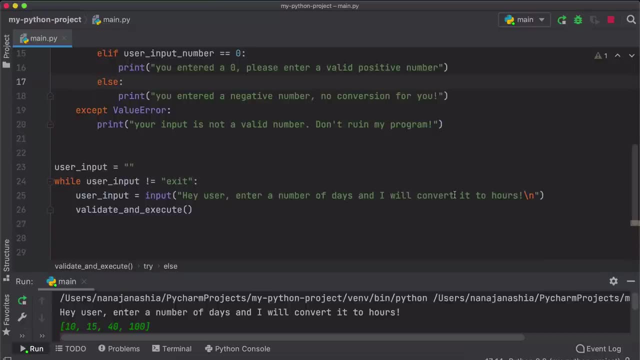 change the value of the list. so we're going to copy this and let's actually see what happens if we change that and make our program actually accept that as a valid input. so how do we actually implement it now? let's go through this logic theoretically first, before we start implementing. 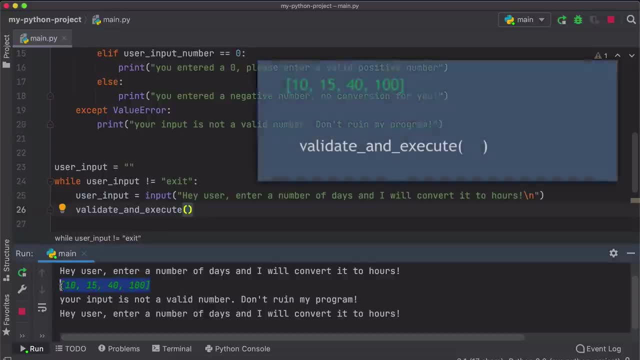 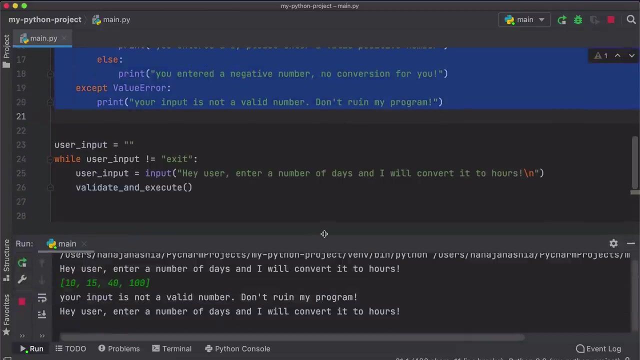 it. what we need here is that we want to read this list and we want to do validation and execution for each value, one at a time. so that means that validate and execute function needs to be called for each value in that list, right? So basically, this function or all this logic needs. 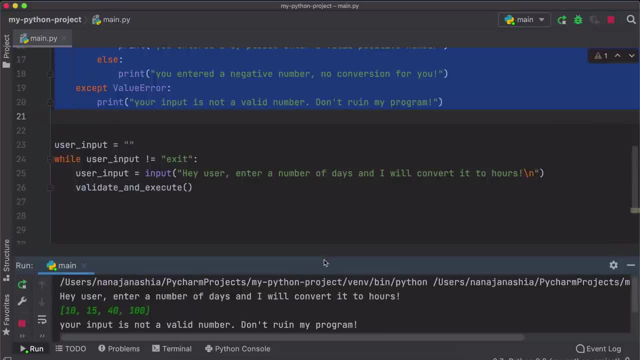 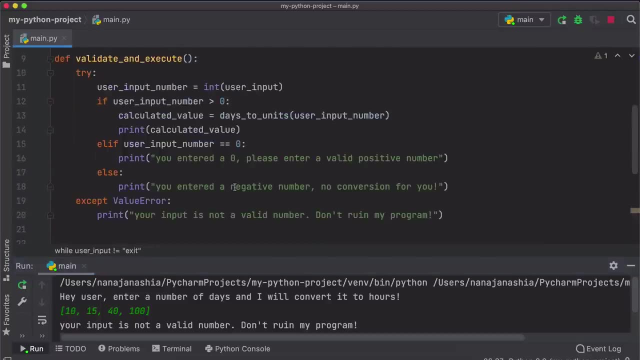 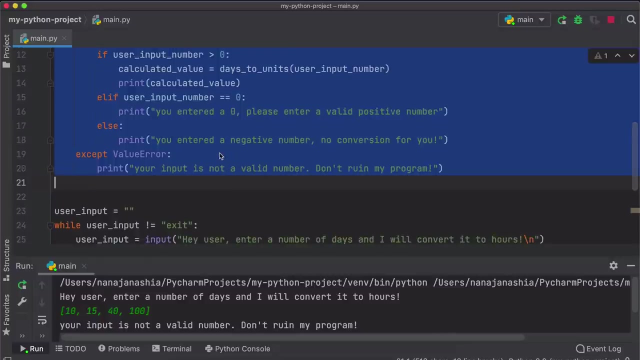 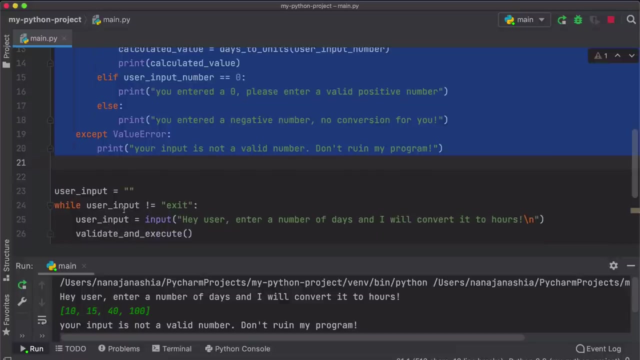 to be executed for each element. Now how do we get the individual elements of the list? So you remember the definition of a loop. Loop is basically executing same function with the same logic multiple times, And the number of times basically depends on the condition. right Here we have a. 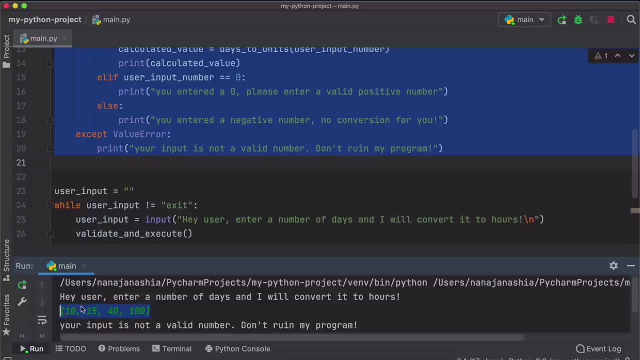 condition for while loop and the condition for executing the same logic for each of those elements is going to be the number of elements in that list, right? So we want to execute the logic as many times as we have elements in the list, And for that we have another type of loop called. 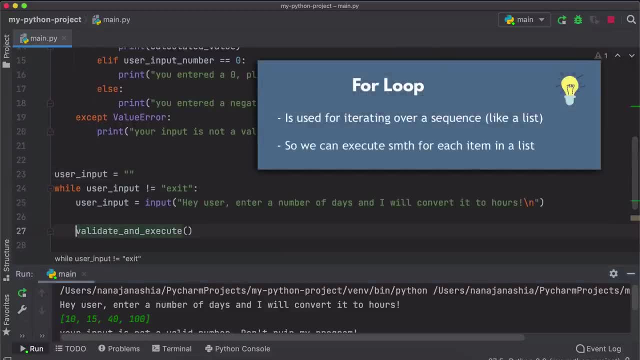 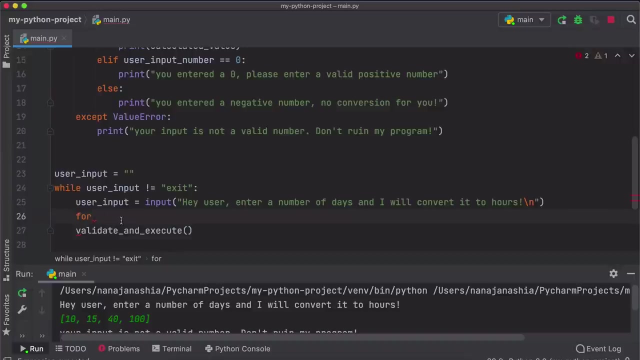 for loop And basically we want to execute, validate and execute function using a for loop. The syntax for for loop is a little bit different. First of all we have for keyword, just like for, while. Then we have the element as a variable, So we can call that number of days, So this variable, basically, 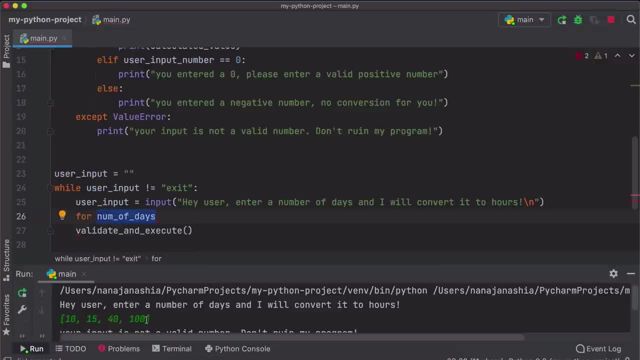 represents each of those elements in the list. And then we have in, which is again a keyword of Python. So for in basically puts together the for loop logic in Python, So Python knows what we are trying to execute. And finally we need the. 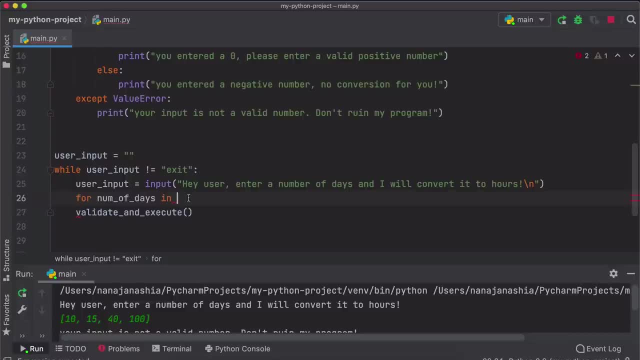 list that we're executing this loop on, And our list is our user input And that's our for loop. However, again, you remember the indentation. the logic that for loop executes needs to be indented, So it should belong to for loop. So now we can read that for loop statement as follows For each element: 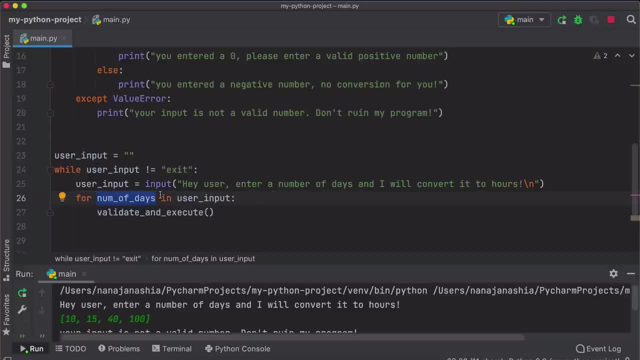 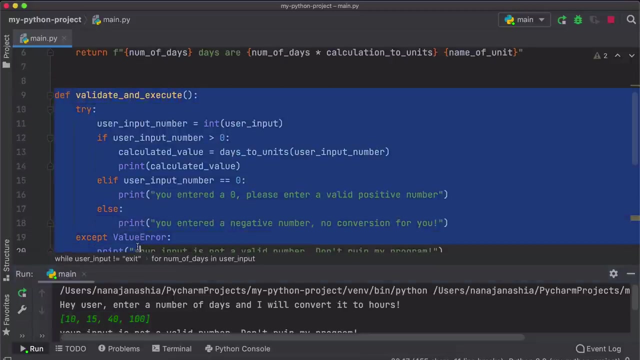 which we call, we decide to call number of days in a list called user input. We want to execute this logic, exactly what I said before. So for each element in this user input list, we want to execute, validate and execute function. We don't have a condition written here. 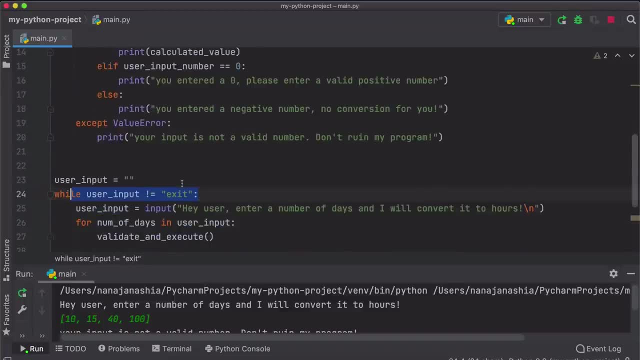 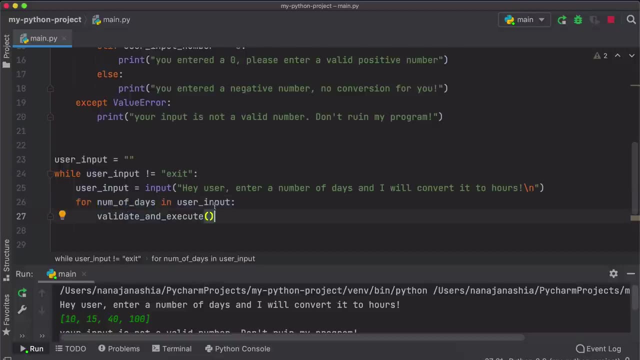 like we did in while loop or if statement. So the condition is basically implicit, right? The condition says however many elements there are in this list, that many times that function or that block of code here will get executed. So if I provide five elements, you will be executed five. 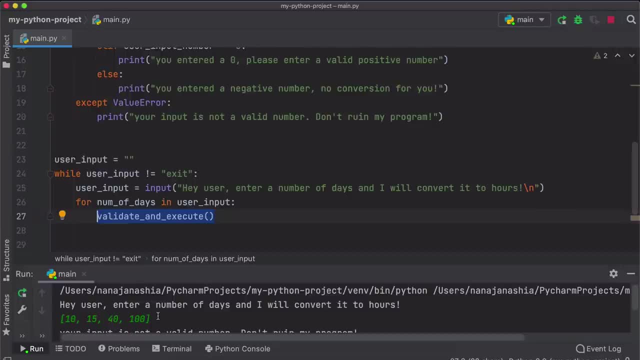 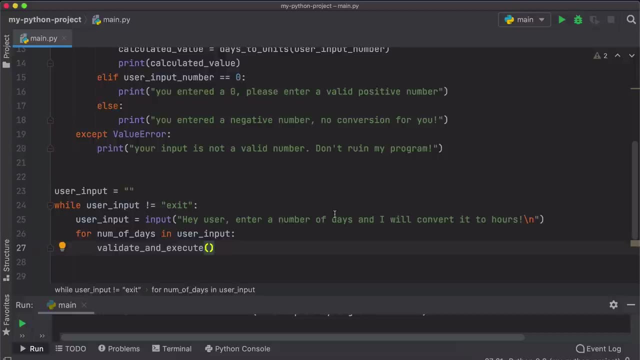 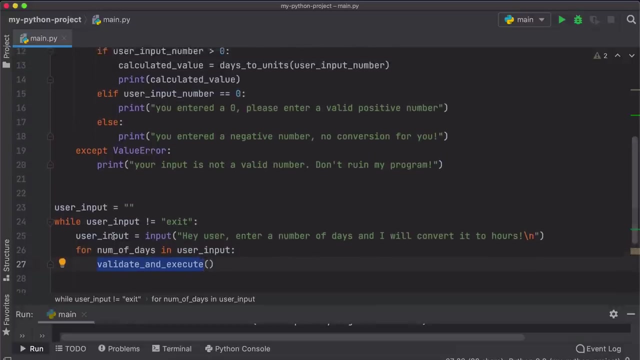 times. If I provide 10 elements, it will be executed 10 times, And that's exactly what we want. However, there are still a couple of things we need to do for this application to work properly. First of all, validate and execute function still uses user input right here, So instead we want it. 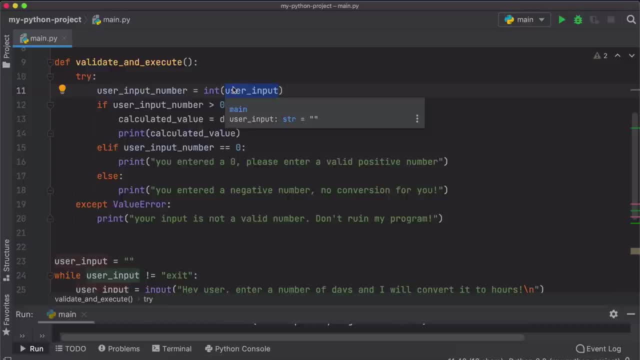 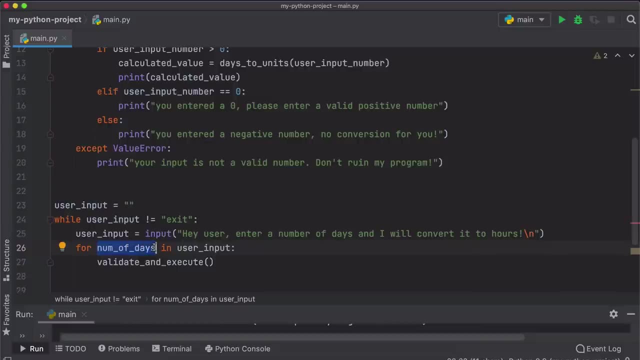 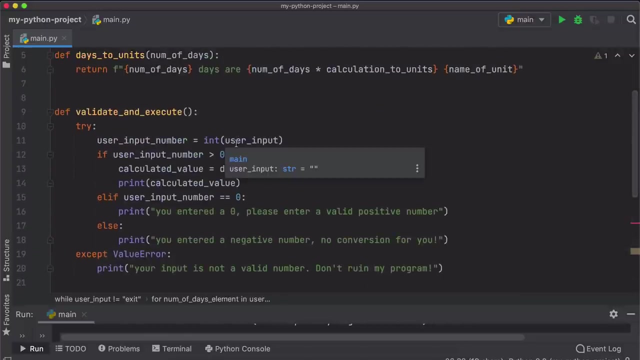 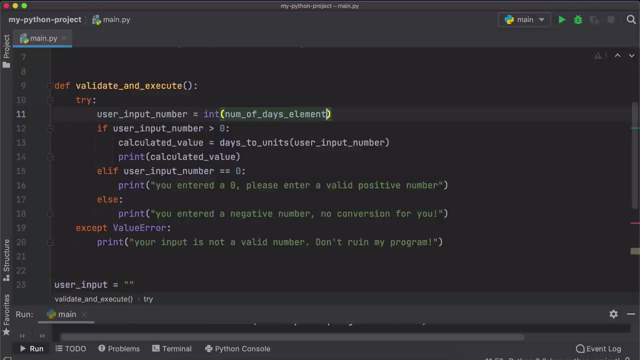 to use the individual values of the user input, because now it's going to be a list and not a number, So this element can actually call it number of days element. This value should be used here instead, Right? So we're going to use that element instead of the whole user input list and paste it here. 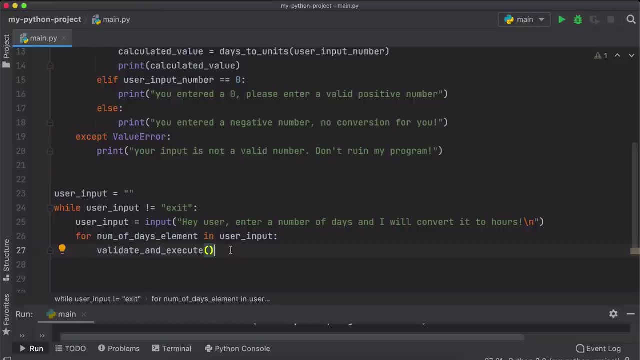 So that fixes the first problem. And the second one is, as you know, user input is always a string. So even if we provide a list of days, it is still going to be a string. So we're going to use that element instead of the whole user input list. 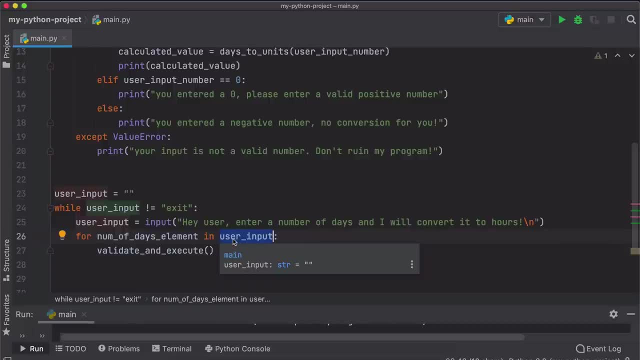 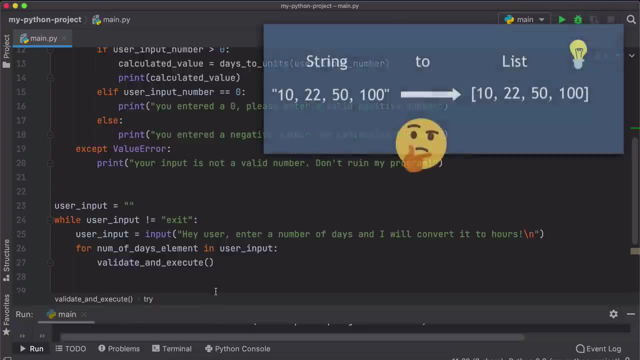 to be considered as a string, So we need something similar to this right here. So the list of numbers that are provided as input needs to be converted in a list in Python, And we can actually do that in a convenient way using user input. dot split and split is a function. 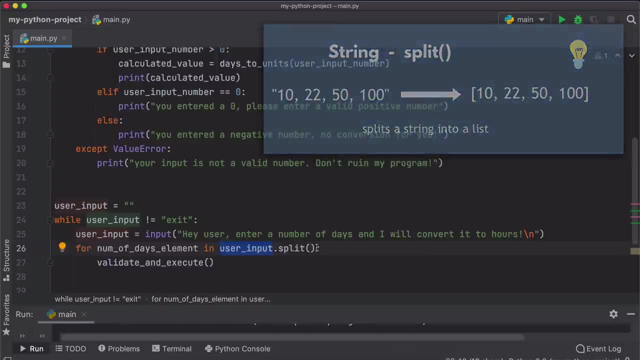 that will take user input as a parameter and will give us in this data type, So split function basically will return a list of all those inputs values. and again note the syntax of executing the split function. We're not just calling a split function like this with: 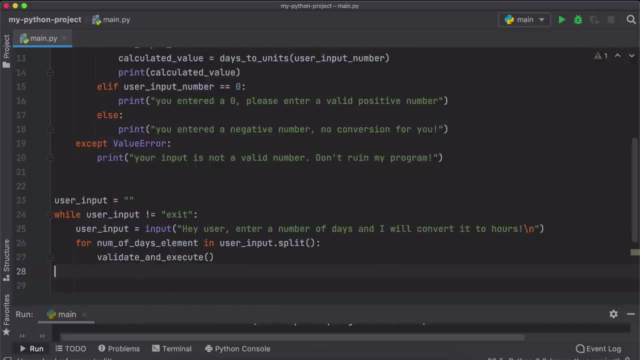 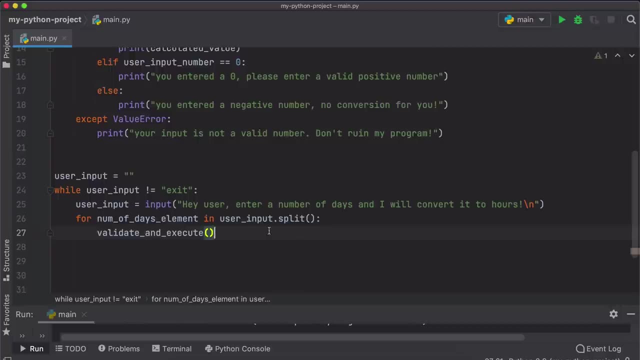 user input as parameter. Instead, we are basically calling it on user input, And I'm going to explain more about this type of functions in Python later, But for now, let's actually execute this application and see what happens. So, first of all, how am I going to provide a list to this application? 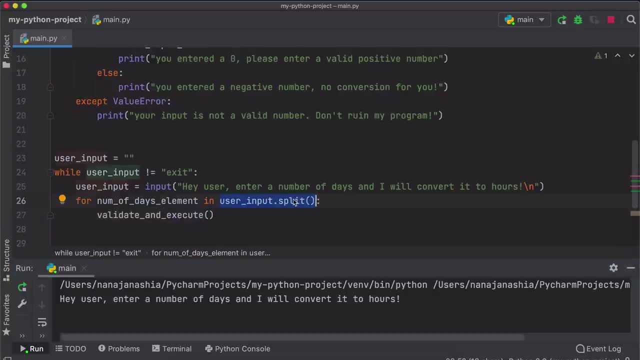 so that user input dot split can actually convert it into a proper list in Python. And the way I should provide the values are list of values with spaces between them. So basically like that. So why spaces? How come it's not a comma or something else? 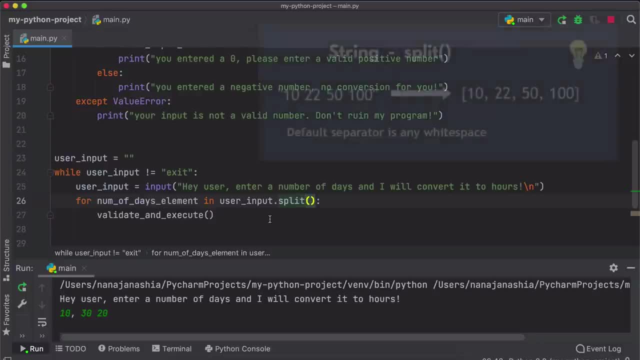 The reason is because split function by default splits that provided list on spaces and then creates a list value out of them. So that's the default behavior of split. However, we can override that behavior and we can decide. you know what we want the input to be: a list of. 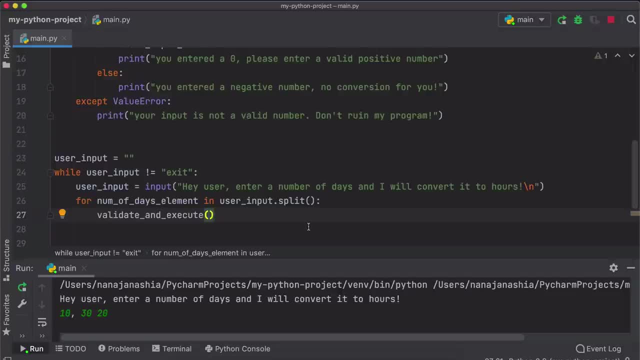 numbers That are comma separated instead of space separated. So what we can do is right: here we can do split on a comma. So that's what our split function here will do. And now, if I re execute it and I can do commas, now 40, 55. So that's going to be user input and split. 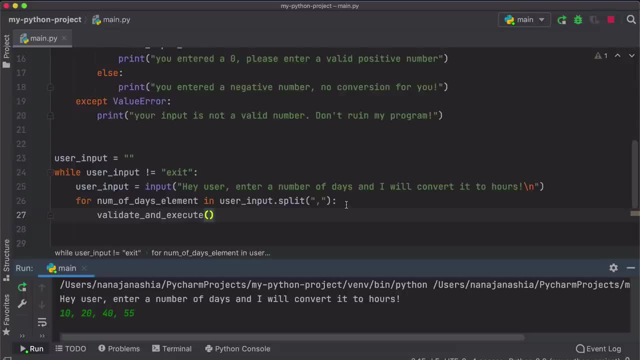 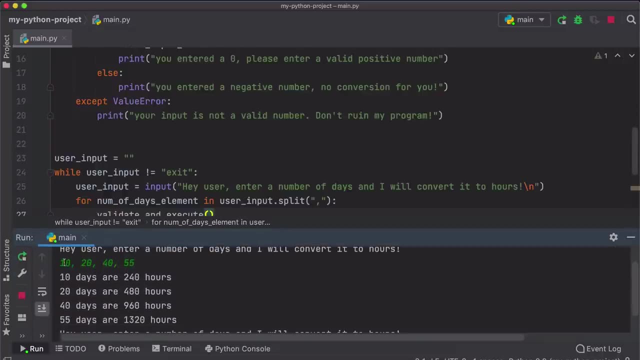 with comma, And then we can see that it's actually going to convert it into a list value in Python. So let's execute it And, as you see, it worked fine. We have a calculation for each of those values. Now let's actually play around with this And let's say we provide a list with some 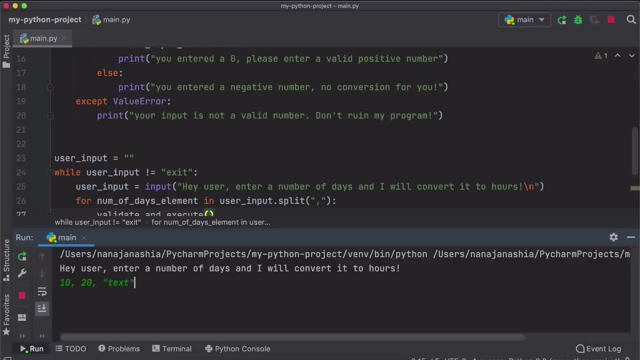 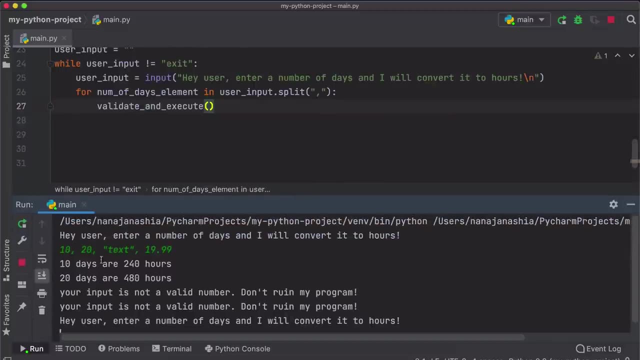 values and somewhere in between we decide to add a text and then maybe a float. So let's see what happens now. And you see that for those two valid numbers the calculation was done properly And for the other two, basically, the validation kicked in and it says that these are invalid numbers. However, again, 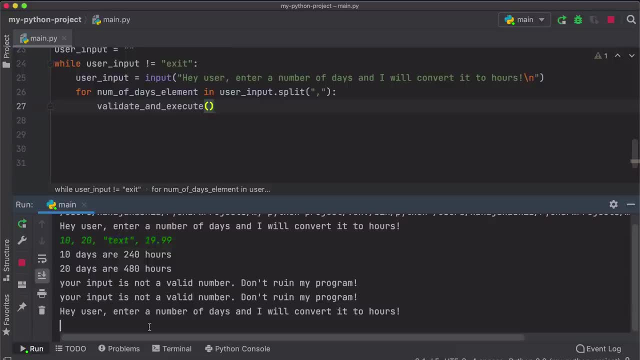 our application ran without any problems and we can even provide another input. So now let's actually do 20, maybe a bullion even- and a negative number. execute And you see that for 20, the number of hours got calculated True is obviously not a valid number and minus. 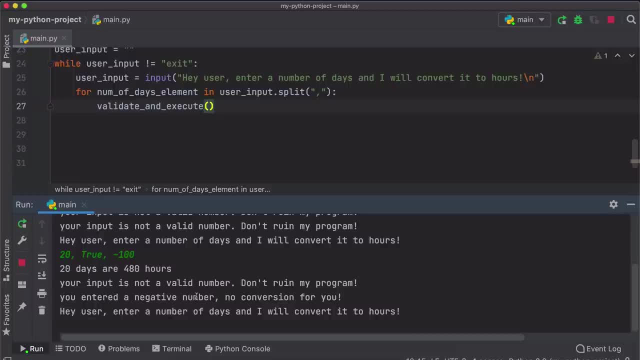 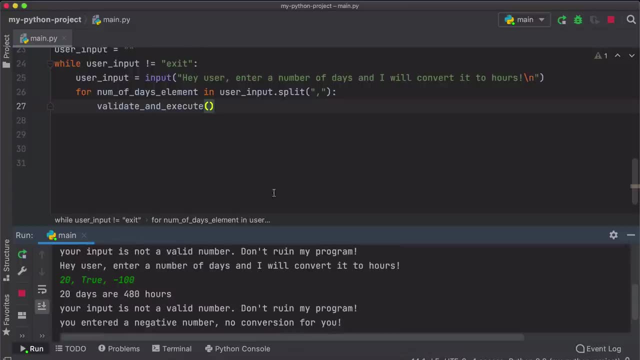 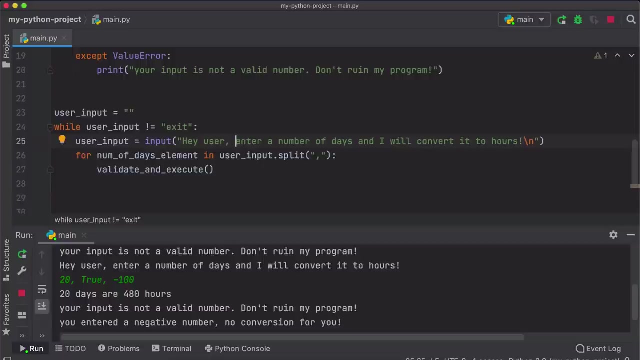 100 is a negative number. So everything works perfect, validations in place and we can provide a list here. now, And as a final optimization, we can actually change this message here that says: Hey user, enter number of days as a comma separated list and I will convert it to ours. So now we can provide either just one. 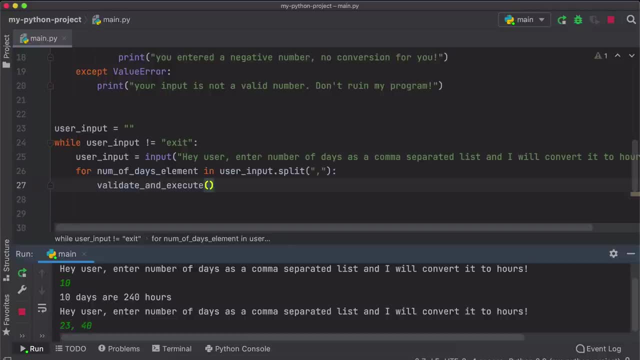 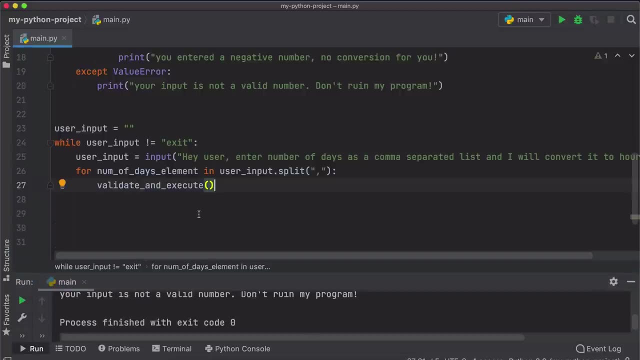 value and it works fine. or we can provide multiple values as a list. And again, if you want to see how that list actually looks like and check the type that it has in Python, let's actually printed. So first I'm going to print type. 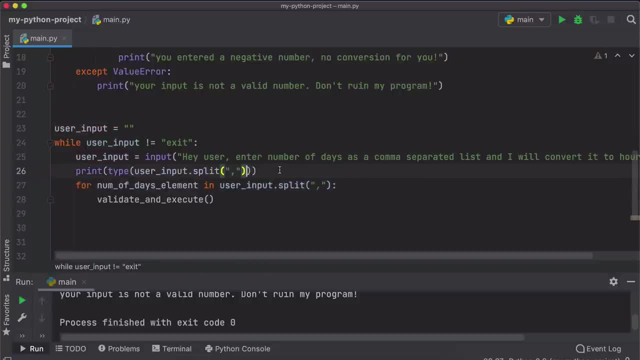 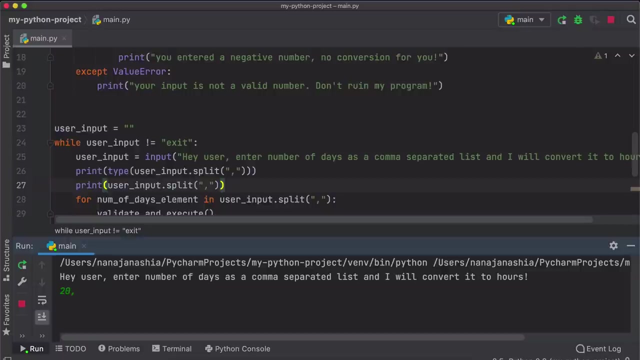 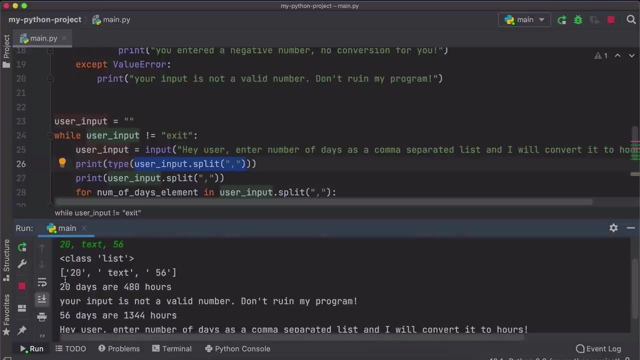 User input Split And then I'm just going to print that list itself. So let's execute And let's provide Some values, And here you see, this is the class list, So basically the data type list, And that's how. 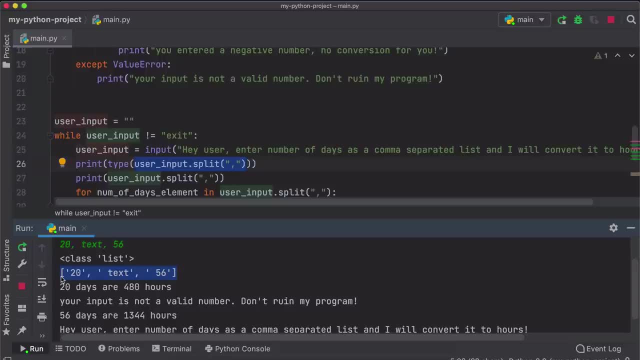 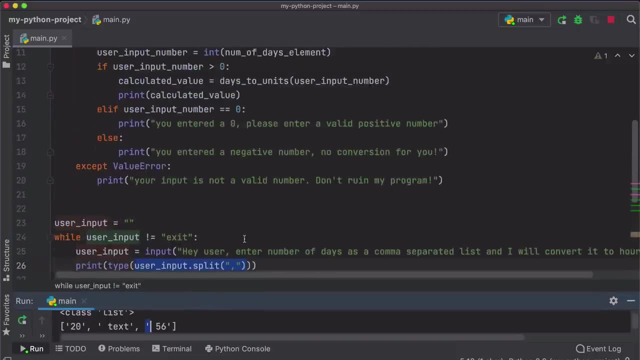 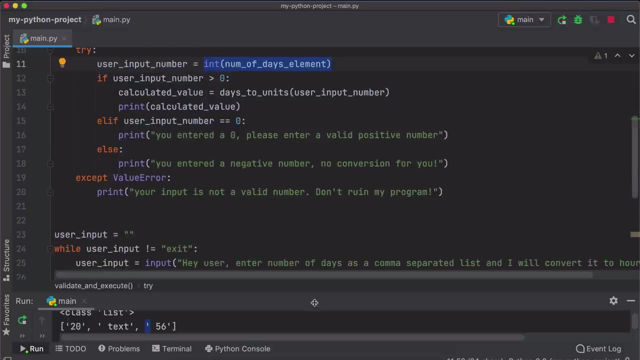 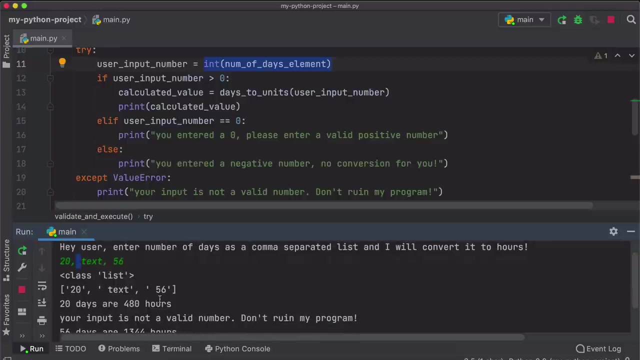 our list looks like. So we have the square brackets here and each element inside as a string, because we have the quotes here and later our application then transforms it or tries to transform it into an integer, And you also see there are some additional spaces here, because that's how we entered the values. 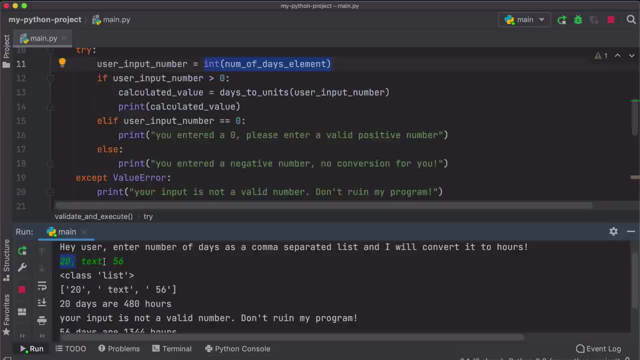 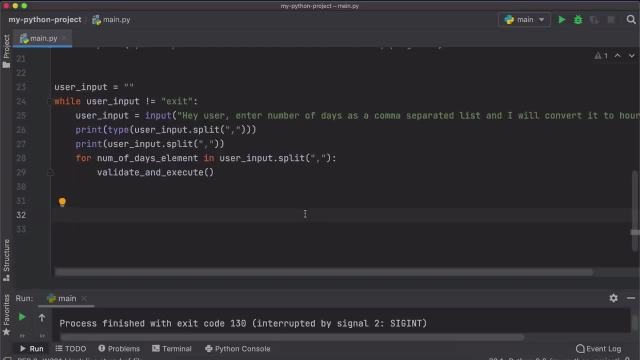 So basically the split splits the values on comma, So this space also becomes part of that element. So to fix that leading space in each value, we can basically just add a space here. So it will split on comma and space. And let's test it. 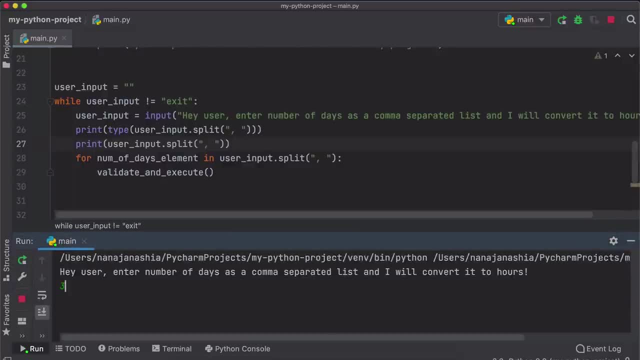 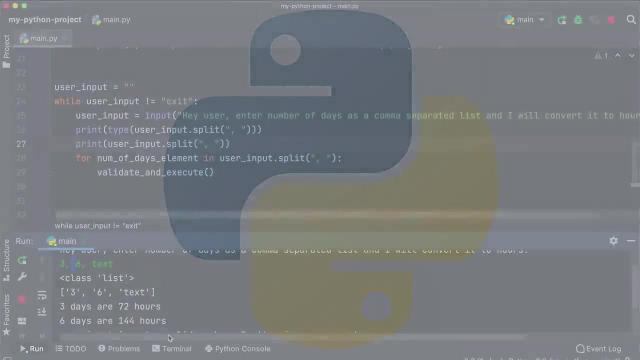 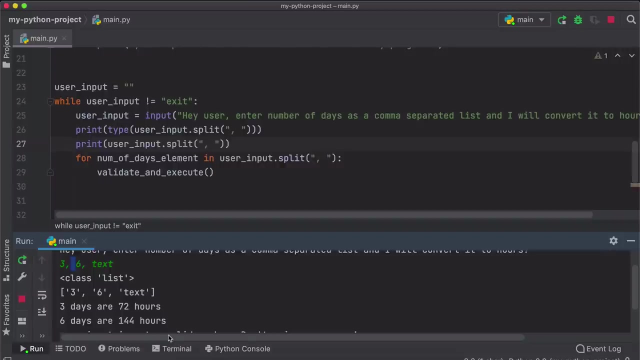 Out And there you go: We have our values without the space before them. So you saw an example of when we actually need to use list data types. In this example, we wanted to allow users to basically just input multiple values at once as a list, But obviously this is just one of the use cases for a list, and 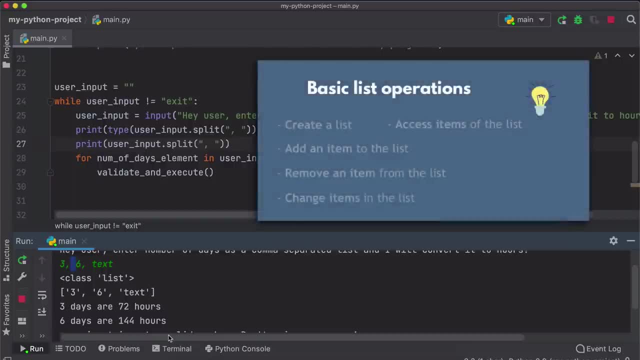 one of the specific examples. because throughout the application you can create lists and you can use the elements of that list in another function, so you can use it for multiple use cases. And just to show you some basic syntax of how to create lists within your code, inside your 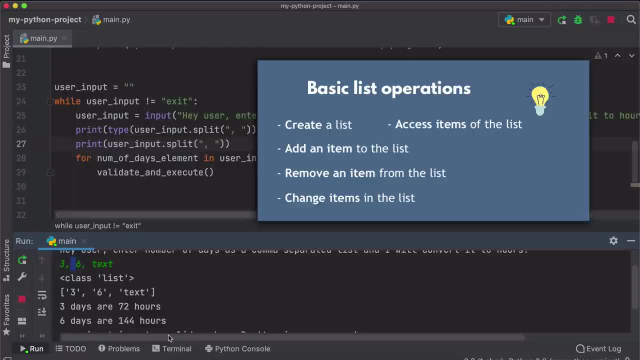 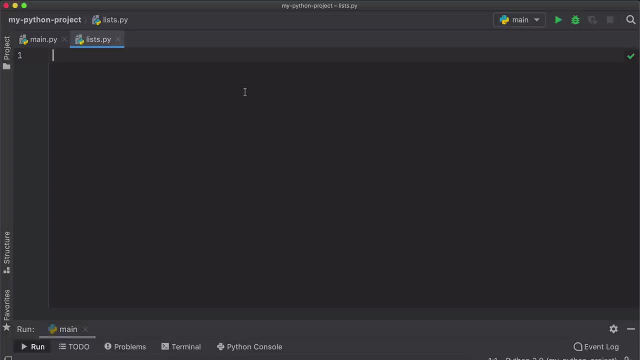 application, So how to initiate it and then how to Use that list. I will show you the examples here. So, basically, to create a list in your code, you would use that syntax that I showed you earlier, with square brackets, and inside that you would have list of elements and this could be strings. 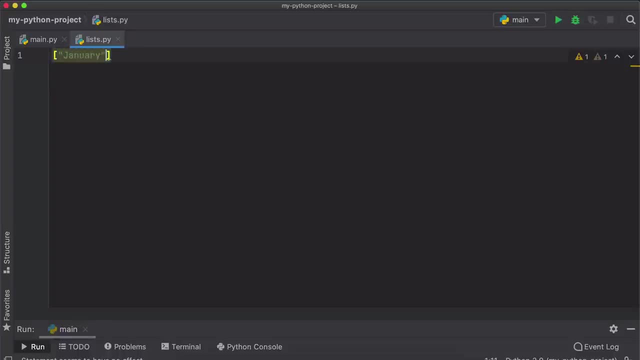 So it could be, for example, names of month, let's say like this, And then we would have to assign it to a variable Right again, just like we did for strings or integers or other data types. so we can call it my list, and this will give us a list with three string values inside. 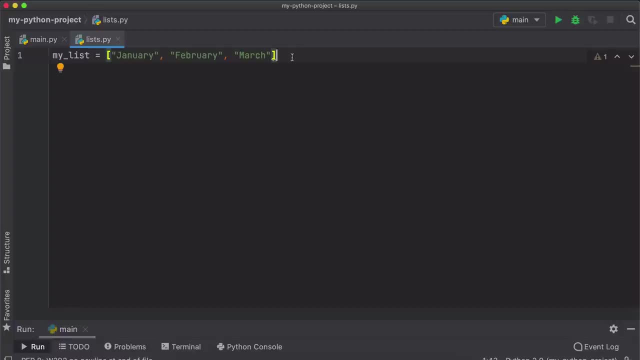 And once you have created a list, you can then use it to read the values from the list, Right? So basically to get the individual values elements out of that list. So, for example, if we wanted to print out the first element of my list, then we would access. 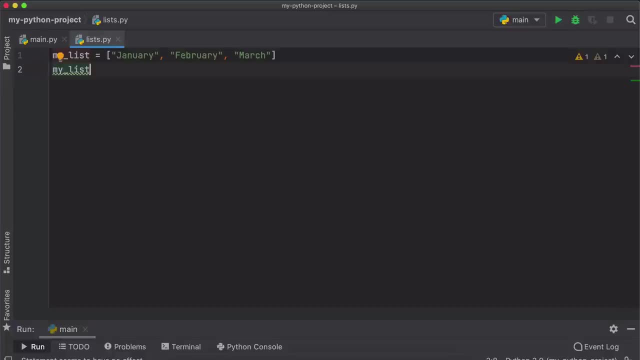 that using my list and then following syntax, with again square brackets and then index number of the element which is starting from zero. So this is the first element with index zero, This is the element with index one, index two and so on. All right, 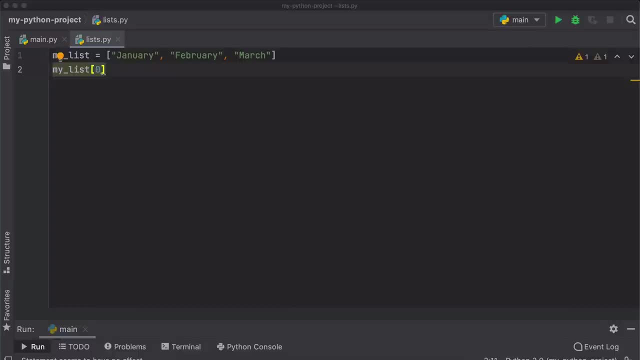 So Could be confusing, because it starts with zero, not with one, But that's how the specific element of a list can be accessed, Right? So if I wanted the March value here, the third element, then I would just type in index two. 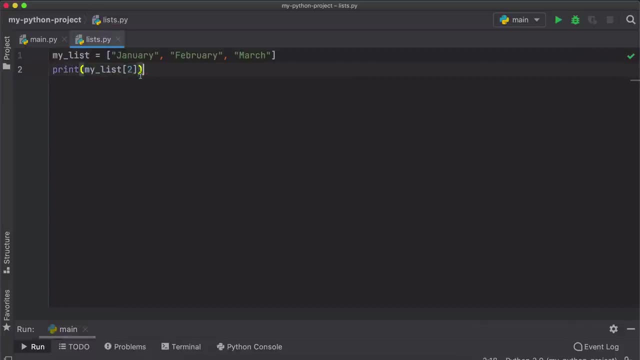 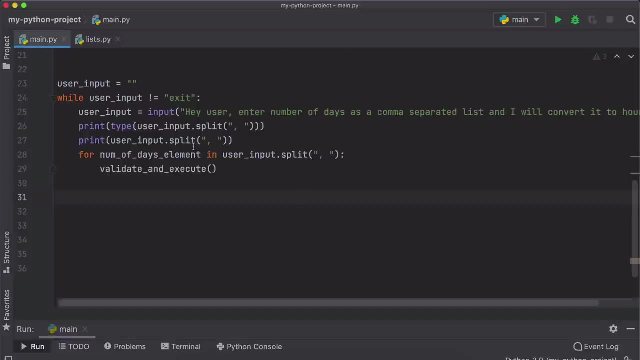 And this is a syntax of getting elements from, at least if I just want specific values and not each element one by one, as we had in this example, Right? So one way to use a list is to Basically loop through it and get one element at a time. 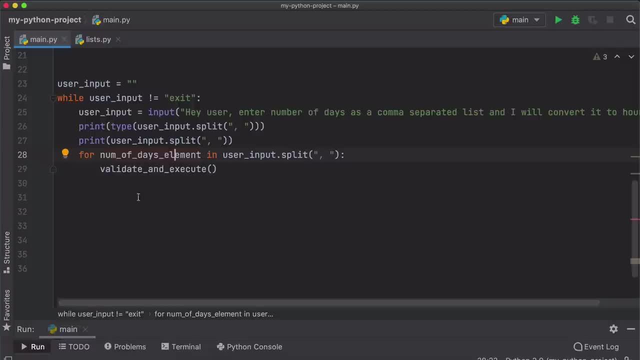 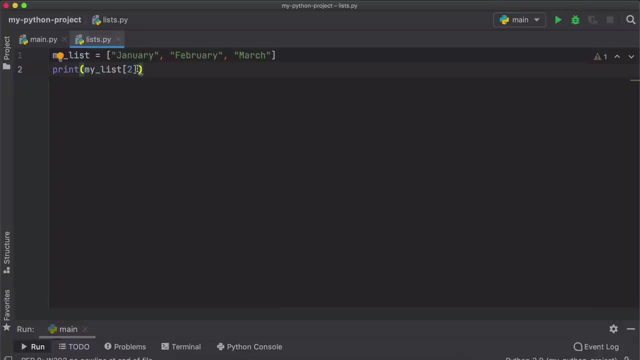 And that's why we don't need to use index here, because it gives us elements one after another. Or maybe we don't want all the elements or to do something for each element. We just want specific values from the list for different use cases. 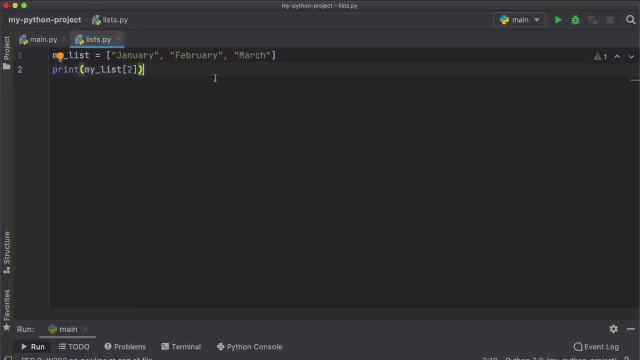 In this case, we can access them individually, like this, And in addition to accessing the values from a list or basically reading the values from a list, we can also add values To a list, And we can do that by typing my list. 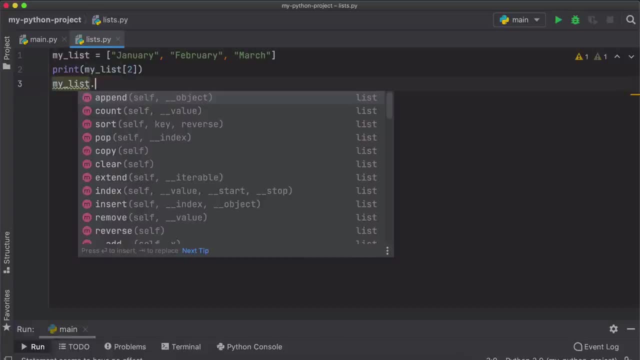 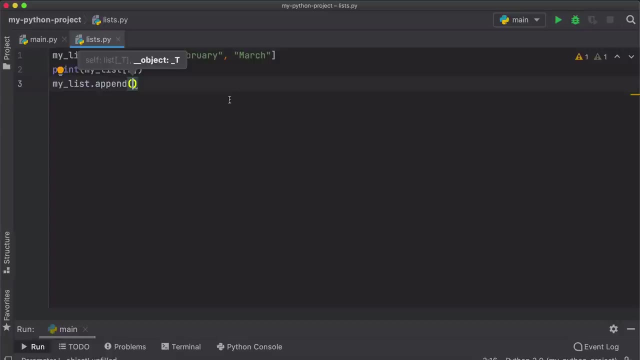 And then on the my list, we're going to do dot and use the append function, Right? So append will basically take the next element or another value, basically, and add it to the list of elements already in the list, Right? So let's say, we want to add the next month. 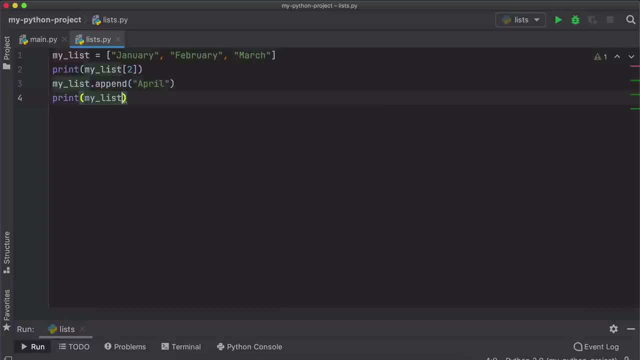 And now, if I print My list, we should actually see this here with April as a fourth element, Right? So let's execute, And there you go. So first we have March here printed out, which is the third element right. 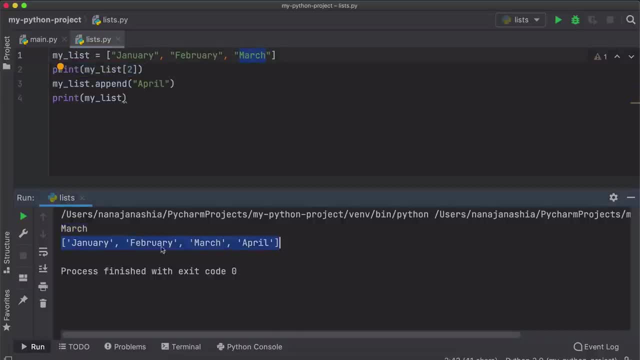 Index two, And then we have my list. append that its fourth month name into the list. So after a pen, this is how my list will look like And now again we can access the specific element. for example, if we wanted to access the newly added element on index three. 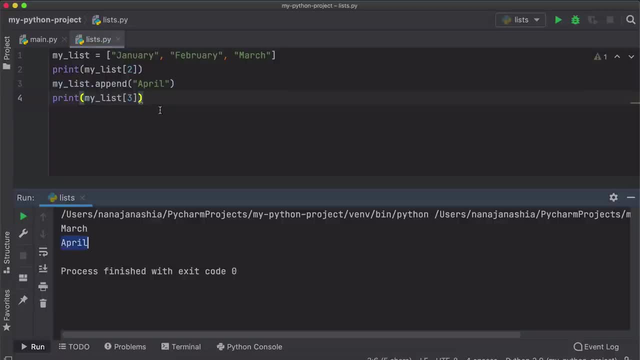 So that's going to be the fourth element, And there you go, We have the new element printed out. And also an interesting note is what happens if we use an index here which is too high, So basically pointing an element that doesn't exist. 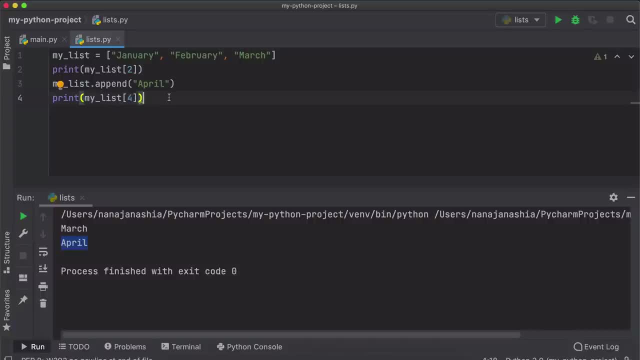 Right, So instead of three, let's say we have four here. So this will Point to the fifth element, And since we only have four elements, let's actually see what's going to happen. So I'm going to execute this. 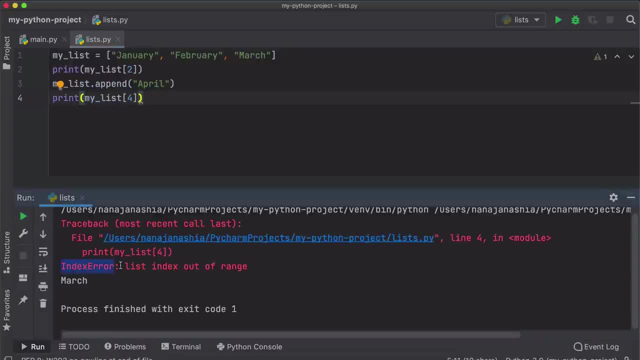 And there you go, You see an error, index error that says at least index out of range. So every time you access, or you try to access, an element at the index that doesn't exist, you will get this least index out of range error. 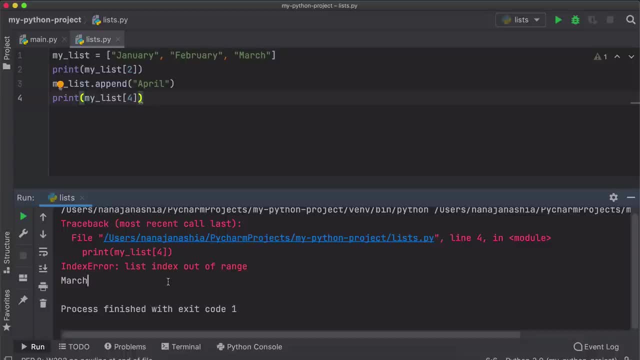 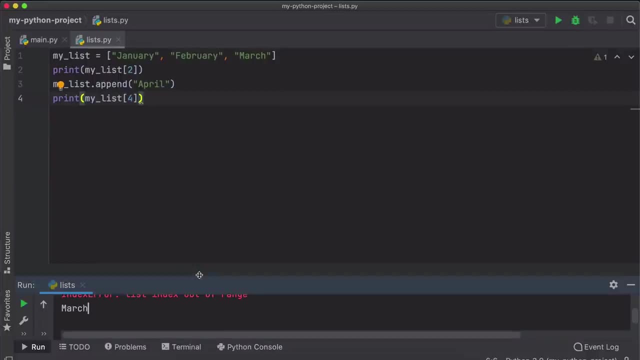 And this is actually something that may happen pretty often When Working with lists- if you're accessing the values like this. So this is how you work with lists, how you create them and access values in them, as well as add some values. 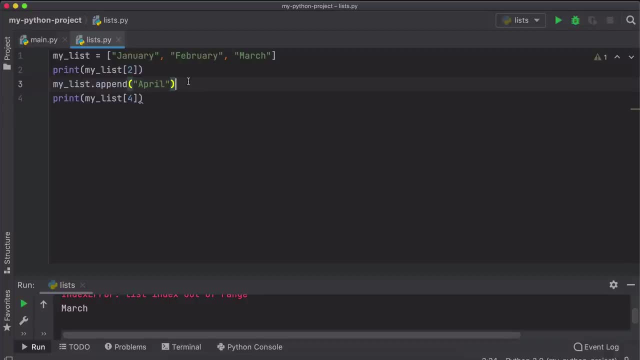 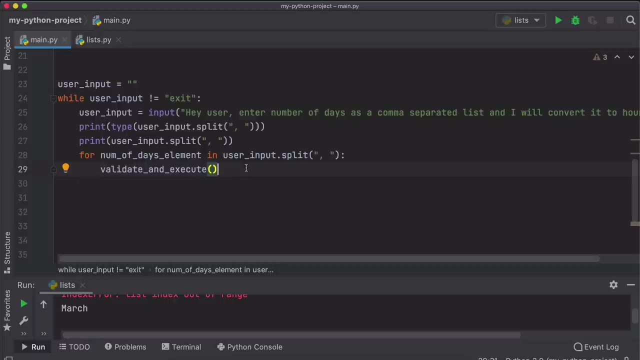 However, note that most of the time, if you are using lists, you're going to be using them in a for loop, because most of the time, you would want to do something specific for each element in the list. So this, basically, should give you an idea of syntax of lists and how to use them. 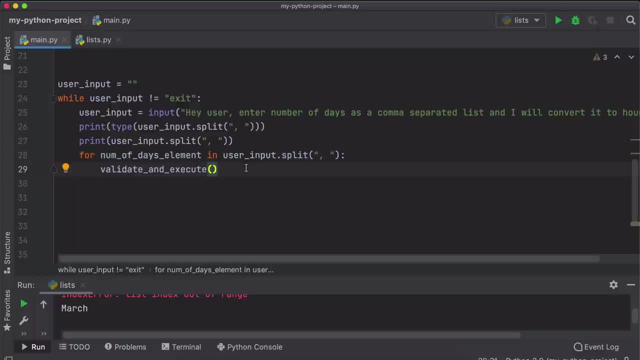 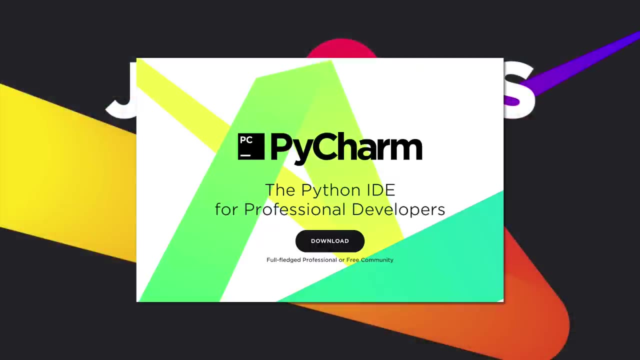 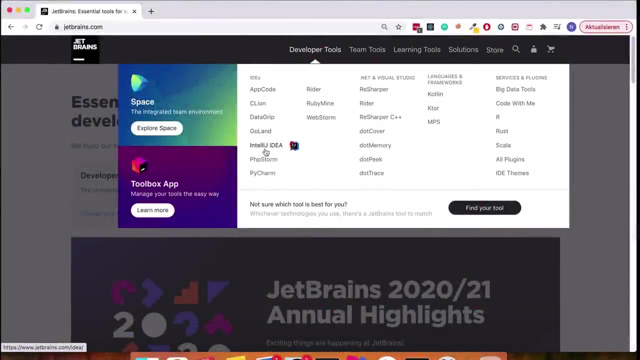 Generally, and also how to use them in combination with for loops. Here I want to take a few seconds to thank JetBrains, the creators of the awesome PyCharm and IntelliJ editors, for sponsoring this complete course. Besides all the great existing products they have, they recently introduced Space, which is an 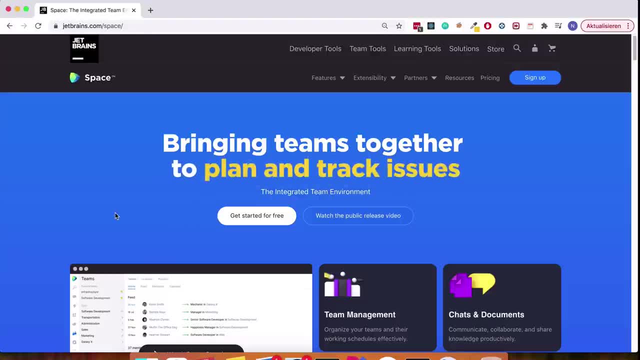 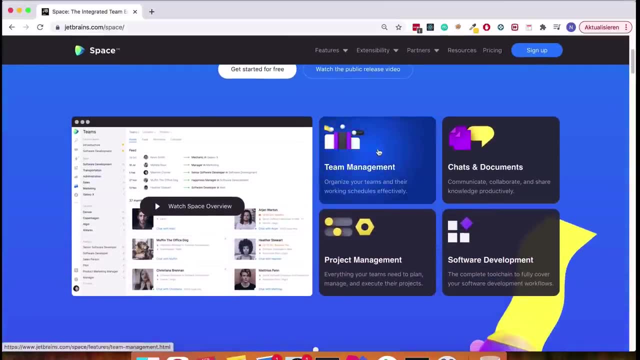 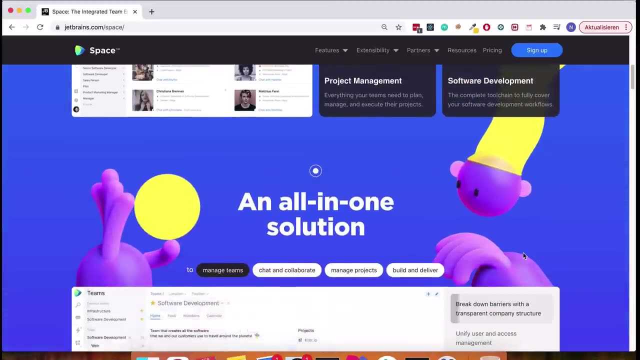 all in one team collaboration platform, covering software development, project and team management. And the great thing about Space is that every single tool you would need in a company to collaborate and work together in a team is in one space. So you have tools for chats, blogs, planning and creating tasks. 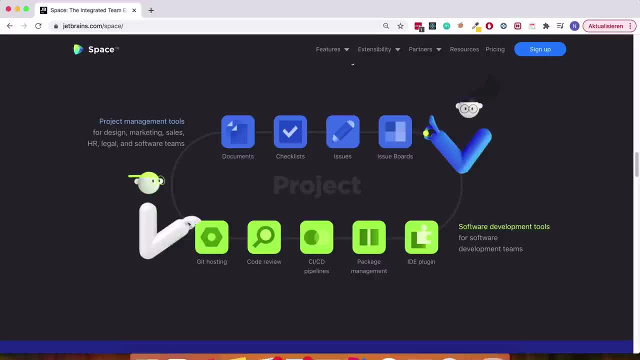 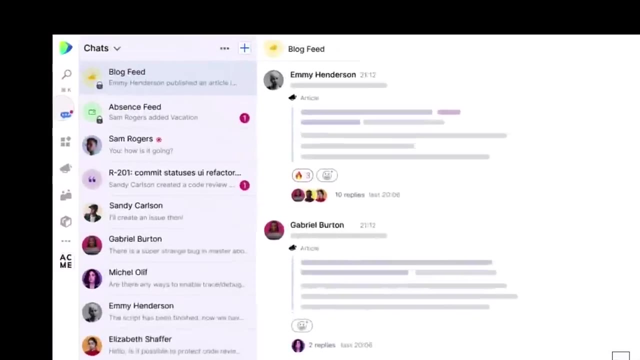 meetings, but also software development tools like version control, CI, CD, package repositories and much more. So all of these in one platform and, in terms of productivity, the great thing is, you get all the notifications In one place, like code review, updates, newly created issues, new blog posts, etc. 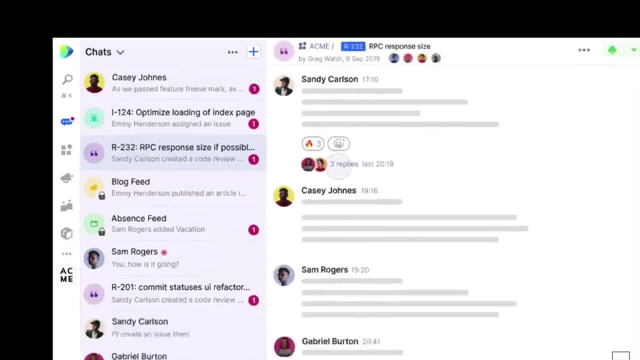 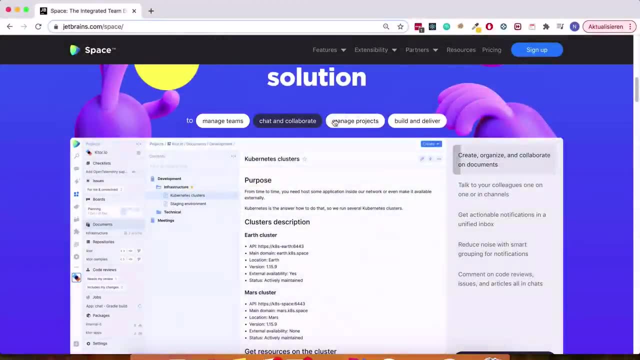 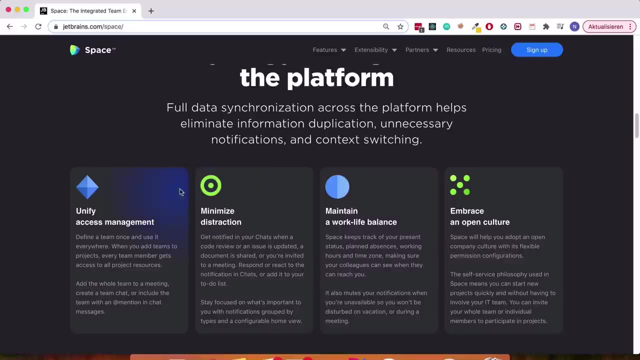 You get all of these in chats, where you can react directly in place or add them to your to do list automatically. So I think the main value of space isn't that it has all these tools, but rather the fact that it integrates them in such an intelligent way. 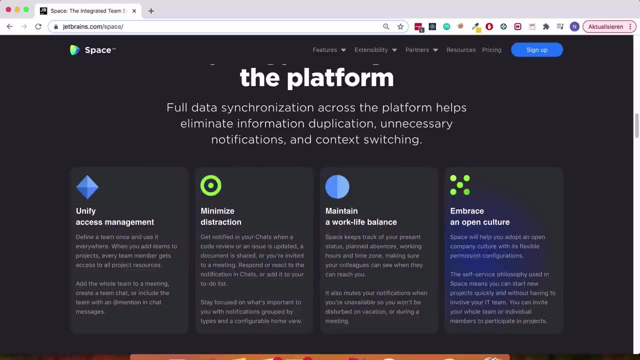 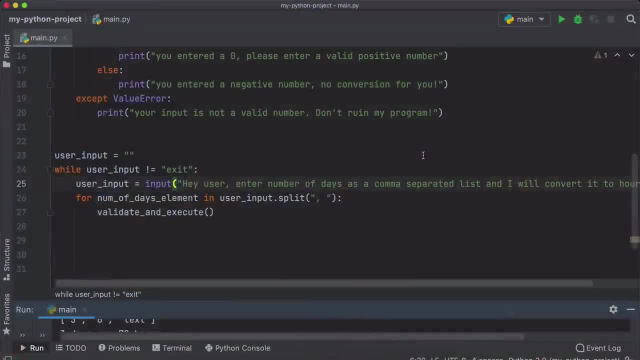 that it improves the team communication and productivity overall. Now let's go back to code. Now, at this point here I want to mention a pretty minor and simple detail, but something that is also very important and useful in programming, and that is comments. 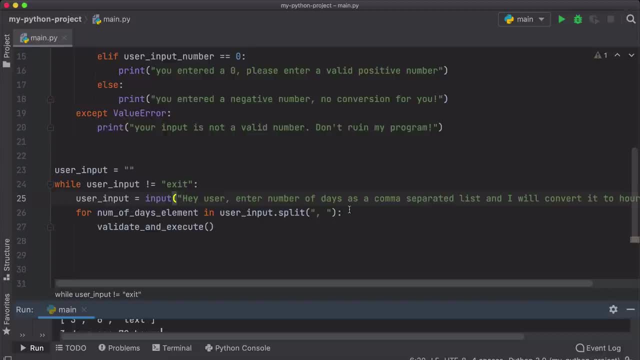 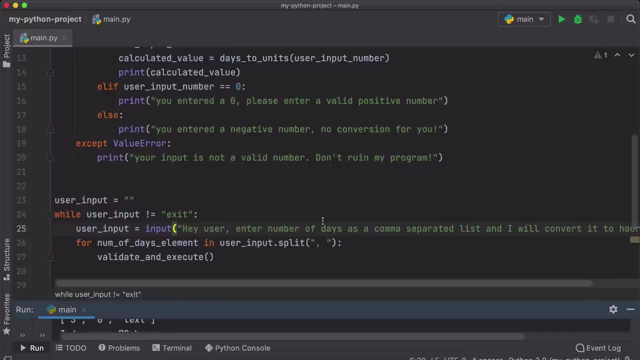 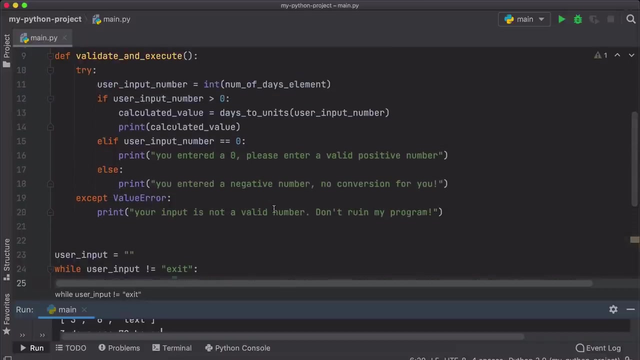 So how do we write comments in Python And why do we need, or in which cases are comments actually useful? One usage of comments is basically to give yourself some notes on your own code. So basically, if your code gets a little bit complicated and it's not really clear what the logic or the function body is doing, 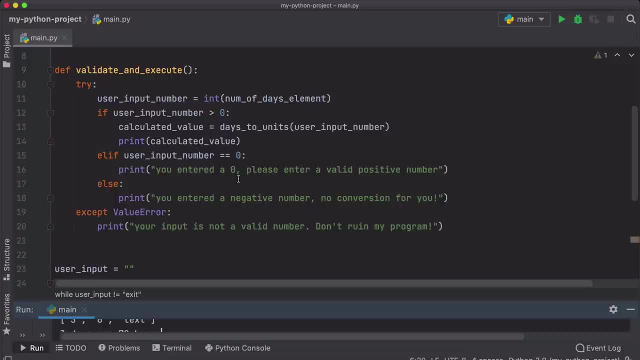 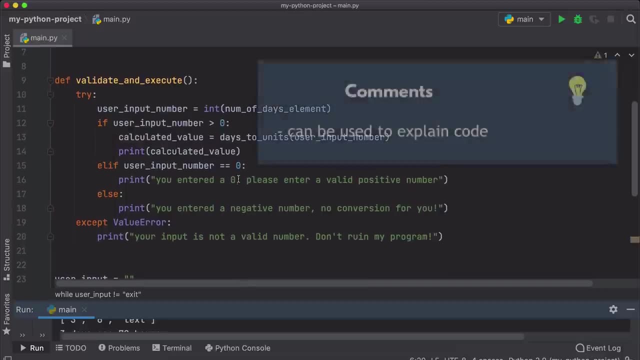 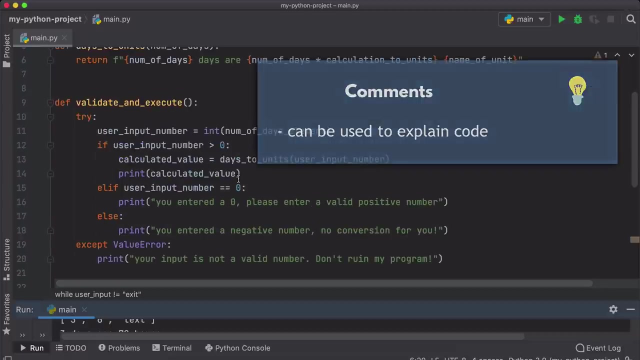 it could be because of bad programming, but also because the function logic is just little too complicated. So you want to add some textual notes to the code so that you understand what's going on there, even when you look at that code days or maybe weeks after you wrote it. 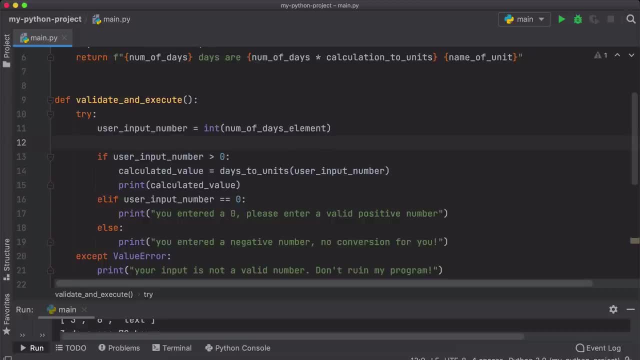 So for example, right here we may want to add Some notes about what This part here is doing, and comments in Python are written with this character. So for example, I want to add a note here. We want to do conversion only for positive integers. 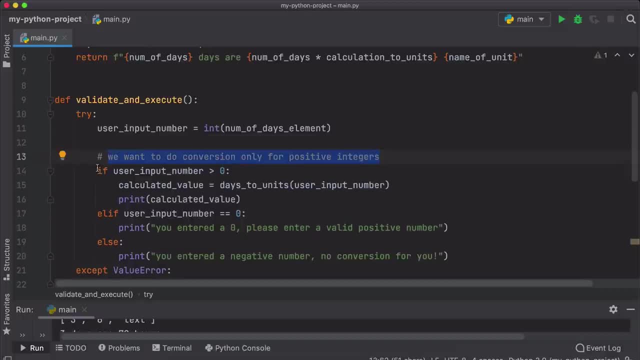 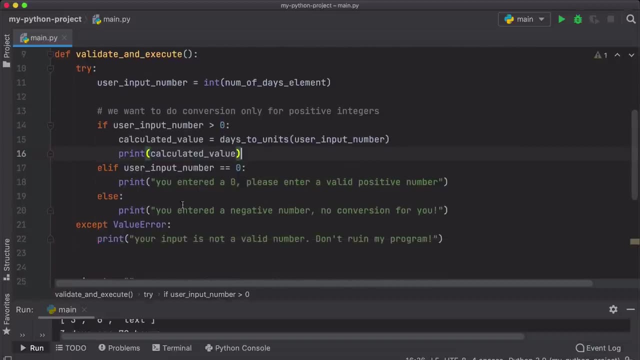 And that's basically my note that summarizes all that logic right here. And it is not only useful for myself, in case I forget what this complex logic actually does, but also for your team members. So if you're working in a team and your code gets really complex and it's difficult to keep, 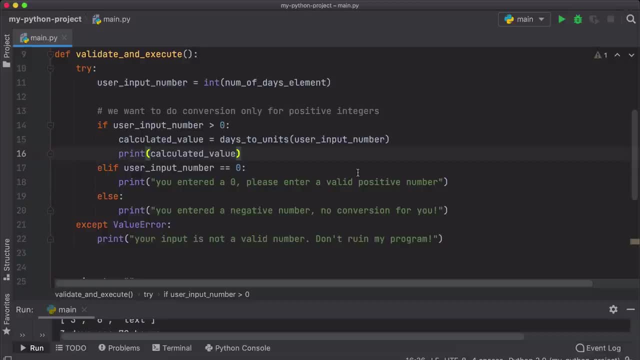 an overview of different functions and variables and what all these things do. you can basically add these comments as notes to your team members so they can also understand what you thought or what kind of logic. So if you're working in a team and your code gets really complex and it's difficult to keep an overview of different functions and variables and what all these things do, you can basically add these comments as notes to your team members so they can also understand what you thought or what kind of logic you're writing. 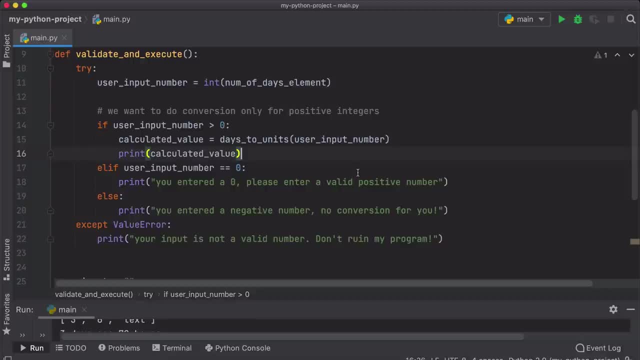 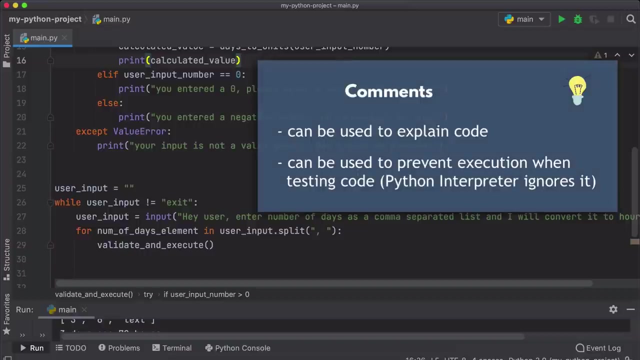 thought or what kind of logic actually you were thinking about when writing this code. So comments is a way of communicating your thoughts and your logic on your code. So that's one use case for using comments And the second use case if you have a piece of code that you do not want to delete because 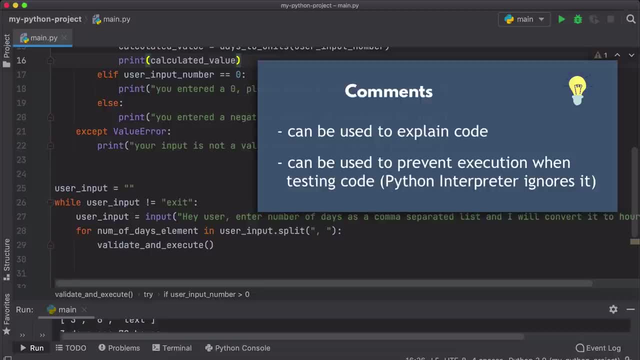 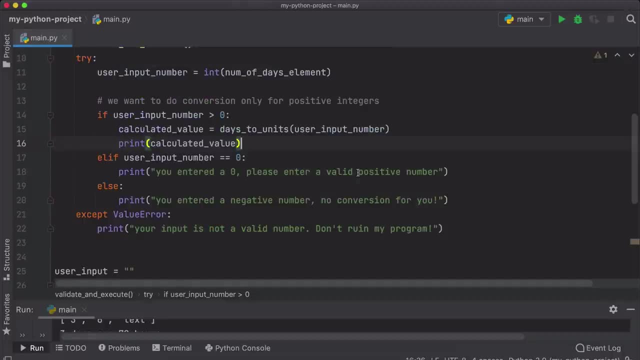 it has some logic or it has some example that you want to keep as a reference, but you don't want that code to be executed. So basically, you can comment out code so that it still stays there but doesn't get executed, And the way to do that is just basically having this character before the line. 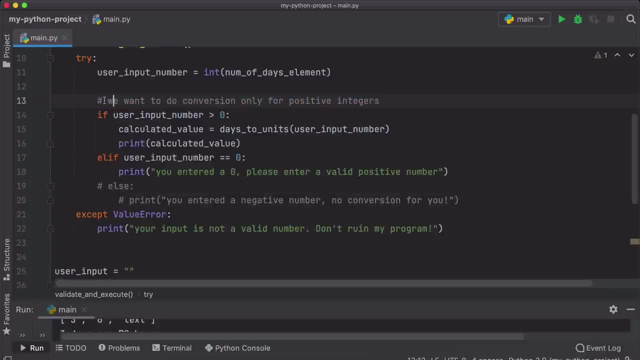 And also note the color of the comment in the editor is gray, So it's immediately visible that these are the comments. And now these two lines will not get executed by the program. They will be ignored, But they are for your own reference. 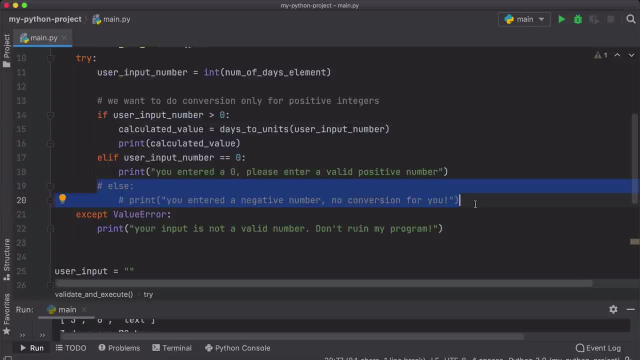 In case you want To keep it there. for example, this could happen if you are unsure about the change and you want to delete that whole code from your application, because you might actually need that eventually. So you're not sure about it, So temporarily comment the code before you permanently delete that. 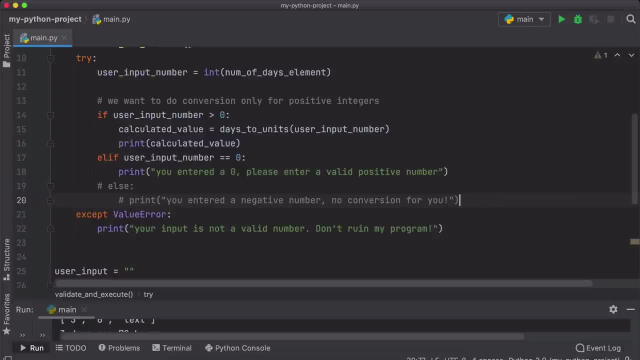 So these are some of the use cases of comments. Now, if you have multiple lines of code that you want to comment out, or maybe hold text that you wrote as a note. So, for example, you want to comment out all this Four lines here. 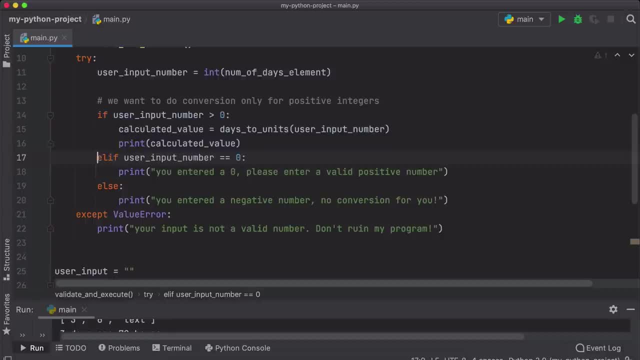 Obviously you don't want to do this in front of every line, So for multi line comments you can actually use the following syntax, which is three quotes: at the beginning and at the end. And again, you see, the highlighting is different here, which basically is highlighting of a. 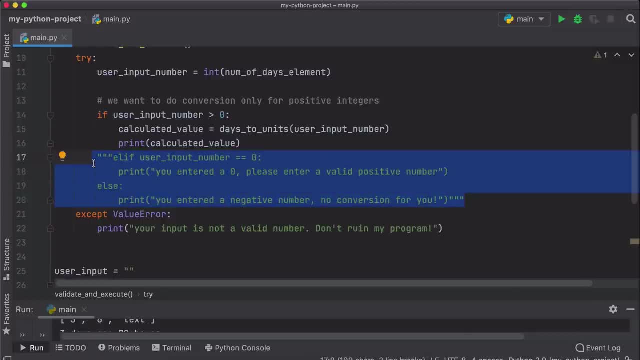 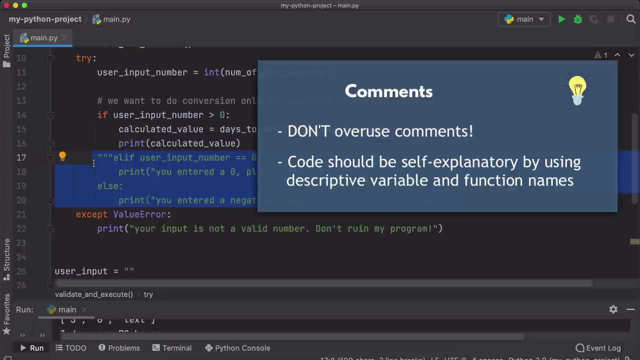 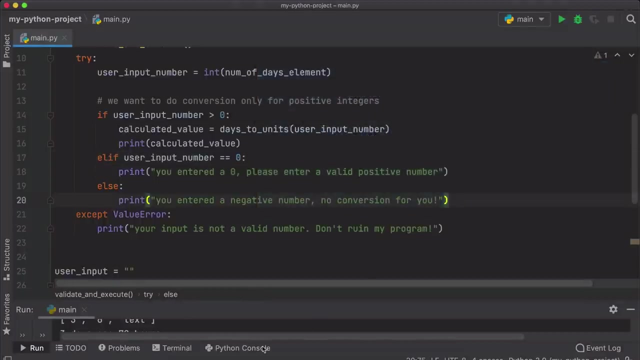 string. However, it is ignored by the program and it will not be executed. As a Best practice, you shouldn't have too many comments in your code, because it will just add additional clutter and your code will look basically unclean, So you should use them only when needed. 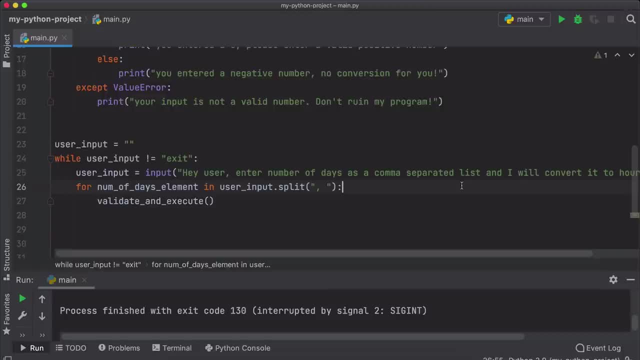 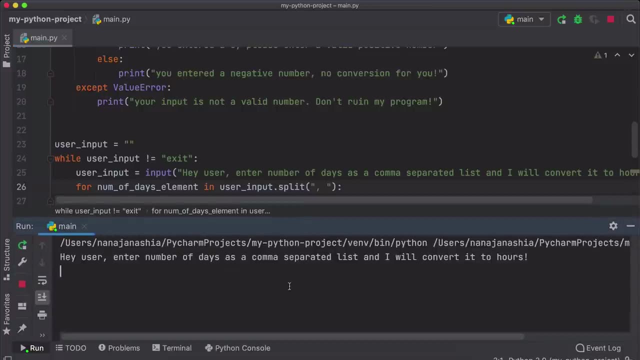 In this part I'm going to show you another data type in Python called set. So what is a set? Let's start our application again and let's say I provide here inputs, values as a list, let's say 20.. 40 and 20 again. 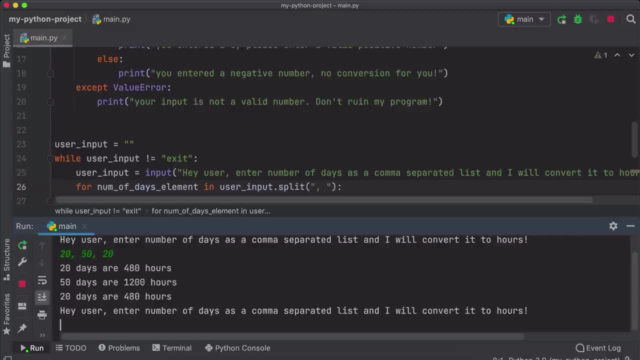 So basically, I have duplicate values in my list and when I executed I see that the program got executed for each element and I have duplicate results because I passed in the same value twice. Now again, users, they can input any value they want, either intentionally or accidentally. 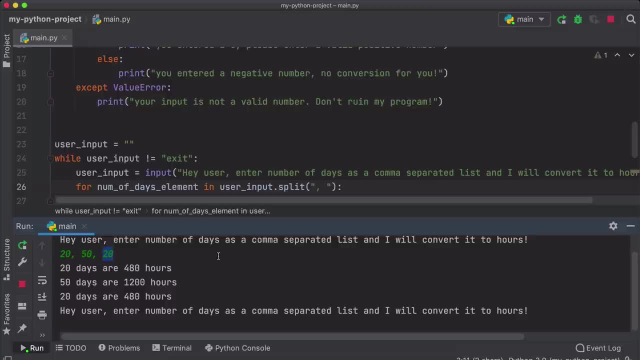 This could be bad values or things that That don't make any sense. So let's say we want our program to behave in a way that if a user provides the same values twice or three times, we only want to calculate the number of hours for that value, just once. 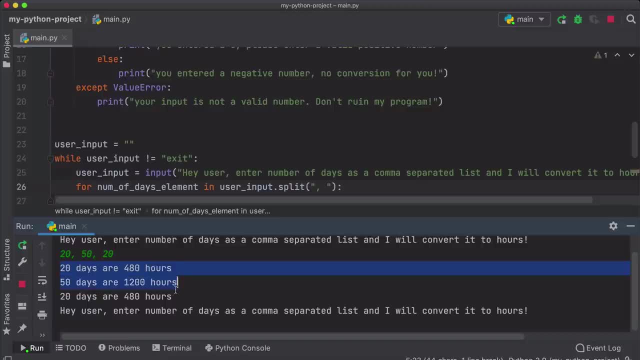 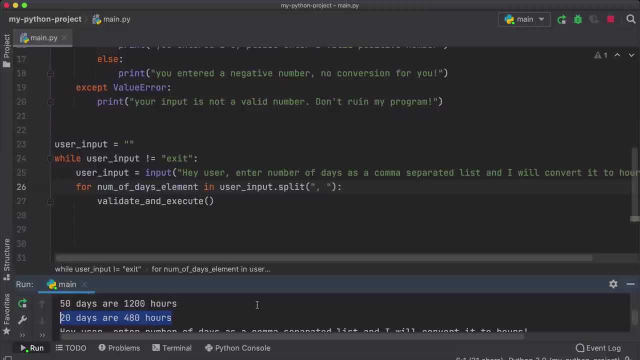 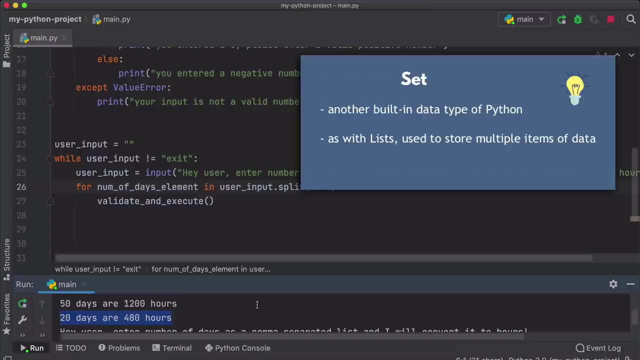 So basically for this input we want just those two lines and basically ignore the execution. again for the same value, And you probably already guessed that's where set data type will help us. So set is basically a list of elements, but with unique values inside. 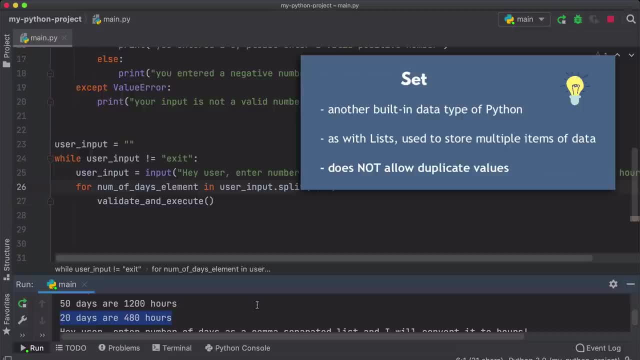 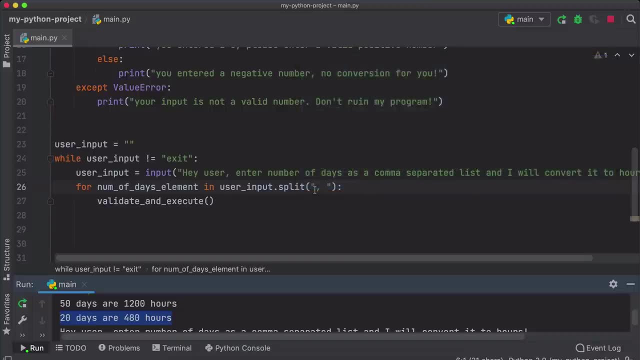 So list data type allows duplicate values: the same value multiple times. Set does not allow duplicate values. So how do we use set instead of a list? And it's actually very easy to convert an existing list into a set, And we can do that using a function called set. 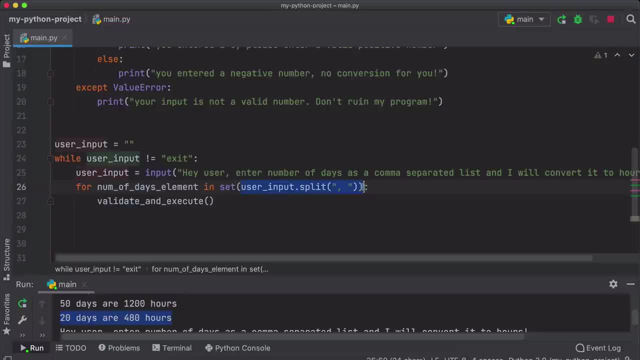 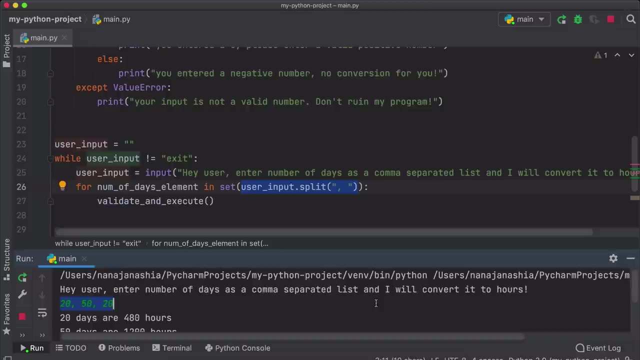 And basically the parameter of our set function will be the list. So if this list here contains any duplicate values, that will be basically just filtered out when we convert it into a set. So that's how it works. And again for demonstration, let's actually print out how set value looks like. 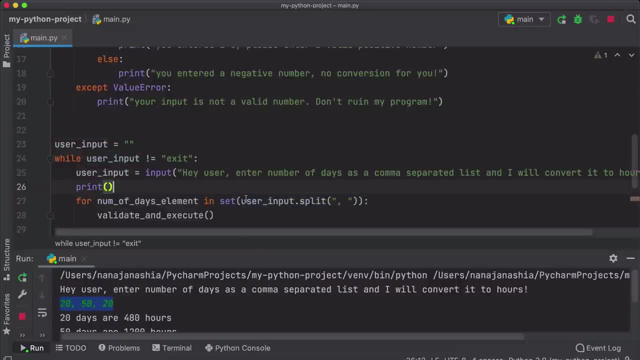 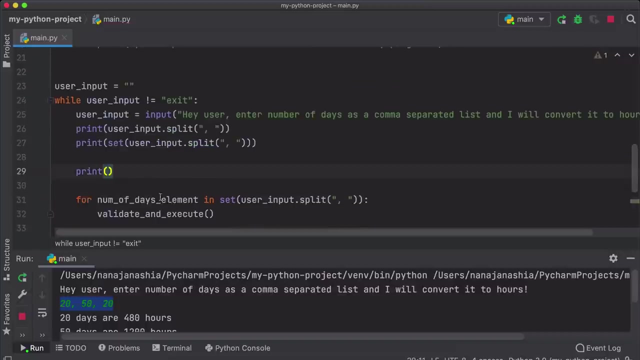 So I'm going to print the list first so that we can compare. Then we're going to print out set and let's also print out the types, And I don't want to repeat this expression over and over again. So what we can do, even though this is just for demonstration, we can actually extract it into a variable. 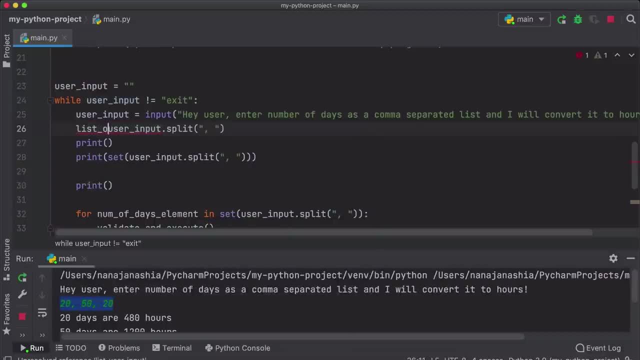 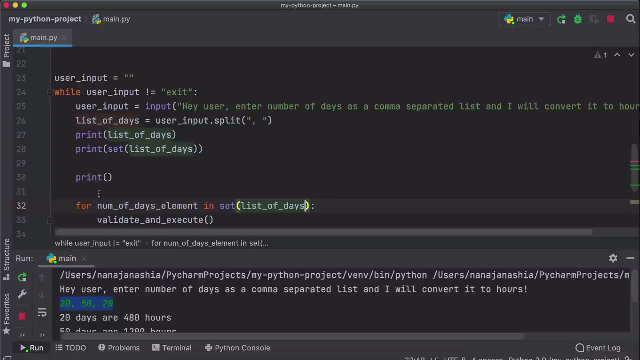 Let's say list of data, Let's say list of days, like this, and we can use it everywhere we need. And this is a little bit cleaner because we don't have to repeat the same expression over and over again And again. let's print out the type of list of days and then print out the type of a set of list of days. 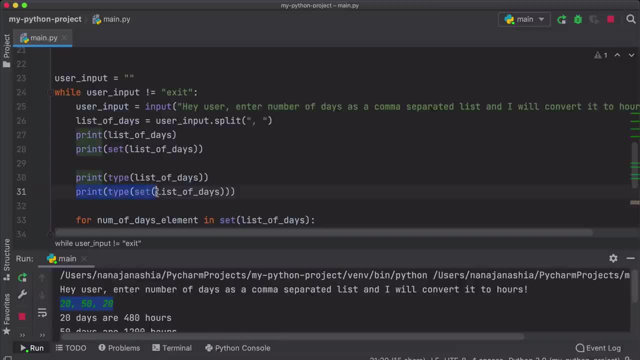 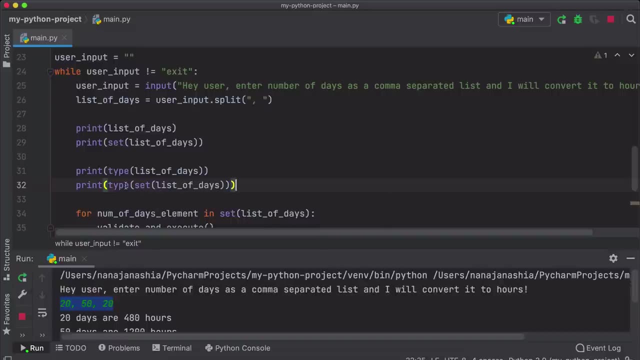 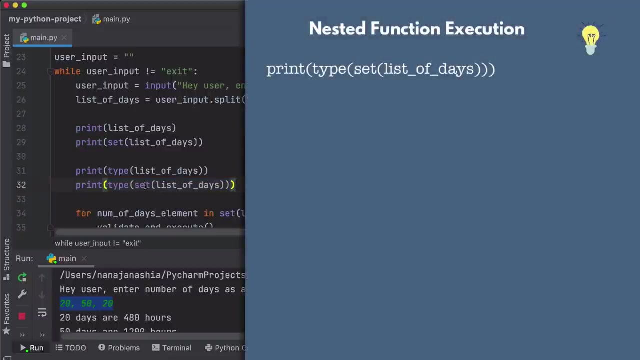 And again you see that Next function calls three times And this should give us some interesting value that we can compare list and sets. And just a small note here that whenever we have this nested function calls, think of the execution from inside out. 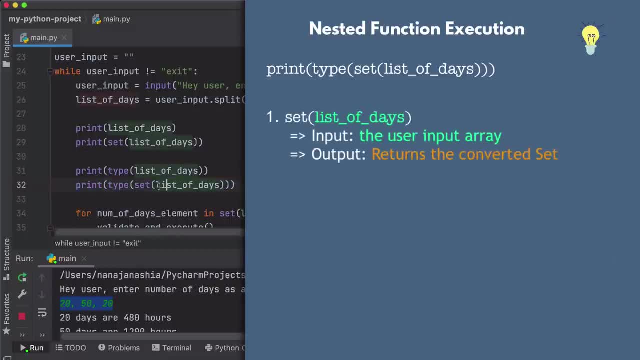 So the first function that will get executed in this chain is actually the set Right, So it starts from the last function in that chain. So set function will get executed and convert that list into a set, then type function will get executed on that resulting set value and then print will get. 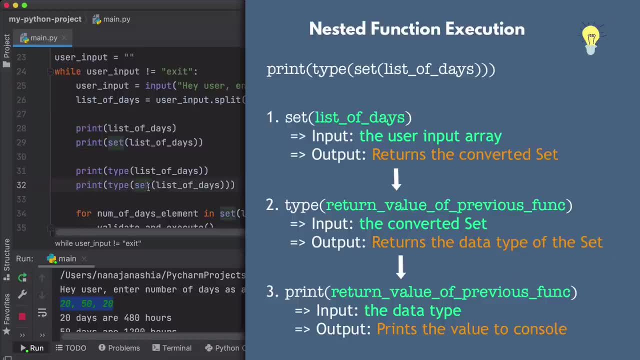 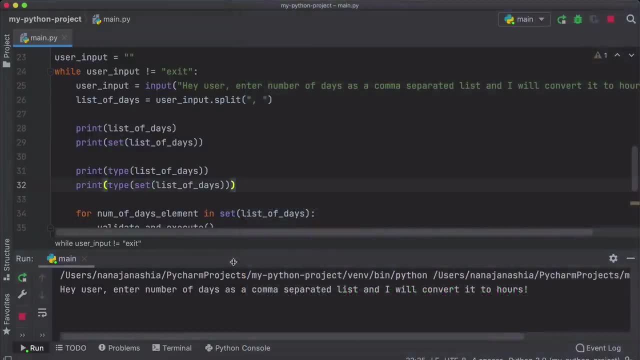 executed and print basically the result of the type. so the order goes from innermost function to the outer functions. so let's save it and execute. and now i'm gonna again provide a list. let's say 10, and then 45 and 30 and 10 again and enter and first of all we see that 10. 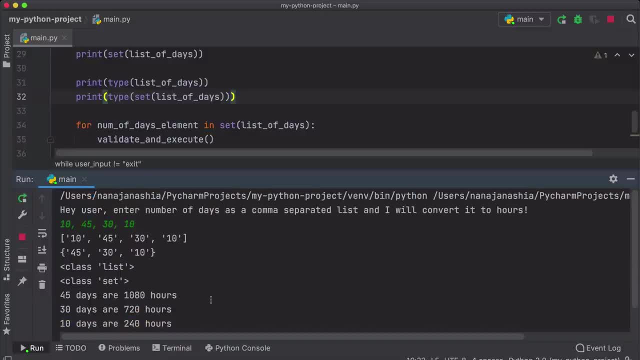 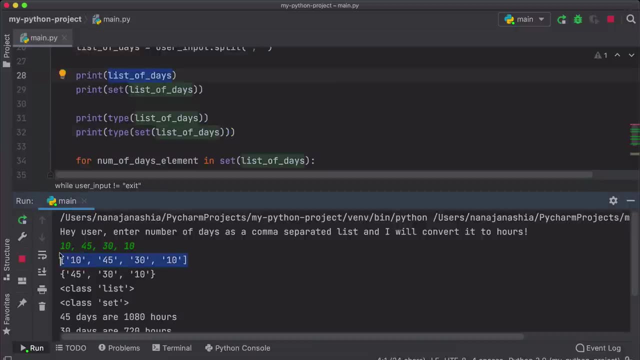 only got executed once and not twice, and we can also see. the first one is basically value of a list and you see the list here. the second one is a set and you already notice the difference. that list basically uses square brackets and set is represented using curly braces. 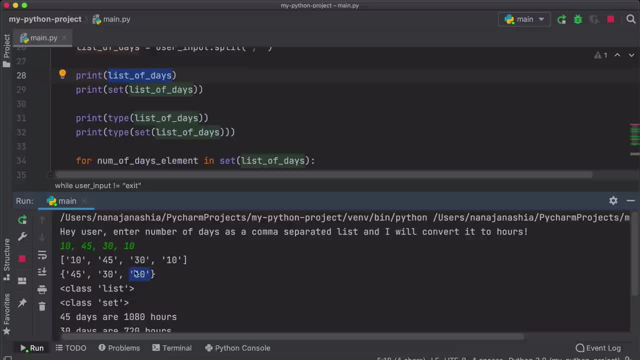 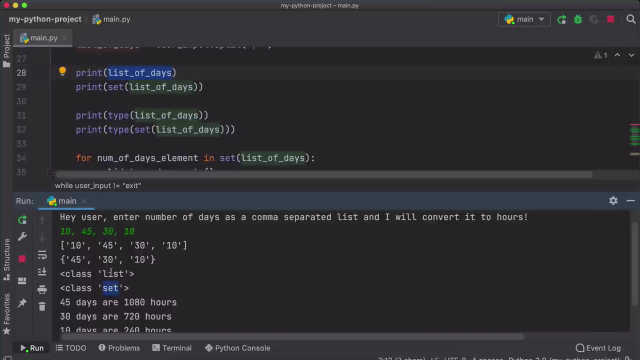 right, and again it has value of 10. just once and again we have the data 10 and we have the value of 10. just once and again we have the data 10, and again we have the data type of a list and a set. so just to demonstrate that they are actually own, separate data types. 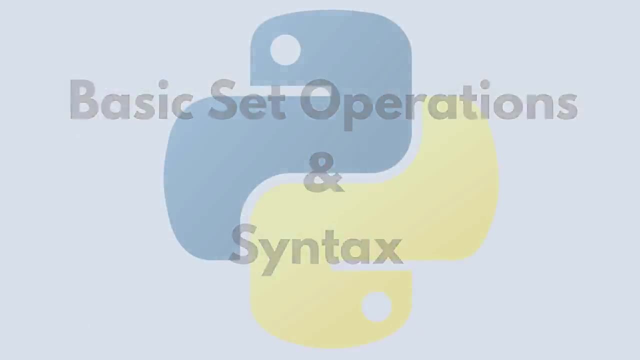 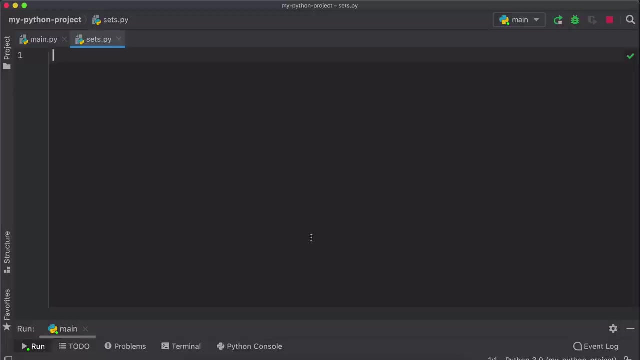 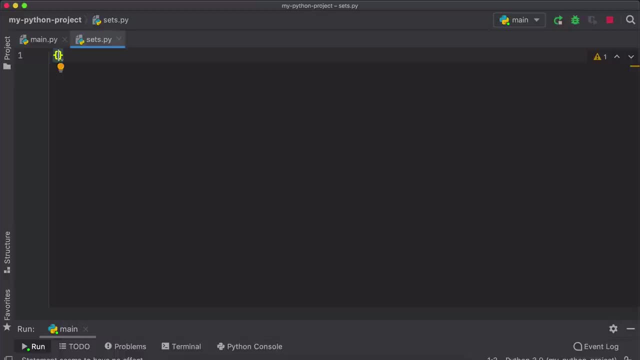 strings and a set of a list and a set of a list and a set of a list & pdl call and called these strings or numbers or pullians as its elements. let's use the same example we use with lists. so I'm gonna just basically: 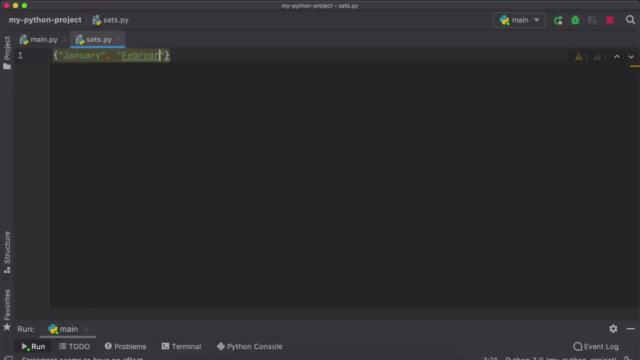 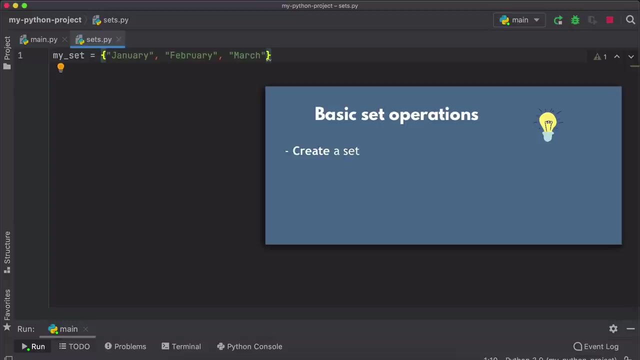 type in names of the month here. so let's say we have again January. Feb, March give us a set that we can create ourselves, not just from the user input, and now we can access the values, the individual elements from the set, and we can also add elements to the set. 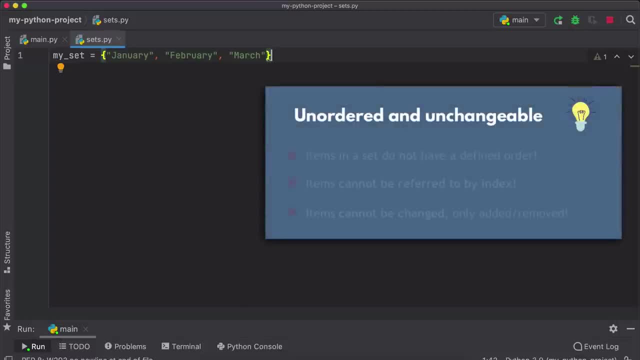 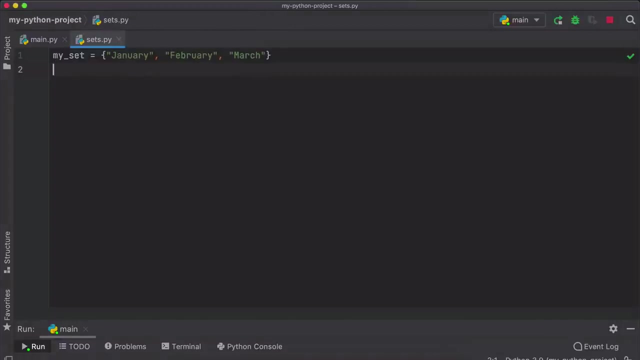 However, we cannot access the individual elements of the set like we did on lists, Right, You remember, on lists we use the syntax with square brackets and the index of the element. in sets We cannot actually do that. Instead, we can only access the elements of a set in a loop. 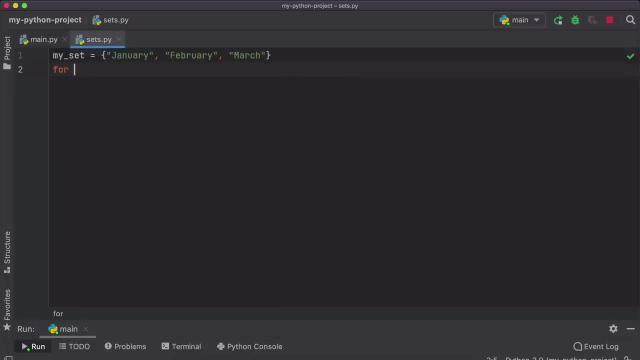 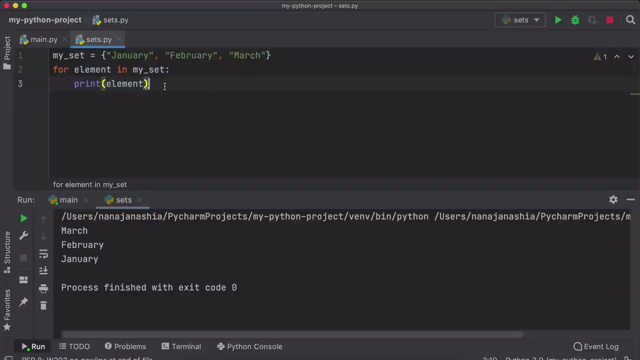 So, for example, in a for loop, we would write elements in my set and then we can basically print that element. So let's execute, And right here you see all the elements printed out. And again, as I mentioned with lists also previously, most of the time when you're 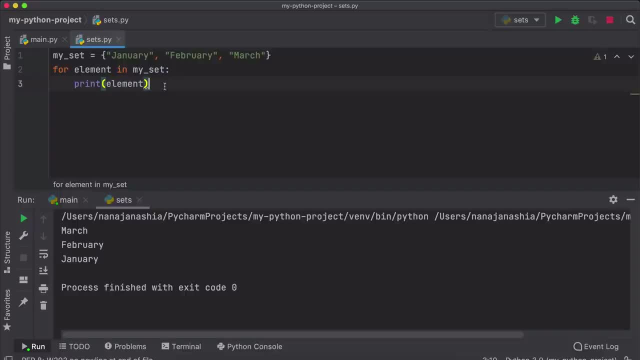 working with lists or sets, you're going to want to look through the elements, because you probably would want to do some operation on individual elements or some of the elements Right, Instead of just grabbing individual one or two values from that. Now, how do we add elements to a set? Let's see it as well. We can add elements to my set. 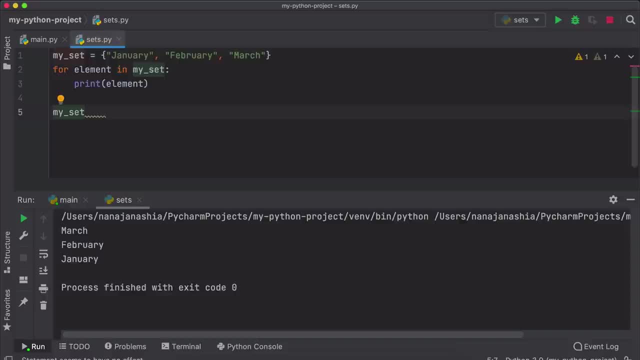 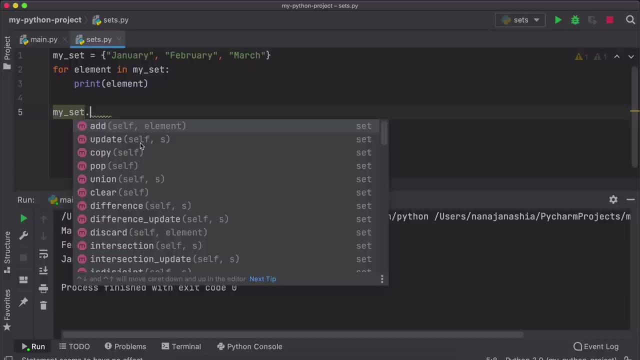 using my set, So the set itself, the variable name, And then, if you do dot, you see a bunch of built in functions. Again, set has its own built in functions which are completely different from what list has, And it has a function called Ed. 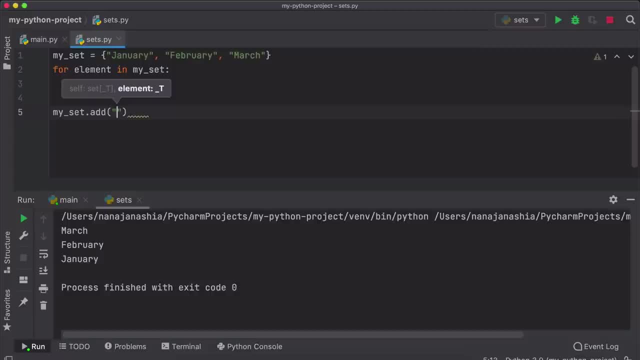 And here we can basically add a new element Again. let's do April, and now we can print my set And execute, And there you go. So we have here individual elements that are printed out and we have the new list after we edit April. Now one thing you probably already noticed: 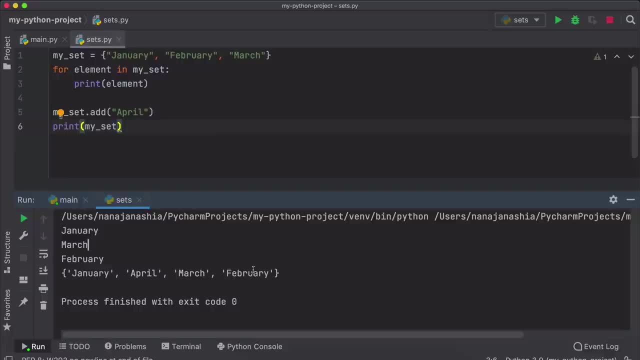 when working with the set, like printing its elements or adding a new element, it doesn't work in the same sequence as with a list right. So for list we basically had this: January, February, March, March, April, March, February March February, March, February, March. 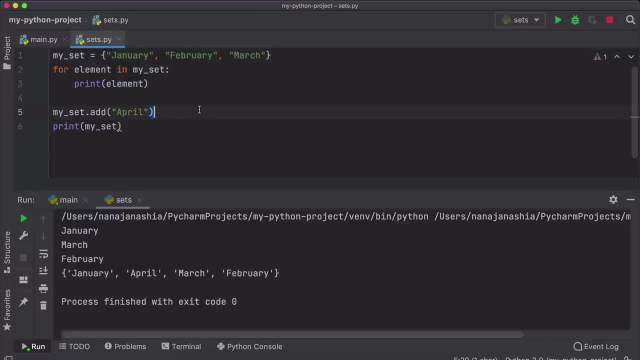 March in this exact order And when we added a new element, basically it got edit at the end, right, as a fourth element in said it's not order, It's basically in a random order, right? So if I execute this again, we run. you see the order changed here and here as well, Right? 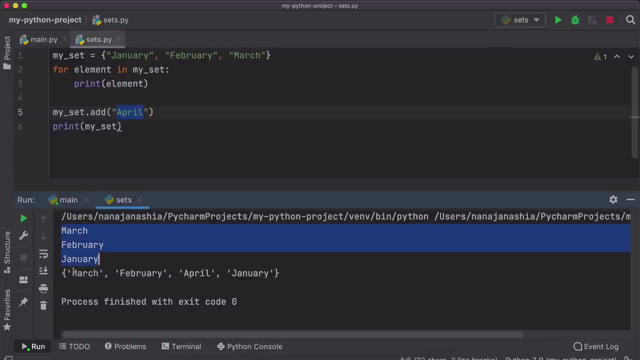 And if I do it again, there you go. So this order and this order basically changes right. So So, as you see, working with sets is actually pretty different from working with lists. So this means that set not having or not allowing duplicate values is basically just one of. 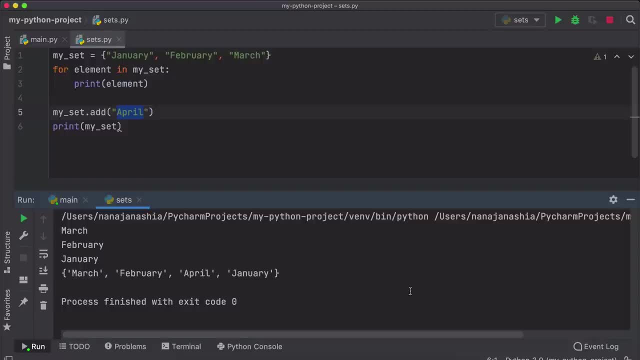 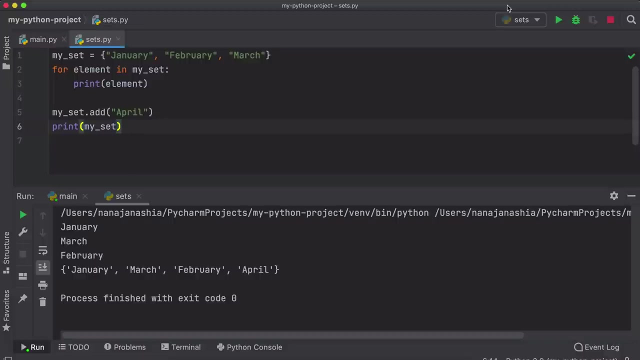 the differences between sets and lists. And of course you're probably wondering: I can add elements, I can access elements. What about removing elements right from lists or sets? And you can do that actually the same way for both sets and lists. 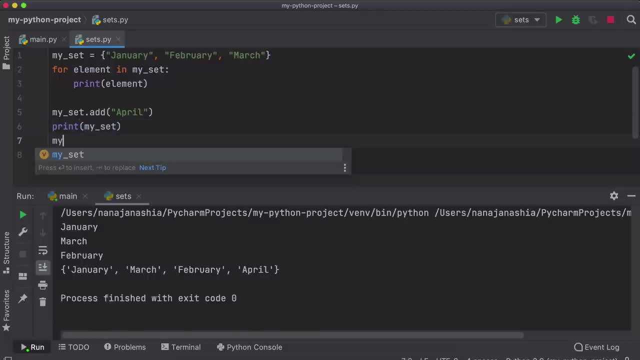 So, for example, if we want to remove an element from a set, we can execute a built in function called remove, and remove basically takes a parameter which is the value itself. So let's say, if we want to remove January from here, then we're going to pass the value. 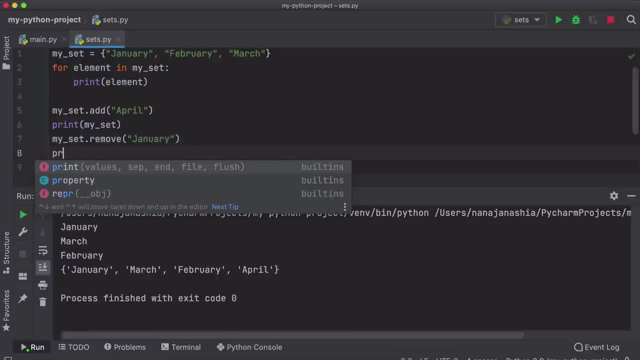 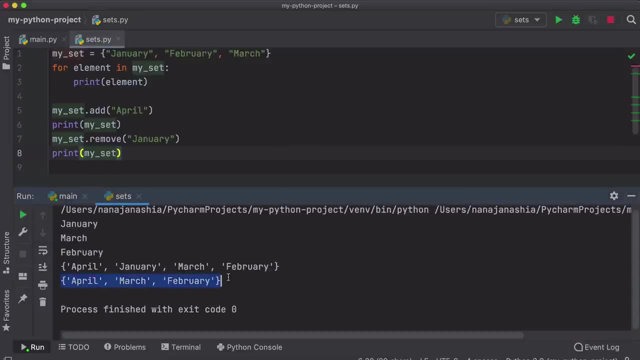 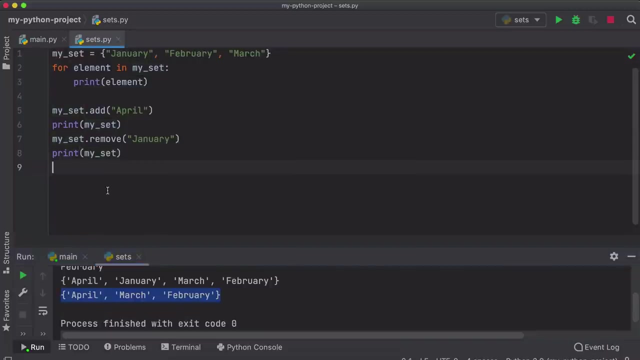 to remove function. And now if I print my set again after the remove gets executed and let's run it, And here you see, the last print basically doesn't have January inside And, as I said, it works the same for lists. So let me demonstrate that as well. 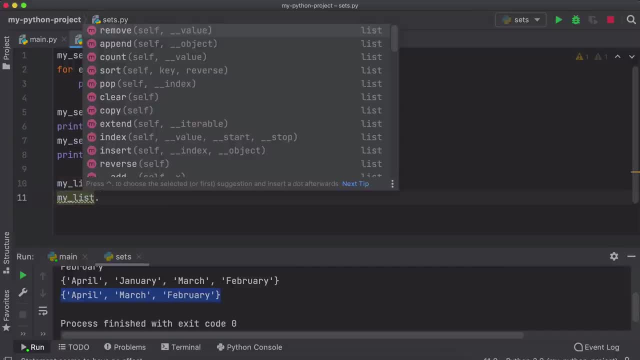 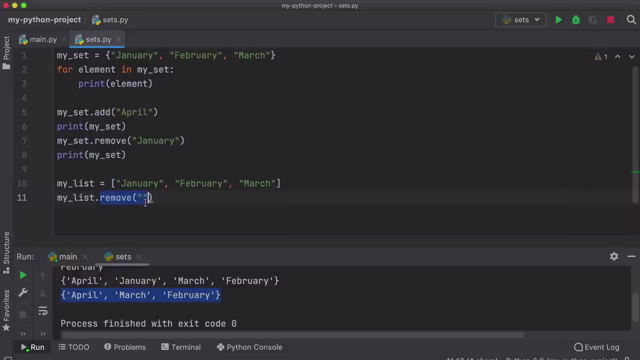 So on my list, which has its own set of built in functions. one of them is remove, which in this case is called the same for both sets, Set and list, And this remove built in function also accepts the value of the element you want to remove. 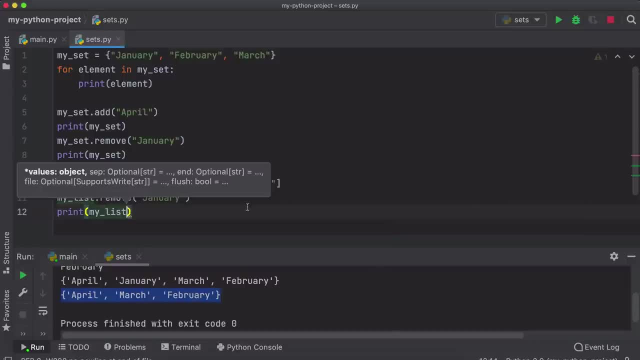 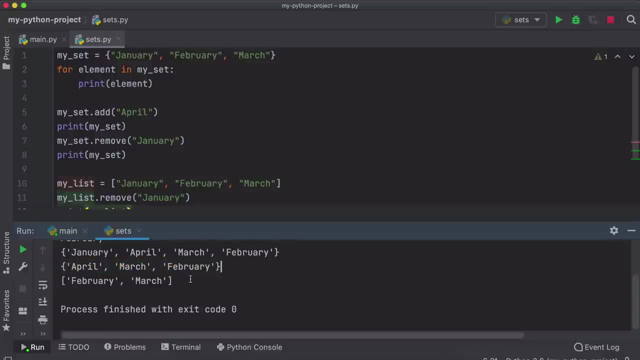 And let's print it again, My list: Execute. There you go. This is a set with the syntax, with curly braces, and this is a list which now doesn't have January inside because we removed it And, as you know, this can have duplicate values. 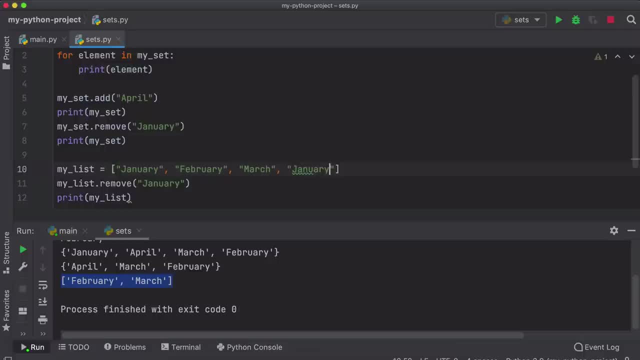 So if we have January again here, So two times, and we do remove January, it will actually remove the first occurrence of that value. So if I execute this, you see the first one got removed and the last one or the second January value is still there. 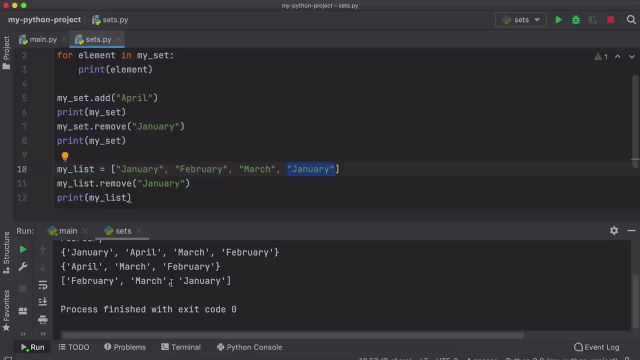 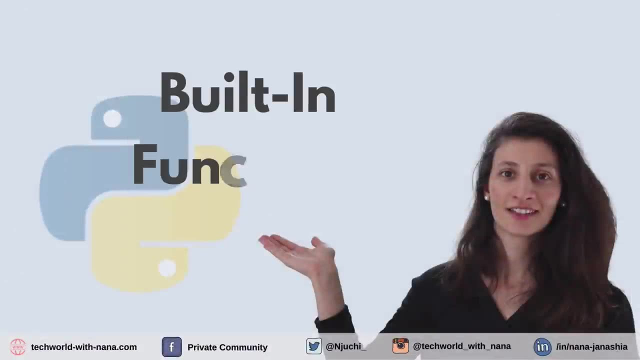 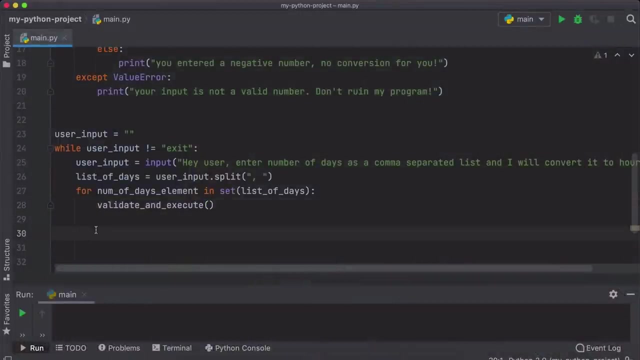 So that's how you work with sets, basically, and also how to remove elements from sets and lists. So at this point I want to take time and review the functions that we have used from Python itself, So the functions that we ourselves didn't actually write and the functions that Python 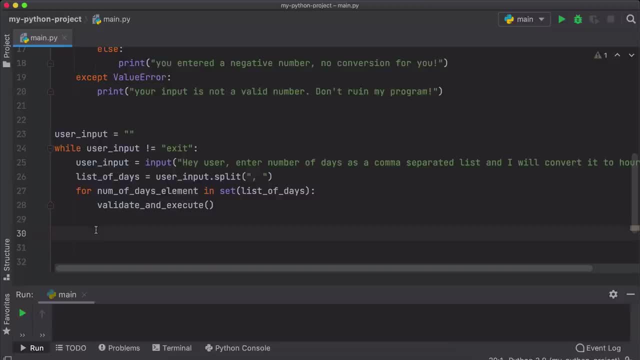 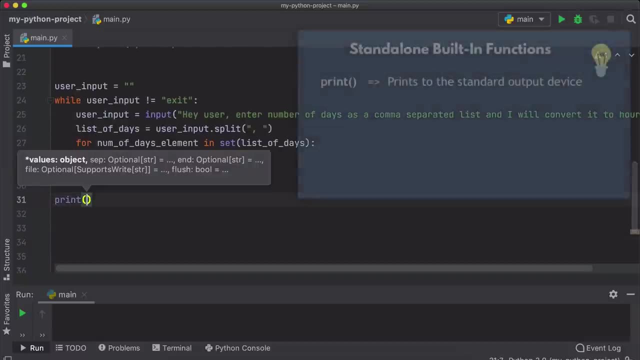 basically makes available for us to use are called built in functions. So till now we have used function print, which basically just takes Some input- This could be a string, This could be a variable, This could be a number, doesn't really matter- and basically just prints it in the output. 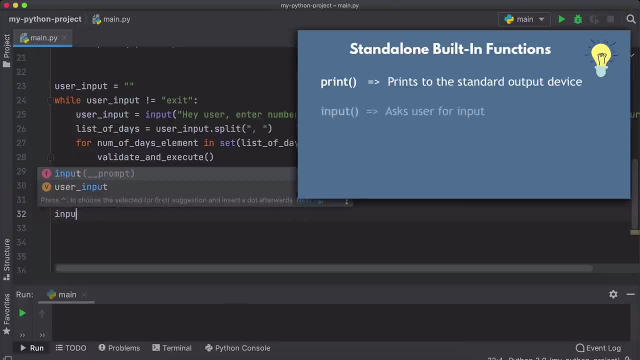 console right in the terminal. We also saw input function that basically takes user input. Again, we can provide a parameter which will be a message, or leave it empty. We also in the last example. so an example of set function Okay, Which basically takes a list and converts it into a set. 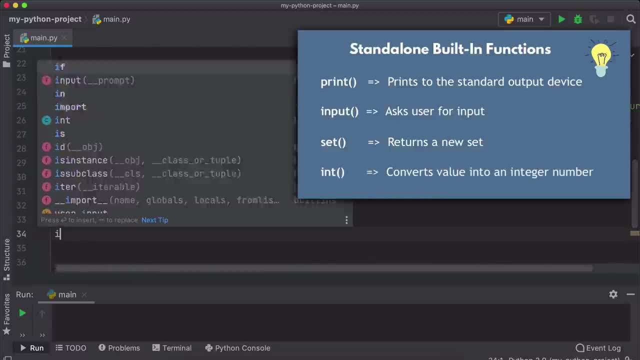 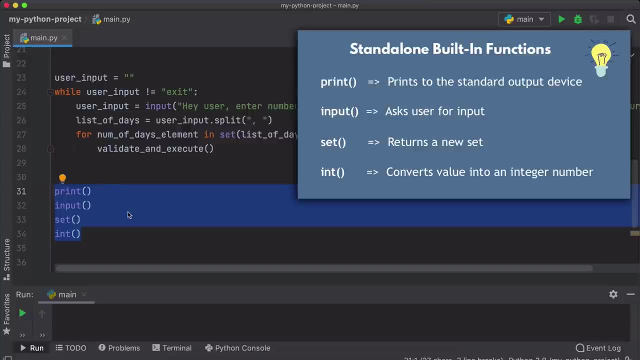 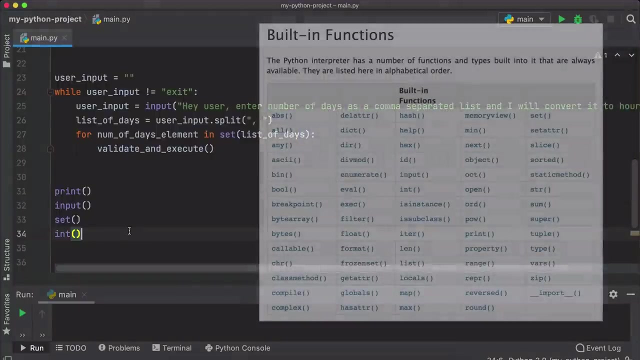 And another example is: int again takes a string as a parameter and converts it into integer. And all of these are built in functions because Python provides them to us so that we can use it in our code. And in Python there are a lot of very useful built in functions for different purposes. 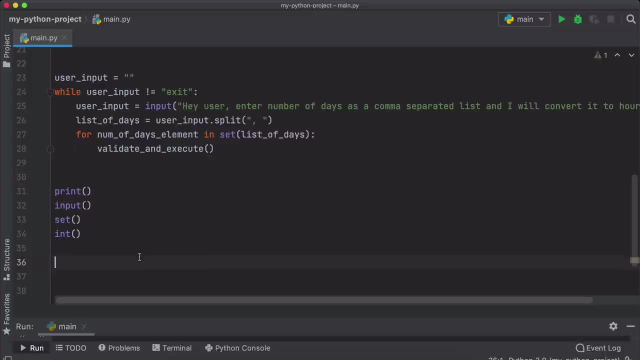 And, as I mentioned, most of these functions, We accept a parameter and then do something with that parameter, that input, that we provide that function and give us an output again. print basically provide something here and gives us the output in the output window here in input. 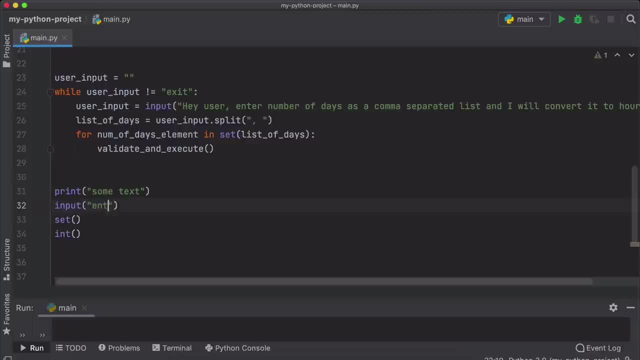 We can provide some message. There will again print input here and the rest of them are giving value. So we can provide a list and, the same way, a parameter here, which is logical because the purpose of a function usually is to take some input like this as a parameter: do something. 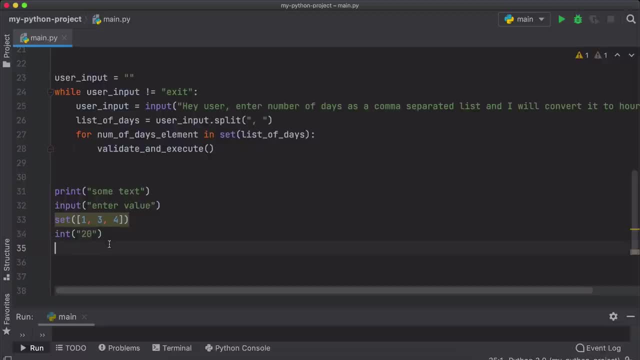 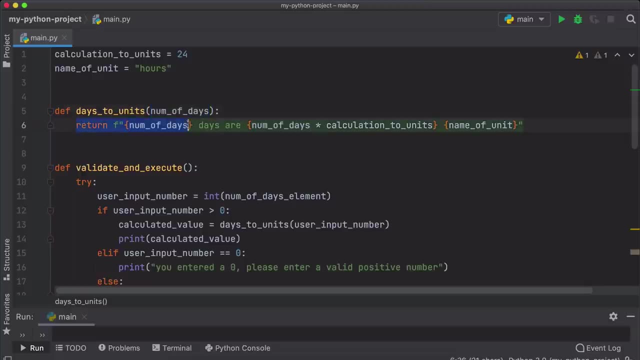 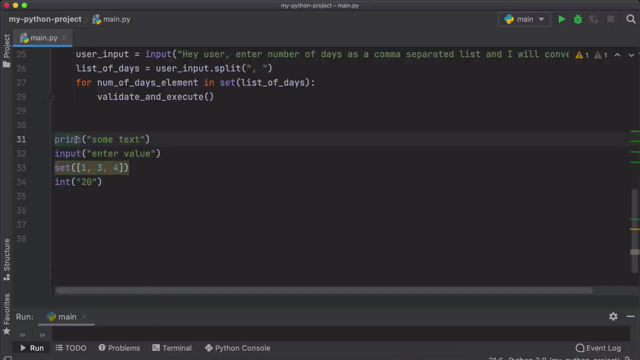 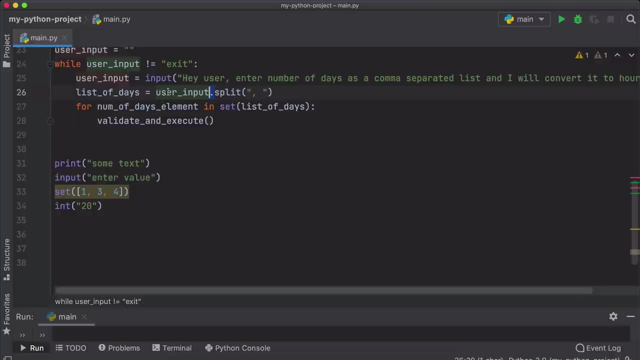 with that input and give us an output from that parameter. And we have created our own functions that also take some input And give back some output like this: And in addition to built in functions that are called like this and our own functions, we have also used the third type of functions, which is called directly on a value right. 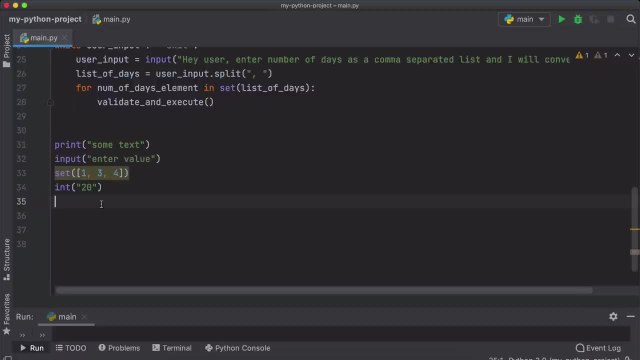 And this is an example of that, So basically directly on a value. this could be a variable, but also the string representation of that itself. So if I had a string like that, So basically directly on that value, call a function like this: 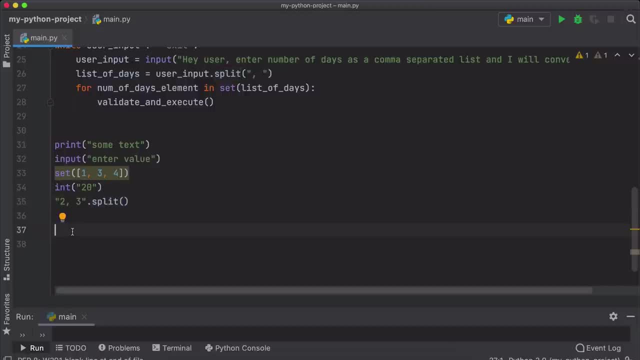 And these are also built in functions because Python makes them available to us other than the syntax. There is one major difference between this type of functions that are called directly, like that, and the functions that are called on the value itself, And the main difference is that each data type has its own set of functions. 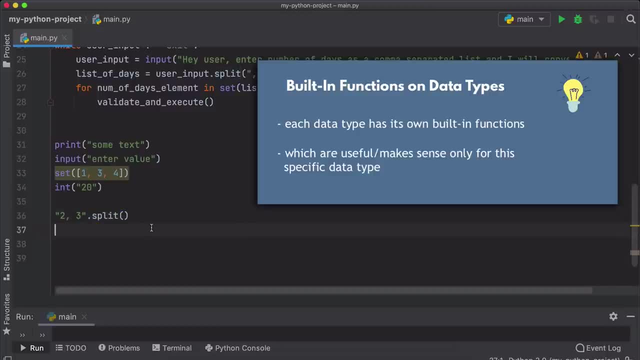 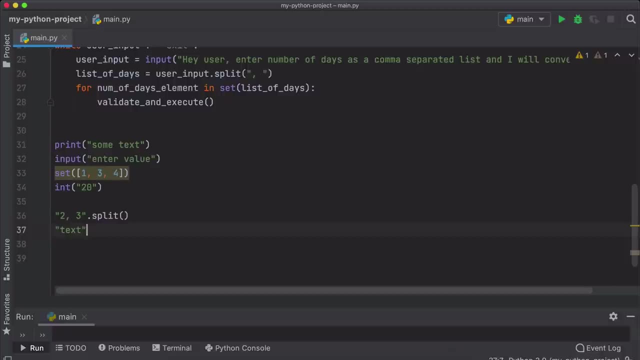 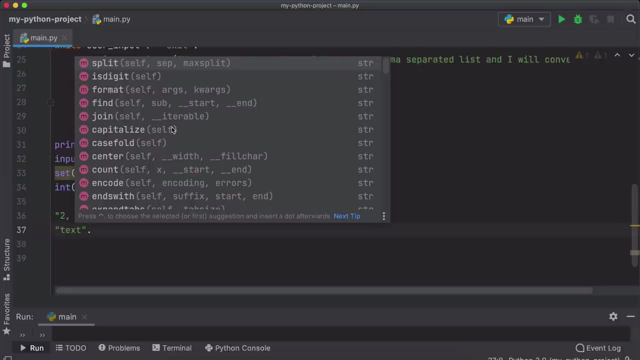 that can be executed like this. so again, let's take example of a string. and if I do dot here, you see the IDE pie charm basically gives me a list of all the functions, again built-in functions in Python, but functions that I can execute on a string value. and again you see, split is digit. 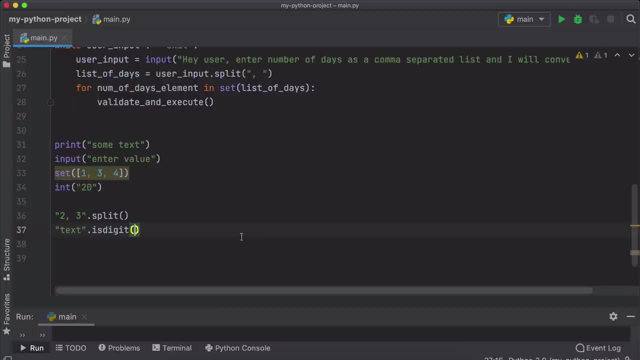 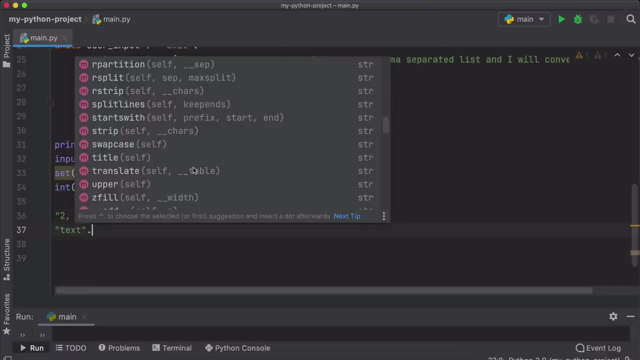 this is the one that we use in one of our previous examples. that basically checks if that string is a representation of a digit or just the regular string and, as you see, lots of different functions. so all of these are provided by Python to do different stuff, like turn the string literal. 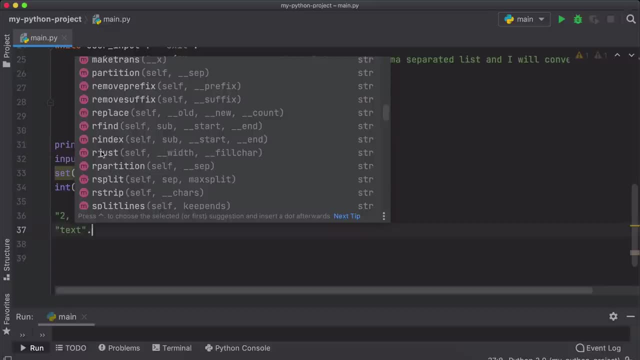 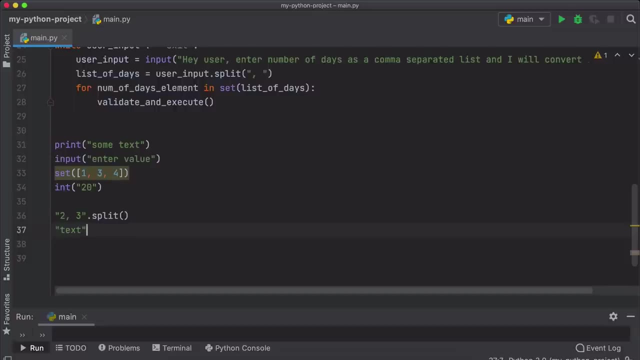 to uppercase or replace a letter, for example, in that string and so on. but the main point here is that those functions are only for string but, as I said, each data type has its own list of functions that can be called on that data type. so for a demonstration, let's take 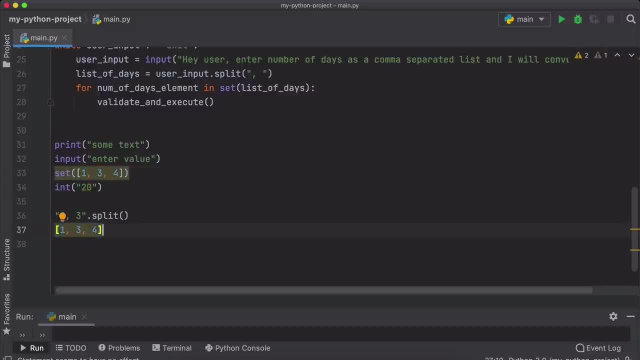 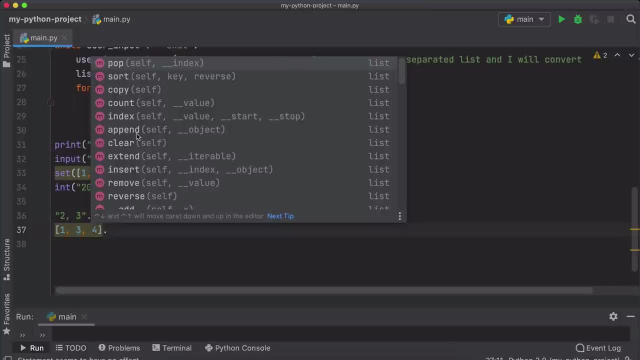 a list and if I do dot here again, you see a list of functions that I can execute specifically on list values. and there are lots of functions that I can execute specifically on list values. and there are lots of things that you can do with lists, like add elements to it, remove elements from it. 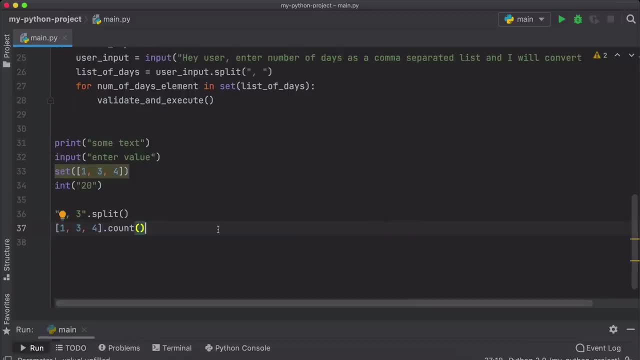 sort the list, copy and so on. so that's basically a major difference between this type of functions and functions that can be executed on specific data type values, but the concept is the same. here you also have a function that gets a parameter, an input, and gives you an output, and the parameter for this type of functions is actually the. 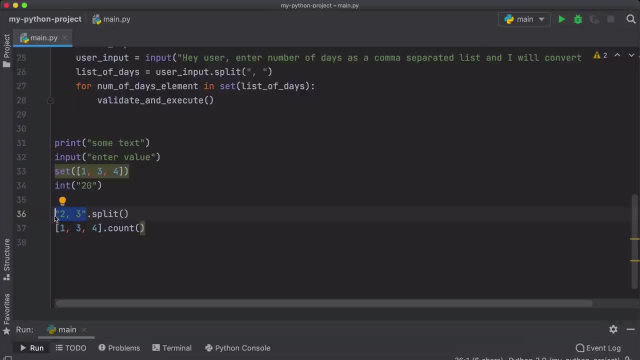 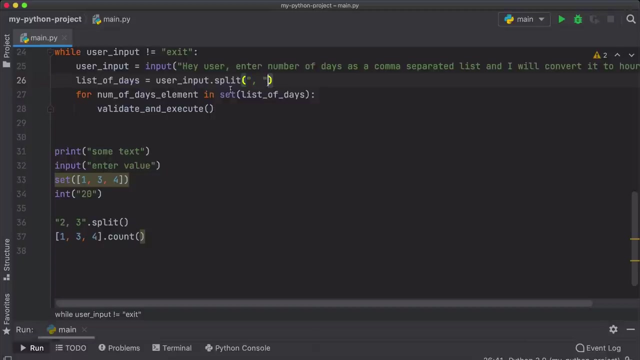 the value that we are calling that function on. So the string here to three is going to be parameter of the split, And in addition to that we can also provide additional parameters, For example for split. you saw here that we were able to add a comma space to tell the split function on which character to split that text. 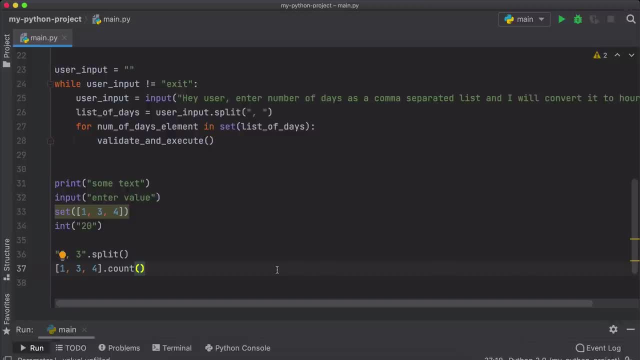 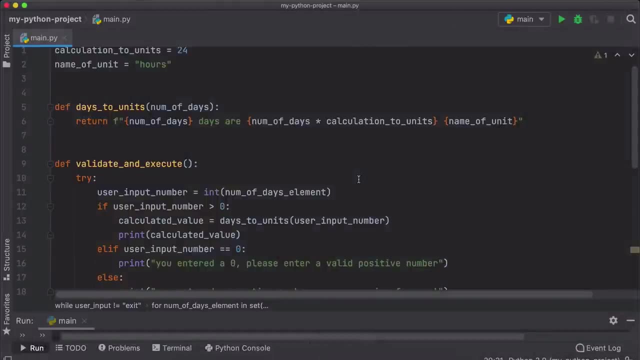 So that was function comparisons in a nutshell. In this part we're going to learn a new data type in Python called a dictionary, and we're going to do that by modifying our application and modifying how users can actually input the values. Now our program currently takes the number of days and turns it into a number of hours. 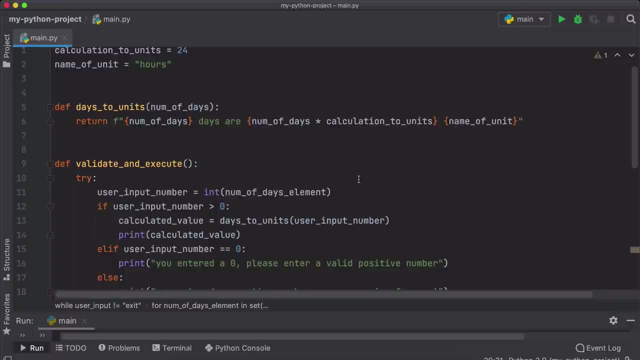 What if we wanted to make our program a little bit more advanced, a little fancier, and basically allow users to also decide what you're going to do with that data type? Well, you know, we're going to have to look at how the user should convert a number of days into hours. 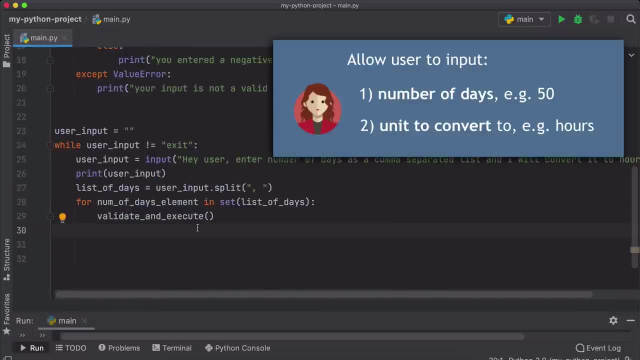 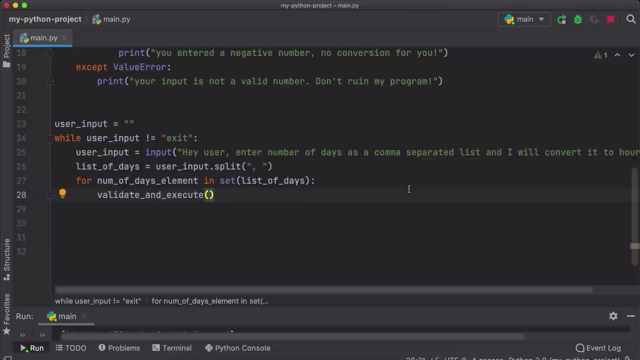 and what are the conversion units it should be converted to. So user gives us the number of days and tells us whether to convert it into hours or minutes. So instead of the whole list now we're going to get just number of days and the conversion units. 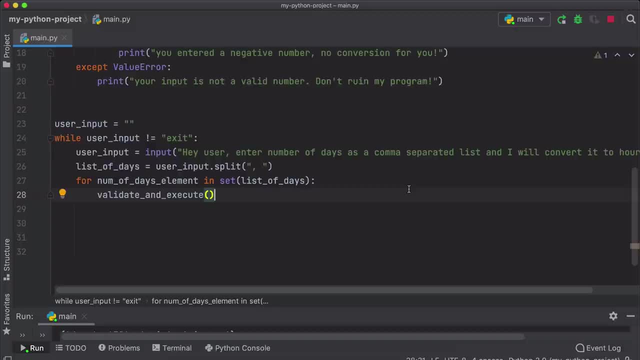 And this change may be a little bit complex in terms of syntax, So I will try to explain everything step by step. user to be able to give us the number of days and units in one input. So first of all I'm going to adjust the text here. enter a number of days. 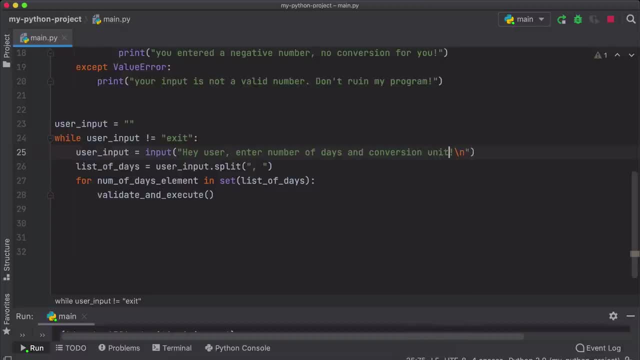 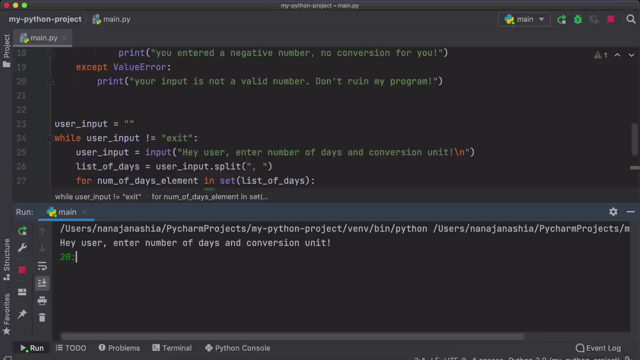 and conversion unit. Now, there are a lot of different ways we can allow a user to do that, But what we want to do is something like this as an input. So basically number of days, colon and minutes, or number of days and hours. 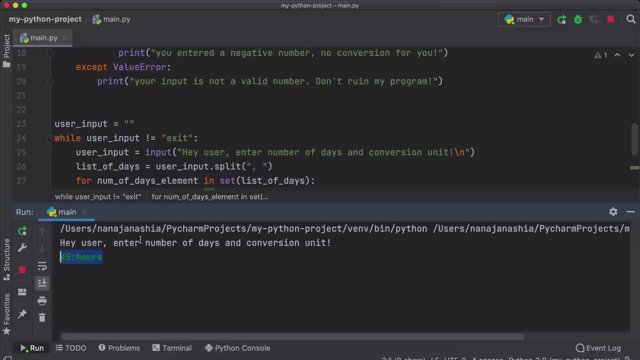 Again, this is our own decision. We decide how the user input should look like, But this should be a nice way of providing both of those values, basically colon separated. So instead of a list, we're going to have a single input with two values. 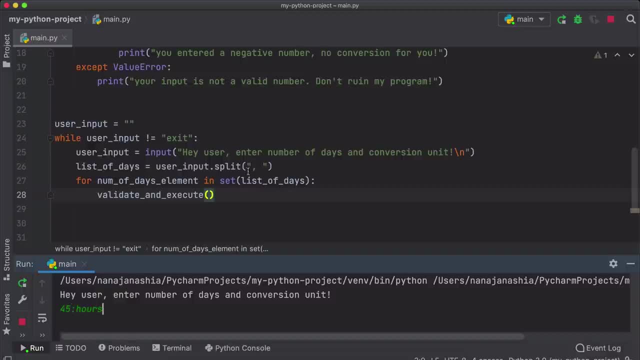 that are separated by a colon. So on the next line, I'm going to change this split here into a colon and this will give us user input. This whole value, split into two values, is a list. This is going to be day and days and unit. 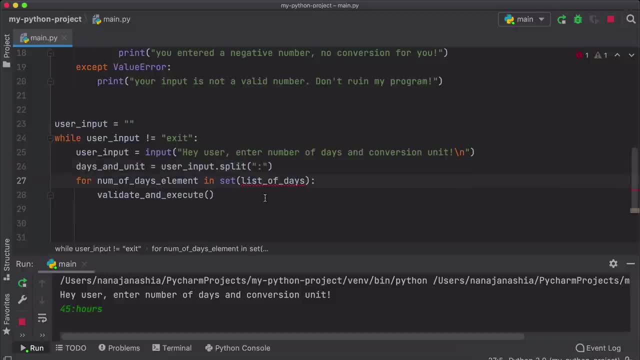 So list with these two values and let's actually get rid of these four loop, because we're not iterating through a list of numbers anymore And to begin with let's just Print out the output or the results of days and units variable. So I'm going to refresh and let's do two hours and enter. 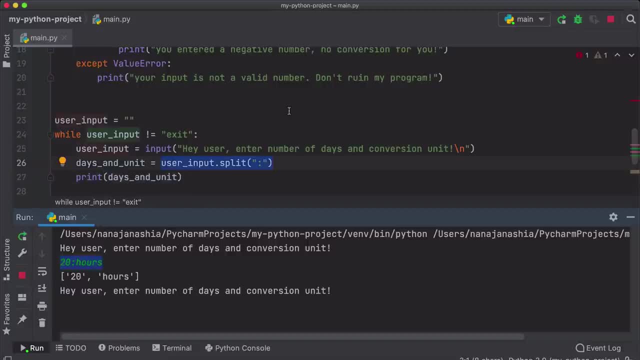 And this is what we get. So, basically, splitting this string on colon will give us a list with elements 20 and hours, and note that 20 is still a string, right, Because that's how we get the input. And now from those two values, 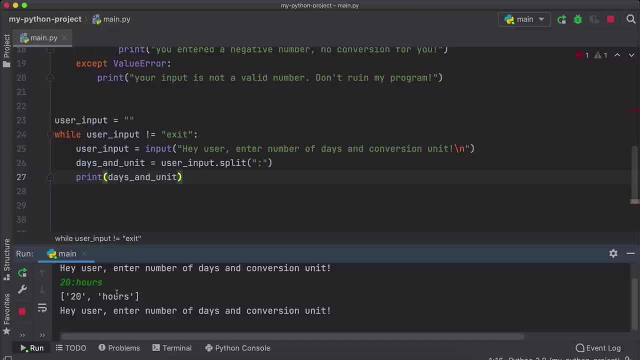 we're going to create a value of a data type called dictionary. So in Python we have another data type called the dictionary, which basically looks like this: So you have curly braces, just like we had for a set, And inside we have key value pairs. 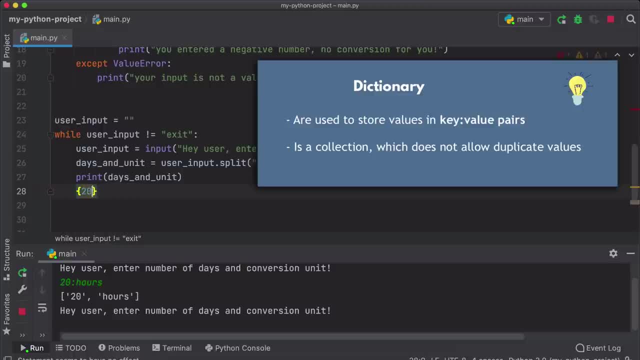 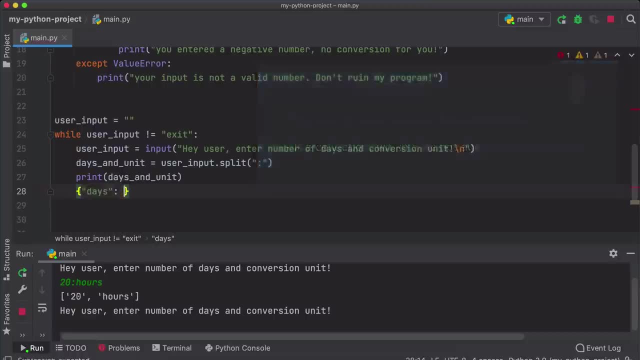 So we don't have just single elements like this, but rather we have key value pairs. So key in our case we have key value pairs In our case is days, and the value of that key in our case would be 20, and then comma separated. 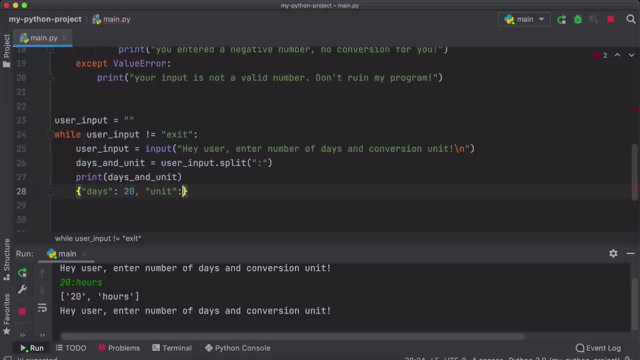 Another value would be unit and a string hours. So basically, this is the syntax of a dictionary And obviously the difference between a list and a dictionary is that we have descriptions for each of our values. So we want to create a list of our values, represented as key value pairs. 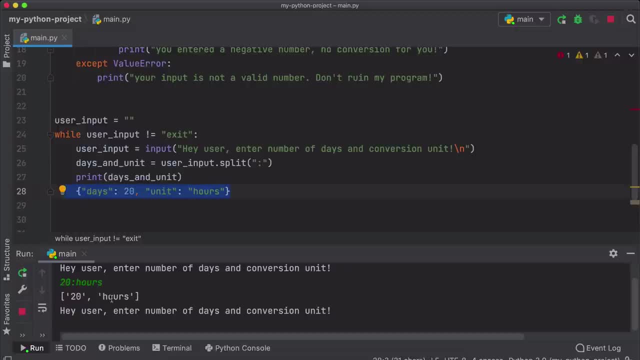 So we want to create this construct right here from those two values And since this is a data type, we can create a value and assign it to a variable of that data type. So let's call it days and unit dictionary equals. And obviously we don't want those values to be hard coded here. 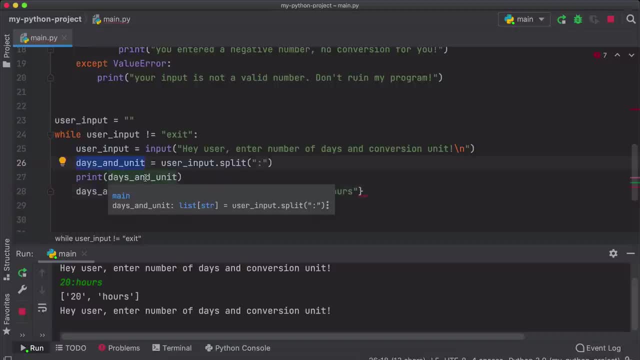 We want to get it From the list. Now, how do we access an element of a list? How do we grab the first value, which is 20, out of that list? And to do that, there is a syntax to access the elements in the list. 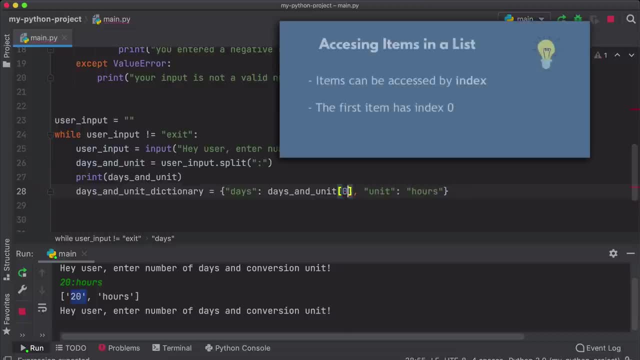 the list name and then you have square brackets and index of the element which, if you remember, you already learned in the section of lists. So again, days of unit list. is this one right here? and with index zero we are accessing the first element, index. 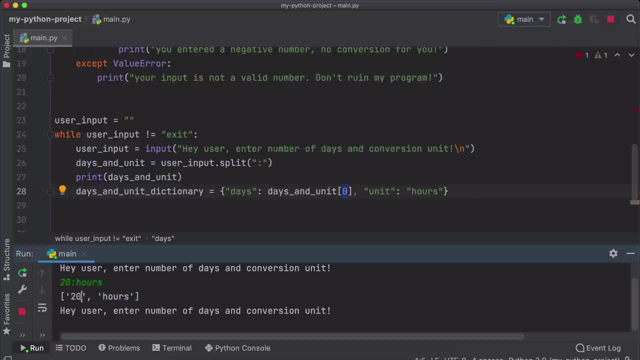 One is the second element, and so on. An index is basically just location, This is location zero, location one, and so on. So this will give us the first value And obviously the second value is going to be the same syntax with index one. 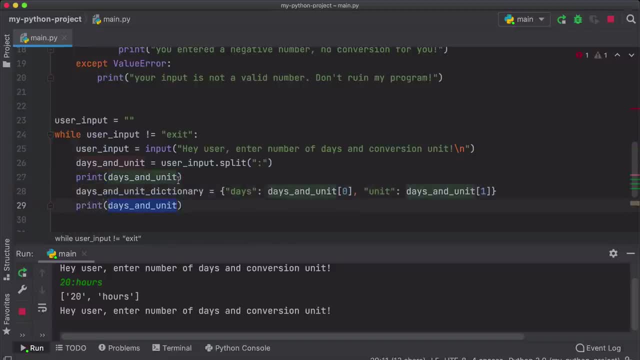 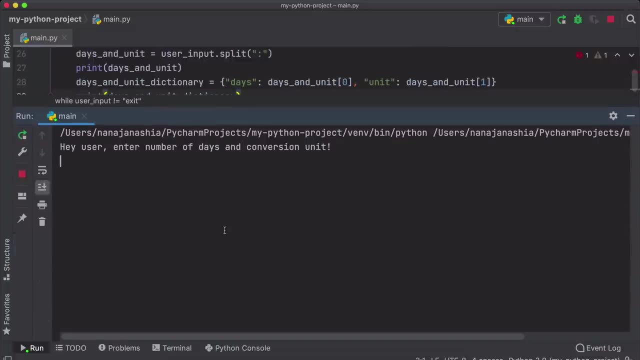 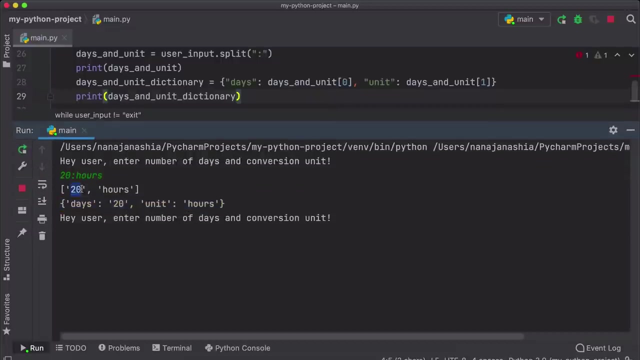 And let's actually print that one out as well, So that we see the results. restart the application. Let's do 20 hours. So again, this is our list: 20 hours as two separate values And this is a dictionary that we created using those two values. 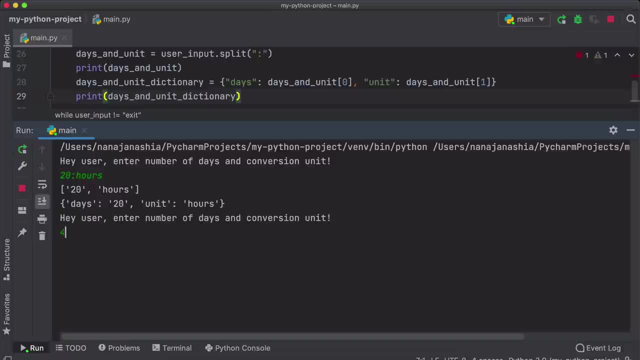 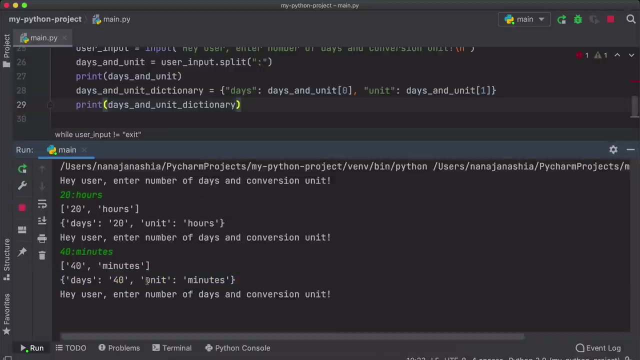 So we have key value pairs, basically And the same way for minutes. we would end up with a dictionary that looks like this. So now we have these two pieces of information in one variable, And now we can give that variable to our function so that it does the validation. 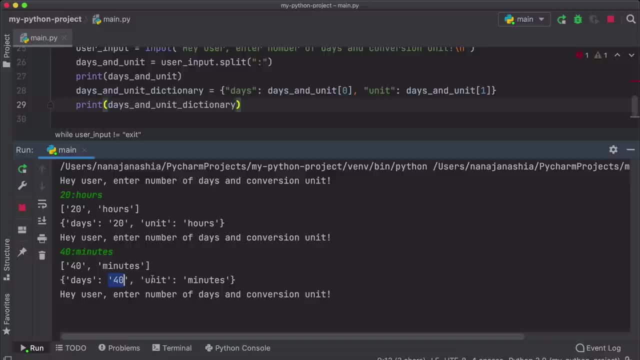 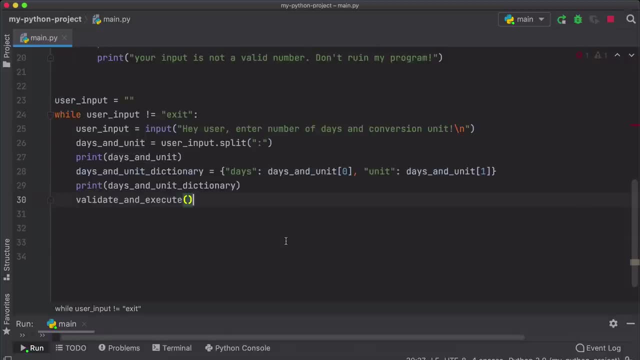 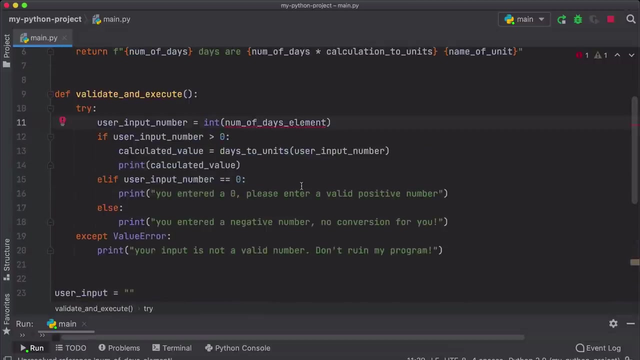 first of all of the number and calculation based on the units. So on the next line we're going to call our belly date and execute function And, as you see, we have this red line here because something is wrong First, so we don't have this variable called number of days element anymore, because we deleted the for loop instead. 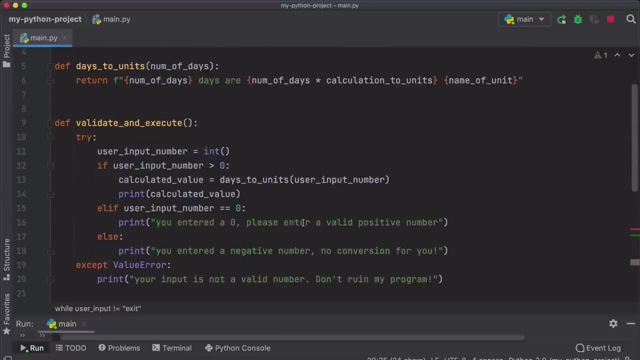 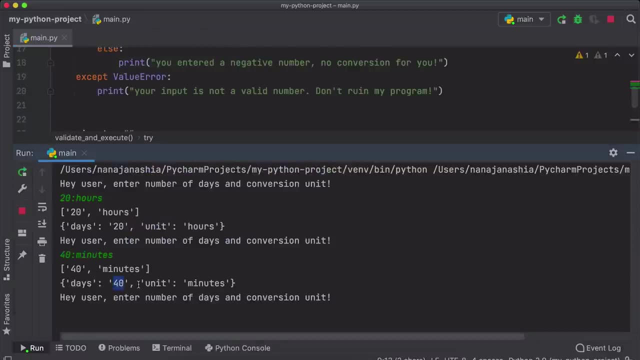 We have days and you need dictionary, and here we are validating the integer value of the input number in the same way. We need to validate this input number here as well. So now the question is: how do we access a specific value in this case? 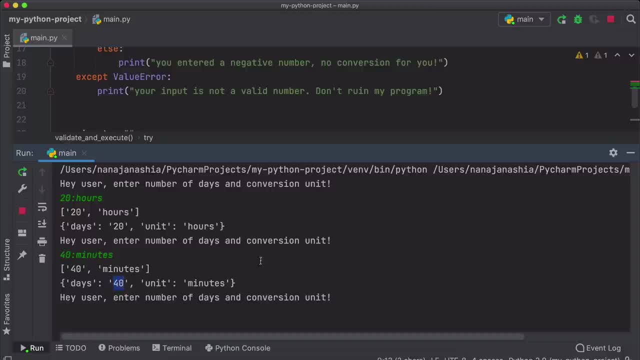 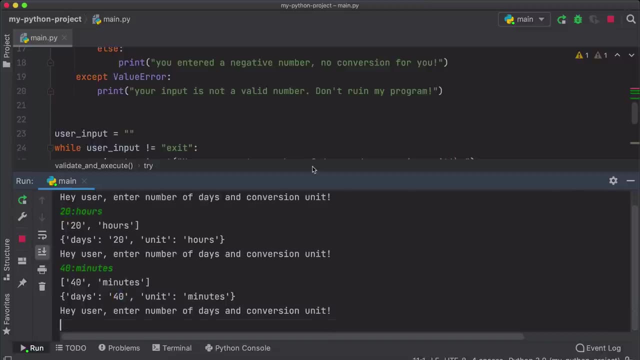 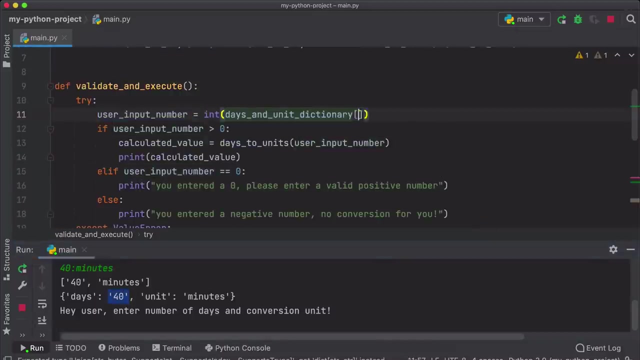 The value of days here in a dictionary, because we have to validate this value as well, because I might as well have entered text instead of this number. So the way to access values inside a dictionary is again using the square brackets, just like we did for list. 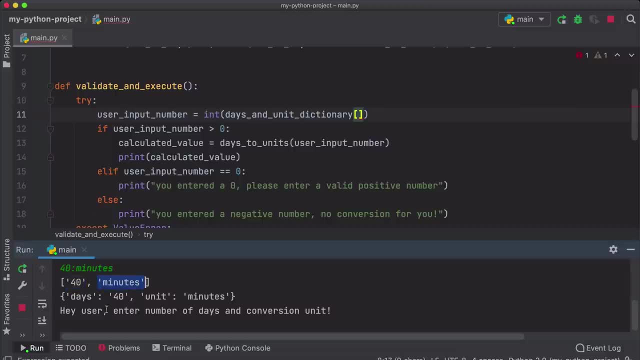 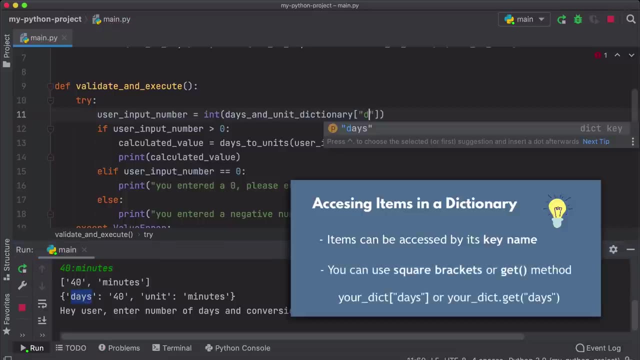 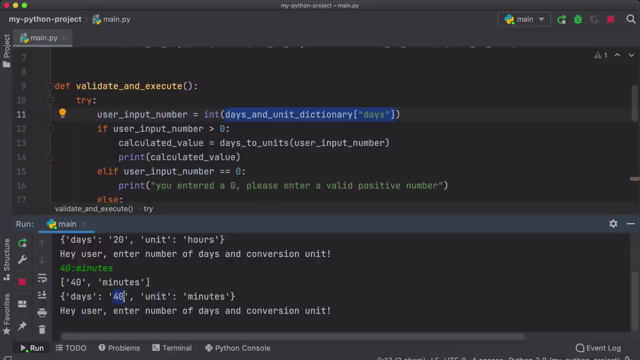 But instead of an index, index zero or index one- we don't need to use an index because we actually have a key. So instead of index, we're going to use the key like this, or unit, And this will give us value of 40,. 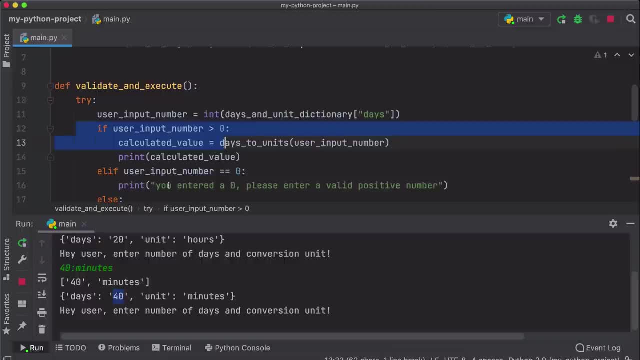 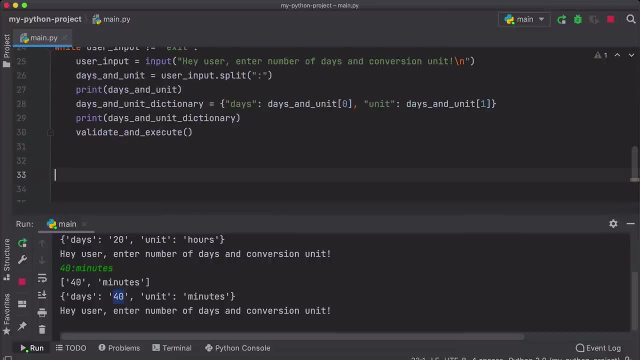 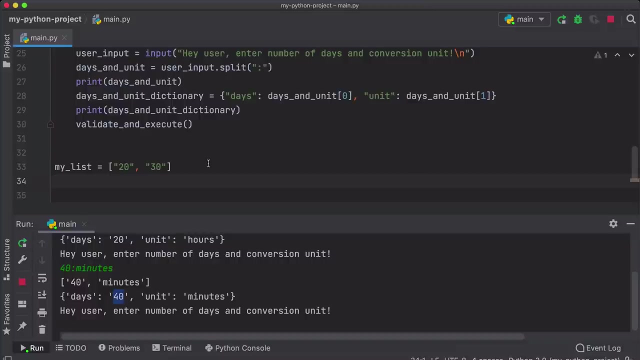 which will then be converted into an integer and then validated right here. So again, I'm going to copy this for comparison. So to access an element of a list- let's say my list here, and let's do 20,, 30,, doesn't matter- in order to access the elements of that list, 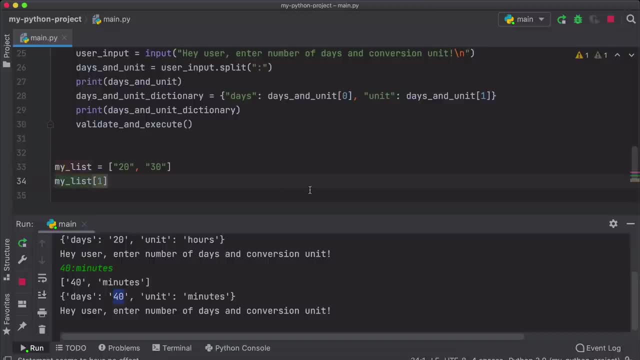 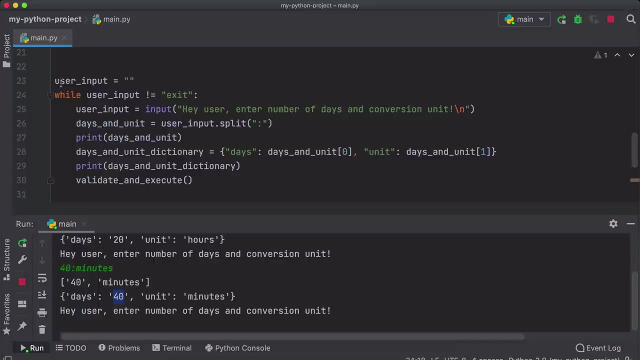 We can do that using an index, So this will basically print number 30 again. If we had other elements here, we can do index two, so that will print out 100.. And let's actually check that And remember to comment out a multi line code. 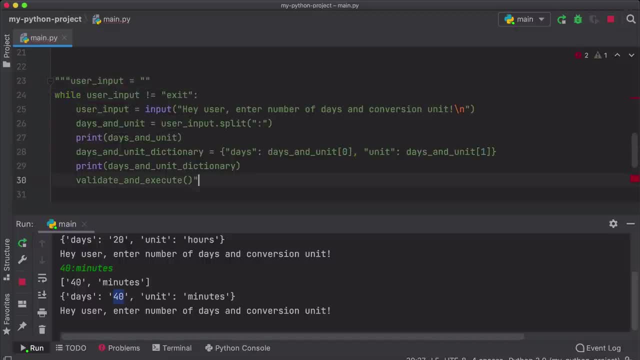 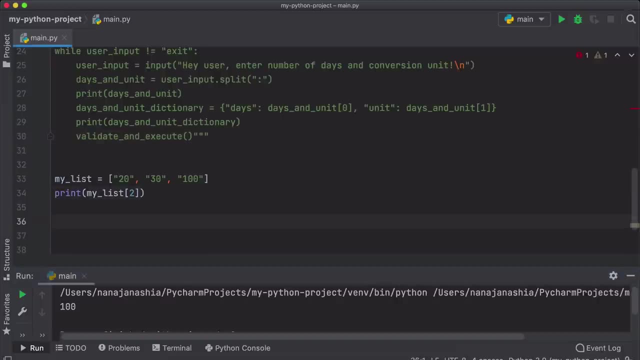 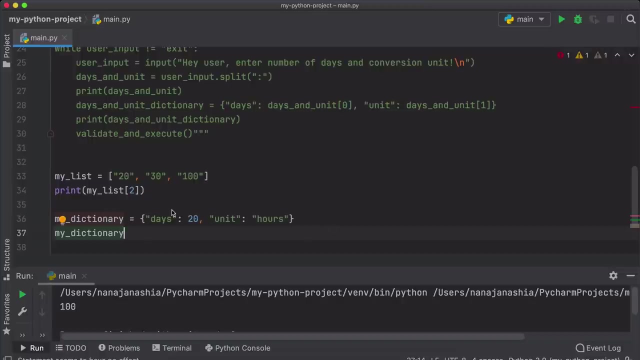 we can use three quotes: at the beginning and at the end. It's refresh and there you go. Hundred was printed. Let's do the same with the dictionary. So we have a dictionary. These Like this and to access an element inside the dictionary: 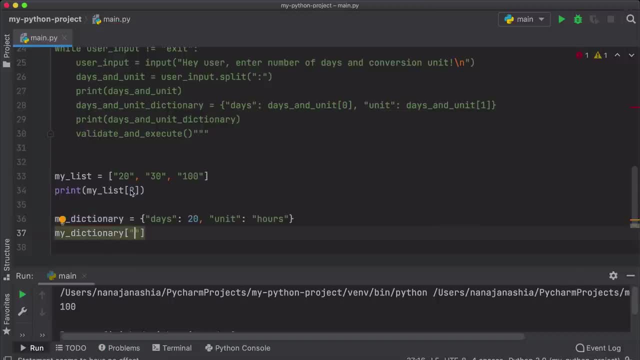 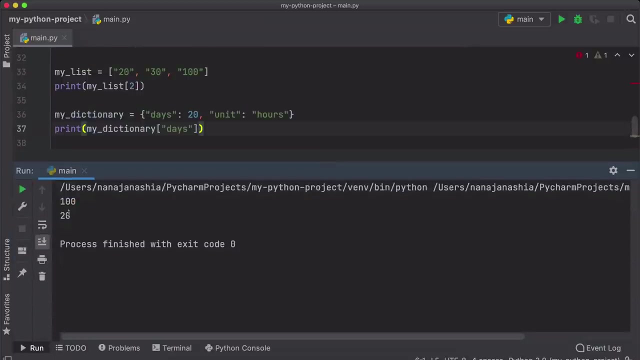 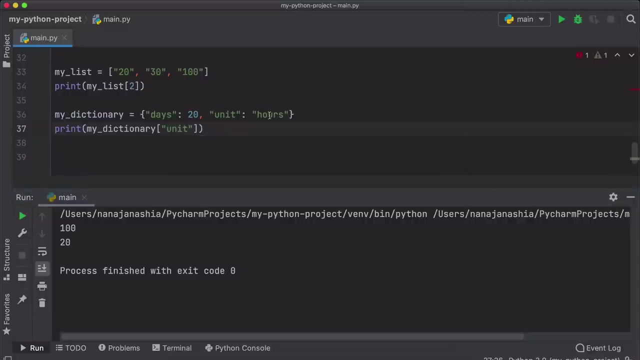 we use the square brackets and instead of the index, like here on the list, we use the key itself. And again, I'm going to print this. And There you go. you see value 20 and I can also access Unit value and, if I executed, I see ours, and so on. 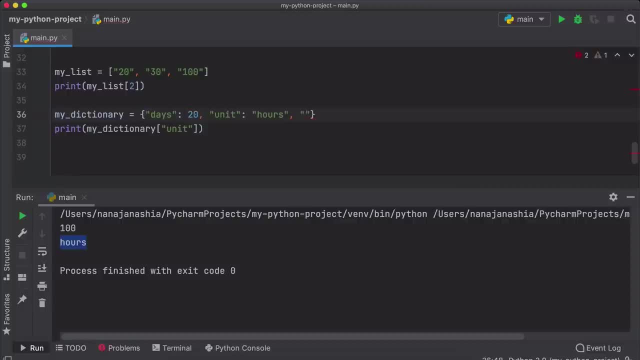 and I can add any number of key value pairs in my dictionary as I want. So, for example, I can add a message here: Good, And I can access that message like this: So this is how you create a dictionary and that's how you. 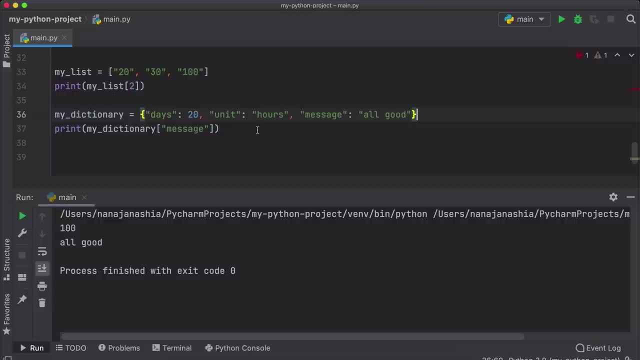 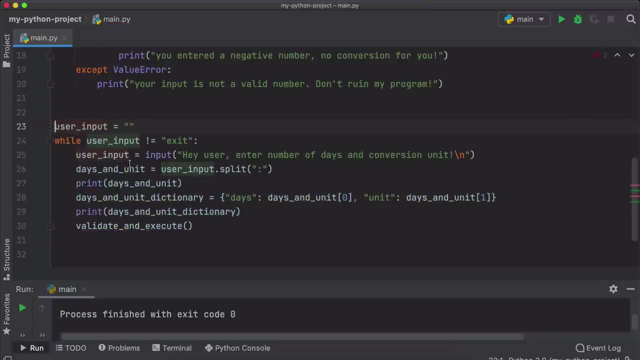 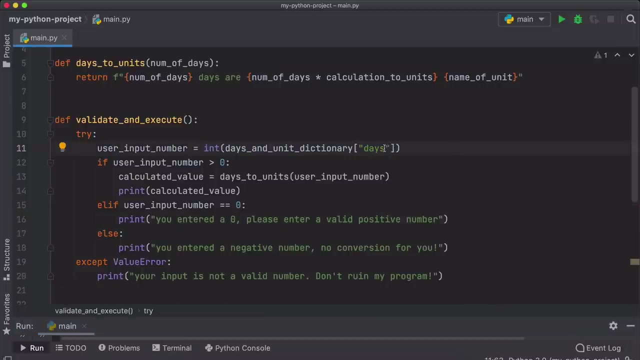 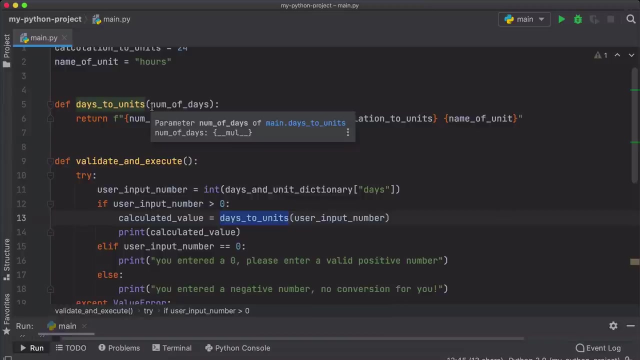 Access the values in a list or in a dictionary. So let's clean this up: Comment in our code again like this and Get back to our code. So basically, again, this is how we access the number of days in our dictionary and in our days to units function. 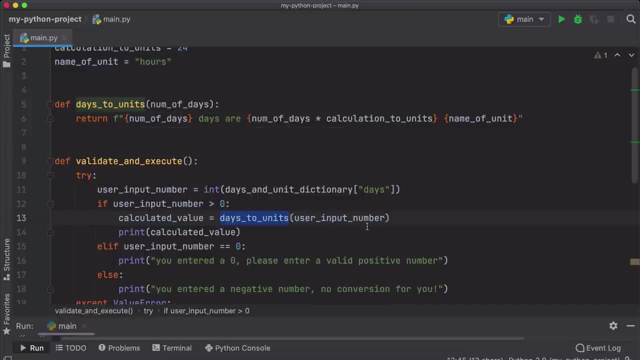 we need both of those values and we can Pass in those values separately. So we already have a user input number from the dictionary and the second value would be The unit From the dictionary. However, we have to add that second parameter to our function. 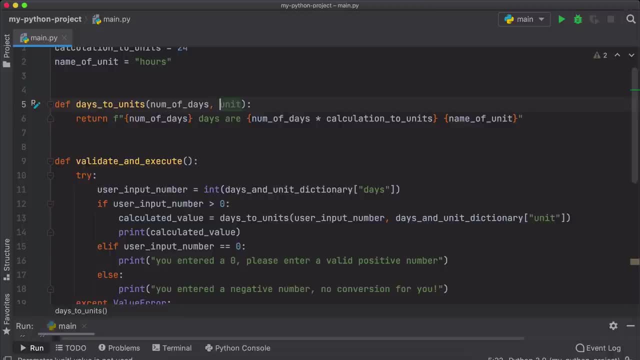 So let's do that Unit, Let's call it conversion Unit. So now we are passing Both of these values to our function. So we have the user input number here, which is already converted into an integer, and the second one. 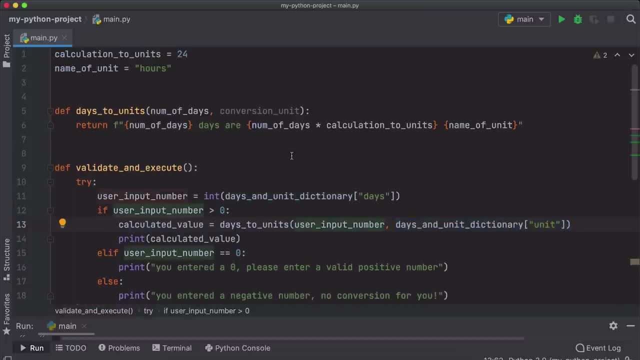 which is the conversion unit. And now we can finish the logic in this function here. Right now we are using this hard coded calculation to units, which is 24, and number of units, which is hard coded hours. So, first of all, 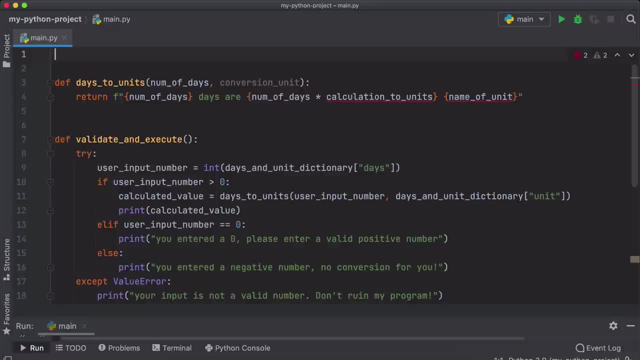 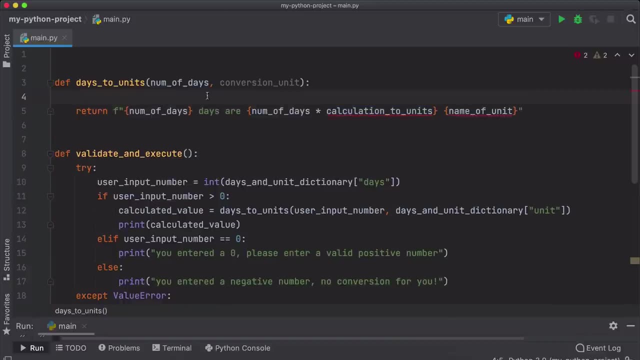 I'm going to remove those Two. We don't need them anymore because we get those values from the user And now we have to substitute those two. So here we're going to check if the conversion unit is hours Equals hours, Then we're going to return calculation with hours. 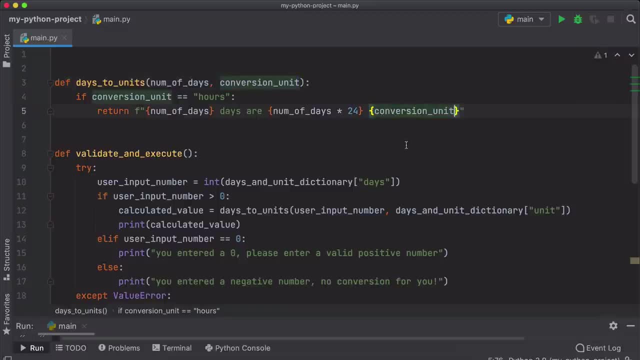 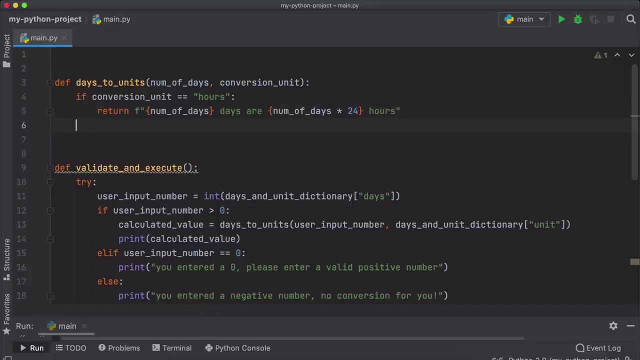 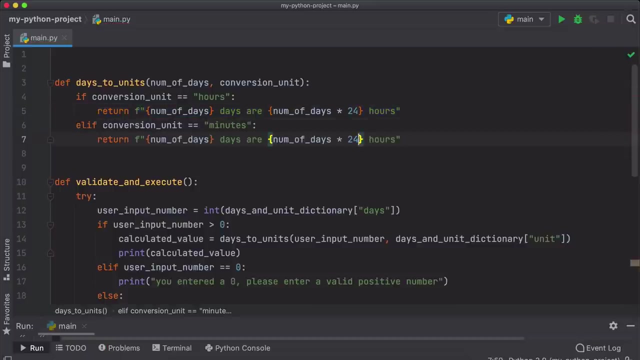 It's going to be 24 and conversion unit here. We can also hard code hours here, because we know it's hours Else if So, if the conversion unit is Minutes, Then we can return Calculation for minutes and a text like this: 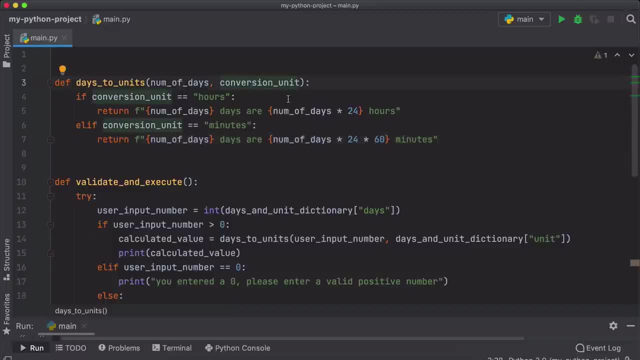 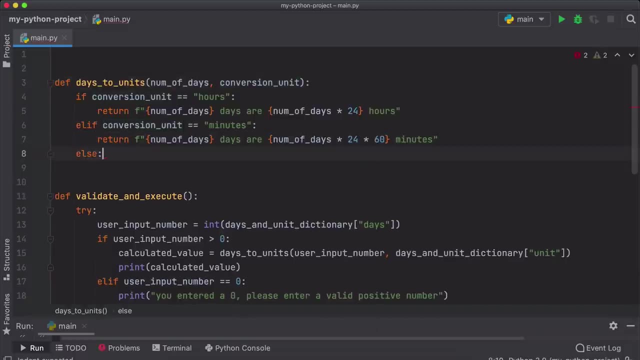 And it could also be that the conversion unit that was provided is not None of those, or maybe some invalid text, And in this case we're going to add final validation. So if it's neither hours nor minutes, then we're just going to say: 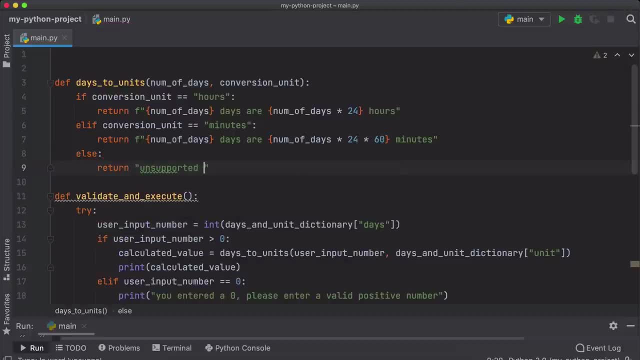 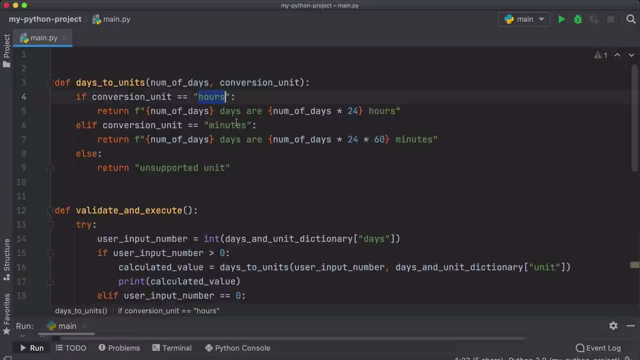 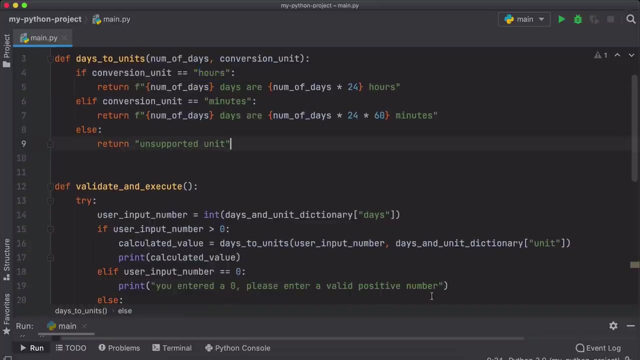 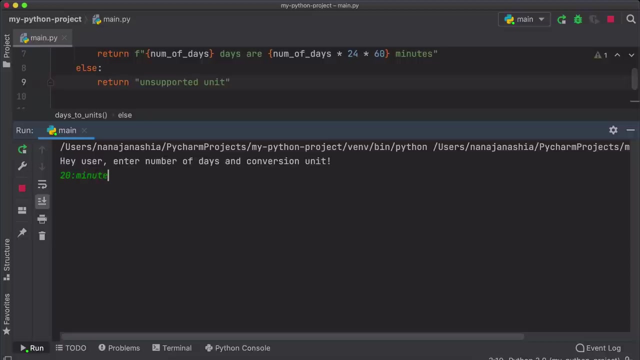 you know what? Unsupported Unit. So basically we don't do conversions other than those two. So we just tell the user that's an unsupported unit. And now if we execute our program and enter value, There you go, We have our output. and same way if we do. 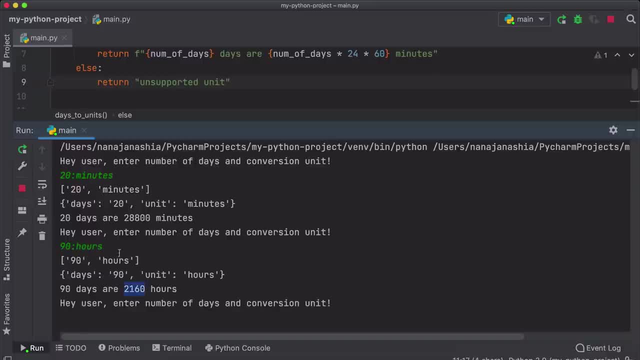 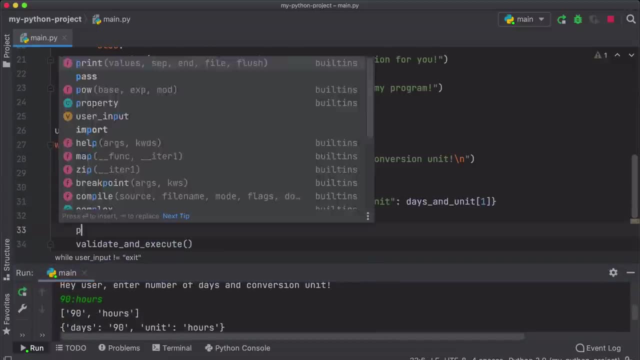 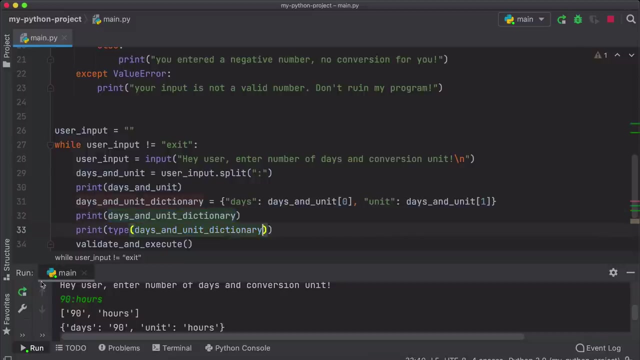 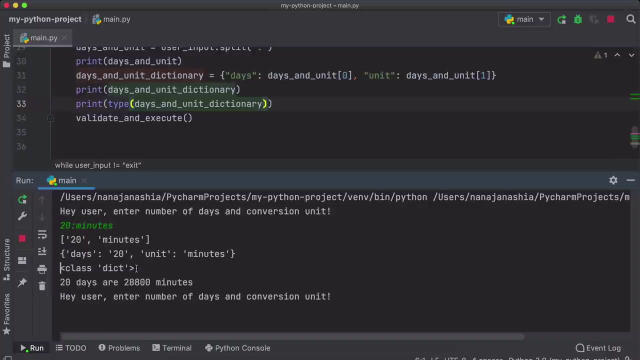 90 days to hours. We have our calculation in hours. So that's how dictionaries work. We can do one final thing here and, as usual, print out The type Of our dictionary. And there you go, You see class of type dictionary here. 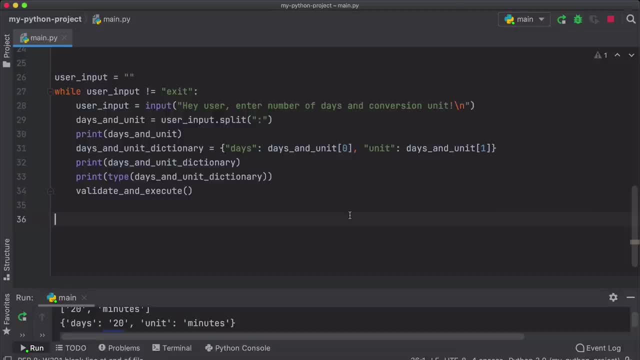 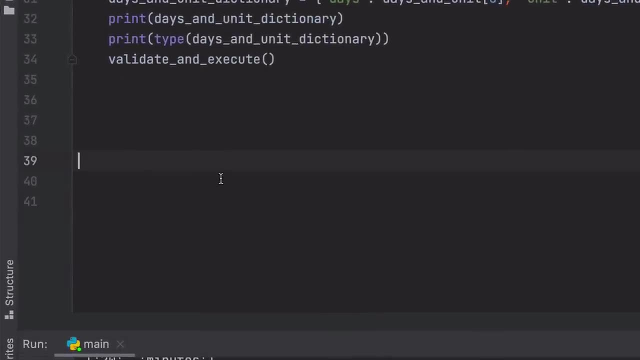 which is another data type, And at this point we can actually summarize all the data types that we have learned so far. So let's give us some space here. So first one was string, So basically a message or Some output Like this: 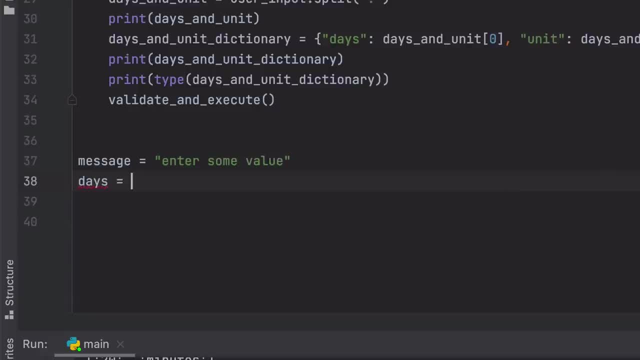 That's our string. Then we have integers. example of that We saw already days. Then we have float numbers which, for example, can be used for price Or weight of a product, Etc. We also have learned Boolean data types When we check some kind of condition, whether if it's true or not. 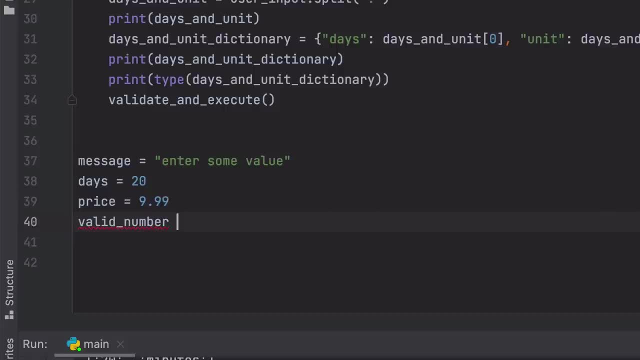 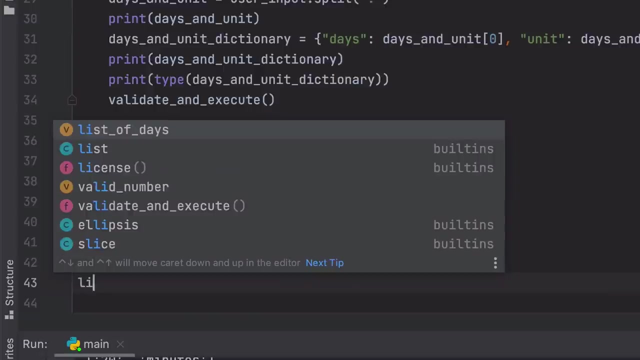 So, for example, is it a valid number Or is the user input exit? We also learned a data type of lists, So, for example, usage list of days Like this, including duplicate values and list data type can be used for strings as well. 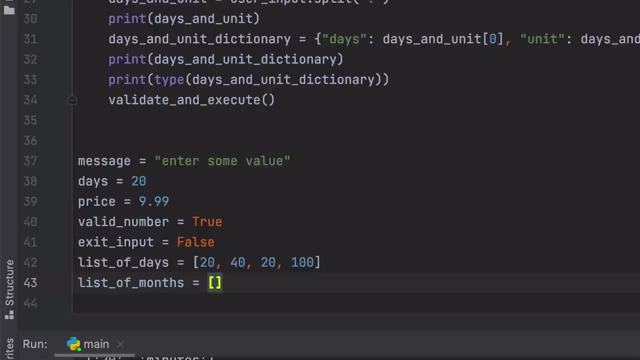 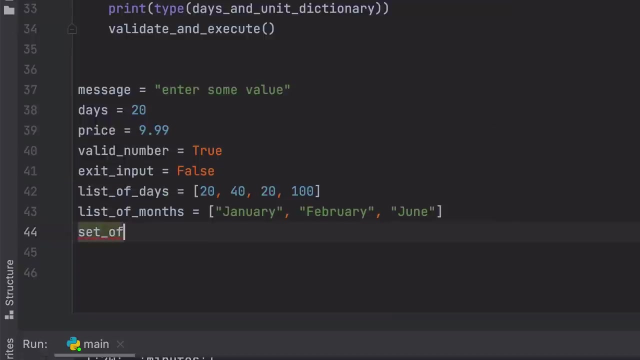 Not only for numbers. So, for example, we can have list of month Like January Really matter. We also learned a data type called set, and set basically is very similar To list, but it doesn't allow duplicate values and its syntax is with curly braces. 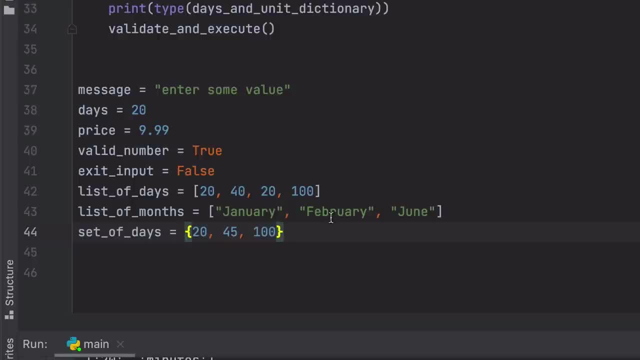 So the same way, we can have numbers or strings or Booleans or any other data types inside a set. And the last one that we learned was a dictionary, And let's take our own example: day in unit, And dictionary is basically a collection of key value pairs and the syntax is written like this: 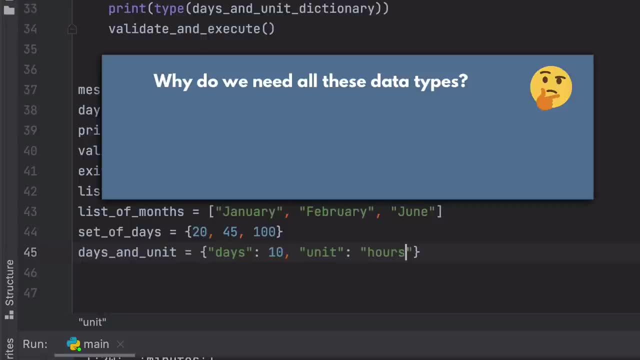 So why do we need all these different data types? Well, depending on the use case or what exactly you are trying to achieve in the program, you're going to need a different data type to achieve exactly that. So each data type has its own specific purpose. 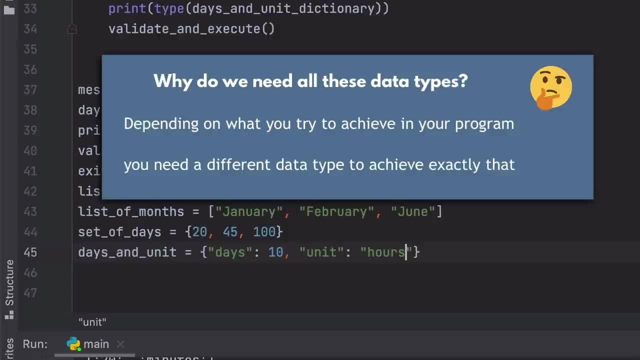 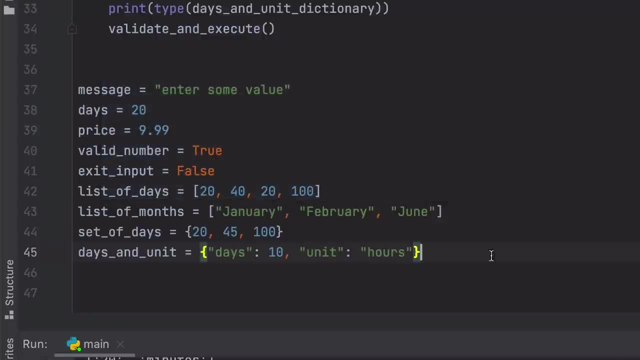 And throughout these days to units calculator. I try to demonstrate the purpose of each data type and when we need to use them. So these are all the data types that we learned. These are also most of the data types available in Python and the main ones that you're going to be working with. 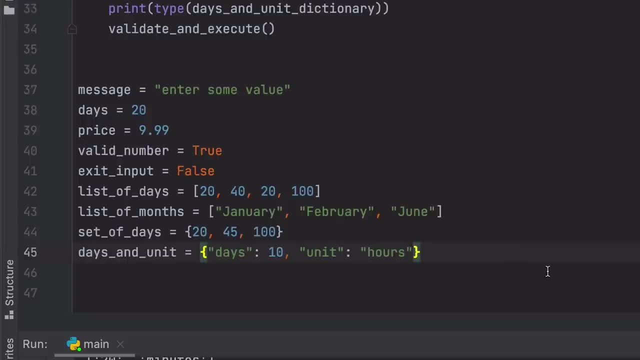 So this should give you a good foundational knowledge about data types in Python and also note that most of these data types you will also encounter in any other programming languages because, as I said, these are the core data types and most of the programming languages actually support these data types as well. 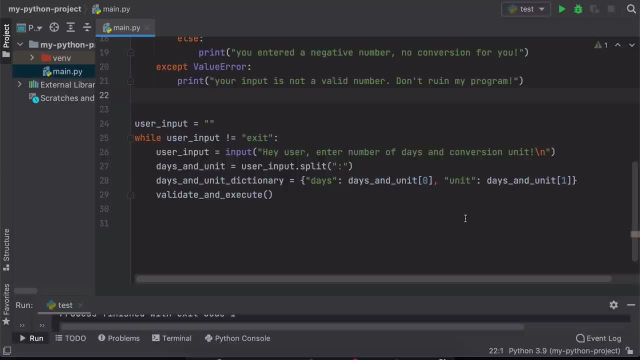 Till now, we have been writing all our code in one single file. So basically, we have a project with just one Python file and we're writing all the logic inside that file. However, you can imagine that if you're writing a little bit more complex applications that have much more complex logic. 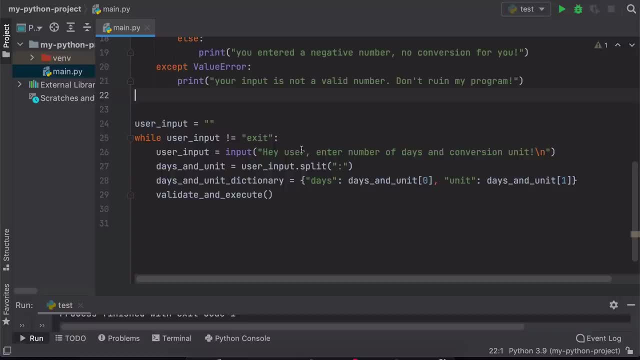 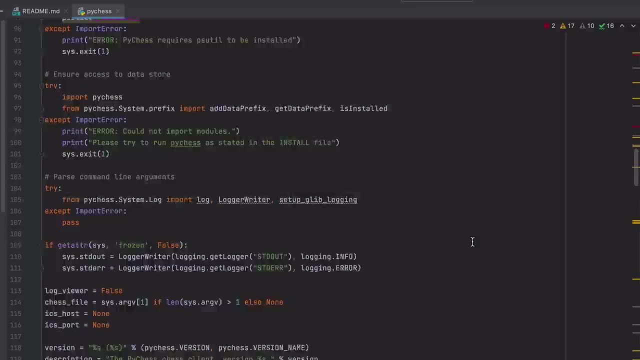 so they end up having lots of functions. Obviously, you're going to end up with a Python file that has hundreds of lines of code, maybe thousands of lines of code, And it's not very practical to manage all this logic and all this code in just one file. 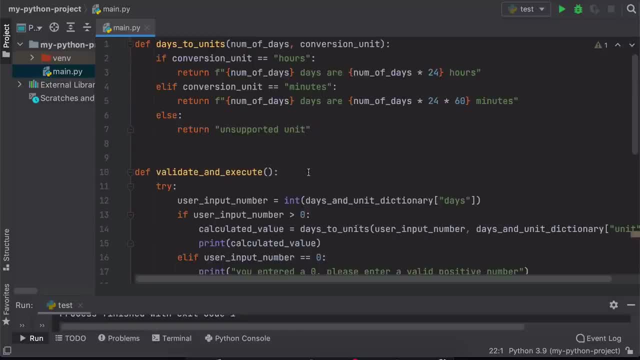 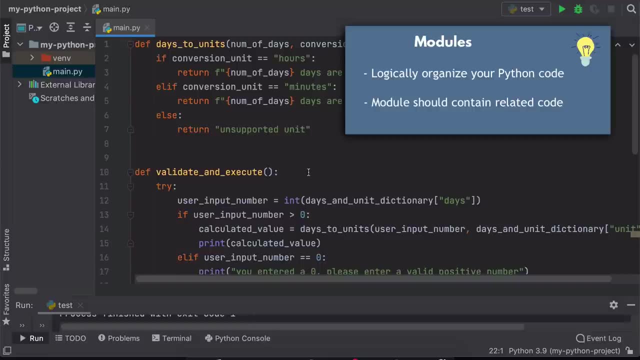 So instead you need to structure your code and divide Your logic between multiple different Python files, and you do that with modules. to give an example, Imagine a web application that has basically many features, like Facebook, for example. Obviously, you can put all the Facebook logic in one single Python file. 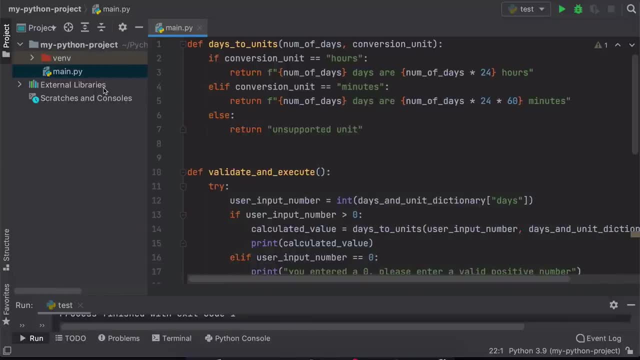 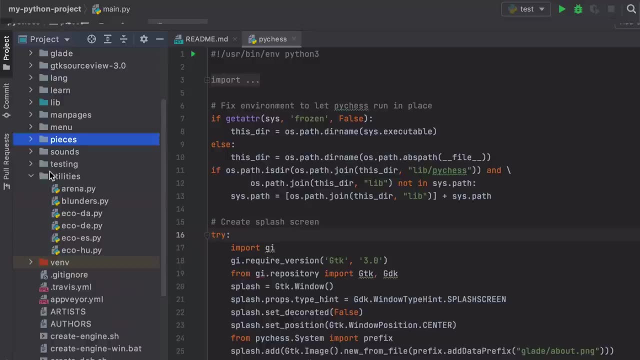 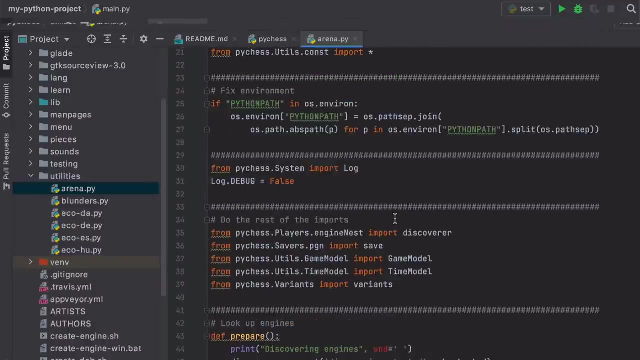 right, You will have a structure of Facebook project with sub folders in your project which all contain multiple Python files, So you would have, maybe, packages for each feature, and each such feature has a lot of functionalities, So they will be all grouped then again in multiple Python files. 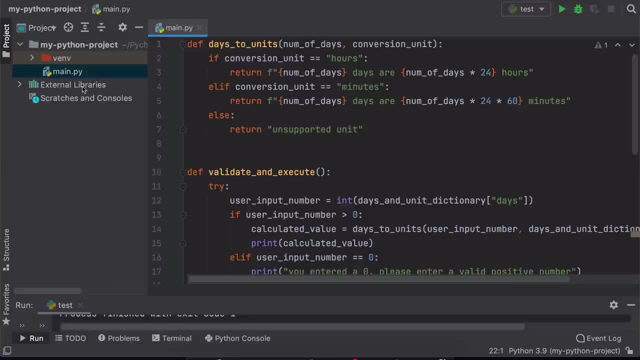 right. So you would end up with a project with a hierarchy of folders and lots of, lots of Python files inside. Now the question is: if I have multiple Python files in my project, how do I connect them together? So, for example, 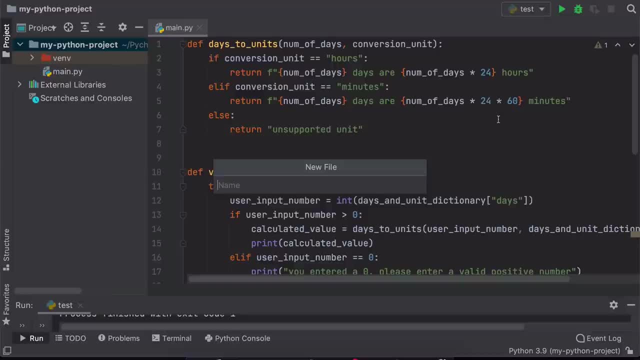 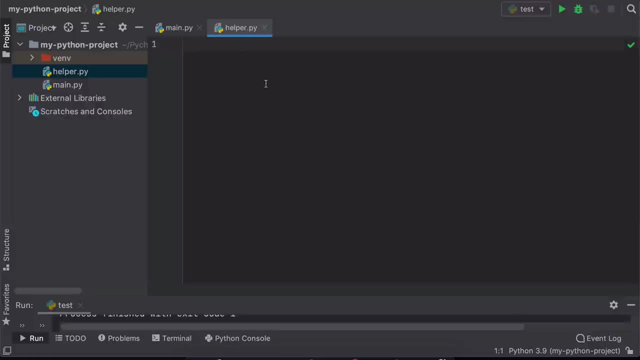 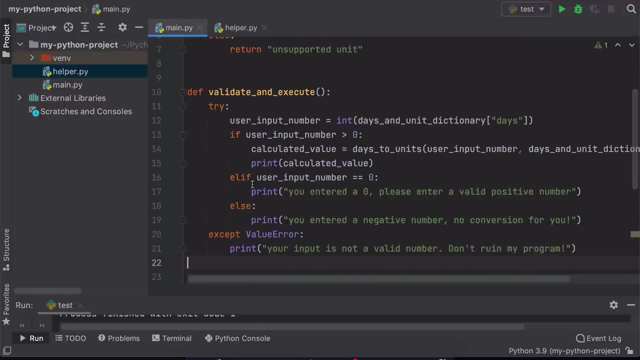 if I have, I have another file here and let's call it helper dot P Y, And if I have some logic here, basically functions defined here, how do I use them Or how do I reference them in another file? And the way it works in Python is using the concept called modules. 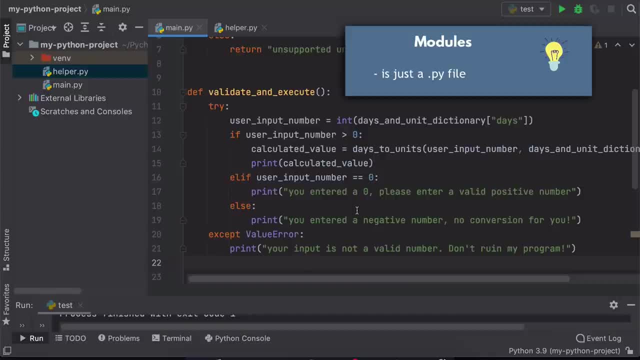 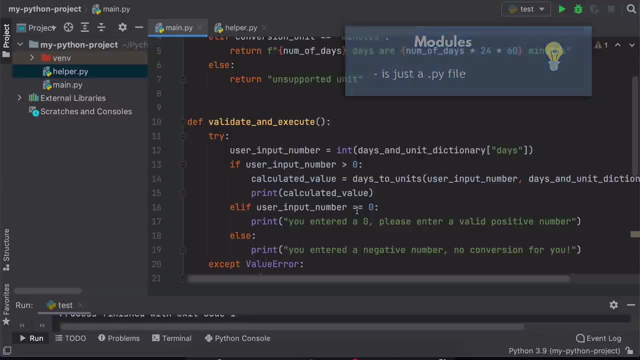 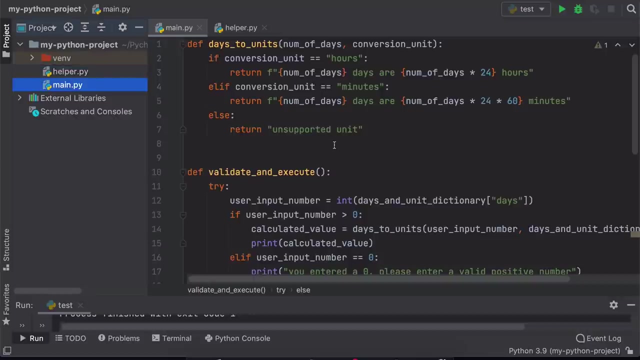 So a module is basically a Python file that contains functions or variables that you can use in another Python file, So basically any Python file that you have in your project. both of these in this case are modules, and you can reference one module from another. 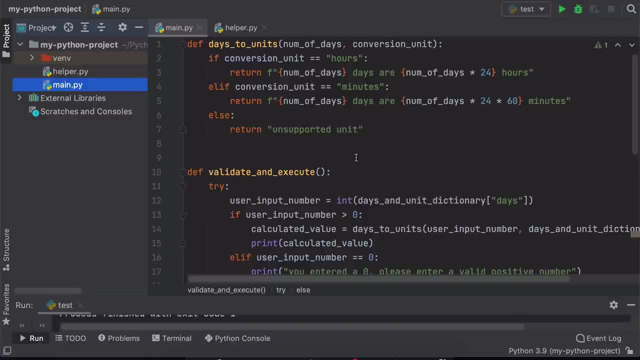 So basically the idea is that you can structure your application, your program, using modules so you can make your project modular. So in this part we're going to create our own module in helper File and we're going to reference that in main dot Python. 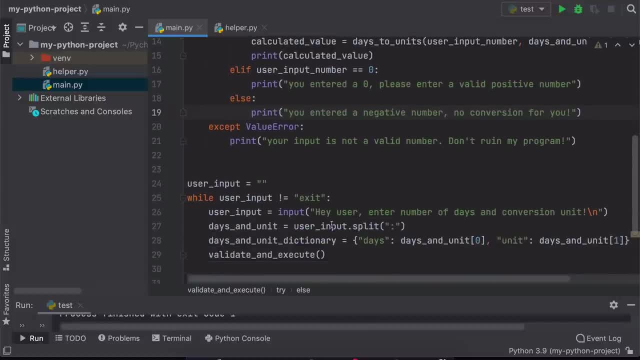 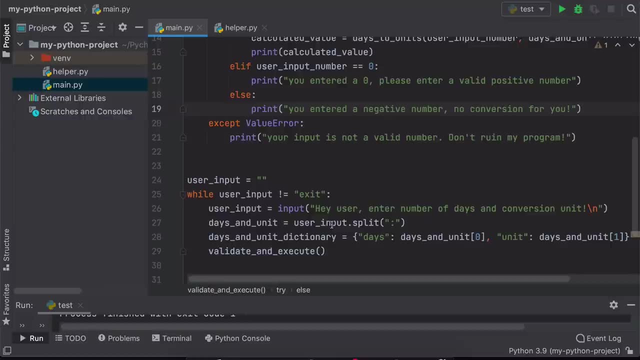 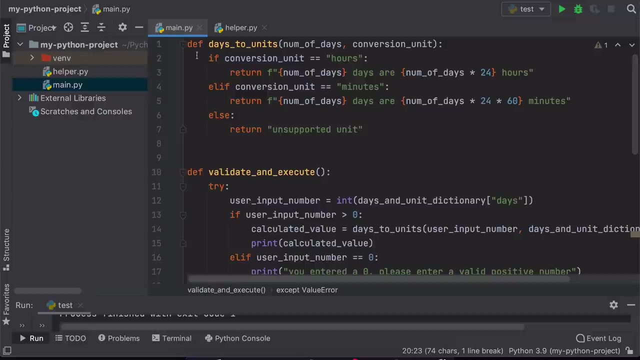 And let's say, in mainland Python I only want the code that basically starts the program right, All the functions, all the logic. I kind of want it hidden away and group together in a separate file. So what we're going to do is copy this entire thing. 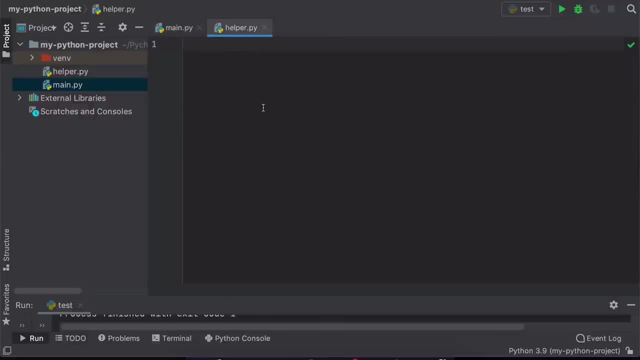 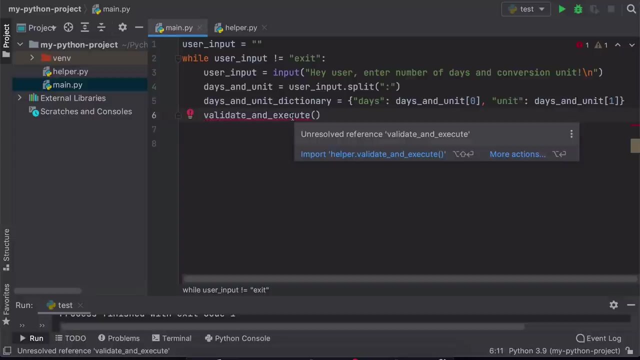 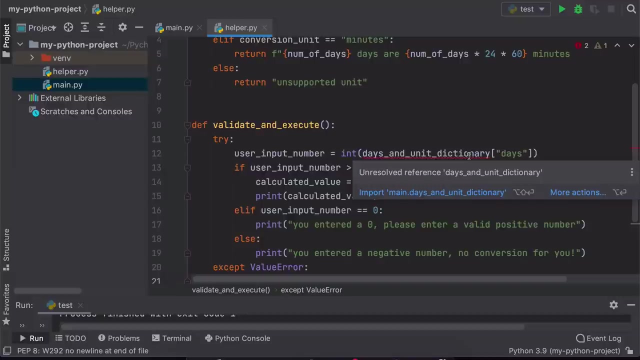 So both of these functions basically and paste it in here. So now you already see a couple of red lines here, because now the reference is obviously broken, right? So main dot Python obviously doesn't know anything about validate and execute function, right, It says unresolved reference and the same way days to unit dictionary is unresolved for helper. 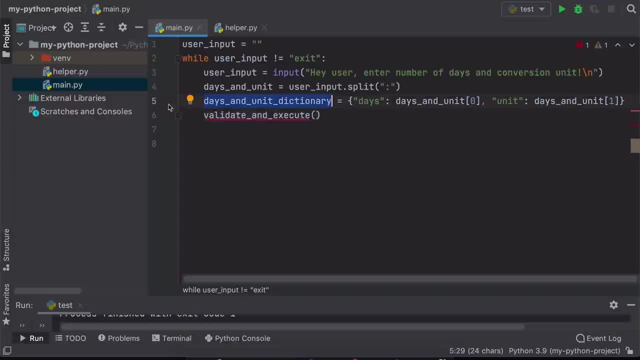 because it doesn't know anything about main dot Python and the variables defined right here. So the first thing we need to do is we need to Tell main dot Python file where to find this validate and execute function. right, We have defined it in helper Python. 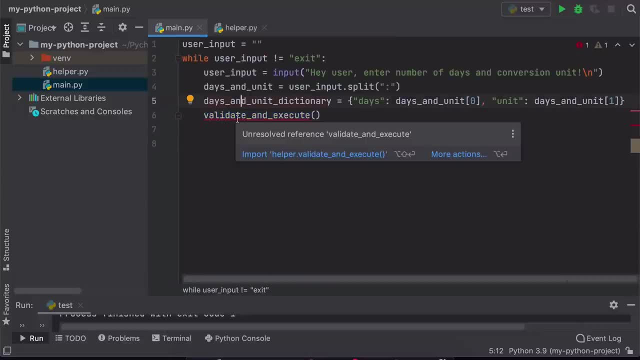 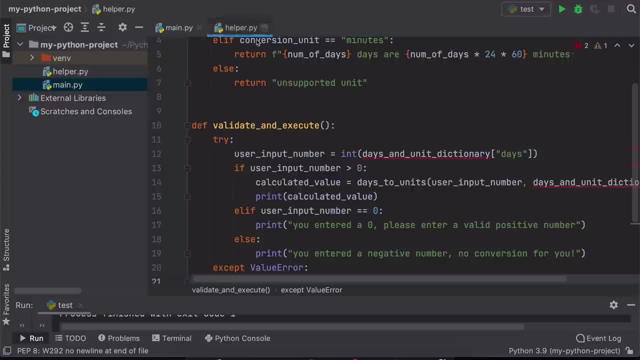 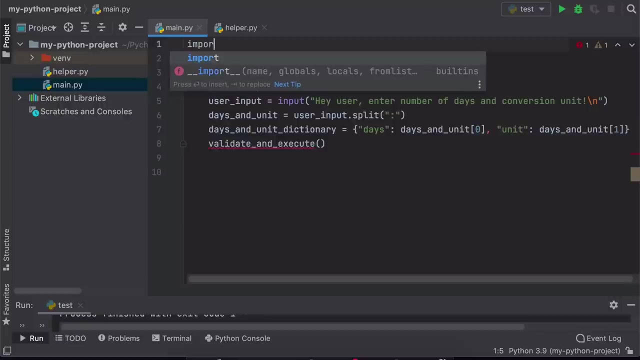 So that's what we need to define. How we do that is using something called an import statement. So basically, import this whole helper dot pi module inside main dot Python and we do that very simply using an import helper. right Helper is the name of the file and therefore name of the module. and right now, 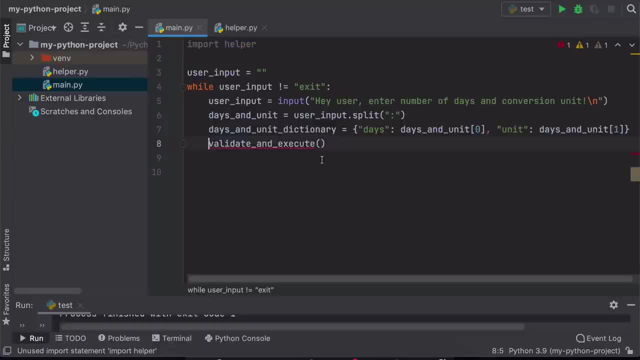 it's great because we're not using it And the way to use it is helper dot and the function name, and you see the red line disappeared. So again, what we did is we told main dot Python There is a helper module in this project and please import this whole module and all the functions that this 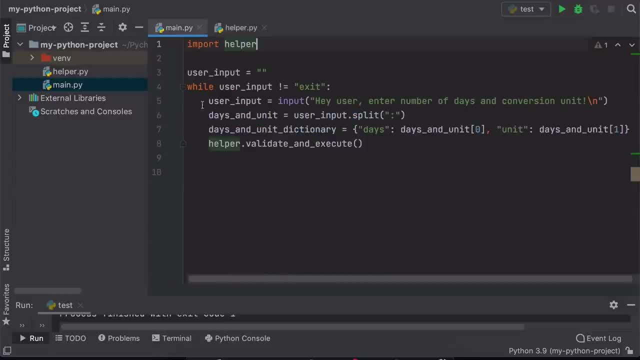 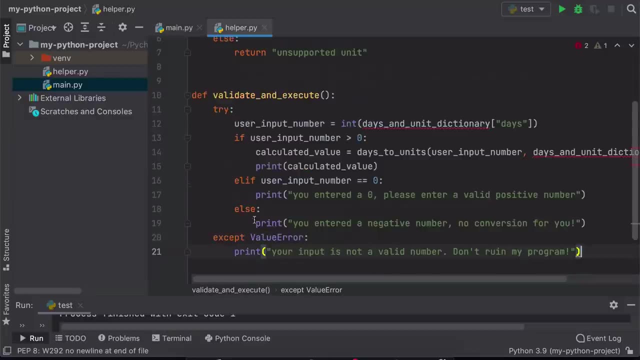 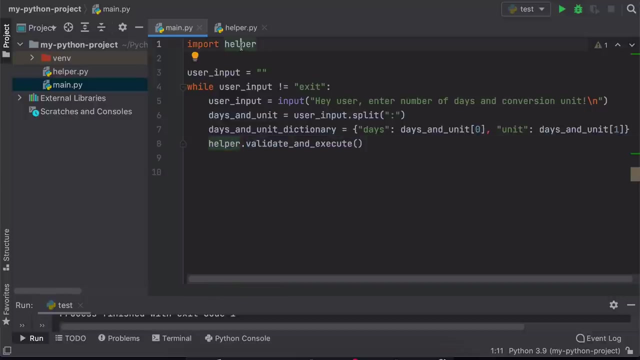 module has and make it available in main dot pi. And then once we have that helper module, we can reference any functions if we had any variables using module name dot function. So this has to be the name And if I hover over it, 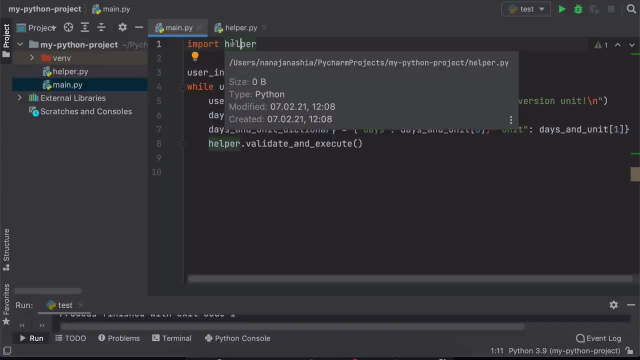 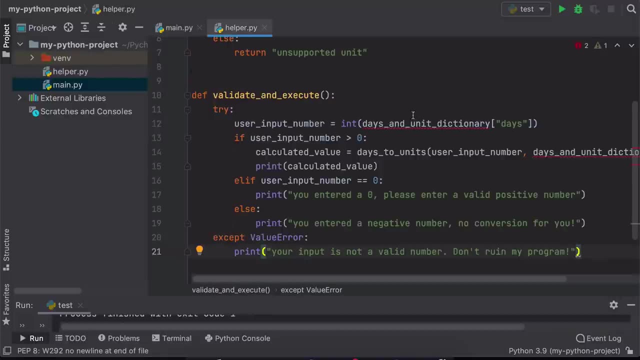 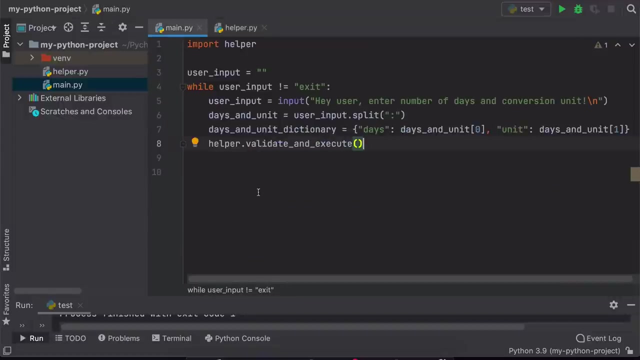 you see that pi charm actually displays the whole path to that helper dot pi file. And now know that here we still have red line, because this is a variable which is defined in main dot pi, but a helper module doesn't know anything about it. 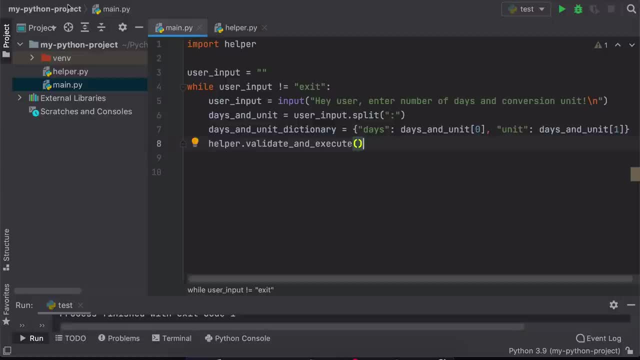 And that's an important distinction here, because we imported helper module inside main, So helper modules functions are available here, but not the other way. So in order to make this dictionary available in validate and execute function, we would need to pass it in as a. 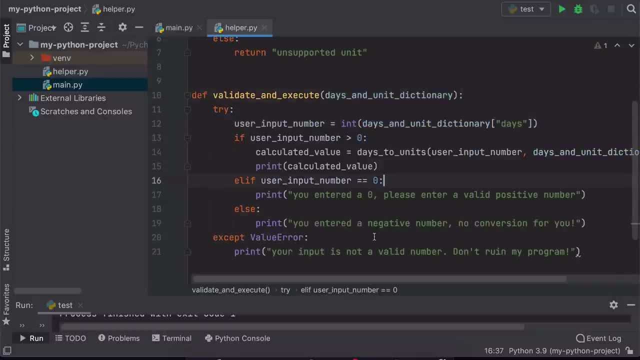 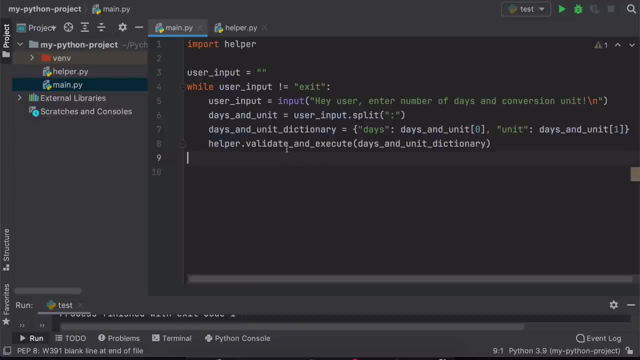 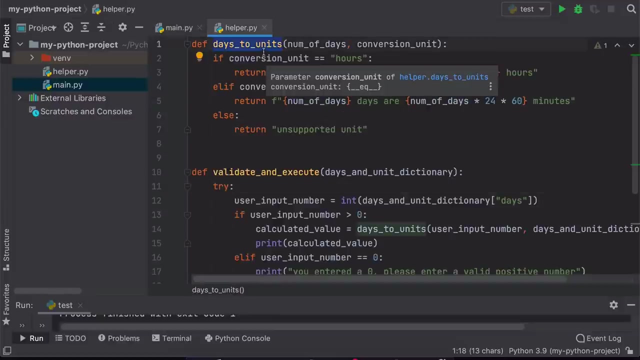 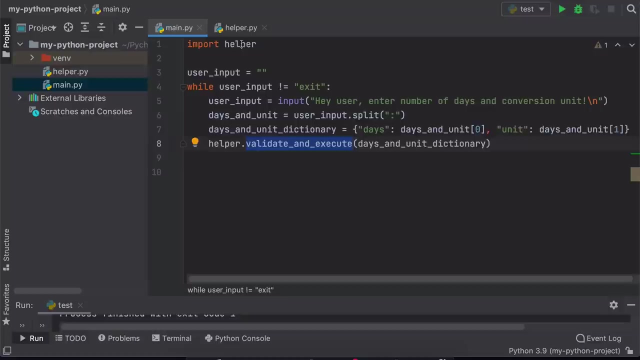 a variable like this, and this will work now. Now note that in main dot python we actually only need this validate and execute function. We don't need the days to units function, because this function is only used by validate and execute function. So that means that we don't need to import the whole entire module inside main dot pi. 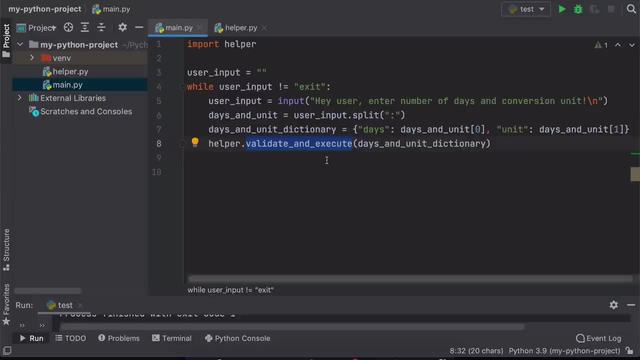 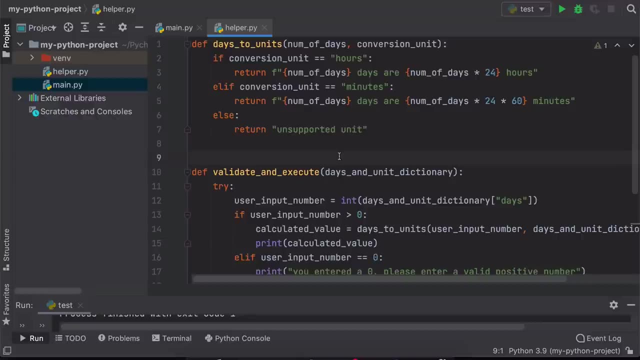 We actually only need the validate execute function, And this is a small example. but if you had a module with 2030 functions and you just needed one of them, you wouldn't need to import the whole module just for that one function. So what you could do is you can pick and choose which specific functions you want to make available inside another file or another module. 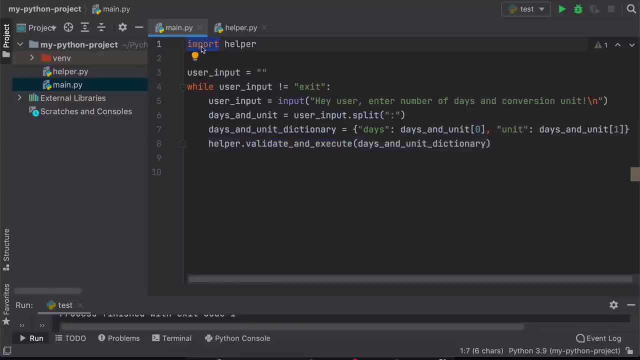 And you can do that very easily using the following syntax. We say from helper: that's the module, again import and the name of the function. like this: And now, because we are accessing and importing that specific function, we don't need to use module name anymore. 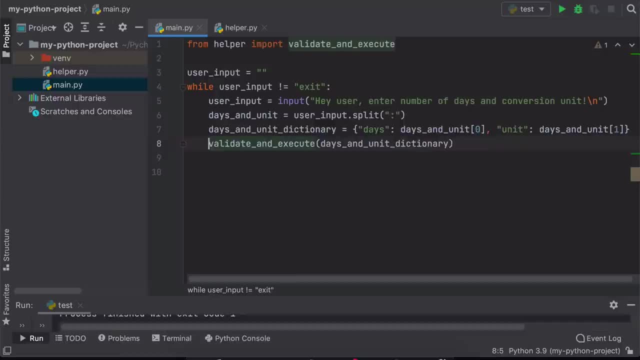 We have that function available directly, so we can delete the module reference here And we have that function Available like this. So again, instead of having entire helper module with all of its functions and other stuff, we only have one specific function available here. 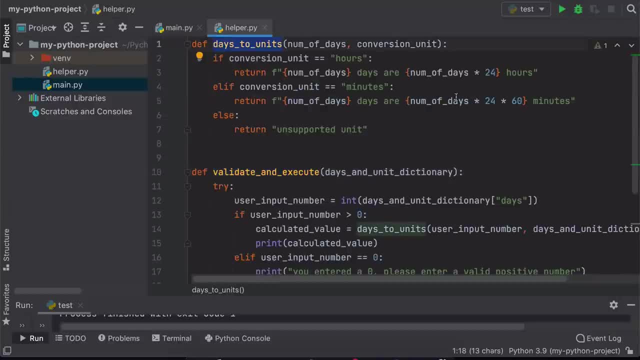 So that means we wouldn't be able to use these two units, for example. Now we saw an example of a module that has just functions right. However, module can have many other stuff, for example variables, and you can make those variables also available. 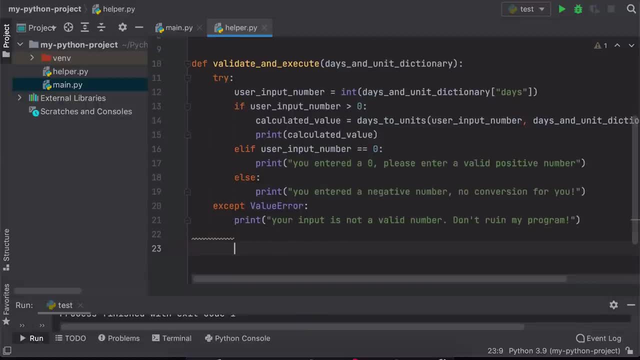 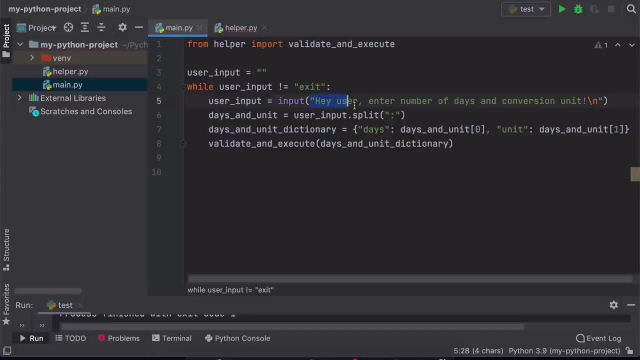 For another program, And that's an example. here I'm going to create a variable called user input message, And this is our user input message, and we can actually put it into a variable instead of having it defined like that. So I'm going to copy it and paste it here. 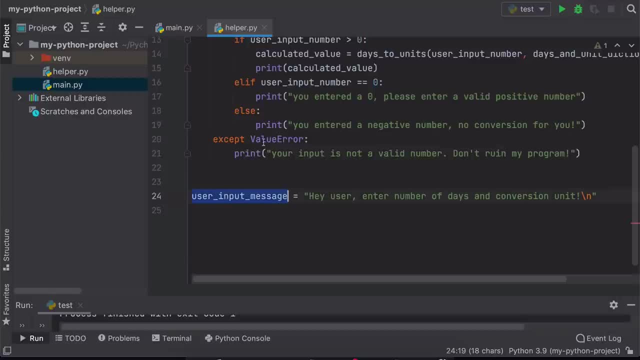 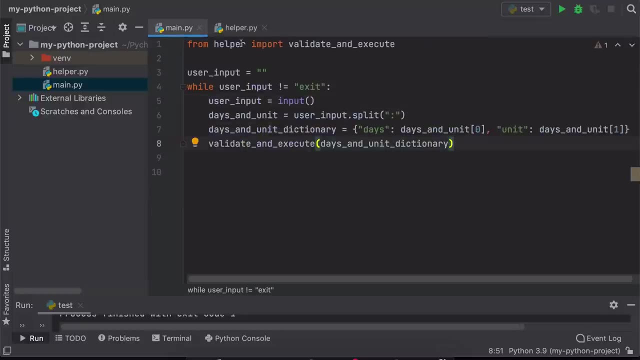 So now we have the user input in a variable in another file. Again, how do we access it? in main dot pi, in this statement at the top, We can actually import several things from a module. right now We are importing a function, We can also import our variable, and we can do that also very easily like this: 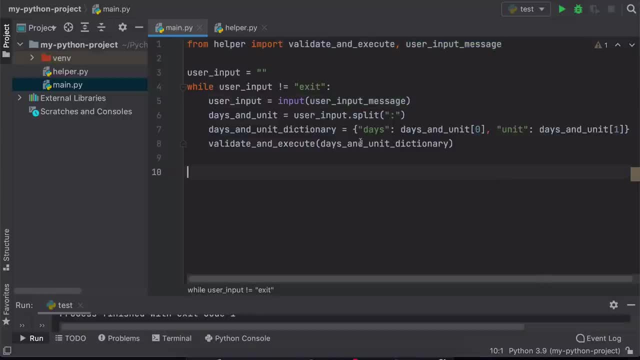 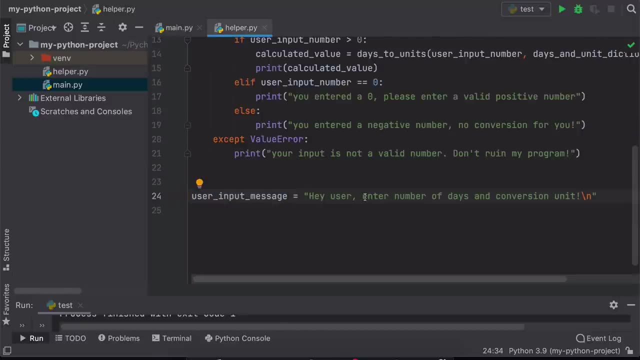 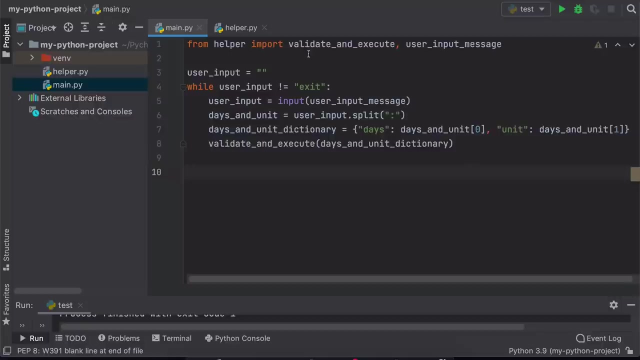 And we can use that user input message Here. So basically, if you have again 20 functions and variables from the module and you just need maybe five of them, you can import them individually. like this: Just basically just list the names of functions and variables. 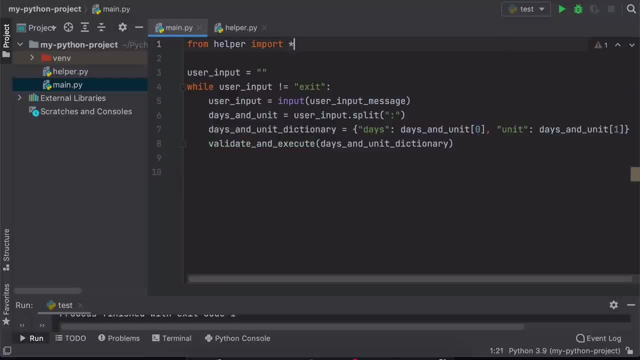 What you can also do is import all. This is what this asterisk sign represents, So we're basically importing everything from the health Her module. again, this is kind of a waste if you just need a couple of functions and variables from that module and not the entire thing. 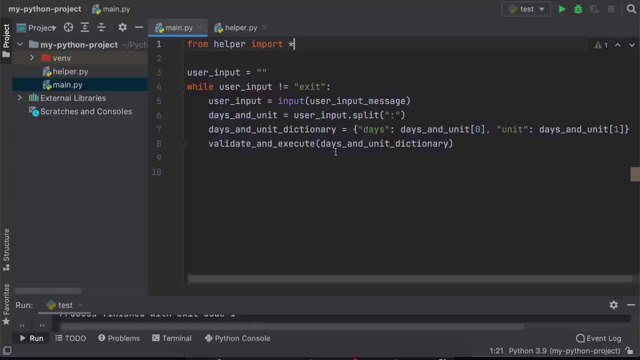 However, with this syntax you can import everything. And now you may be wondering: what is the difference between importing everything from the module and importing the whole module? because in both cases you have everything in the module available. The difference is in the syntax. 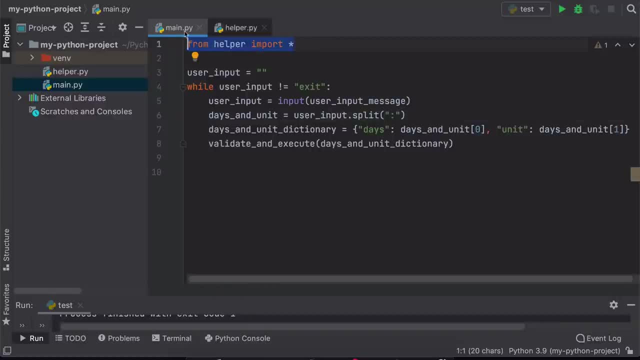 because note that if we use this from import statement, you don't need to use name of the module every time you're accessing something defined in that module, right? So we don't need to do helper dot function name or helper dot variable name. 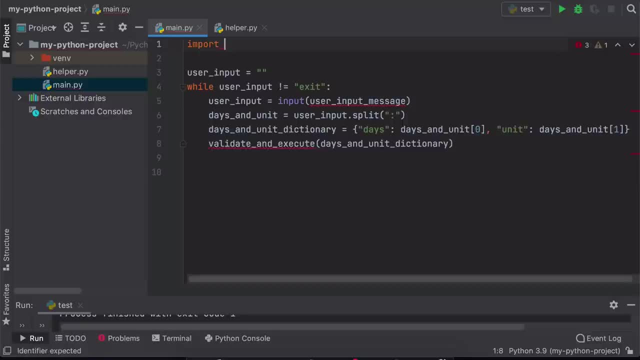 Whereas if we imported the module like this, you see we have red lines because we would need to do helper dot or module name dot whenever we use something from the module. Now, this could be a matter of taste. So, basically, which one you want to use? 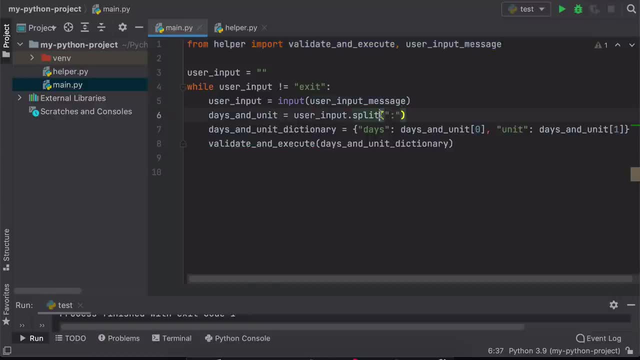 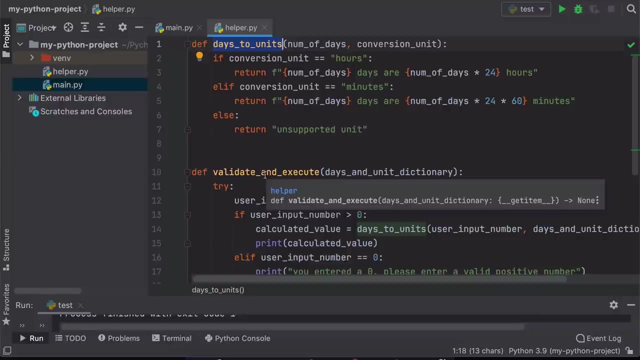 I personally think that this is the most efficient and also cleaner way of using specific functions, variables, et cetera defined in a module. And, as a side note, the things that are defined in a module that you can use basically in another file are called definitions. 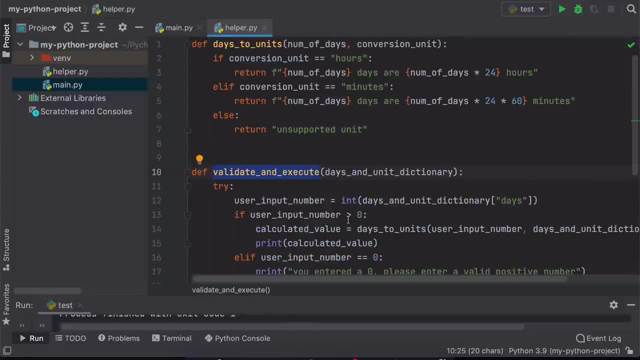 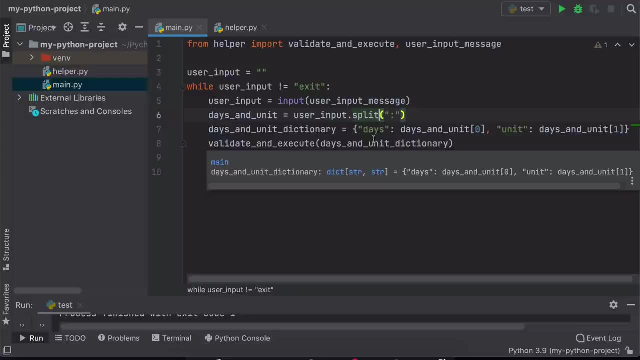 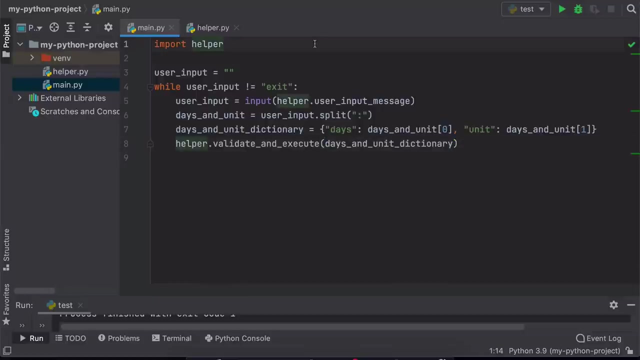 So all of these, those three elements here, are definitions of a module and you can use any of those definitions in a file where you import that module. What you can also do when importing a module is you can rename that module basically to whatever you want. 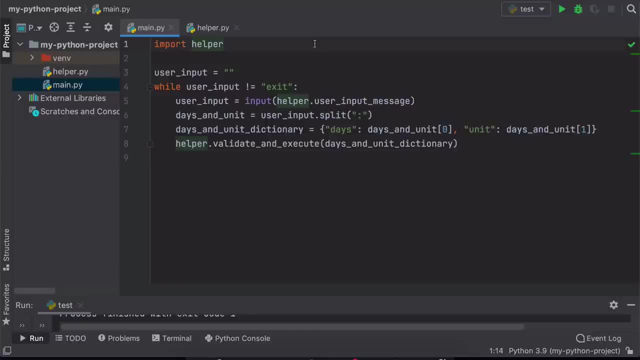 So if the name of the module is too long or you just want to use a different name, you can do as and then basically write a name whatever you want, like each, for example, and then obviously you need to use that New name everywhere. 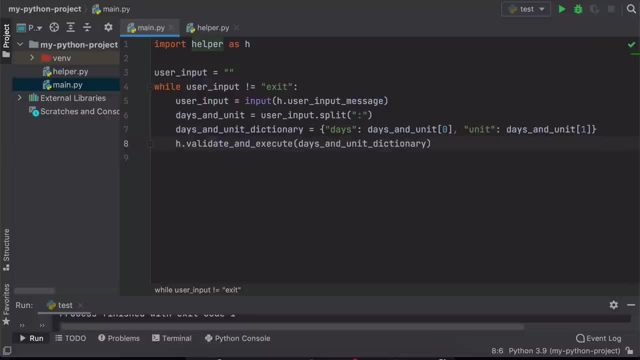 you access functions or variables of that module. So basically, how you import a module and whether you rename it is a matter of taste, basically how you want to do that in your code. However, I think that importing specific elements from a module like this is most efficient and also cleanest way to do that. 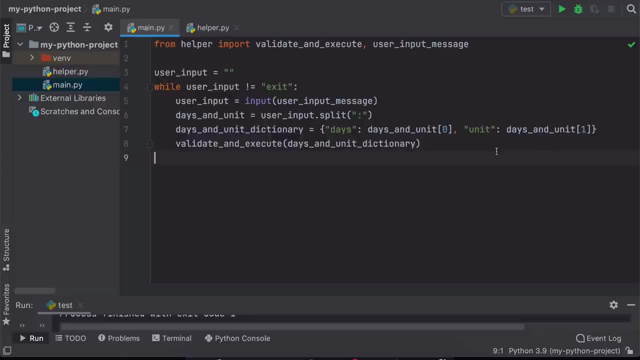 So we saw how to create our own module and use it in another file. So, basically, if you had 100 Python files here, with each one of them having their own functions and variables, you can cross reference them from each other using the import statement very easily. 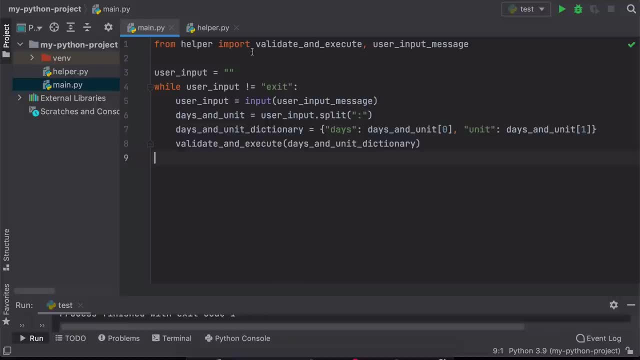 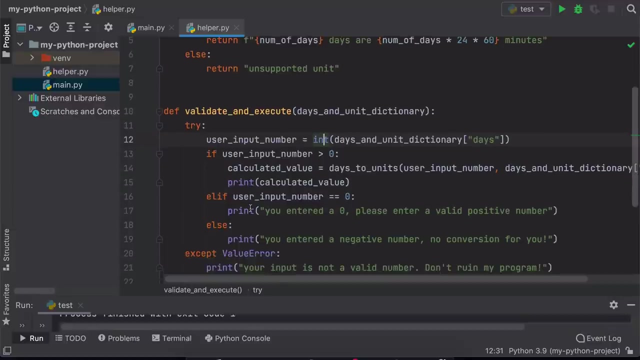 Now, in addition to creating your own modules, we can actually use modules that Python itself already includes. So, just like we use some functions that Python gives us out of the box, like inputs or ends, So basically all of those the same way. 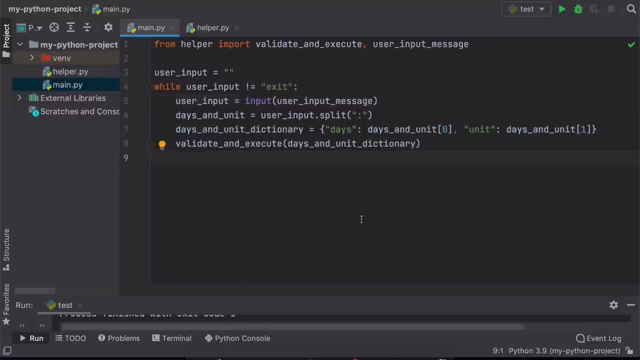 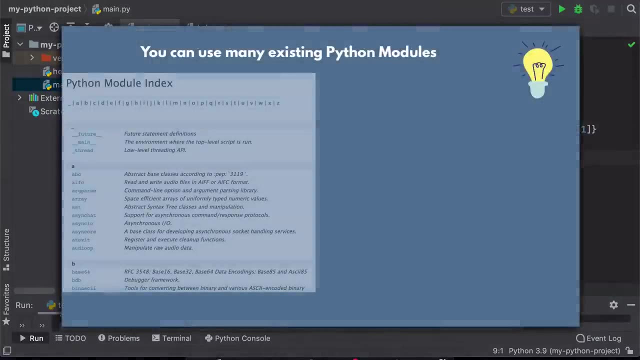 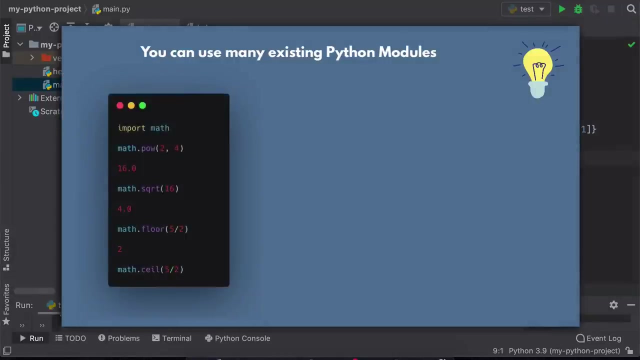 Python also gives us modules for different scenarios so that we don't have to write this logic ourselves, And there are a lot of useful modules that Python actually includes, for example, math module for mathematical operations, its own module for working with dates or date times, module for working with specific files, and so on. 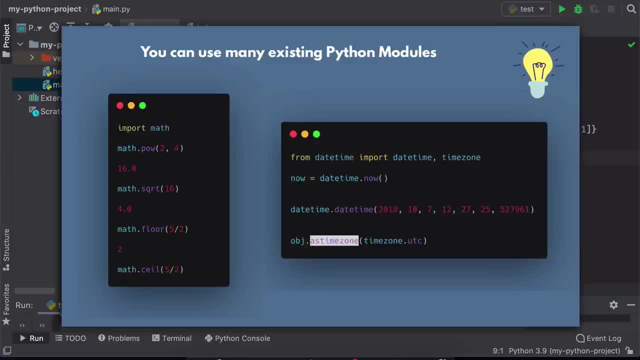 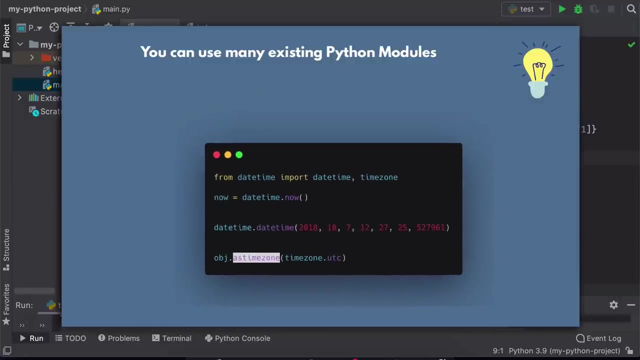 So, basically, for many different use cases, Python already gives you ready modules and these modules will then contain multiple functions and variables for that specific use case. Again, if we take an example of a date, so if you have an application that works with dates and times, 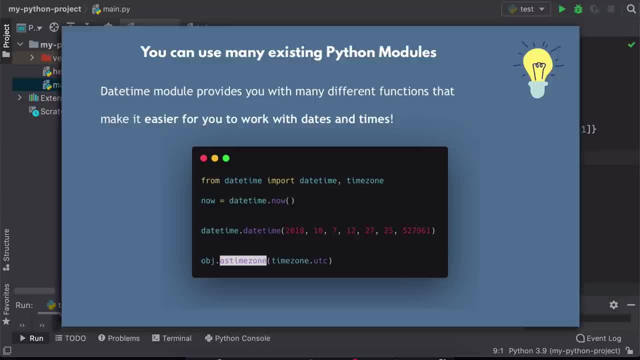 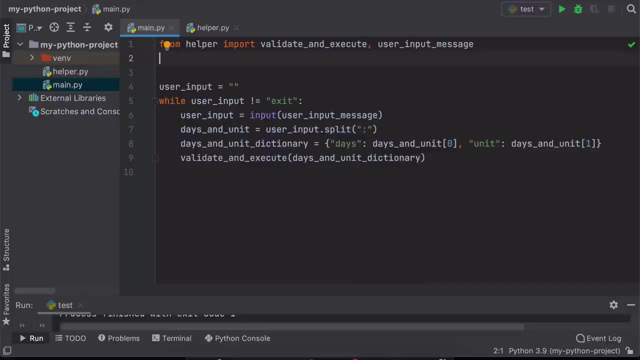 you have this module from a Python that gives you a bunch of useful functions for working with dates, And again, this means you don't have to write this logic yourself, but rather use the existing one. So to give you some examples of modules that Python provides us with, 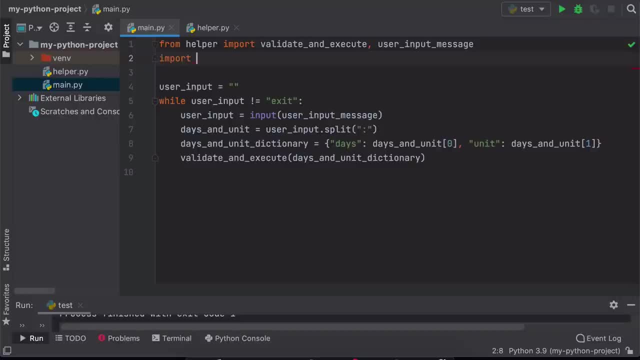 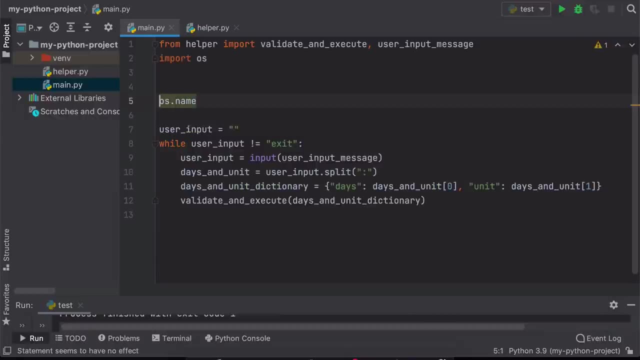 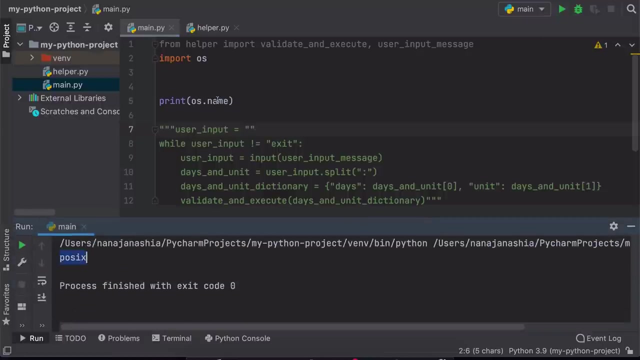 for example, if you want to work with the operating system, there is an OS module so we can print out, you can get the name of the OS, for example- and I'm going to comment all this out and run and you see the name of the OS and other useful module. 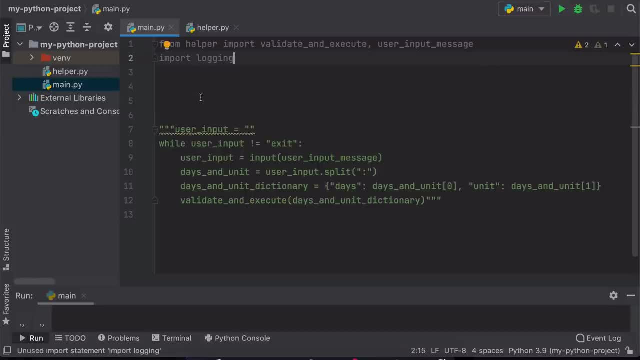 Python offers is logging. So if you want to use logging in your application, the logging module gives you different functions to log an error message or warning, et cetera, as well as basically just configure how the log. it will look like again to see an example: 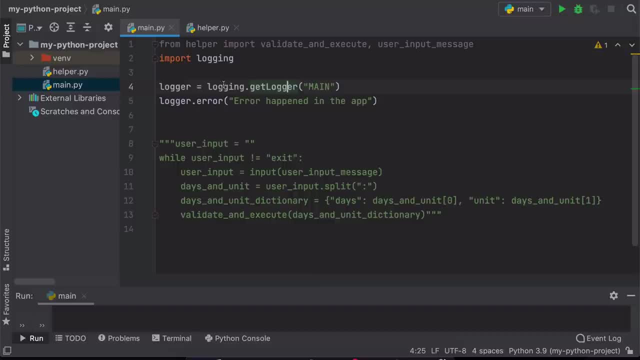 Again, it may look a little bit complex here, but essentially just using the name of the module and then functions that it gives you. Obviously you need to know the functions and you need to know how to use them, and you can get that information from documentation. 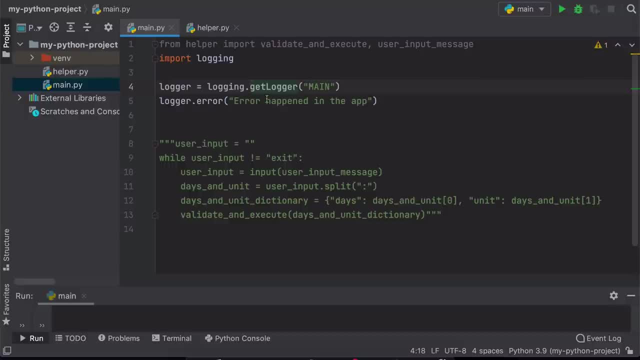 Or if you're using PyCharm, it actually gives you all the information about this function And the module if you just hover on it, so you don't even need to Google or check out the documentation And basically we're creating a logger and we're logging an error message. 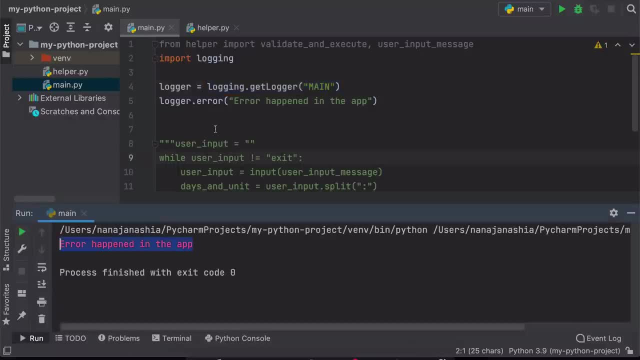 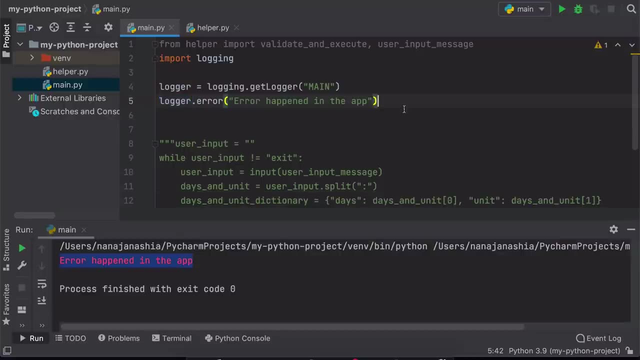 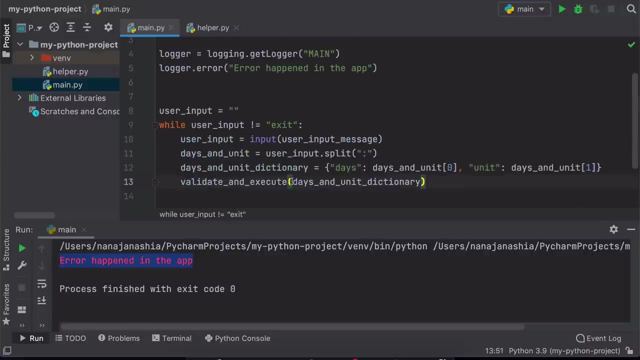 So if I execute this now and here you see the output of the logger, error happen in the app and logging in application is actually a very important feature. So that's why logging module is available by default in python and a use case In our application would be right here. 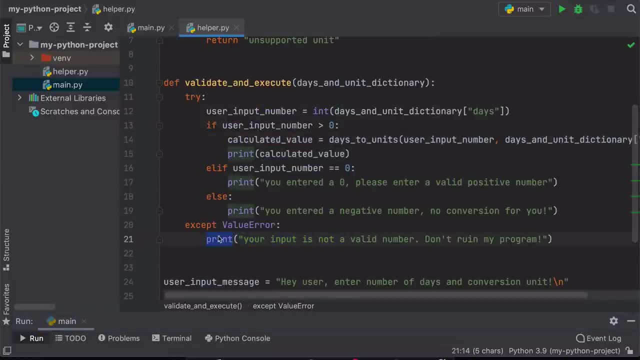 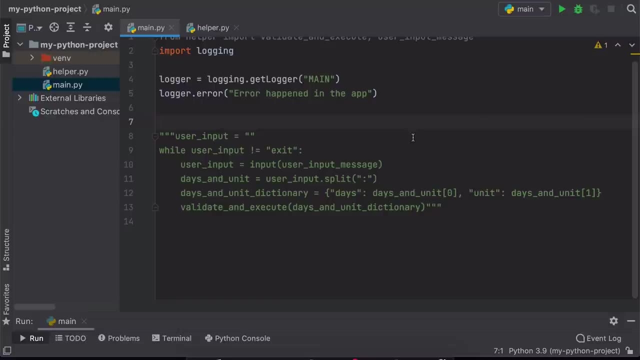 If an error happened, for example, instead of using a print, basically just log an error. So these were just some basic examples, But, as I said, Python comes with lots of very useful modules that you can use in your applications for different use cases. 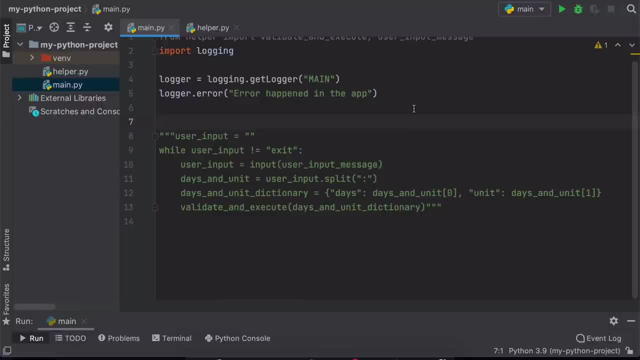 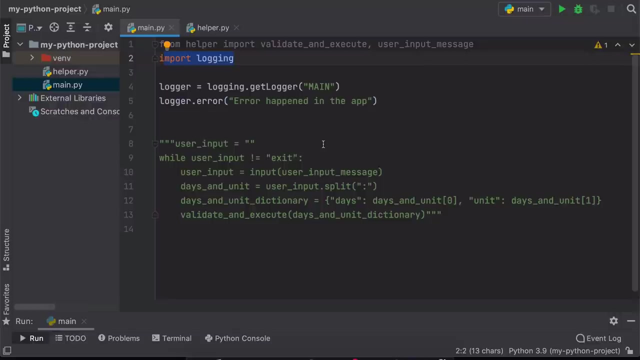 And that, of course, makes your work easier, because you can just use the logic instead of having to write it yourself. And the modules that are part of python, so that you can import them like this directly, are called built in modules. We learned about built in functions. 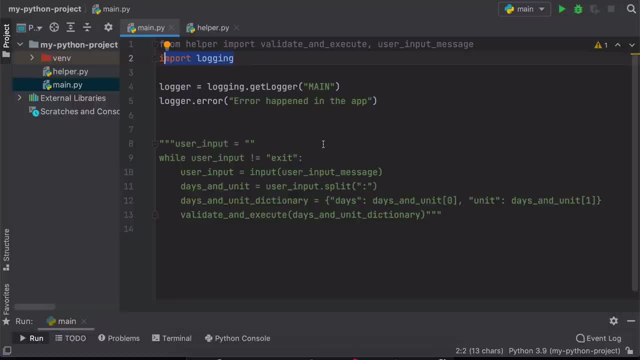 So these are the functions that python makes available to us directly, And there are built in modules that we get from python And, by the way, if you're wondering where this module actually comes from, so where is the physical location on our machine of where this module files actually leave? 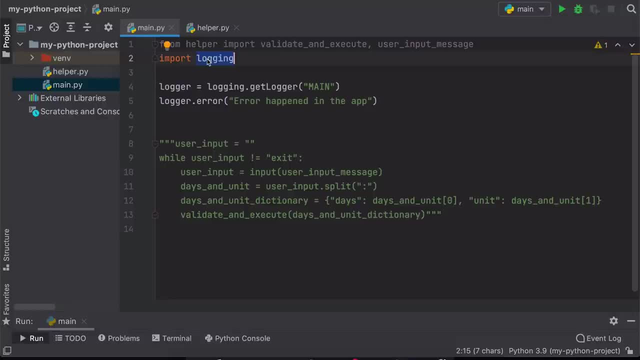 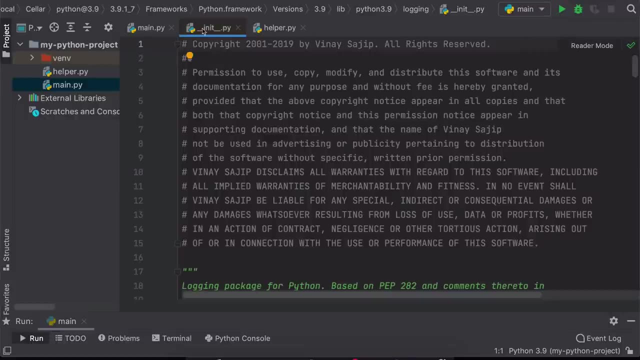 If you're using pie charm, you can actually hover over it and hold down the control key. Or if you're on Mac command key and click inside, you see the file opens up, which is the module, the logging module. Since, I said, module is basically just a python file that has multiple functions. 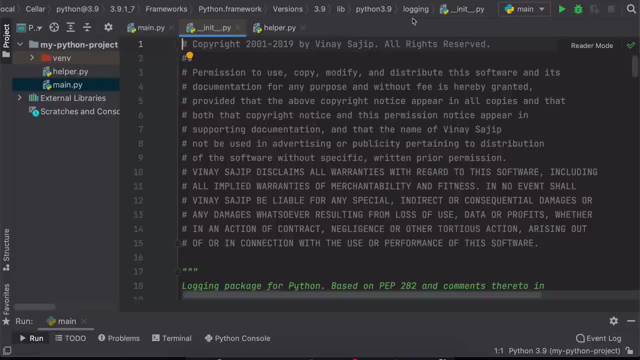 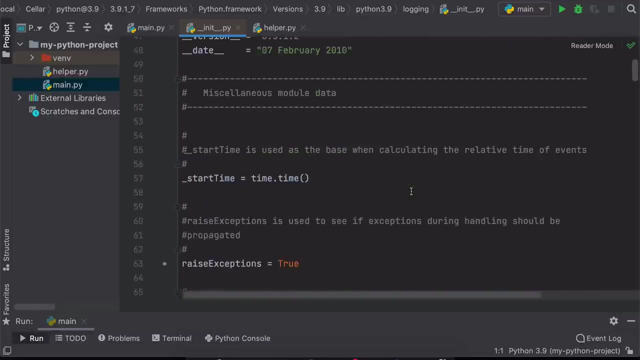 variables et cetera available and you see right here on this top line the whole path for that python file. So that's the location Of that module file locally on my computer and inside this python file basically again have python code. 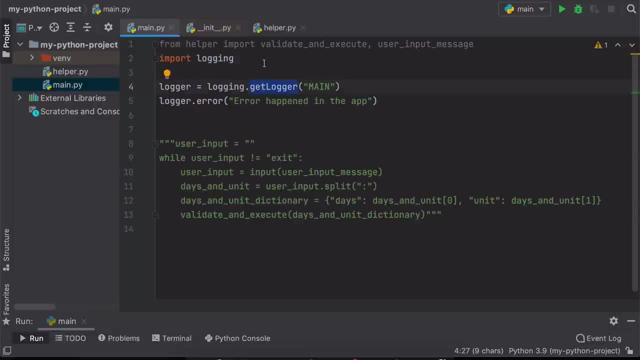 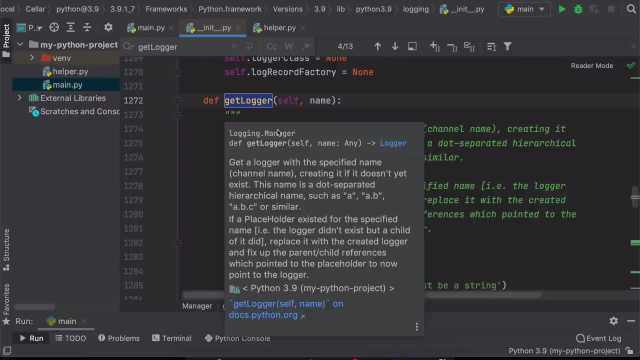 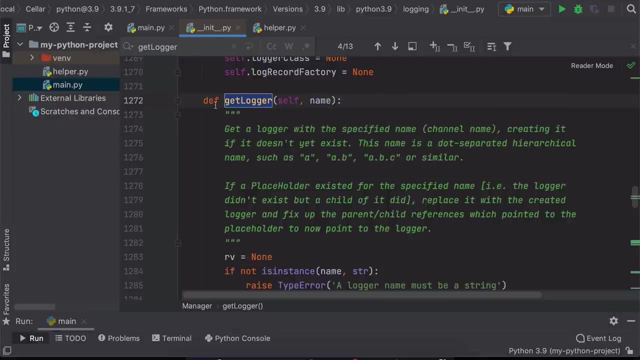 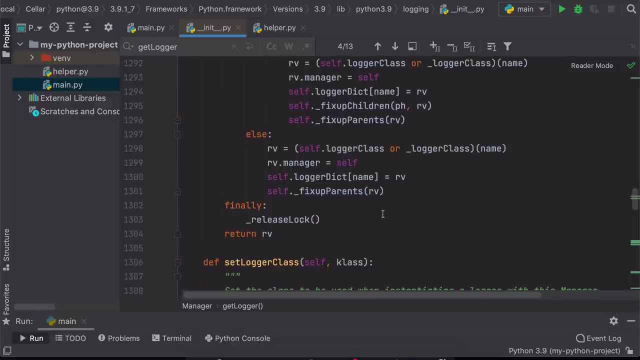 And if we look for get logger function here like this- right here you will find the definition of that function, right. So somebody implemented this function and called it get logger, And this is basically the logger: All the things that get executed behind the scenes and you as a user of python. 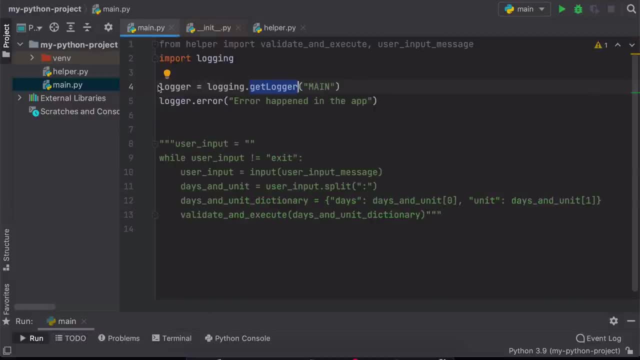 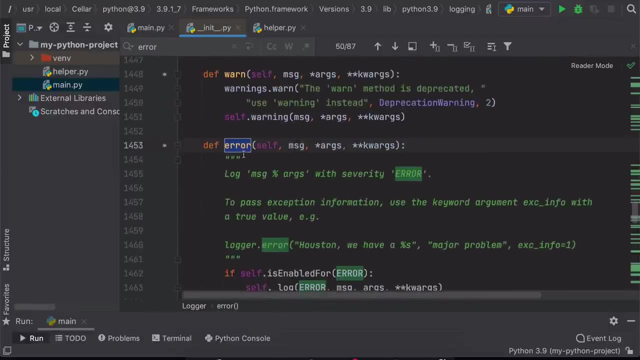 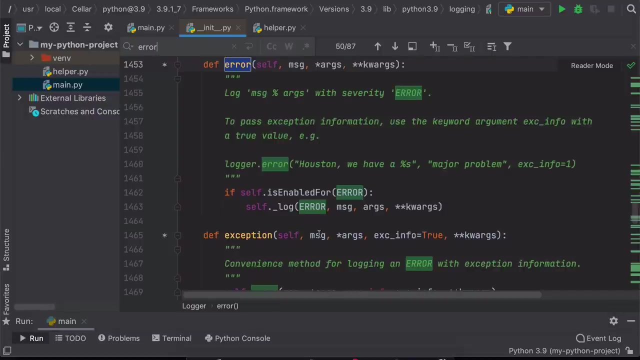 basically can use the name of the function and write your own programs with it. And let's also look for error. And there you go. We have air function as well right here, And obviously this is a more complex code here than what we write. 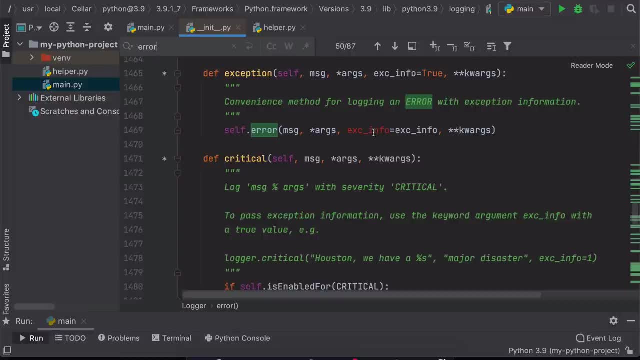 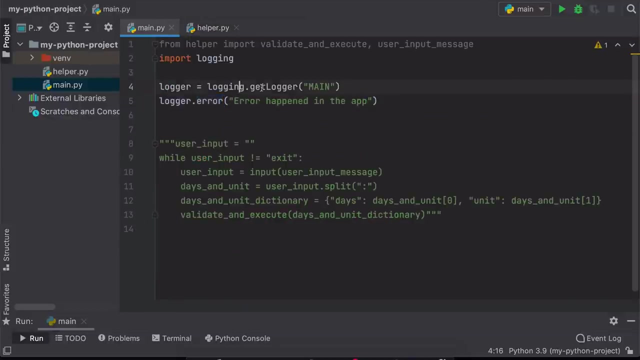 But just to give you an idea, that this is actually a file on your machine that comes with the python version that you install locally and all the functions are defined already there by python developers and you can just use them like this without worrying about how the logic is actually implemented. 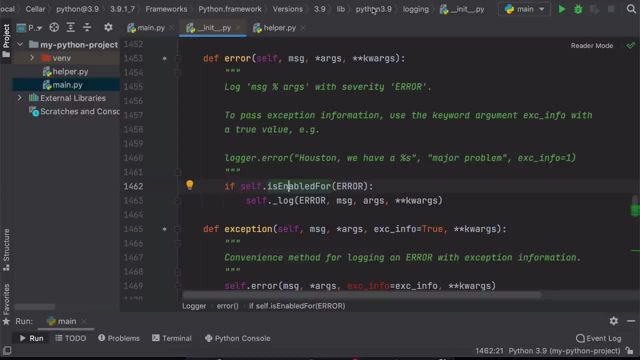 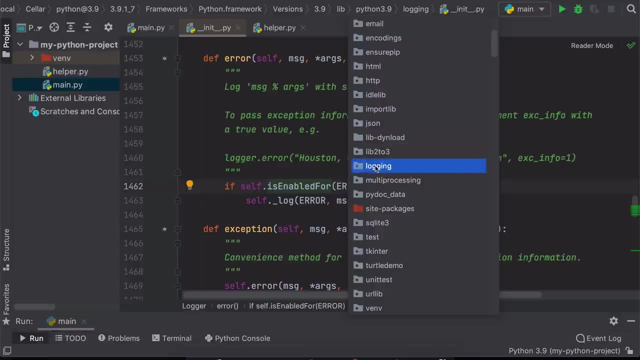 And another interesting thing is, if I click here in this python three point nine, Like this, logging is basically one module that we used, And here you will see the list of the complete list of all the built in modules that you get from python. 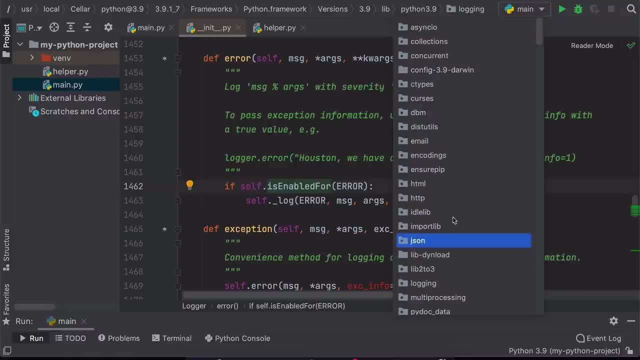 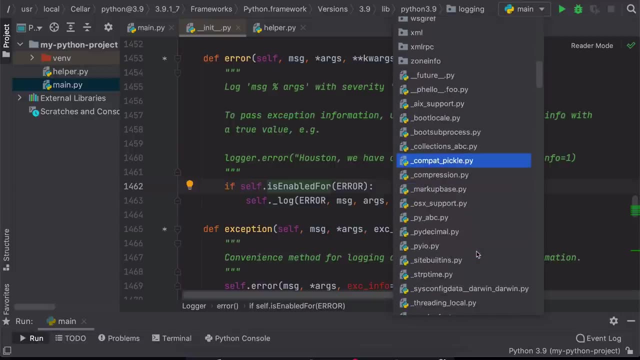 So some of them are folders like logging, for example, email and bunch of other stuff, And the operating system module, for example, that we used is a python file. Then you can find right here. So these are the built in modules. 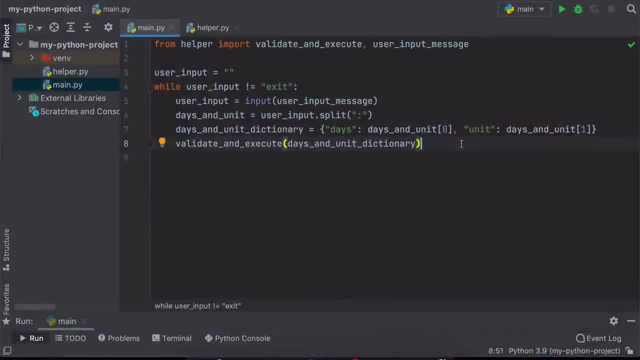 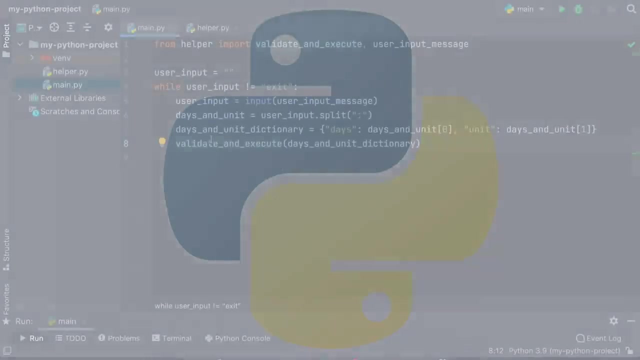 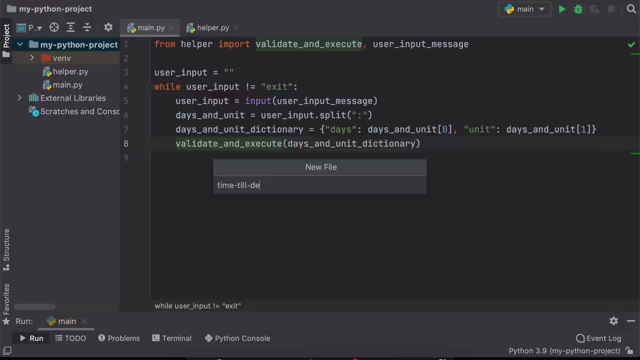 So now that we know what built in modules are and how to use them, that's actually see a realistic example and also write a little more interesting application using built in module. So what I'm going to do is, in my python project I'm going to create a new file and I'm going to call this time till deadline. dot pi y. 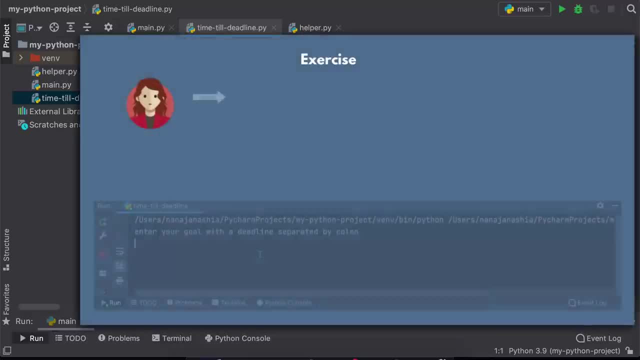 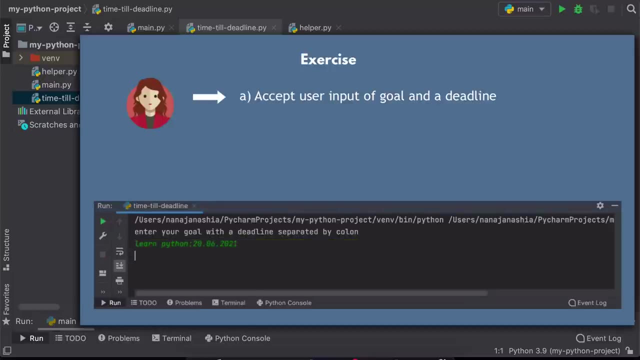 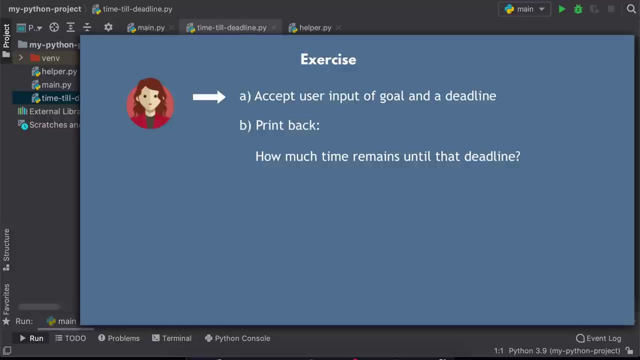 And we're going to write An application that basically accepts a user input of a goal and a date like a deadline date And then we're going to print out back to the user how much time it is remaining till that deadline And that deadline will be a date. 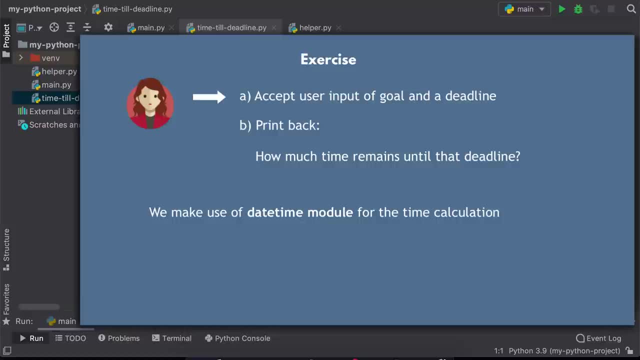 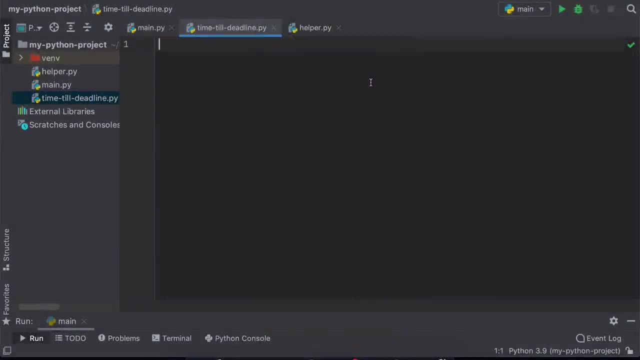 write some date in the future. So that means that we're going to be working with dates And in order to work with dates we are going to need python's built in module That allows us to call functions and do some processing and stuff on date values. 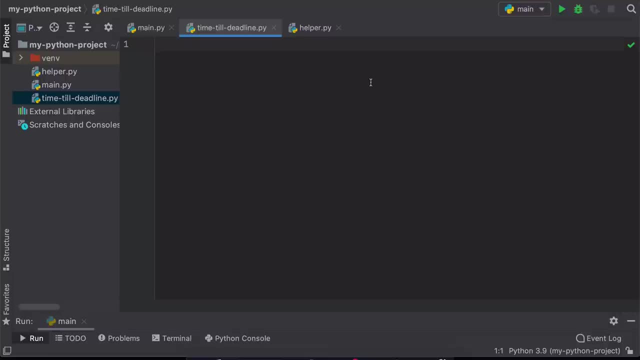 And that module is called date time, So import date time. So let's have that import statement right there and we're going to use it in our program. So the first thing we want to do is let the user give us an input about their goal and a date or deadline. 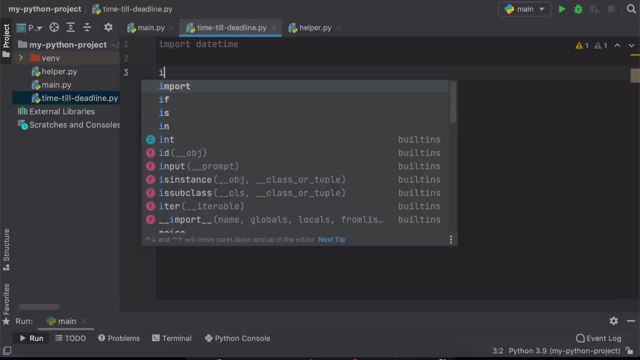 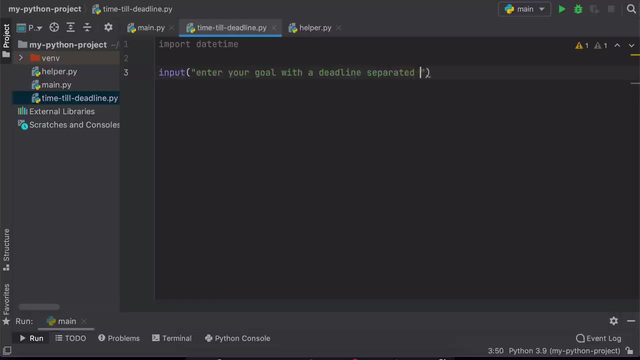 For that goal. So let's do that first. We already know how to ask for user input with a message. So we're going to say: enter your goal with a deadline Separated by color, And we also know this already Basically. 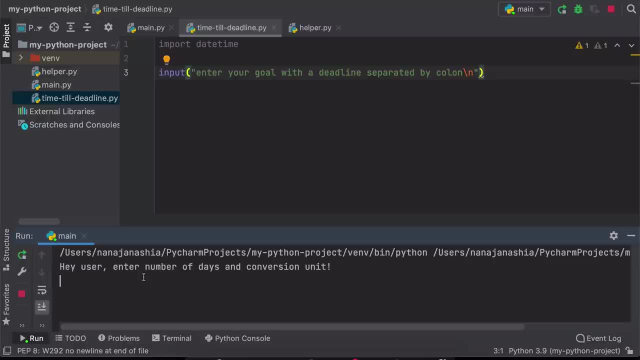 what we want to do is user to be able to enter their goal like learn python, colon and a date. And let's say again, this is totally up to us to decide where the ones basically setting the rules here. So let's say we want the date to be entered in following format: 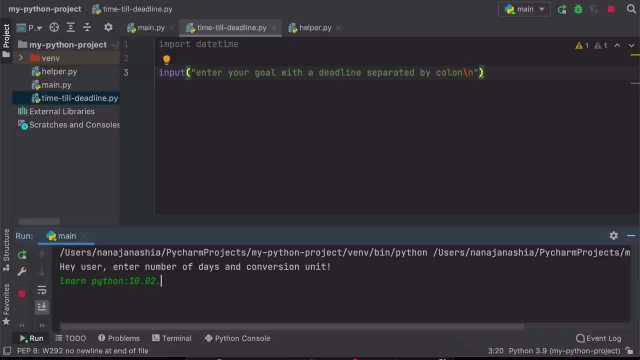 Day, Month And a full year like this. So that's the format that we're looking for And this is how user should input the value. Otherwise, with a different format, it's not going to work. So we're going to save that input value into a variable. 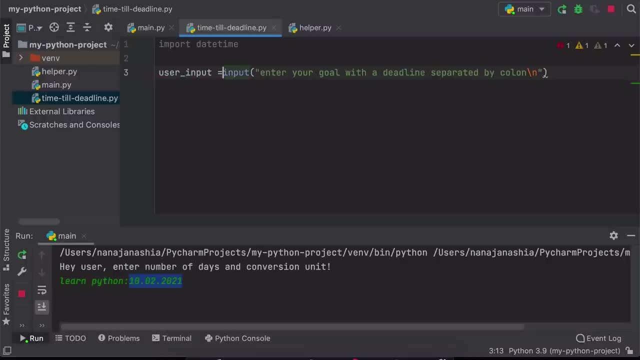 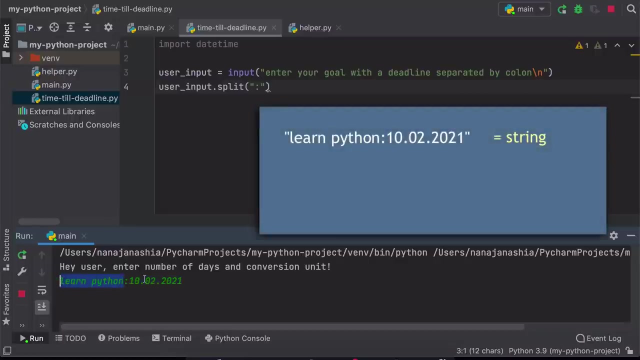 Let's call it user input. So we have the user inputs. Let's do the split again on a colon. Remember, we have this whole thing as a string, as one string. So we want to split it into two parts. So we have the goal here and the deadline. 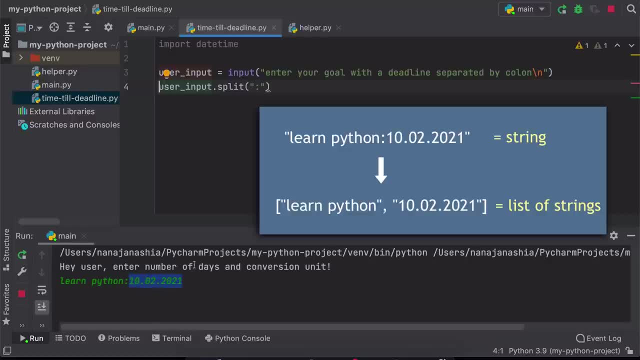 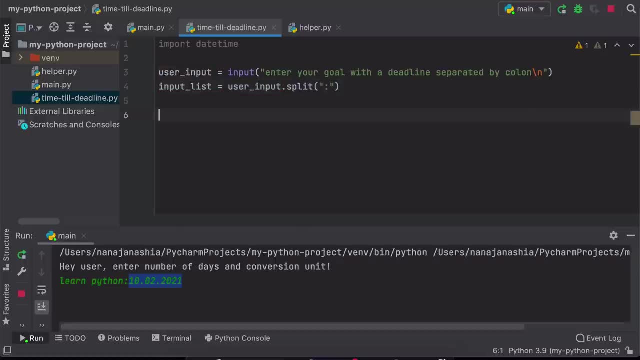 And this will give us a list With those two values, And let's call it input list. And now from that list we can actually extract or get those individual values using a list syntax, So accessing the elements from the list- which is what we learned already- using an index. 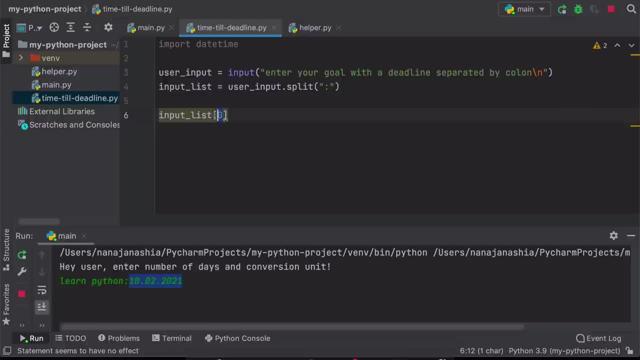 Right, So we have input list index zero, which is going to give us learn python, And let's save it as a goal variable. And let's create another variable which is going to be date. Let's call it deadline, And this will be the second value in our list. 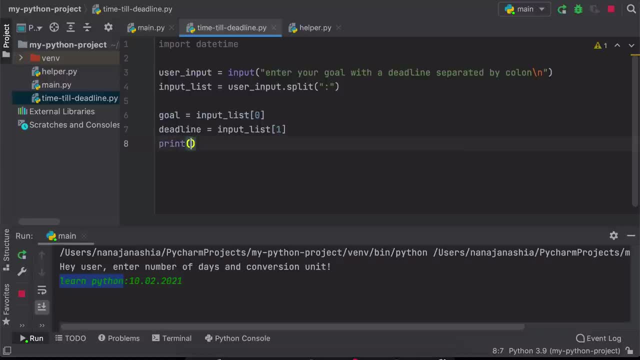 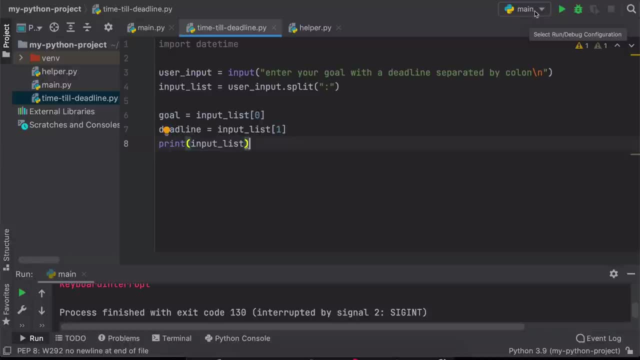 And we don't want to execute main python file. is that we want to execute this one right here? We basically just want to ignore everything else in this project. So how do I go from Maine to this file? Execution very easy in this editor. 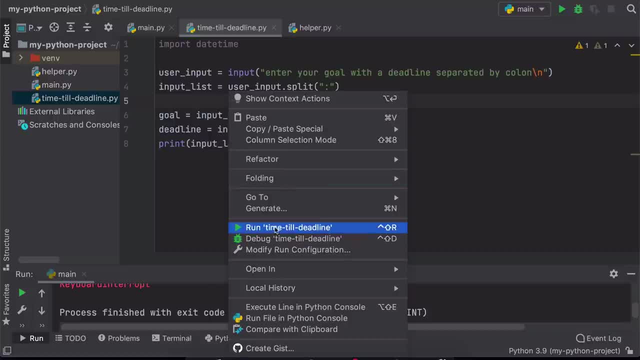 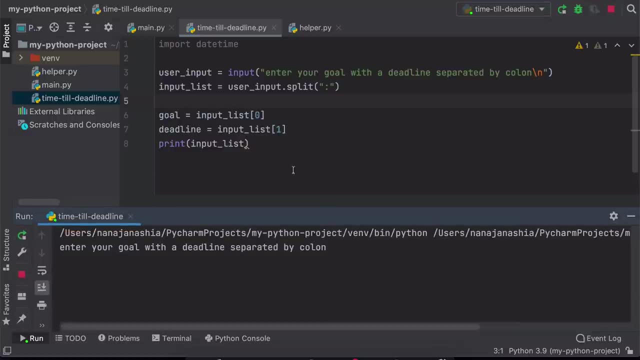 Just do right click And you see here run time to deadline and I'm going to execute this. Everything else is ignored in the project. We are basically just working on this one right here. So enter your goal with a deadline separated by Colin. 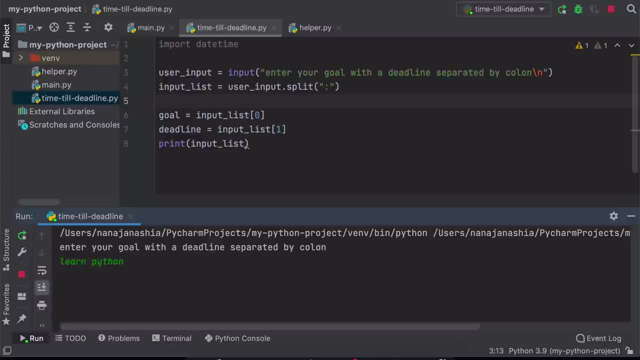 Let's do that I'm going to do- learn Python, Colin- and then let's enter some date and enter, And this is the output. So we basically split that into two values and put it in a list right here, and very important to note here- that both of these 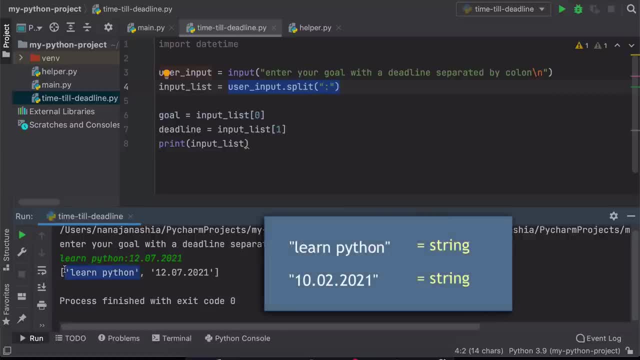 elements in this list are strings because, again, user input is always interpreted as strings. So this was a string and it was split into two strings, which are learn Python and this date. here, However, we don't want date or deadline as a string. 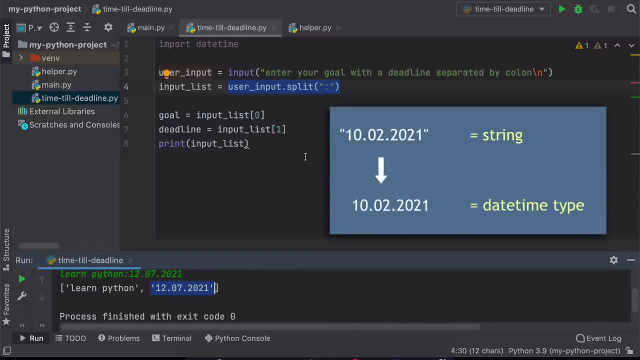 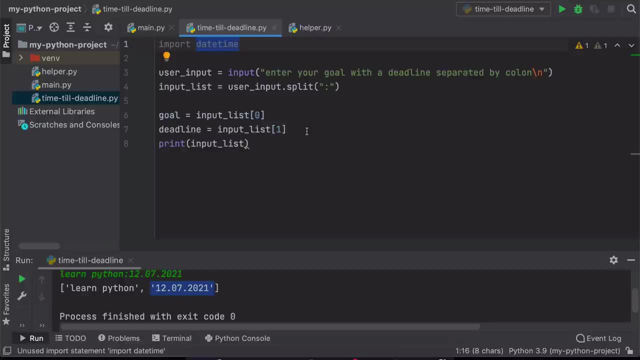 We want deadline as a date, And exactly for that functionality we need this date time module. because we don't want to implement it ourselves, We want Python to give us a ready function from a module that will basically just let us convert the string into a date value. 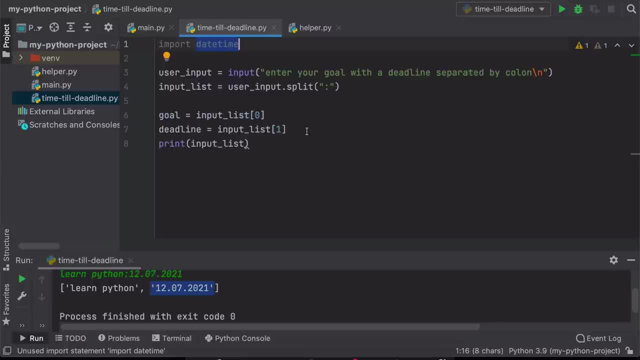 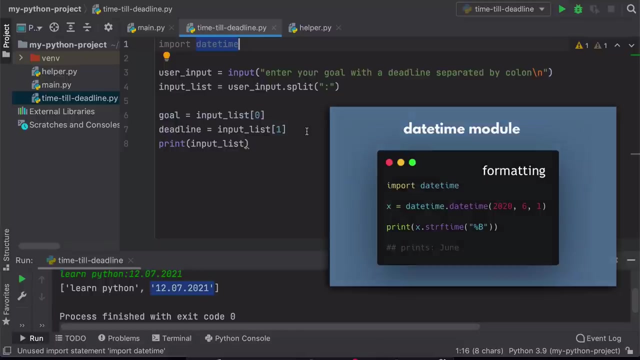 and converting string to date is just one example usage of date time module. But you can use this module to work with dates generally, like creating new dates, formatting the dates, updating values, et cetera, and we're going to see some of those examples in this section. 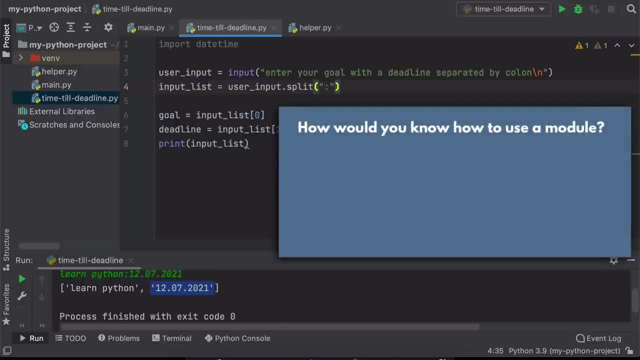 Now, if you're learning this type of thing alone, you don't have me basically teaching you and giving you an example. the way you would do that is you would basically research and maybe Google how this is done in Python And you would basically see some examples of using these dates: time. 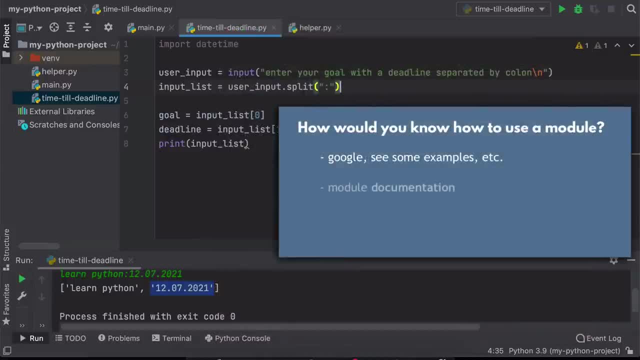 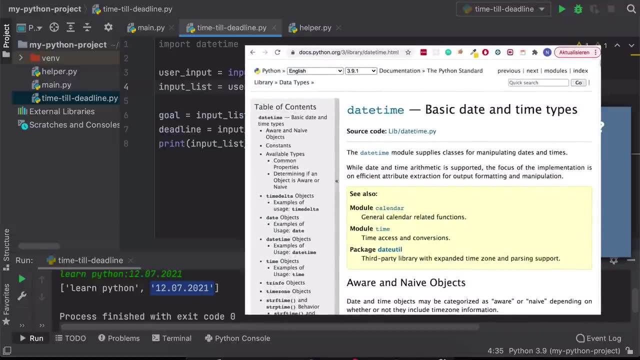 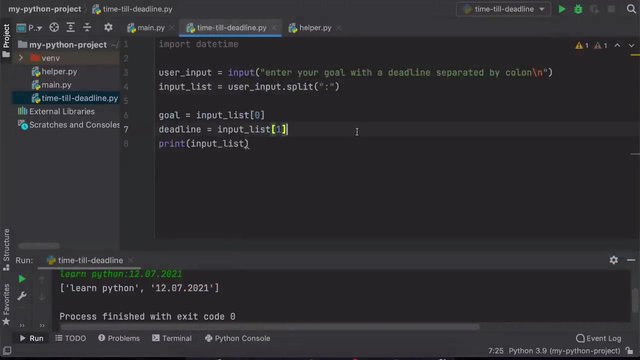 and what the name of this function is and how to use that as well. As each module has its own documentation page where you can look up the syntax and usage examples, because obviously you're not going to know how to do that by yourself. So the way we convert a string into a date using this date, 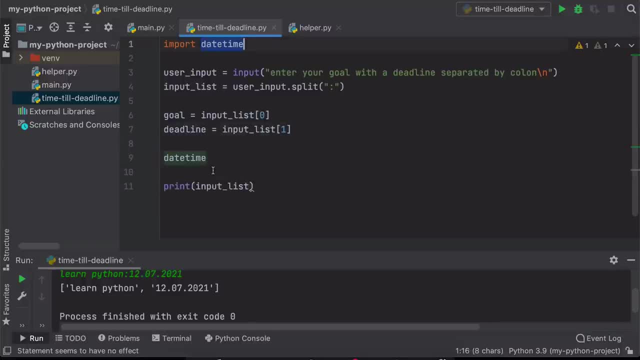 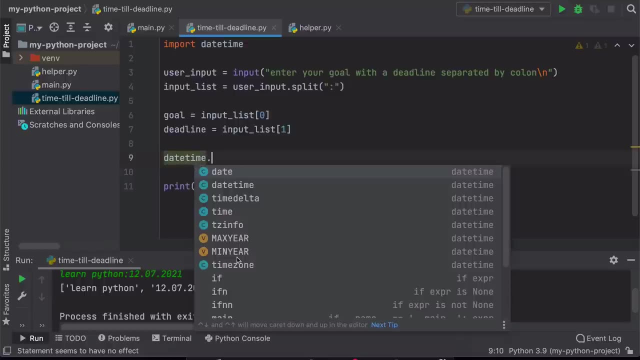 time module is on this date time module. If I type in that, I will see a list of all the definitions that date time module gives me Right. So I have date, date time Time, et cetera. The one that we need is date time, because the function that we need 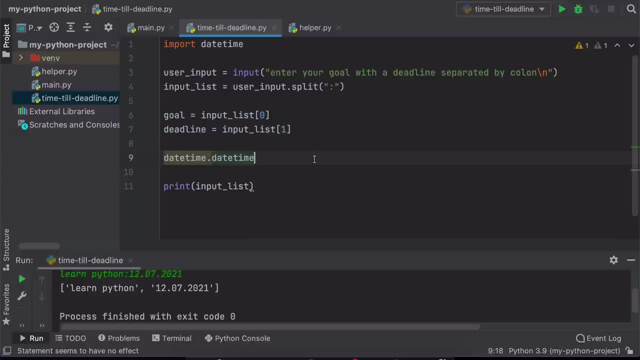 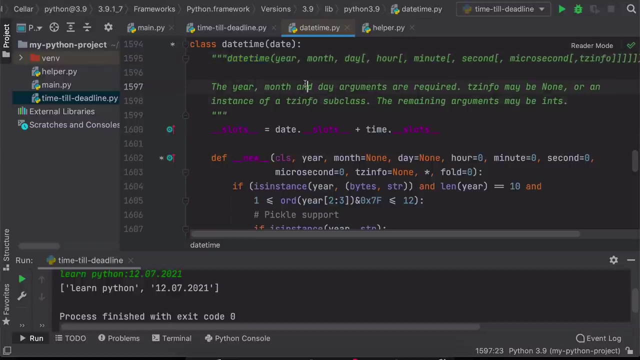 for conversion is inside that definition. And don't be confused here, because we have date time twice here. The first one is a module and the second one is a definition in that module And we can actually check that as well. So I jump into this date time module and inside that. 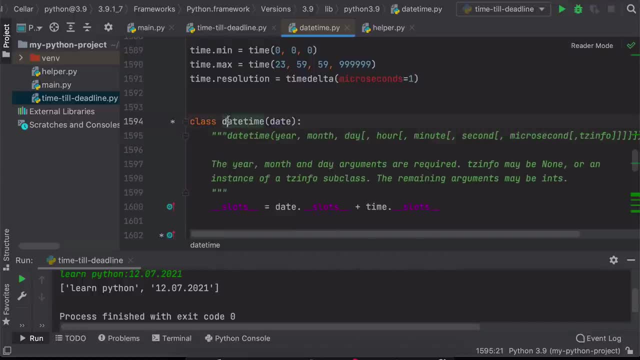 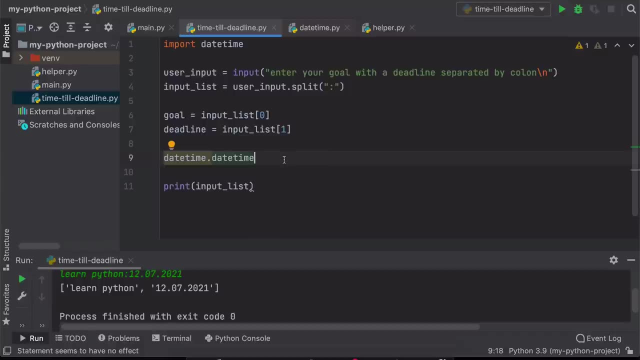 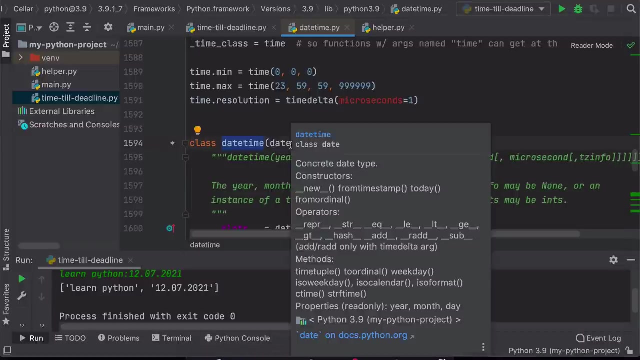 if I look for date time again. So Right Here you see this date time definition and on that date time definition we have now functions that we can use. And, as you see, this is not a function or a variable. It says class here, which is another concept in programing. 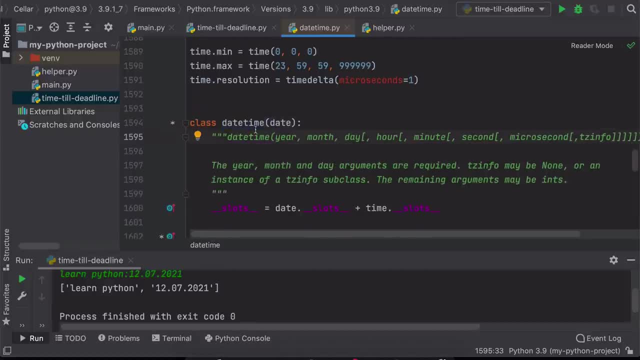 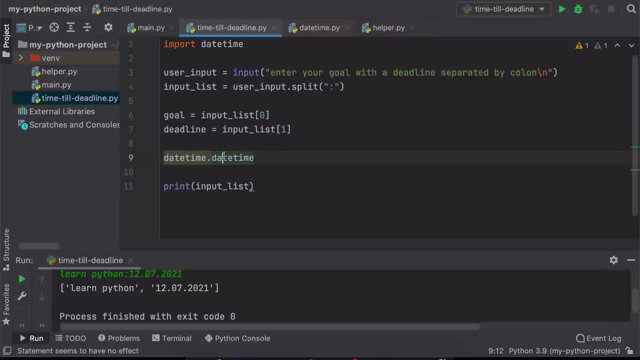 We're going to see later. So just for now, think about this as a container of functions and variables inside that module, And that's why we have to access it like this. And then, on that, date time Definition is class. We now have functions that we can use to do the conversion. 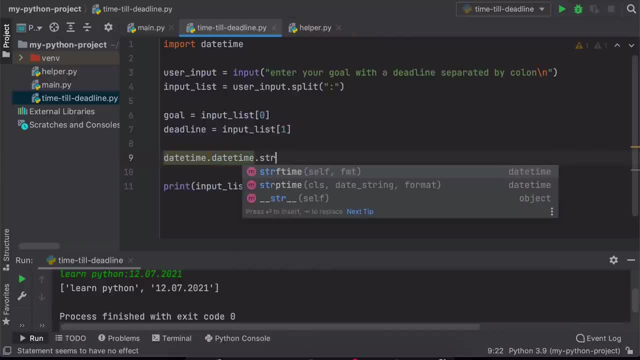 So the function we need is called STR, So string P, time, And this function will take a string representation of a date and will convert it into a date format. So our string representation is deadline and we need to pass in the second parameter because, remember I said 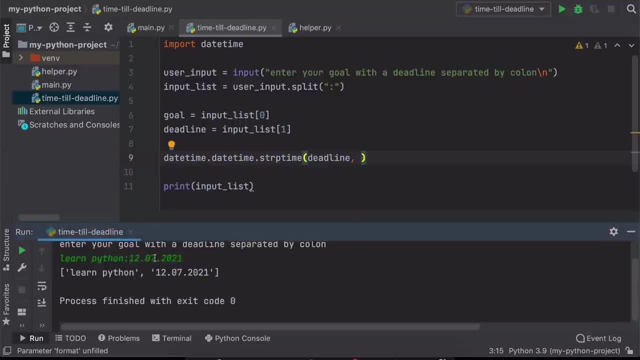 we basically decided that the date should be entered like this, with points and a full year here And, as you know, there are lots of different formats and types for dates, right, Depending on a country or a language, or even within that language. we basically have multiple different formats. 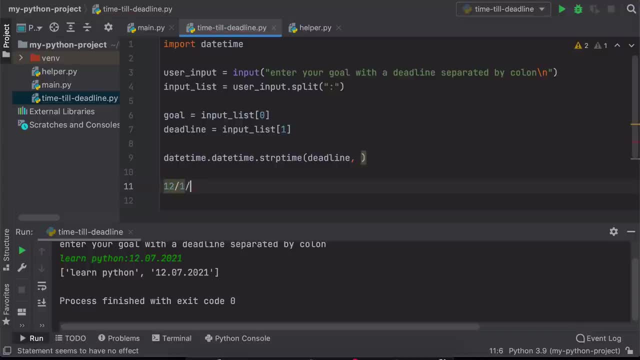 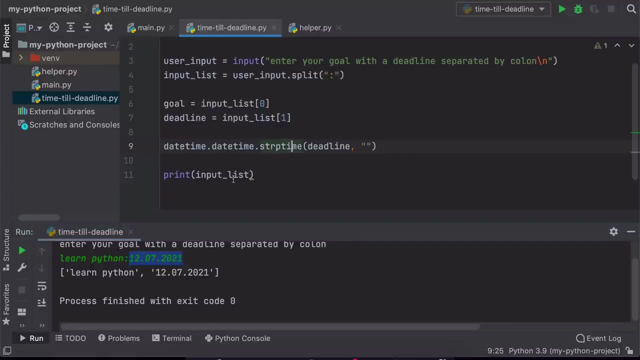 Right, We have formats like this, or we could also have a shorter version of the year, Etcetera. So we need to define here the format that we want Python or this method here to use when converting this string into a date, again, because there are so many different formats available. 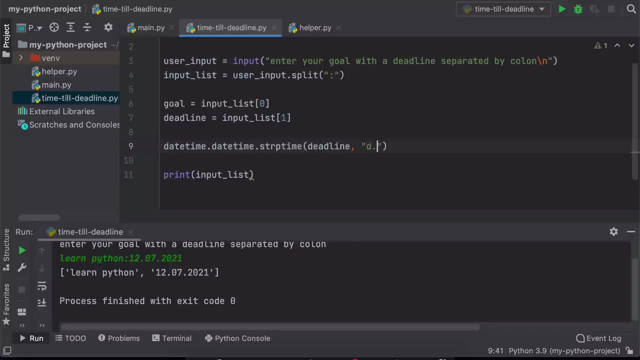 So what we have here is a day, Then we have a dot, then we have a month, again a dot, and then we have an ear. So this is kind of a main structure of a format. However, formats for dates have their own specific. 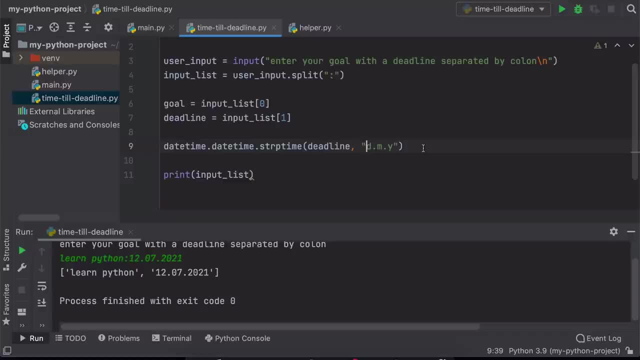 syntax, and this is actually for all programming languages. So what we need to do is put this percentage sign in front of every letter. So again we have a day, month, year. and there is one more thing about this format. This format right here matches this date. 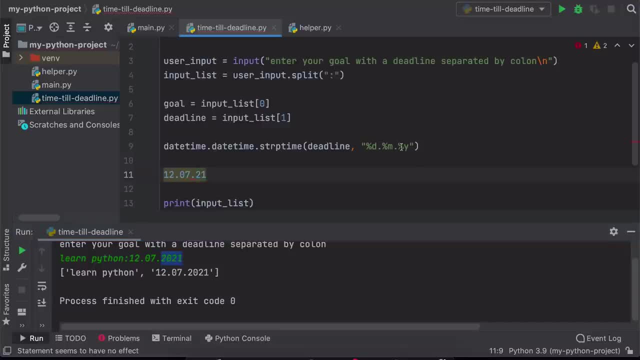 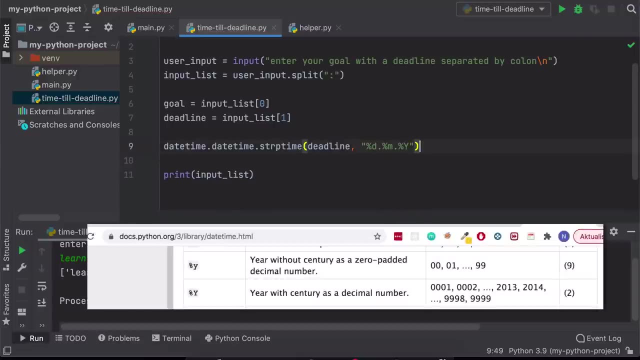 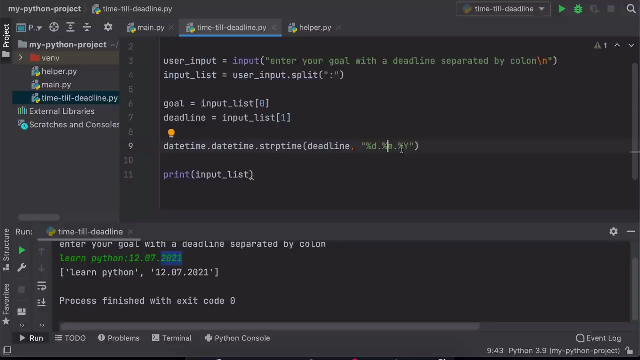 However, we want the full date, not just the last two, And the format for that would be a capital Y. Again, this is something that you would look up in the documentation of the module instead of knowing it by heart, But just know that these type of formats are used when working. 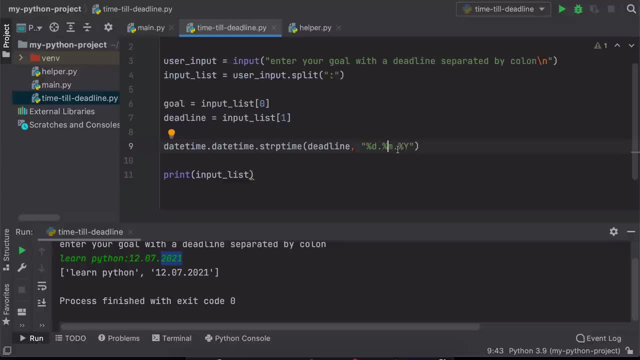 with dates, and this is not specific to Python. You will actually see something very similar in all the other different programming languages and that will do exactly what we want. It will take this date here and give us a proper date format from it. Let's actually test this. 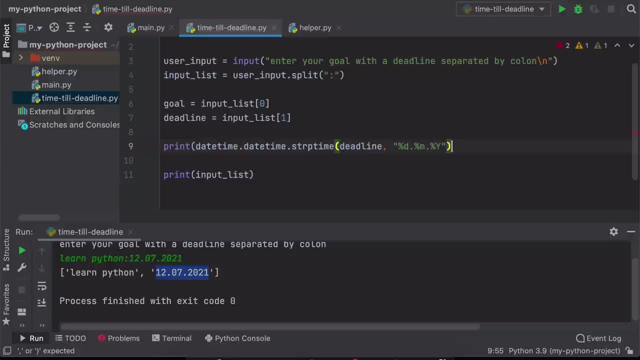 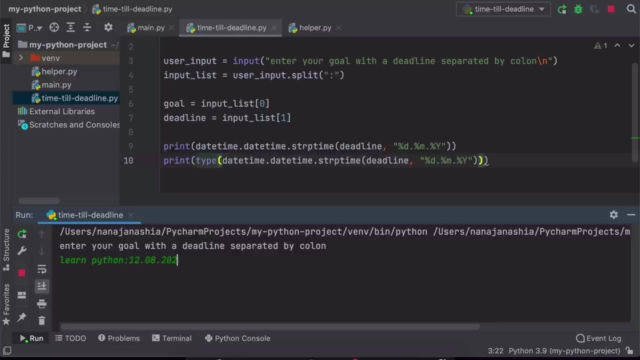 So I'm going to print this first and I'm also going to print a type, a data type, of that value. So let's execute- I'm actually going to copy that, so I don't have to retype it over and over again- and enter. 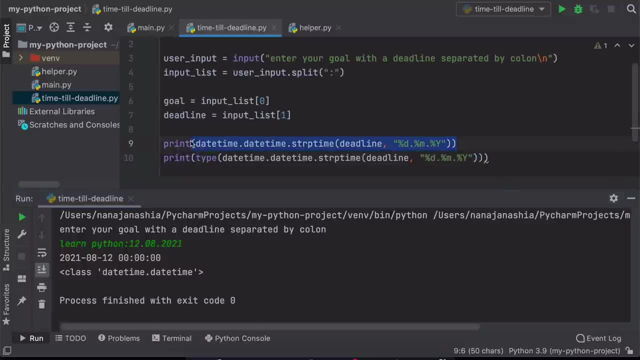 And here you see, we printed first of all the date, not a string, and this looks like a proper date and not a string anymore. Note the change in the format Plus. we have these zeros here, which represent hours, minutes. 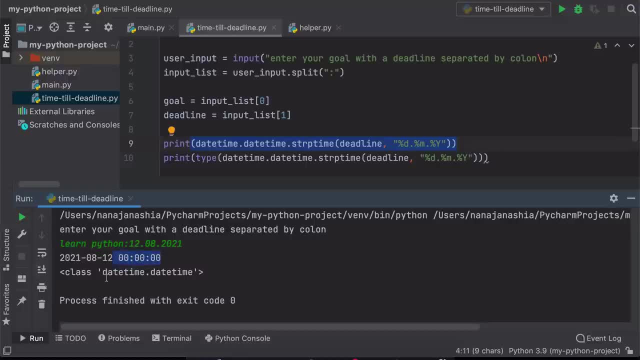 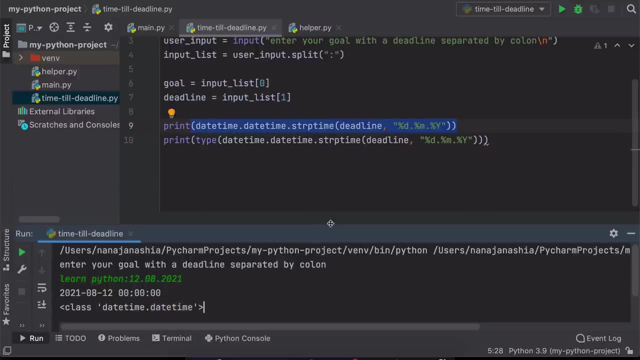 and seconds. We didn't set any of those. So these are all zero And we have the date time type again. Note: date time for a module name and date time of the class name. So this is the type of our Converted date and the reason why we needed to convert that. 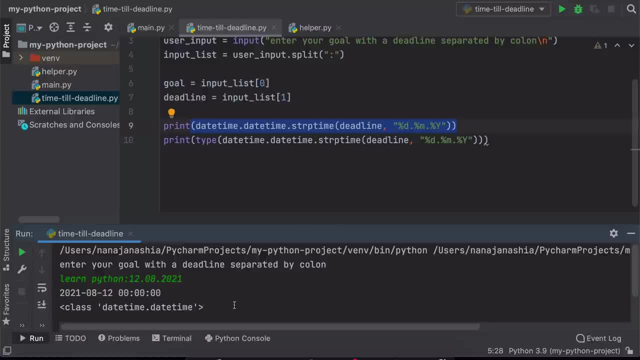 string into a date is because we want to calculate how many days or how many hours are remaining until the deadline from now, starting from today, and to do that calculation we need to have date type, because we can't do that on a string. Great. 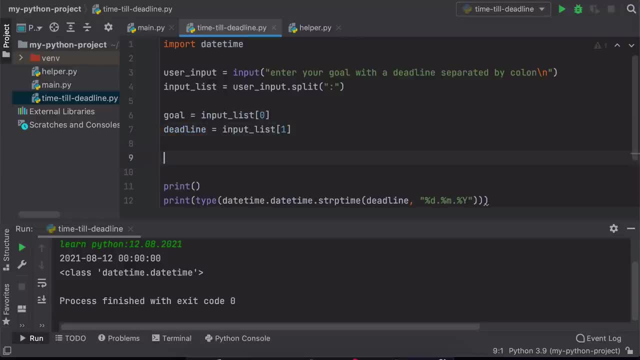 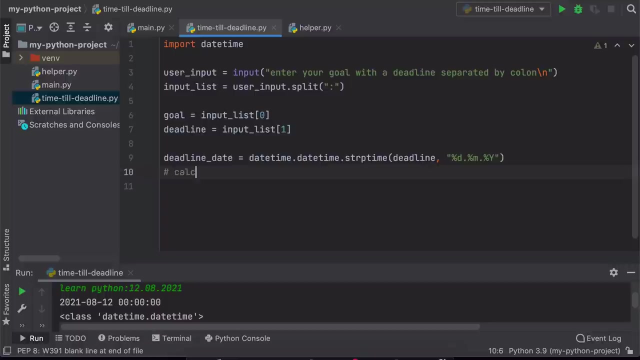 So now we have our deadline represented as a date. so let's actually Assign this to a variable, say deadline date, like this, and remove this. and now we need to do a calculation: How many days from now till the deadline? we already have the 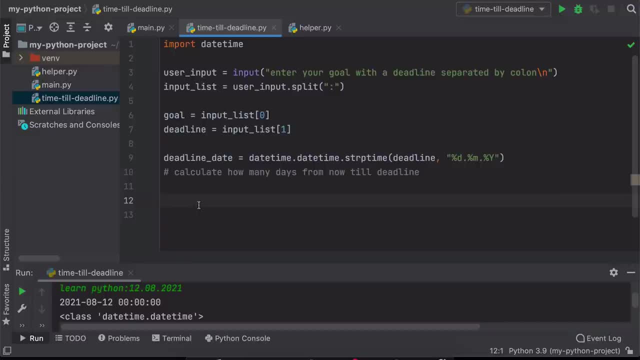 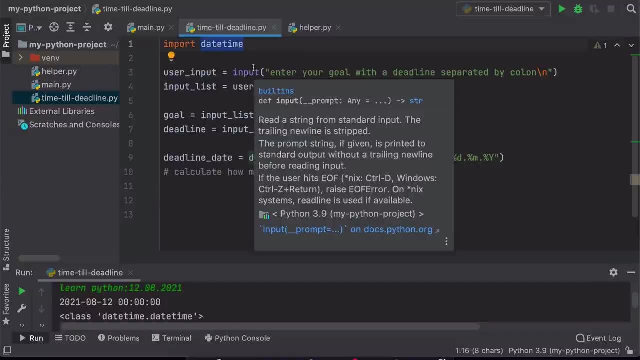 deadline we need now again. now is, or today is also a deadline, So we can actually do that. And since we have this module date time, we can also assume that this module will give us some function to tell us the date of today. 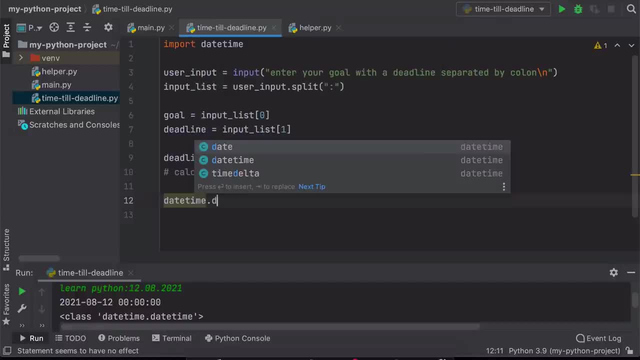 And if I do date time again, date time class, And today you see that we have this function available and this will basically give us the date of today. so, depending, obviously, when you Execute this program, it will give you always the current date. 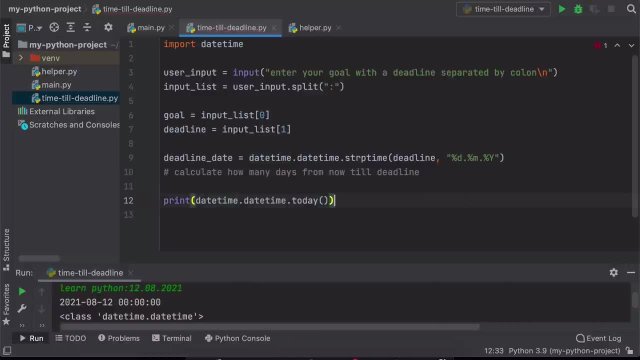 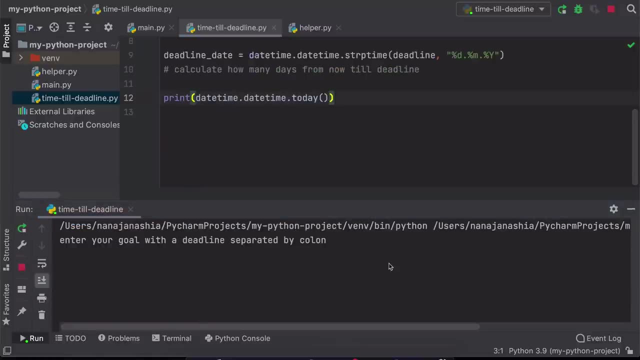 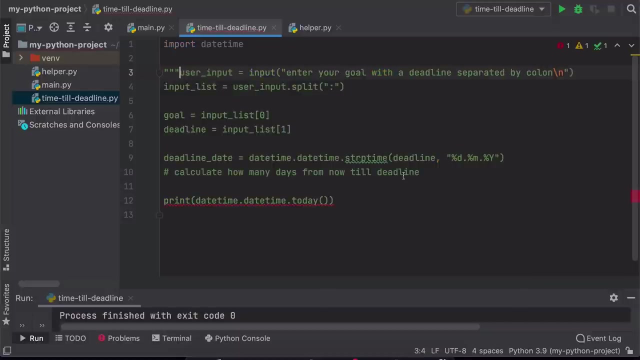 So let's print it. today for me it's 7th of February, so if I execute it now, I'm going to enter this. and today is 7th of February for me, So if I execute this, it's actually coming this out here. I. 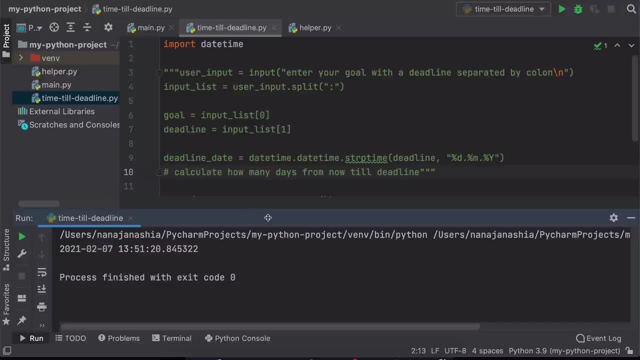 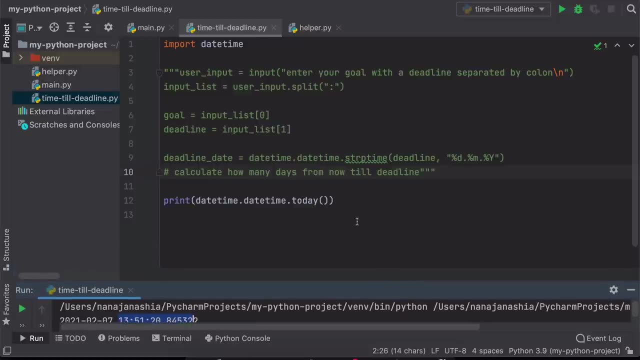 have the date for today, which is 7th of February of February plus the exact time it is now. but we don't care about the hours and minutes and seconds, We just care about the day. So that means we already have deadline and we. 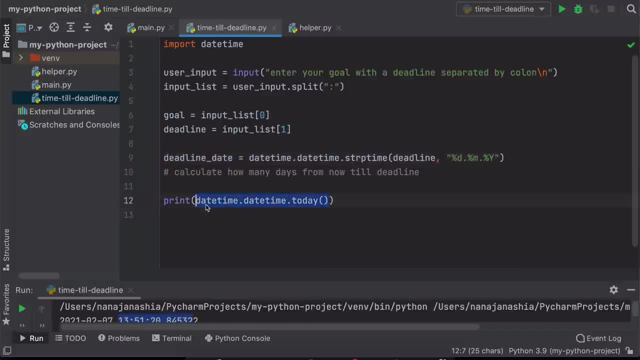 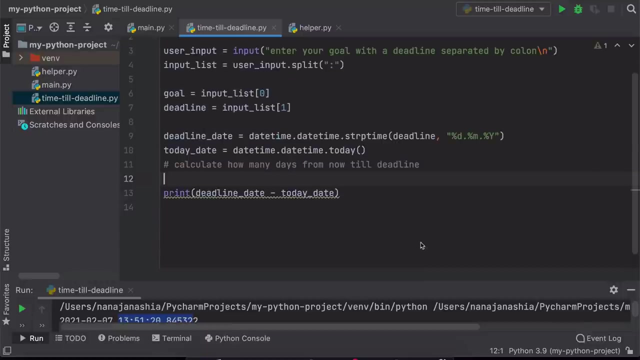 have today. Let's also add it to a variable like this, And now we can actually do the calculation. Calculation is super easy: We just say deadline date minus today date, And this will actually give us the difference between, or time difference between, today and the deadline date in the future. Again, let's actually 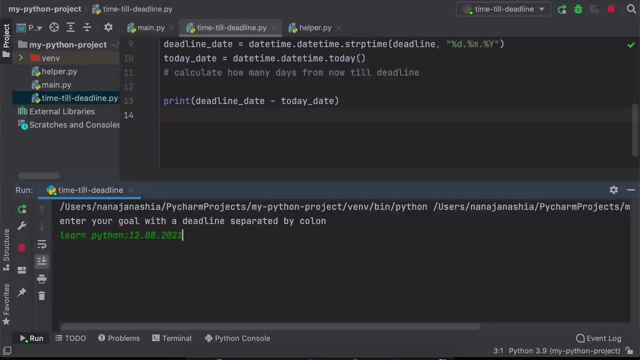 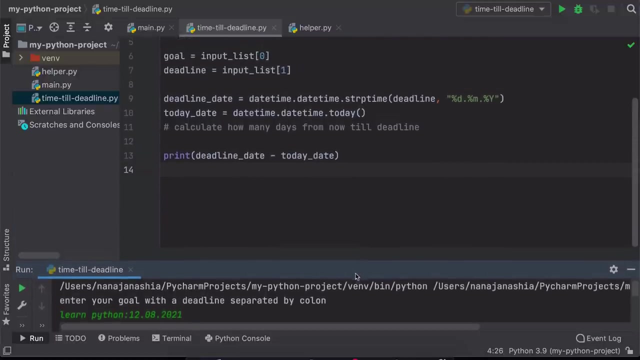 try this out And you see that. So this is 12th of August for me. today It's 7th of February. So the program calculated that there are hundred and eighty five days until the time, Plus how many hours, minutes, seconds and milliseconds. So that was a pretty easy calculation. 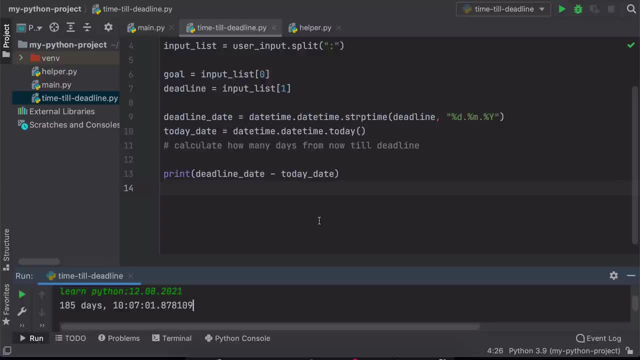 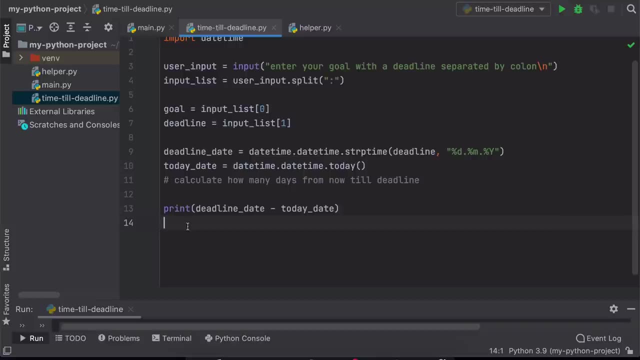 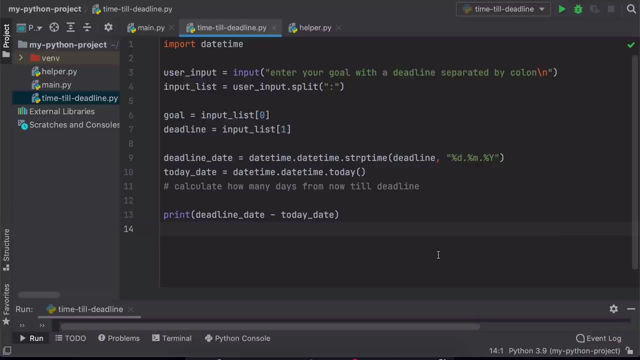 Now what we want to do is tell the user some kind of message, and we want the message to be: dear user, the time remaining until the deadline for your goal- Whatever the goal was- is this. So let's actually put that text message together and bring it back to the 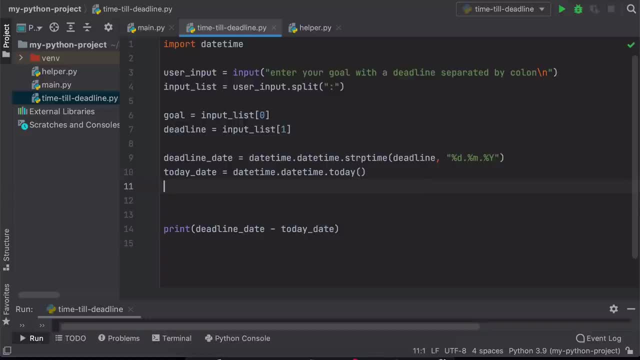 user. I'm going to save it into a variable, let's call it time till. and the message: dear user, time remaining for your goal. and here we want to print what the goal actually is. and you remember how we format a string. when we want to use a variable, we put: 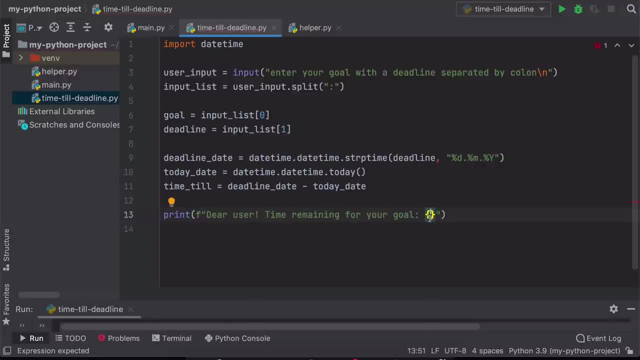 an F here and in curly braces. now we can use variables or numbers or some other expressions which are not string. so first of all we're printing back the goal. so time remaining for your goal- whatever goal they entered- is time till. so time remaining for your goal, whatever goal they entered, is time till. 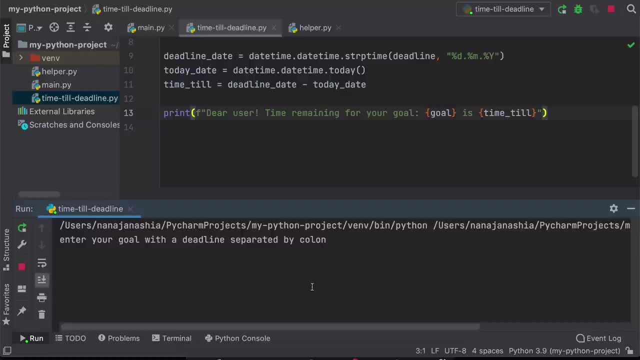 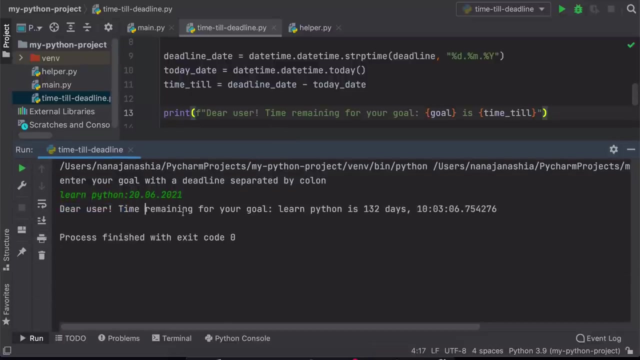 so time remaining for your goal, whatever goal they entered, is time till, and let's execute our program and let's give it some other value. like this and enter- and here we have our message. dear user, time remaining for your goal- learn python- is 132 days and this many hours, minutes. 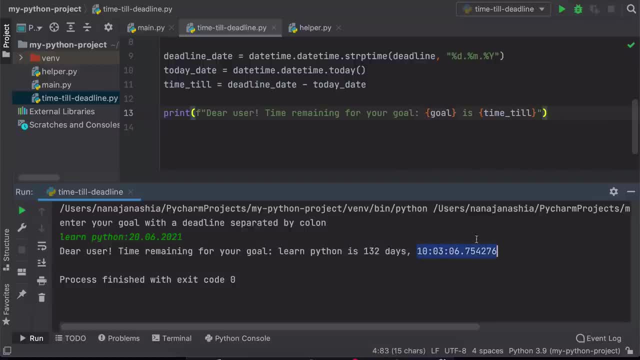 etc. now let's say we don't care about this whole thing here, etc. now let's say we don't care about this whole thing here, etc. now let's say we don't care about this whole thing here, we just want to know how many days are. 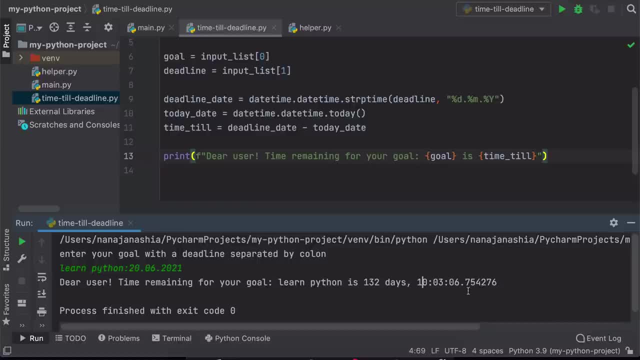 we just want to know how many days are. we just want to know how many days are remaining. so how do we get rid of this remaining so? how do we get rid of this remaining? so? how do we get rid of this part? here again, very easy, and the time. 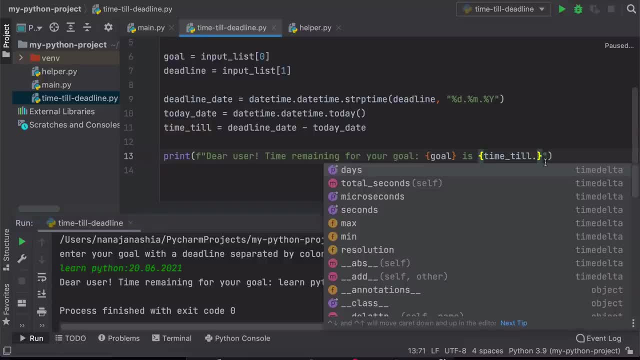 part- here again very easy. and the time part- here again very easy. and the time till: if i do dot, here i get a list of till. if i do dot, here, i get a list of till. if i do dot, here i get a list of suggestions for functions or variables. 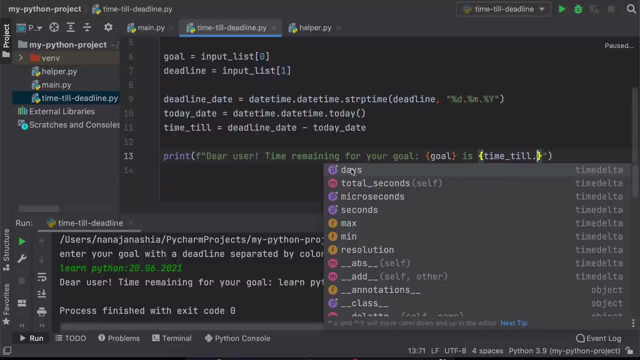 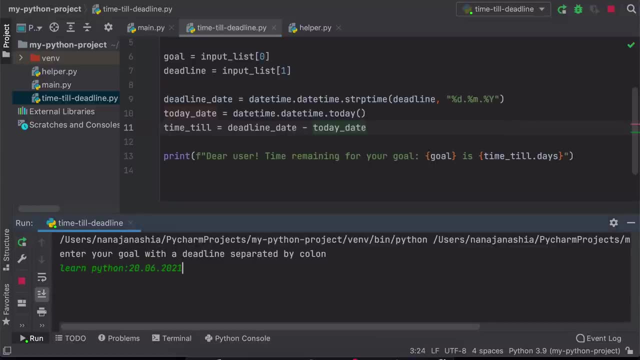 suggestions for functions or variables. suggestions for functions or variables that i have available and one of them that i have available and one of them that i have available and one of them is days, as you see here. so if i click here and save and I'm going to reuse these inputs because I don't want to type, And as you see, 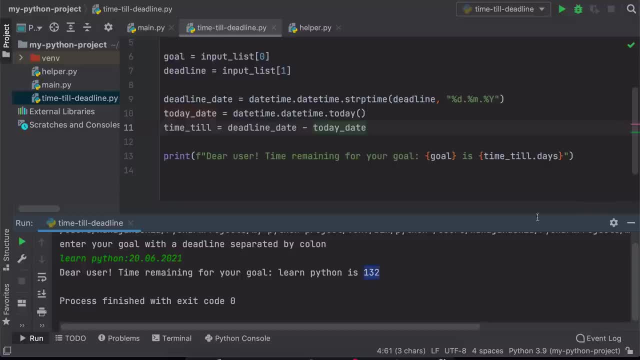 we got rid of this whole thing here and we just have days, and let's actually write days. And there you go, We have a cleaner output now for our user. And finally, what if the deadline was just a couple of days in the future and the user wanted to know how many hours are remaining till? 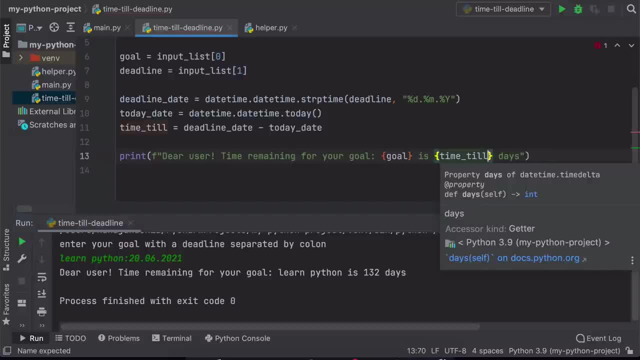 that deadline. We can do that by getting rid of these days and again type in dot and we have something called total seconds here which gives us the time different in total seconds, And now we can reverse, engineer and calculate the number of hours from this total seconds, which is pretty. 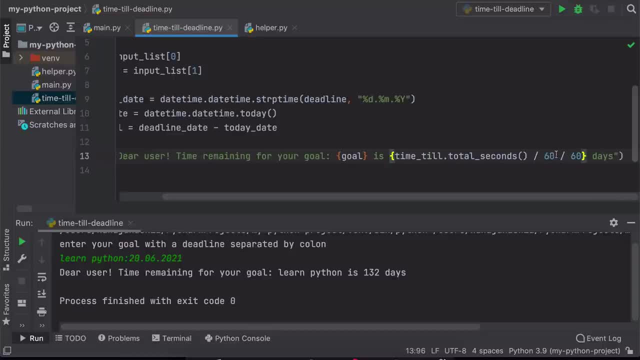 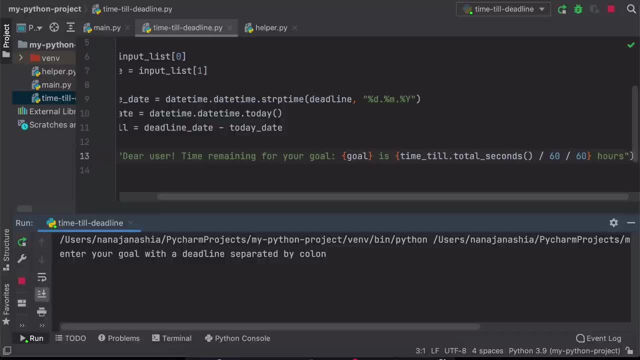 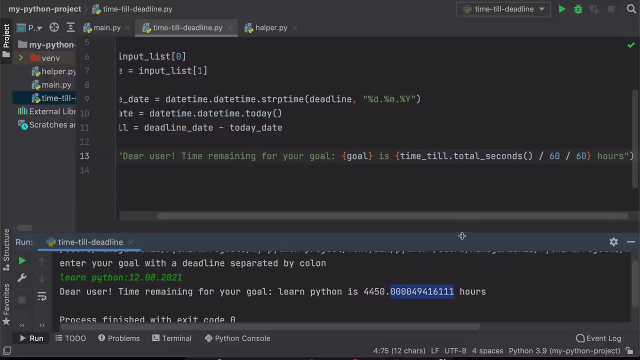 easy Like this: calculate minutes and then calculate hours. And I'm going to execute this again. And here you see the number of hours with a decimal precision. So we have four thousand four hundred fifty hours. point some fraction number here Again. 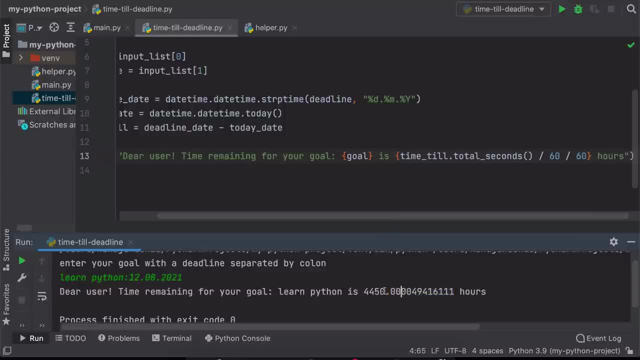 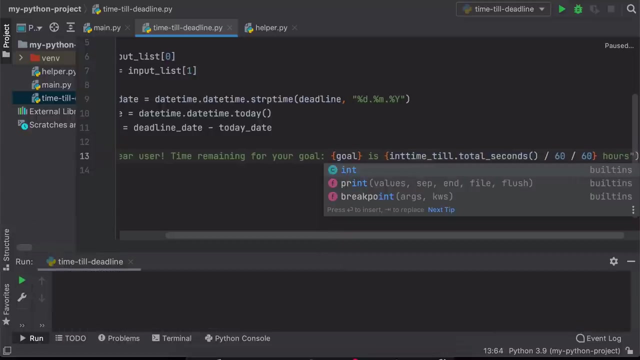 we want to get rid of this extra stuff And, as you see from the syntax, it is actually a flow number with a dot here. So what we could do is basically convert this whole thing, this float number, into an integer. So convert this whole thing into an integer using 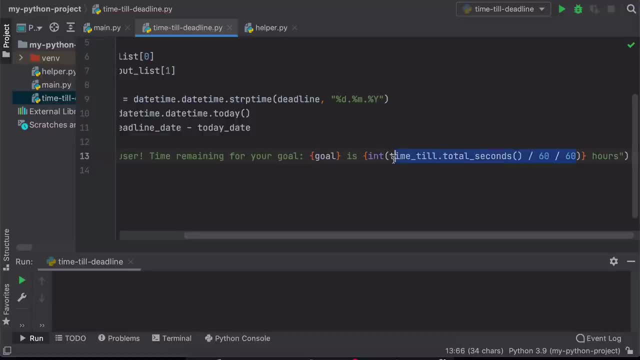 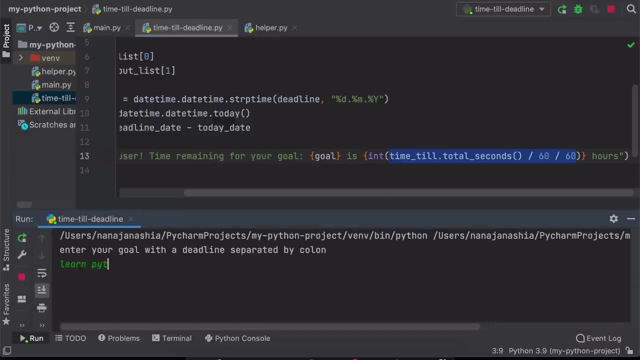 int function And we need this whole calculation here inside the int function And let's execute it again. Learn Python, and let's choose a date which is near, And there you go, We have a whole number: Fifty seven. again, cleaner output. 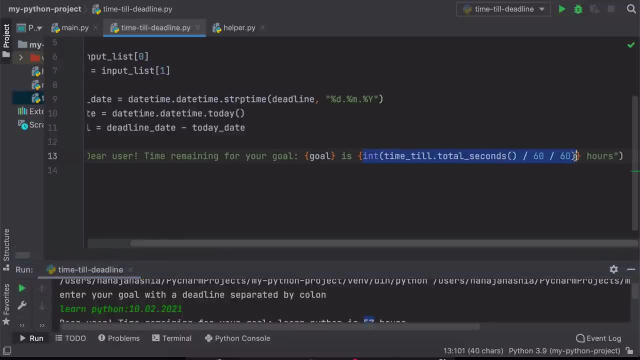 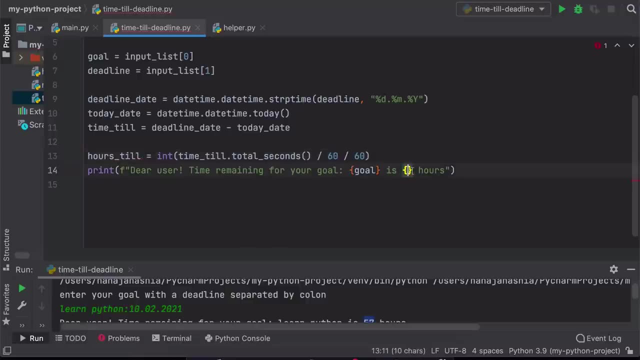 And as a code optimization we could take this whole thing out into a variable and call it hours till, To make our code a little bit cleaner. So now we have the whole program that takes user input and basically prints back to them how many hours are remaining till the deadline for. 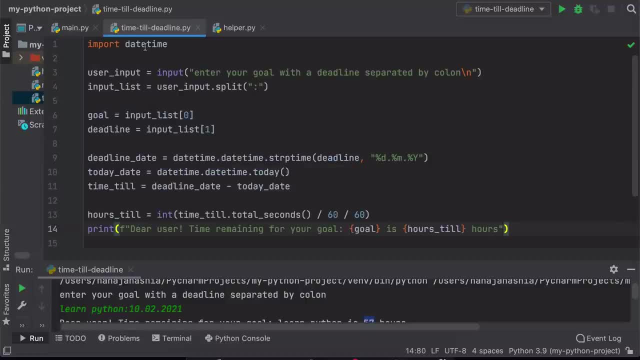 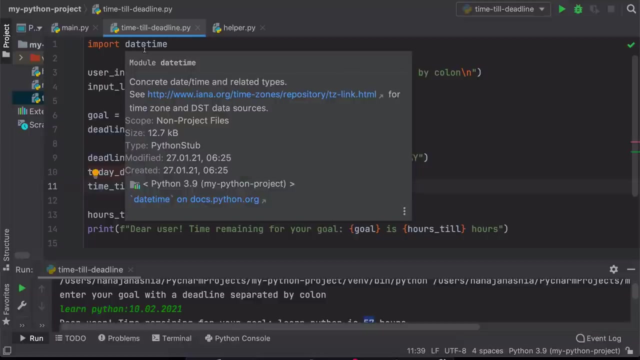 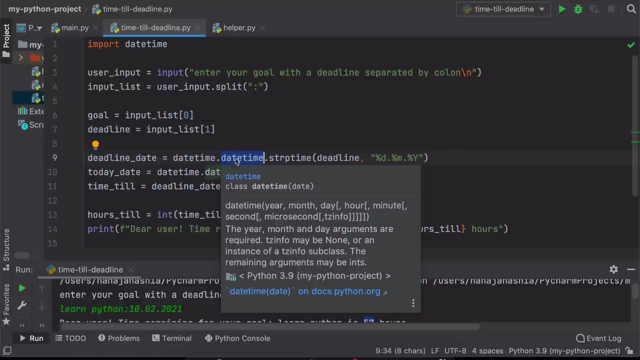 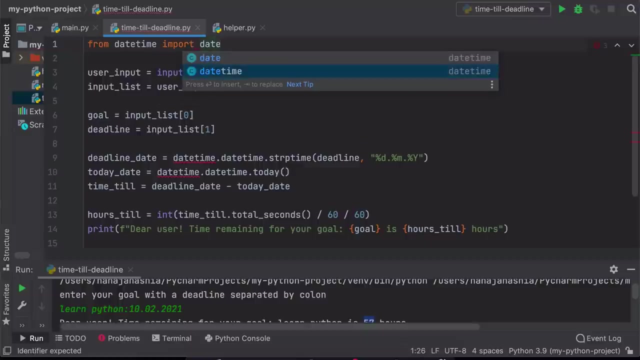 their goal And for this program we used a date time module built in day time module from Python, and we also learned a new data type, which is import date time definition, which is a class in this case. So now you don't need to use the module name. 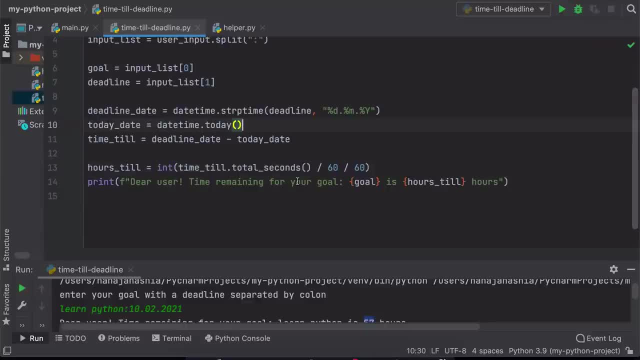 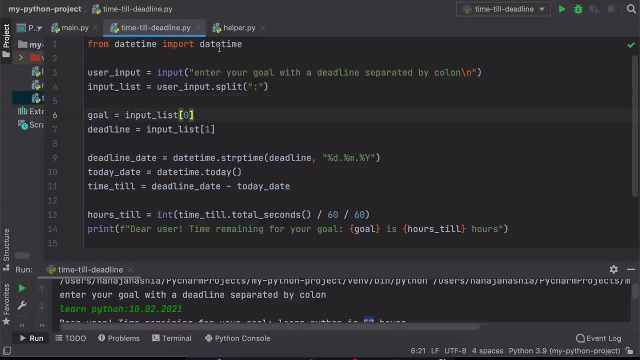 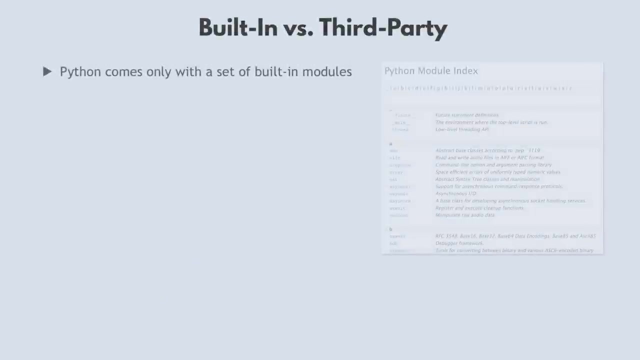 So let's get rid of those, And this could make the code cleaner as well as make the import more efficient, because we're not importing the whole module, even though we just need one definition from there. When you install Python, it comes with a set of modules. 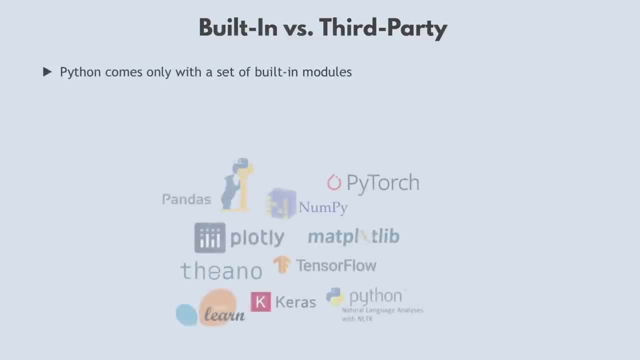 that are built in into Python. However, there are many more modules for other different use cases, like web development or data science and machine learning, et cetera, that are not part of that installation And these are basically external modules, not built in modules. 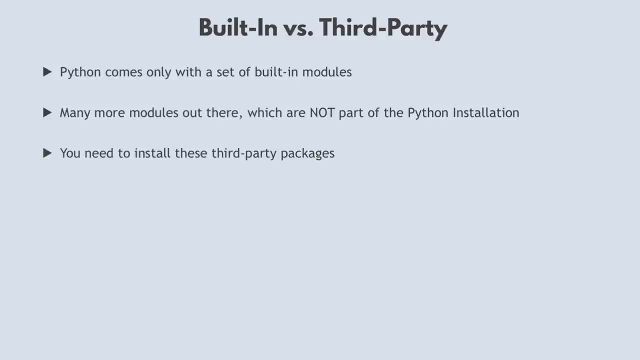 that you have to install as you need, And this makes sense because the built in modules are the ones that most of Python programs will probably need And depending On what specifically you are doing with your program, whether you are developing a web application or creating some, 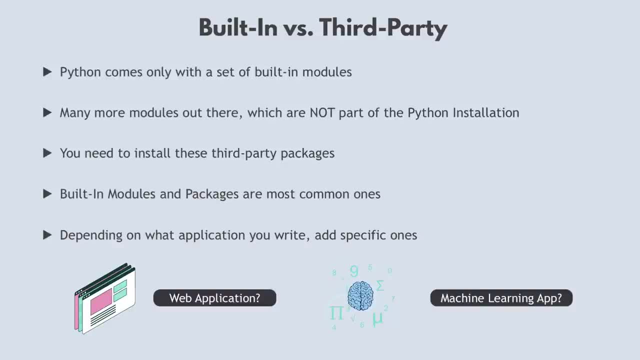 machine learning program. you can then add and install them as you need, And there are hundreds of such external modules for Python out there, And obviously it wouldn't be practical to have them all on your laptop when you're just going to use maybe a handful. 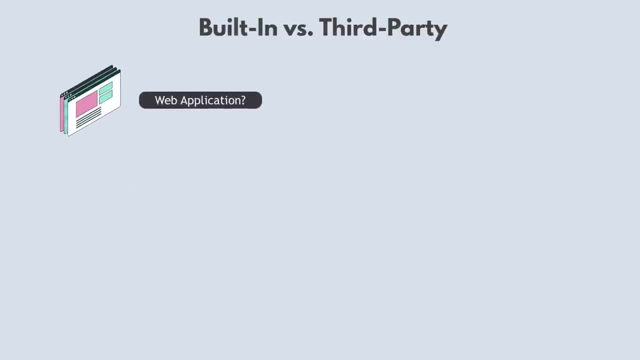 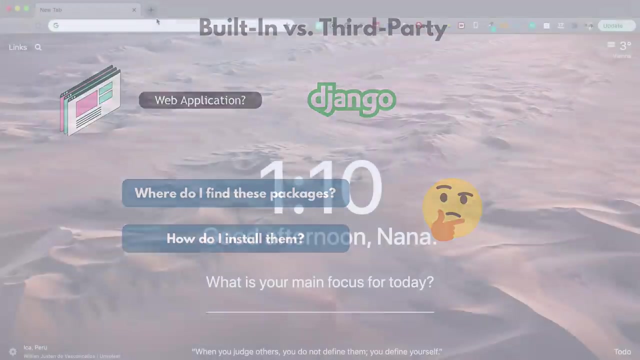 of them right now. if I need to install an additional module, for example Django for web development, Where do I find these modules and how do I install them? Python modules actually live in a module repository where you can find them, And that module repository is called Pipey. 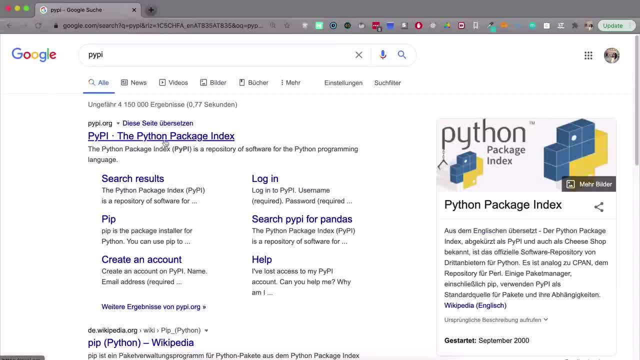 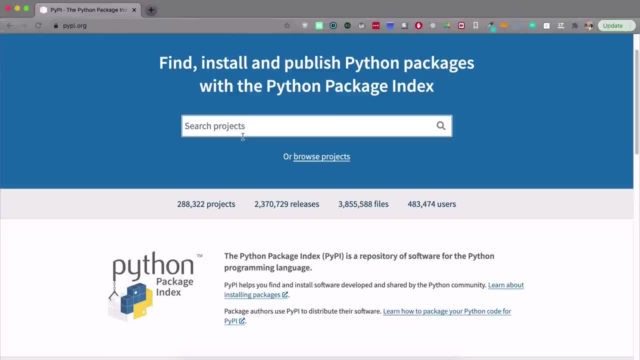 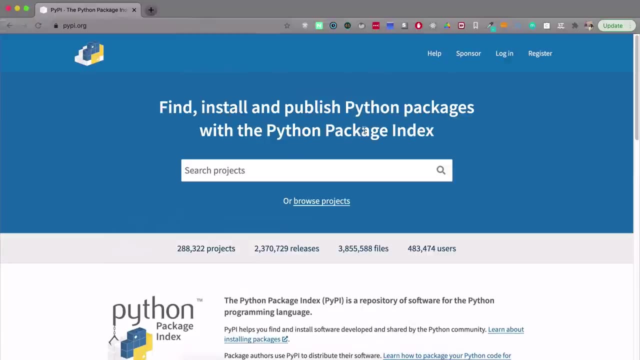 So if I look for Pipey right here, you see the Python package index. If I click inside, you can search for any module that you want to add or install additionally for your project And you can see that you can add modules to your application. 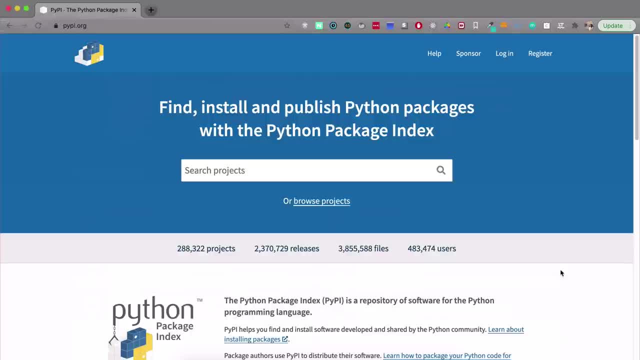 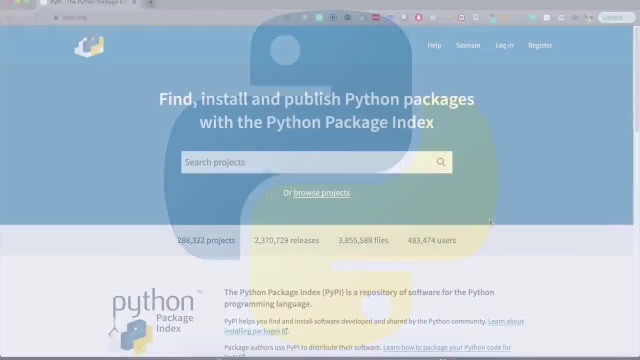 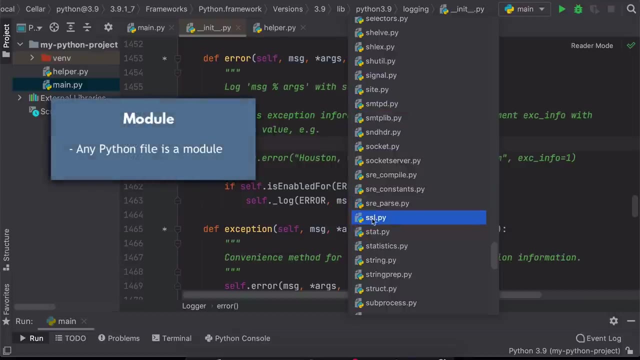 And here you see this word package everywhere instead of a module. So what is a package, or what is the difference between package and a module? To give you a simple comparison, module is basically a Python file, like this one right here that has a name of that file. 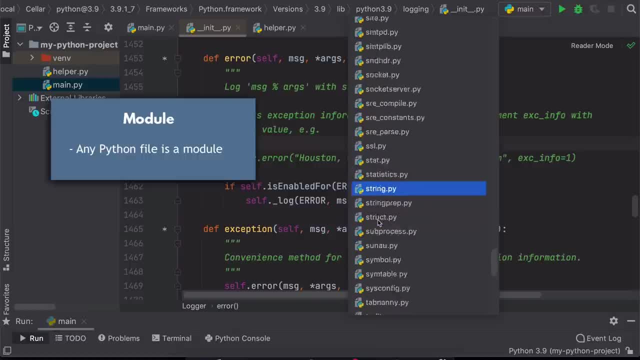 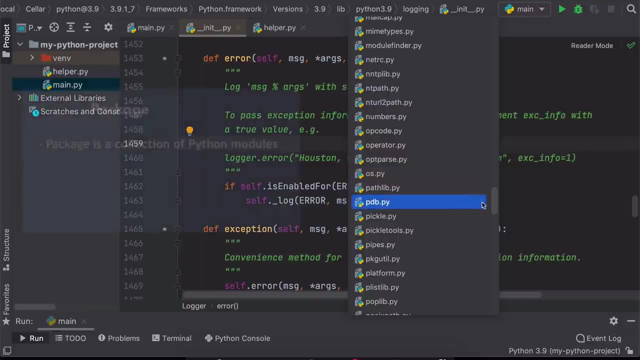 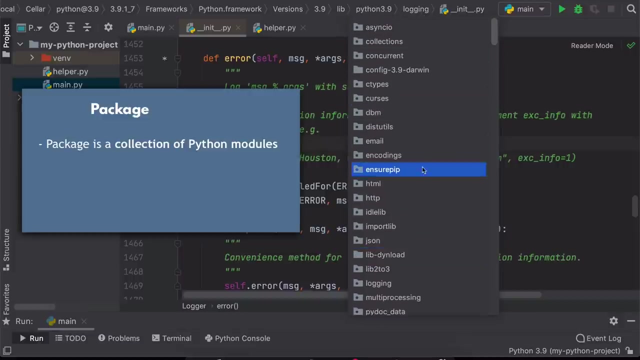 Right, So we have an SSL module, or the one that we used earlier. We have this OS module, Right? So module is one Python file that contains all these functions and variables that you can use. Package is a collection of modules, So if we scroll up and logging is actually one, or example. 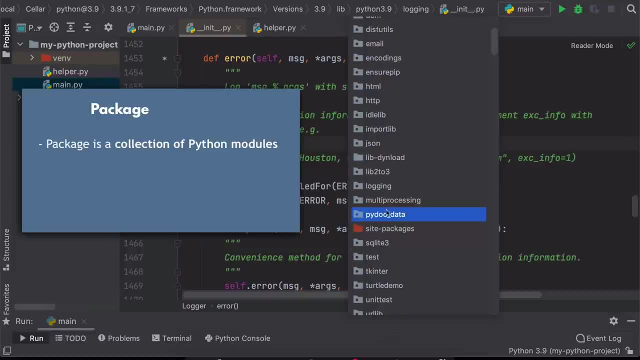 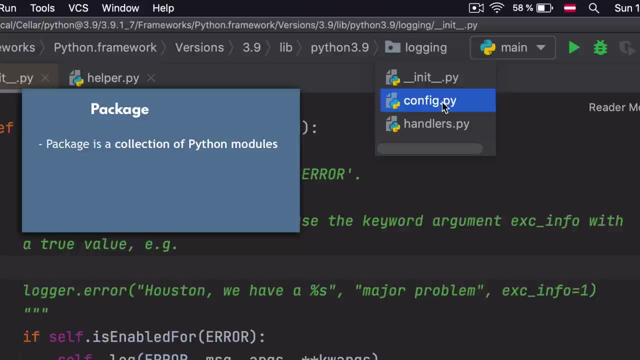 So these are actually packages. And again let's go to logging. So package basically contains multiple Python files And use it in the same way. You basically import the functions and definitions from the module And, as you see clearly, the difference is that package is. 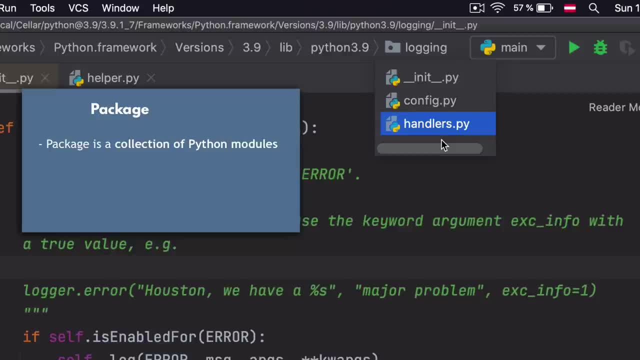 more structured. So, for example, the code is not available in just one single Python file, but is divided like this: In our case, we have two Python files and package always has this init Python file And this file basically differentiates a normal folder. 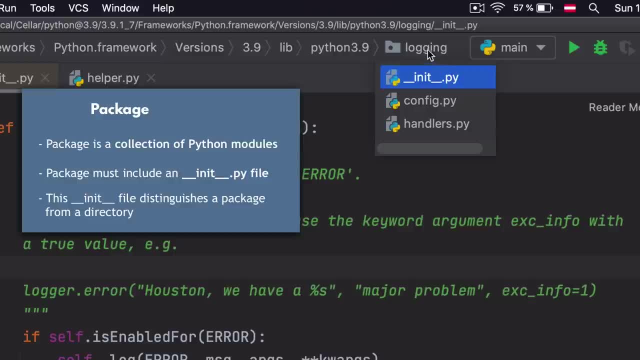 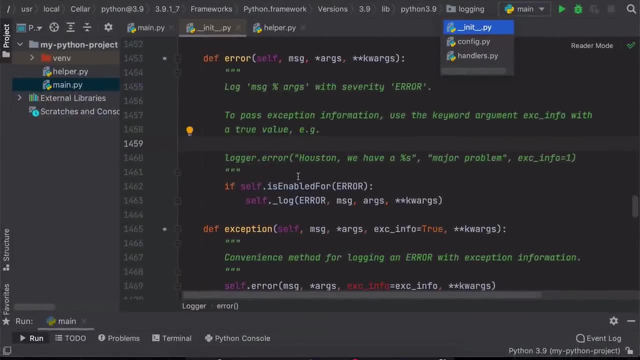 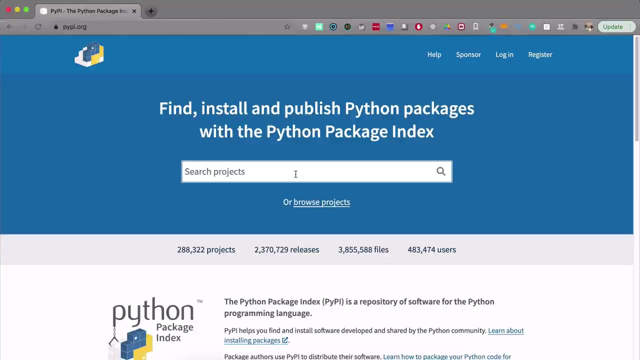 like we have Right here with a bunch of Python files from an actual package with Python files. So that's the difference between modules and packages, And many external modules, basically, that we want to use in our projects, are actually packages. So basically, package is a good way to define some hierarchy. 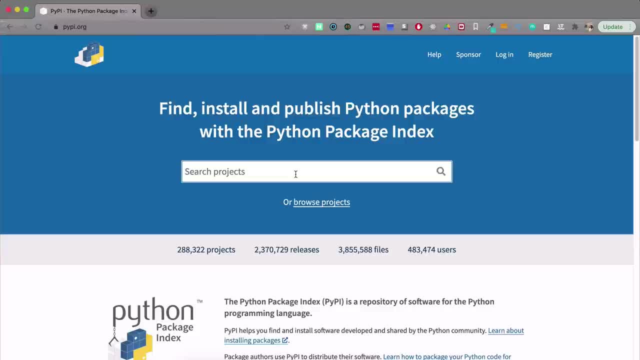 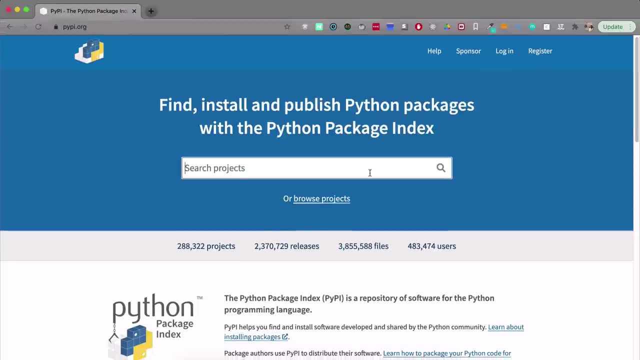 and structure for your modules and kind of group them together. So that's why you see package here as a name instead of module. So now that we know the difference, let's actually search for a package for our project. So, for example, if I type here Django, you see Django packages. 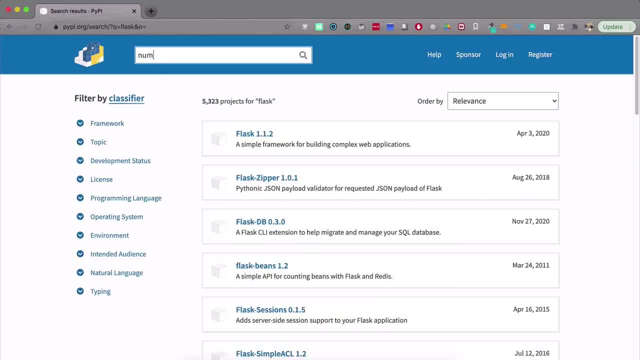 that we can use from here. We also have NumPy and so on. However, in programing, when working with and using these external packages, a typical example would be where you need to implement some logic. For example, you want to: 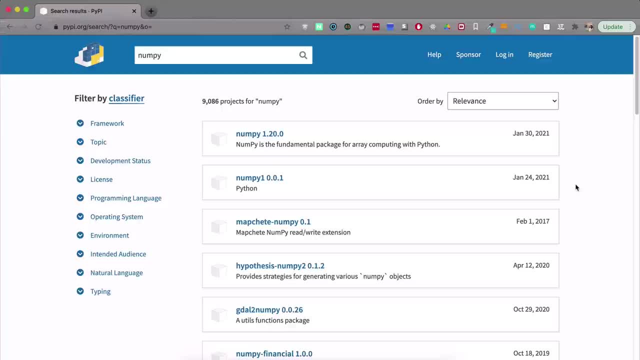 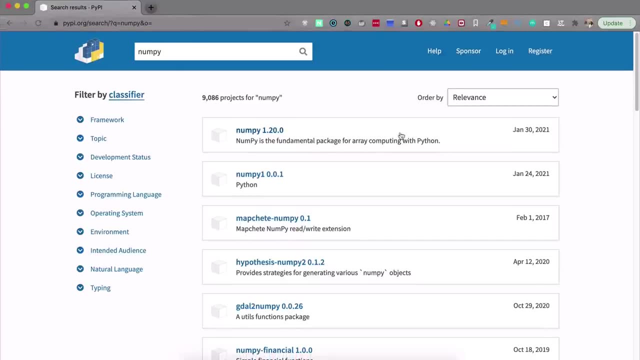 Right, A program that basically talks to AWS maybe, and you don't know exactly the name of that package, but you know what you're looking for. So in this case, instead of the exact name, you would actually type in here in the search projects box, a description of: 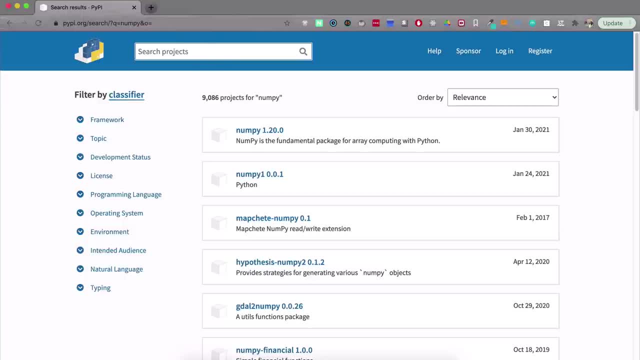 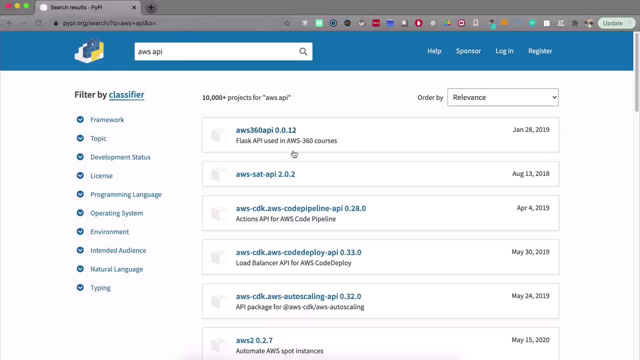 what you're looking for. So let's say, we're looking for an AWS API package, right? Something that will allow us to connect to the AWS API, And, as you see here, We get a list of different packages for that to choose from. 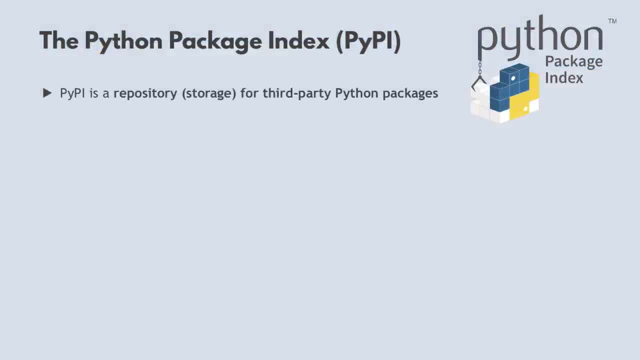 So basically, Pipey is a repository or storage for all of those modules and packages And people can also publish their own libraries like individual developers. for example, they can publish their own packages and modules there and make it available for other programmers to use. 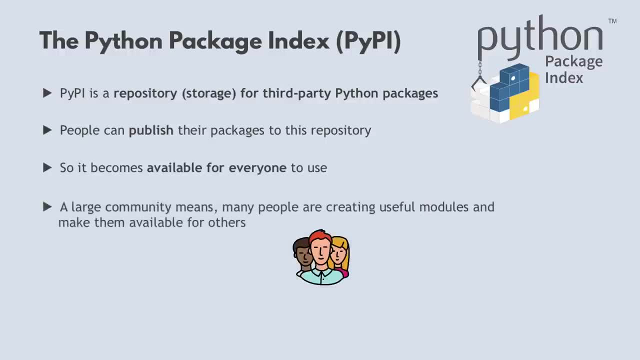 And that's one reason why a large community is so great for a programing language, because then you can make use of all these modules and packages that others in the community have developed. So for any kind of functionality you need in your application, you could imagine that there is a module or package that helps. 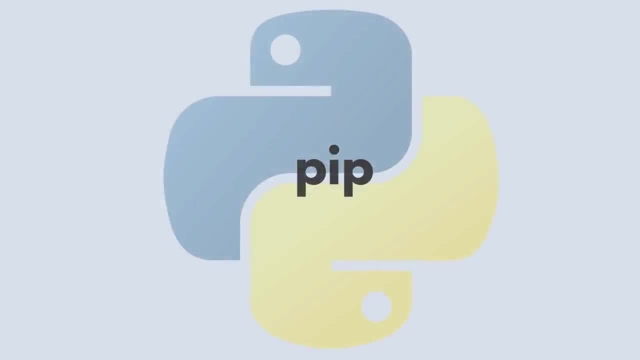 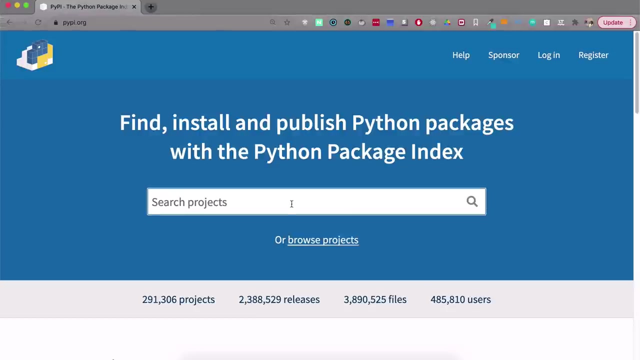 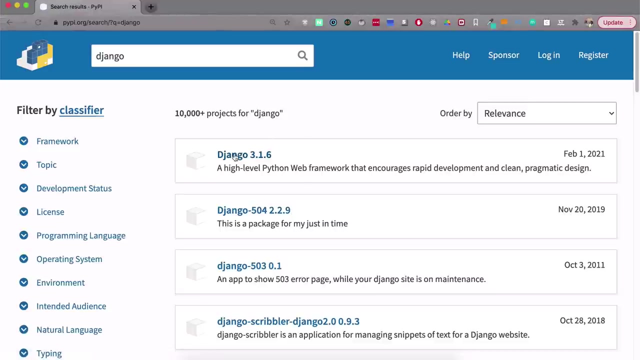 you do exactly that Now. let's say I need a Django package for my web application. So first I find the package and now I can actually check some of the documentation For that specific package. So if I click inside I see some description for the project. 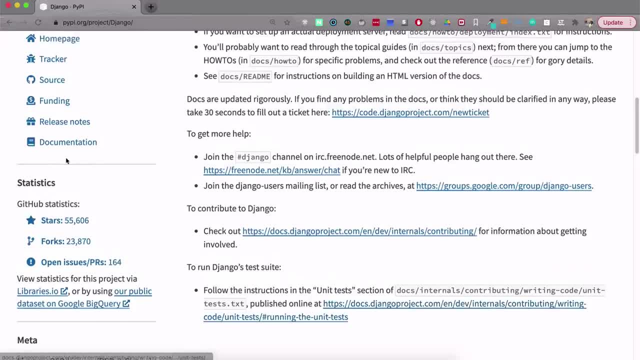 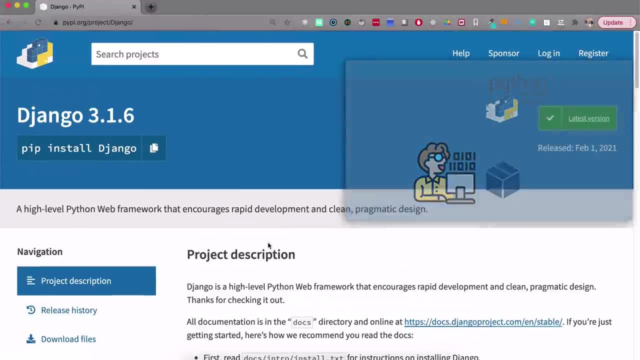 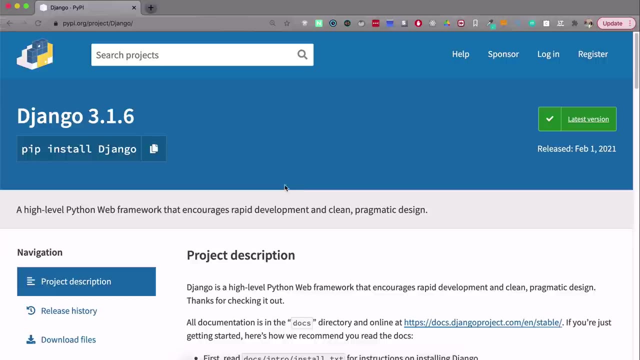 as well as documentation and some other links. Now the question is: how do I actually install this package locally so that I can use it in my project? In Python, we install packages using a package manager tool called PIP, and right here on top, below the package name. 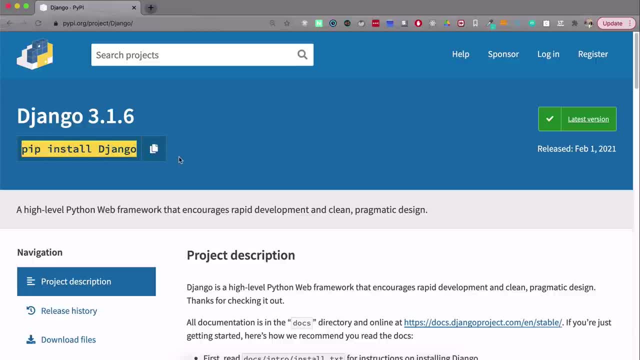 you actually see a command: PIP install Django. So this is actually a command that will install that package locally on my laptop. So we install packages in Python using this PIP command. So what is this command or where does it come from? 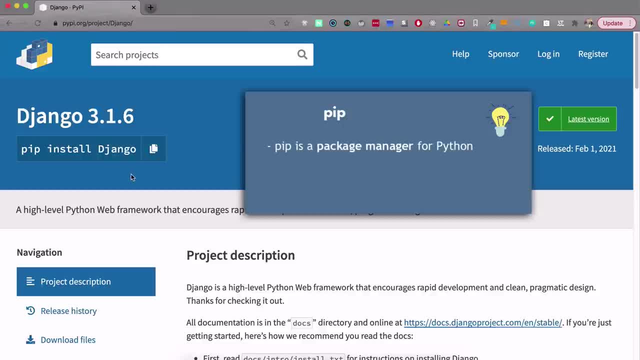 PIP is a package manager for Python And, if you know, any other programing language. basically, the concept is the same. Every programing language has its own package manager tool. for JavaScript It's NPM, for Java it's Maven or Gradle, and for Python. 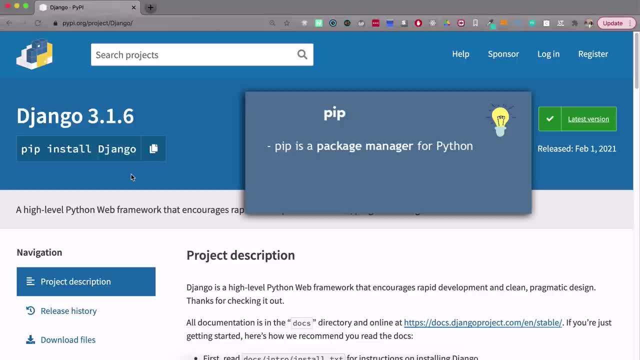 it is PIP And one of the main tasks or usages of a package manager tool is to install external packages or libraries, or also called dependencies, for your project. So if Python needs this Django package, basically it's the job of the package manager to install that package and make. 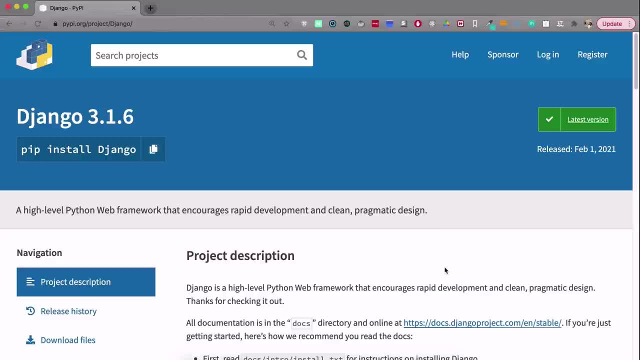 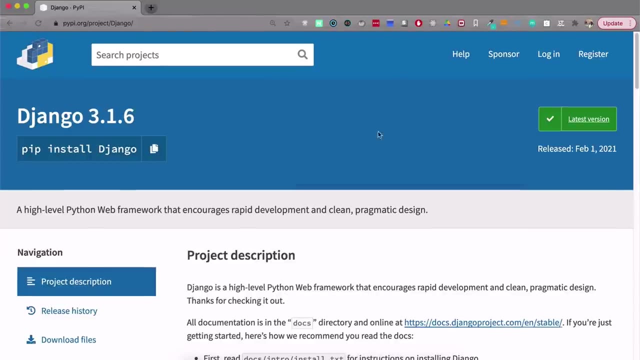 available. So if Python needs this Django package manager tool, it's the job of the package manager to install that package and make it available for Python. Now, where did this command come from? Do we have PIP command available? Well, in Python version three actually, PIP is packaged inside. 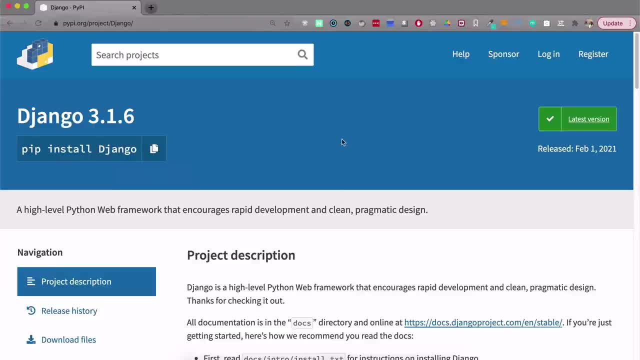 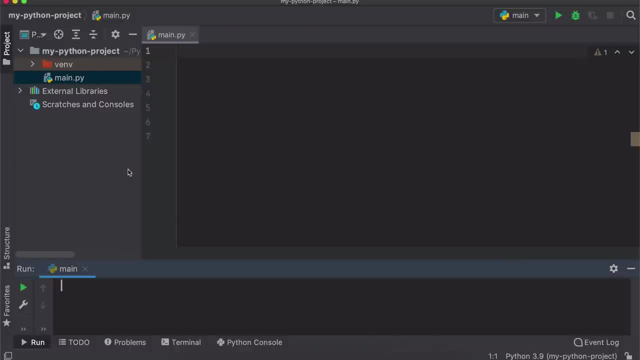 the Python. So when we installed the Python, we actually installed PIP as well. So basically, we're going to copy this command PIP, install Django, And we're going to execute it, Actually from the terminal of PyCharm. 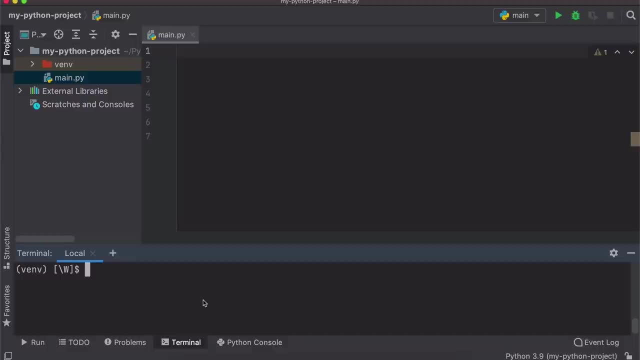 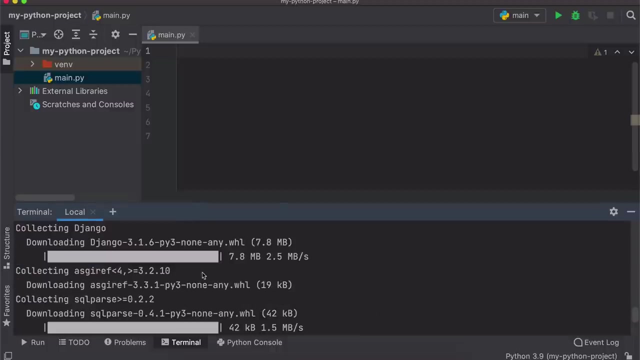 So this is actually pretty much the same terminal as you have outside like this. So we're going to execute this PIP install command directly in this PyCharm terminal. So I'm going to copy it here and do PIP install Django And you see it is downloading and successfully installed. 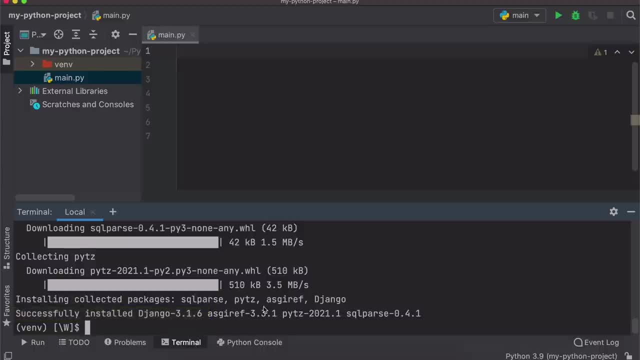 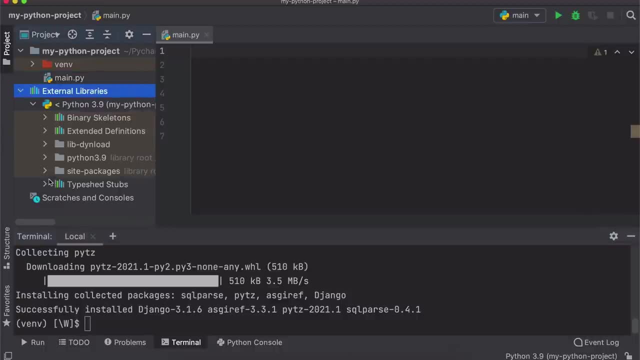 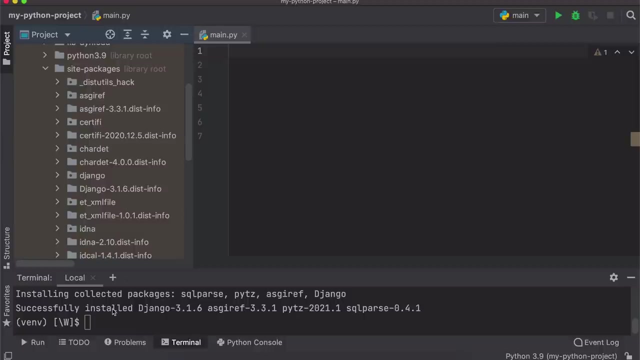 Django three, point one, point six, And we can actually see that package from our editor directly. if I expand this External libraries and site packages And scroll a bit down here, I have Django three, one, six version installed, so I see that the package is now. 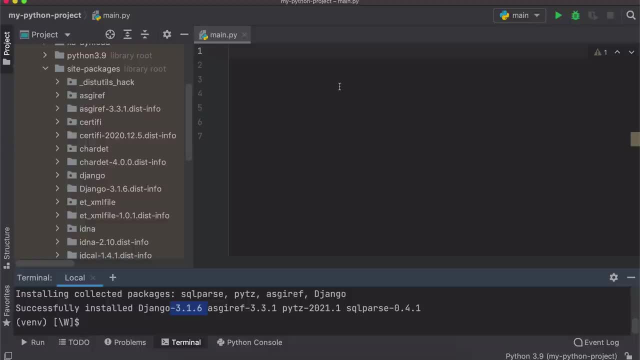 available in my project and to also test it in the code. I can do import and Django. and you see that PyCharm actually recognize that I have Django package locally So it gives me that package as a suggestion. so that will basically import the whole Django package so we can now use. 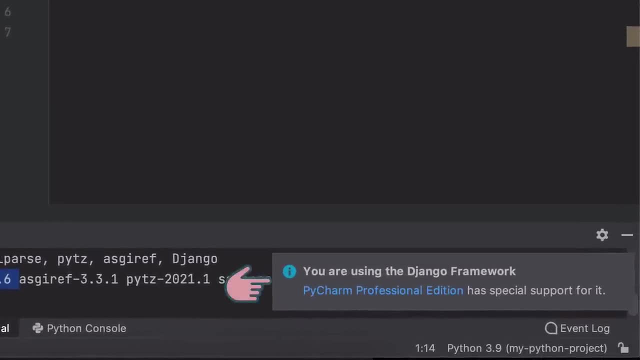 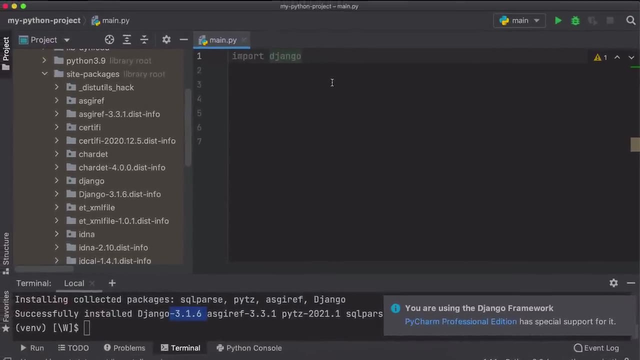 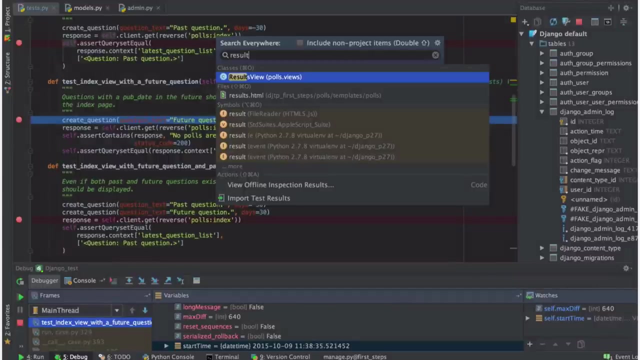 it in our application. Here you see PyCharm actually noticed you are using, or want to use Django web framework. As I mentioned in the beginning, the PyCharm professional edition has special support for different Python web frameworks, supporting you with syntax highlighting. 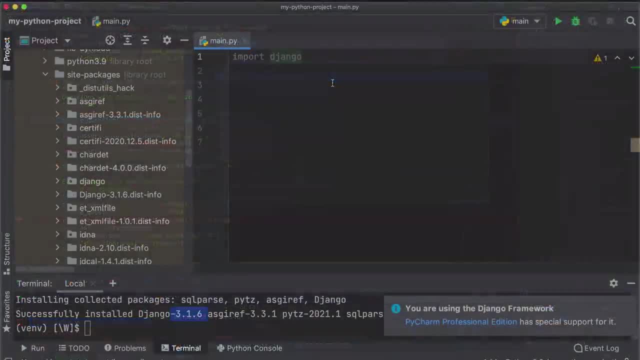 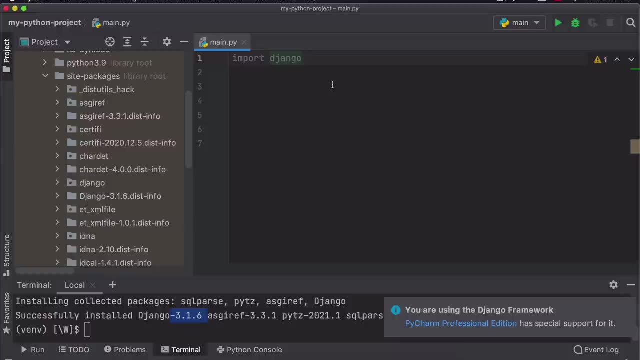 suggestions, database integration and so on. So again, if you want to try it out for free for three months, just use my code in the video description. in the same way as we install the package, we can also uninstall packages using PIP, and let's also actually demonstrate that PIP uninstall. 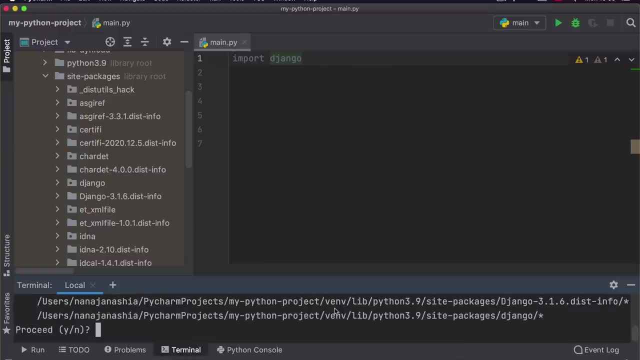 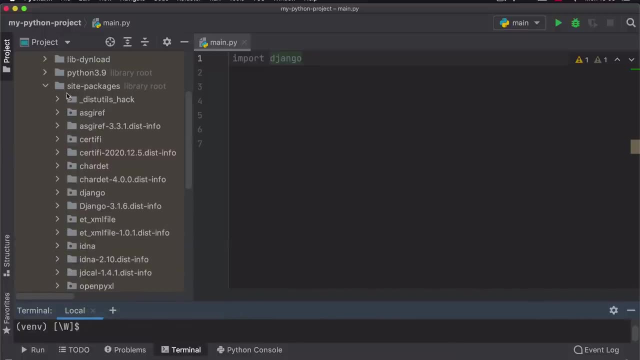 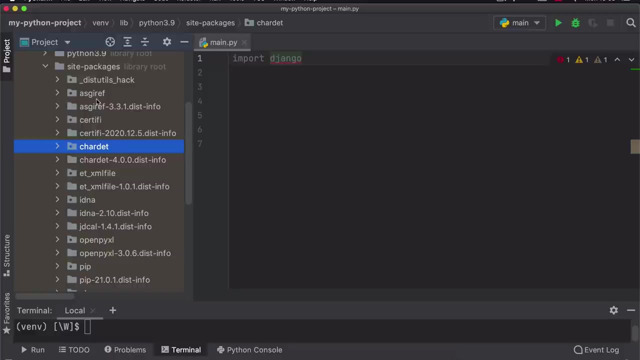 Django and let's confirm that- successfully uninstalled Django. Now, If in the site packages I click inside, you see that Django packages are gone. so this site packages folder got updated, Django was removed and you also see that in the code editor. 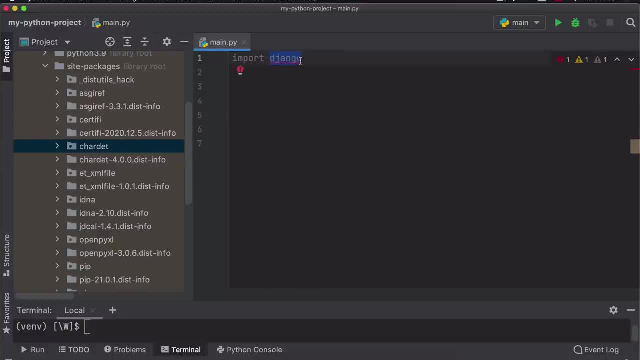 Now I have this red line under Django because PyCharm cannot find a module called Django And also, if I do this, obviously it won't give me any auto suggestion for that. So that's how you can use PIP to install. 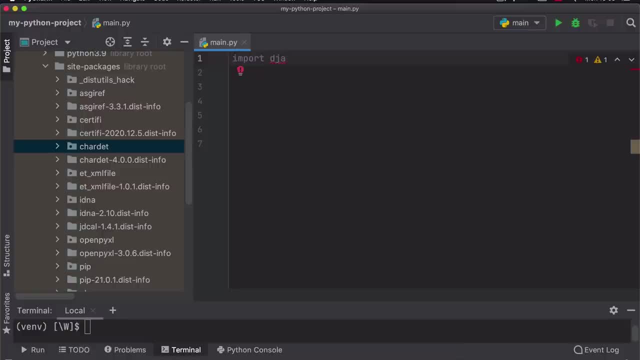 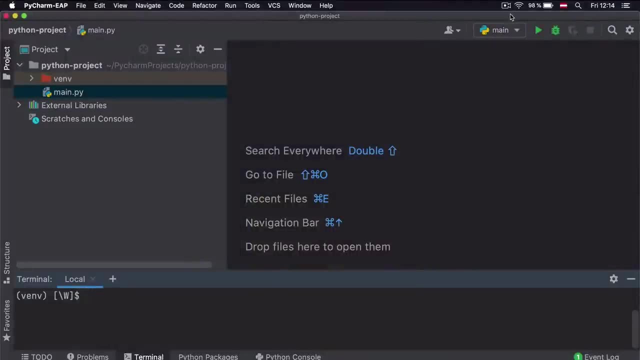 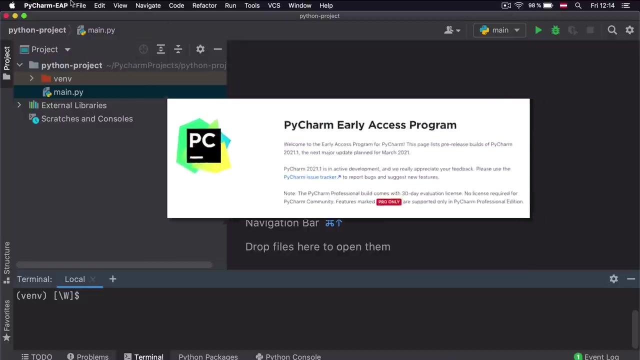 Packages and also to uninstall packages for your application. Now here I want to show you another cool alternative to installing and uninstalling packages directly in the PyCharm ID, and this is actually a feature in the latest PyCharm release, and for this I need to switch to an early access. 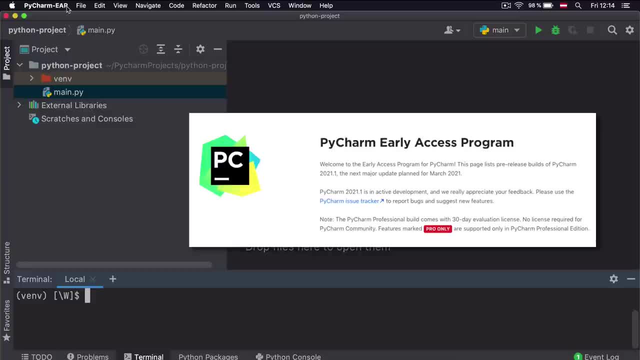 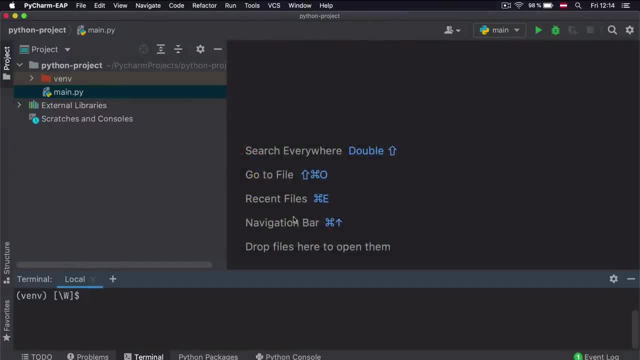 PyCharm version. So you see, here says PyCharm EAP Early access to show you the feature. However, when you watch the tutorial it probably will already be included in the latest official PyCharm version, so you should have that already. 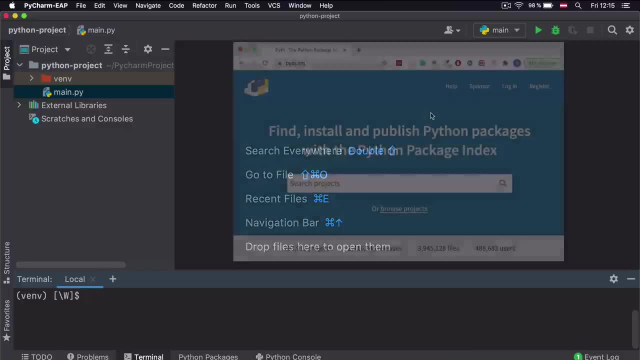 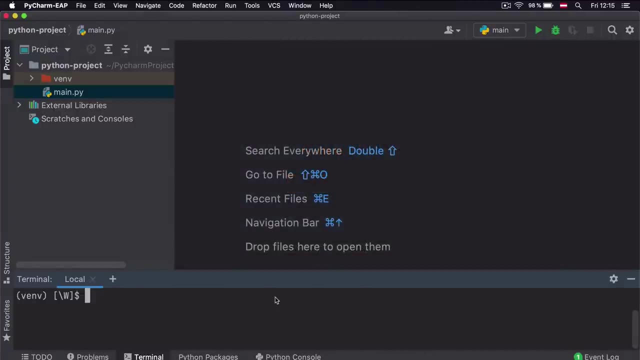 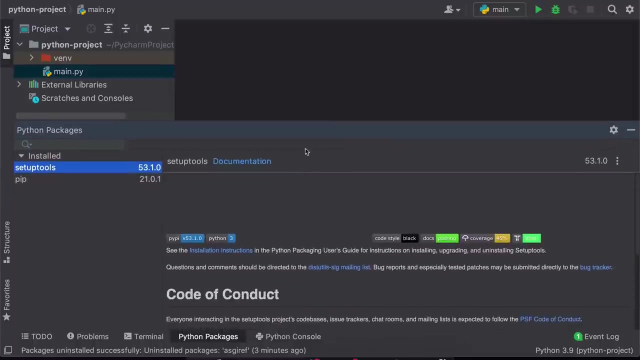 So instead of us basically finding this package in PyPy and then executing PIP install commands right here, what you can do is, down here you have another tab called Python packages, So if we click inside, this is a place where you have everything that you need to know about the package. the package. 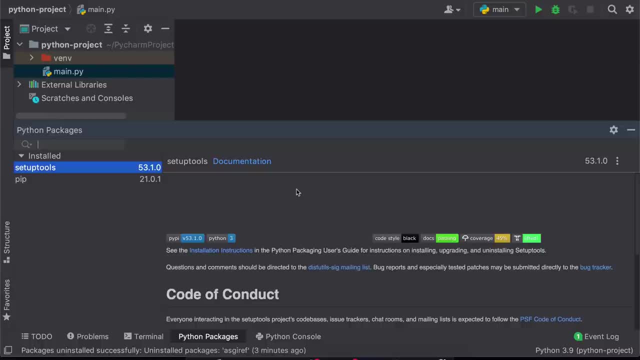 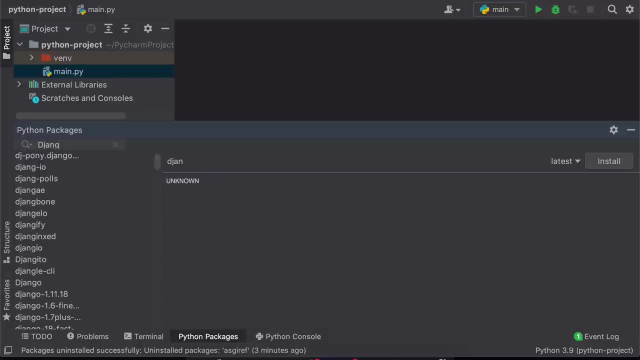 search and all these features basically in one place. So, for example, in order to install Django, we can just search for Django right here, And you see that when I type in the first couple of letters I already get suggestions. So this is a list of all the packages that start with this. 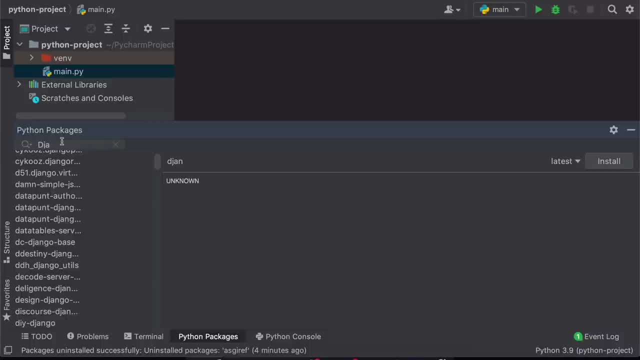 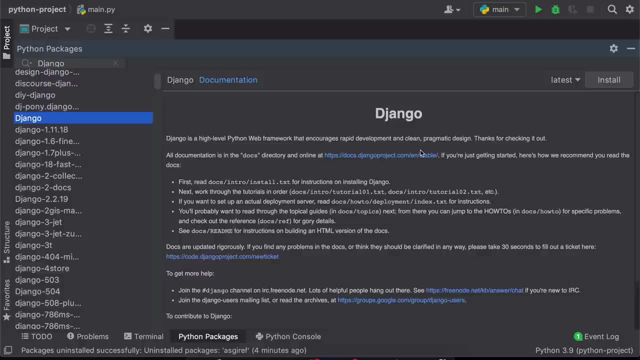 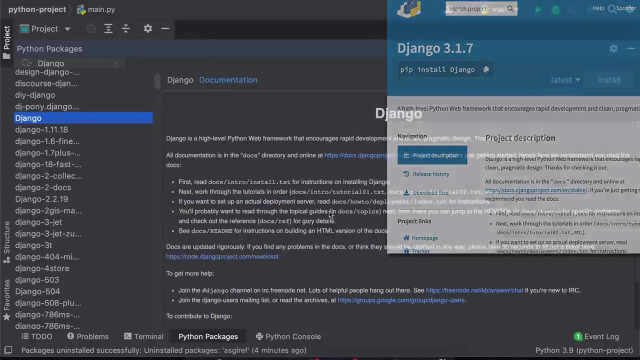 name that are actually available in PyPy. So let's type in Django and we see that right here. Yeah, Yeah, And on the right you see the documentation of the package that you would actually see in Pipey UI. So you have that in place as well. 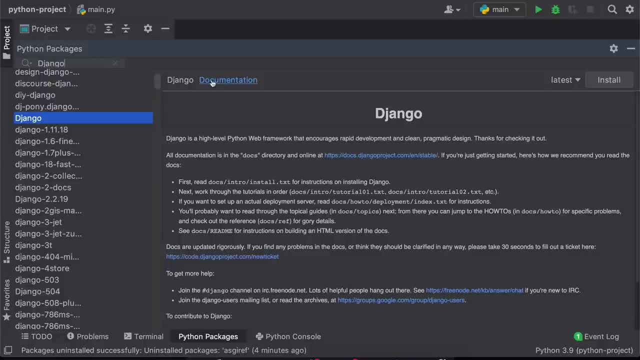 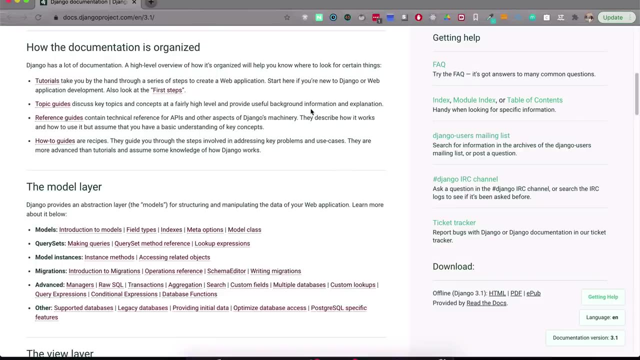 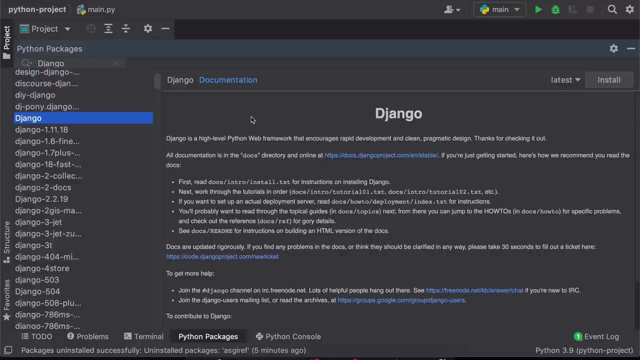 And in addition to that, what they added is the documentation link. So this is actually the package- how to guide- and the full documentation with examples, etc. So very convenient way to basically get all the information about the package, search the package and then to install the package. we can choose the version here. 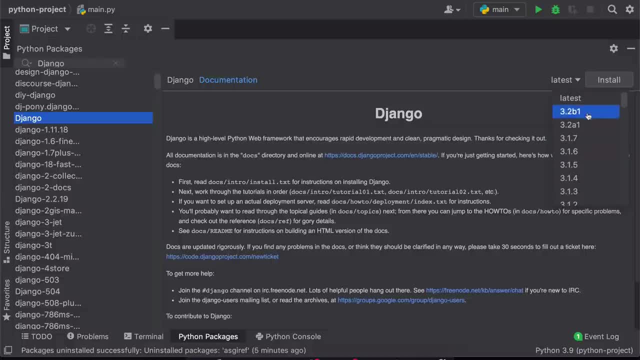 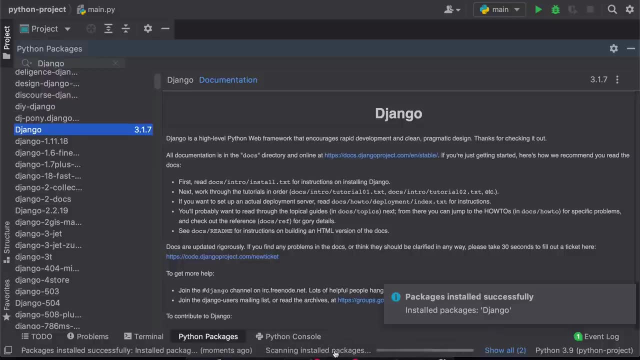 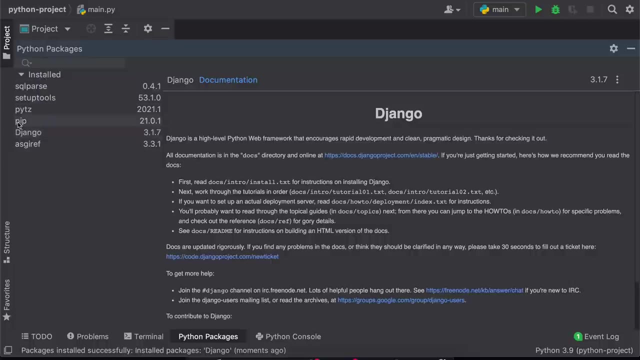 So either you can leave the latest or basically select the specific version And then, once you have selected that, you can just click install And here you see installing package. and there you go. So now in installed view here. So we just had PIP and set up tools, these two things installed. 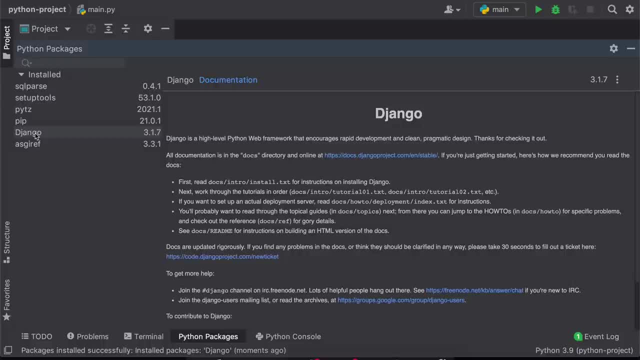 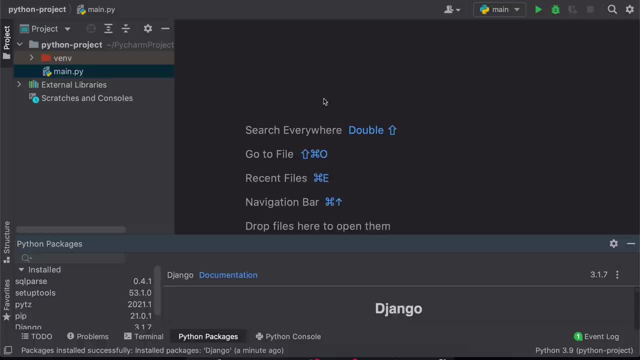 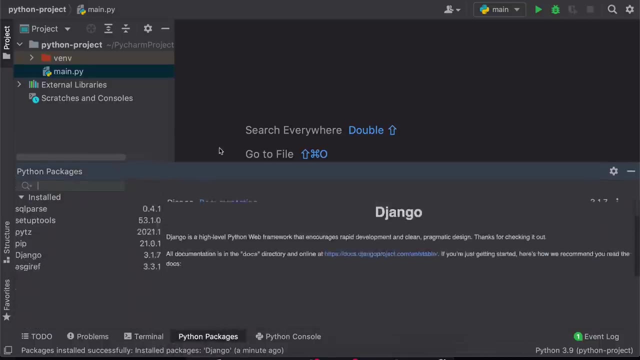 And right here we have now Django in the install Packages list. And again, while you are now using the installed package or library in your code and basically want to look up some examples or you want to check some documentation, right, you go back to the package. 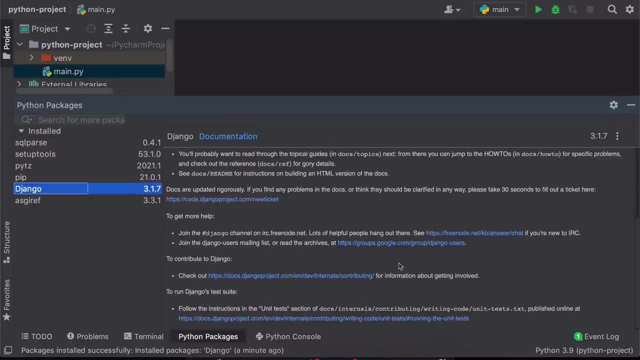 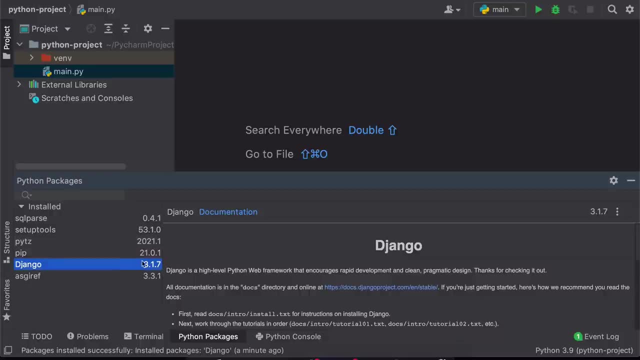 click inside and you have links to documentation and the package information as well, And also just by looking at this list you know which versions of which packages you have installed. So I think it's really cool Way to manage all your packages- to install packages. 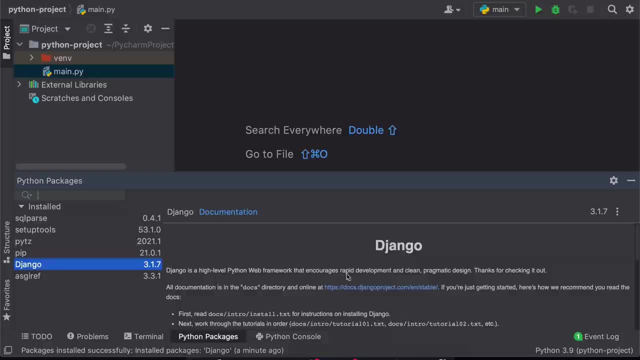 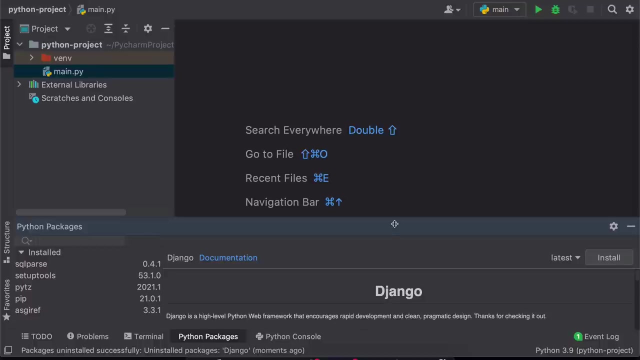 And, for example, if you want to uninstall packages from your project, then again just clicking to that specific package right here, you can just delete it and it will be removed from your application Like this, and no Django anymore here. So a very cool addition to PyCharm, because this will be very convenient to work with. 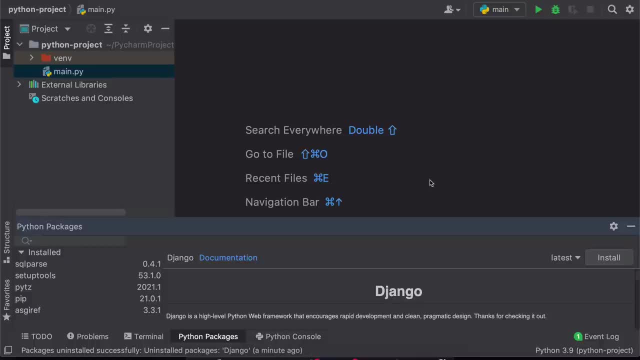 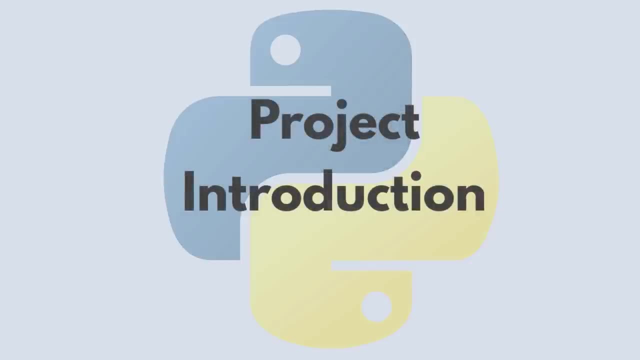 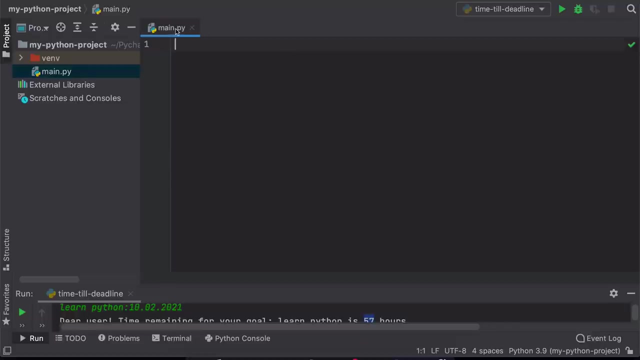 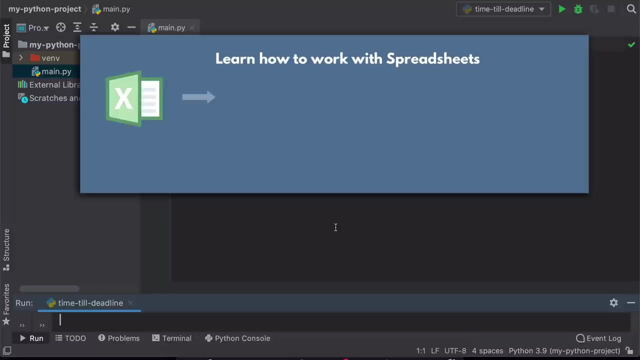 Packages. So now I will switch back to my other editor again and continue from there. So basically I have just cleaned up my Python project. We have this mainpy, which is empty, And we're going to write an application that will read a spreadsheet file from our local file system. 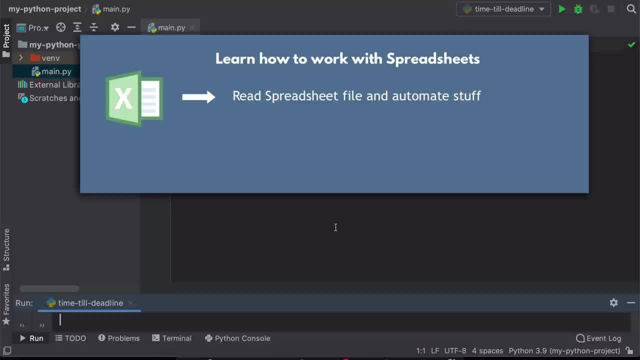 It will read some information from that spreadsheet file and do something too When it's logged in. where can we do that? Fantastic, Yay, Great with the data, And this could be a very useful use case if you're working with. 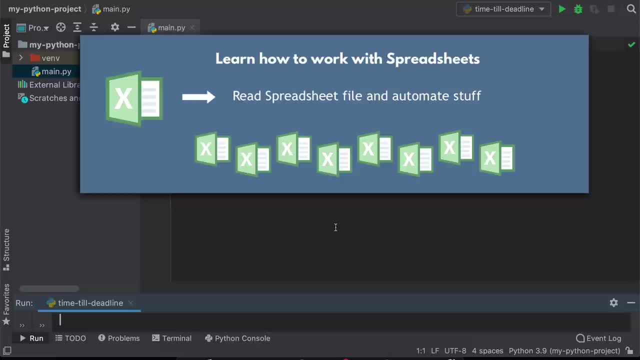 lots of files and you want to do some data processing in those files and you don't want to do that manually by automating or writing a program in Python that basically can do anything in a file or across multiple files. So let's see exactly what we are going to be doing. 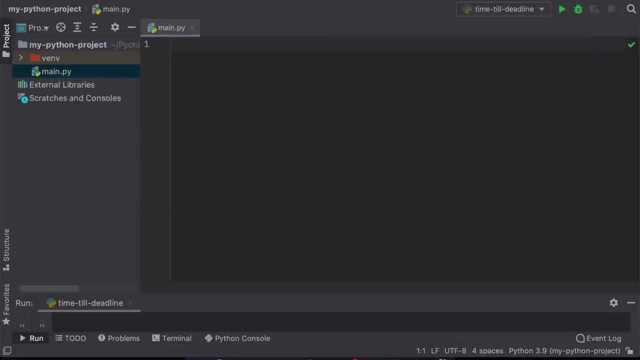 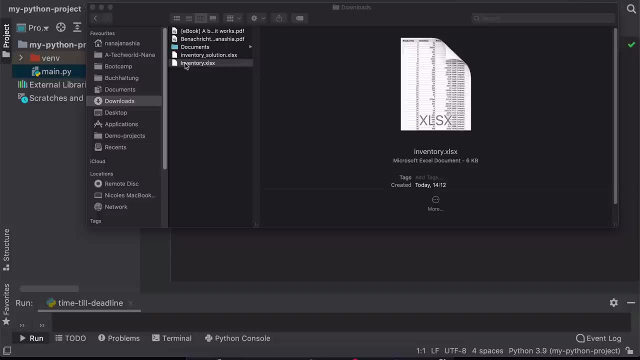 with this program. So, first of all, we're going to have an input file, a spreadsheet file that we're going to be working with, and that spreadsheet will look like this: It's called inventory. That's how it's going to look like. 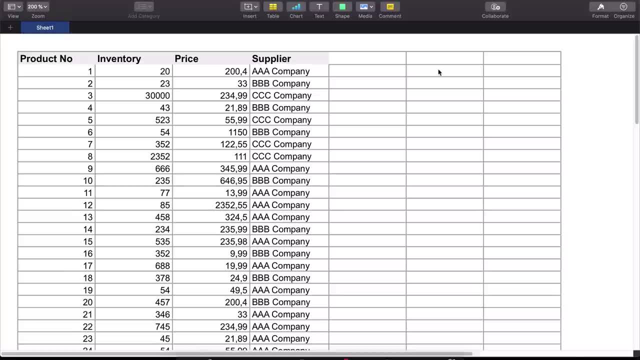 So basically, this file simulates something that many companies would have and employees of their company would be working with. So we have this list of product numbers, inventory for each product, price for the product and a supplier. So this could be an example file from a company that 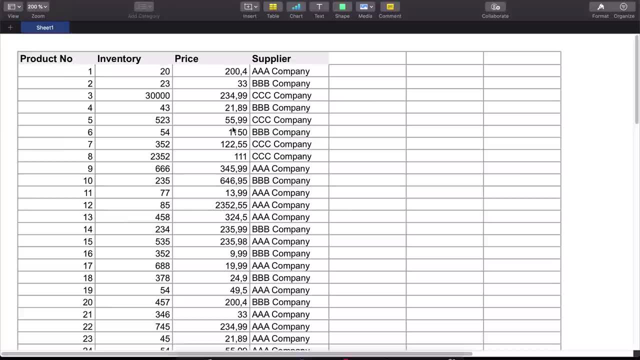 is basically dealing with selling or buying products. So what we're going to do is we're going to read the information from this file and we're going to do something with that information. First, we're going to write logic that calculates how many products we have per supplier. 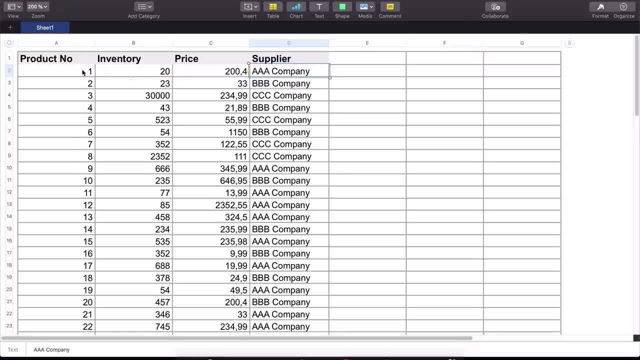 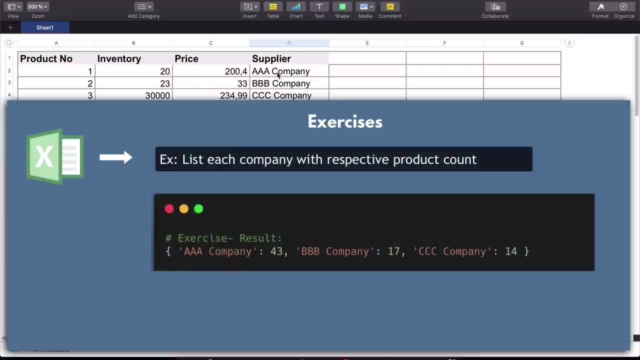 So we have three supplier companies here and per supplier we're going to calculate number of products from that specific company And, as a result, we're going to list the company, So all three companies With their respective number of products. then we're going. 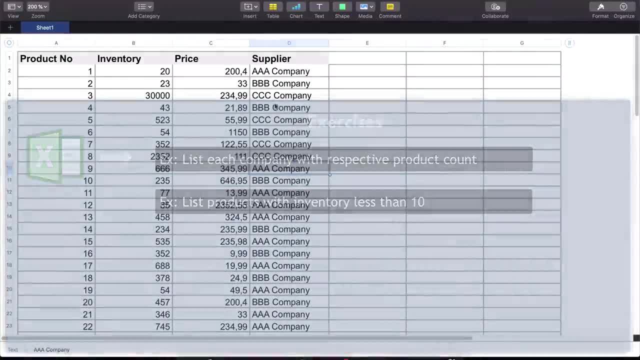 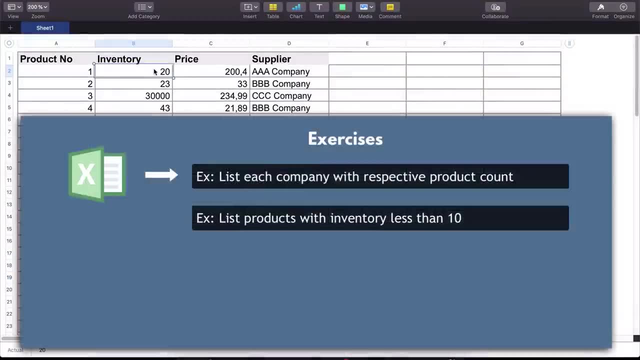 to write another logic that lists inventory products that have inventory which is less than 10.. So basically those ones. The third exercise is going to be to list each company with their respective total inventory value And finally, in the last exercise, we will calculate. 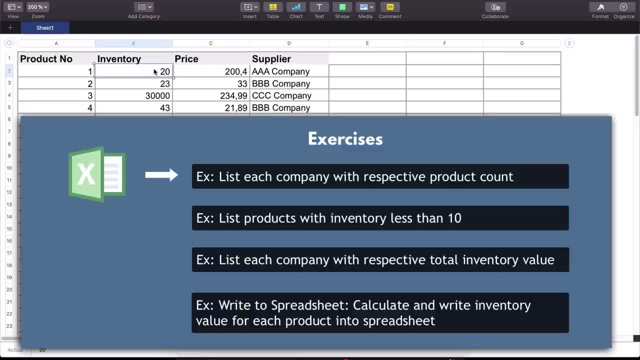 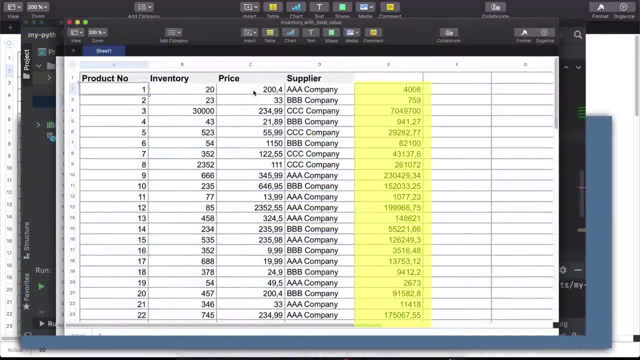 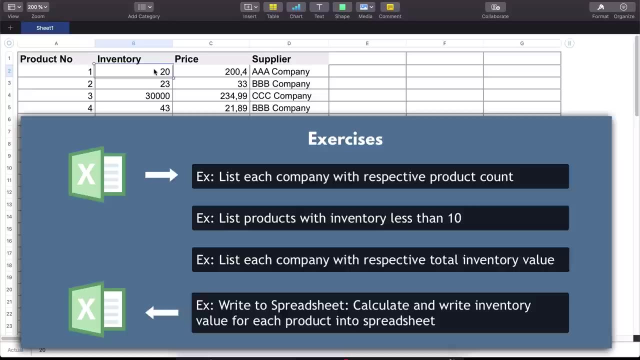 the inventory value for each product, So product amount times price, and we're going to write that value to an additional column in the spreadsheet And after that we're going to save that updated spreadsheet file programmatically using Python. So we're going to see how to update a file and then save it. 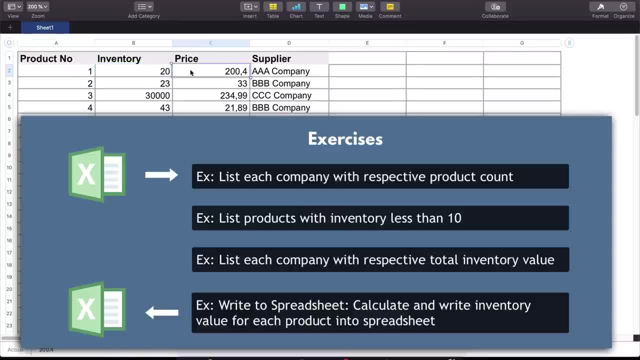 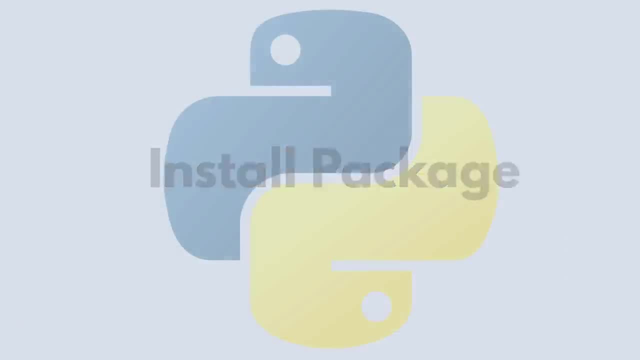 programmatically in Python. If any of this sounds a little bit too complicated for you, then just bear with me. I'm going to explain everything step by step, and it's going to become much clearer when we actually start writing the logic. So the first thing what I'm going to do is I'm going to 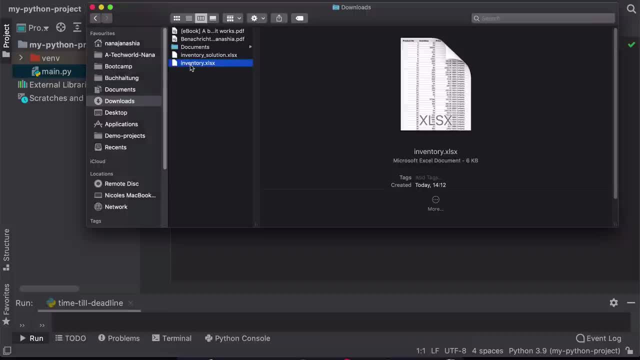 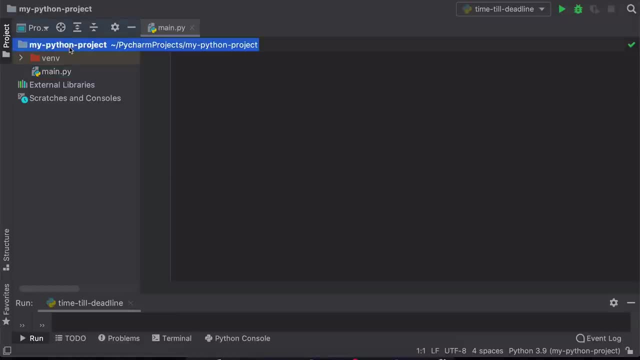 take this file that I have in the downloads folder and I'm actually going to move that into my project, so I'm going to copy that and I'm going to drop it in here so that we have the file right in our project and so we can basically just 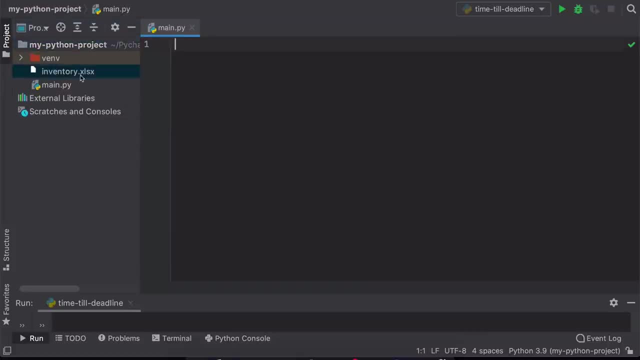 read it easily and OK. and here is our inventory file, So that's taken Care of. So, obviously, what we want to do now is read that file. So basically, let our Python program read the contents of that file right here, because we want to write some logic based. 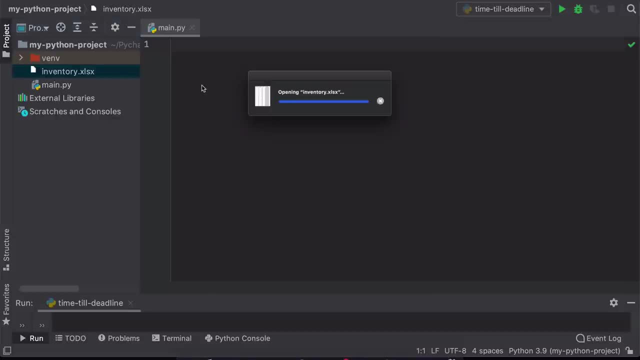 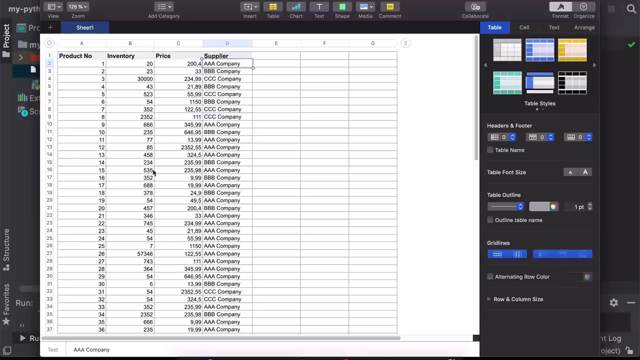 on the values that are in this inventory file. Right, We want to calculate stuff, We want to list some stuff, and so on. So, basically, we want to work with these values And in order to do that, we need to read all of these. 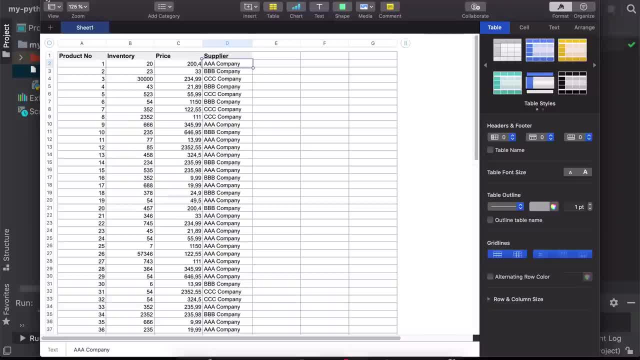 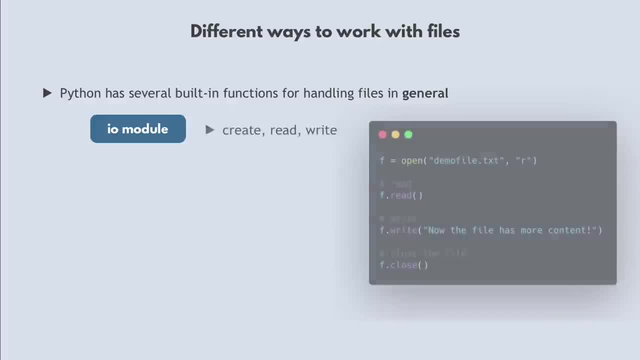 values into our program so that we have them available. So how do we Now? there is actually a built in module in Python that allows you to work with files generally. Right, It's not specific for a spreadsheet or for any other file type. 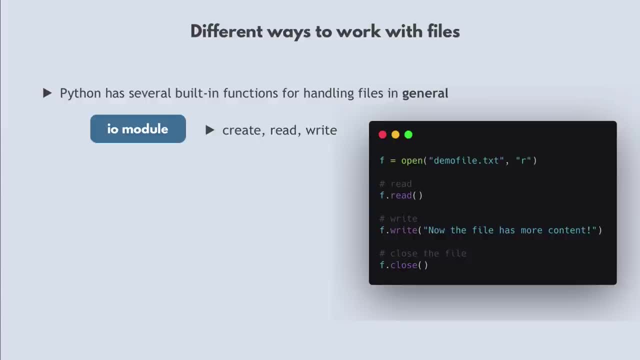 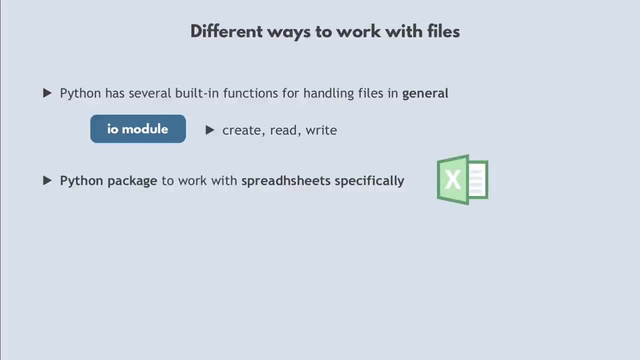 It's for different types of files generally. However, there is an external package that allows you to work with spreadsheets specifically, And the obvious advantage is that that external module that allows you to work with spreadsheets, or was created to work with spreadsheets specifically, has much more. 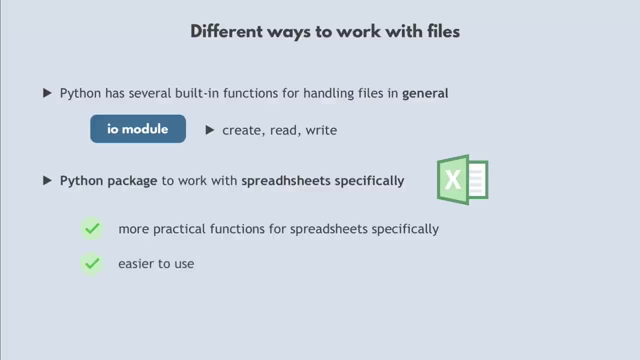 functions and is much easier to use if you are working with spreadsheets, compared to this built in file module. So that's one of the cases where you may have multiple ways of actually implementing some functionality for application, And then you have to make this decision of maybe finding a 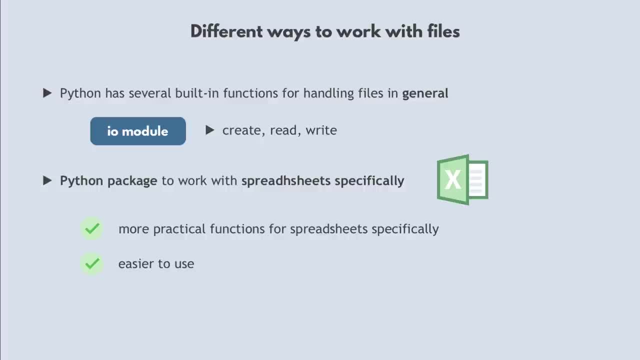 better package or better module which is available externally, that will make it easier for you to implement that functionality. So that's what we are going to do for our project: We're going to choose the package that is actually made for working with spreadsheets. 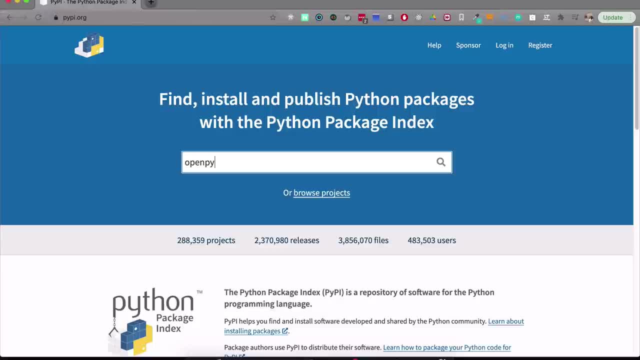 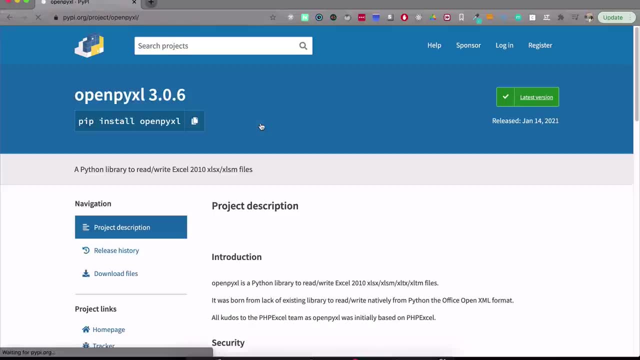 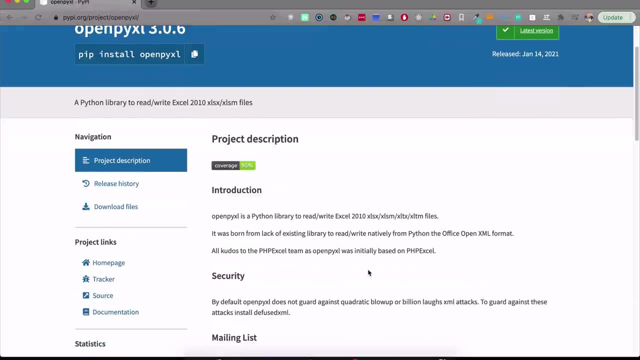 We're going to use that one and it's called Open Pie XL And if I search for it, this is the package that we're looking for And if I click inside, basically we have some information about this package. So here we see a description. 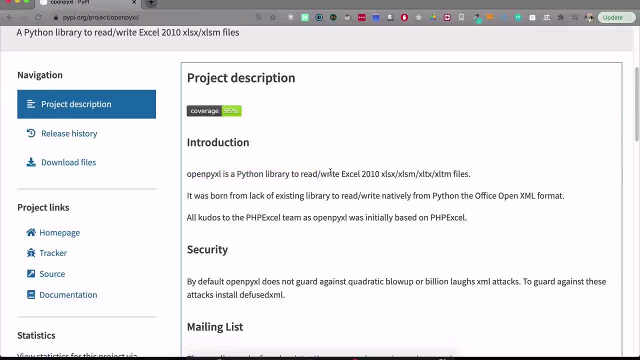 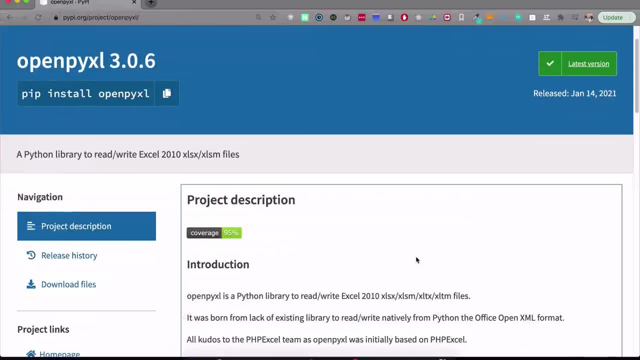 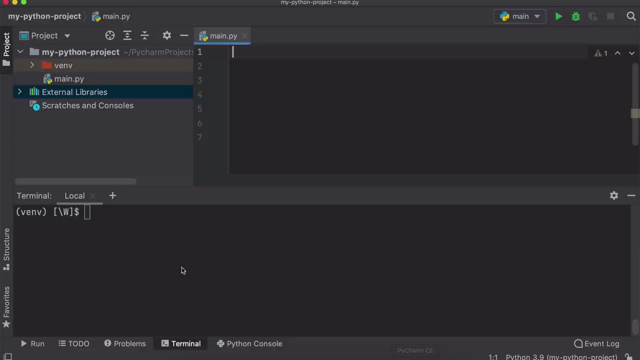 It's actually make this bigger description library to read and write Excel files with all of these formats. So this is the library that we're going to be using in the same way as we did before. We're going to copy that command and execute it from pie. 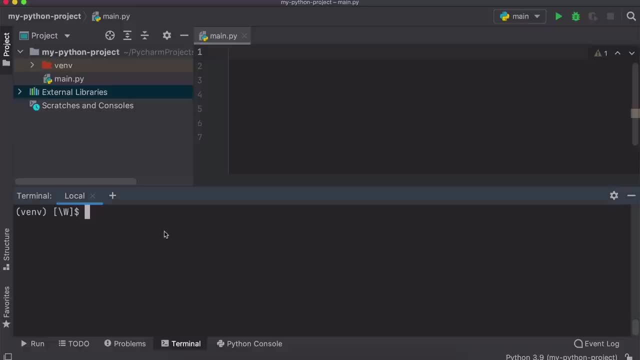 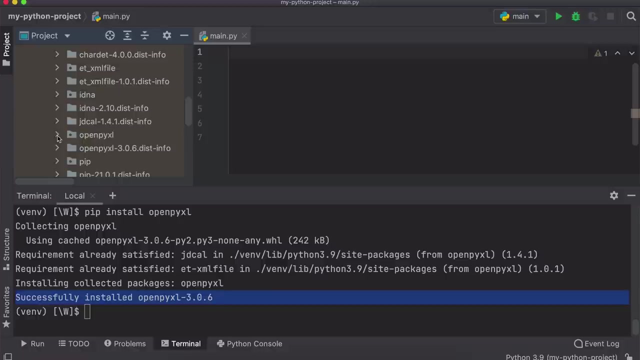 charms integrated terminal. So from here I'm going to execute this command and install our module And, as you see, successfully installed Open Pie XL and this is the version of the Module that we installed and in external libraries, site packages, you should be able to see our Open Pie XL package. 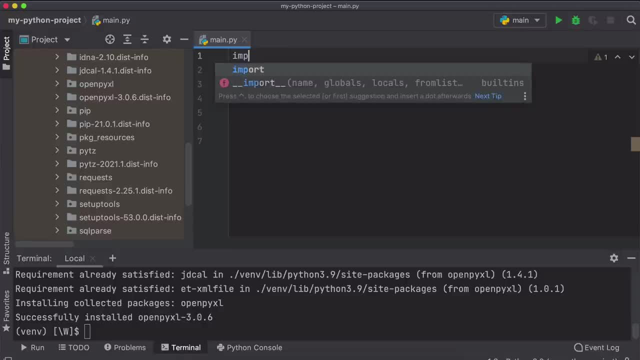 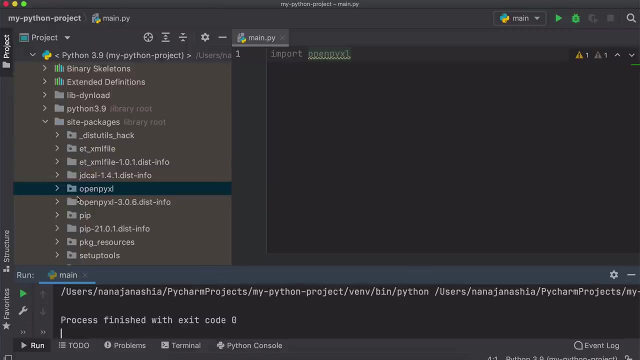 and now, because the package is available locally, I can do import and open pie XL. again. I get a suggestion from pie charm because the module is there and now we are able to use that package for our application. And one small note here, if you're wondering why there are: 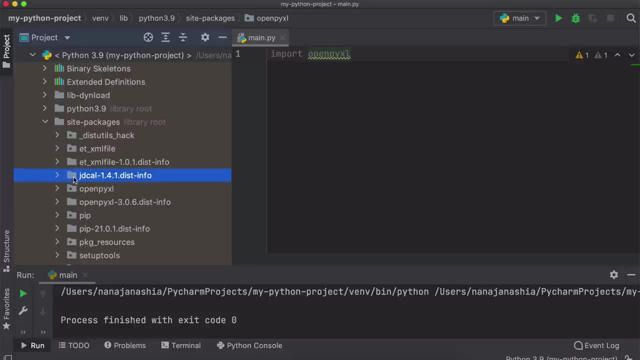 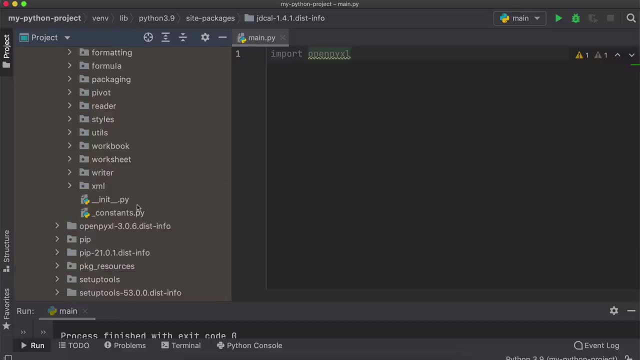 some Packages with basically a dot inside and some without. these are the packages that we install, Python packages, and we know that because there is this init Python file inside. and the ones without the dot they're just folders with bunch of files inside, but they're not Python packages, so to say. 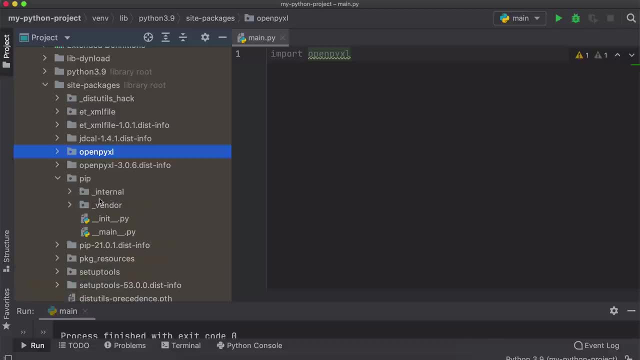 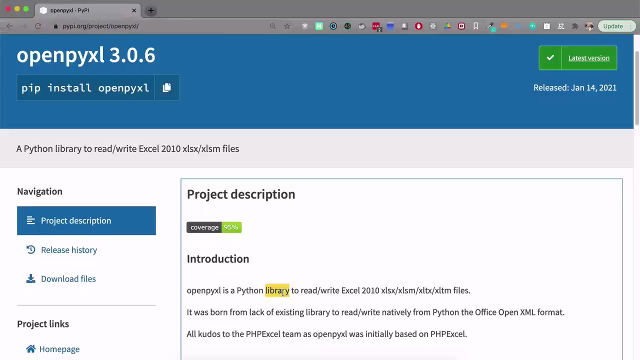 And inside some of those packages we see other packages as well, with their own init file. So basically, Hierarchy of multiple packages. and this point I'm going to say that the word library basically describes package that includes multiple other packages. so basically, which has a hierarchy. 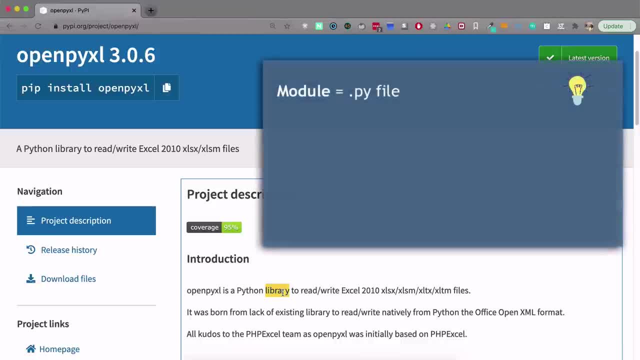 of packages. So we have module, which is basically just one Python file that we can use in our project. Then we have package, which is a hierarchy of multiple modules with an init Python file inside, And then we have library, Which is basically multiple packages together in a hierarchy. 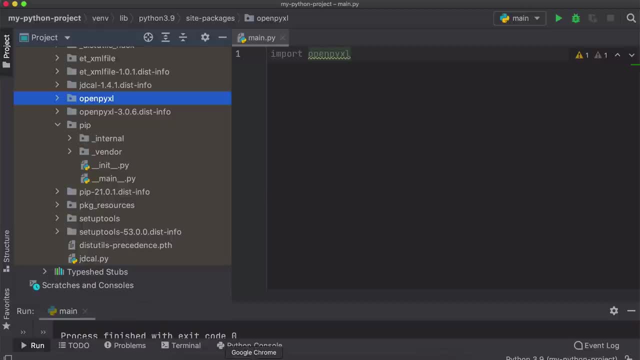 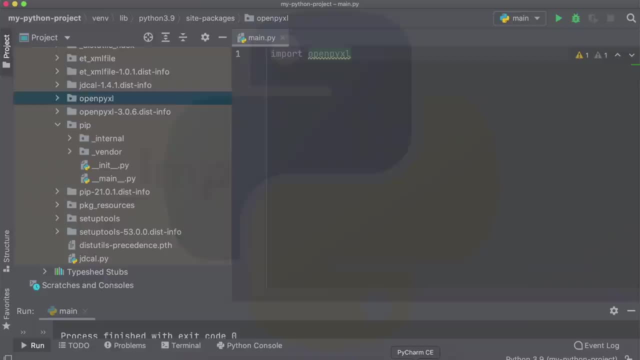 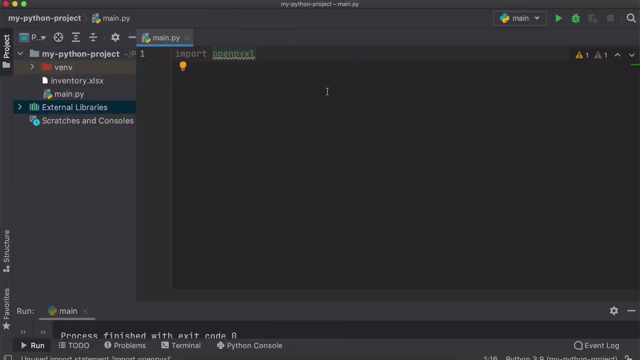 just like we see right here. So note the difference So you don't get confused when you see library package and module, especially if used interchangeably. Great. So now we have our module in place, so let's use it now to read our spreadsheet file and again, you basically have to. 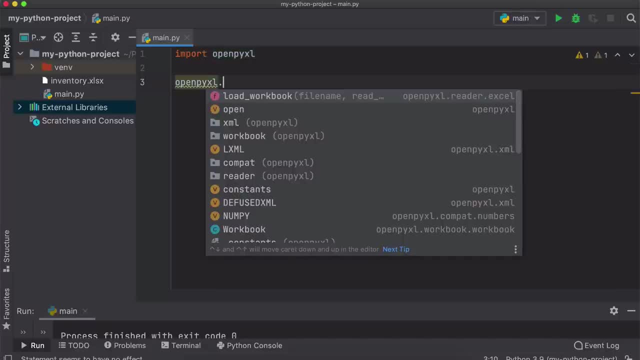 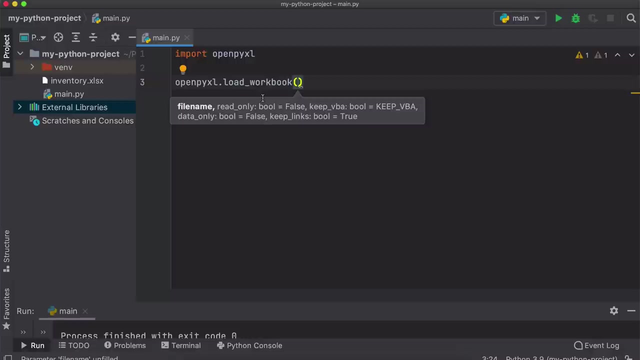 know the function names to do that. if you don't, you can do dot and get suggestions and load. workbook is actually the function that we need in order to read our spreadsheet file. So I'm going to choose this function and obviously we need to tell this function which file it should read. 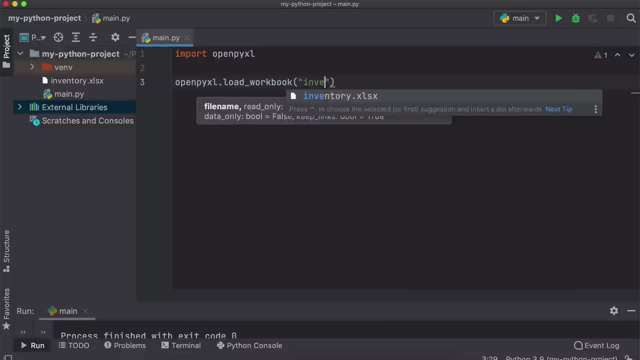 So as a parameter we're going to say: please load inventory file. and we even get a suggestion because we have this inventory file here and there you go. Now this function will load the workbook and all its content, And later we obviously want to do something with that content. 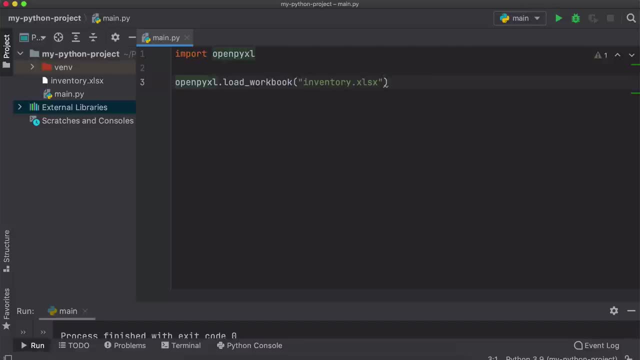 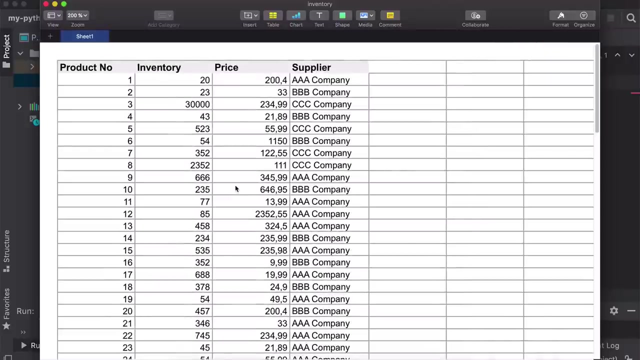 So in order to be able to do that, we need to save it first as a variable And let's actually call it inventory file, like this, And this will give us the file contents. Now let's actually open that file again And let's see exactly what we need so we can have multiple. 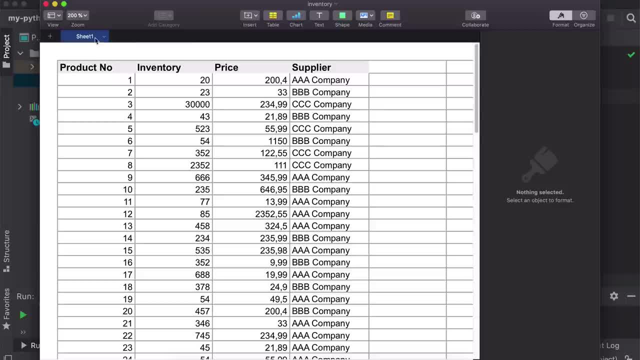 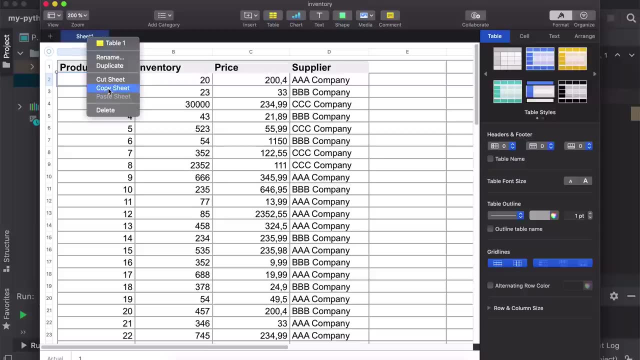 such sheets, basically per file, So we need to tell the program which one it should use exactly. So, for example, if this was called a product list, you would use that name, But we're going to go with sheet one, So we're going to use that name basically. 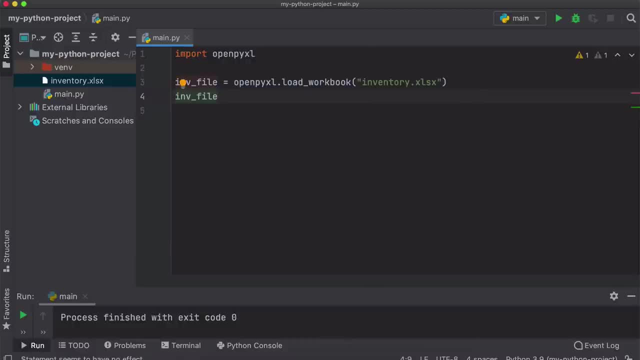 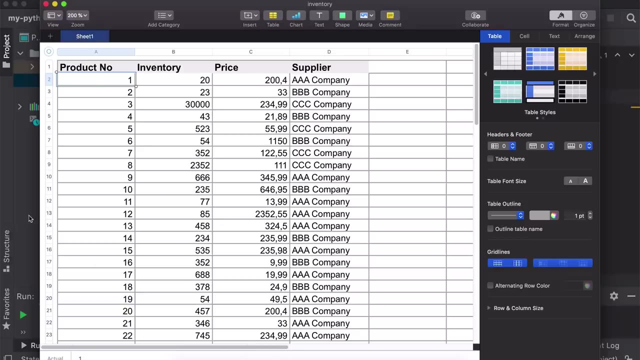 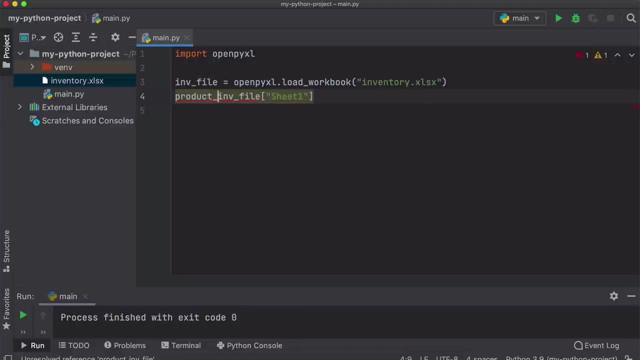 And we're going to grab that using following syntax, And you remember the syntax probably from using a dictionary. So this will give us this one specific sheet and all the information inside, And we can also save that into a variable. So let's actually call that product list. 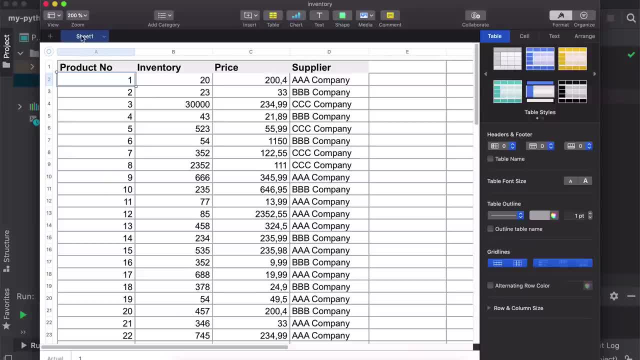 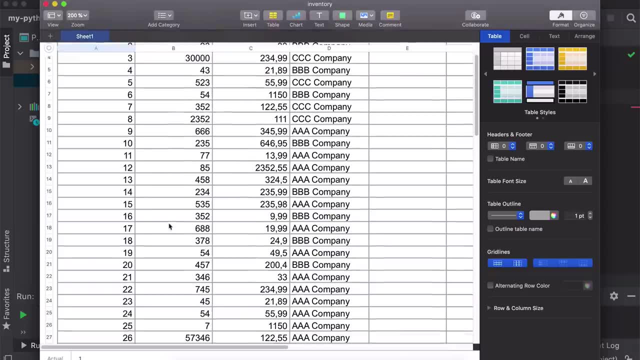 So now we have read the whole file and we have read this specific sheet of that file And now we have all this information in that variable. So now we can read any of those values and do calculations, et cetera, using that variable. 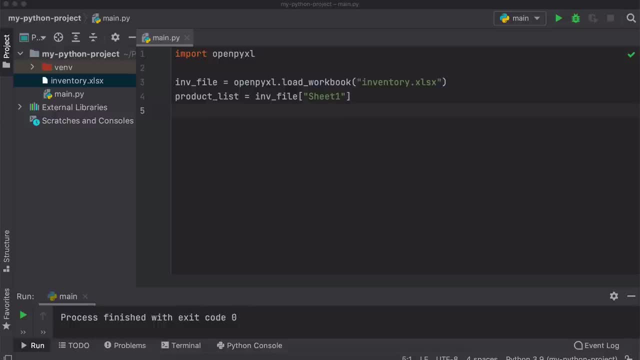 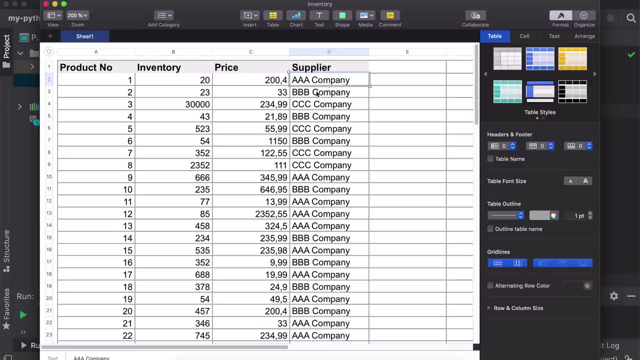 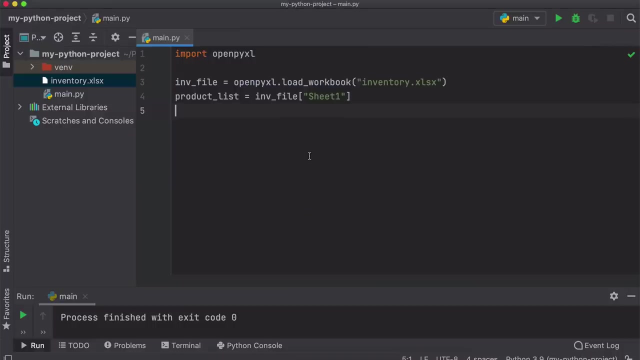 So let's get to our first task, And the first task is basically to calculate how many products we have per supplier and then list the names of the suppliers with that respective number of products. So let's go back and do that. So the results, what we want to get, is basically products. 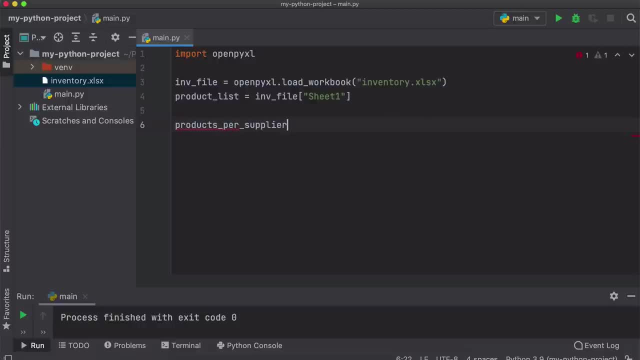 or number of products per supplier. Right, That's basically what we want to get as a result. So we're going to create that variable and we're going to set it to an empty dictionary. So by the end, Our program should give us something like this: a dictionary. 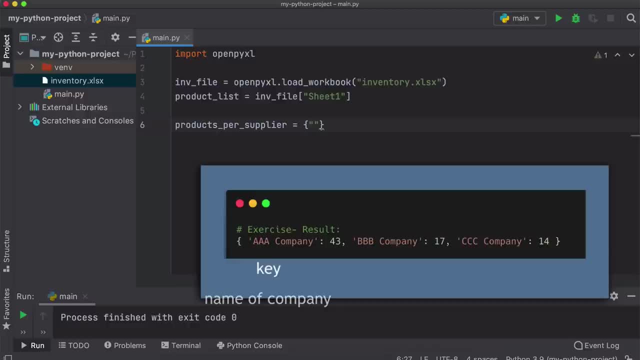 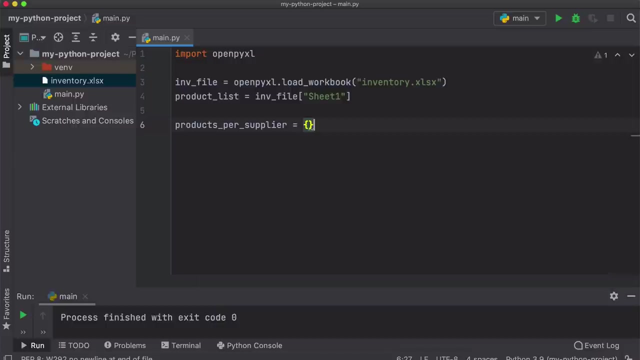 where the name of the company is the key and the value is basically product count for that company. And since we have three suppliers or three companies, we're going to end up with a dictionary with three key value pairs per company. So we are starting with an empty dictionary for products. 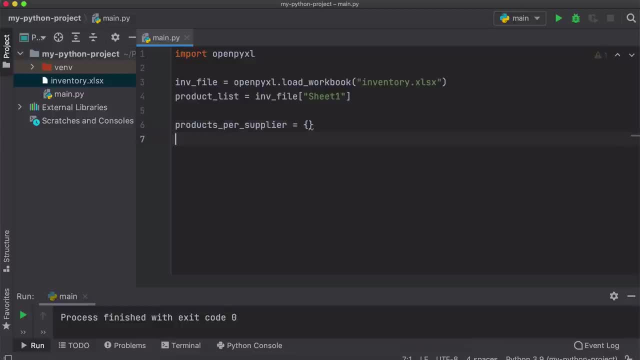 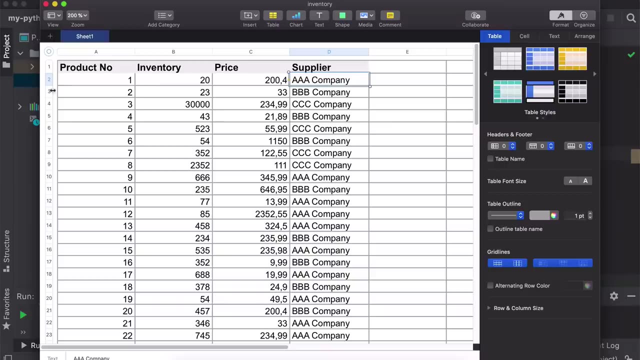 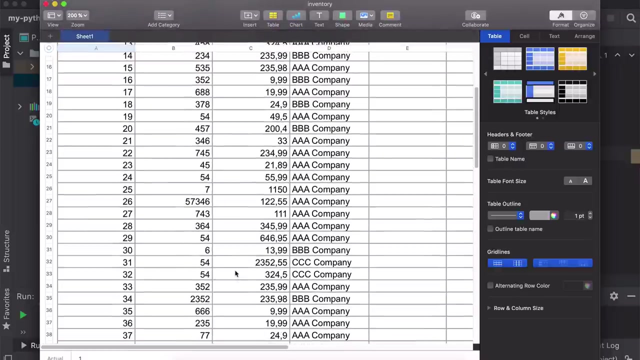 per supplier. And now let's see how we can programmatically calculate this. First of all, what we need is we need to go through each of these lines basically. So we have this row, So we need to go through each and every row in order in. 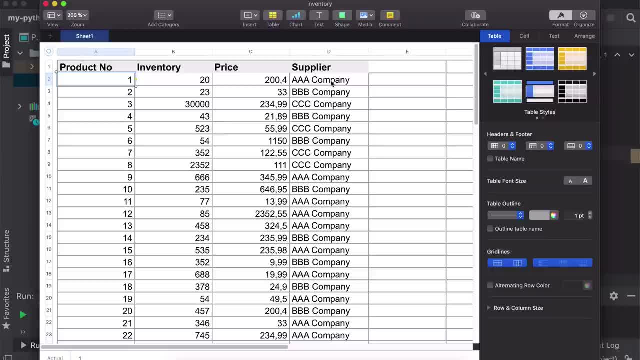 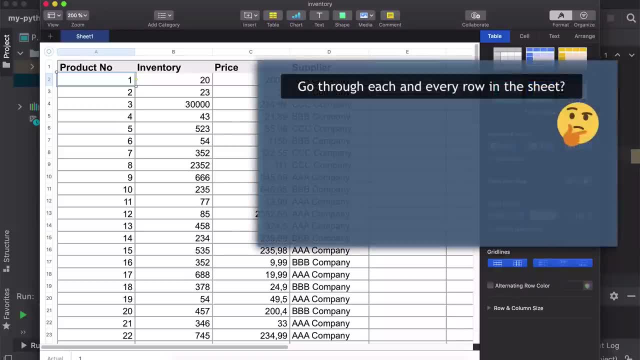 sequence and we need to get or check a supplier name for that row. And you remember, whenever we execute a logic on multiple values over and over again, so basically same logic or same function gets executed For multiple different values for a number of times. that's. 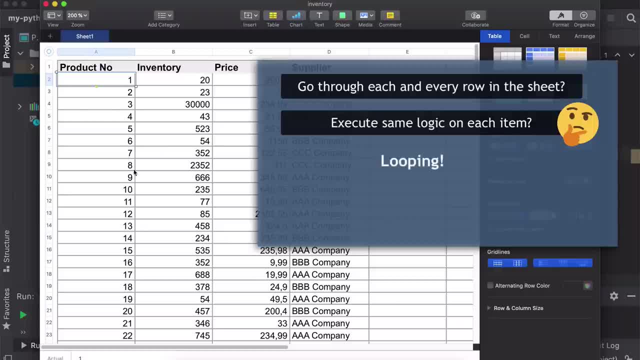 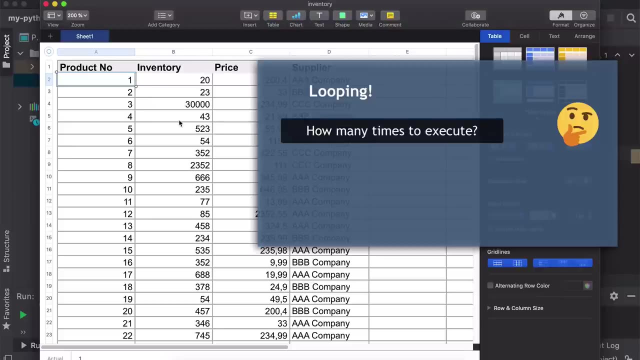 basically a use case for a loop, Right? So we're looping through those rows and we're doing the same thing per row, which is getting the name of the supplier. Now, as you also remember, loops have conditions, right. We need to tell the loop how many times it should execute. 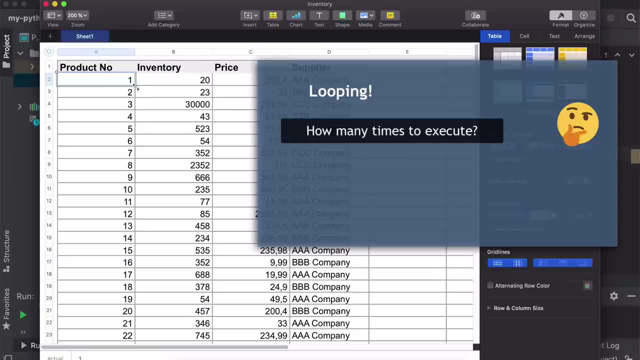 that specific logic And if we check our file here, how many times we want to execute the logic Right, The answer is as many times as the number of products. So if we scroll down we have seventy four products. So we need to do that seventy four times for each product. 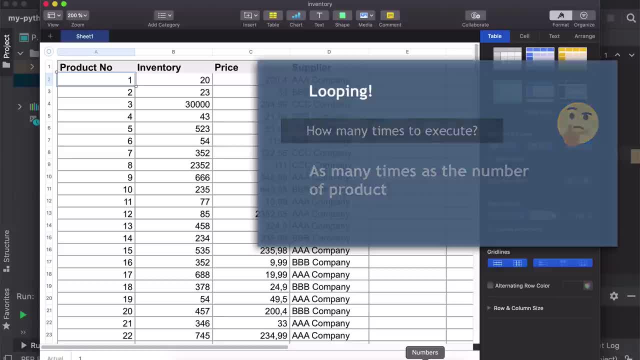 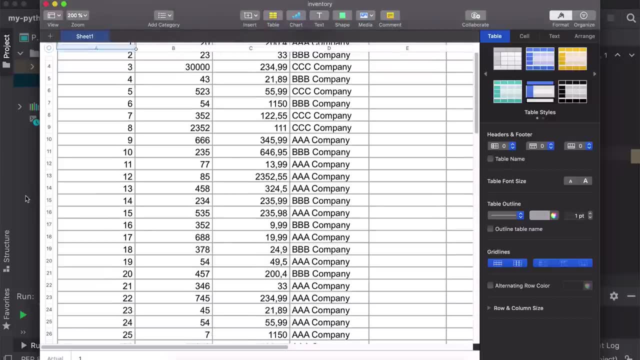 So basically as many times as the number of product. and obviously we want this program to work for any spreadsheet file, right with any number of products. So we need to calculate or we need to read that value also from the file. So basically we need to read how many products are on this list. 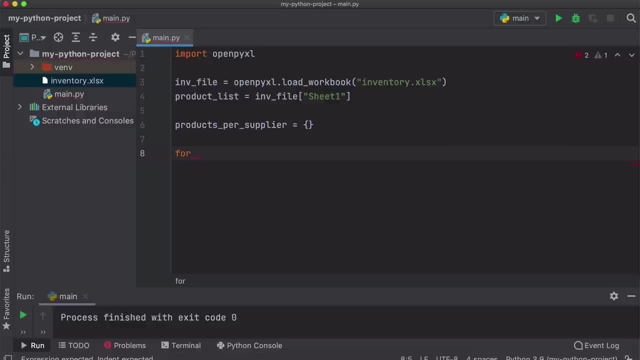 So let's see how we can do that. First of all, we're using for loop to execute the logic for a specific number of times, And if you remember from for loop syntax, for then we have the specific item. So what is an item in our case? 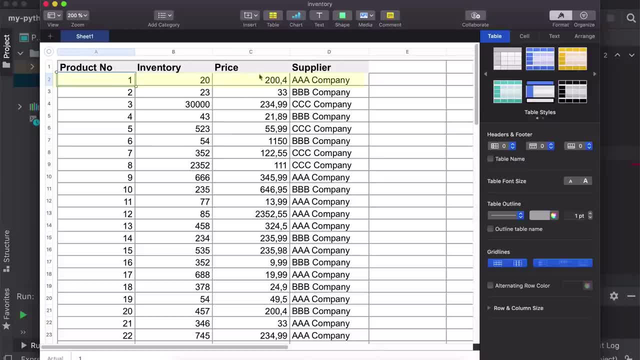 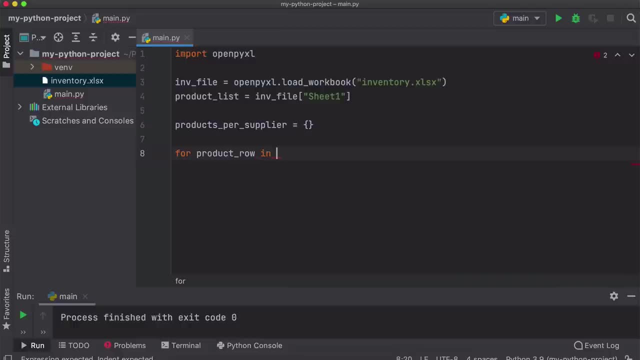 Our item is a row, right? Product row is going to be an item of iteration, So looping, basically, So we can call Our item product row and then comes in, and now we need that condition. How many times? And again, this should be generic. 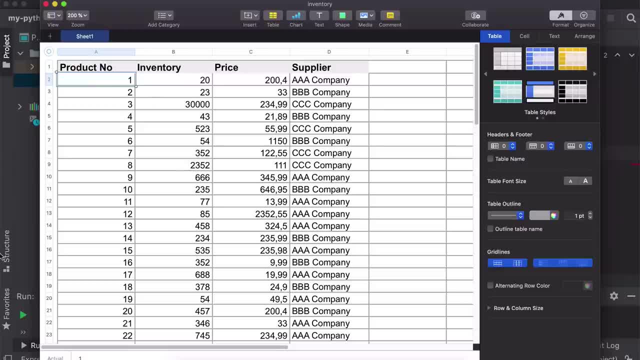 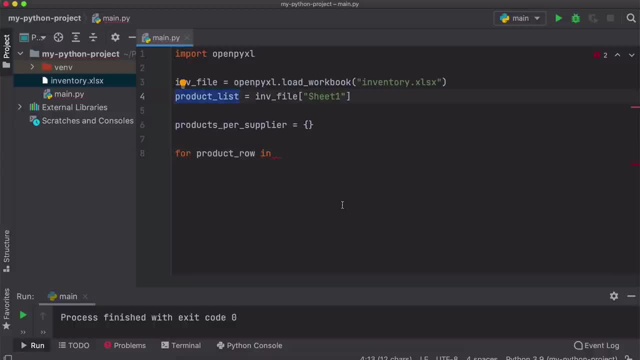 So we need to calculate or we need to read the number of lines here, number of rows here, from the file, And the way we can read that is to remember. we have all the information we need in that one specific variable, which is product list. 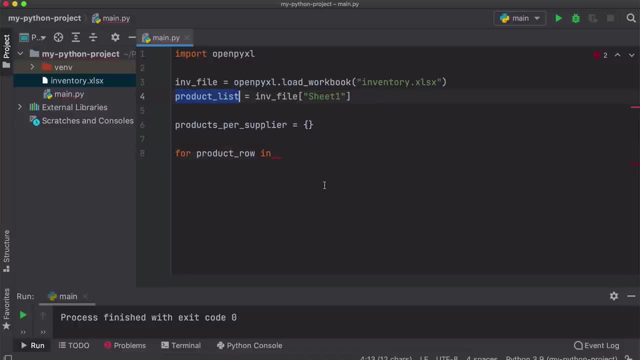 And that variable has the value for number of rows, which is called Max Row. Now, how do I know that Max Row attribute is available for product list? I basically just looked it up on the documentation of the module And, as I previously also mentioned, 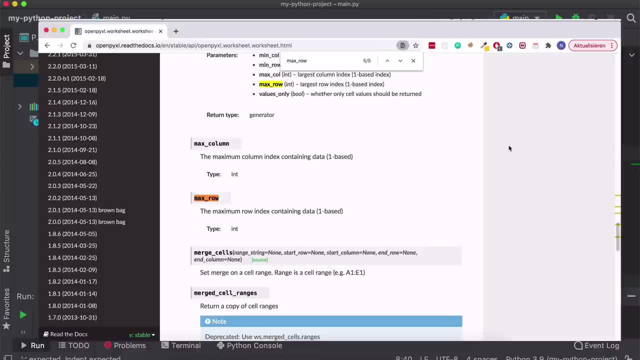 whenever you're using a module, this module will have a documentation. So if you need some functionality, if you need some values, you can basically just search inside the documentation which functions and variables are available to get the functionality or values that you need, and we can. 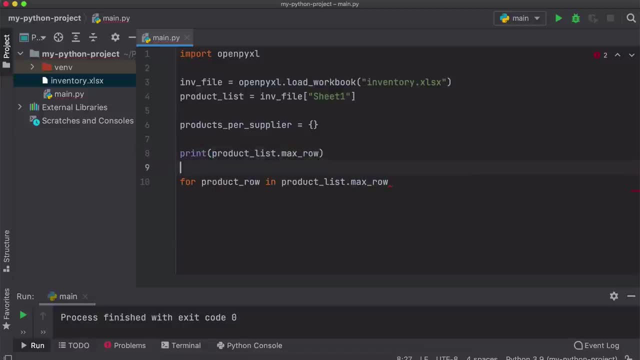 actually test it. We can print it out like this And, as you see here, seventy five. So basically, Max Row will always give us the number of lines or number of rows in that specific sheet, so we know how many times to iterate. 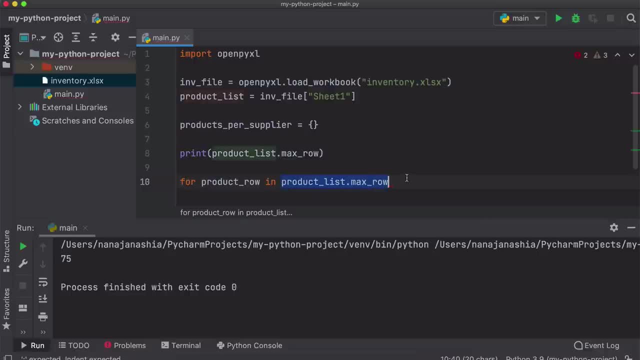 Now, whenever we're providing a specific number in a for loop, like seventy five, for example, in this case we need to put that number in a range like this, So we can't just say seventy or, in this case, Max Row. 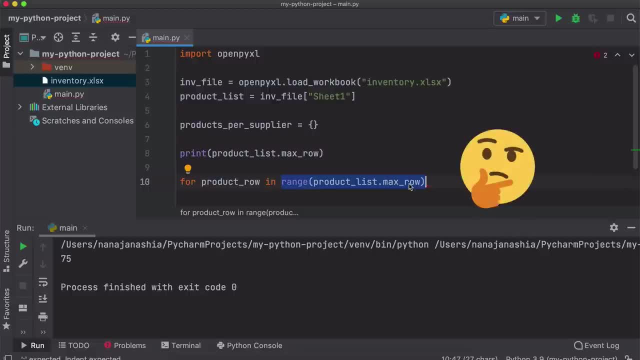 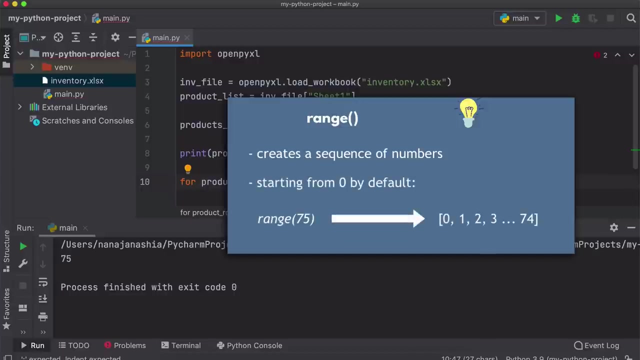 Now, why do we need a range here and why is number just not enough? Because the for loop is for iterating over a list and the range will create a list of numbers to iterate through. In our case, range of seventy five will create a list of. 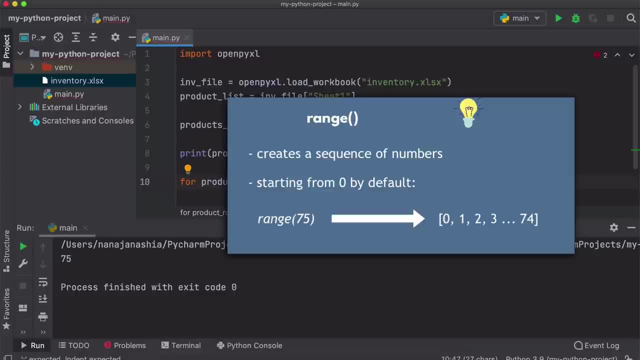 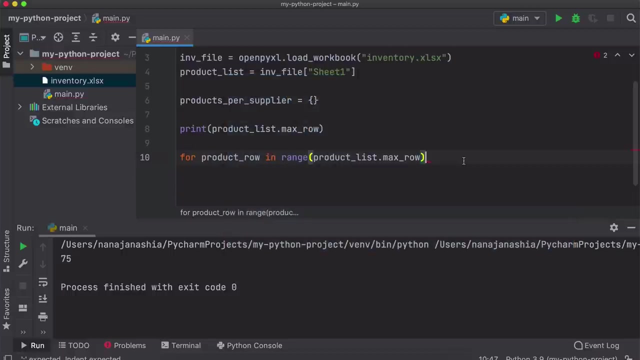 numbers, or sequence of numbers, from zero to seventy four, And with that we're going to have a valid for loop where, for each item in this list of numbers, some logic will be executed. So that's why we need a range here. And now there's one more thing that we need to fix. 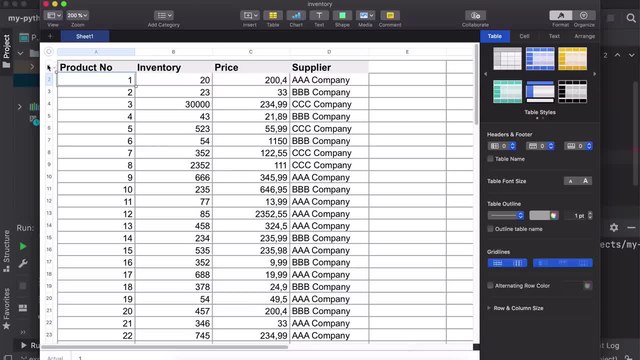 We go back to our spreadsheet, You see that the first row- So this is going to be the first row- basically does not actually include the product information. It just includes the titles for each column, Right? So we actually do not want to read this line. 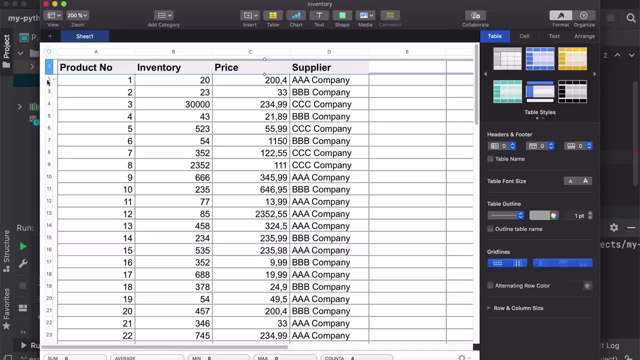 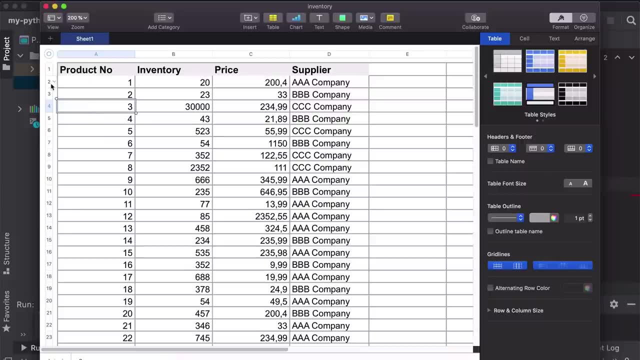 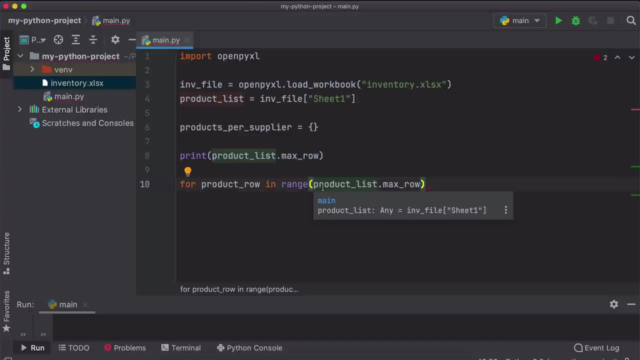 We want to skip it and we want to start from the second row. So, instead of starting for loop from the first row, we want to start it from the second row, and in order to tell Python to start at row two in the range function, we're going to pass. 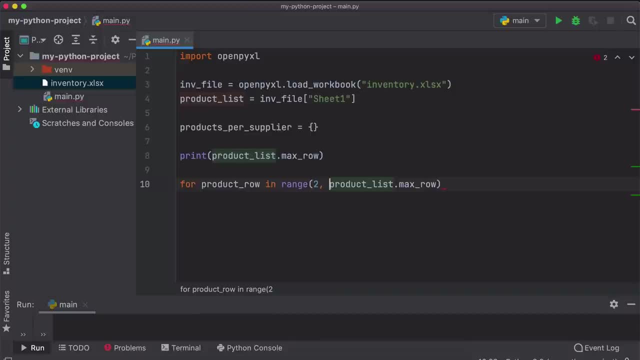 first parameter two. So basically, this will give us a new range of numbers starting from two instead of starting from zero, And since we're using those numbers in the range as an index for the rows, the first number is going to be two. 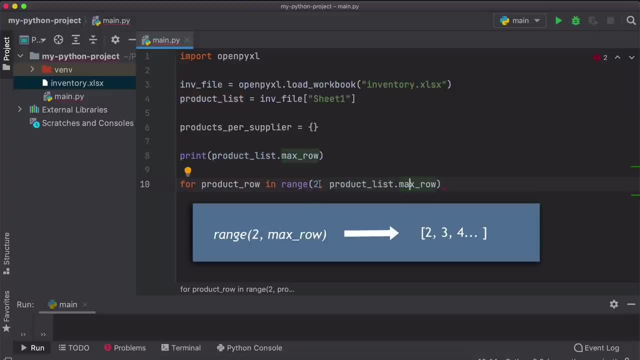 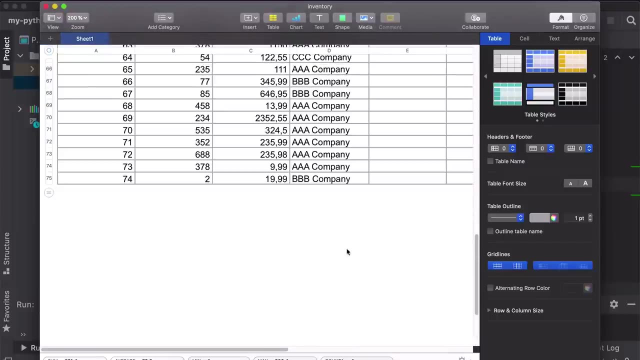 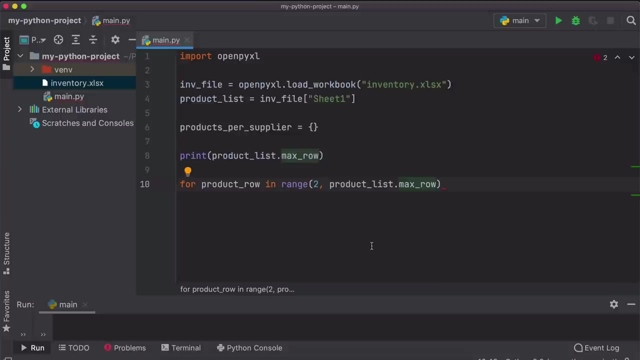 So we're going to start iterating from the second row, So this will be the start point and this will be the end point. So, basically, from here to the end. Now there are two things specific to a range that you should be aware of. 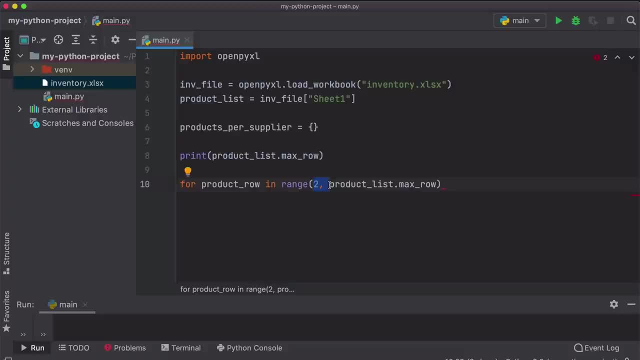 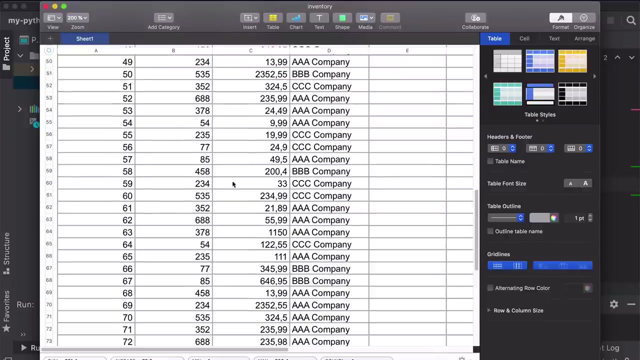 First of all, when we do not provide the start index, basically the start number in the range, by default it's actually zero. So it's not one but it's zero And obviously we don't have a line zero here. So if we executed it with the default one, 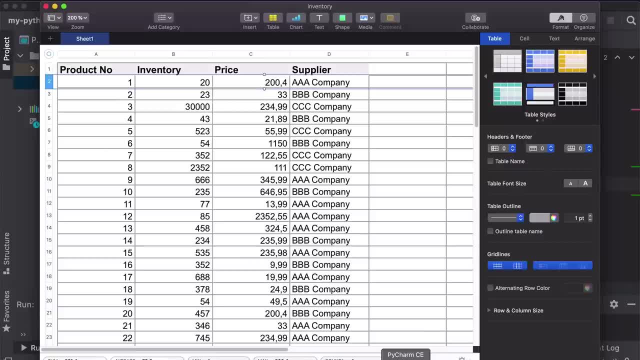 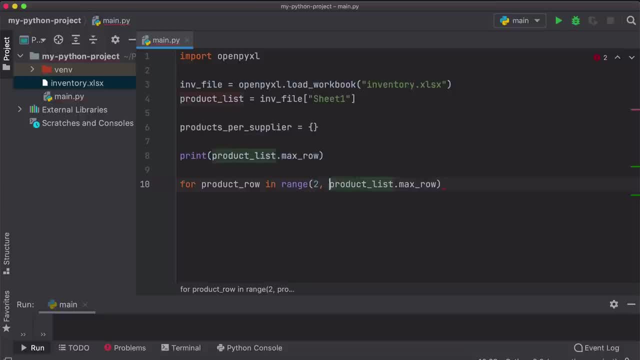 we would get an error. So that's one thing to consider. that range actually by default starts at zero and not one, But for us it doesn't matter, because we're skipping the first one anyways and we're starting from line two because our spreadsheet doesn't have line zero. 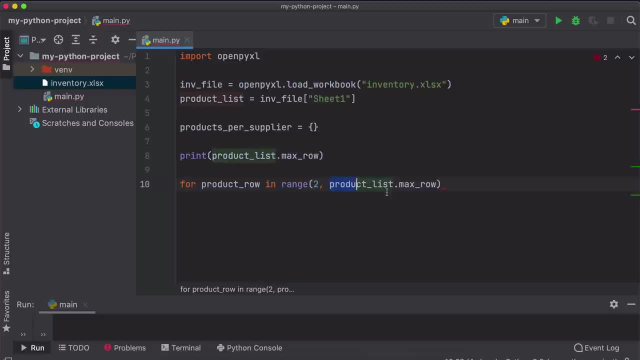 Obviously, another specific of the range is that the second value here basically the last number of execution in the loop. In our case this is going to be seventy five, Because we have seventy five lines and we printed that out here. that number is actually exclusive. 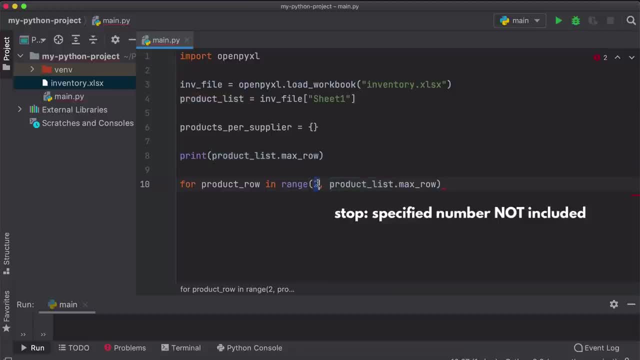 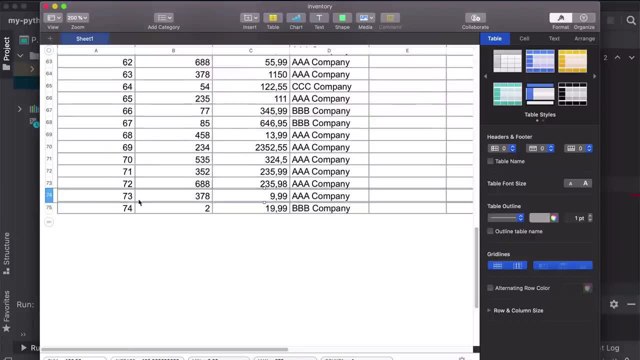 It's not inclusive. That means that the range will execute from line two to seventy five exclusive. So basically, till here. this line will not be included in the loop again. That's a specification of the range which we need to fix And basically want to tell you know what we want: that iteration. 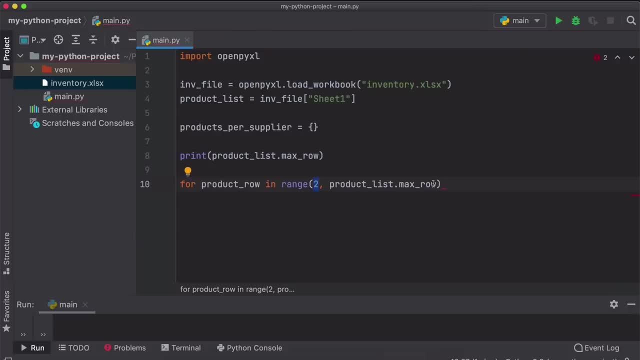 including the last number as well, including that next row, And a simple fix for that is going to be to do plus one here. So, basically, whatever the next row is, we want to include that one as well. So we want to add one to it. 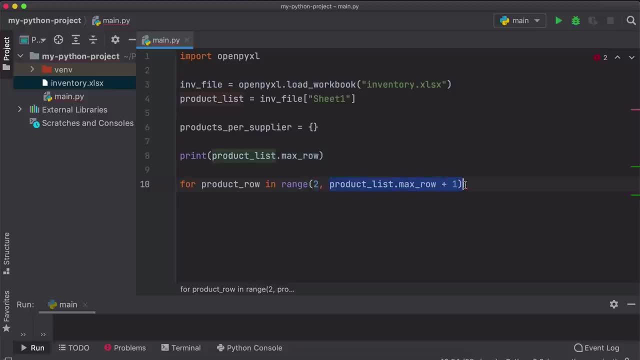 So now we have a range starting from two and ending in seventy six exclusive. So obviously the seventy six line will not be read and this will now give us a range that we need. And now that we have condition for the loop and we have said 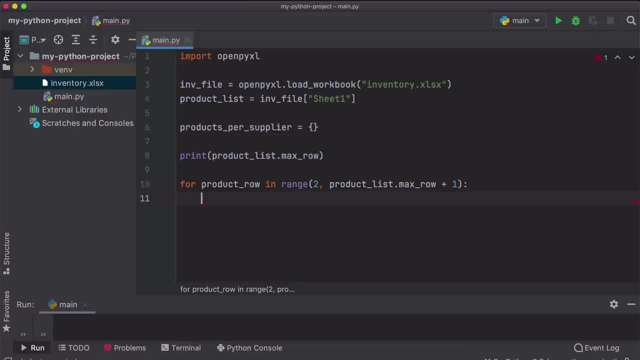 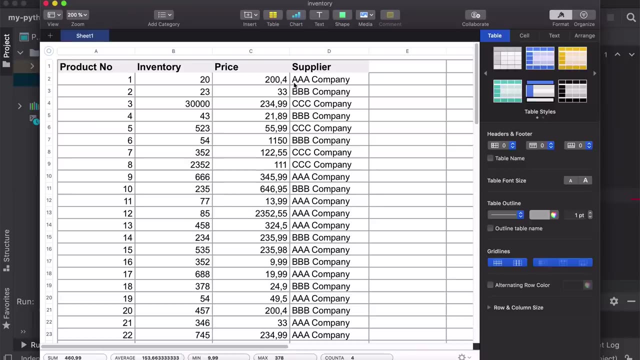 how many times they should execute. let's actually execute the logic itself. So what is the first information we need from that product row? for each row, We basically need the supplier name so that we can increment or start counting how many products the supplier has. 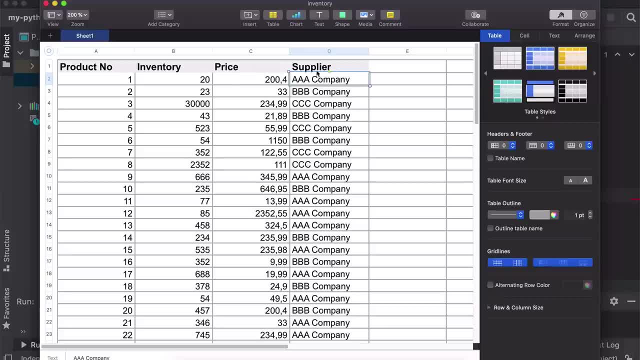 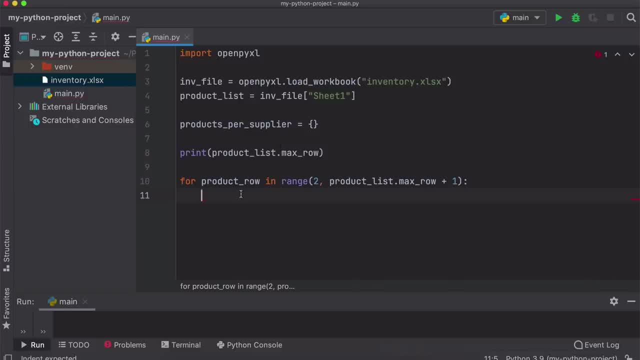 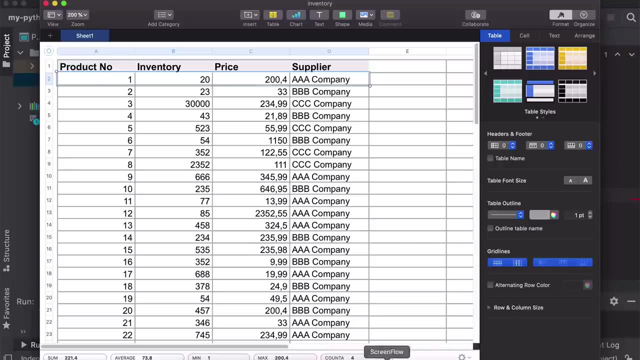 So we need this one, two, three, fourth column and the value in that fourth column for each and every row, Right. Let's go back to a tour. How do we get a value in the cell? You have to imagine when we iterate we have one row per. 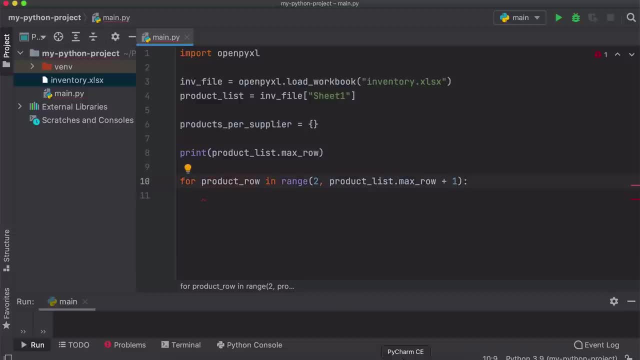 iteration. So, right, here we actually have this product row, which is just one row, and we have four columns here and we want value in this specific cell and we can get it using first of all product list because, again, we have all the information here on this list. 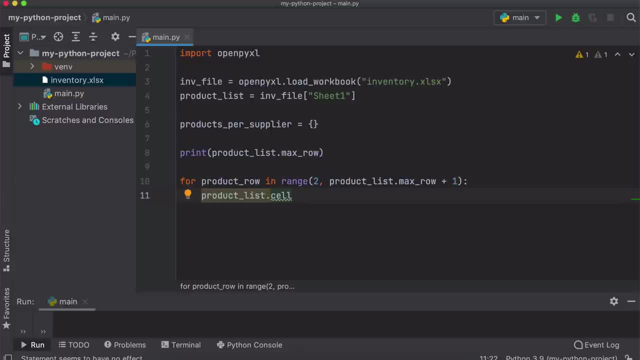 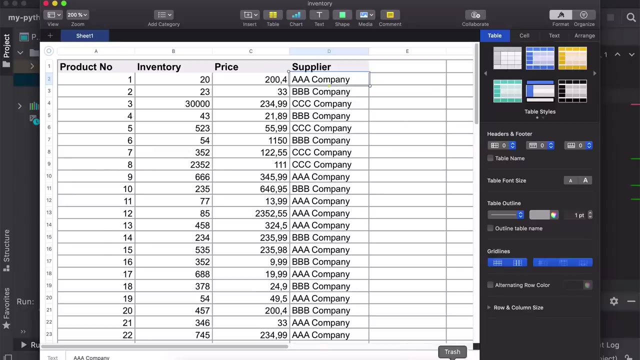 We need a cell, right, We need a value of a cell. So that's the name of the function and the cell basically takes two parameters. Again, product list contains the whole sheet here, so the whole list with all the rows and columns, and we can get. 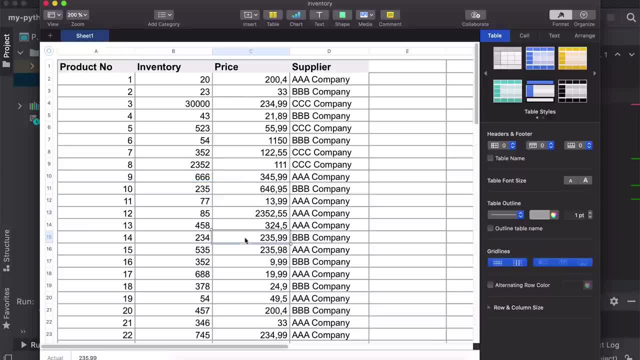 a specific cell value. So whatever we are, doesn't really matter, from that variable, by providing two values: the row number and the column number, That's it. So row nine, column one, basically, will be this specific value. Row five, column four, will be this specific value. 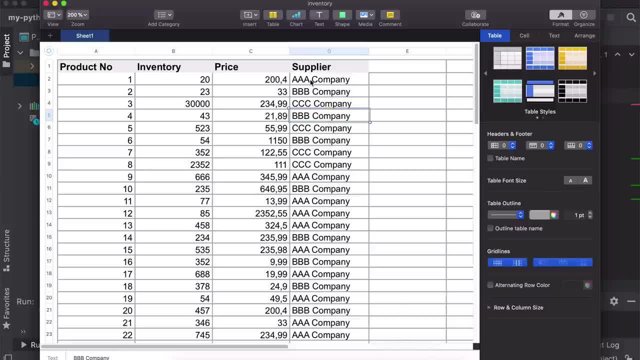 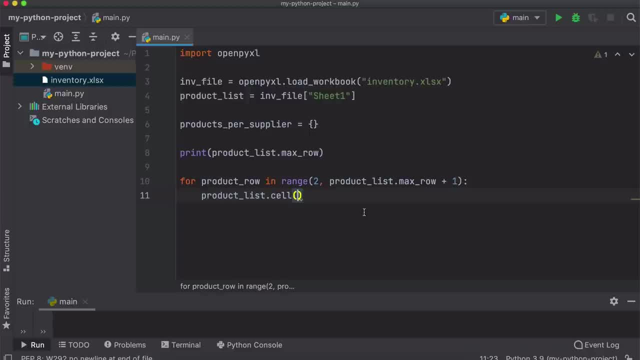 So for each iteration we're going to do exactly that. So for our case, the supplier is always column four And the row is dynamic because we are iterating and therefore we're going to use whatever row we're at at the current iteration. 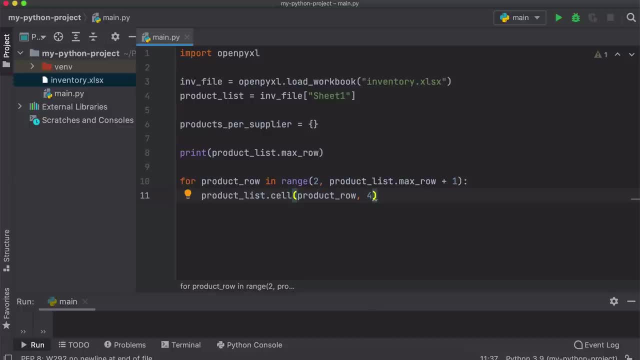 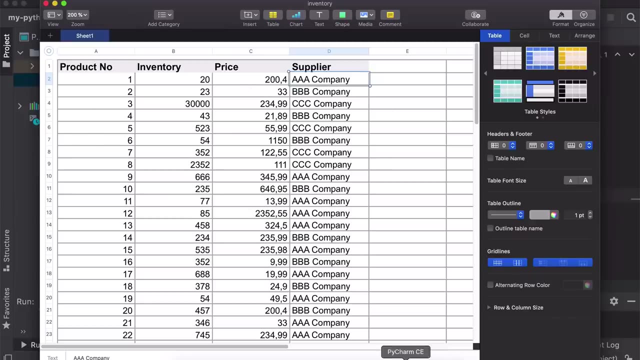 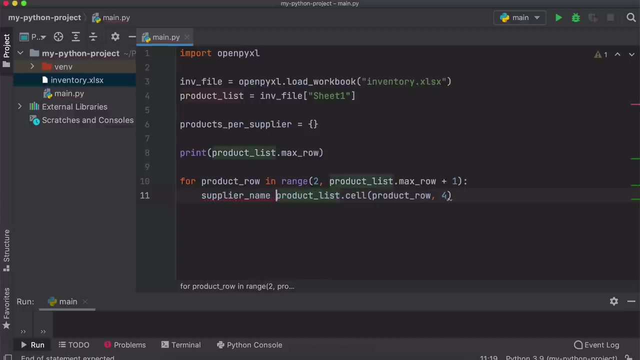 So that's the first parameter and column four, as I said, and this will give us the supplier name for each and every row. so we can grab that value like this And this is going to be supplier name, So we can save it in a variable as a next step. 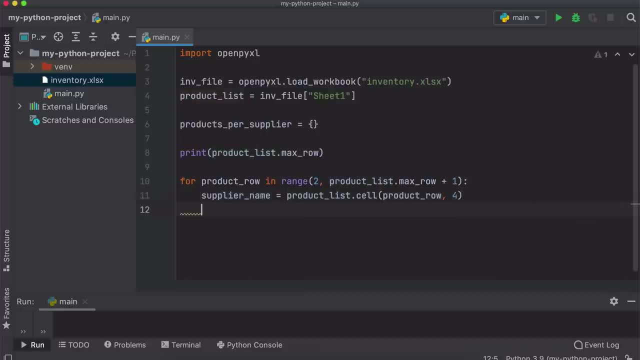 We're going to start building how many products each supplier has. We're going to start building a dictionary with the name of the supplier and then how many products they have. So we're going to be building this dictionary here. So this is a reminder now for what I said previously, that 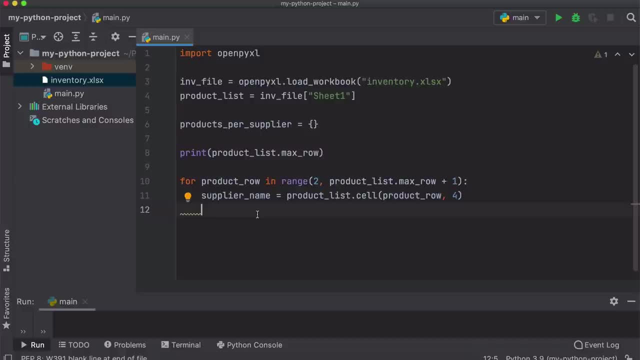 you don't need knowledge of math in programing. Rather, you need logical thinking right. So you're going to get tasks like this, where you have to basically logically decide how you are going to do a certain task and think all this through. 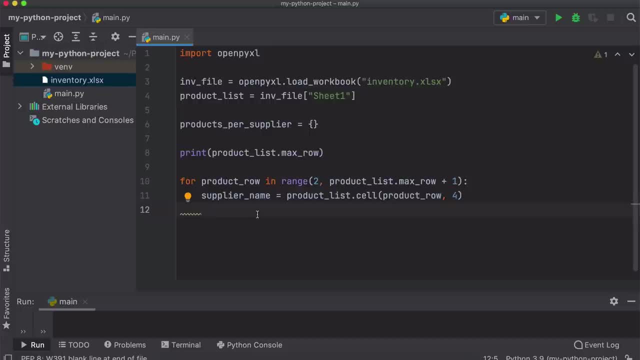 Right. So programing is more about logic rather than pure calculation or math, which is actually more interesting and cooler, And that's exactly what we're going to need in this example. We're going to need some logical thinking to basically build this application. 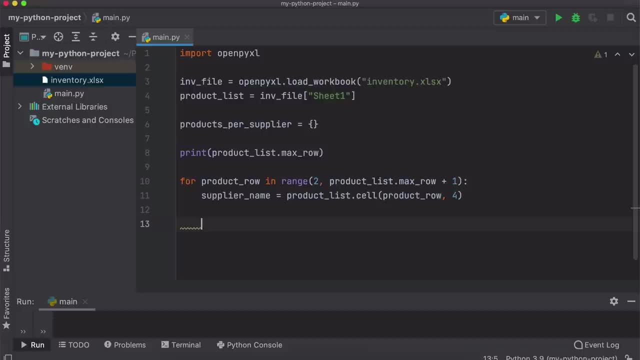 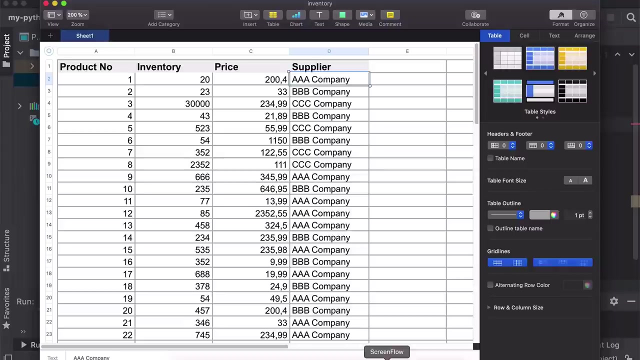 So bear with me on this one, The first thing we need to check here. So think about this iteration on the first time and second time. the first time, the list or the dictionary is actually empty. So we want to add the first supplier to the list, right? 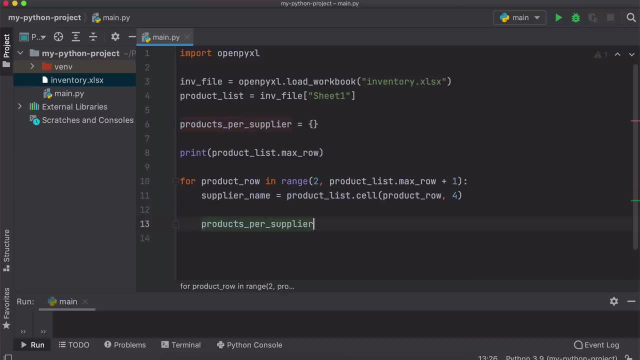 away Right, So we're going to grab that, and the syntax for adding a new entry in a dictionary is like this, where we have a key and a value here. So, Basically, what we want to end up with is a supplier name. 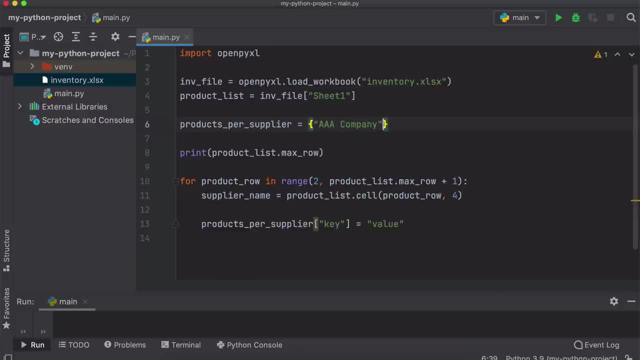 like a company and number of products for that supplier. That's the dictionary that we want to end up with. Then it's going to be BBB company and so on. So the very first supplier goes directly into the list and we're going to need the name of that supplier. 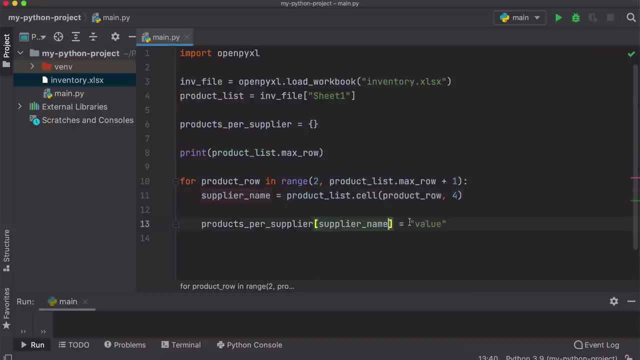 We don't know where it's going to be So. So name as a key and value is going to be one at the beginning. This is the very first iteration. So after the first iteration we're going to have the first company name, supplier name and count one for that on the 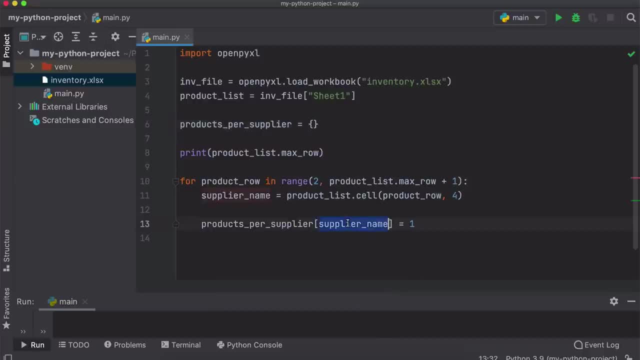 second loop, Second iteration. Basically, if the next line is a different supplier, like here for example, then New entry will be added, because we have a new key now with count one Right. So now we're going to have company A with one product. 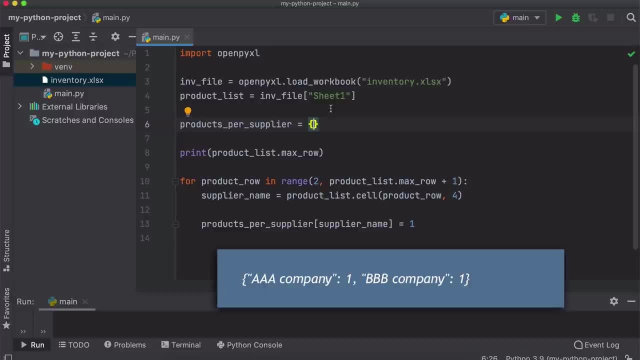 company B with one product. Now what happens when, on the next iteration, we get company A again, Right? What we want to happen is company A, the product count to increase to two, Right, Because now we found another product that is a product. that is not a product. 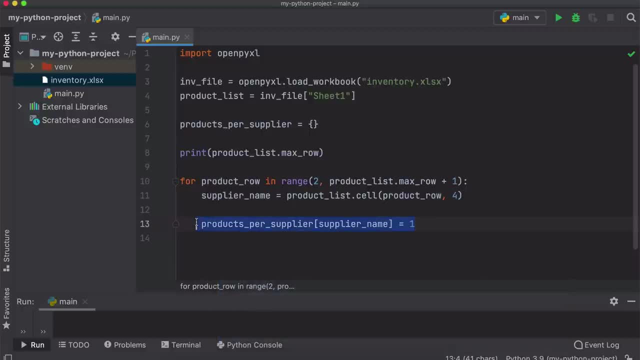 Is supplied by the same company. However, with this line, we're actually overriding and setting it back to one. So how do we make sure the number of products gets incremented instead of always setting it to one? What we're going to do is, before we execute this line. 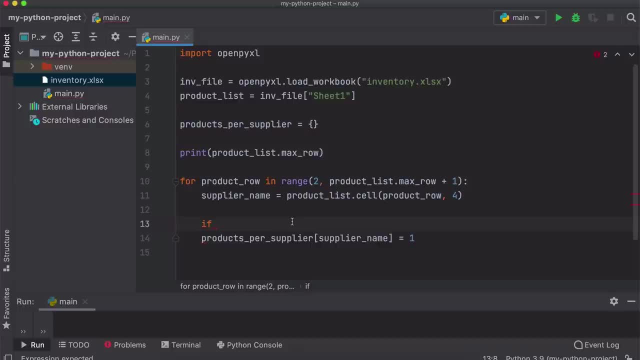 we're going to check is it a new supplier or an existing one, Because that makes a difference. So how do we know if it's a new one or an existing one? We can look that name Up in the dictionary. If we have already added that name in the dictionary. 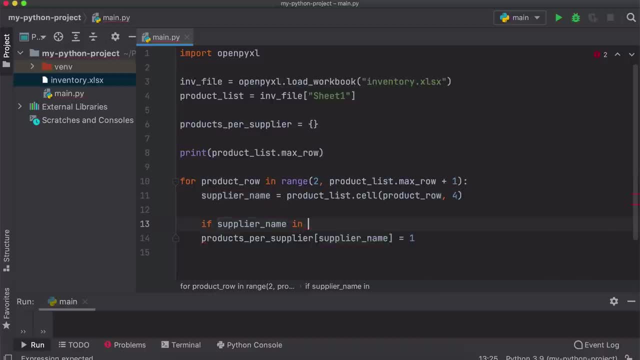 then it's going to be there and we can do that very easily again with the syntax if supplier name in the dictionary. it's actually very readable syntax that says: is a supplier already added to the list or is it a new one? So if this is true, again remember, if conditional. 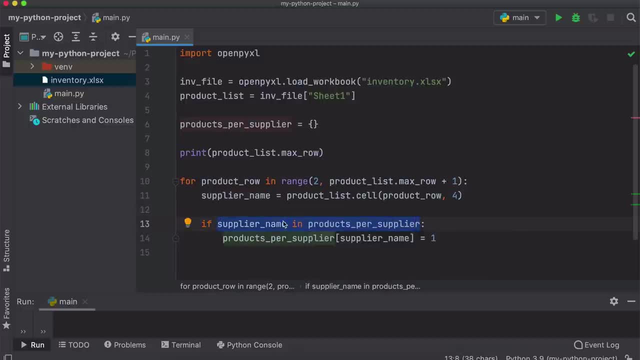 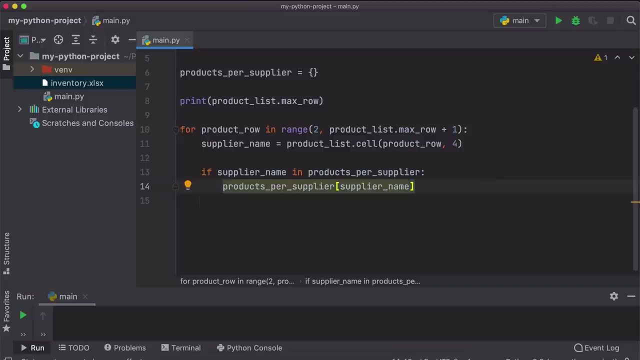 So, if this is true statement, if the supplier name is already there, then it is an existing one. So we need to increment the product number instead of setting it to one. So instead of assigning a new value, we want to grab that value, the existing one, and basically add one to it. 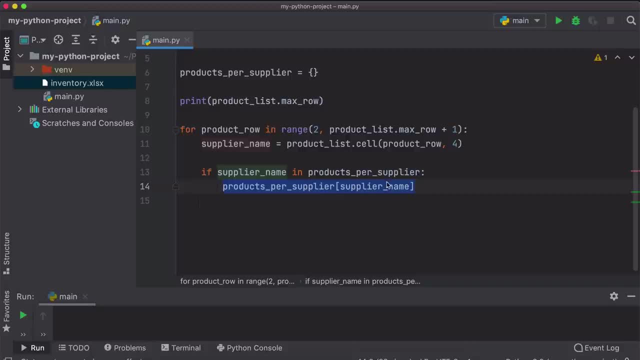 Right, Just increment by one. So getting a value from a dictionary- you probably remember the syntax already- using the key And we can save it into a variable. Let's call it current number of products like this: Remember we're using a key in order to get the value and the 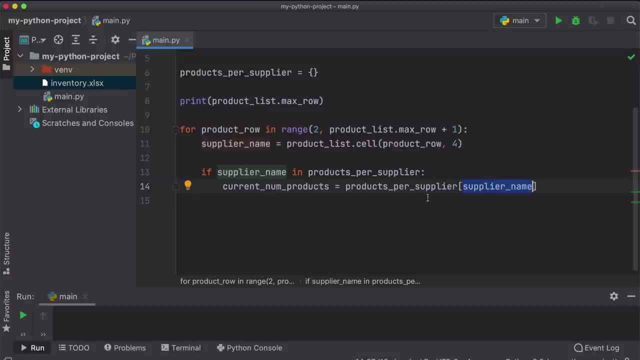 key is a supplier name. Value is the product count. So this will give us the current number of products. on the first iteration This will be one, or after the first iteration we're going to have one product for that specific supplier And 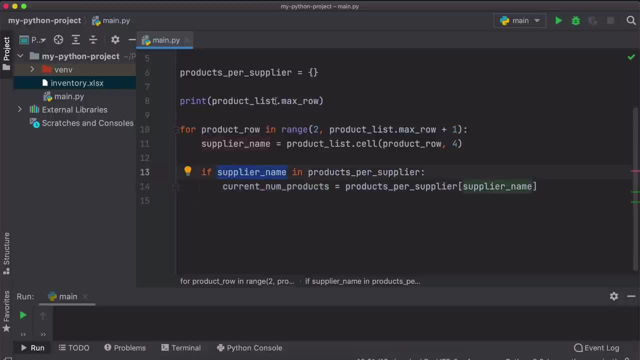 If we already have that supplier in the dictionary, we want to increment the number of products for that specific supplier by one, because we just want another product from that supplier. So we want this value to now be plus one, Right? So current number of products plus one. 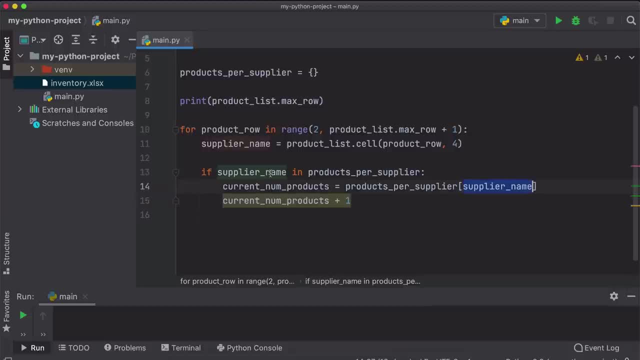 So that's the new value that we want for the existing, for this current supplier. And How do we assign it back to the dictionary again? We grab that and assign it. So, as you see, taking the value from the dictionary has the same. 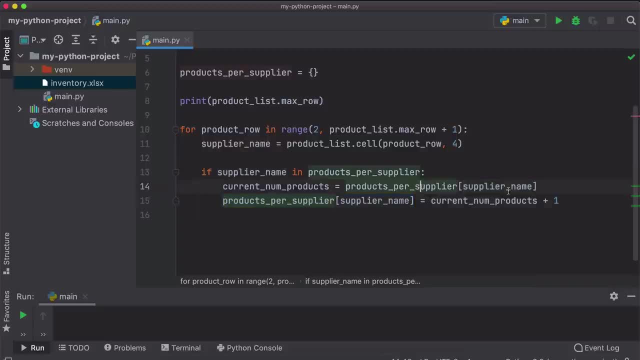 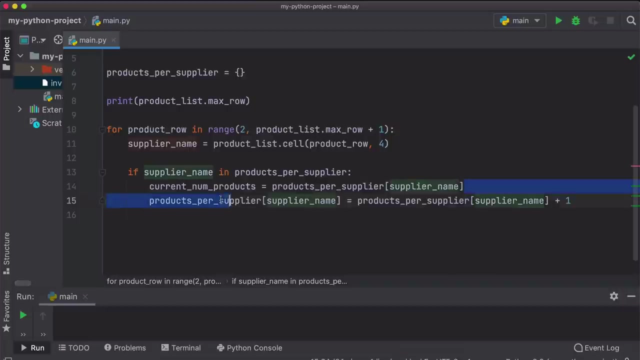 syntax as setting that value in the dictionary. In fact, we could actually use a shortcut here. So instead of current products, we could just take that value and add plus to it and then set it back as a new value, And this will basically just give us a one liner for the logic. 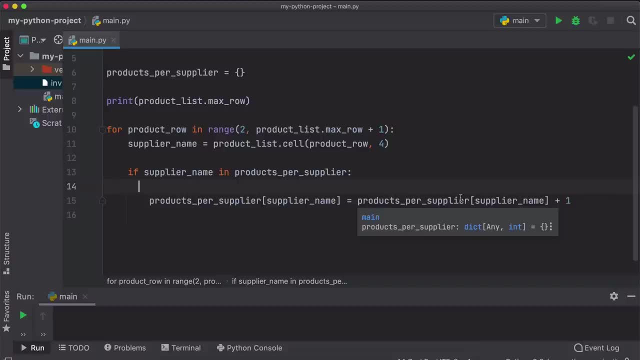 Depends on the taste whether this looks nice or not, or whether it's better to have a new variable and increment the value like this. Let's actually leave it like this. So this logic will take care of adding a product count every time we find another product for the same supplier. 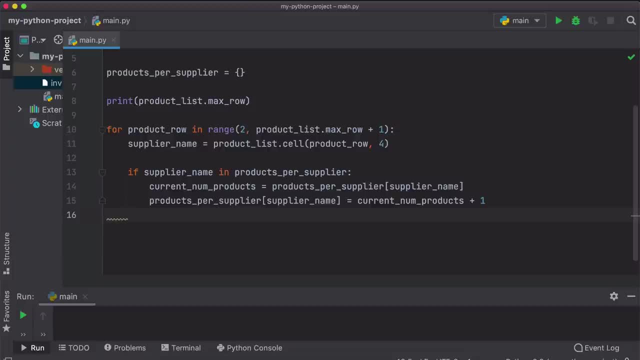 However, now we have to decide what happens when it's a new supplier. So if this condition is false, If the supplier name is not on the list- and this is going to be the case on the very first iteration as well, because the dictionary is basically empty- 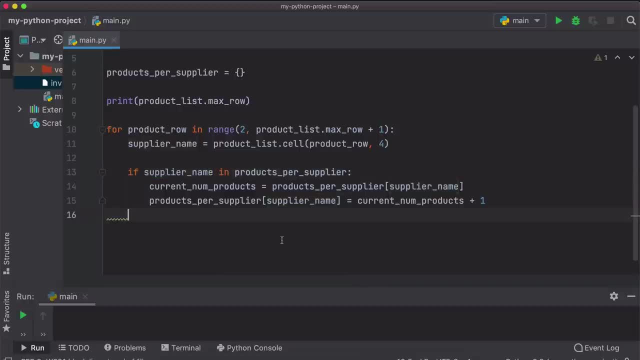 So there are no supplier names And for that case else, we're going to do what we had before, which is just setting that number to one Right. This is going to be the first value. So this will do two things. Basically, it will create a new entry in this dictionary. 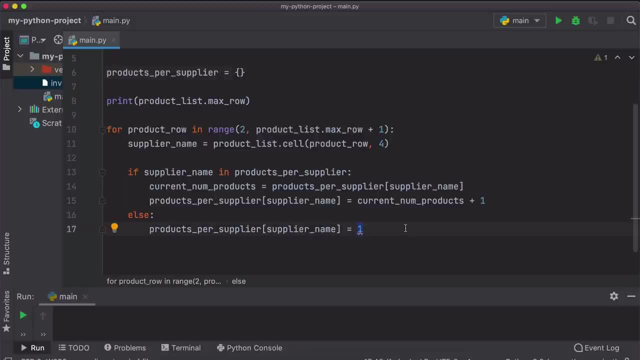 for this new supplier and it will set the count number to one for that new supplier. And that's it. That's actually our logic, And let's actually try this out and print it out. So right here I'm going to print: adding a new supplier and. 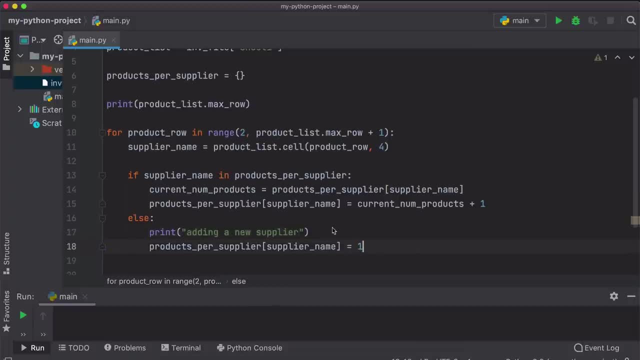 this is going to happen three times because we have three suppliers so we can safely print it. because just going to happen three times. There is one more thing we need to Fix here, and that is getting the value from the cell. So if we actually execute this now, let's comment this out and 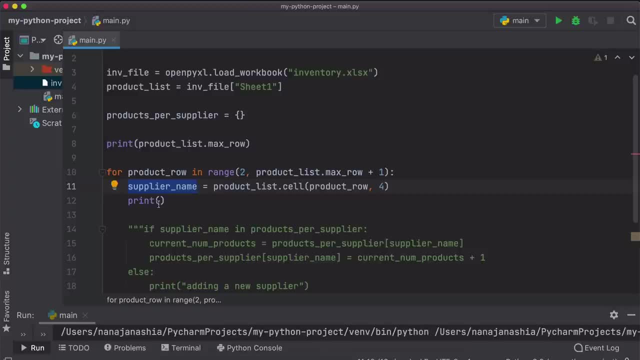 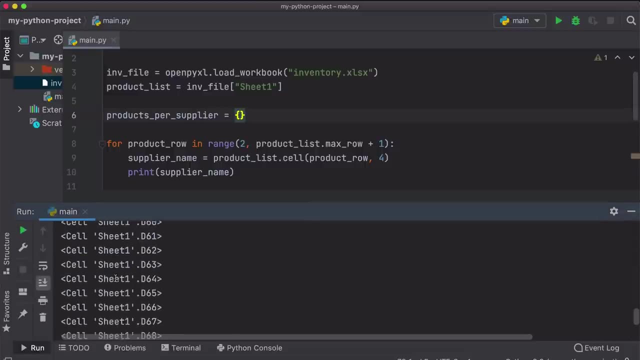 actually print out what the supplier name is. Let's actually get rid of this line- We don't need this- and run the program. You see, here we have cell information, so it's not actually the, the value, the name of the supplier, but it's just. 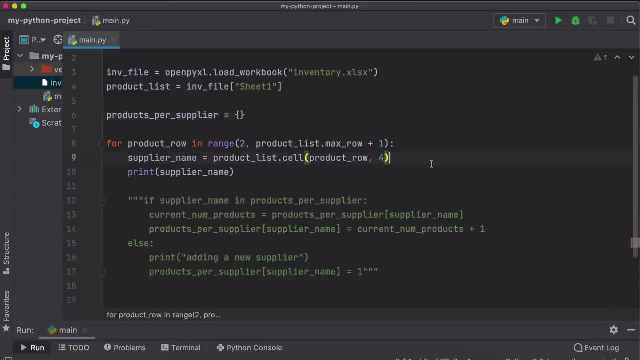 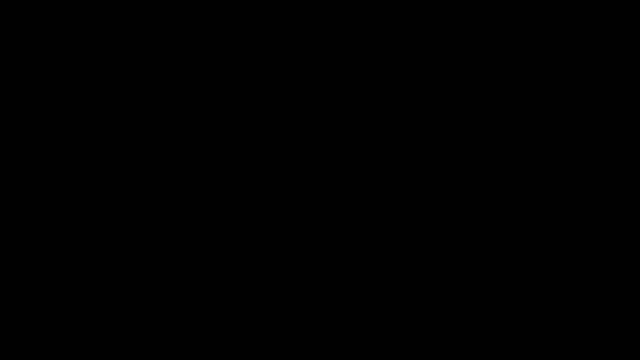 the object cell, And the reason for that Is because we're accessing a cell but we're not actually extracting, getting the value out of it, And we can do that using this value attribute on that complete object, again something that you can look up in the 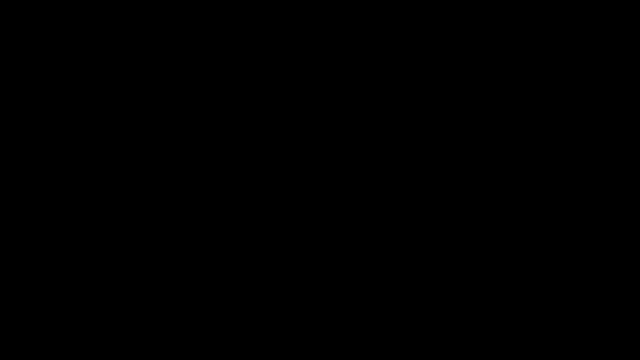 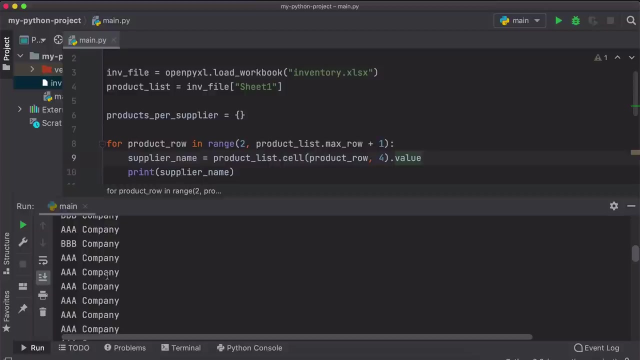 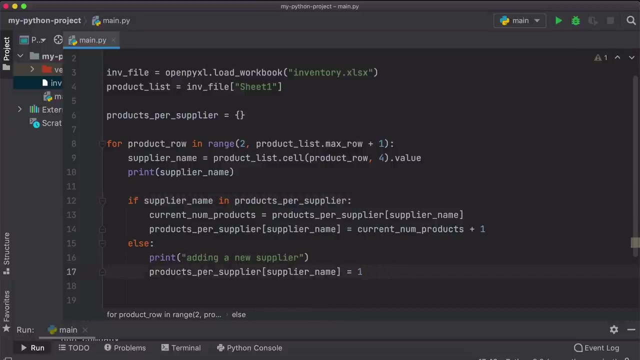 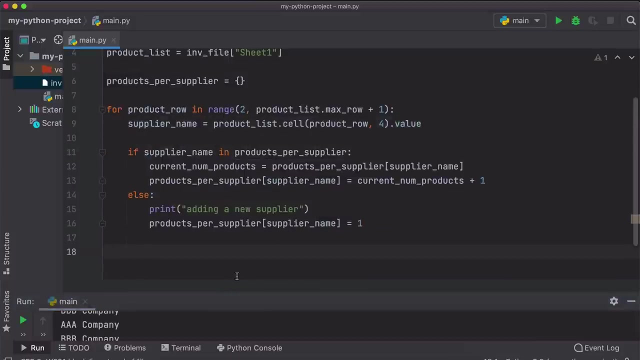 documentation of these open pie XL module. So now let's run it again. And now we have the actual values of that cell and this will take care Of that small problem. And now we are ready to execute our program. And after the full loop, actually let's print out the: 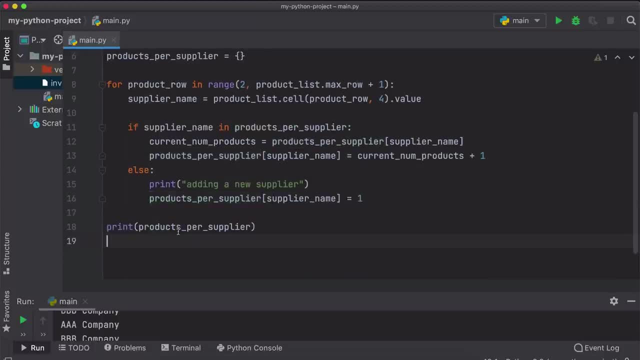 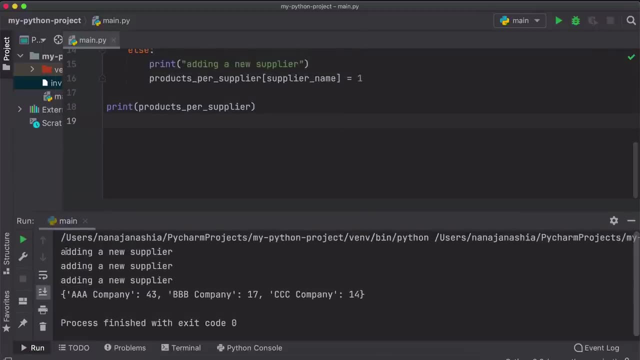 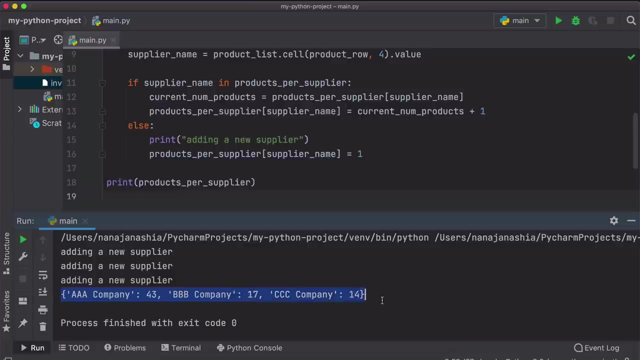 dictionary, because we want to see the results of the dictionary that we are building here, And I'm going to execute it now. And there you go. First of all, we have three times adding a new supplier, because we have three suppliers. And this is the resulting dictionary and it looks actually. 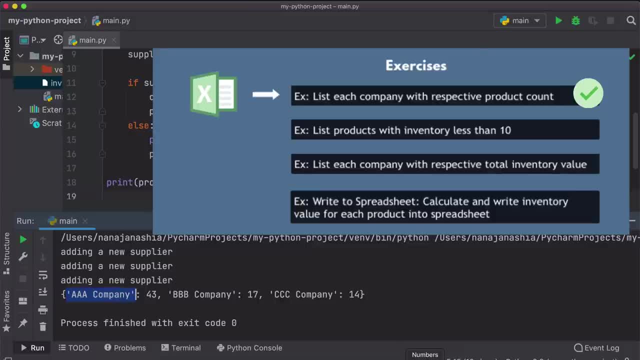 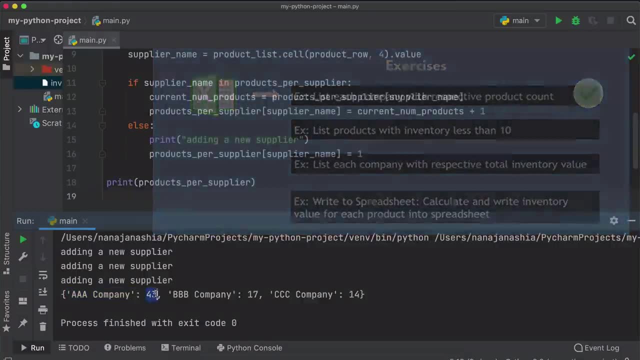 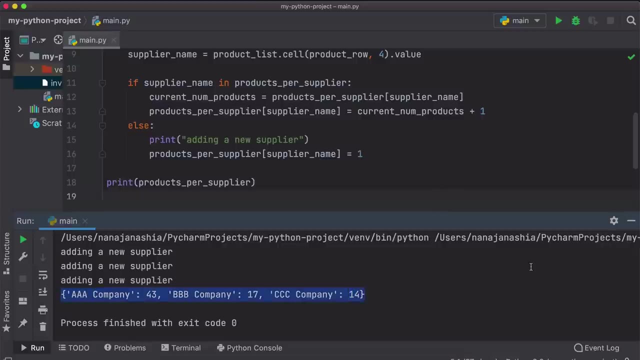 very good. First we have company eight, because this was the first on the list and we have a number of products that were counted for that company. Then we have the second one with number of products and the third one, So it looks like our program did exactly what we wanted. 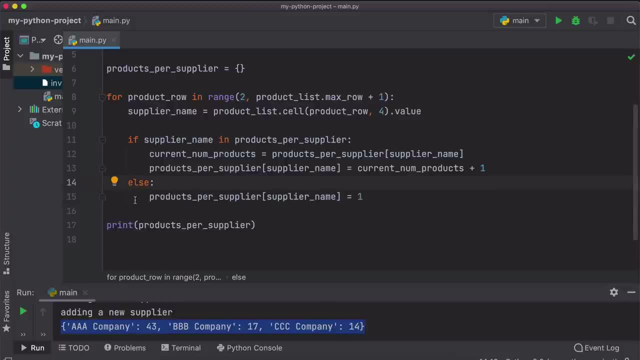 So that takes care of the first exercise. Now I want to note here one small thing, which is an alternative syntax for getting values from a dictionary, which is actually a more recommended way of doing it, which is, instead of having these brackets here, to have a get. 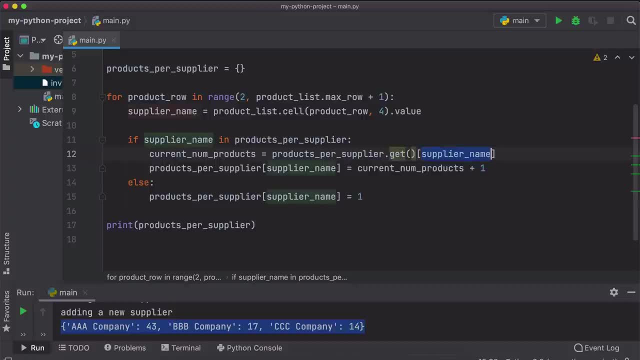 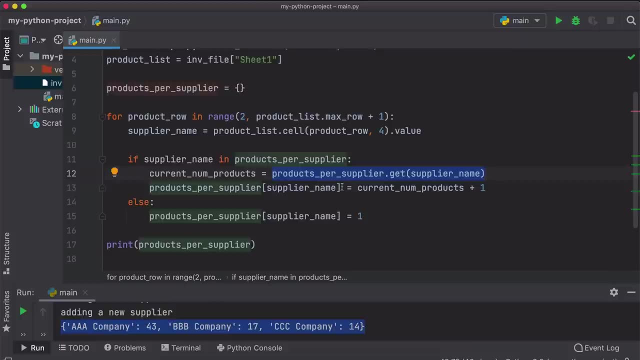 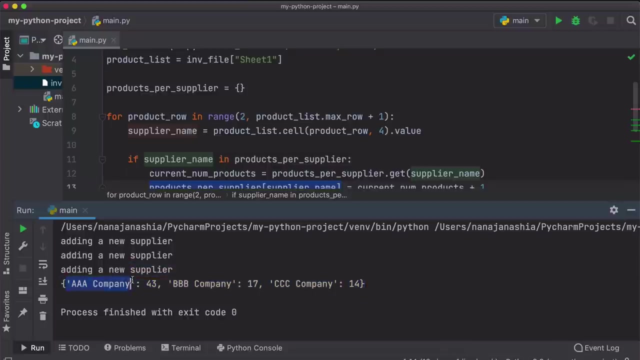 method right to use a get function with the key name. So now you see the difference between those two. So this is setting the value of that key. again Remember, key is this one here and this is the value. So we are accessing the value of the dictionary using that key. 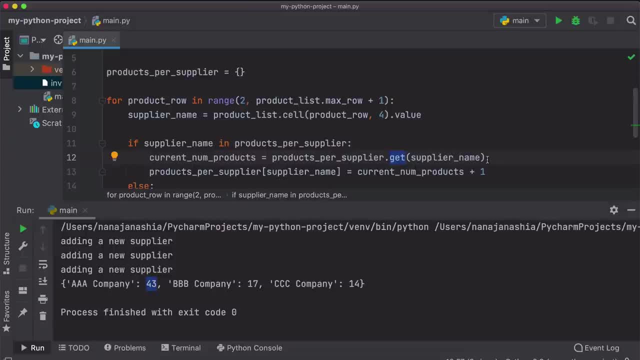 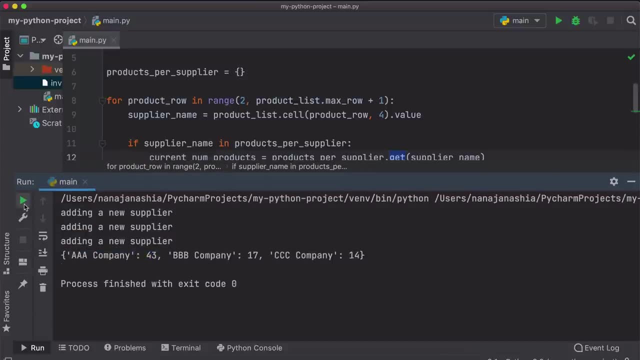 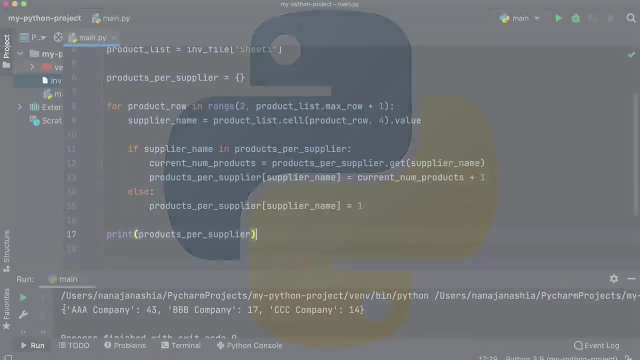 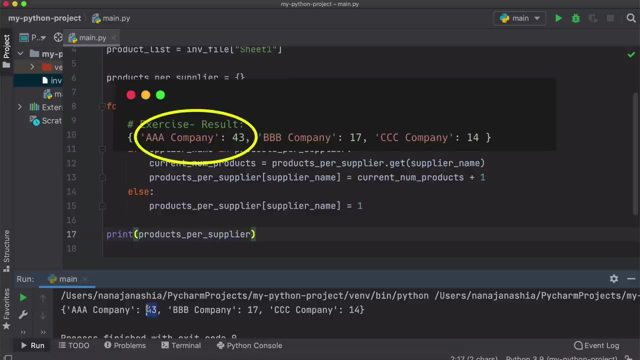 and get function is actually another way of grabbing this value out of a dictionary using the key name. Again, if I execute this, I should see the same result After the first exercise. basically, we see from which company or from which supplier we have the most product or the highest number of products. 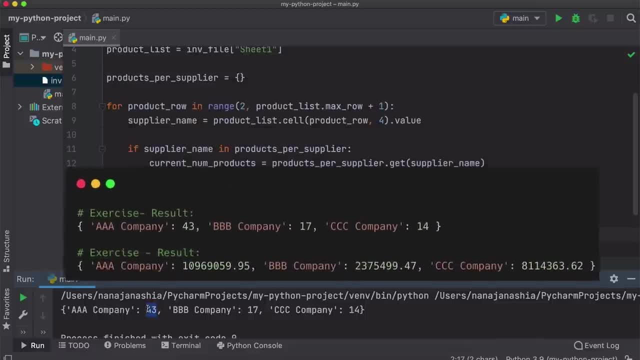 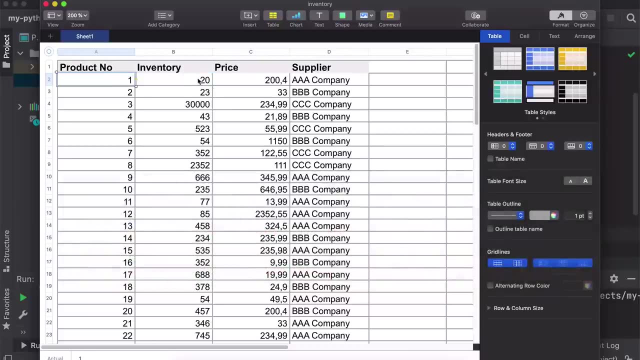 Now in the second exercise we're going to calculate the total inventory value per supplier. meaning in our list for each product we have a number of units for the product and the price. So basically, for each supplier we want to calculate how much is the total value. 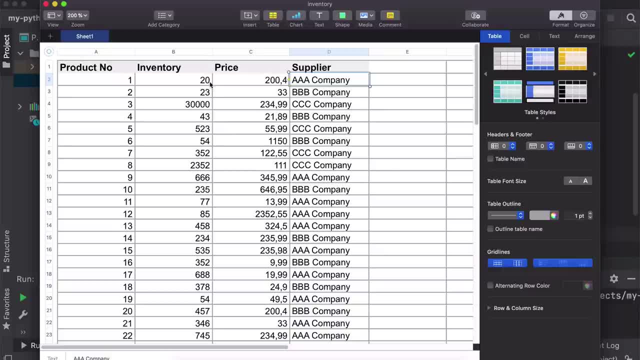 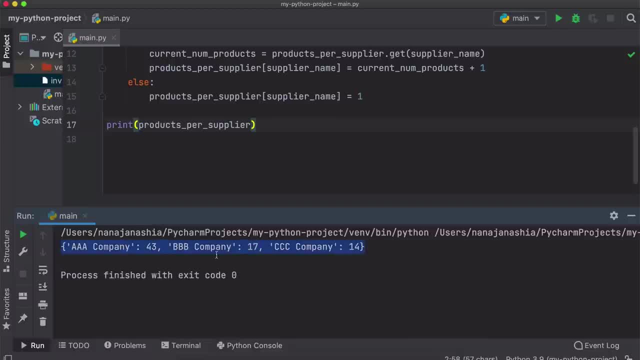 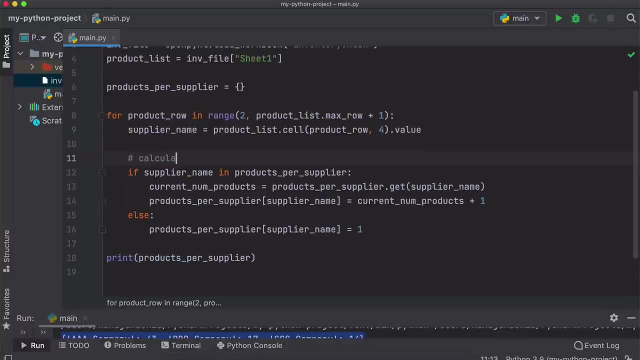 of inventory Of their products, all their products, And again, as a result, we want to create a dictionary that basically tells us that value per company. Let's go ahead and do that. So this was calculation: calculation for number of products per supplier. 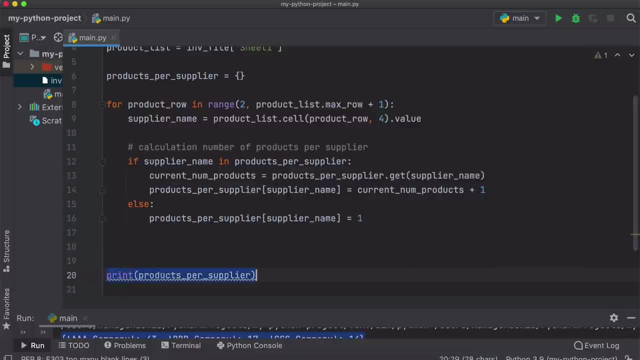 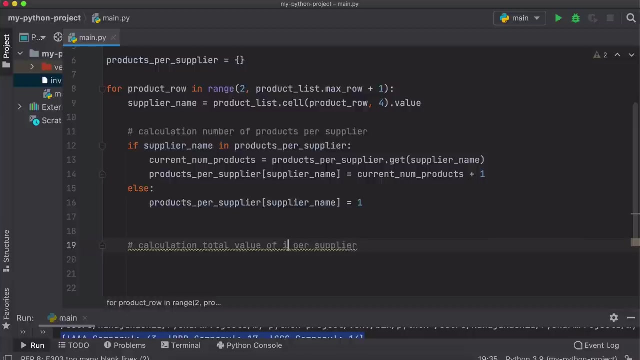 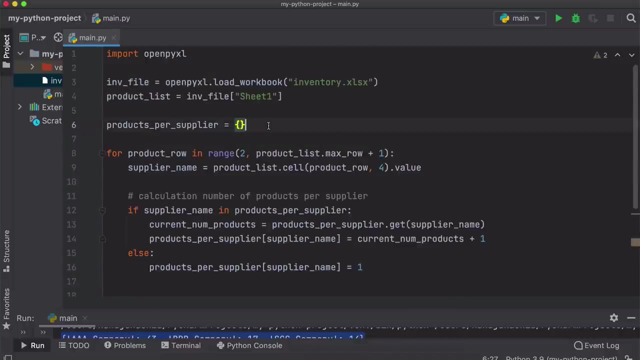 And here we're going to give us some space- And to calculation: total value per supplier or total value of inventory Per supplier. that's what we want to calculate. So, just like we did before, we're going to create a new dictionary now and we're going to call it. 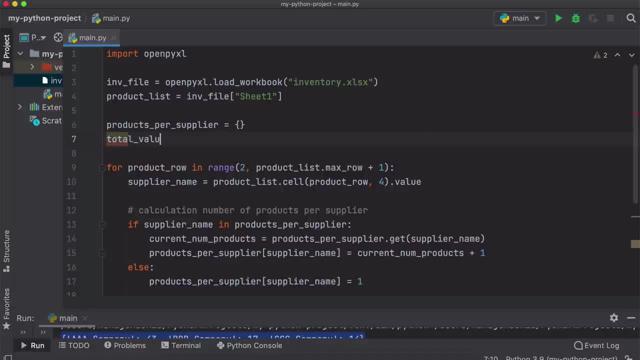 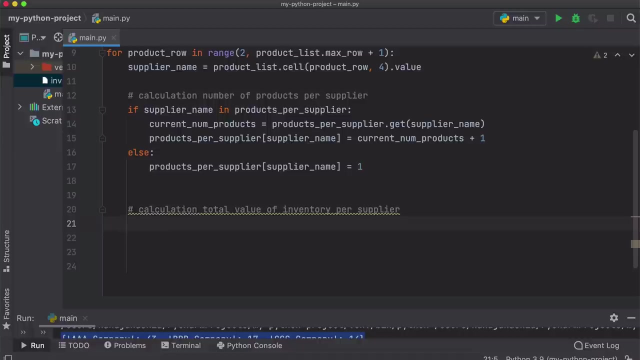 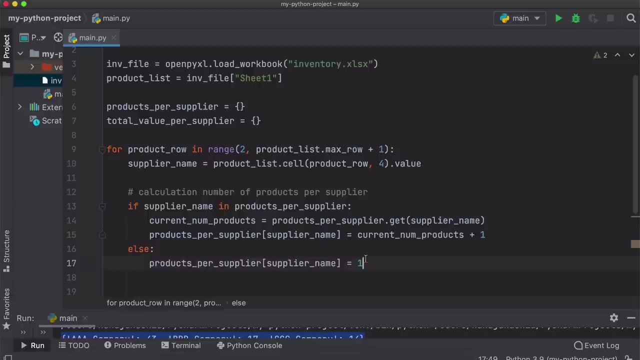 appropriately total Value per supplier and start with an empty dictionary. again, for starting in an easy way, Let's consider the first, the very first iteration, for the first supplier. How are we going to calculate for the first supplier, for the first product? So I'm going to take this new dictionary and 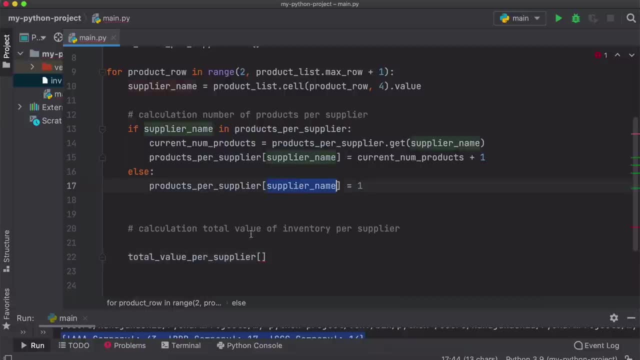 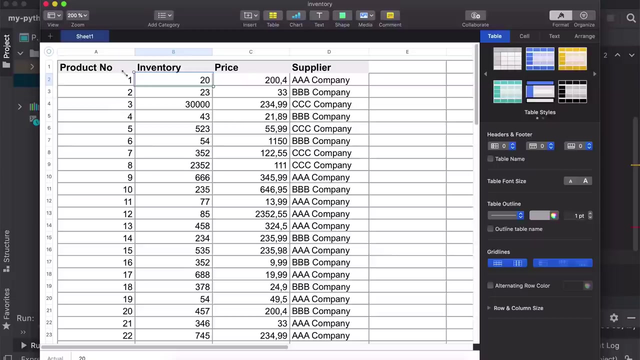 With our familiar syntax I'm going to do supplier name. So that's going to be our key, and the value of the very first iteration, for the first product, is going to be Inventory times price. So for the first product, we're going to calculate how much or how many of the product items we have and number of price. 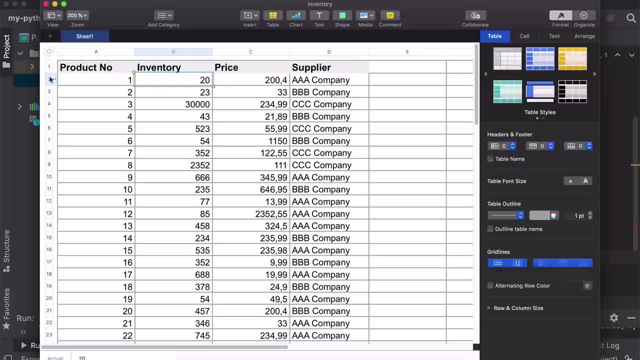 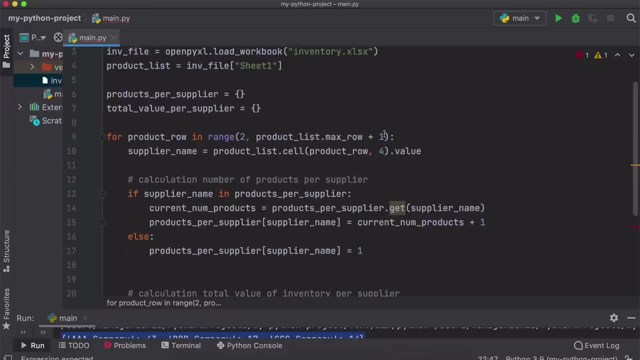 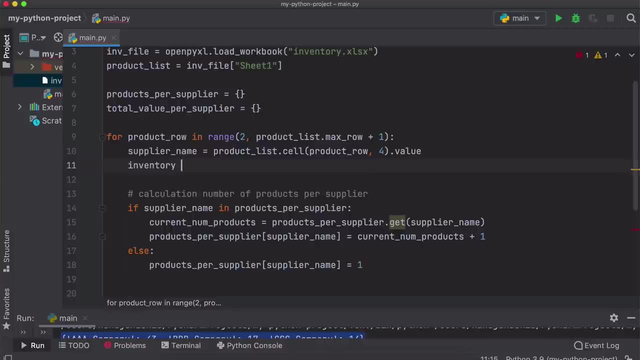 Right. That will give us value of the total inventory for that one specific product, And that means we need those two values. right now We're just getting the value of the supplier, so we need inventory. I'm actually going to copy this: so we need to sell for product row and column. inventory is on column two and value. 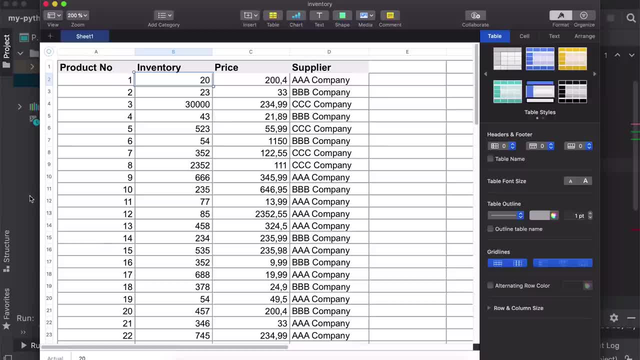 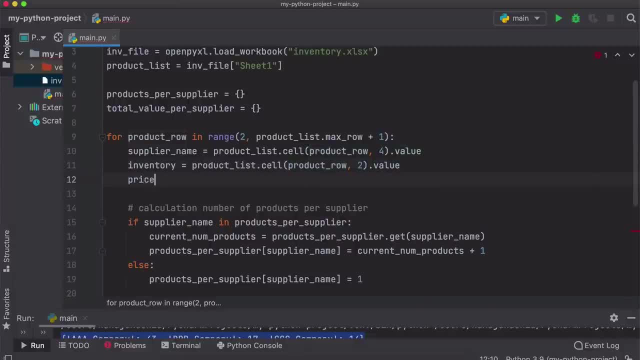 So, whatever the product Row is going to be, so for each product, basically for each row, we need always the second column, So all these values here, and then we need price, which going to be product least sell, and we're looking for. 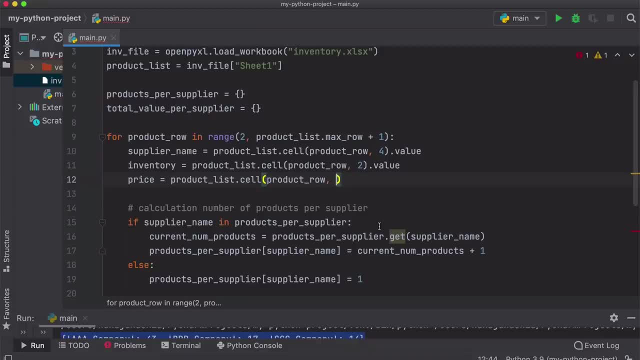 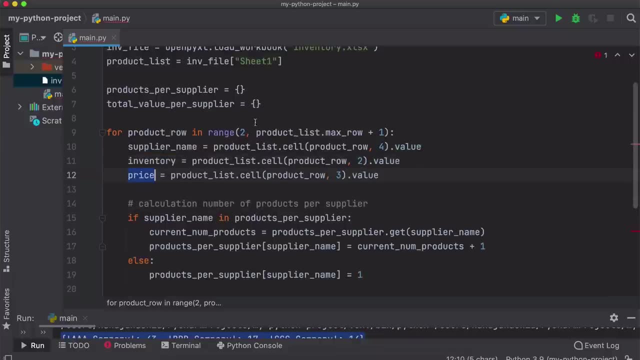 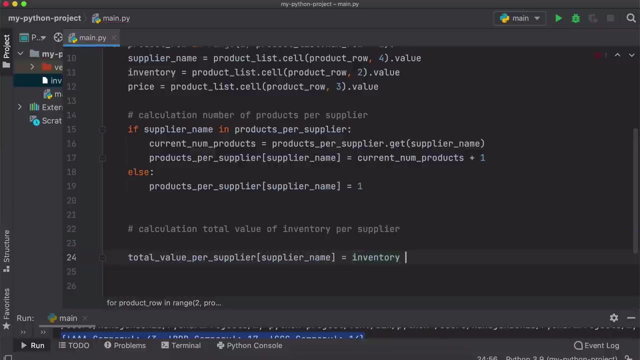 The third column for every row, Number three and value. So now we have inventory and price Per product and the way to calculate value is basically inventory, That's the number of product items times price. Very easy, That will give us the first value for the first supplier. 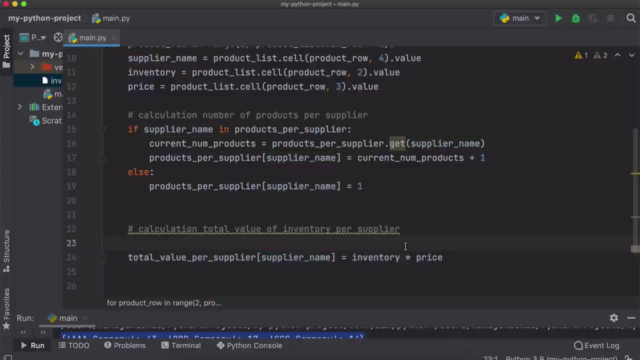 Now again the same way if we are getting a new supplier. So basically, in the next iteration, if it's a new supplier, then this line will get executed and everything is fine. However, if it's an existing Supplier that we already have in the dictionary, then we have to add to that previous value, right, instead of setting a new one. 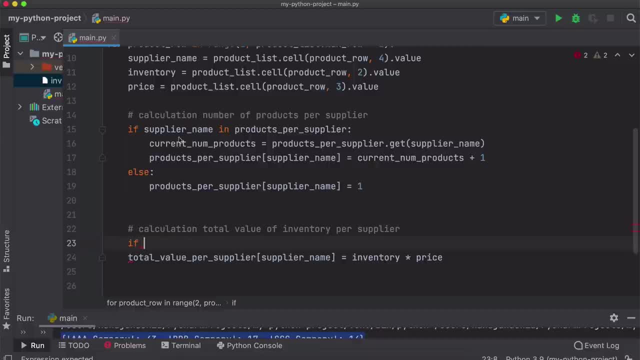 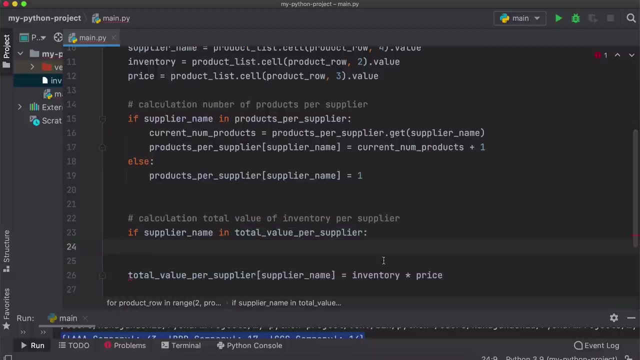 So we're going to do very similar logic as we did here. So we have the supplier name, we're checking Is it a new supplier or an old one, an existing one, this time in our new dictionary- And if it is, we're going to. 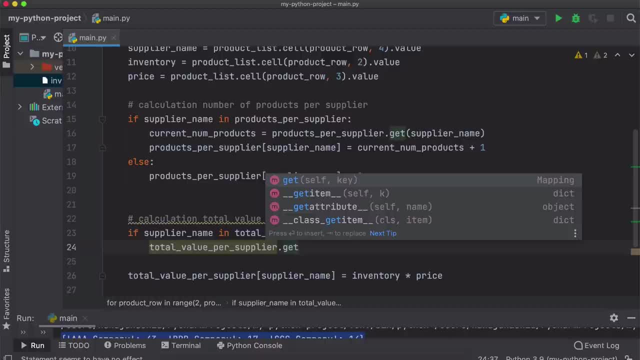 Grab that old or existing value again using this get syntax here. Existing value now is hundred. We want to add to that hundred, right? So we're going to grab that value. This is going to be current Total value, And then we're going to 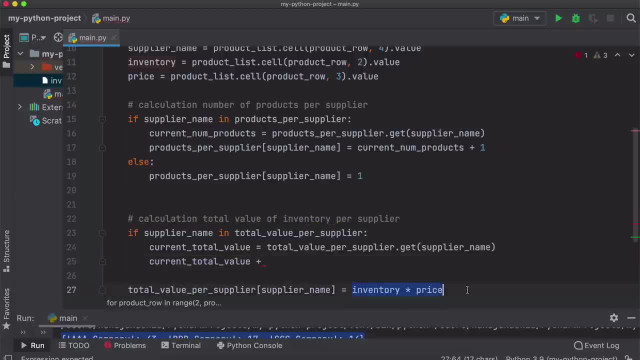 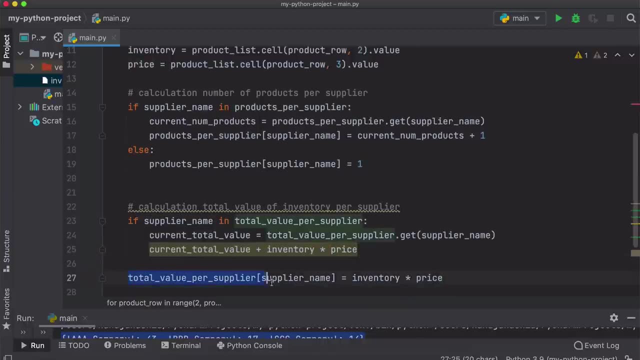 Add to that current total value The inventory value for the current product and assign it back to our dictionary. Now our variable names are a little bit long so the code kind of looks a bit cluttered, but it's easy to read. and descriptive: 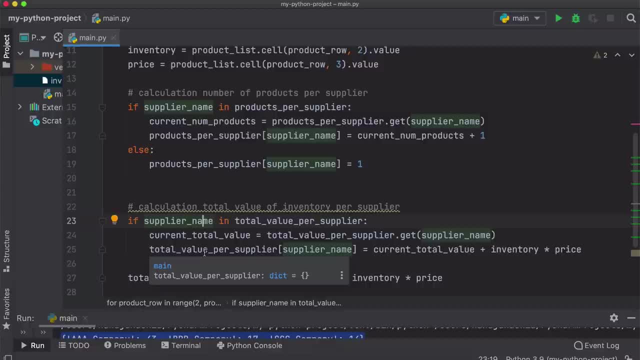 So you can also go for shorter variable names to have a cleaner code. Again, matter of taste, I usually name the variables Something descriptive, something that basically really differentiates or says what the value is about And that basically takes care of. 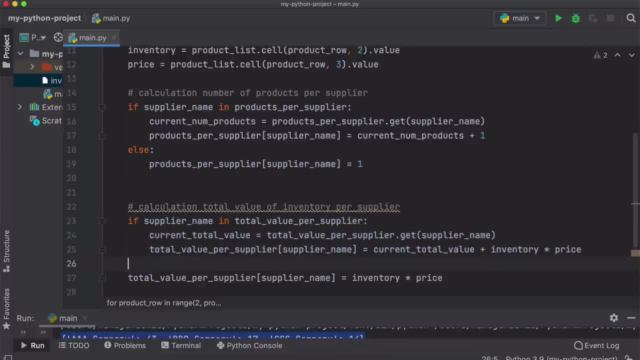 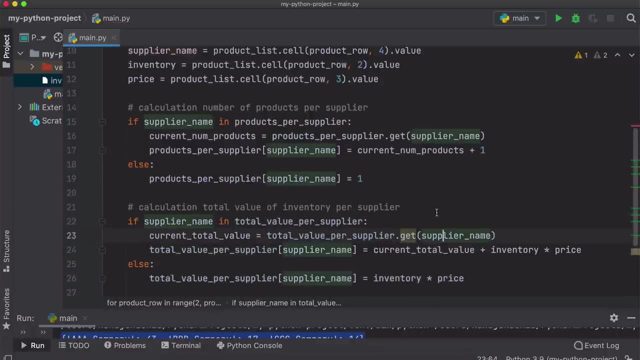 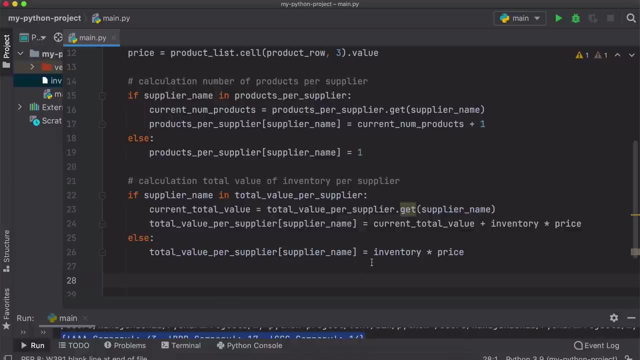 Existing suppliers or the suppliers that we already have in the dictionary. else we do this, And this is complaining about too many blank lines, so let's fix that, And that's basically our logic. again to go through it: once for new supplies, Once for new supplies. 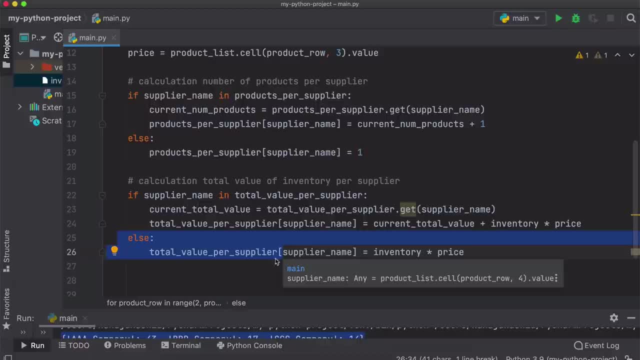 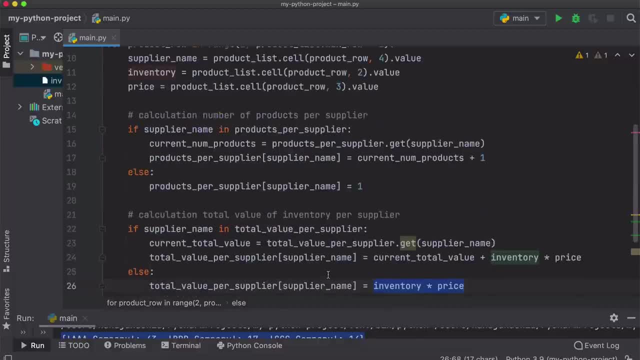 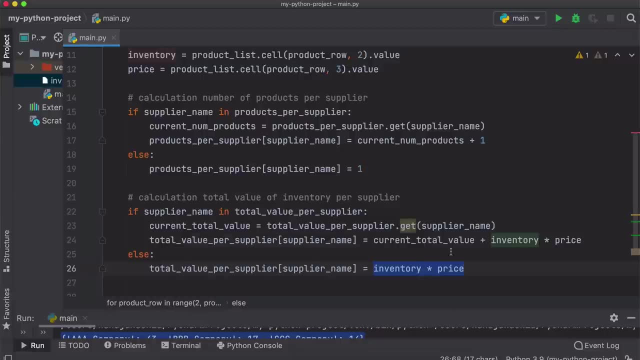 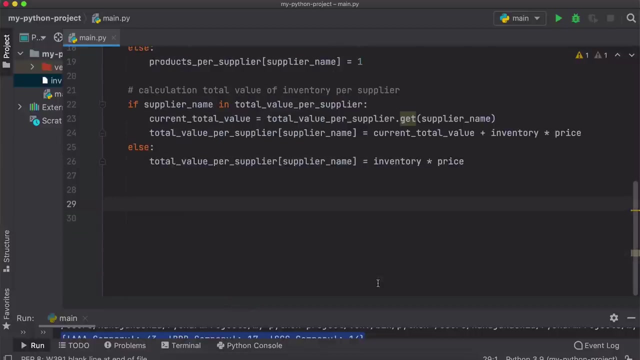 Because, remember, we are iterating through products and then every time a new product iteration happens for the same supplier, we basically just add an inventory price or total value for that specific product, for what we already have in the dictionary. So now let's again print out our dictionary. 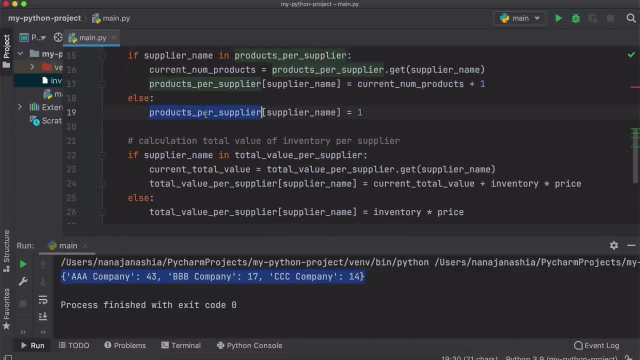 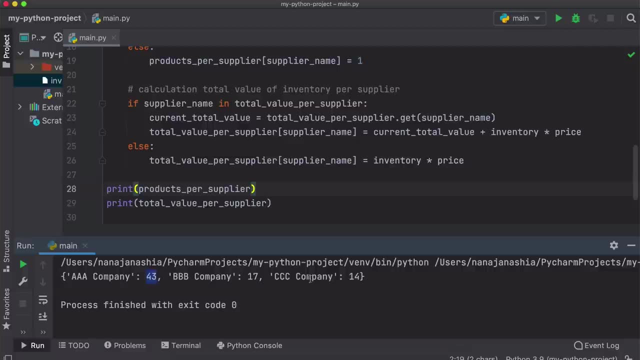 Let's actually print both values. So the first dictionary is this one right here: Supplier and number of products. The second one is going to be supplier and total value of all the products they have in the inventory with us. execute, and there you go, we have both dictionaries. 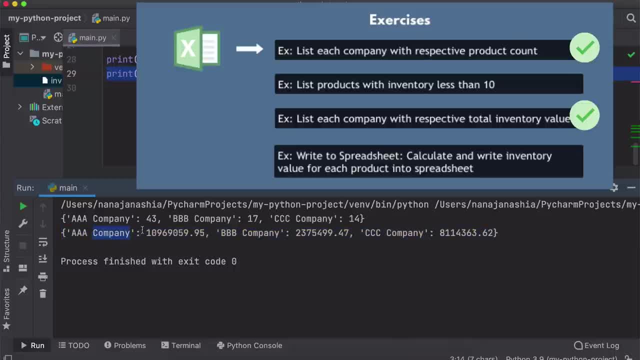 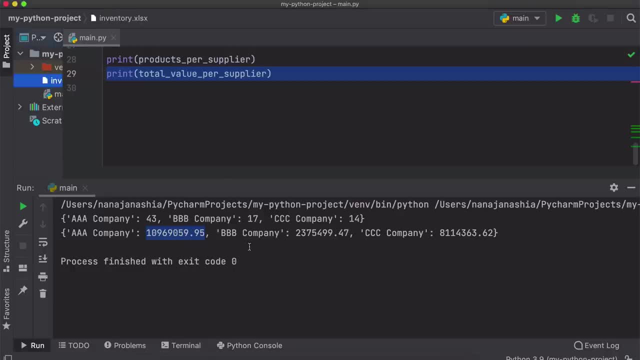 printed here and here, you see, for each company we have the value in price, basically right here, the value for the total inventory of all the products they have on this list, and we see that value per supplier and the values are decimal numbers with cent precision. so 95 cents, 47 cents, because the prices are 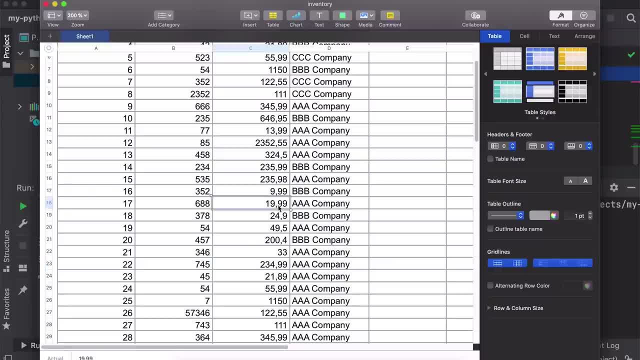 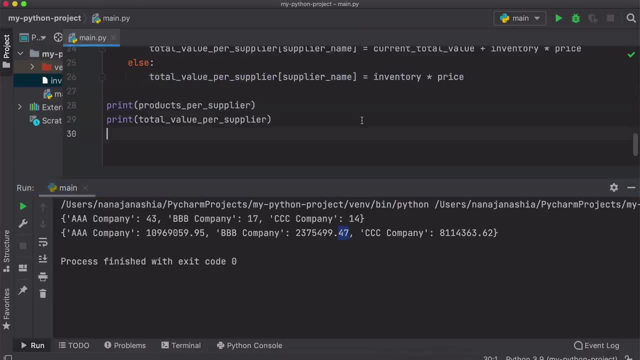 obviously like this as well, and, if you're wondering, this comma here is actually a German format for number precision, so this is going to be actually equivalent to English dot, and we don't have to worry about this, actually, because Python reads it and interprets it correctly, so no problem. 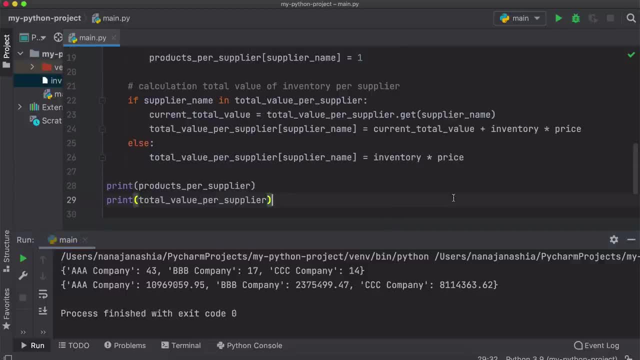 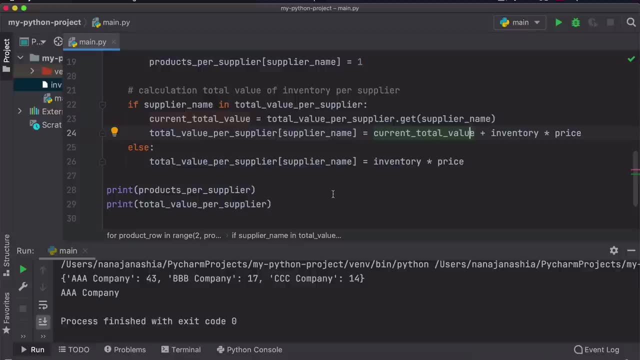 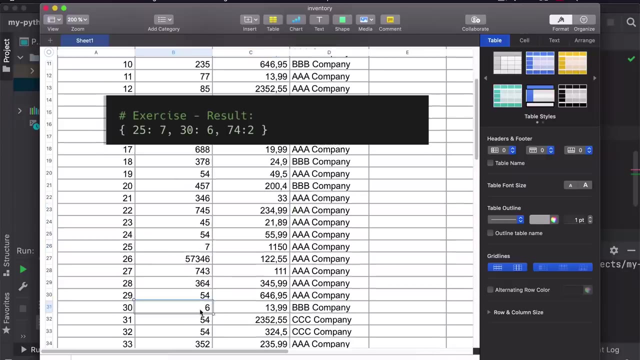 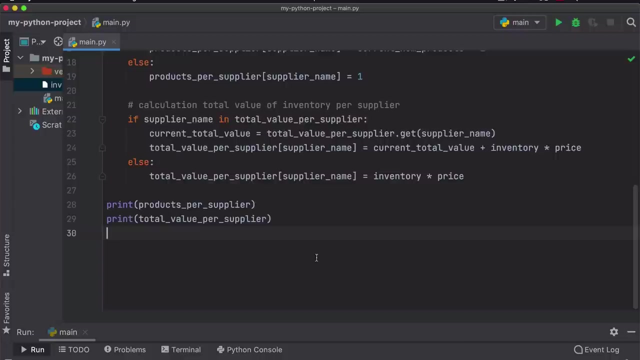 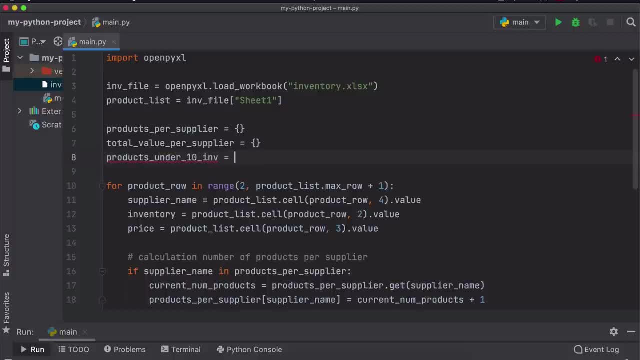 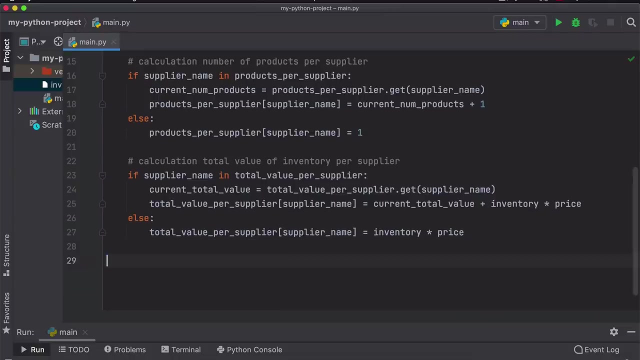 Inventory under 10 like this, and the value in the dictionary should be the product number, which we have in the first column, and the inventory count. So let's get rid of this print statements and let's do calculation. We can do logic- products with inventory less than 10.. 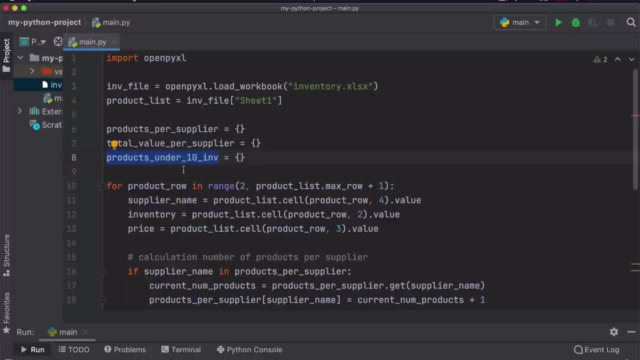 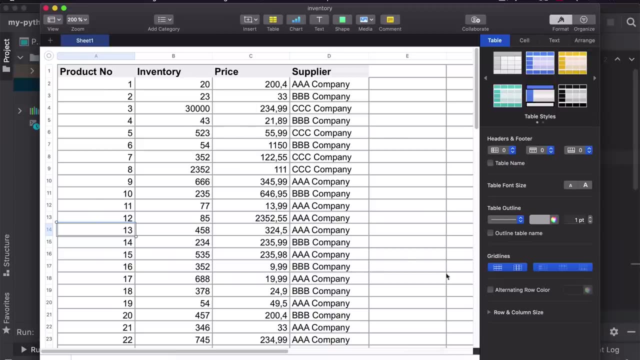 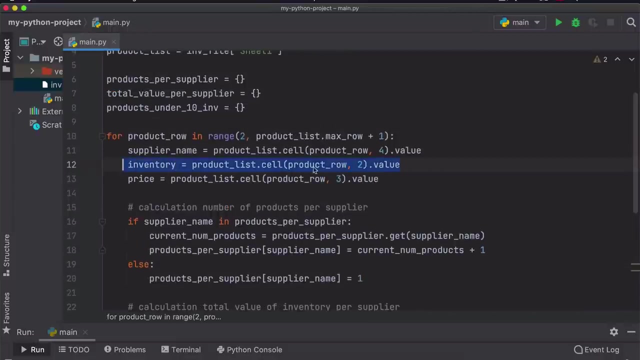 So basically, as I said, for each product which has inventory under 10, we want to print out or we want to save in a dictionary the product number and the inventory count. So we have the inventory count already, the value from the cell. 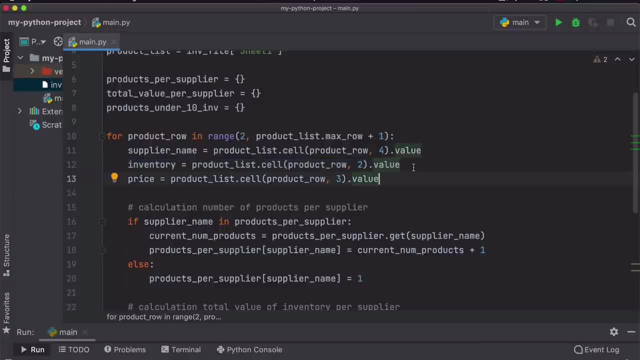 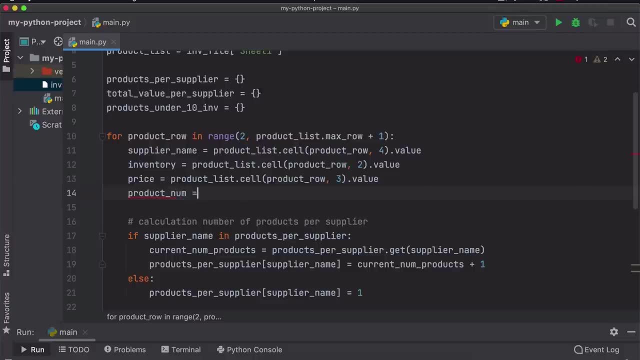 but we don't have the product number, We're not accessing it, So let's actually do that Product number, And we already know how this works. This is going to be the first column right, This one here, and this gives us product number. 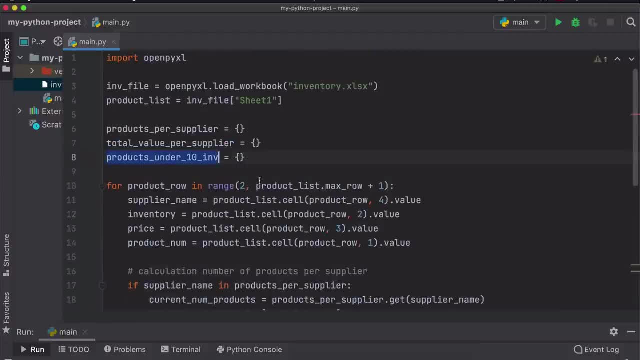 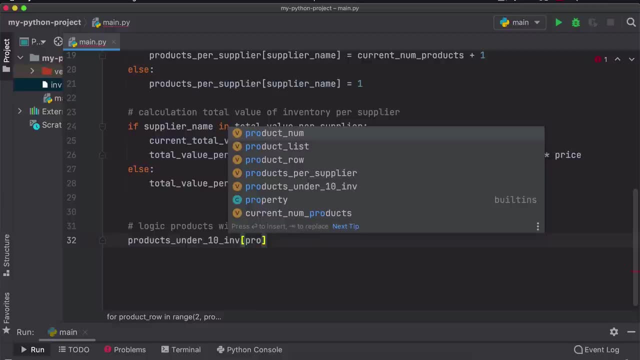 And now in our dictionary- products under 10, we want to add value like this product number and it's going to be set to value of the inventory like this. However, we don't want it for every product. We want it only for products with inventory less than 10.. 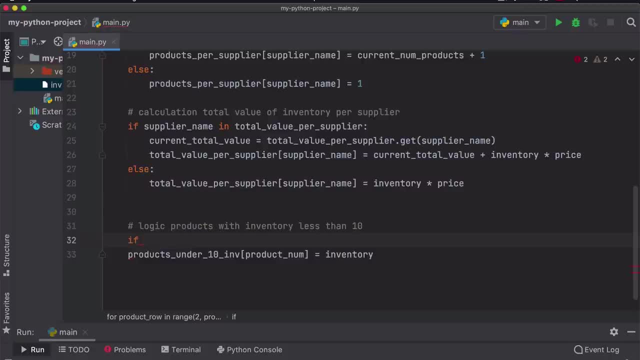 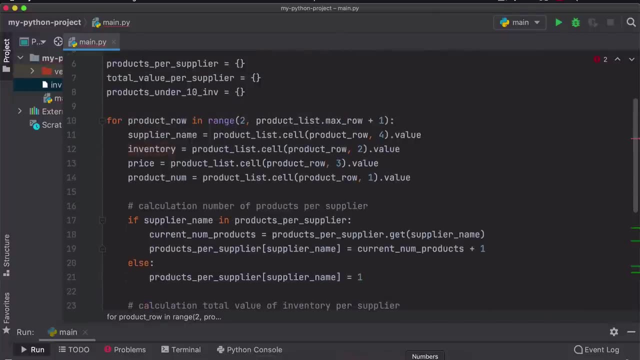 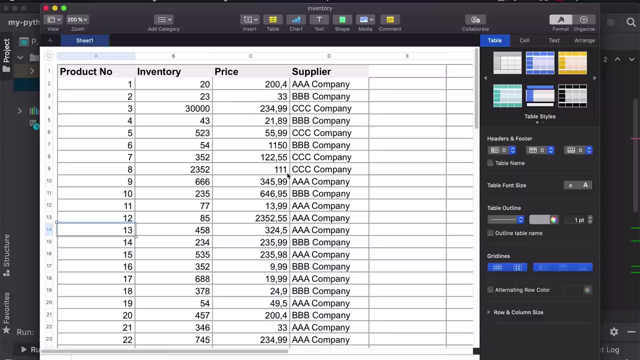 And that's going to be an easy if conditional here, If inventory again, remember this logic. all this logic happens for each product row, right? So all these get executed for each of these rows. So basically, we have inventory Number on each iteration for each specific product. 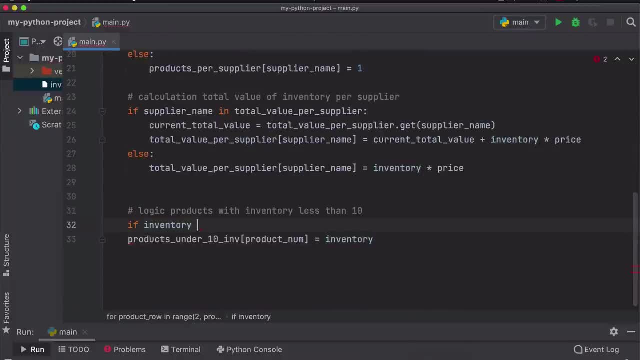 And that's why we can just say if inventory is less than 10.. So if the value on that specific row is less than 10, we want to add that product, the current product that we are iterating on on the list, and set the value of inventory as well. 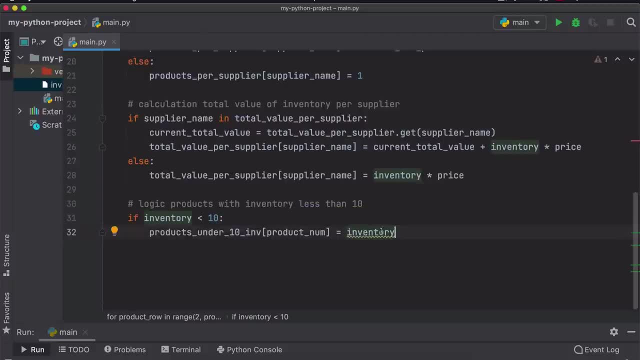 Again, we have some complaining here because of the lines, and this Will be the logic basically, And a use case for this type of calculation would be: if we find products that have inventory which are less than 10, means we need to reorder them, right, because they're going to get out of stock soon. 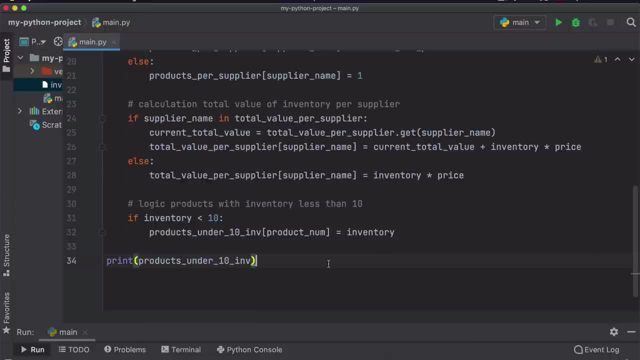 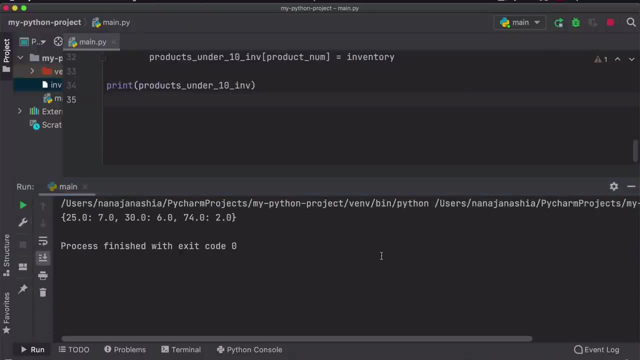 And now, at the end, let's print the list of all the products that have inventory less than 10.. So I'm going to execute it And here we have the product number And inventory counts. So we have three products, basically, which have inventory less than 10.. 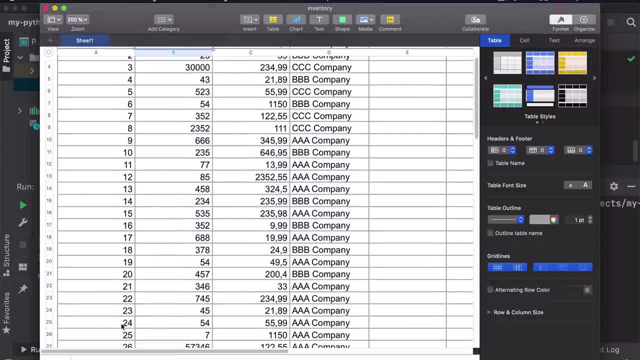 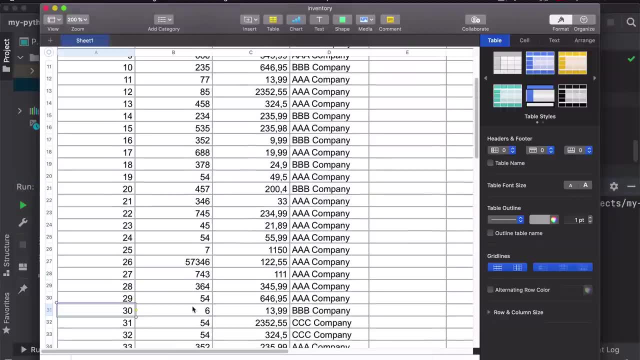 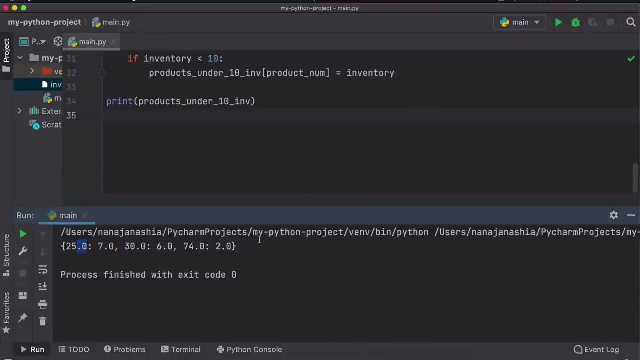 And let's actually check that product number 25 right here, which has inventory of seven, and product number 30, inventory of six, And the third one as well. Now you're probably wondering why we have this dot zero here, because by default those values are interpreted as float. 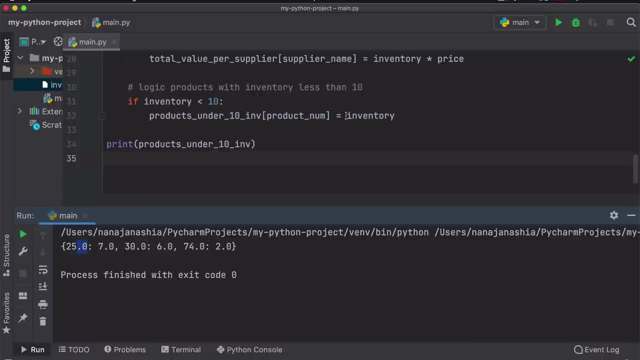 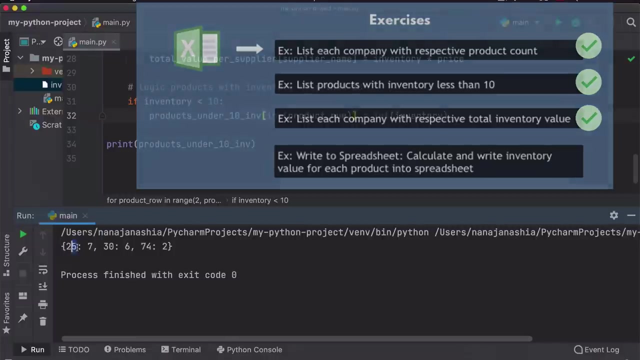 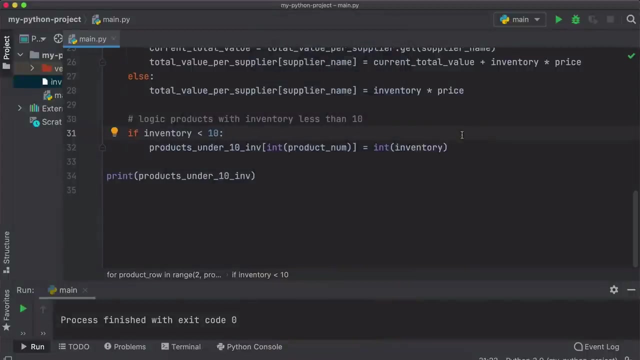 Numbers and not integers. If we wanted to, we can actually fix that using the integer function in both cases, like this, Let's execute it again And we have the integers and not floats. And finally, as a last exercise, what we're going to do is: 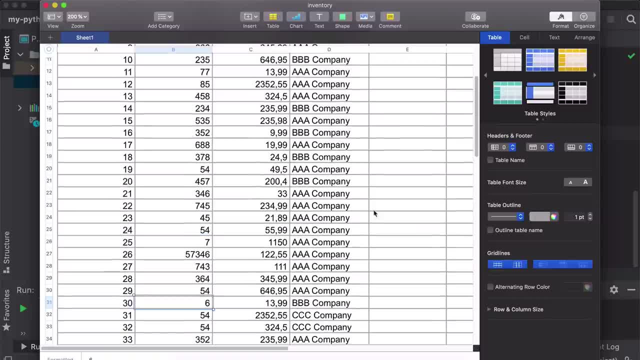 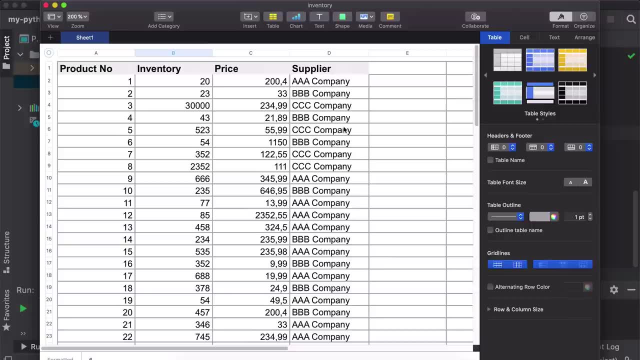 we're going to actually add some value inside that spreadsheet. till now, We have been reading the values and doing some calculations and just printing the result on the terminal. as the last exercise, We're actually going to create a new column here for every row. 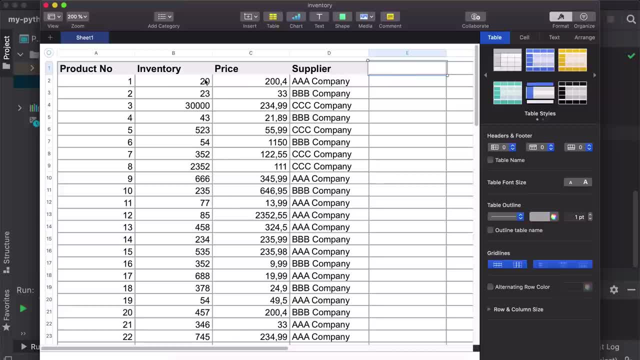 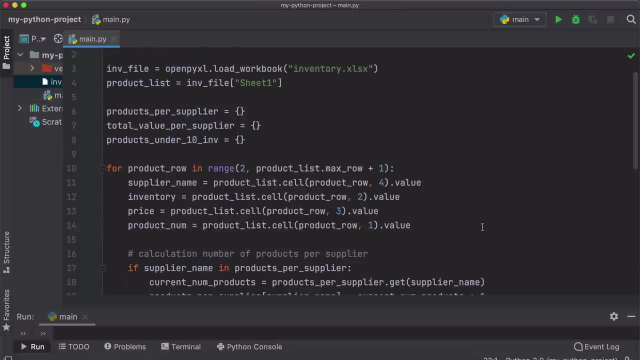 and we're going to calculate basically the total price of inventory, the number of units times the price, And we're going to basically set the value for each product, inventory multiplied by price. So how do we add a column or how do we make? 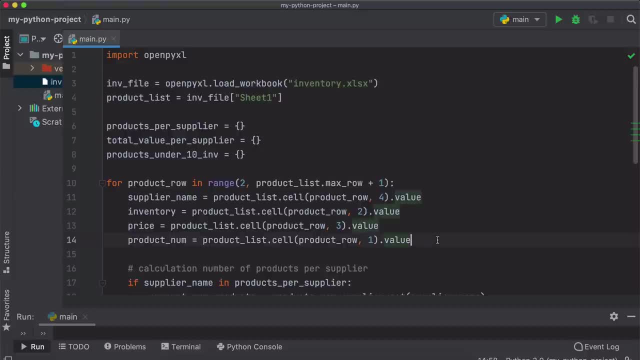 Changes to a file. It's actually pretty easy. The same way as we were grabbing the value from this file and basically reading the values, we can add values to it and add columns and rows, et cetera. So to add a fifth column. 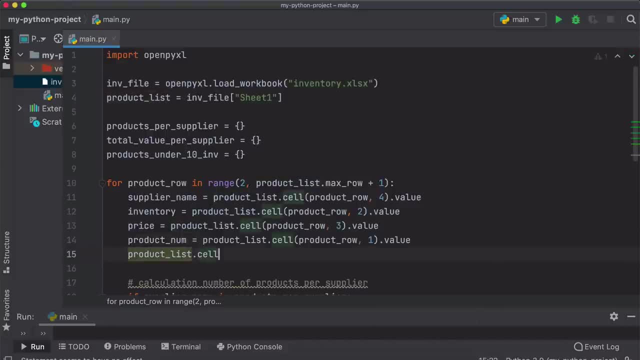 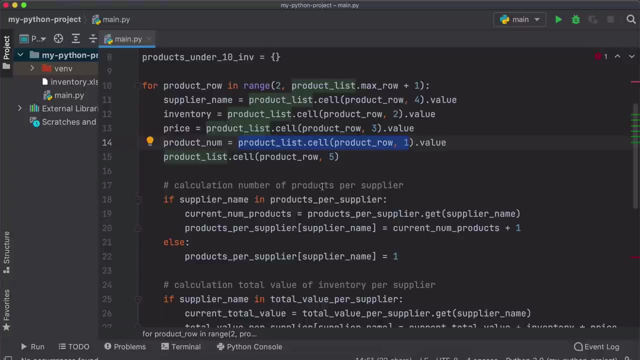 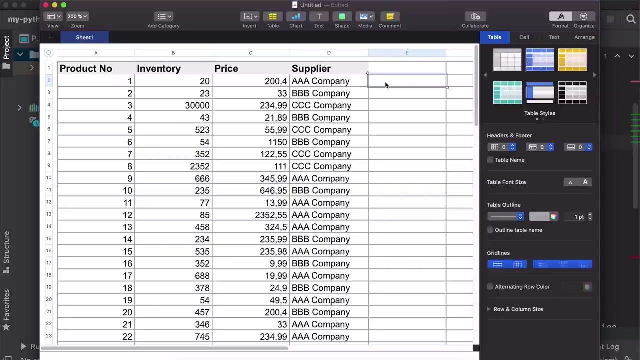 we're going to do product list- sell product row. This is going to be the number of the row and a column number. So the same way we access the cells for all other values, we can basically access the cell on column five. 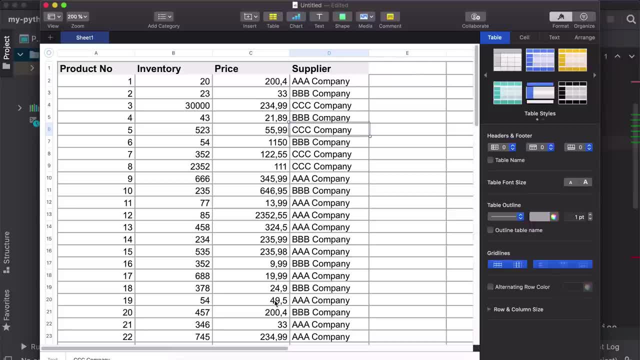 which has an empty value, right? So we're not actually creating a new column, We're just grabbing a value of a column five which happens to be empty, and we're overriding that value. And we could do the same actually for any other columns here, right? 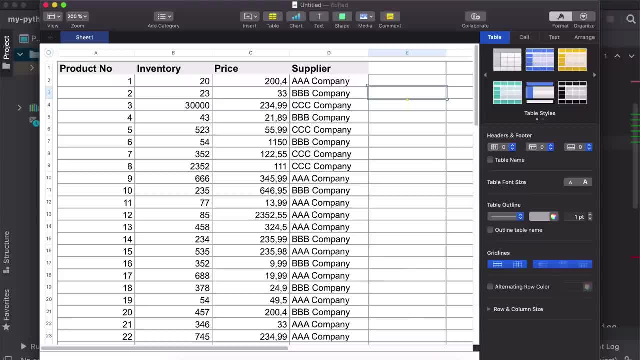 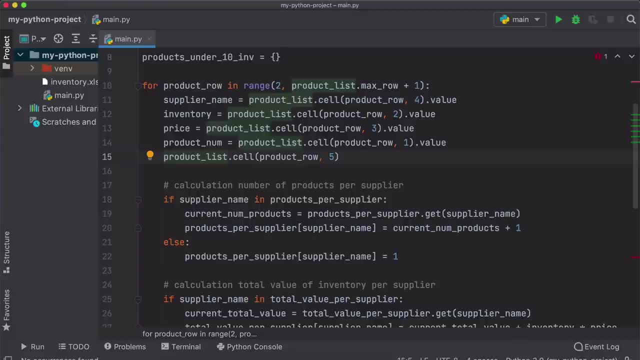 We can override all these values if we wanted to. So that's basically what we're doing. So we're grabbing that. So we're grabbing that. So we're grabbing that cell, and we can now save it into a variable. Let's actually call it inventory. 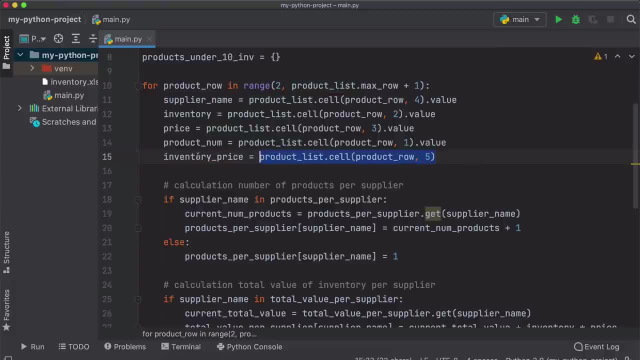 price. So now that cell is saved into that variable so we can reference it. And note here that I didn't add dot value at the end, because if we want to update the cell we need the whole cell object Right, So that we can actually set a value on that. 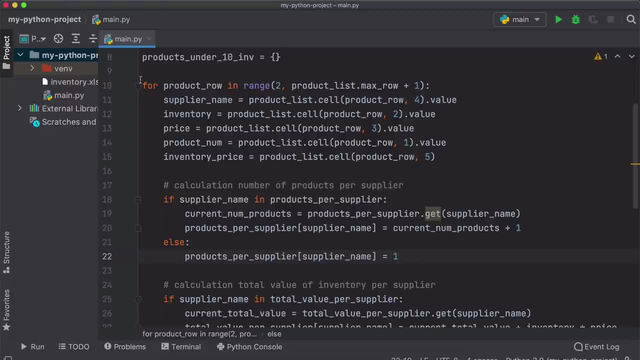 So how do we set a value for that? So how do we set a value for that Specific cell? So again, know that this is iteration. So for each product, bro, the value will be set. So how do we set the cell value? 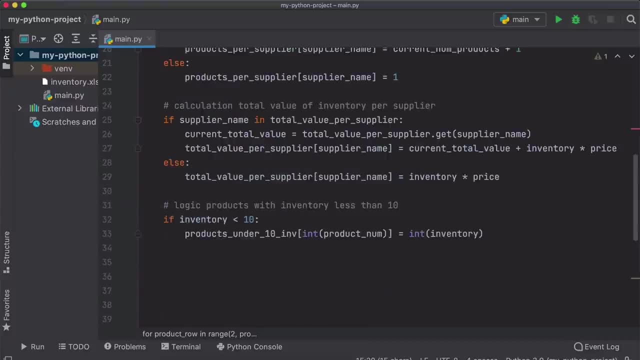 I'm just going to grab this variable here- Inventory price, which is representing the cell in column five, for each iteration. and right here at the end, because this is our last exercise, Let's write: this is a logic, or basically add value: Yep. 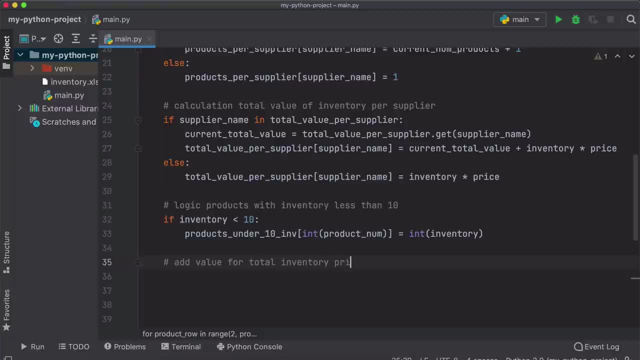 Right, total inventory price, and the way we set the value in the cell is dot value equals, and the calculation for that is actually very easy. we already did it here: inventory times the price for that specific product and that's it. so we're using that dot value here in order to set the 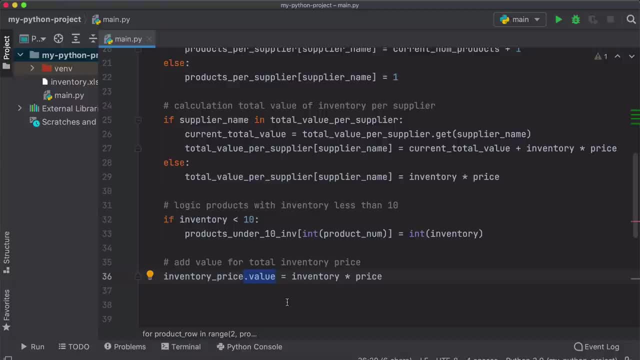 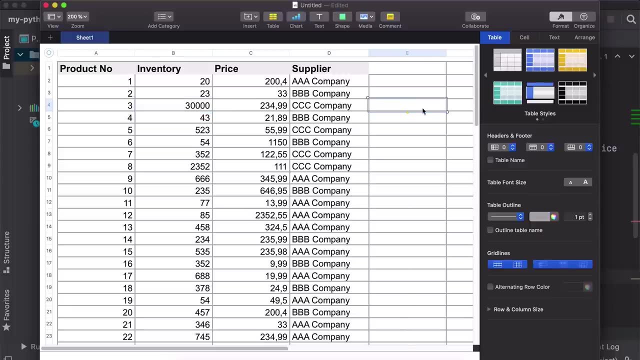 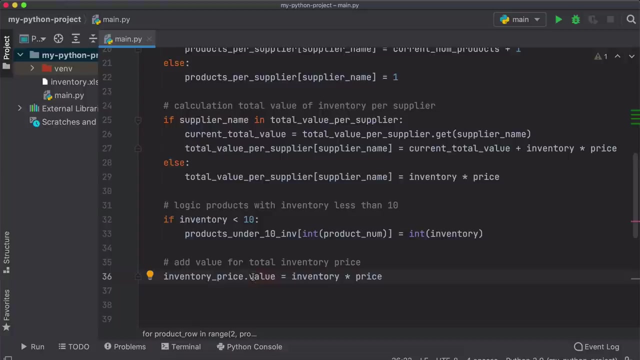 value instead of grabbing the value, and that will actually update and add this calculation or result of the calculation on each line on this column. but note that this will only change the value in a temporary file, but it's not going to save anything, right? so what we want to do at? 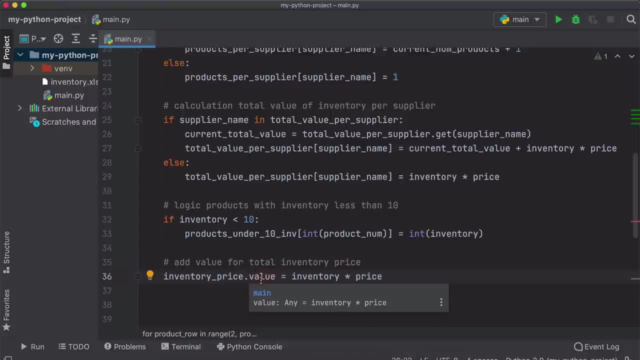 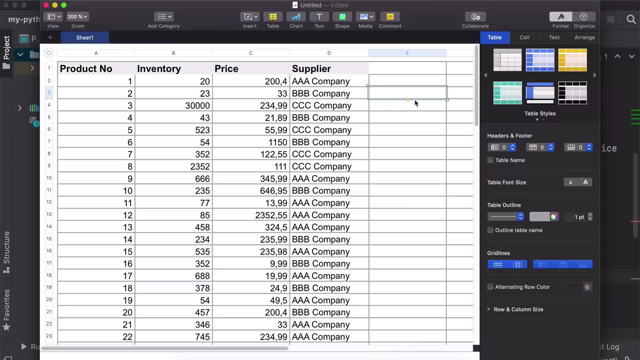 the end, if we want this change to persist, to actually be saved, we want to explicitly save the file. so, for example, if I manually did something here, added some value, I would need to save it here as well. right, so that's exactly what we need to do here, but programmatically, using Python. so how do we save a? 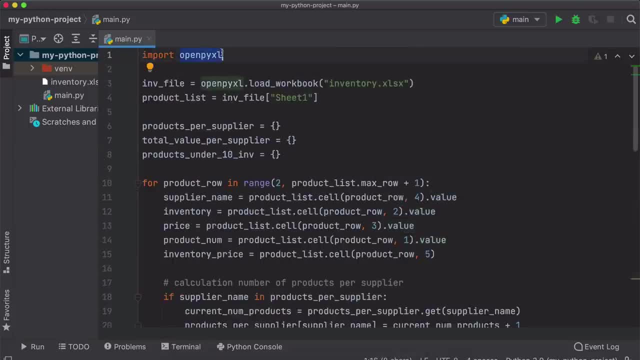 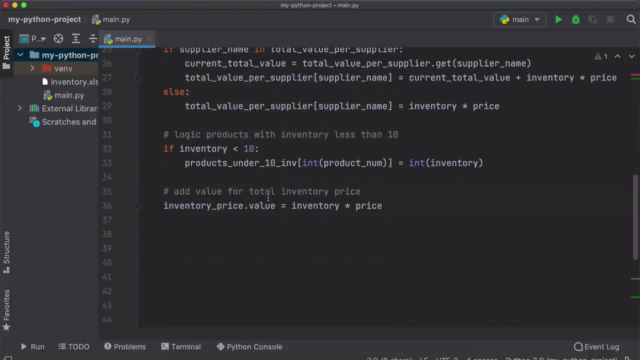 file using Python. again, this package or this module that we use here also gives us a function that we can use to save the file and since we're doing an operation on a file and not a sheet, here, we're going to grab that variable in file and here at the end we're going to call a save function on it and this will save the file changes. 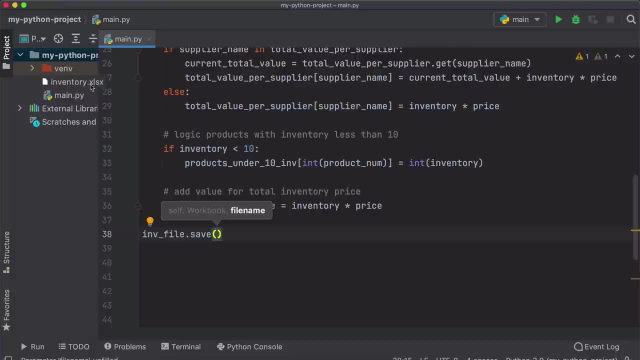 however, we're not overwriting the same file, the existing inventory file. we're creating a new one and because of that we need to provide a name of the new file that is going to be created with the save function, and we're going to call that file, let's say, inventory. 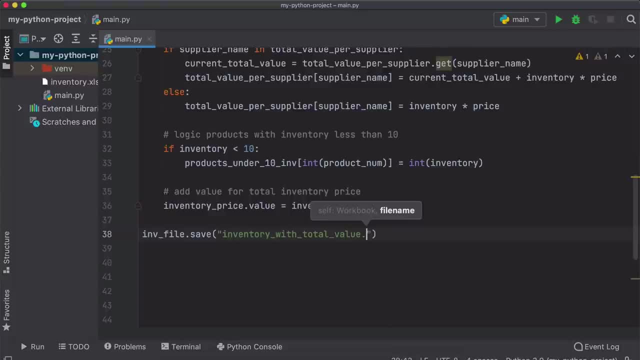 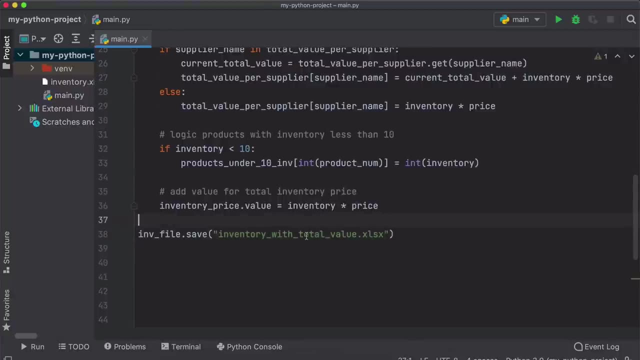 with total value and extension- the same extension as we have here. so this line will now save the changes and create a new file from the original one which has these values generated, basically. so, now that we are done with the fourth exercise, let's actually print out everything. 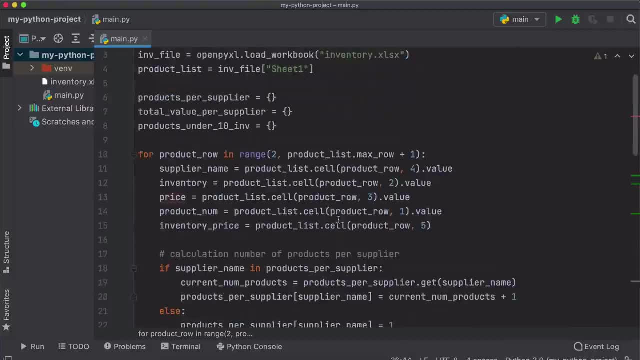 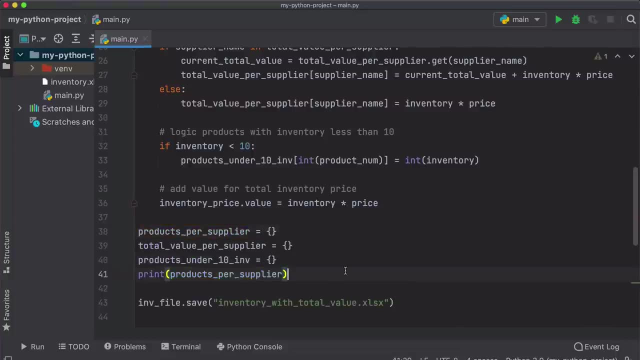 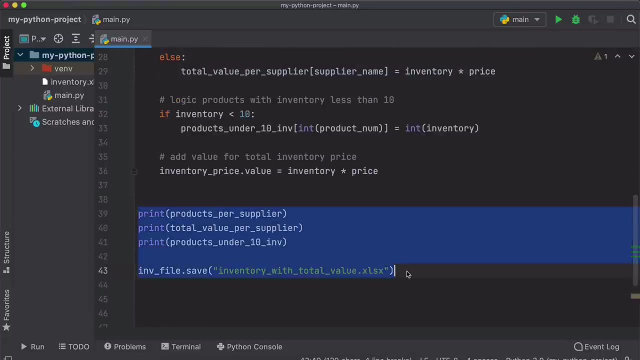 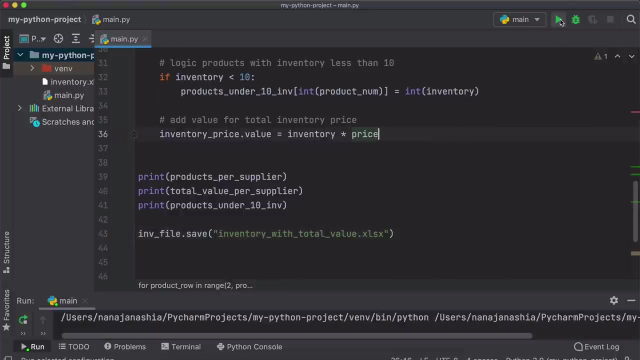 that we've done so far. I'm gonna take all those values. so this is gonna be execution of all our logic: printing these three dictionaries here and then updating the spreadsheet file and saving it into a new file. so with this, let's actually execute our programme and see what happened. first of all, we have all those three dictionaries listed here. 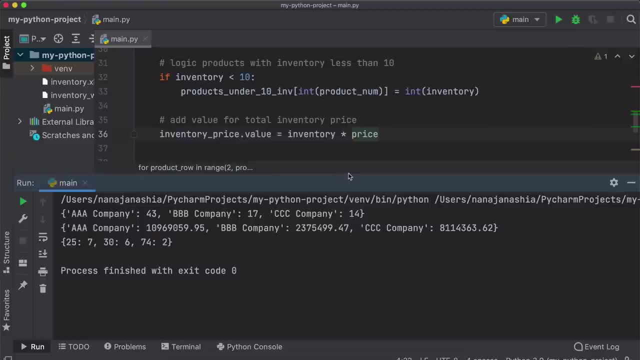 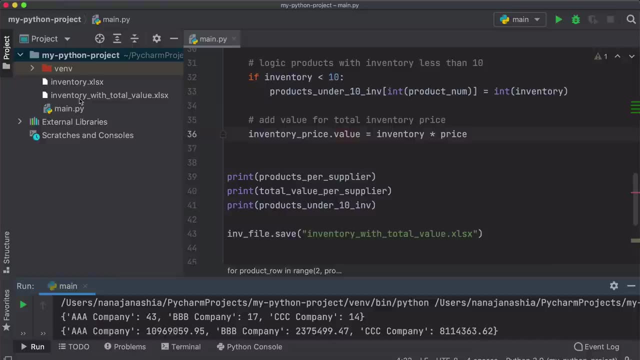 or printed here with the values. and if we pull this aside here you see a new file got generated with the name inventory with total value, and if we open this file we should see that there's a new file and it shows up immediately in the model name field. so if weく Giulo isszy- I don't know if you use this- 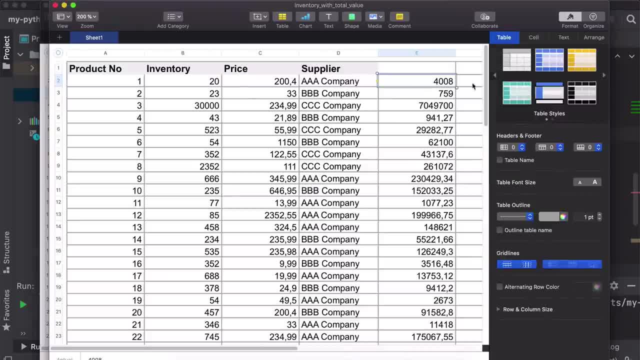 factor, but we're starting to work. I'm going to pass this over to angles is the process. we wanted to make an update. we wanted to actually save the file, so first we do is to express as much video feedback file. we should see that for each row and new column was. 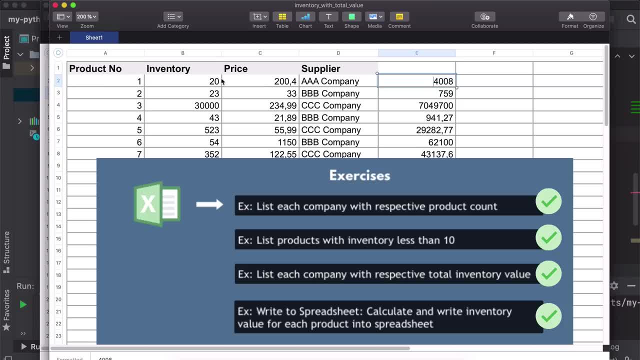 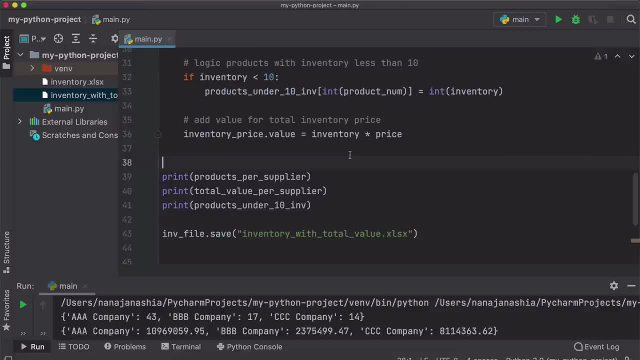 generated and filled with values, which is calculated for each product inventory in price. So that's basically our project. That's how you work with files in Python, specifically with spreadsheet files, And, as I said at the beginning, this could be actually very useful automation logic when you're working at a company. 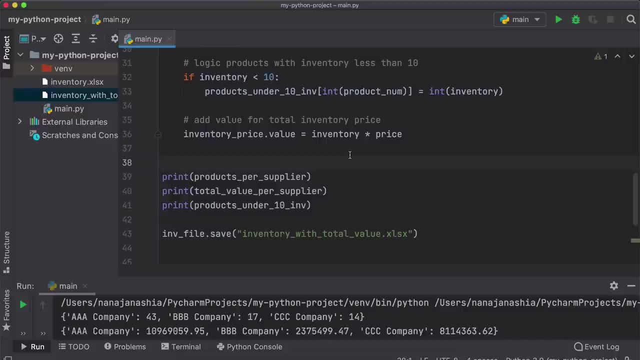 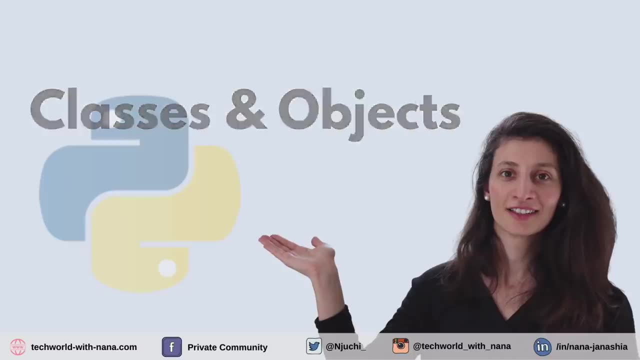 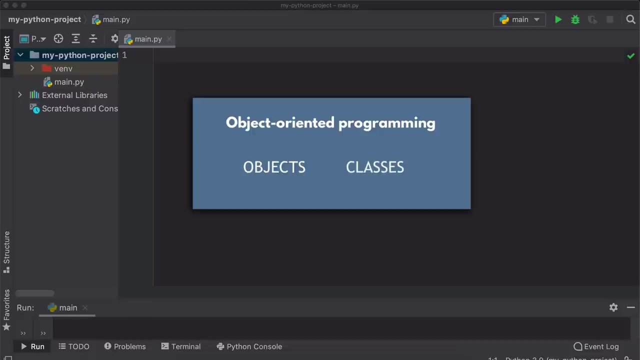 where there are lots of Excel files or spreadsheet files that employees have to work with and manually update stuff inside. In this part we're going to learn the concept of objects and classes in Python and generally object oriented programing. Let's consider an example of an application with lots of users. 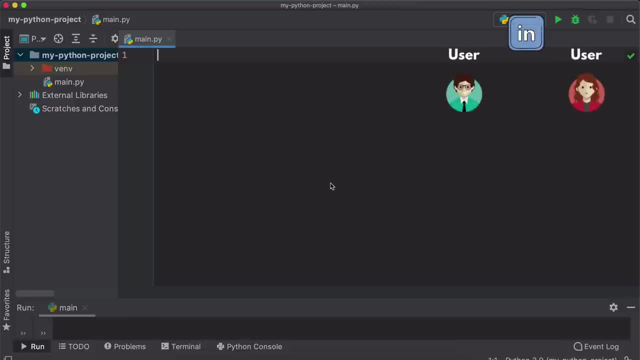 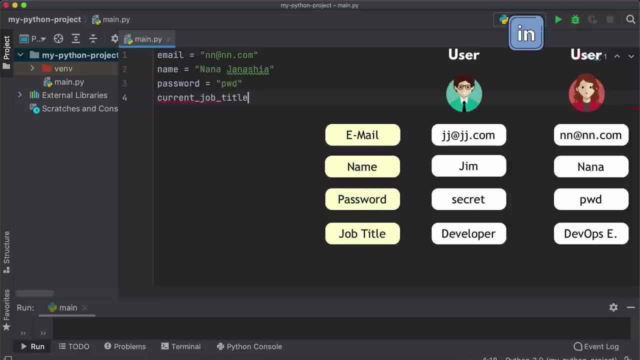 for example, LinkedIn. Right, We have users and each user will have some information, For example email address, name of the user, password, maybe a current job title, Work experience, a set of skills and so on. Right, So each user will have all of this information, but obviously, 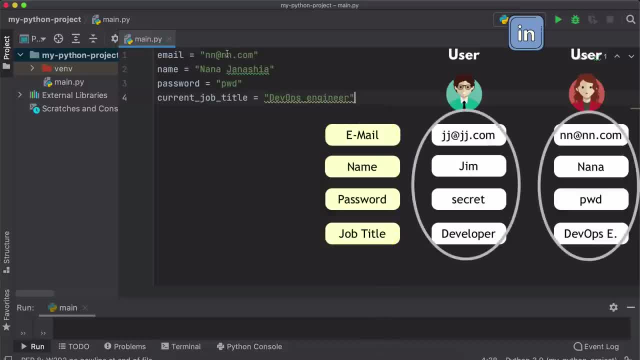 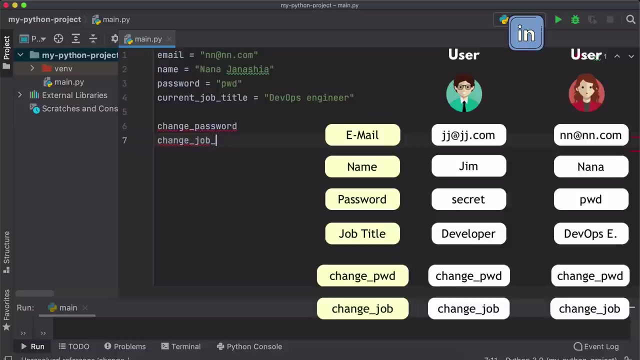 the actual values, the actual information will be different for each user. In addition to that, users are able to do something with their own information Right. So, for example, a user can change their password, change their current job title, add a new skill and again, basically do stuff. 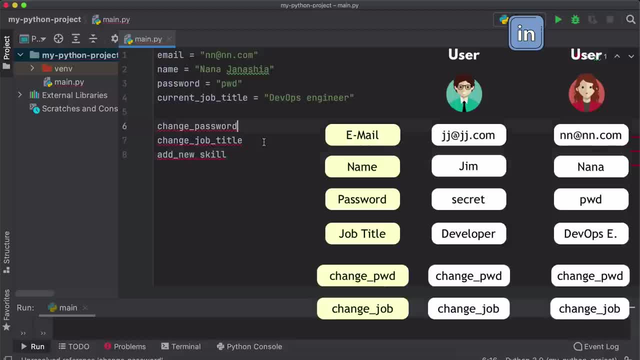 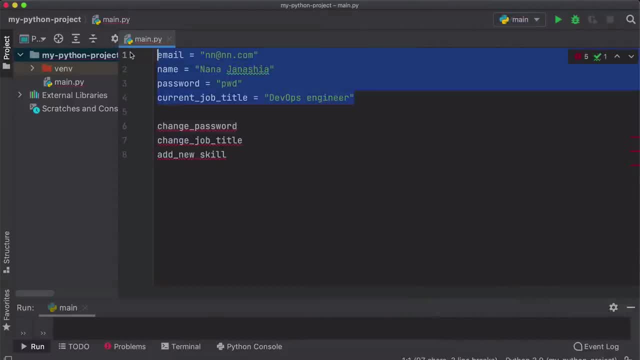 with their own personal information, and our program will be able to handle this user information Plus User changing their information Right. So this will be user data and in order to do something, so to perform some action, we would have functions for that. 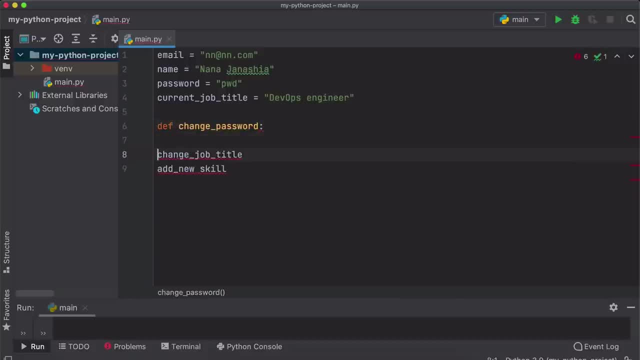 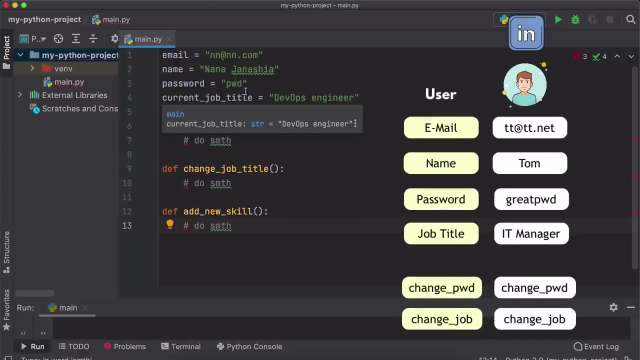 Right, So all of these will actually be functions. However, as I mentioned, every user will have their own data And whenever a new user basically registers for an application, all this data should be gathered for that new user and saved in The application. 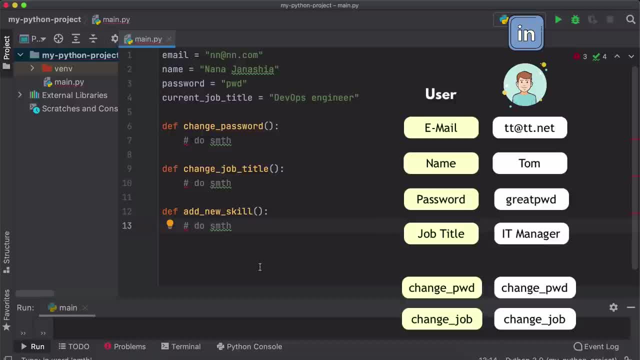 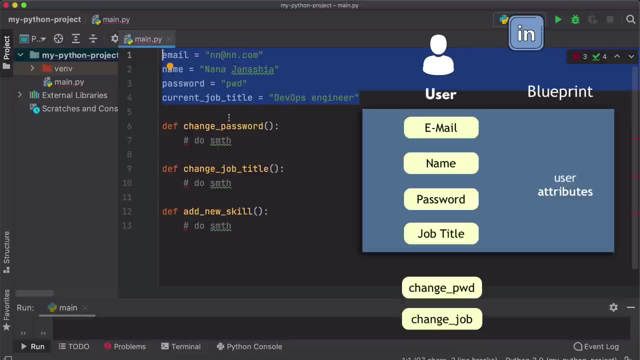 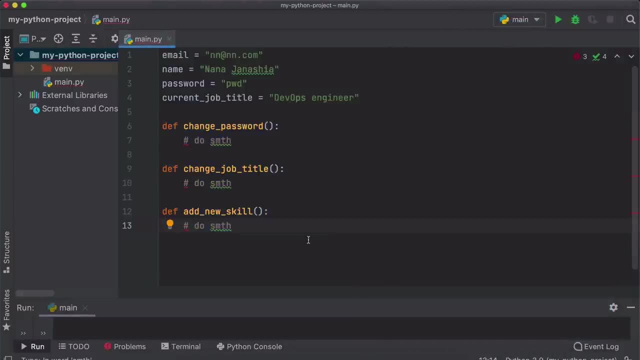 So basically that means that in our program we need some way to define kind of a blueprint for a user for all the data, user information and user behavior, Right Things that the user can do in the application, because if we have 1000 users in our application obviously we can't write. 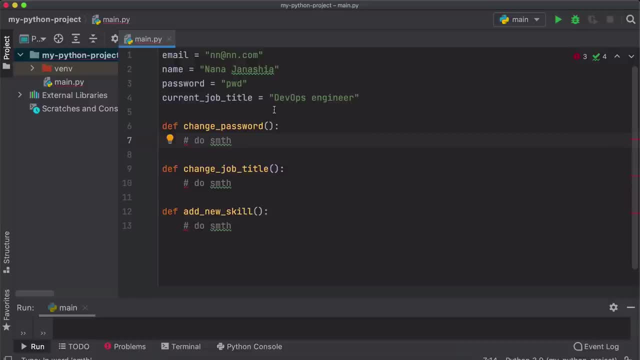 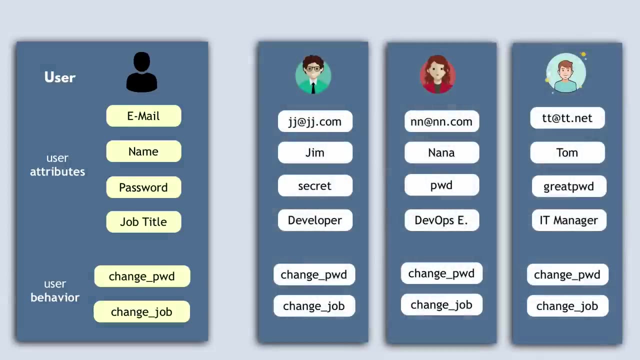 the same logic and same variables thousand times. Right, We want to have a blueprint once, and then we can use the blueprint for all those thousand users, and that blueprint for a user is called a class and a specific implementation of that blueprint is called an object. 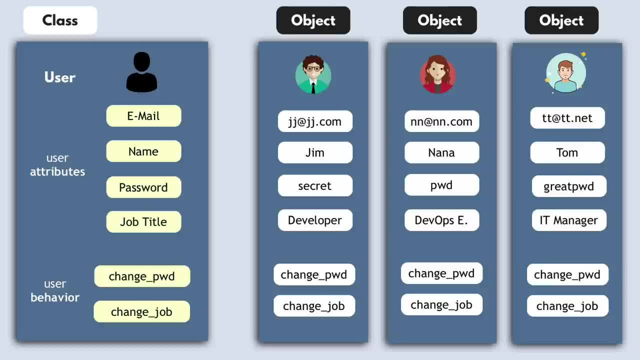 So think of this like a blueprint of a building. Right, You can have a blueprint once which is like a general description of building, with doors and windows and everything that every single building has, And then the specific implementation Of That blueprint will be the actual built ready buildings. 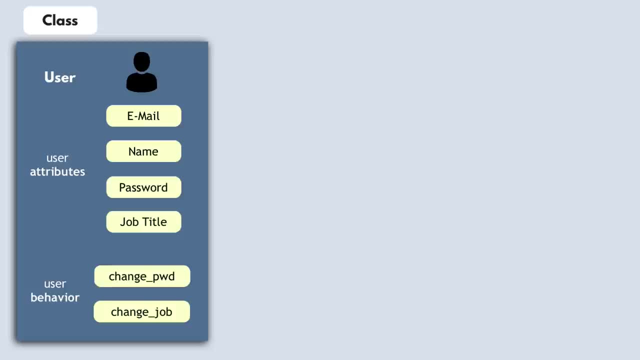 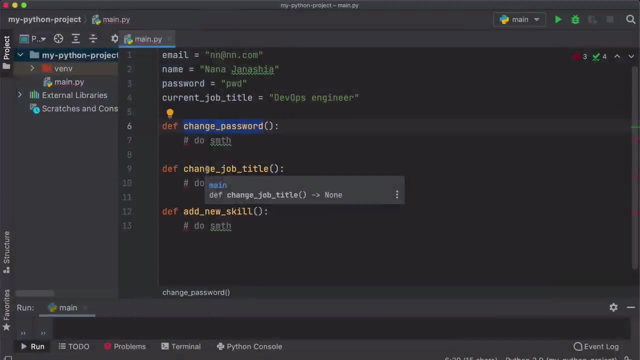 Right, So that's the same concept. We're going to create a class blueprint for a user and the user class blueprint will define what information a user has and what actions user can perform in the application, and object then will contain the actual information, like this: information right here. 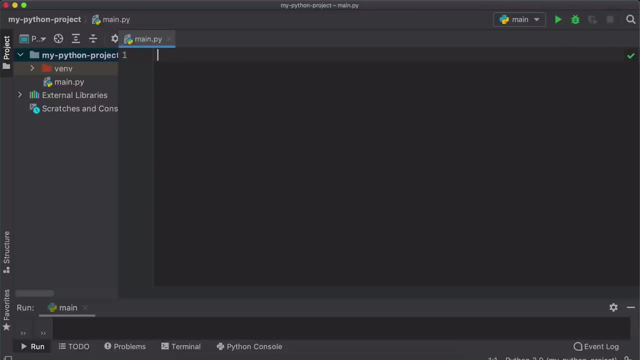 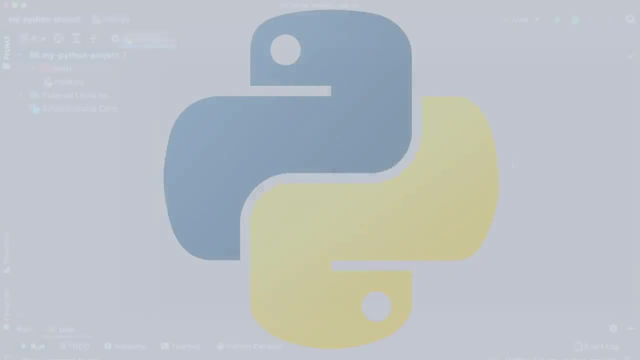 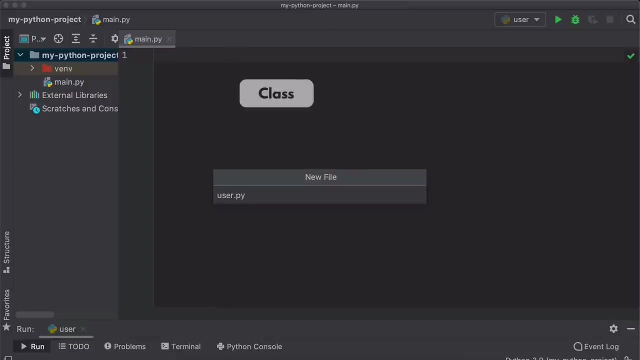 for each specific user. So let's clean all this up And let's now actually create class user. So let's create a new file in our project and let's actually call it user dot pi. So this is going to be our user class and inside that I'm going. 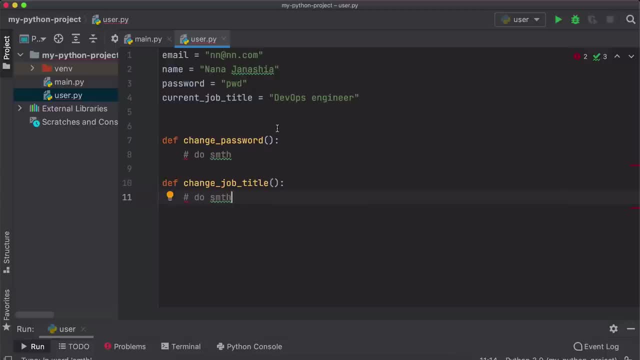 to paste in this piece of code. that basically will represent data for the user and some behavior. These pieces of data are also called attributes For that class. So now let's turn all of these into a class. So first of all, we create a class using class special work and you 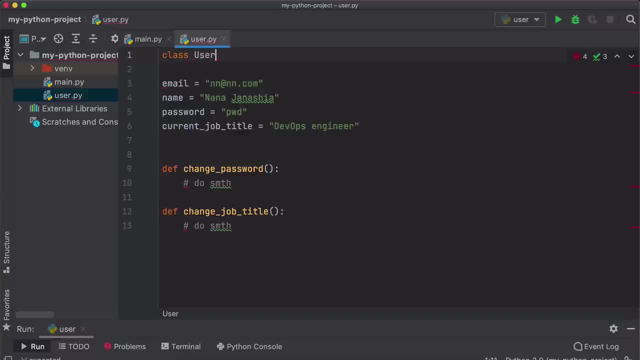 also see the syntax highlighting, and we're going to call that user and you know the syntax already for functions et cetera, with indentation. So this is going to be where our class definition goes. Now note here the capital letter for you, for user and low case user in the 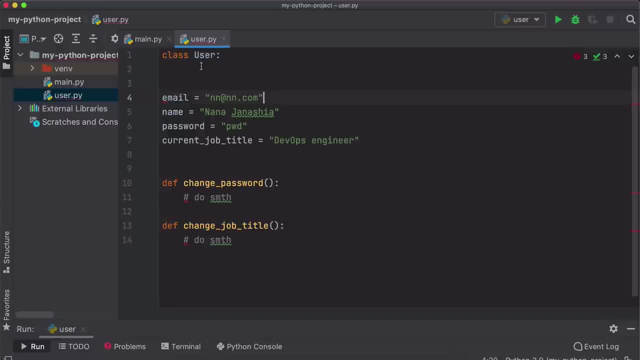 Python filing. So a standard convention is that we call classes with the capital letter and file names are written in lower case letters, and now all of these should actually go inside that indentation Right Like this. now we said that class is a blueprint for specific. 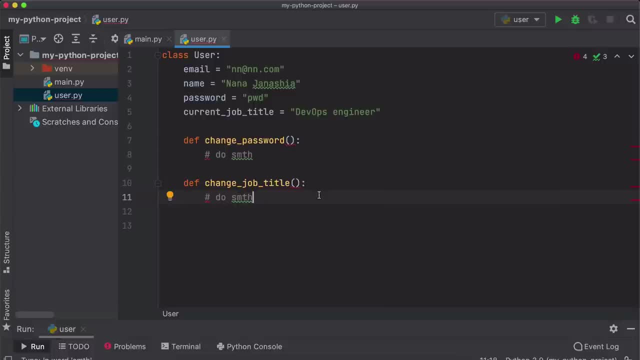 objects and blueprint cannot actually have specific values, Right? So all of this needs to be removed. So in the blueprint we don't have any special values, Right, specific values, we just have the attributes. So basically we say this user will have an email. 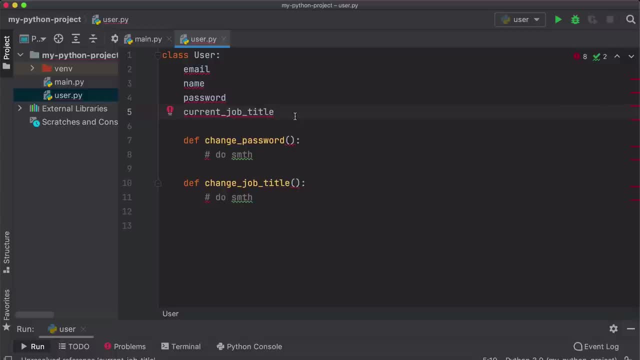 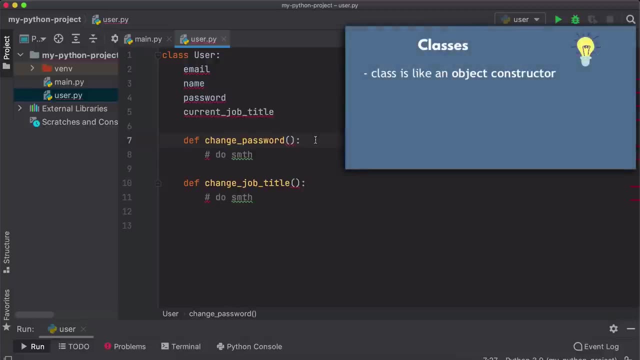 name, password and current job title. The actual values of those attributes will be then set when we create an object from the blueprint. However, we need a function that will actually take those specific values and assign them to an object which is created from the blueprint, And we're 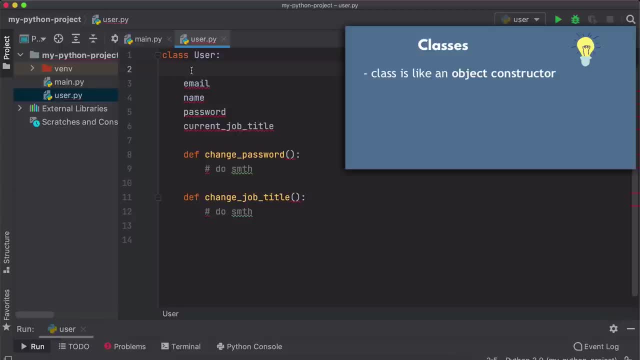 going to create that function right here in the class And that function actually is called init, with underscore or two underscores at the beginning and at the end. A couple of notes here. First of all, you see the syntax highlighting just changed to this different color. Second, 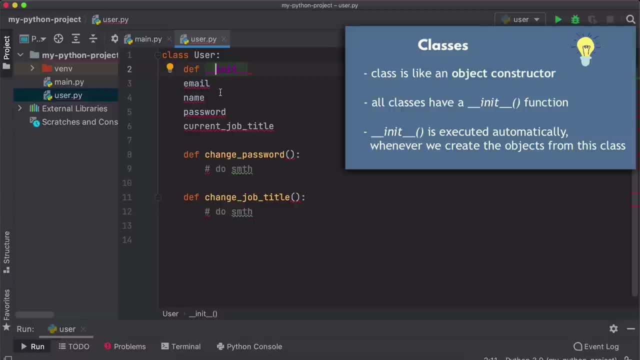 note is that these functions that start with underscore in Python are special functions, So Python basically gives them some special meaning. So it knows exactly what this init function is And we also have to call it in it. We can't just call it whatever we want. 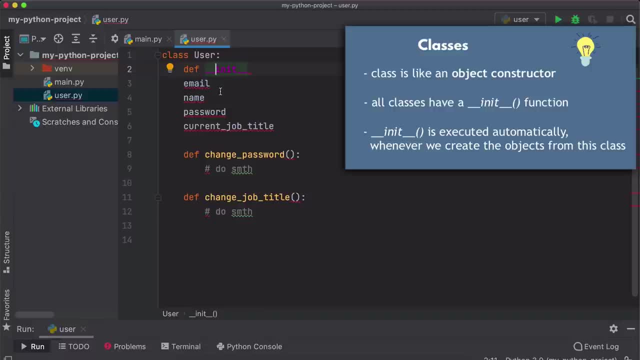 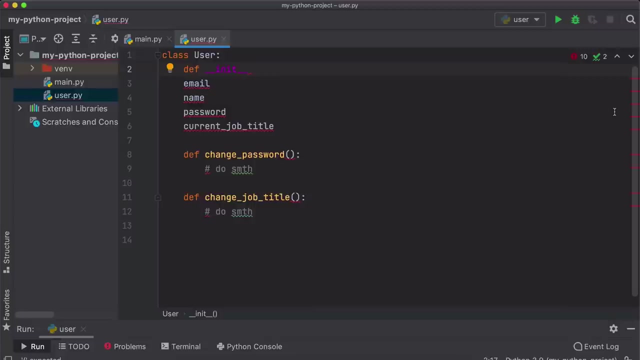 And final note is that this init function in Python is something called a constructor. Again, we have a blueprint and we're constructing objects from the blueprint and this init function, the constructive function, will help us construct objects from that user class. And now for a function syntax. you know that we use these brackets. 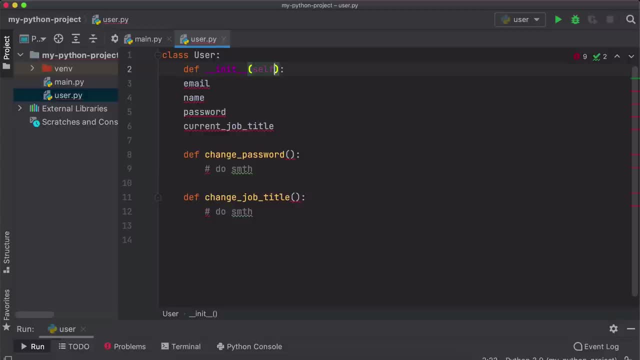 Right, And when I start writing the bracket, you see that self got automatically created as the parameter here, And the reason is, as I mentioned. Python knows what the init function is and that it's a constructor, So it knows that it needs this self as a parameter. Again, self is also a special 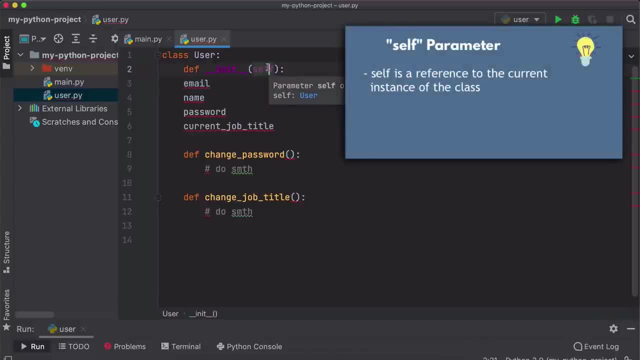 word in Python. It has a special meaning and it actually refers to this class here. right, this entire class. if I hover over it, you see self points to the user class and it will basically just help us access and reference all the attributes and functions within that class. 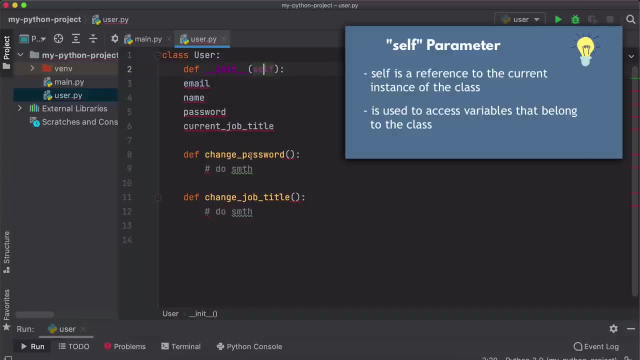 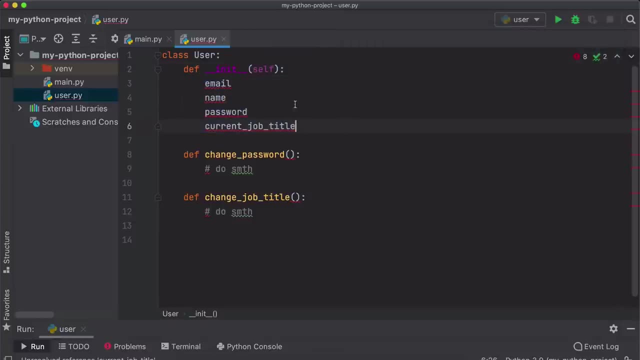 so it's for special usage within that user class and we're going to see examples of how to use that in a second. now you can think of those attributes as variables within the class, because they belong to the class, right? they describe basically what attributes or what characteristics this class has. 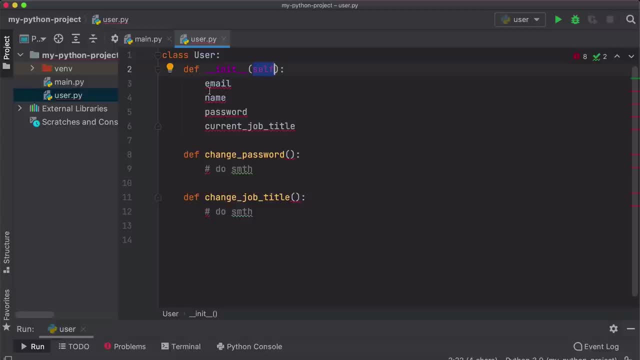 and in order to define that these variables belong to the class, we need to use self here. so, and you see again, syntax highlighting changed and the red line disappeared. so basically, we're defining that email name, password and current job title belong to this class and we're going to use self to define that email name, password and current job title. 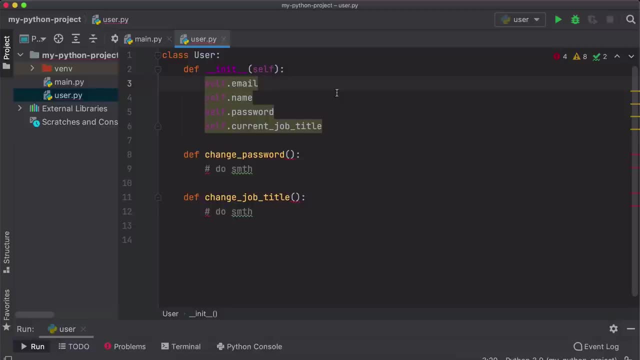 and we're going to use self to define that email name, password and current job title using this self keyword. And now the last thing remaining in this constructor- Again, remember, constructor is to construct new objects. So whenever a new object is created, 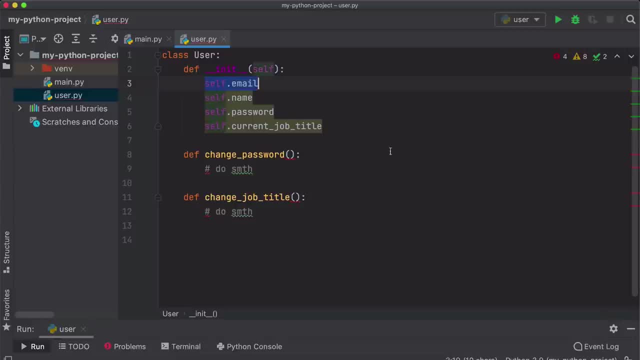 the specific values will be assigned to all of these four variables: Right And those values. those specific values will be passed into the constructor as parameters. So email name, password and current job title. Those four values must be provided to the constructor whenever we're creating a new object. 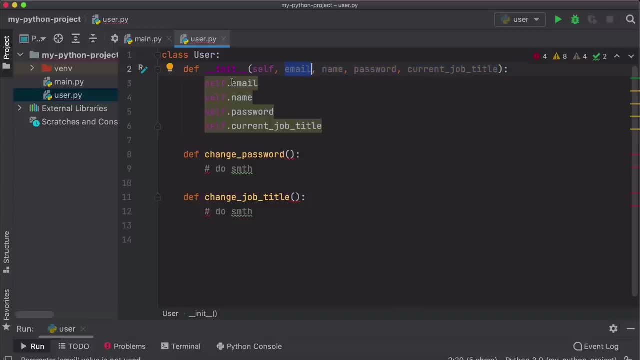 Know that these names here could be different from this. These are not the same. These are just parameters And using these parameter values, we are going to basically set the variables or attributes of the class like this, And the warning is gone as well. 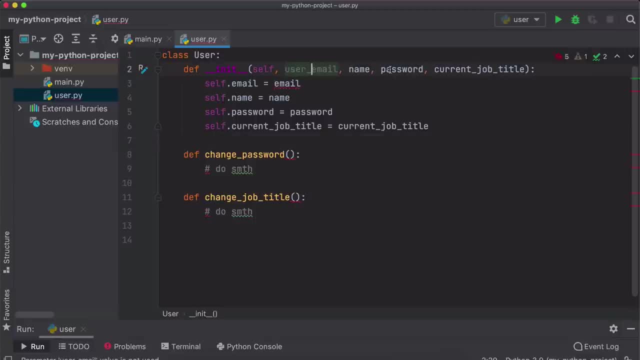 Again, as I mentioned, this could be something else. We could call it user email, So it doesn't actually have to be the same just for convenience. So this function will construct an object with parameters that we provide when we actually create it. 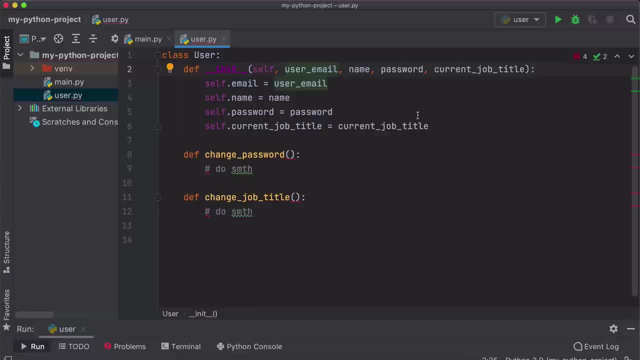 And we're going to see how to create an object later. This is just the definition, As, remember, when you define a function, nothing actually happens until you call or you use That function. So, right here, we're just defining that function so that we can use it later. 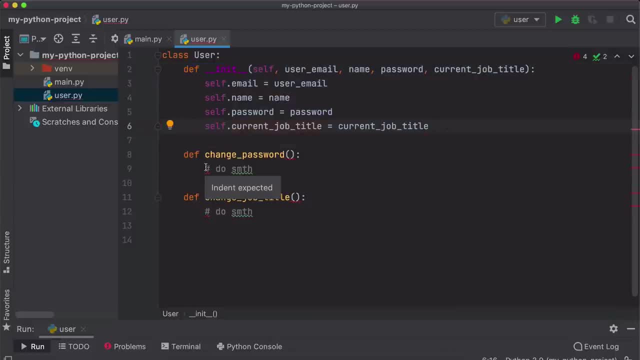 So constructor logic is done. Now we have these two functions that any user in our application can do. Right, Any user can change their password or change their job title And, logically, when change password happens by user. basically, user provides a new password in order to override the old one. 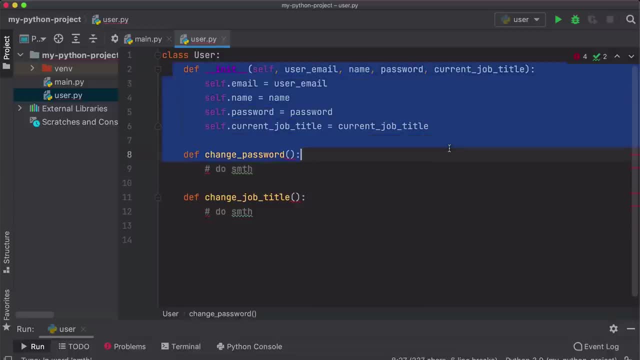 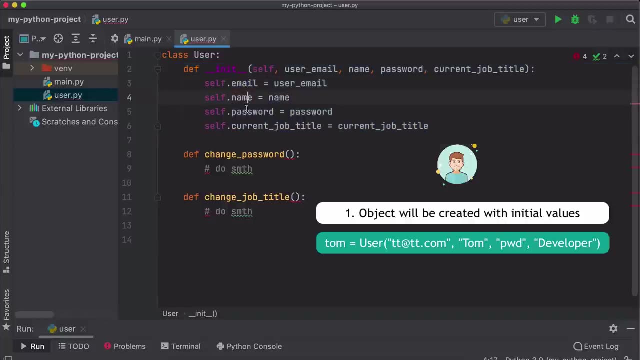 So The flow will be following: the object will be created for the specific user, So the initial data for that object will be provided. So we'll have the user email name, password and current job title And later at some point, user may decide to change their password. 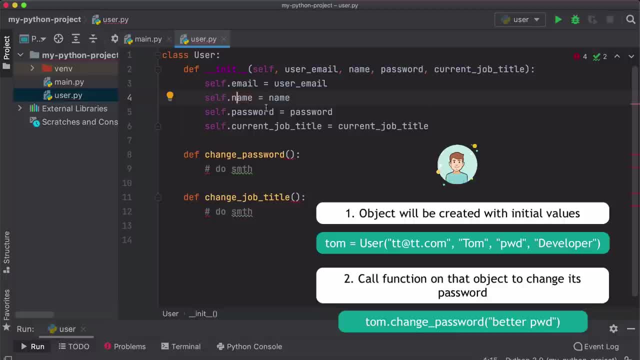 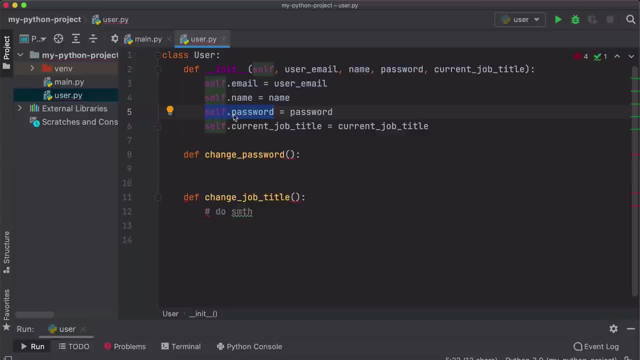 and their current job title, And that means the initial data will be changed, And that means That we're actually changing the attributes Self dot password with a new password right. So logic will be like this: Now we have red lines here. 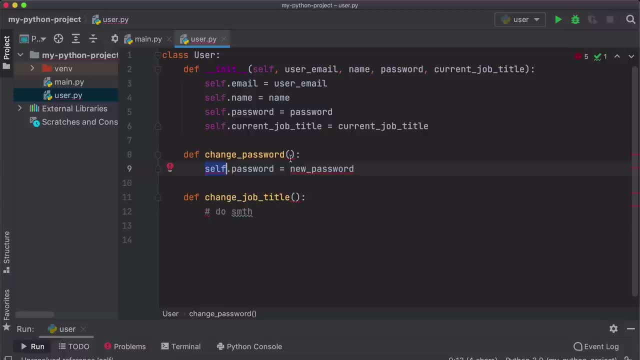 Why? Because we need the self as a parameter. First of all, we also have that as an note right here. So, just like here, we need to actually pass that self as a parameter. That's just how it is, because we need to access attributes of that class in that function. 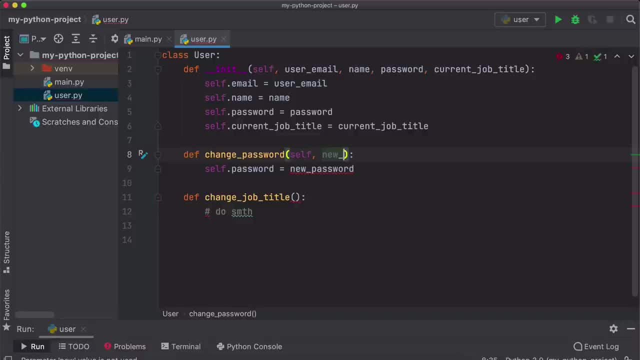 And new password will be a new password. Variable will be the new password, basically that user wants to set. So this will change the initial password with the new one And the same way in change of title we have self as a first parameter. 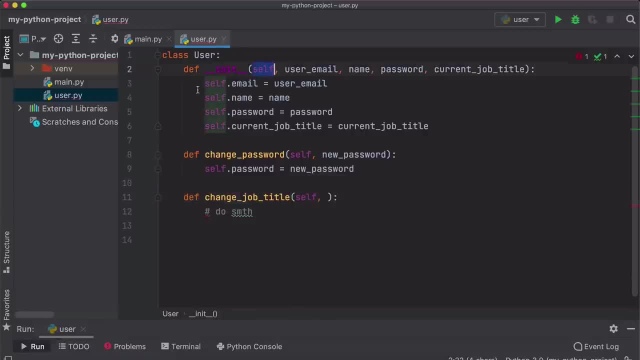 We always need it in all the functions because otherwise we cannot access the attributes in the class and new job Title. So now let's review this class that we created. First of all, we have this class keyword here with a capital letter for user. 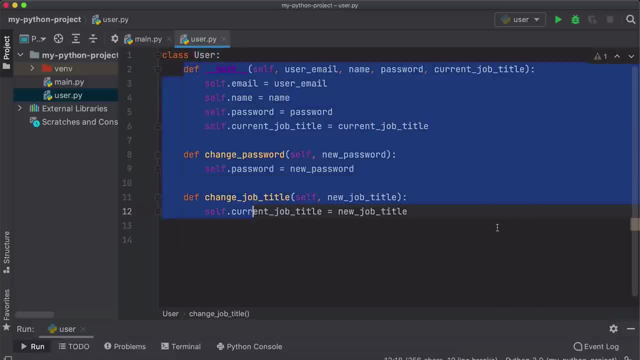 You already know the syntax with colon and then indentation. So this, all of these inside this indentation, is class body, So part of the class logic. First we have This init constructor that sets the initial values of that class attributes whenever we create a specific object for that class. 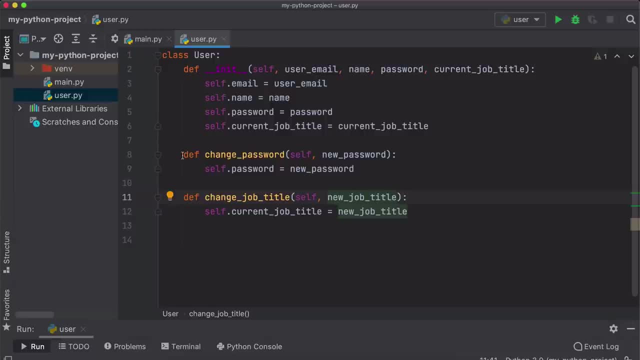 Right, So this happens only when we construct a new object And then on that constructed object we can change password, We can change job title and know that right now we have nothing, basically hard coded, We have no specific values here, Right? 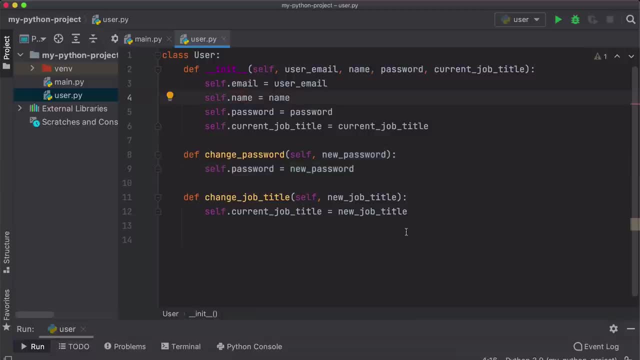 Everything is just parameterized And also this is just a definition for class and its functions. Nothing will actually happen when we execute this because we're not creating any user objects. So if I right click here and execute this run user, You see that nothing happened because the class definition was created, but we're not doing anything with that class definition. 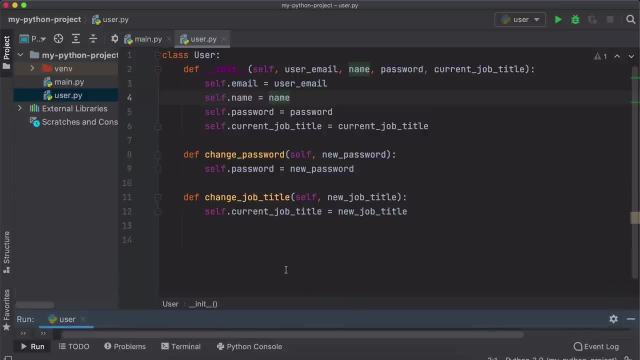 We're not creating new users, So now let's actually go ahead and do that In the same file in user dot p y. I'm going to actually use that class blueprint to construct a new user object in. creating an object from a class is actually very simple. 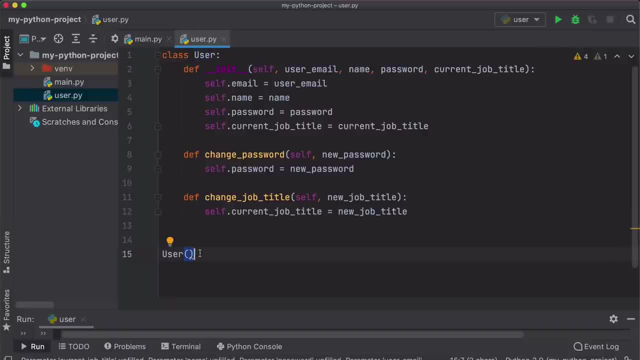 We just write name of the class and parentheses And this is actually the same syntax as calling the function with parameters, and the parameters that we need to give That Class are these four values here. and note that calling these user class function basically in the background will call in it function. 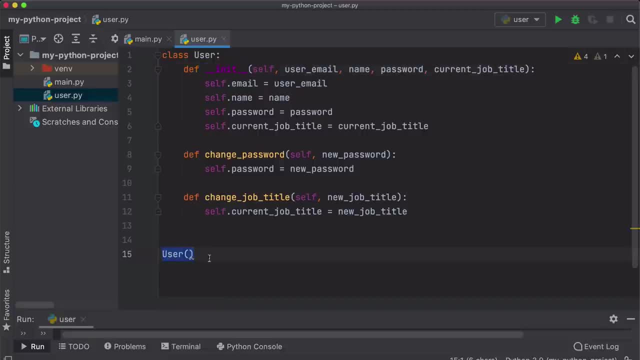 Right, So the constructor will be called whenever we write this syntax with class name and parentheses. and this image constructor, as you see, expects four parameters, So we have to provide all those parameters right here in the parentheses. So let's actually provide them. 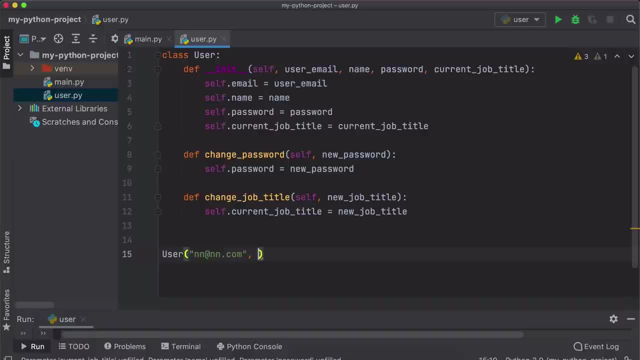 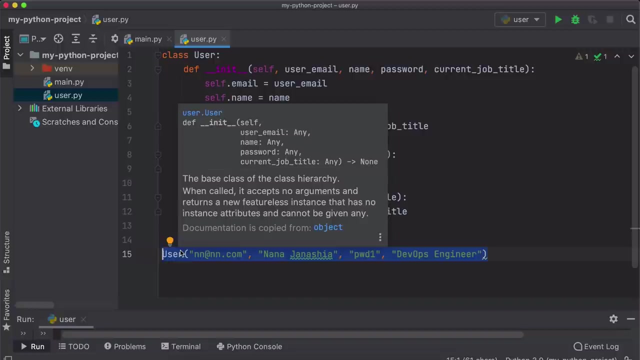 Let's do user email This- My username and password And a current job title- again very similar to calling a function- and this will actually construct a new object from the user class which has these four attributes, And this will actually construct a new object from the user class which has these four attributes. 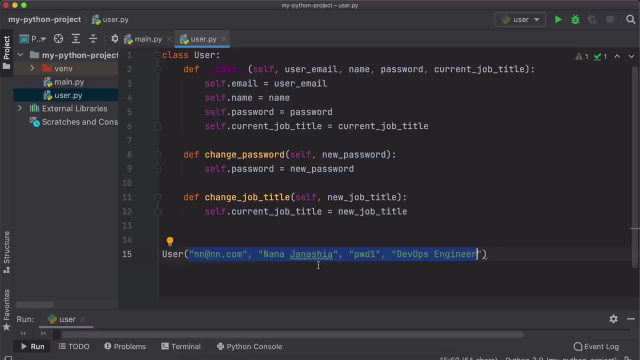 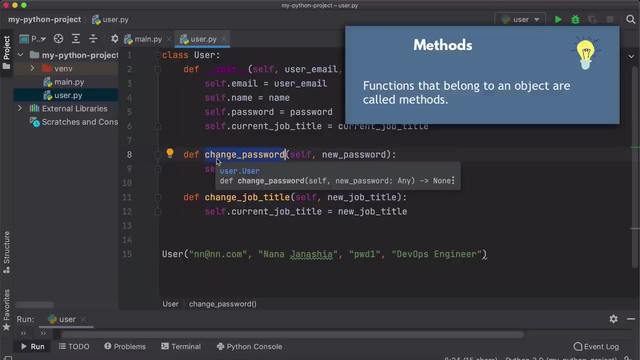 With values that we just provided here and has these two functions that we can use to either change a password or change job title. One note here is that functions that belong to a class are actually called methods, So there's a special name for functions which are part of a class, so we can refer to them as methods. 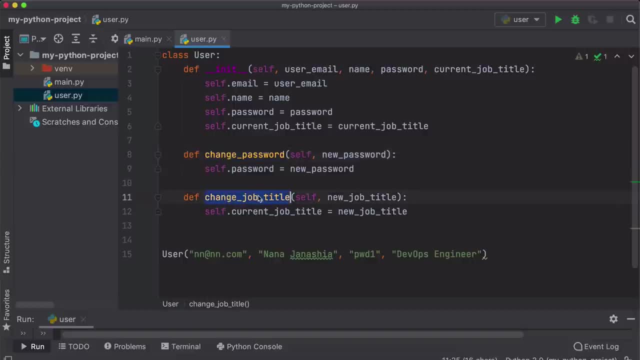 So user object basically gives us two methods. So user object basically gives us two methods. So user object basically gives us two methods That we can use now. again, if we execute this program now, we will not see anything, even though user will be created, because we're not printing anything to the console. 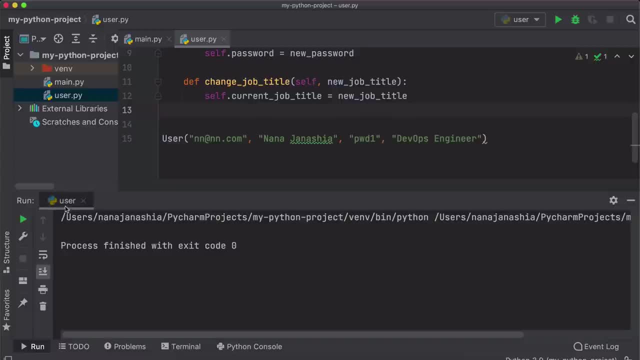 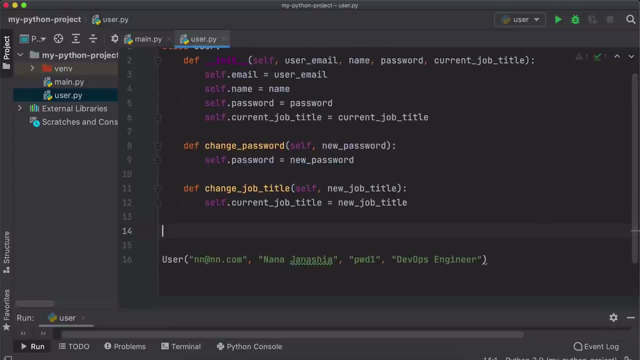 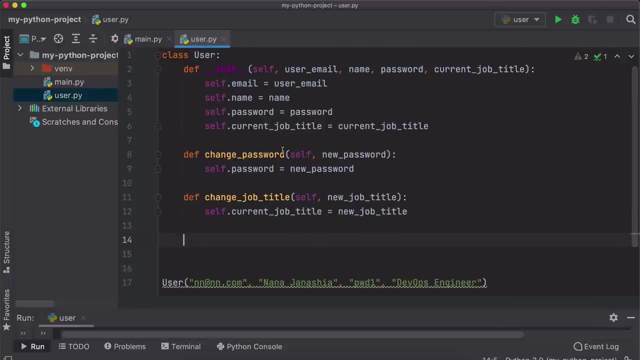 We're not doing anything, So let's do that: run user. Nothing happens, because we need to print a message or some kind of information. So what I'm going to do now is, inside that class, I'm going to create a function or a method, as we learn now, that basically prints back some user information. 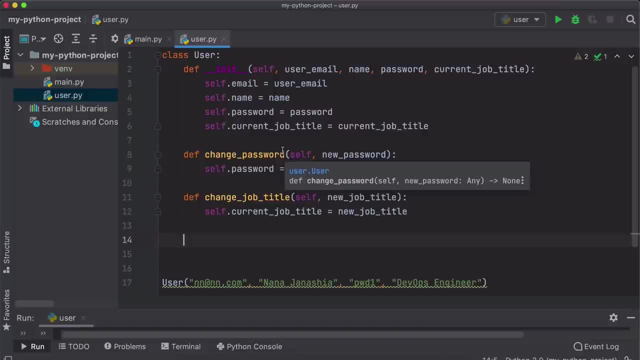 Right, So what I'm going to do now is, inside that class, I'm going to create a function or a method, as we learn now, that basically prints back some user information, Right? So let's do that. run user. It prints me the name, email and current job title, because we don't want to display a password. 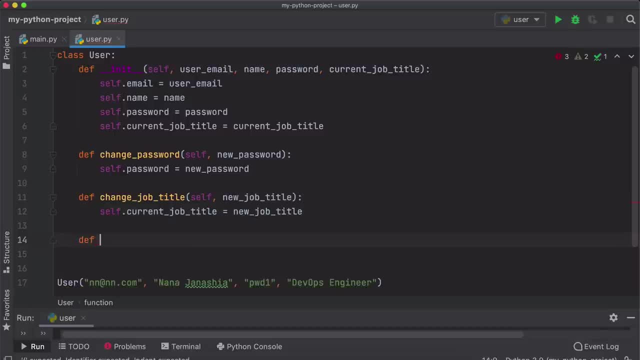 So let's give us some space here and let's create a function called get user info so that we can see something. And again, as soon as I typed in these first parentheses, self got generated, because we need self in every function, within the class and in the function body. And again, as soon as I typed in these first parentheses, self got generated because we need self in every function within the class. And again, as soon as I typed in these first parentheses, self got generated because we need self in every function within the class and in the function body. 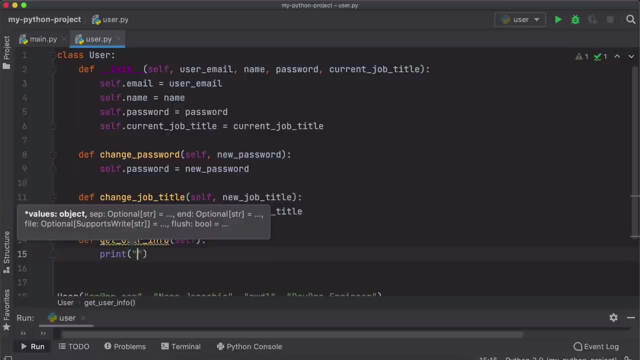 And again, as soon as I typed in these first parentheses, self got generated. because we need self in every function within the class and in the function body We're going to print user information. So let's say user and name of the user which we can access using self. 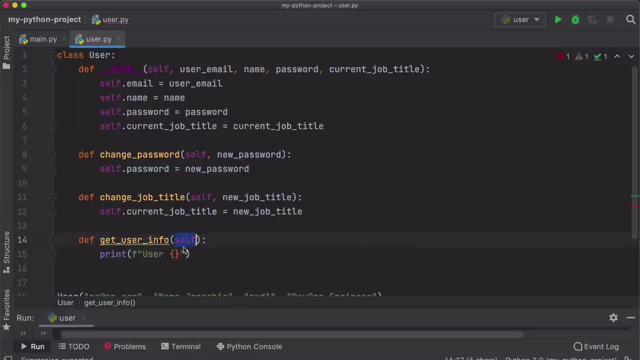 Remember, all the attributes that the object has can be accessed with this special word here. So self dot name, So user. whatever that user's name is, currently works as a and now we need the job description or job title and you can contact them at and. 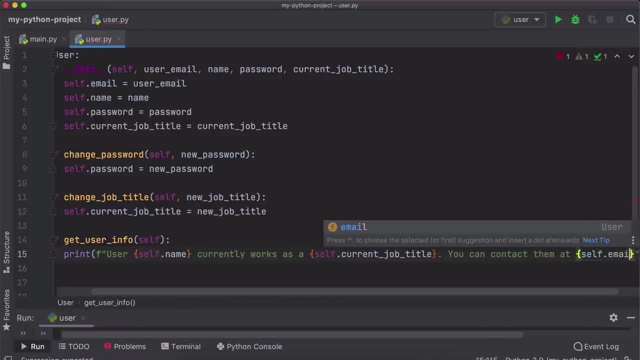 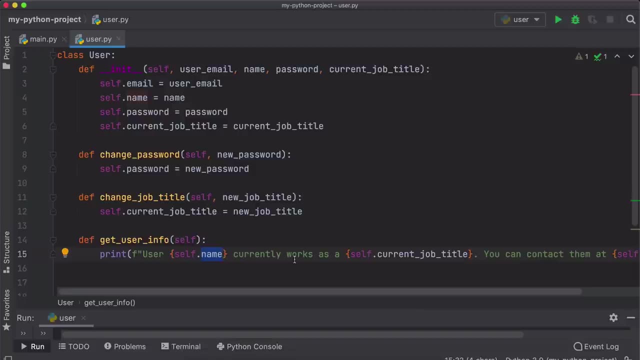 now we can use the email, so this message will be printed for the user again, because this will be used for any user of our application. the message, these parts, will be the same, but each user will have their own different name, different job title and different email address. 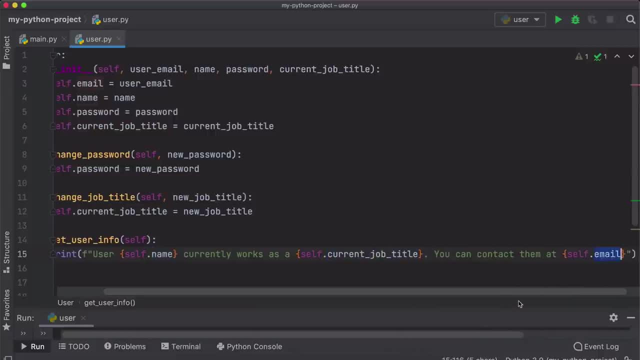 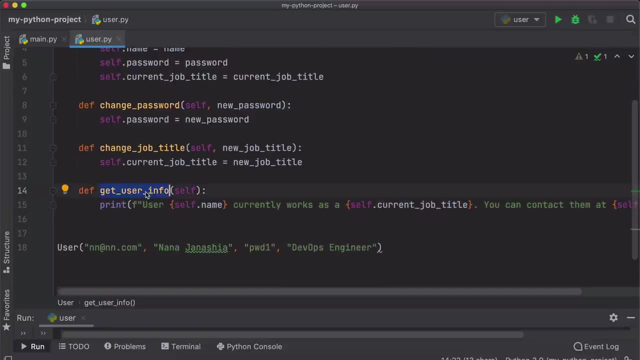 so all of these are parameterized and written as variables, because we don't know these values upfront. so now we can actually use this function or method to print out information of a specific user. so how do we use or how do we call that function of the user? we first save it into a variable. 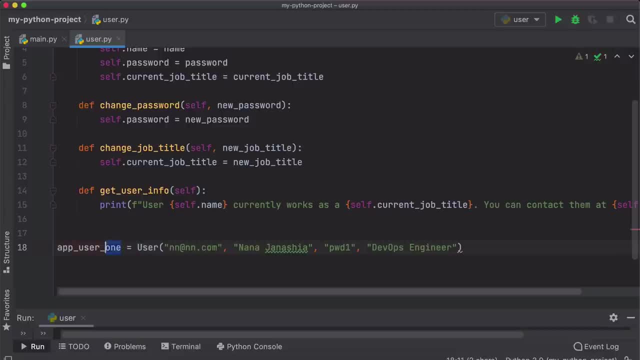 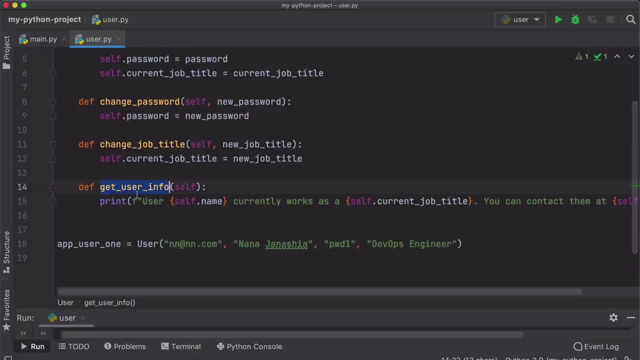 app user one or nana, doesn't really matter, let's call it app user one, so it's generic. so how do we use that function to print out the information about the user? if i do app user one and dot, you see that i have the attributes here. 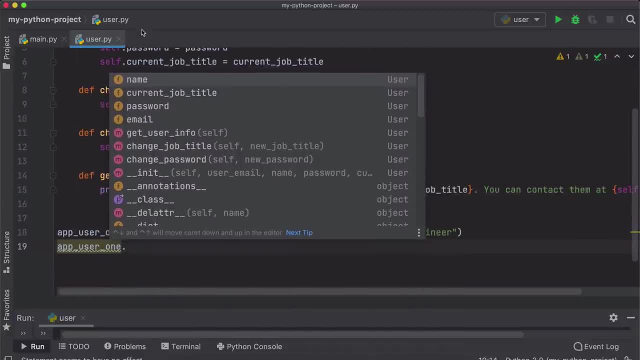 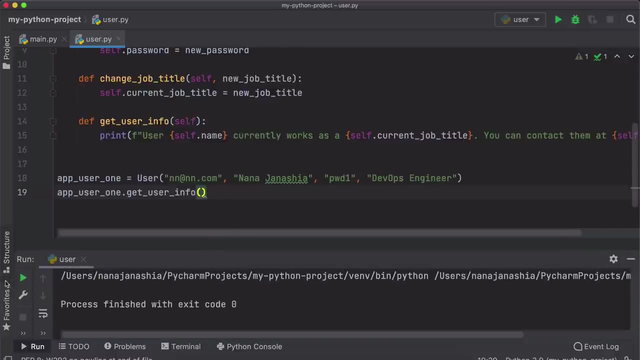 four attributes that our user object has, or use a class. And we have these three methods of the class: get user in for change of title and change password. So, using get info, we can call this function And if I execute this right here, you see user. 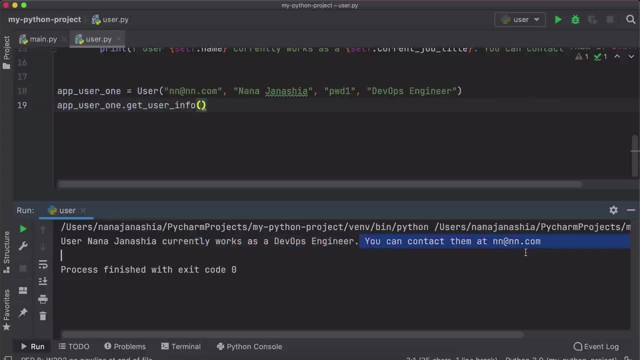 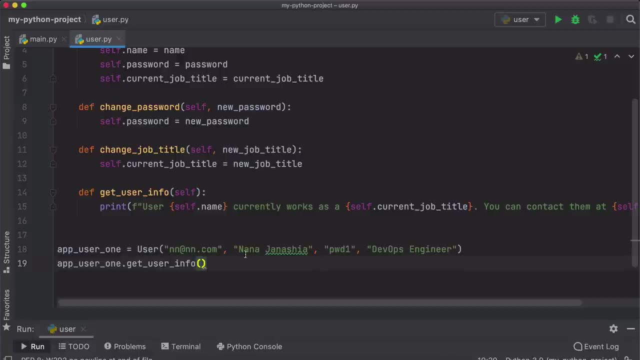 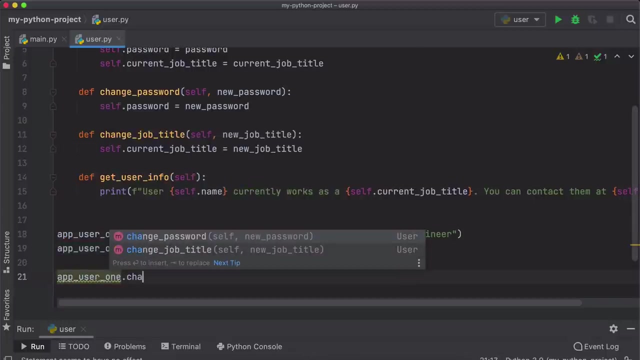 Nanajan Ashiya currently works as a devops engineer. You can contact them at this email. And now let's say we want to change the job title of that user. We do that in the same way If user one dot change job title. 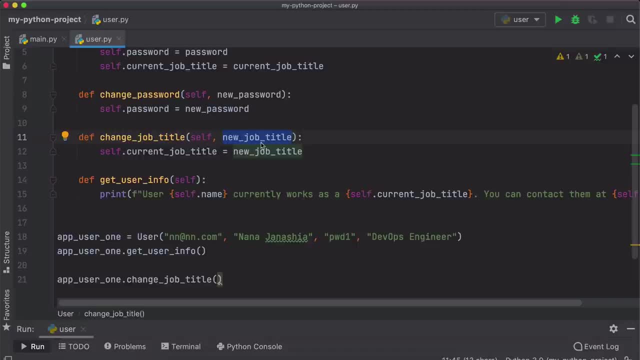 and we're going to provide the job title parameter. Note that even though you see two parameters here on that function, this first parameter is passed in automatically, So we don't have to basically pass that self-right. It's already done automatically. We just have. 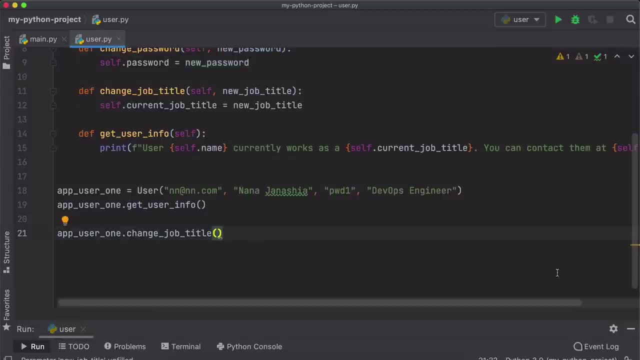 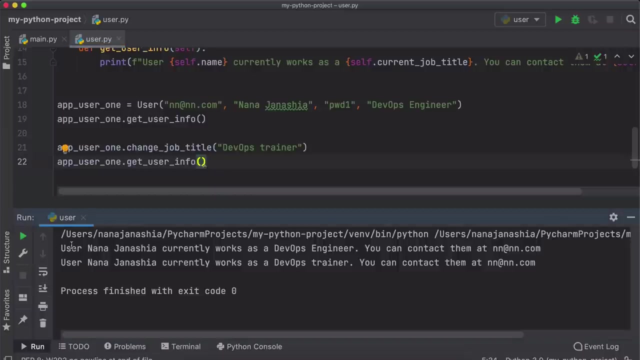 to worry about these parameters. So new job title is, let's say, devops trainer. And now we can call that user info method again and execute. And you see first message printed here before we change the job title: Now it's devops trainer. 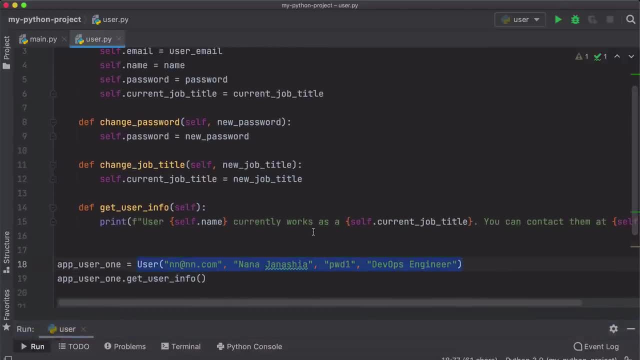 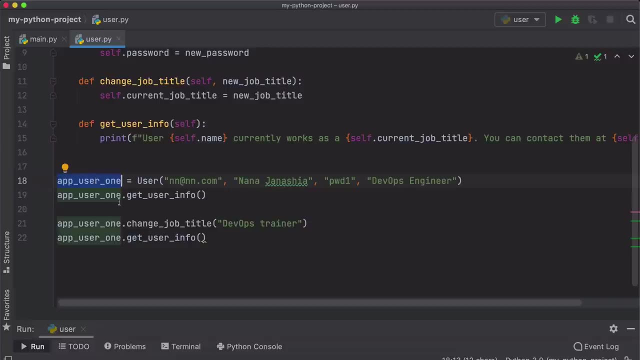 So that's how we can create a new object From a class and we can use methods of that object by first saving that object into a variable and then calling that function on that variable. And obviously now this is just one user, But if we had another one, 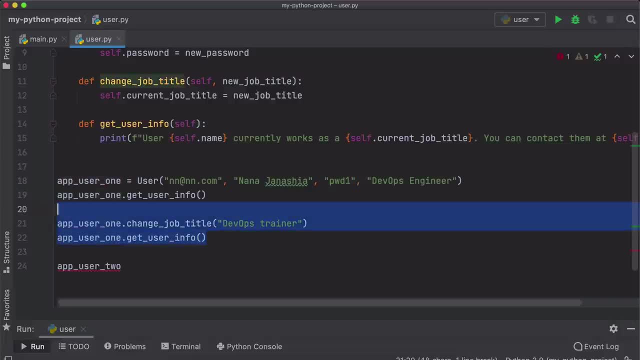 user. to essentially clean this up, we can create a new user with different Values, like this: They have their own email, Own name, Own password and own job title. And again, We can create that user and basically just use the methods defined in the class. 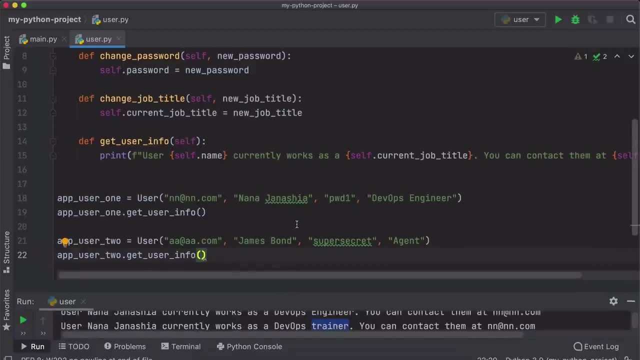 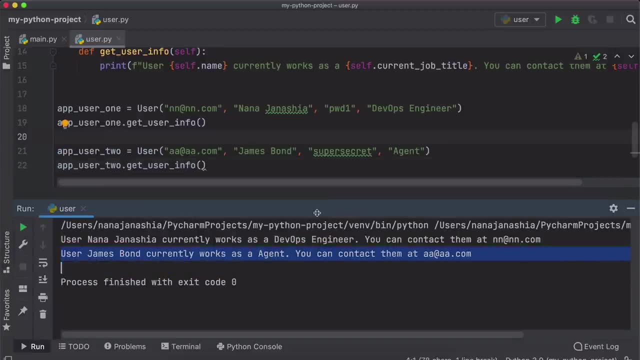 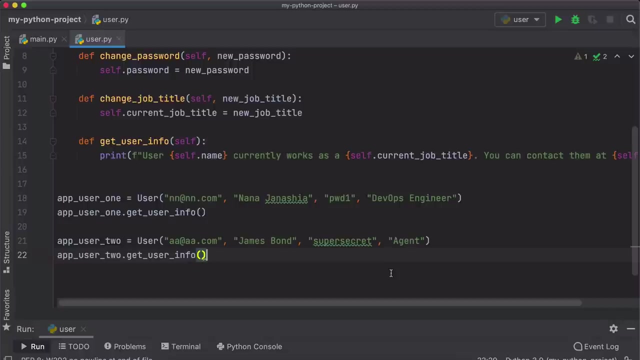 and in two different cases or for two different users, Obviously the user info will be different. So let's execute this And right here you see the user information for both users. And obviously, if you have an application like LinkedIn, you don't have two users or a thousand users. 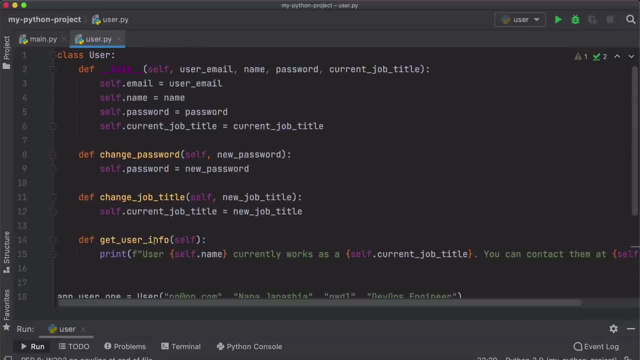 You probably have millions of users, and having a user definition once And reusing it every time a new user gets created or basically, existing users do something in application is only possible when using classes and objects instead of just having all this logic non structured throughout the code. 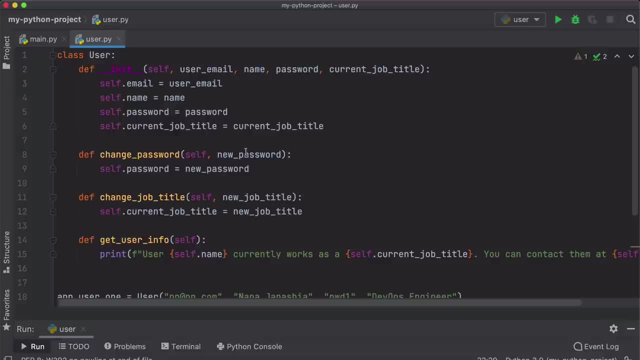 And again, in this type of applications, you would not have four attributes and three methods. You will have probably hundreds of attributes and hundreds of such methods. Now, as you see here, we have created this user dot pi file for user class, but we're also creating these objects. 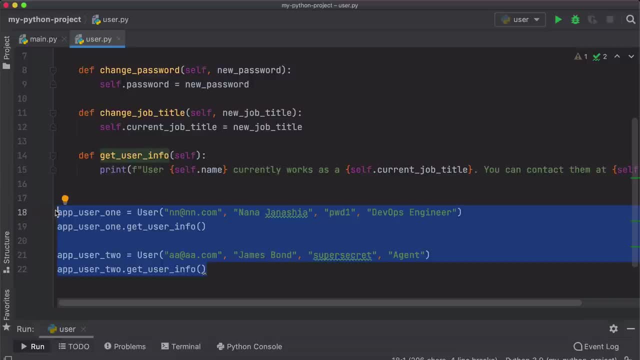 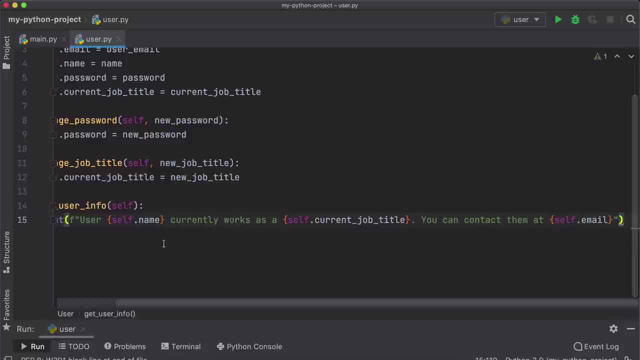 in the same file, which actually doesn't make sense, because the file should be only for defining the class Right. So all of this logic actually needs to move out from here And this should be just only for class definition. So in the application. 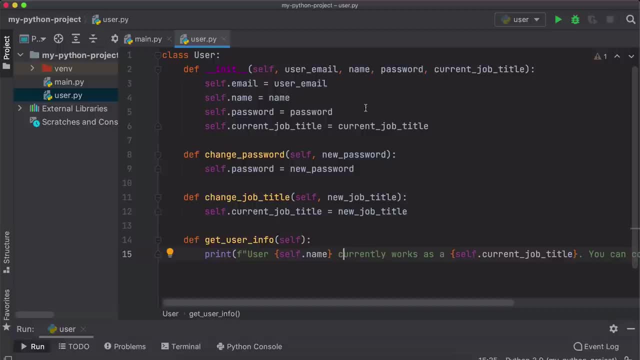 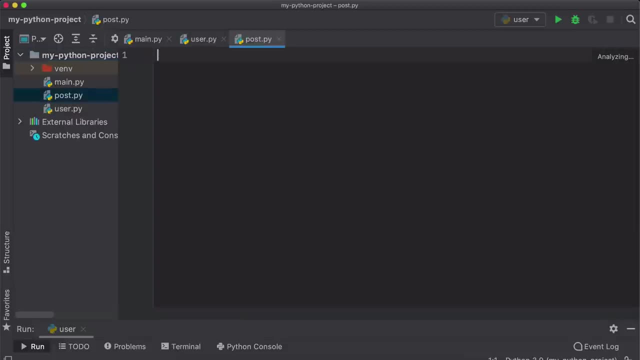 again using an example of LinkedIn, we would have class user and then we would have a class post, Right? Whenever someone posts something, each post will have their own attributes, like the actual message or text in that post, the author who wrote the post. 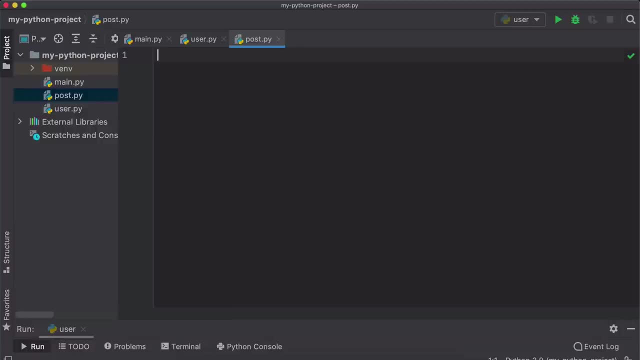 how many likes it has, et cetera, as well as specific functions Right, For example changing the post, commenting on the post, et cetera. So you will have Separate file for each such class right in the application. 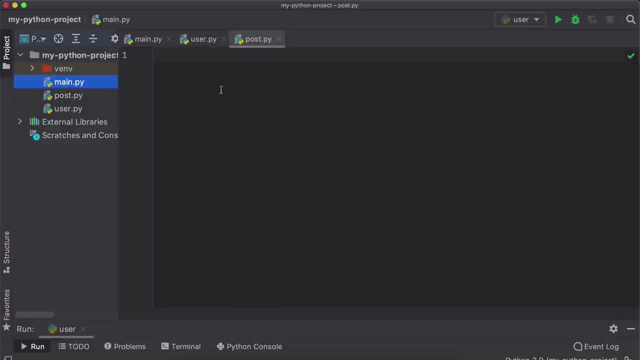 and then you would have one file somewhere else. This could be a main dot pie where you would actually use all those different classes and create objects from those classes. And that means that logic that we wrote here- constructing a user object and then calling some functions on- that will actually happen in another file. 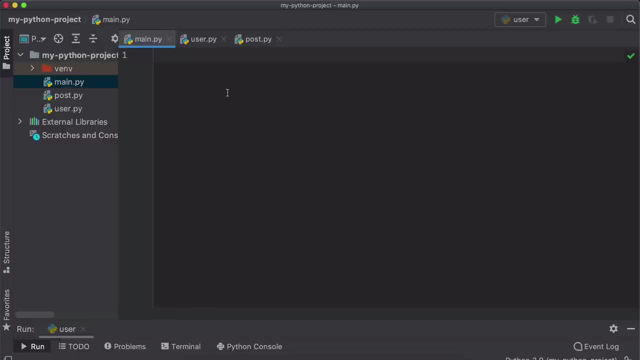 In our case, let's use a main dot pipe. and now let's see how we're going to do that. I'm going to paste in the code that I copied from there, And as soon as I paste in, you see those red lines. 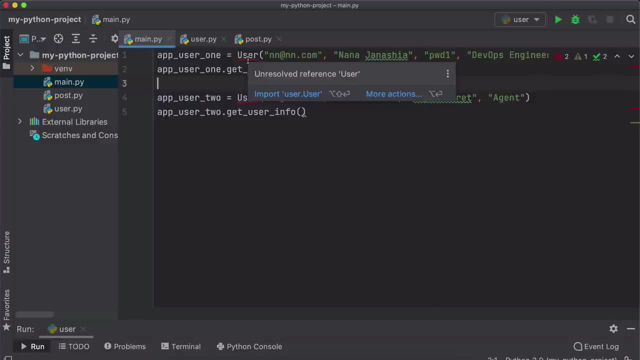 So basically, main dot pie says that it cannot find a reference to user, So this file doesn't know anything about the user class. So how do we fix that? or how do we make this user class available in another file? And if you remember when we needed to use modules or basically functions, variables, whatever, 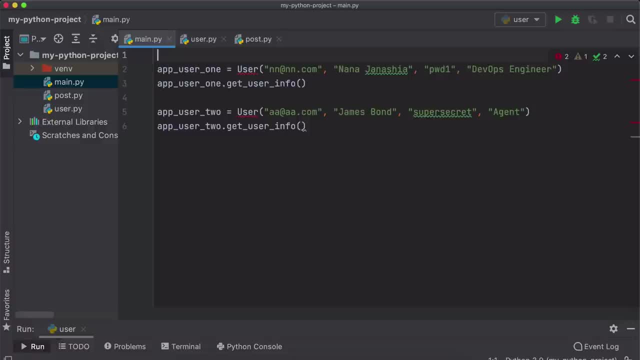 from other files. in Python we use import to basically import those functions and make them available here, or import the whole module to make its functions and variables available here. And the same way we can import classes from another file import user And note here that I'm using the name of the file user, lowercase. 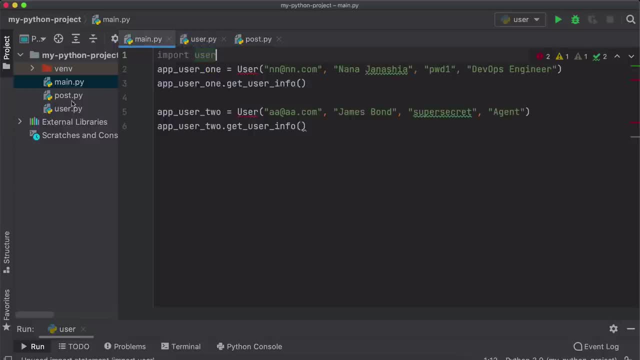 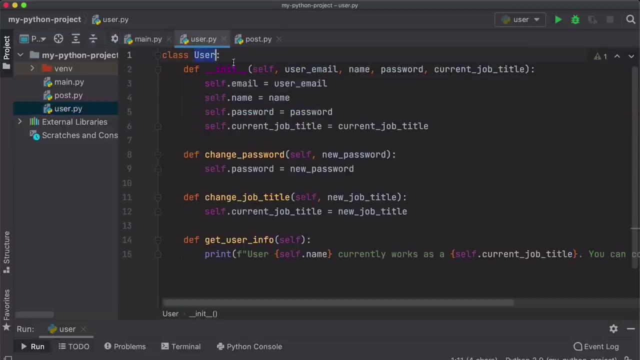 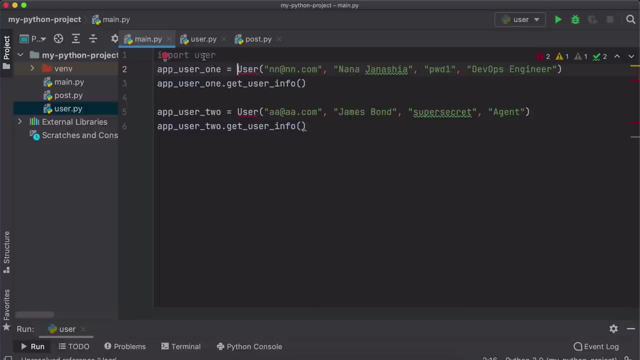 and not the class name with capital user Right. So we are Importing that file. So now we can use anything that is defined in that file And one of them is class called user, And the way we can access that class now is using the name of module. 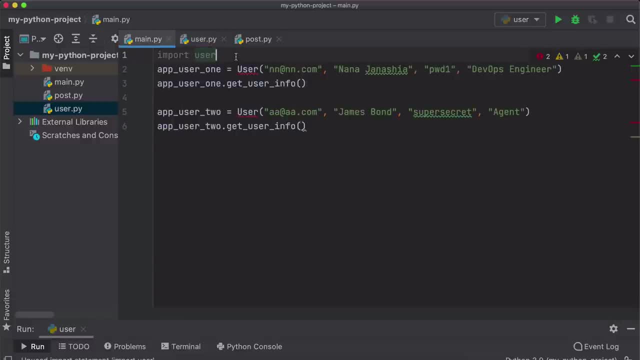 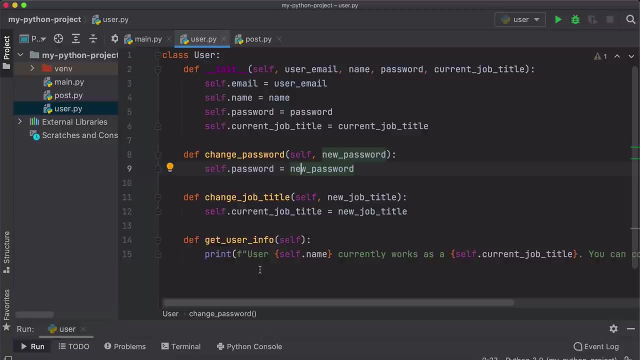 and not the class user itself. And this is basically exactly the same concept as we saw before, because we're importing a module called user. Remember, every Python file That has functions or variables or classes inside is a module. So we are importing a module. 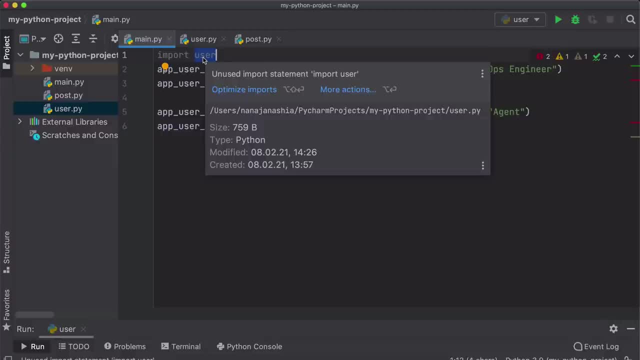 And once we have that module imported, now we can use an excess functions, variables or classes of that module, And we can do that by copying the name of the module, dot. And there you go. in the same way here. So exactly the same concept. whether this is a function or a class doesn't matter. 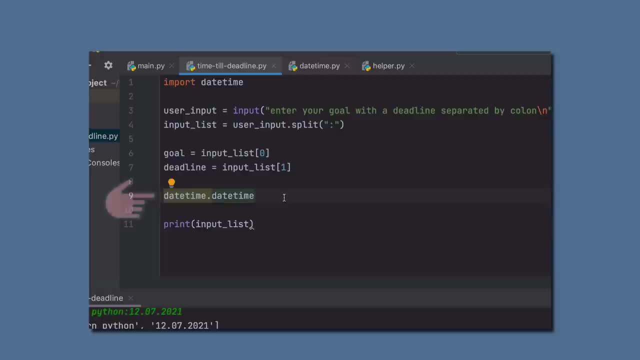 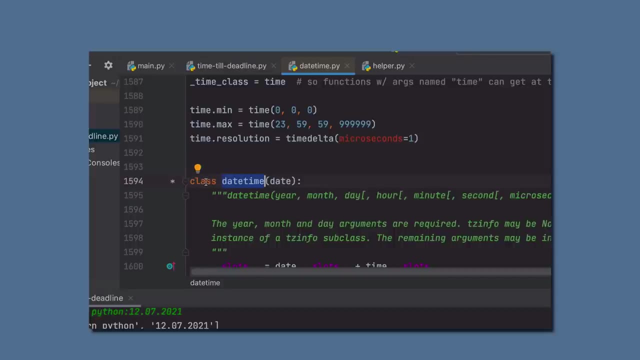 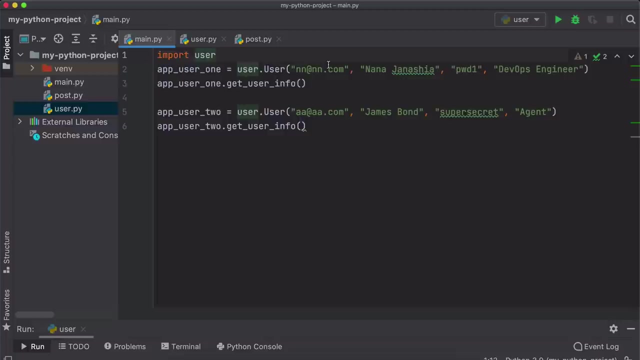 We use it the same way. Remember when we use the date time module with the syntax date time dot date time, And that was an example of using a class from a module. Now, user dot user may look a little bit weird, so we can use our familiar import statement. 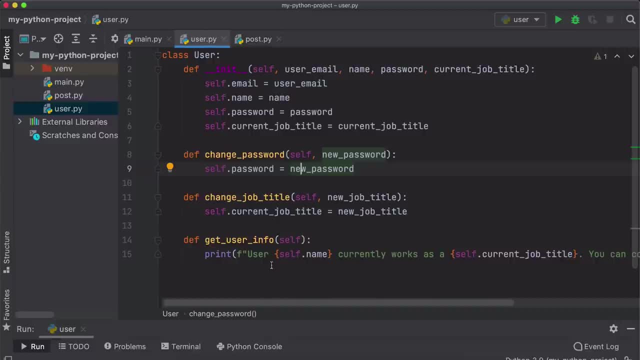 where, instead of importing the whole module, we can pick and choose and import specific definitions or specific elements of that module. In our case we just have one element, which is the class. So we're going to say, from user module, import user class. 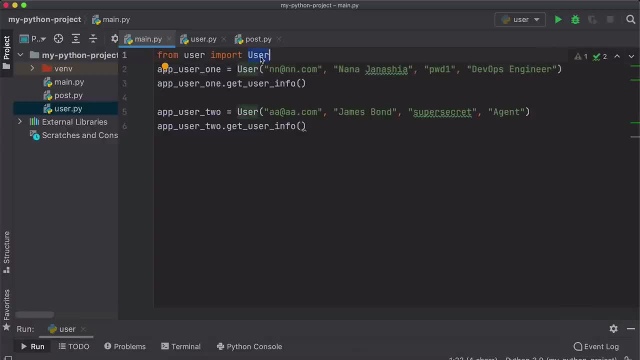 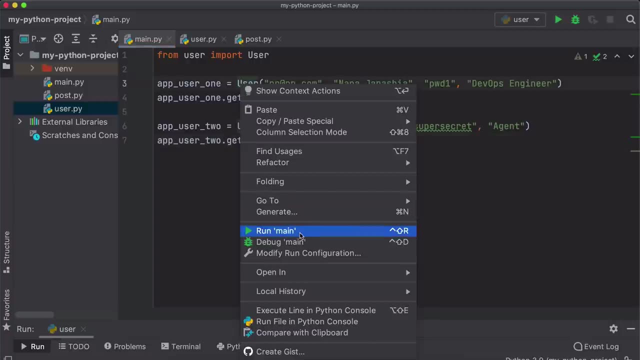 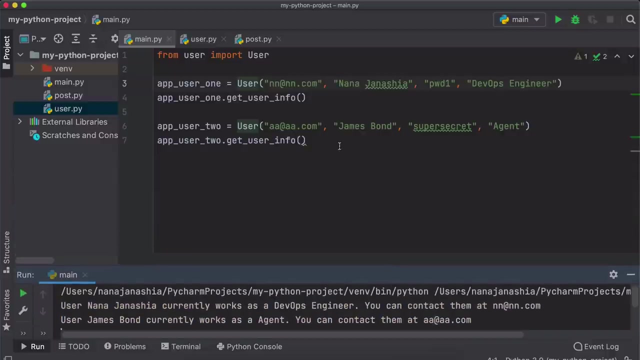 And now we don't need the module name anymore because we imported the class itself. And now, if we execute main dot, P, Y, let's do it again here. We have the same result for two of our users And again, as I said, in applications. 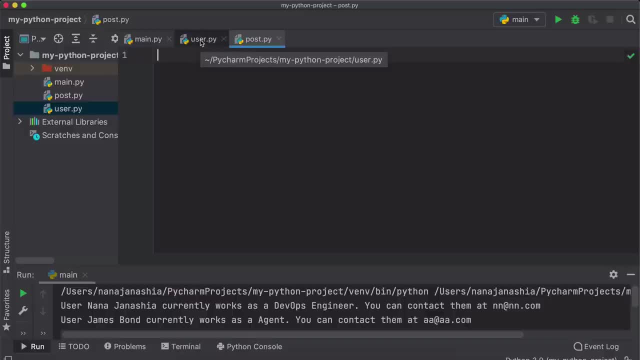 you will have multiple classes that are connected to each other. So, for example, if we have a post here, post blueprint, basically whenever a new post gets created with some specific values like the actual message and creation date, time, et cetera. 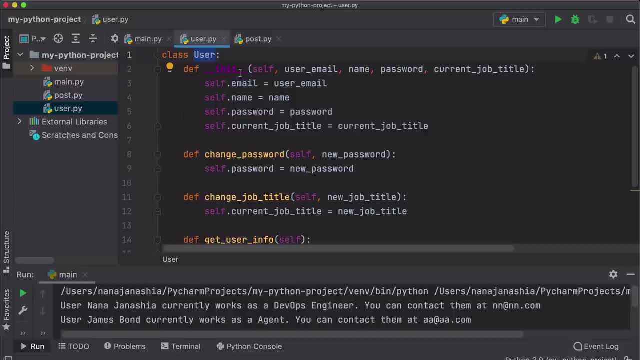 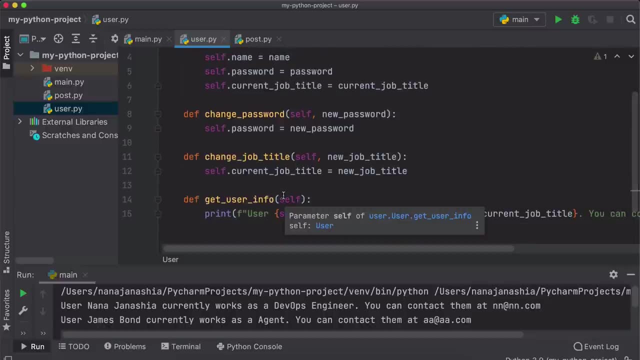 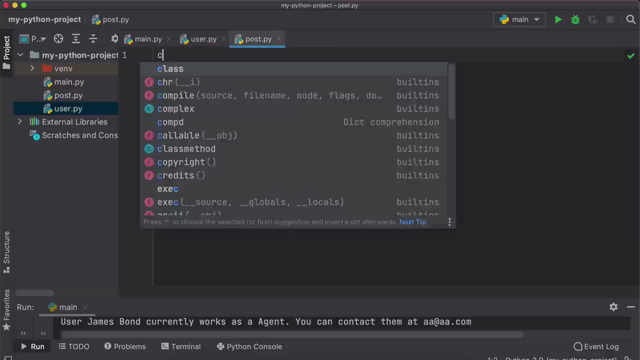 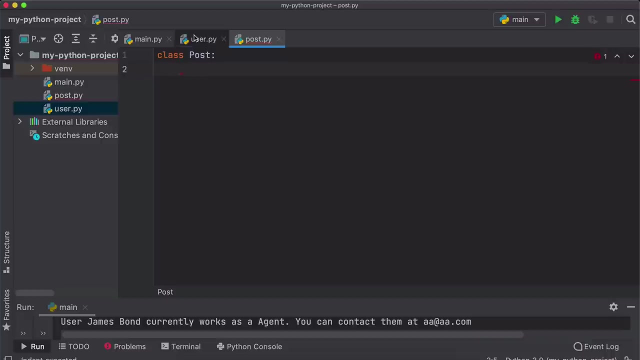 it will also have an author and that author will actually be one of those user objects, right? So you would have some functions here that actually reference the post, And we can also see that in action. Let's actually create a post class And let's give it just two attributes to keep it simple. 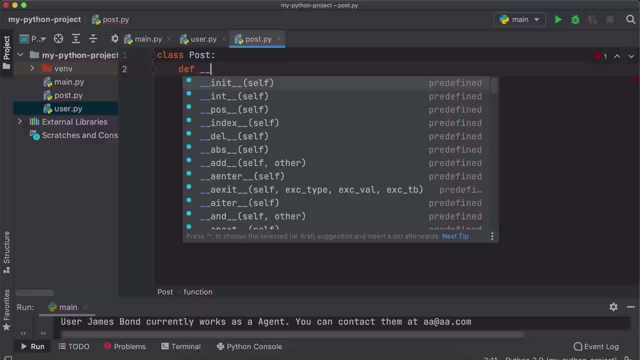 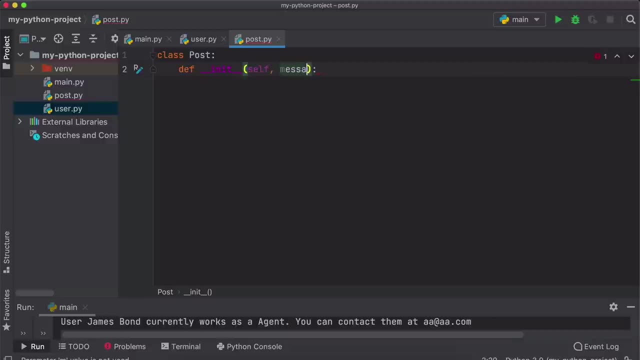 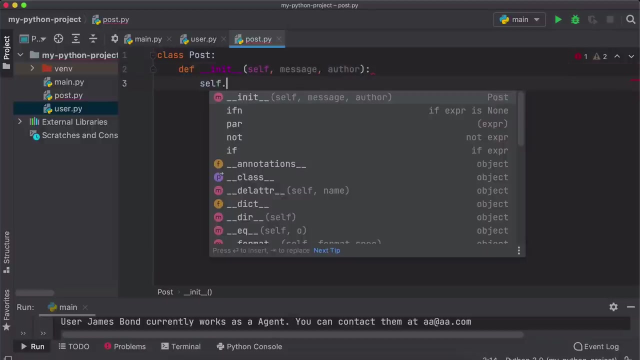 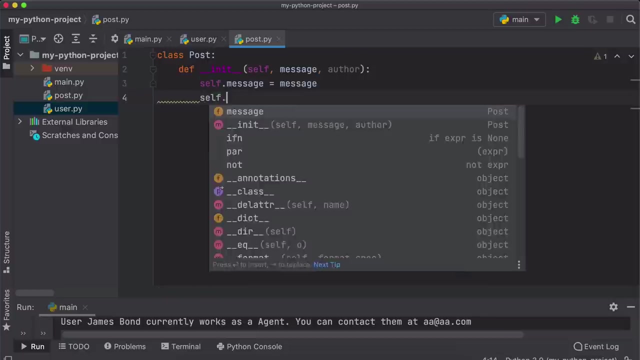 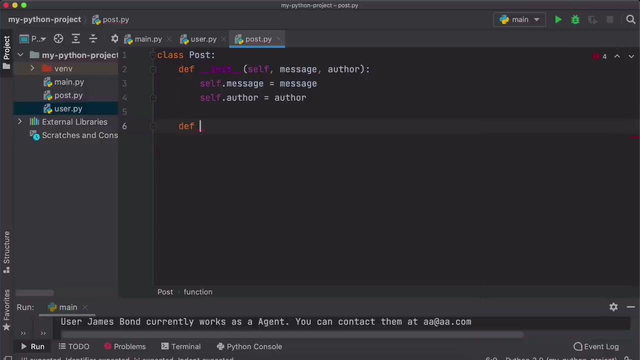 So we need a constructor here in it And we're going to pass in message And author right. This is going to be the user who wrote it, And you know the drill already. And let's create another function which displays a post with its respective author. 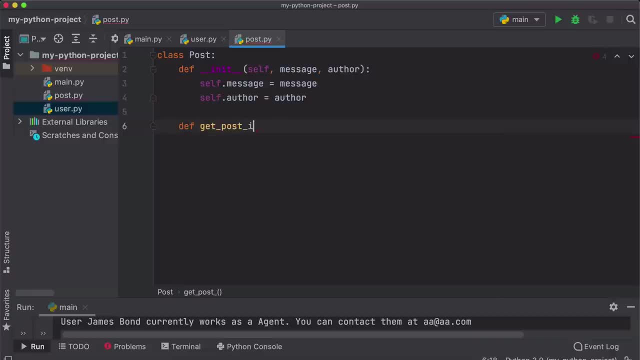 So let's do get post Info Again. we have self here and let's print Post Written by: And the author name. So this is going to be our simple post class and user is able to create new posts. So we have the blueprint for a post and the same way. 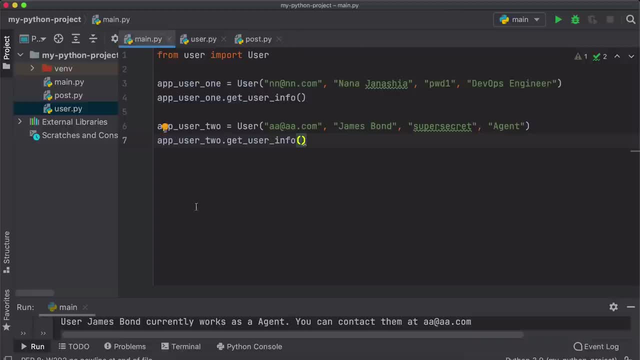 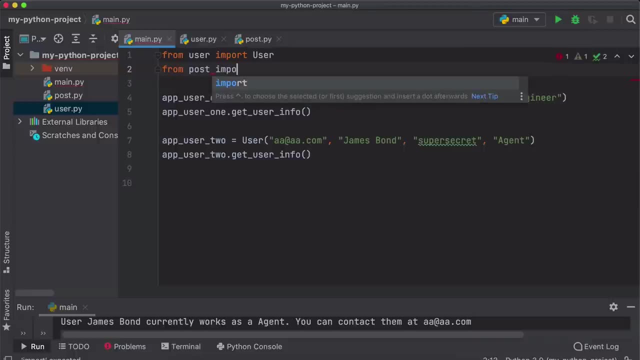 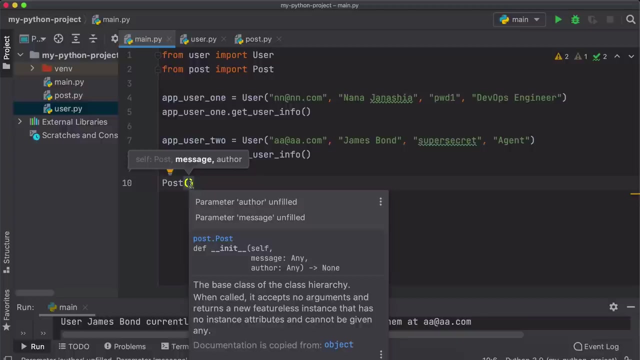 we can create the post inside the main dot pipe. So first let's import the post class And then here we're going to create a new post. in pie charm You get this nice display of parameters that function or class basically expects. 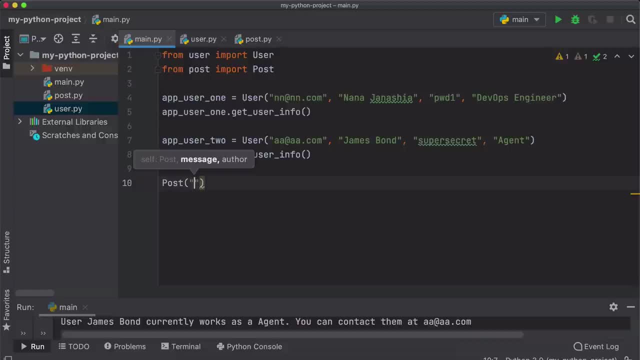 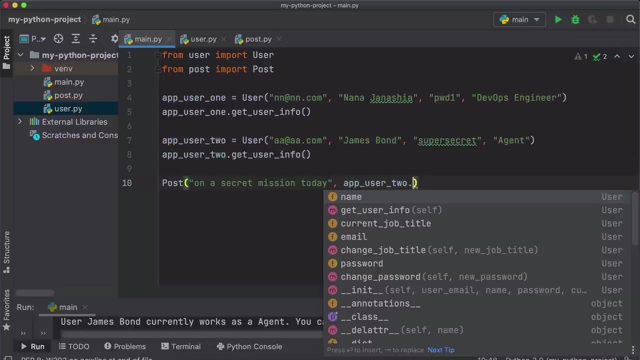 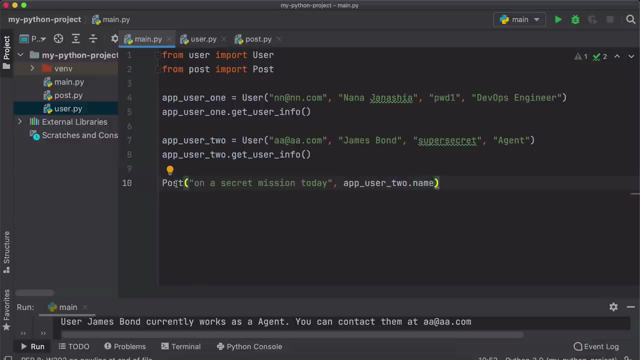 So we have message and author. Let's do some Message or post and as a second parameter we have the author and we can use the name of a user. So let's do a user to name and this will create an object, also called instance in programming. 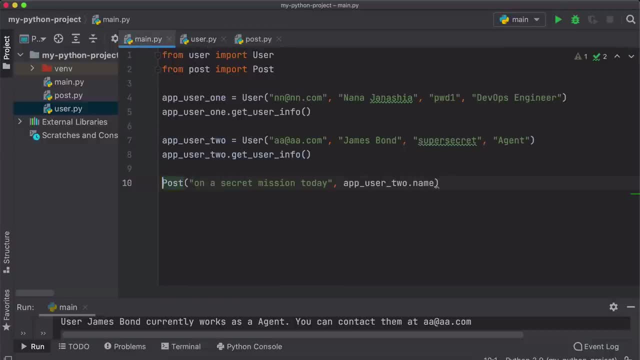 Special Instance of that post class, And then we can print the information of that post first, assign it To a variable- Let's say it's a new post- and on a new post We're going to call get post info. Let's actually run this application now and see the results. 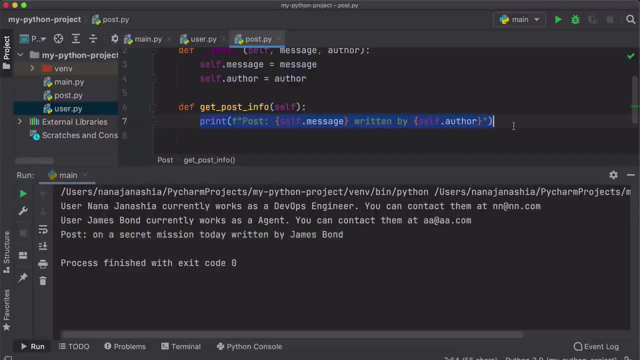 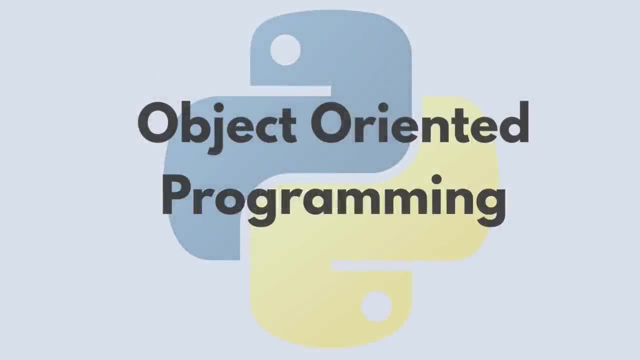 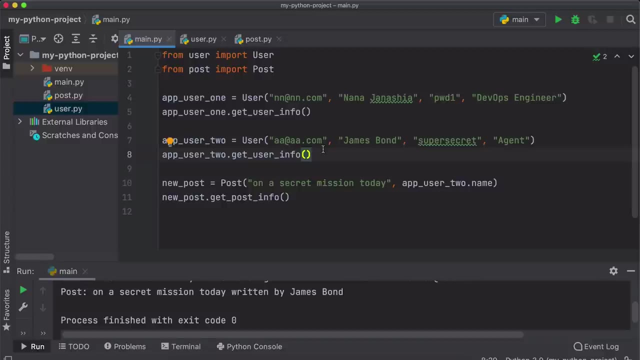 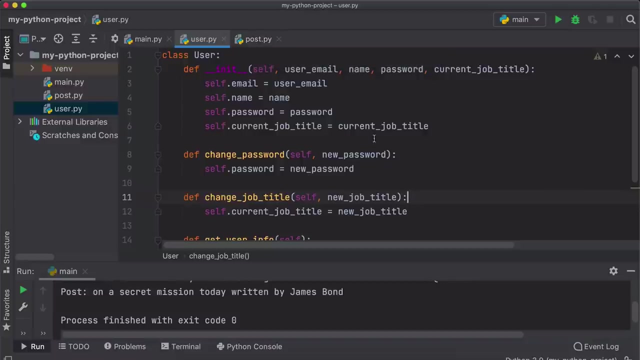 And here we have our post message that gets printed by this get post info method in the post class. And at the beginning I mentioned object oriented programming, which basically means that when you're writing your code with objects and classes like this to create blueprints and then use those blueprints for specific instances. 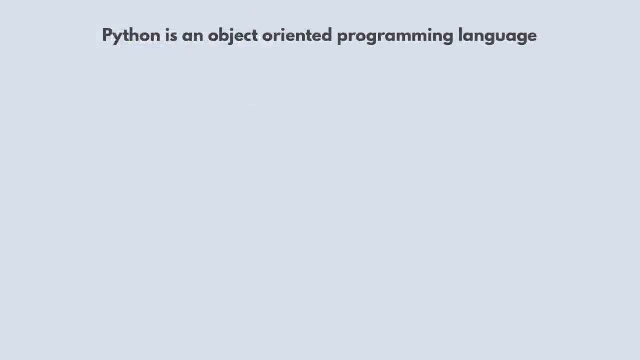 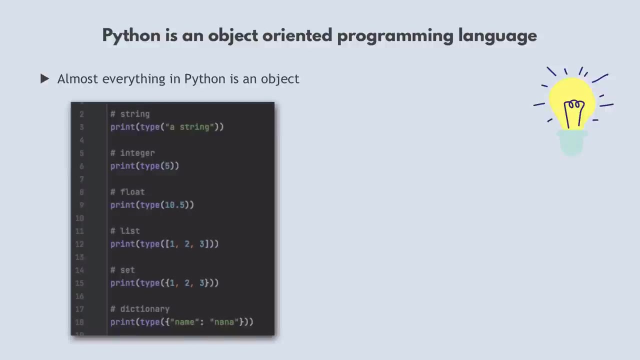 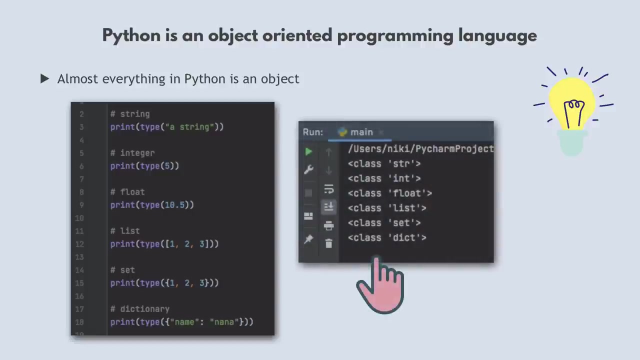 that's called object oriented programming. And also an interesting note here is that in python almost everything is actually an object, For example the data types like string, integer, least set, et cetera. When we printed them out, we saw class of string or class of list. 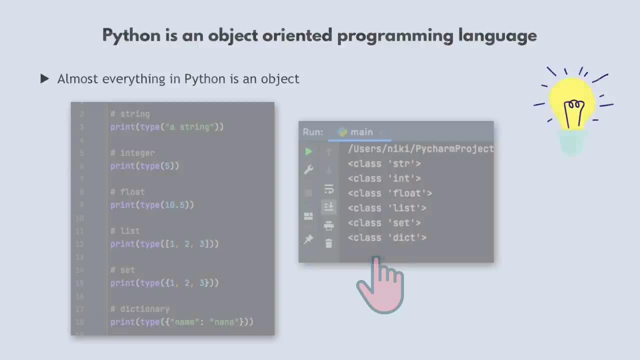 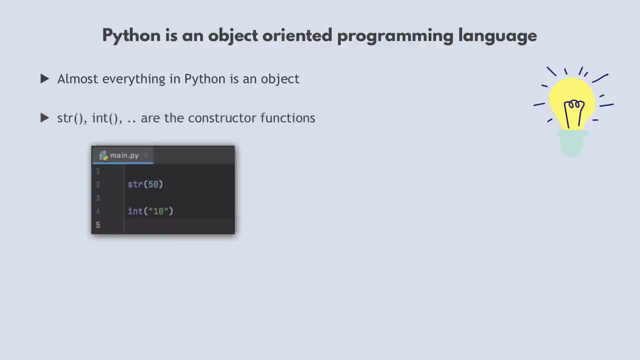 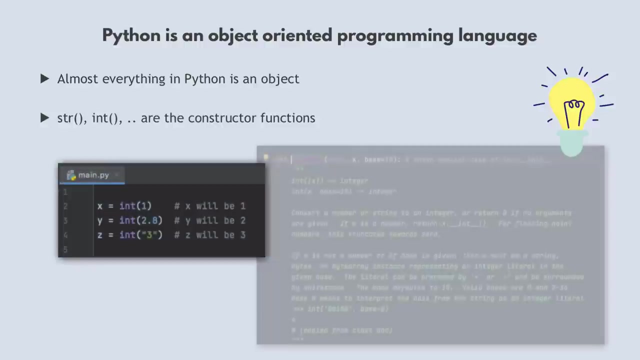 So these data types are also classes in python and these int or SDR for string functions We called were actually the constructor. We called to create a string or integer object and the constructor of int, for example, took a string representation of a number and in 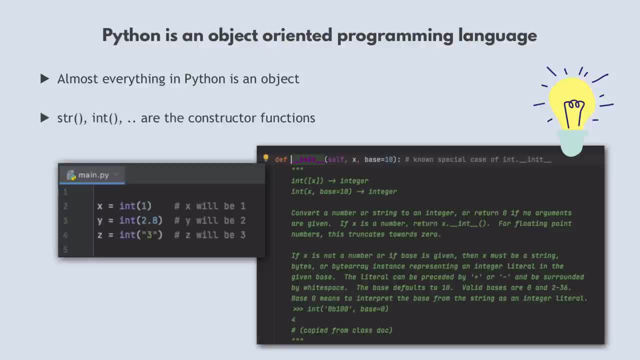 It's in it function and constructed an integer out of it. now for us, in terms of using this, data types and variables, et cetera- It doesn't actually matter, but it's just an interesting thing to know about how this whole thing works in python. 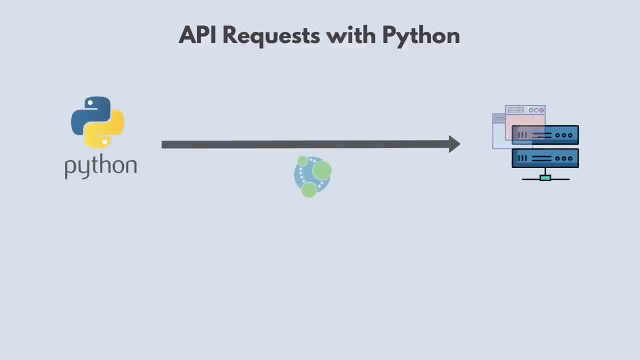 In this part we're going to learn how to use python to talk to external applications. In our case, we're going to use GitLab and an application, and just note here that communication between two applications- in our case our python application and a GitLab application- usually happens using a common protocol like HTTP. 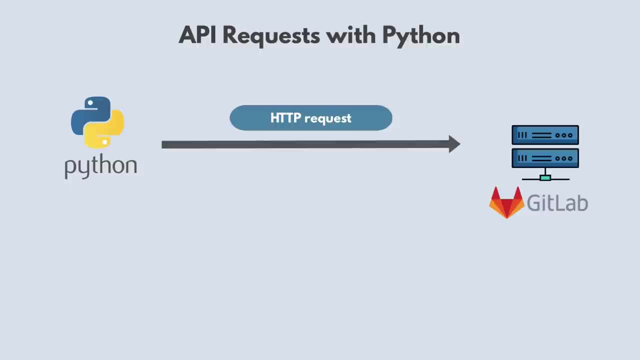 So basically, our python application will send an HTTP request to GitLab application and from the GitLab application it will get an HTTP response for that request. So just know that HTTP is just a protocol that these two applications can communicate with over the internet. 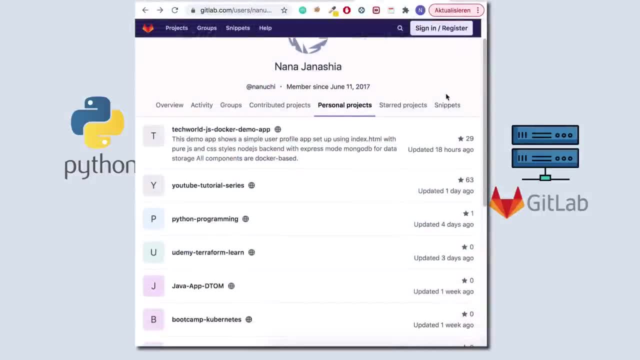 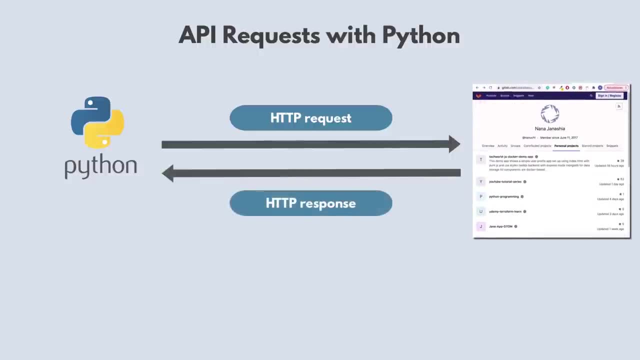 I have a couple of projects on GitLab, so we're going to write a very simple python application that basically goes to GitLab and asks for the list of projects for my user and then just prints it here in our run window, and the concept of one application talking to another is basically done using 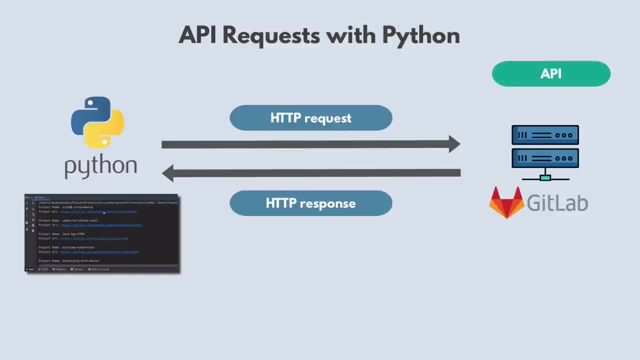 something called API requests, So the remote application, in this case GitLab, has an API. So these are functions, basically, that GitLab makes available for other applications to call, And we're going to call those functions from our python application in order to get the list of projects for my user. 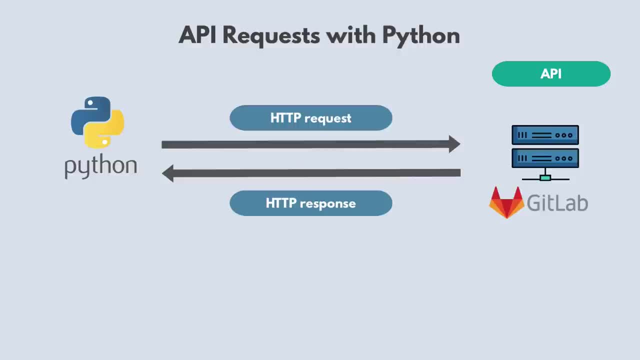 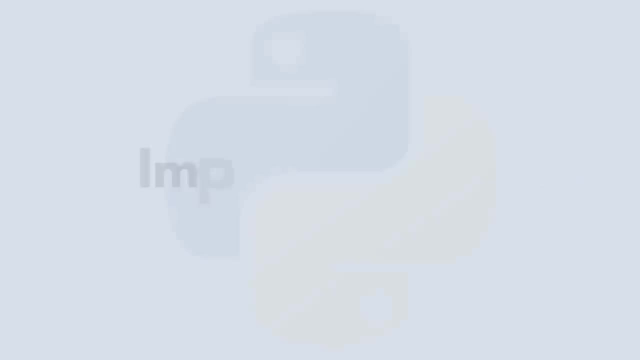 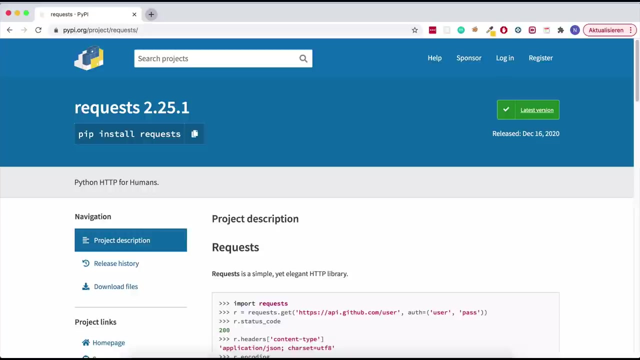 And that communication or python basically asking for this information is going to be an API request or API, And what we get in response from this GitLab API is going to be API response. So let's go ahead and do that In python in order to make those external requests to remote applications. 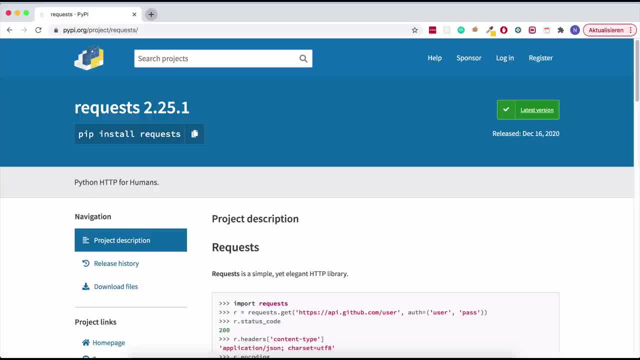 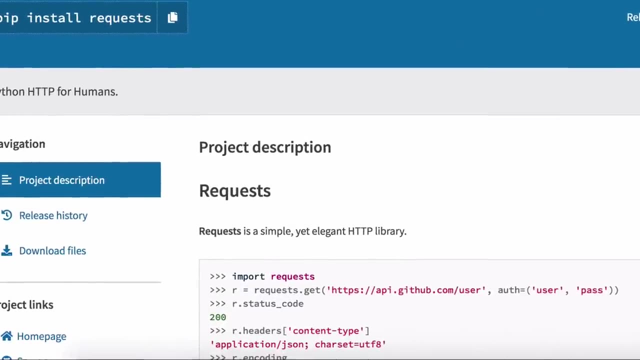 we're going to need a module called requests. This is a generic module that you can use for any external application And, as I mentioned at the beginning, the communication happens Using HTTP protocol between two applications And, as you see here also in the module description, 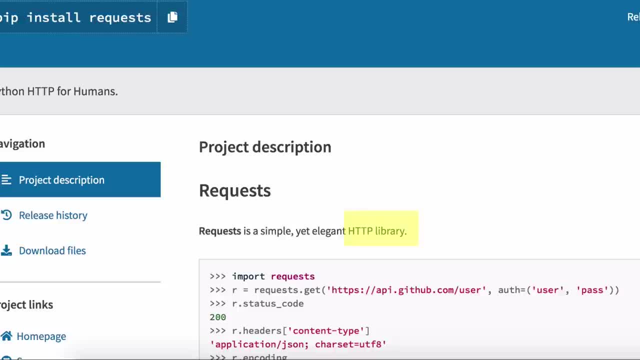 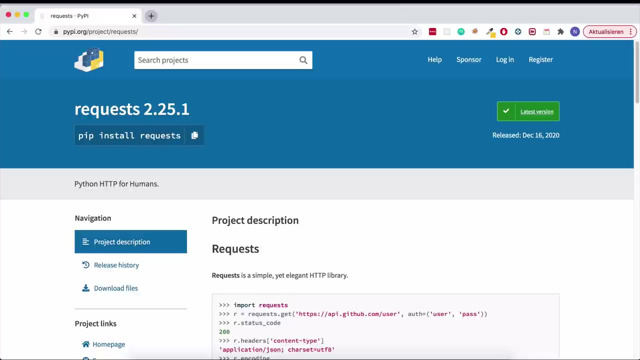 it says an HTTP library which allows you to send HTTP requests and then receive HTTP responses from another application, And that's exactly what we're going to be doing, And this request module is not part of python, So we're going to install it using peep again. 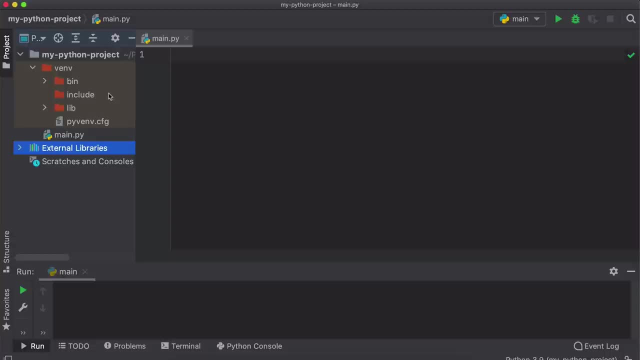 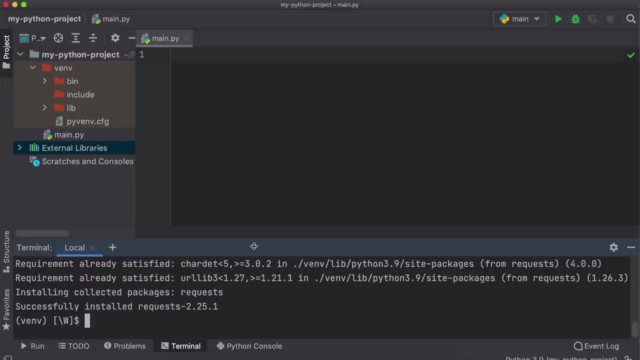 Remember that we're using peep that actually comes packaged With the pie charm. So in the terminal window of my ID of pie charm I'm going to execute peep install requests. Successfully installed request. This is the version of that module. 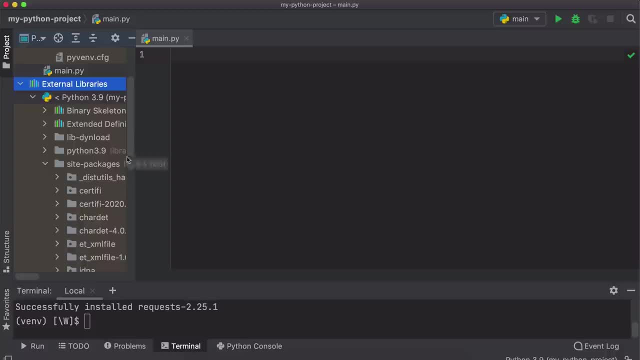 And if I expand this external libraries site packages, I'm going to see the requests package in the list. Great, So once we have the module available locally we can import that module in our file And these requests module now has- or package actually has functions. 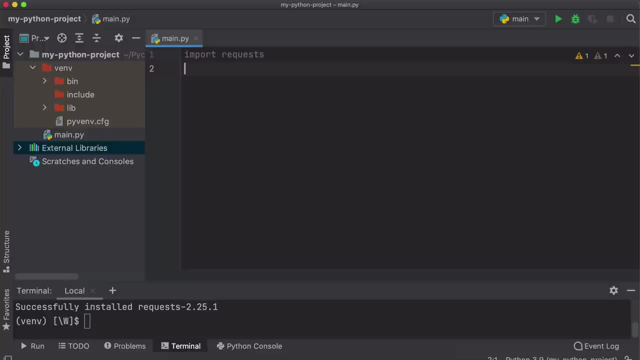 variables and objects that we can use to talk to this: remote applications like GitLab. As I said, GitLab is just one example. You can talk to any remote application that has an API and we can not only do request for getting the the existing information. 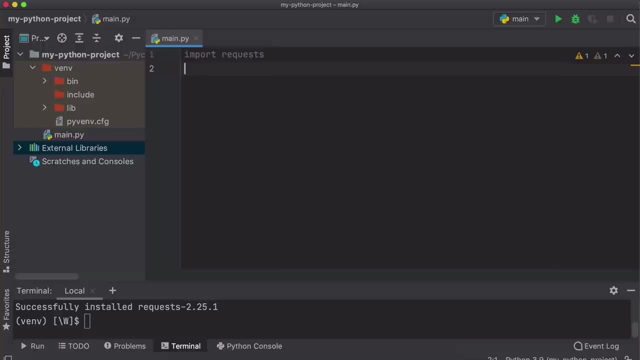 but we can also make requests to change something in that remote application. So, for example, I can write a python application that will actually create a new project on my GitLab account. But to keep the demo simple, we're just going to be fetching information from GitLab. 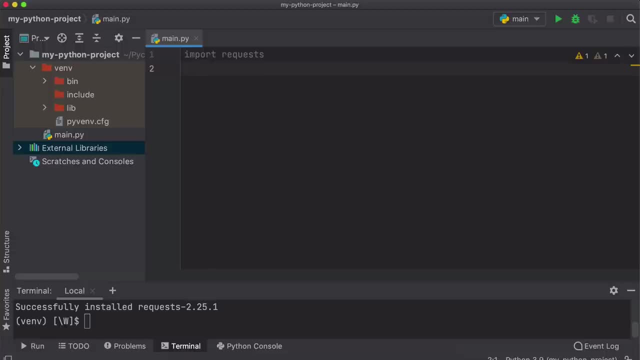 So how do we make request to an API of an application? With this requests module we get a function called get, And get takes one main parameter, which is URL. So basically we need to tell python where to find that remote application, or again. 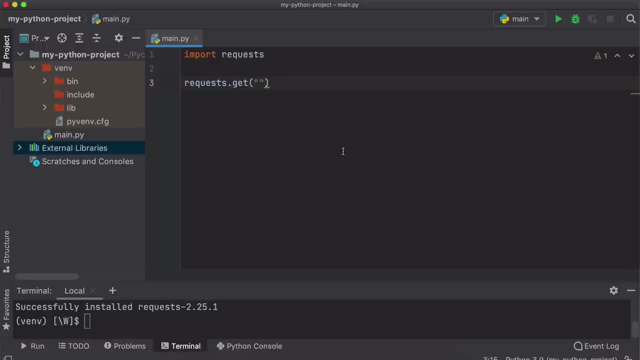 in our case, where to find GitLab to talk to it. So we need the URL of GitLab. And where do you find this URL information of a remote application? You can basically Google that. every application has their own documentation where you can see the URLs. 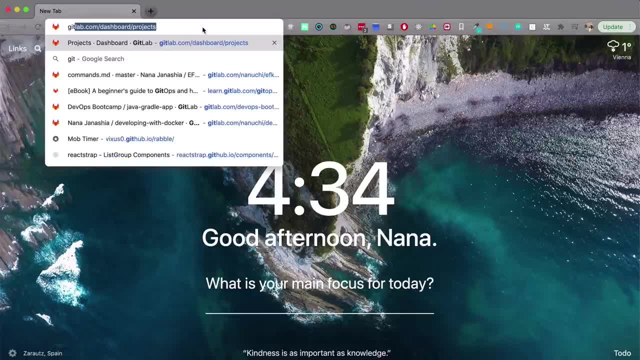 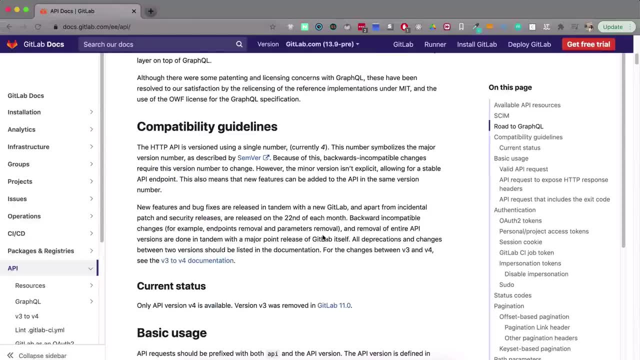 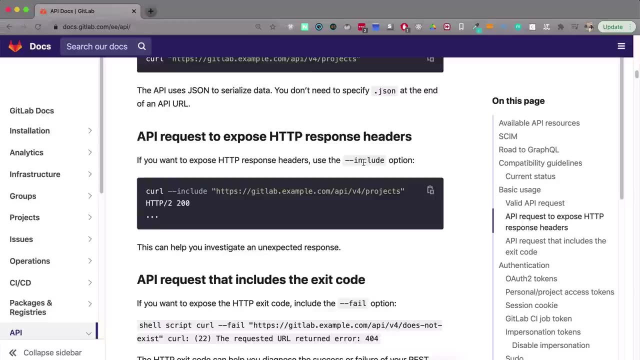 So, for example, for GitLab, I actually Googled it. So if I do GitLab API documentation like this, let's make it bigger. So you have basically description for the API and what type of information you can get from GitLab and also what kind of things you can create in GitLab. 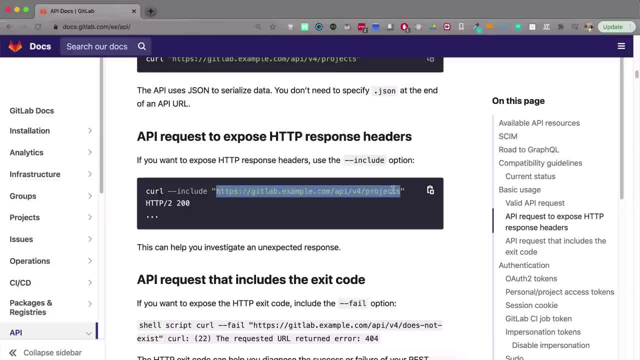 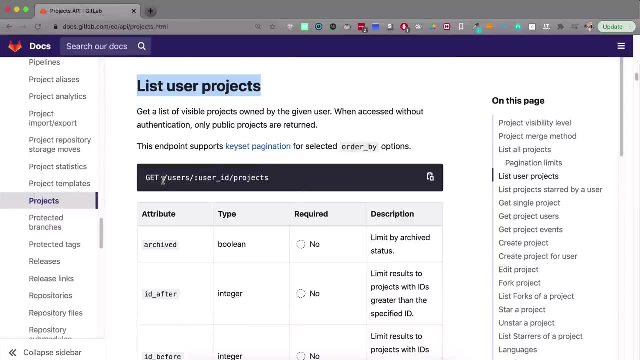 And you see an example API here that basically just lists all the projects. However, we want to list projects of One specific user. In this case, I want to list my own projects And in this documentation I found this list to use, a project section, where I have an example of how to use projects for a specific user. 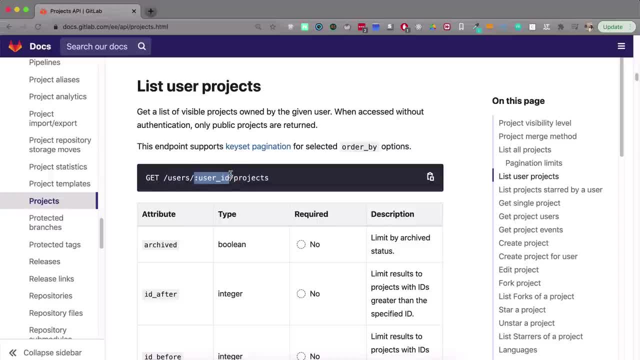 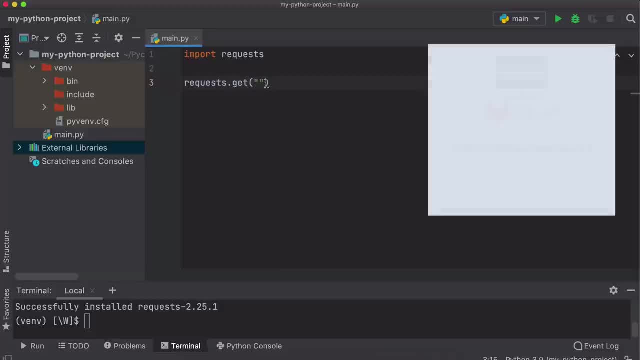 So we have slash users and the user ID. So that's going to be my GitLab user ID and projects. So basically the URL will now look like this: first, We're going to have this base URL, So that's basically HTTPS. 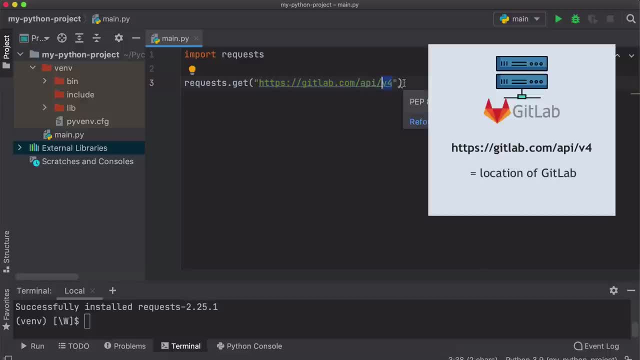 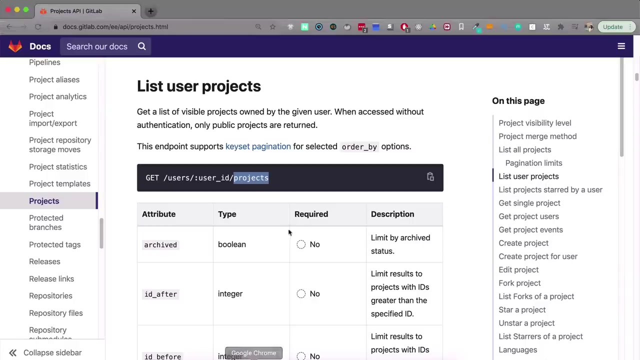 GitLab dot com API. The four and all the things that we want to do is going to be at this base API And after that we can, basically, depending on what exactly we want to do, we can choose one specific action And again, 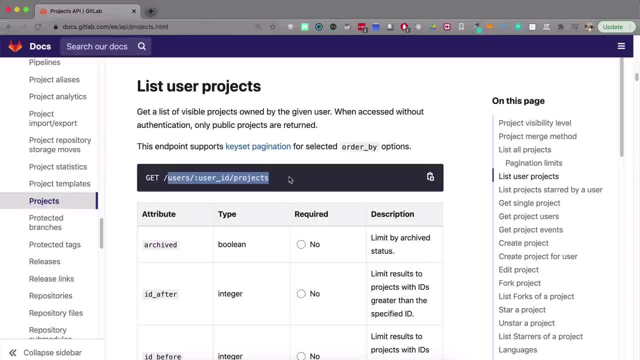 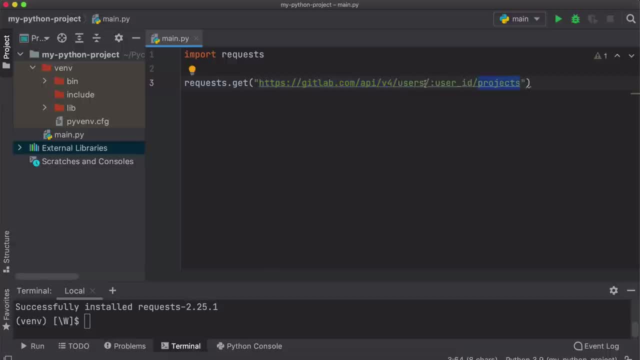 going back, this is the action we want to execute on this base URL. So from GitLab we want projects that belong to user, and right here I'm going to my own GitLab user ID. So if you have a GitLab account, 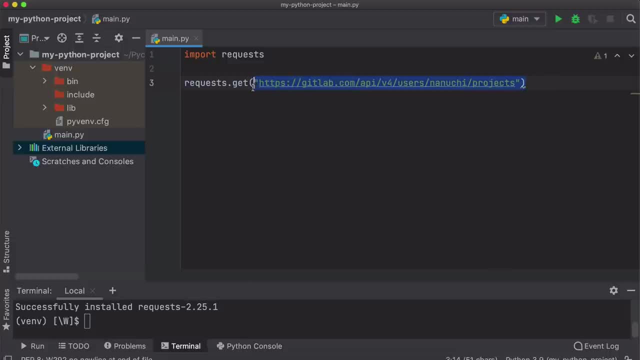 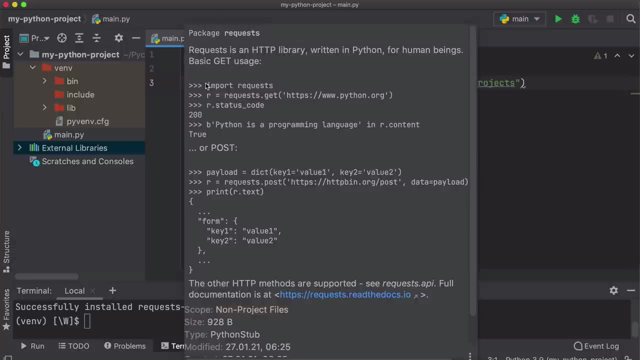 you should get your own user ID here And that's going to be an API URL for user projects And this will actually give us some kind of response. So request dot get will make that request to GitLab and it will return some kind of response. 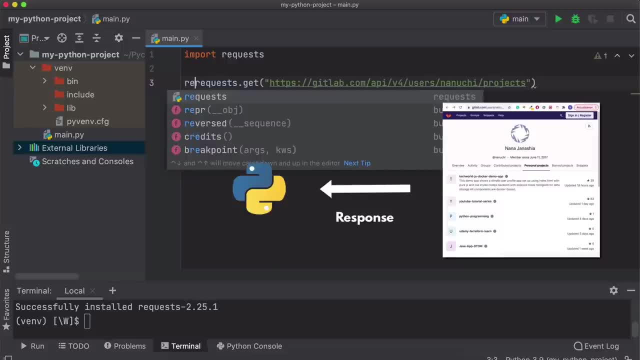 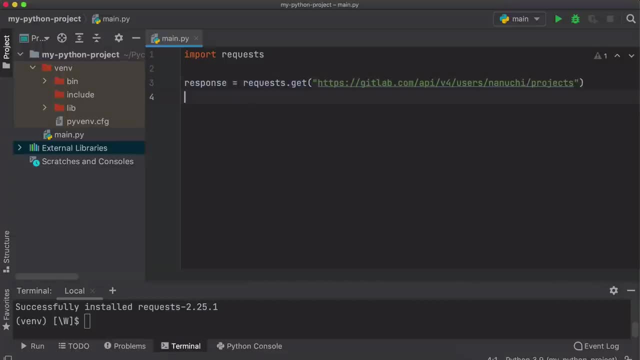 And we can save that response into a variable. So let's call this variable response, because that's what it is, And on the next line let's actually print and see what's in that response. Let's run our application And right here, 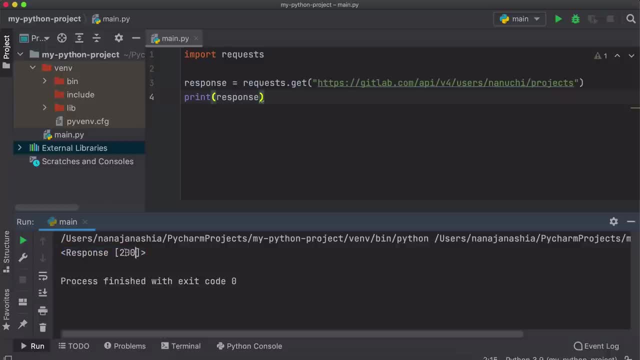 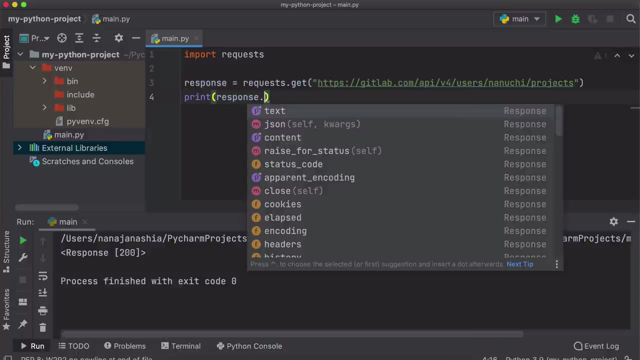 you see, we have an object response with a code here. Two hundred is a code for a successful request, but we're not seeing the actual contents right. We want to see the projects with their details and in order to get that, we're going to do dot and text and let's actually execute this now. 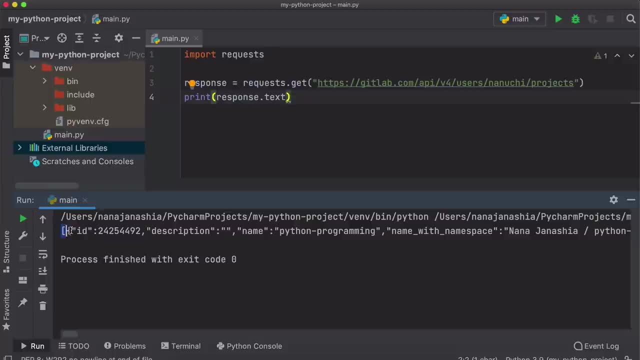 And now you see these square brackets, which means it is a list, because we have a list of projects and this whole bunch of information about projects there, And you also see curly braces. So this is a list of dictionaries and each dictionary holds information of one specific project. 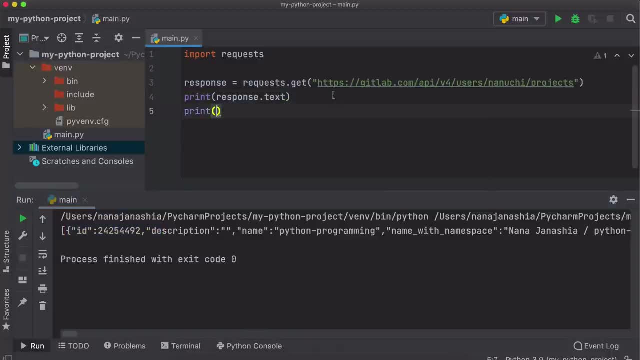 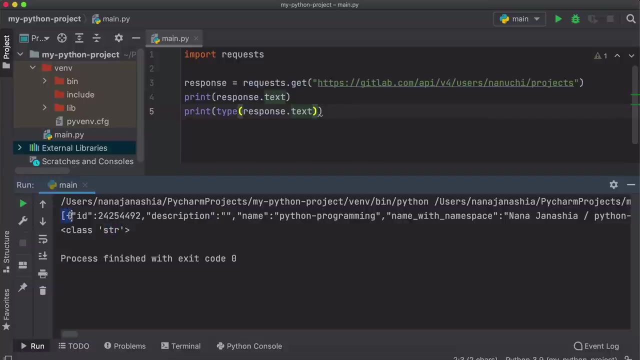 Now, if I actually print the type of that response text Like this, you see that it is a string. So, even though we see the format is actually a list of dictionaries, we're getting a string because we're accessing text attribute. Now, 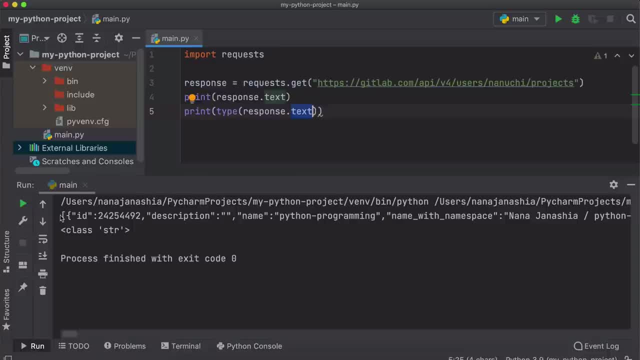 there is actually another attribute which will give us the same, But as an actual list of dictionaries instead of string, and this will be actually a better way to get that information, because then we can work on it, so we can look through it and get the individual elements and access the values. 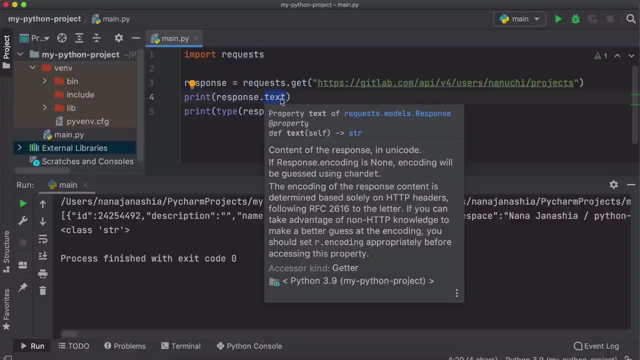 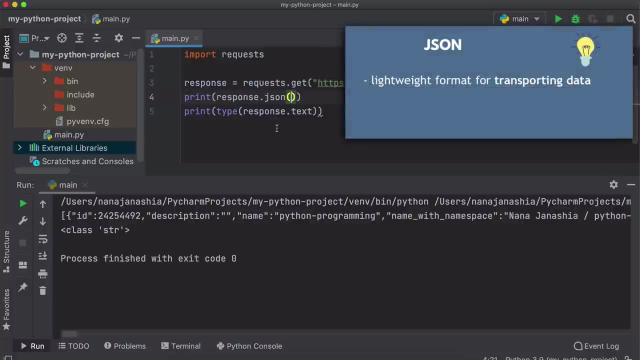 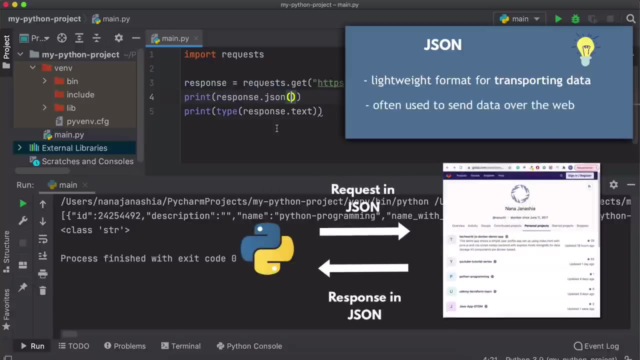 So what I'm going to do now, instead of dot text, I'm going to use Jason. Jason is a standard format that all programming languages understand and usually, when two applications communicate with each other which are written in different languages and with different technologies, with Jason, 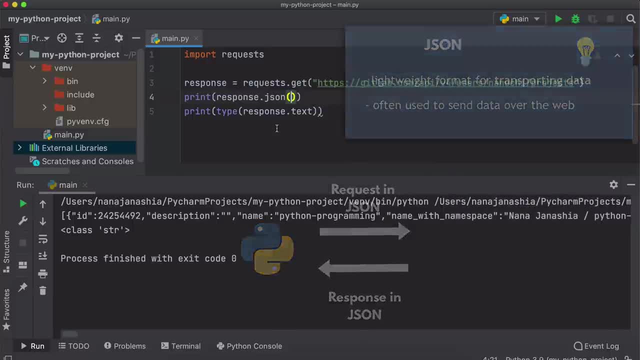 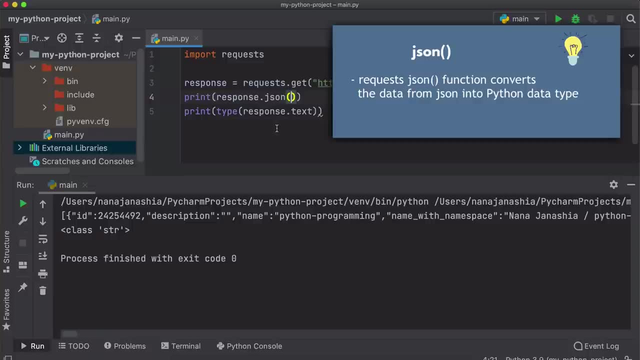 they have a common format for communication and this requests module basically gives us these Jason function to read the Jason format that GitLab sent us. So Jason function will read the Jason response from GitLab and turn it into one of the Python data types. So I'm going to execute this now and 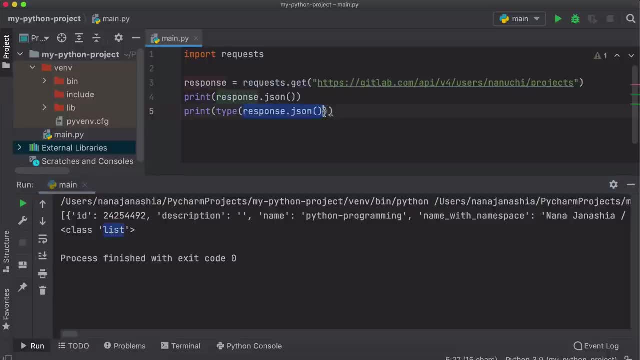 now you see that response to Jason actually gave us list data type instead of string. So again for demonstration, Since this is a list, I'm going to access the first element of that list and print that out. And right here you see, that is actually the first element. 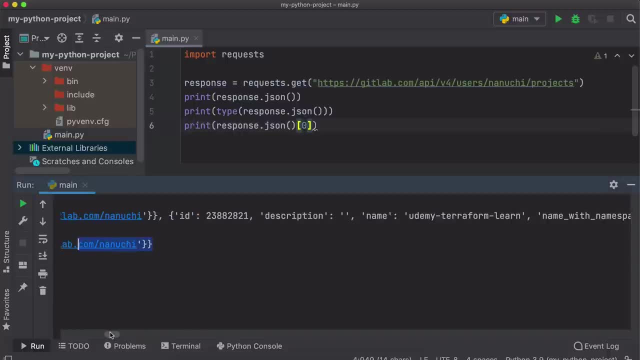 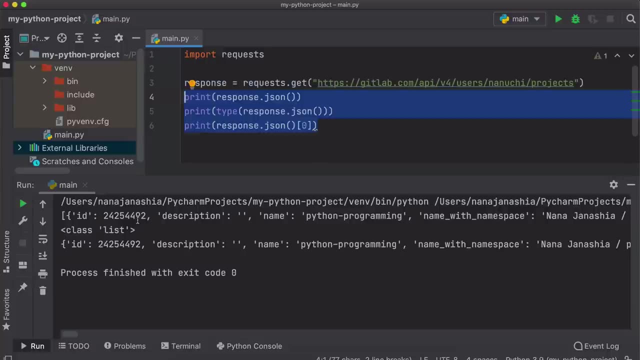 Just the first one from the list, and that element is a dictionary, as you see. So all of this just to give you an idea of what we're getting back from that GitLab API and what we can do with that response or how we can actually work with that response. 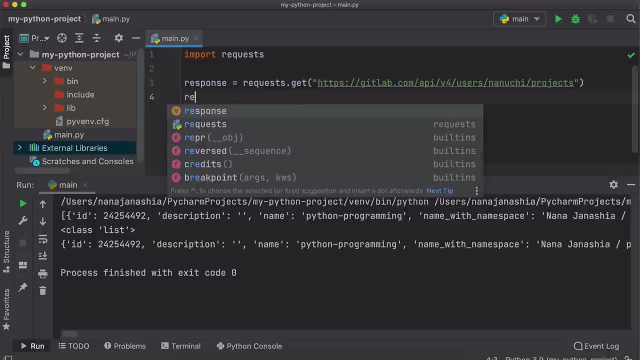 So I'm going to clean all this up, and we saw that response. Jason gives us exactly what we want and that is list of my project. So let's call this Variable my projects. And now what I want to do with this is I want to print out in our window for each project, project name and project URL. 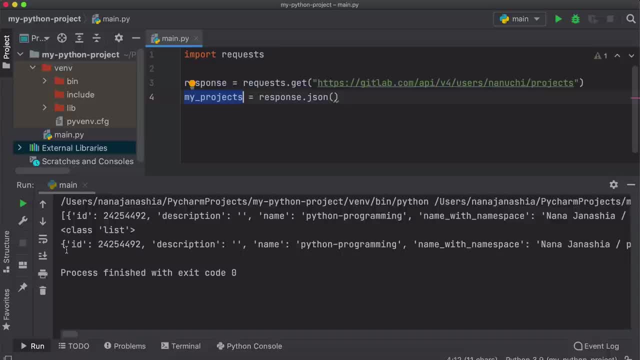 So basically the repository URL for that project. So I don't want to have any other values like ID or description or whatever other stuff I have in this dictionary. I just want name and Project URL for every single project and I want that information printed out in this window. 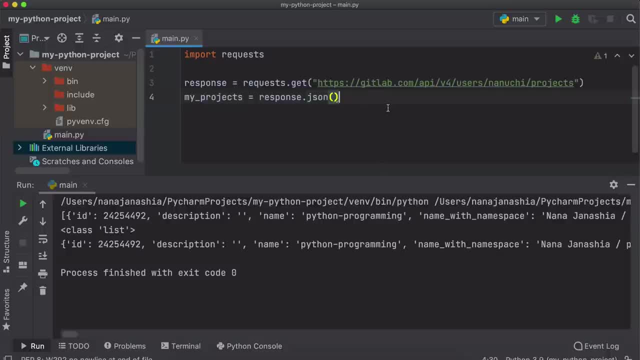 So how do we do that? We have a list, so we're going to loop through that list to access each element inside that list. So you remember, we have for loop, to loop through or iterate through a list and give us access to each element one at a time. 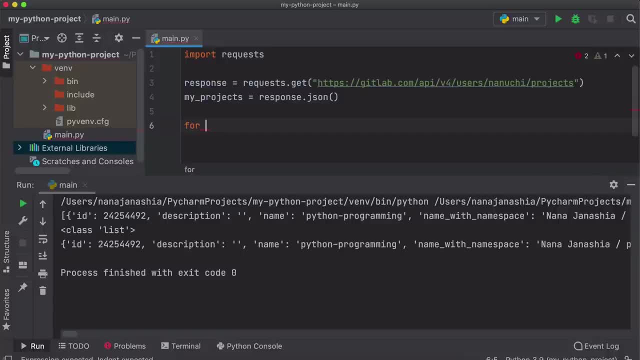 So here I'm going to write For loop, And if you remember the syntax of for loop, we have four and then a variable which will represent a single element in that list, And in this case it's going to be a project. 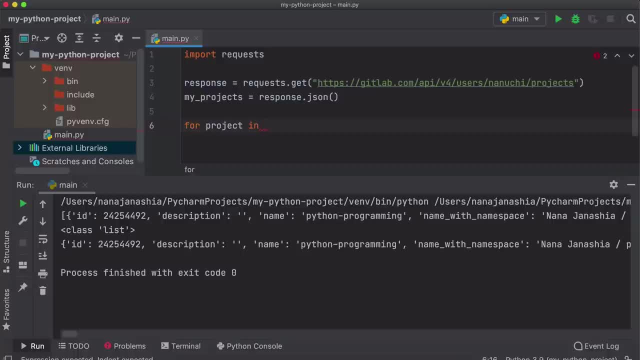 single project And then we have in List: So for project in my projects, Do something. So for every project element in this my projects list, we want to print out the name and the URL. So Right Here I will do print. 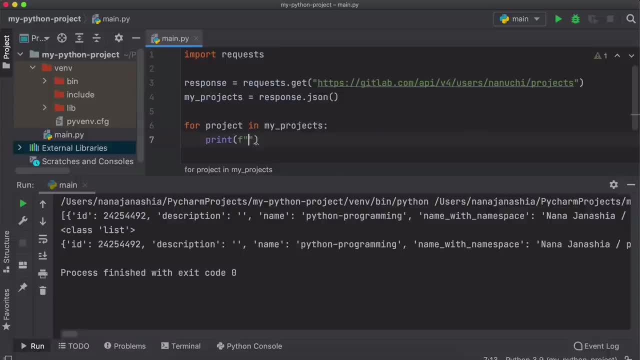 And let's do our formatted string here and let's start writing our message. Let's do project name And the project name will be this one right here. Now, how do we actually access the name of the project in each project element, As you see here? 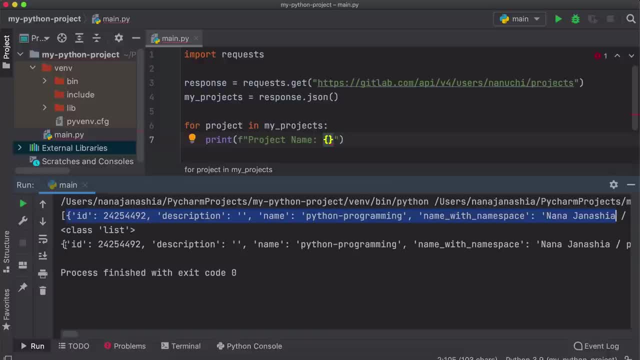 these project elements are actually dictionaries. And how do we access a value in a dictionary using the name of the dictionary, In this case our variable project. So this whole thing is going to be saved into a variable called project And then on the variable on the dictionary. 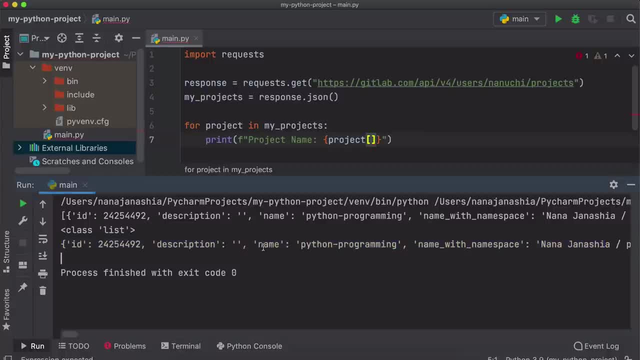 we're going to pass in the name of the key, which is me Now. I've been using double quotes throughout our project and for syntax, for dictionaries as well, like this Right. However, here we have a small problem, which is we have double quotes inside the double quotes. 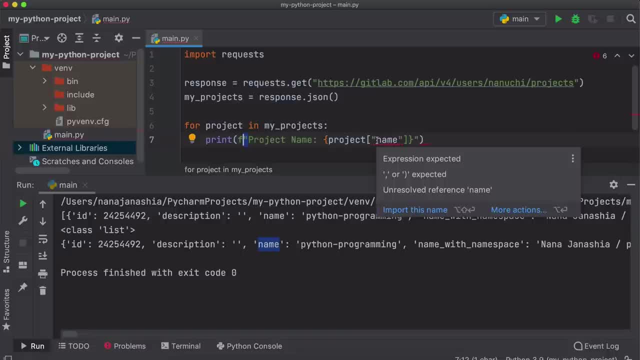 But, as you remember, for string representation we can actually use single quotes as well as double quotes, And this is one of the really important use cases for why we can actually use both single and double quotes for a string, And that is if we have a string inside another string. 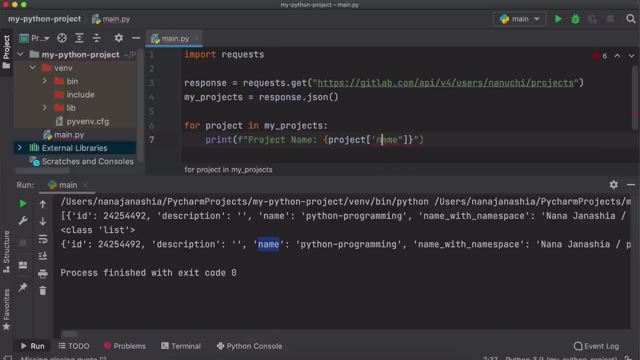 like: right here we can actually use that interchangeably so that we don't have this problem here. So now, as you see, back to normal. everything works, because now Python knows. OK, this is another string which we're using inside this string. 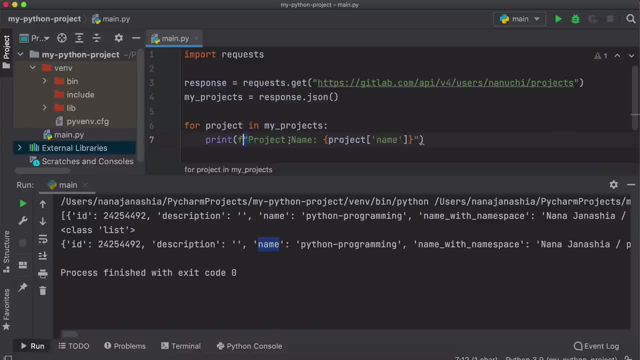 So we can use this interchangeably as we want. So this could be single quotes and this could be double quotes- wouldn't really matter, But that's a really good use case why we need both types of quotes. So we have the project name. 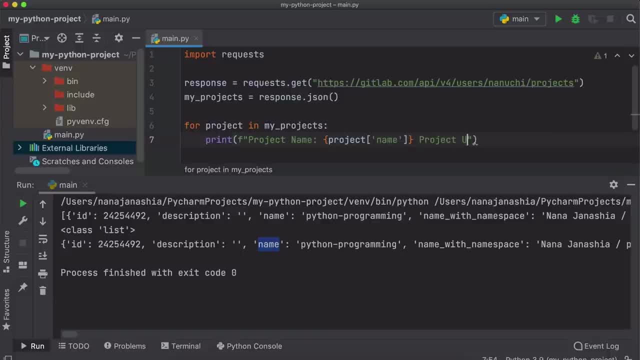 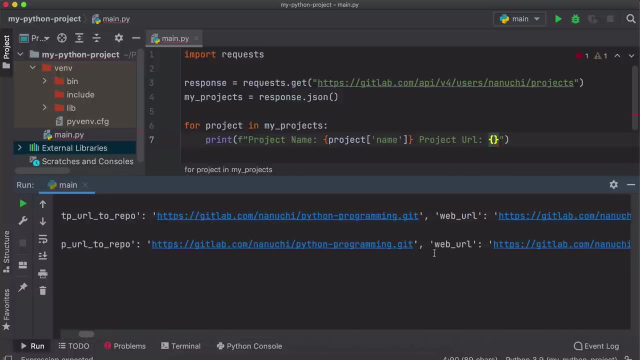 Now we need a project URL, And let's see where the project URL is in our dictionary. This is one element, one dictionary, right, So I'm going to scroll it to the left, and we have web URL. This is what we could use, or we could also use HTTP URL to repo. 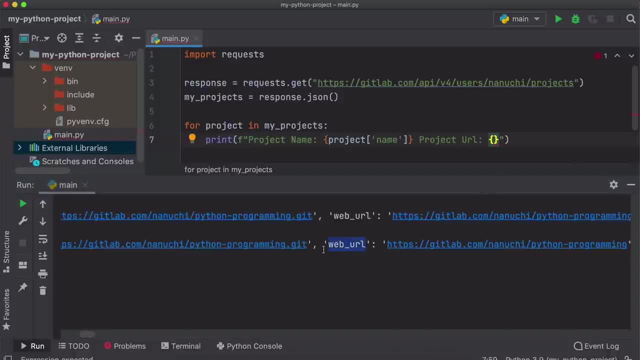 Let's go with the web URL. So again, this is a key inside a dictionary so we can access the value. So this is actually the value we need and we can access that using the dictionary name projects And the key name, which is web URL. 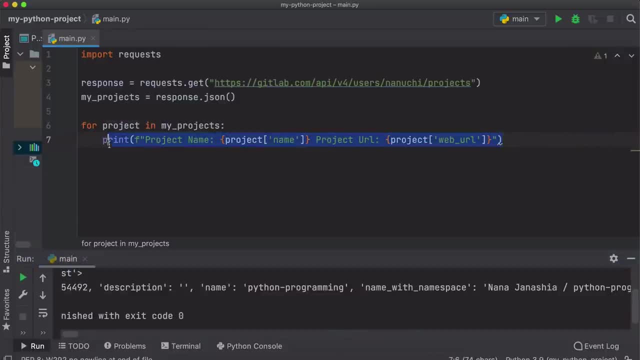 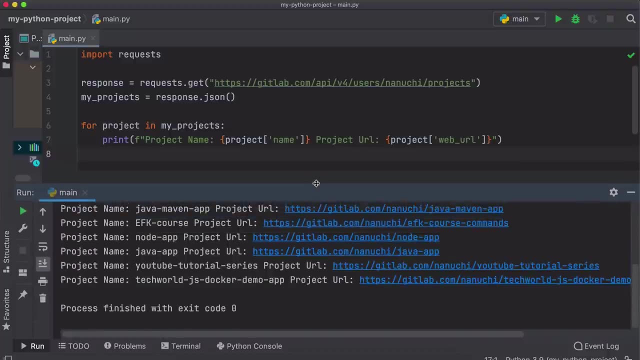 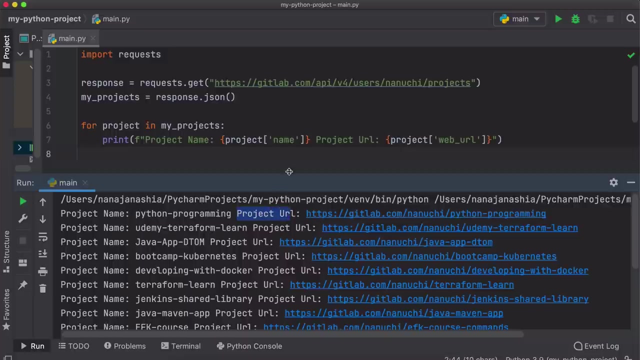 And this is actually project projects, And this code will now print name and URL for each project. So let's actually execute our program And, as you see, we have project name and project URL for each project. We can make the output a little bit cleaner.